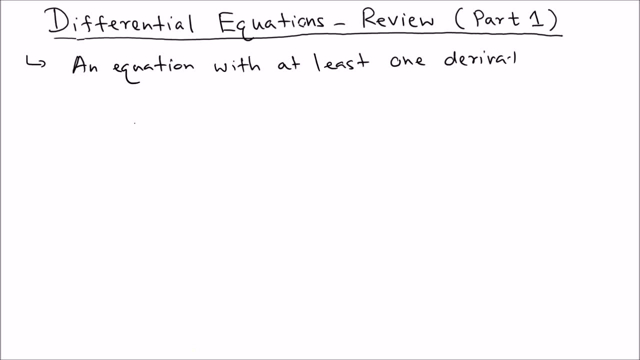 At least one derivative is called a differential equation. It's called a differential equation. It's called a differential equation, For example. so these are two differential equations. So dy over dx. Here x is the independent variable plus y is the differential variable. So this is the differential equation. So 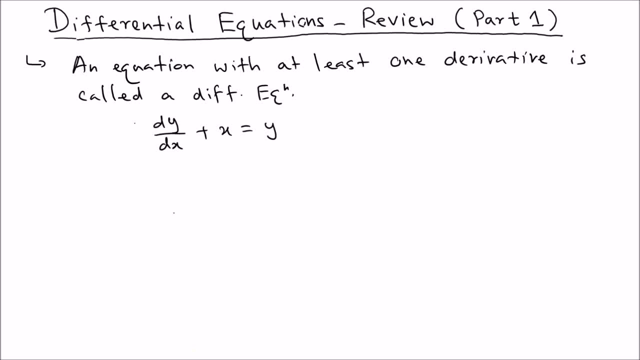 x is the independent variable, plus x equal y. So y is the dependent variable, So x is the independent variable. So that is normally what is in the denominator, And then y is the dependent variable. Y is the dependent variable. 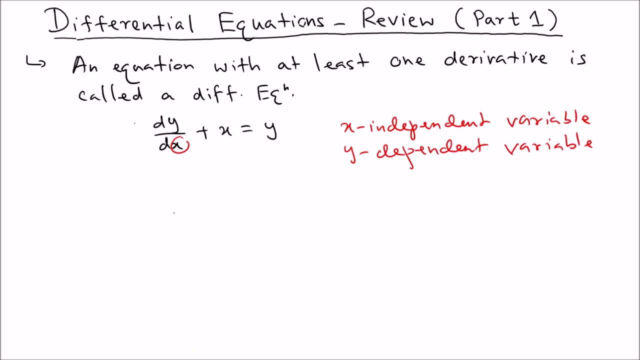 So when you have a ordinary derivative, there is only one independent variable. If there are more than one independent, if there are more than one independent variable, we call it a partial differential equation. We can talk about that later, But that's not the topic of this course. 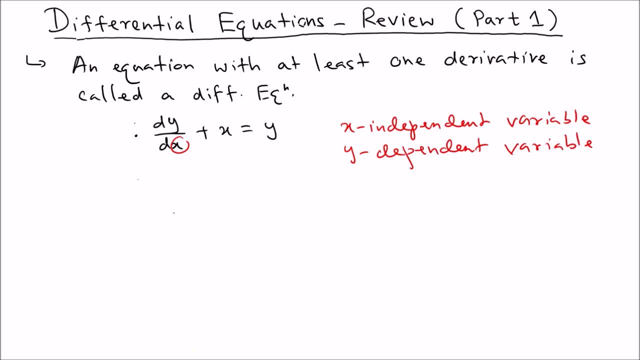 Good. So another example. So for example this one: 3 d squared y over dx squared plus 5.. d y over dx minus y equals 3.. So this is another differential equation, because there are there There's a second derivative and the first derivative. 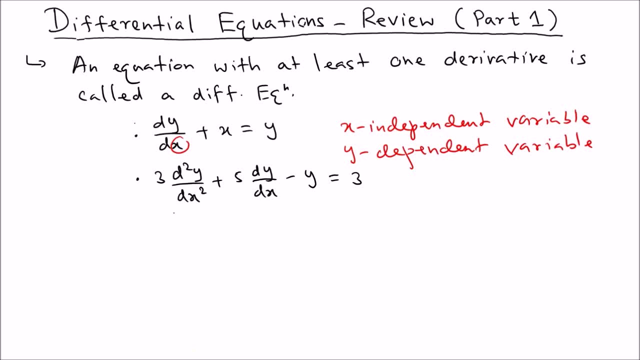 And in this an equation, so it's a differential equation, okay. And then the next thing is what we mean by an initial value problem. So the next one is initial initial value, like this problem. so, in short, we call this: is i v p? 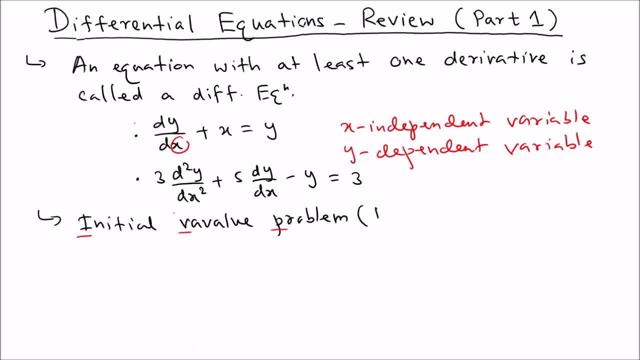 so when you see ivp uh, that means initial uh value problem. so what's the initial problem? initially, problem is a differential equation and initial condition. so initially problem means a differential equation, differential equation plus initial condition. so if you are given these two information and ask you to solve the problem, we call it the. 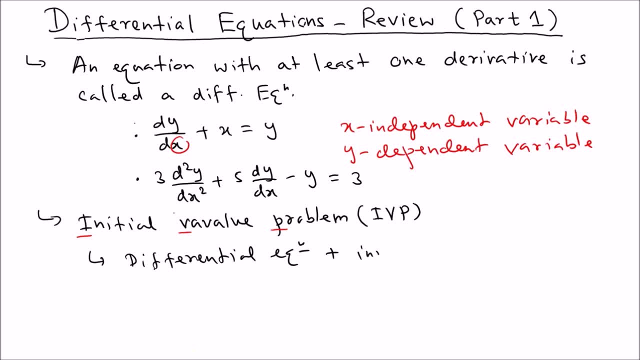 initial value problem. so initial value uh, it can be more than one value uh, depending on the order of the differential equation. if it is first order, one initial condition uh. so let's write that. so if it is first order, we need one uh initial condition, and if it is second order, 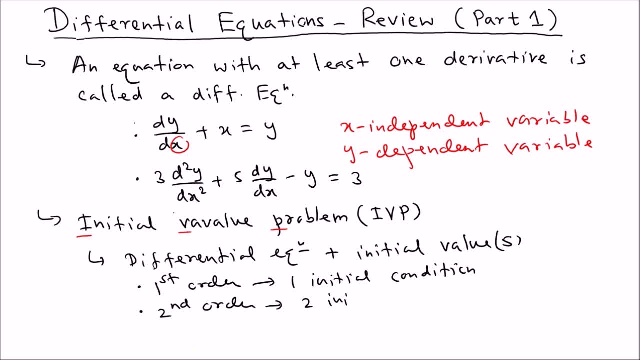 we need two initial conditions. so initial means it given a at the starting point. so for example: uh, let's say there's a system that can start at t equals zero. so if the information given at t equals zero, we call it the initial condition. so normally like it looks like. 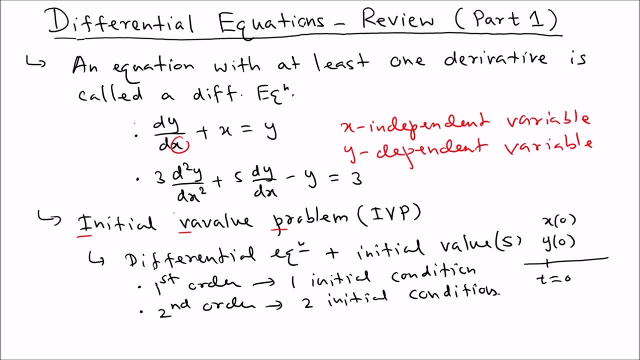 y 0 or x: 0 if x is the dependent variable. uh, and then there's another type of problem, what we call boundary value problem. so what happened? it can give you values not just at the beginning, but some other point, uh, so just write it just for completeness. so what we call boundary 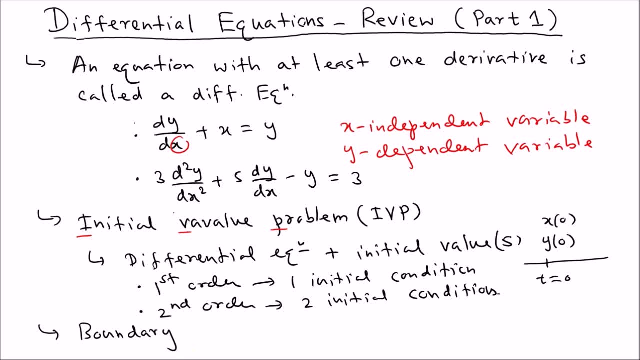 value problem, boundary value a problem, uh, in this course actually we did both uh, so it's called b v p, boundary value problem. so it's a bvp, uh, that means uh. so you can see, not just at 0 but at some other point, like maybe like t equal b or something. 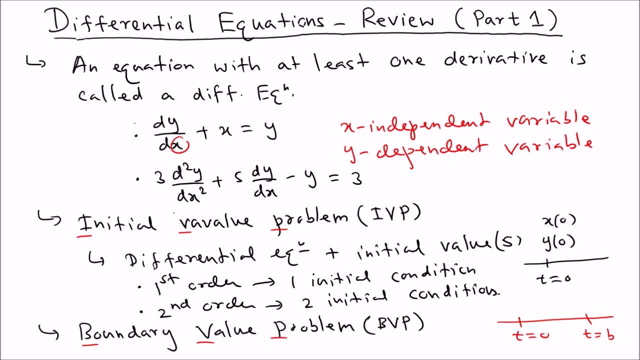 so you can say, for example, a y b equal, something like: why not? so that is what you call a boundary value, brown boundary condition, boundary condition. so initial condition looks like y 0 equal something like a y 1. yeah, that's not probably the right notation, but 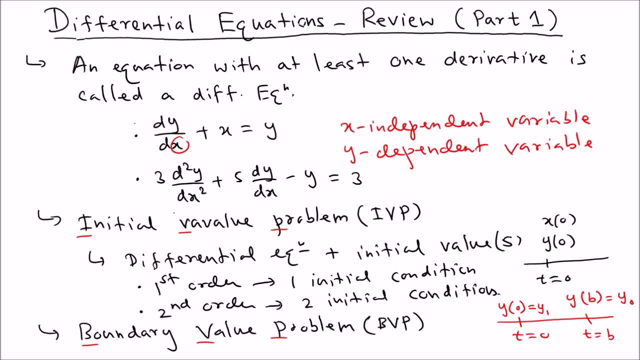 yeah, something like that. so if that is the case, so if you get a boundary value, then you equals a boundary value problem. if you get initial value equals the initial value problem, like that. uh, and then, depending on the degree of the, depending on the degree of the differential equation, 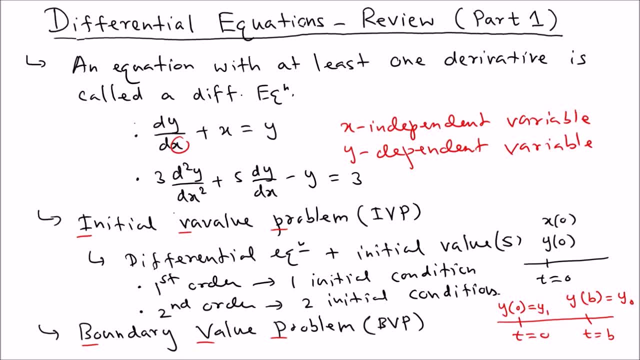 you need to give that many conditions all together. so if it is first order, you need only one condition. if it's second order, you need only one condition. second order: you need, i should say, at least two conditions. but two is like: yeah, two is a minimum. so if the nth order differential. 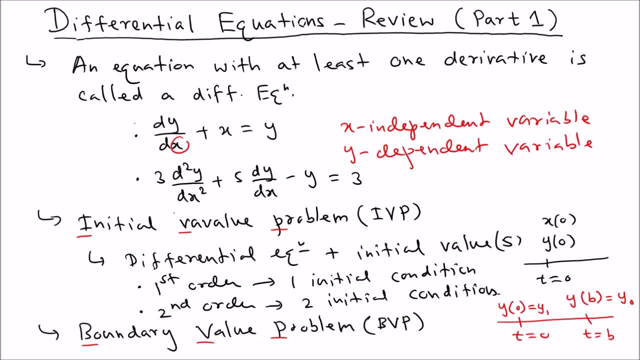 equation you need in many conditions. okay, so that's that's throughout the course. are we gonna use uh that fact? good, now let's uh focus on uh the topics. so we're gonna go one by one and these can reflect the lectures. so in the description you're gonna see: 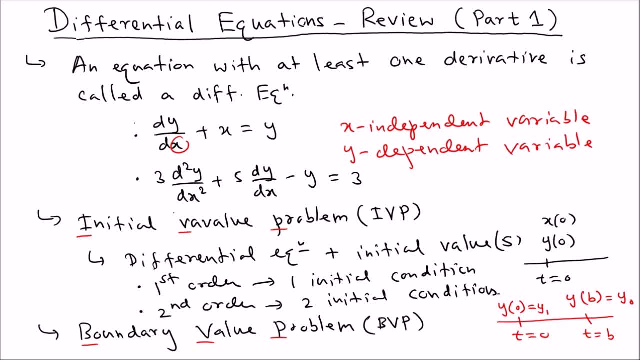 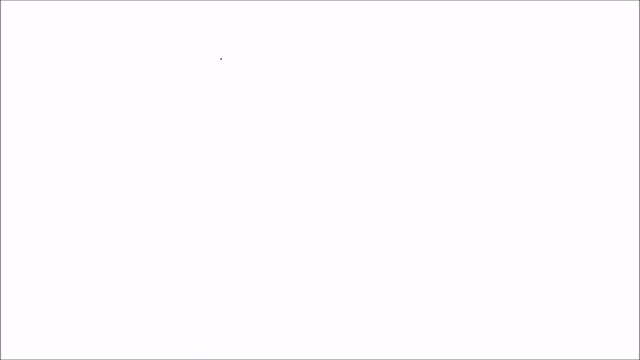 link to the entire lecture, so part by part. so that means if you have some trouble understanding certain topics, you can refer the lecture. okay, so let's start with the first topic. so we're going to go with, uh, what we call the, uh, the first one. what we did was like a verifying solutions. 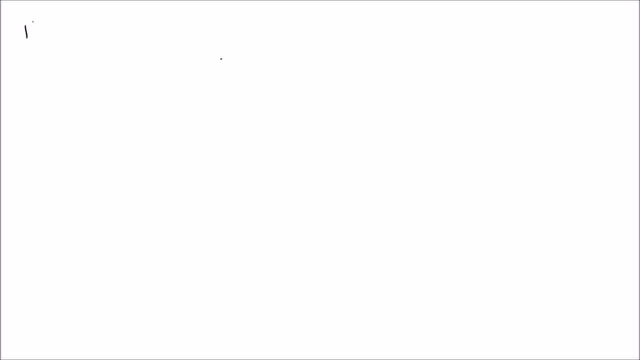 so let's start with that. so the first topic is: we're going to do: uh, verifying solutions. uh, verifying solutions. so what happened here? we are not going to, you are given some expression and you can check whether that is a solution. so that's the idea and we're going to solve the problem later. 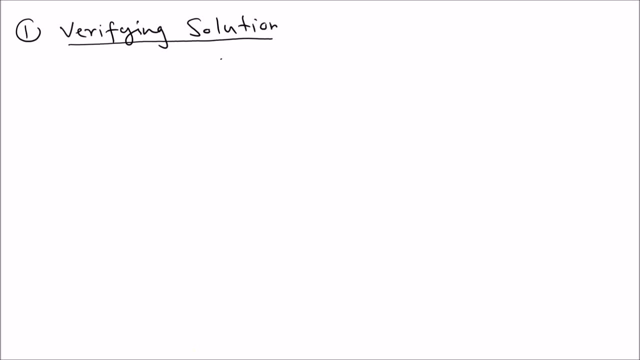 so let's look at a problem like this, so an example like that, so let's say verify, verify that. so remember you, we say we are not say find, we say verify, so the solution is given okay, so it's a different problem, we are not going to find it, we just verify. 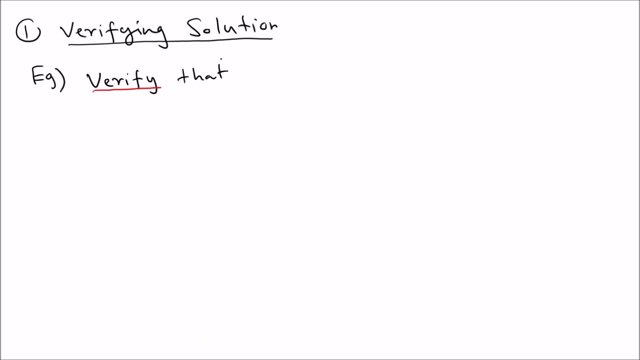 so we need to understand the wording here. verify that x equal c 1 e to the minus 3 t, plus c 2 e to the 2 t. now is a solution. is a solution of x double t prime plus x prime minus 6 x equals 0.. 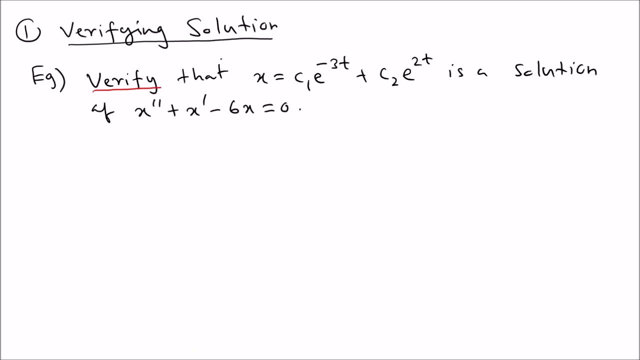 so first verify that that's a solution. so what we normally do is we take the derivatives and plug into the left side and simplify and show that you get 0. that means it satisfies the differential equation. that means that is a solution. so that's so what you did was we verify. we did not find it. 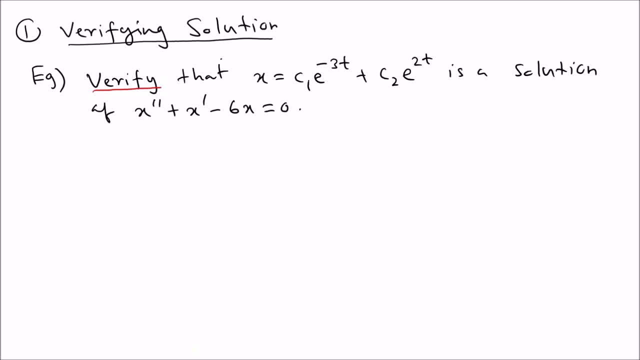 actually we know how to find this one later when you talk about second order constant coefficient differential equation. but that's not the point here. we just verify that that's a solution. okay, because sometimes you can guess. so that's the point, especially when there are very difficult problems. okay, so find. 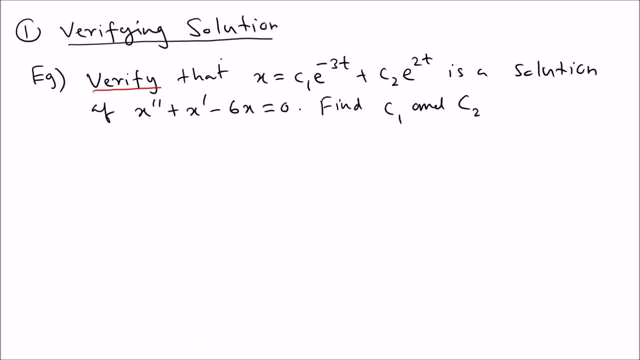 and then we can say find c 1 and c 2, uh, such that. such that normally we put s dot, t dot. but right now- this is the first time, uh, here, so i'm right, such that. but later it's b? s, dot, t dot. okay, such that. 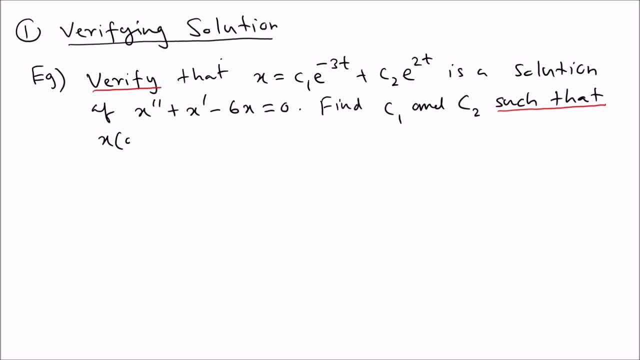 um, such that x 0 equals 0 and x prime 0 equal negative 10.. it can be just some numbers. it doesn't really matter how we do it, but let's see how we can do this, okay. so the answer: ah, let x, t. it's a- i'm going to exaggerate- it's a function of t. 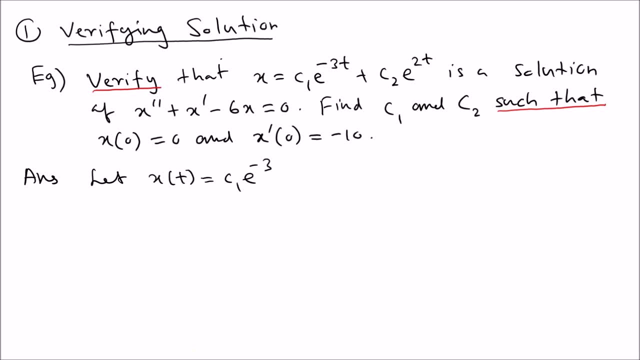 c 1 e to the uh negative 3 t plus c 1 e to the uh negative 3 t plus c 1 e to the 2t. so we're going to use that and then what we can do are taking derivatives. so taking derivatives. 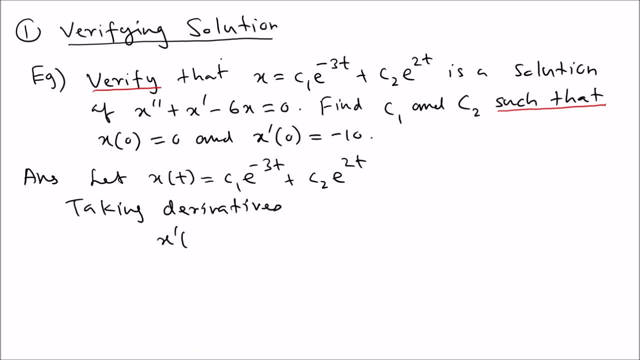 taking derivatives. we have x prime t equal, so we enter the derivative e function. what happened? so let's recall the results are from calc 1. if you take a derivative of an exponential function with the constant here, what's going to happen? the constant come out and nothing happens to the rest of. 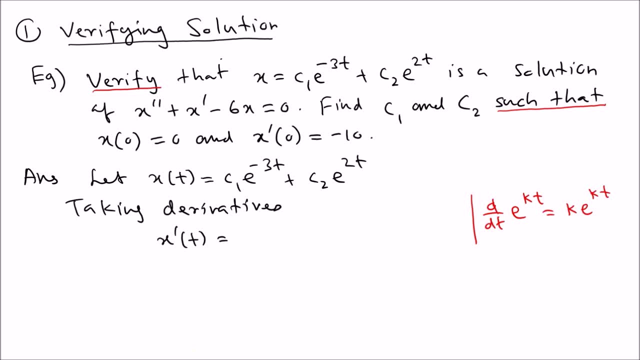 the function. so that's the result. so k, e, k, t. so k has to be a constant, okay. if not, then you have to use the chain rule, okay, so we can use that fact here. so that means the negative 3 c, 1 e to the negative 3 t. 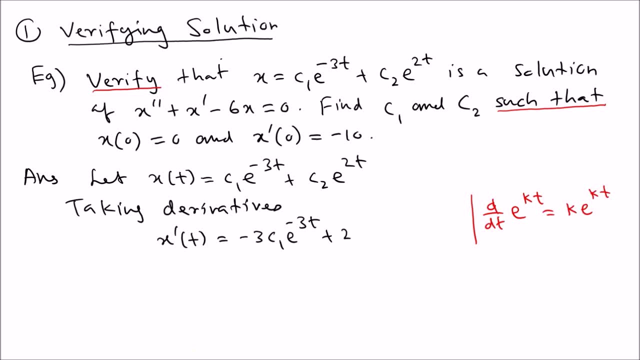 plus the same thing, 2, going to come out. so e to the 2t. uh, we need the second derivative as well. so which for the second derivative? we're going to use the second derivative. so the second derivative is we multiply by another negative 3 that 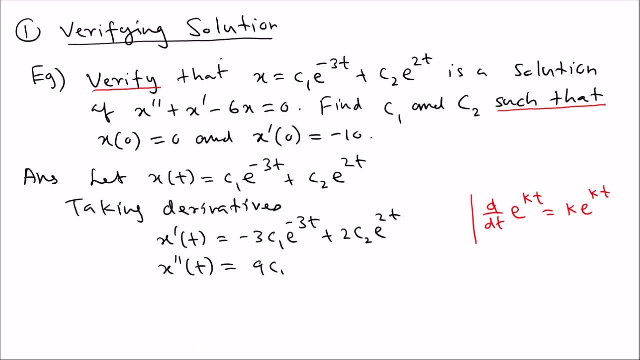 means become 9 c, 1 e to the negative, 3 t- no change. plus this, become 4 c, 2 e to the 4 t. oh see, we can make mistakes very easily, so be careful. this is 2t- no change. good um, so now what we are going to do is we're. 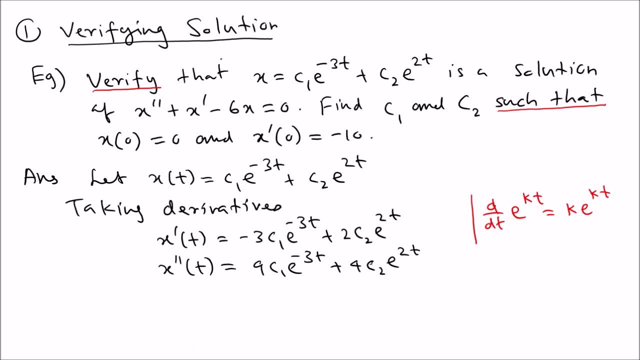 going to substitute. so we simply read this and we are going to substitute it. do this, this in the difference equation, by substituting, by substituting, ah, into the equation. so what we can do, we can start with one side. okay, uh, uh into the equation: x double prime plus x, prime minus 6 x equals 0. 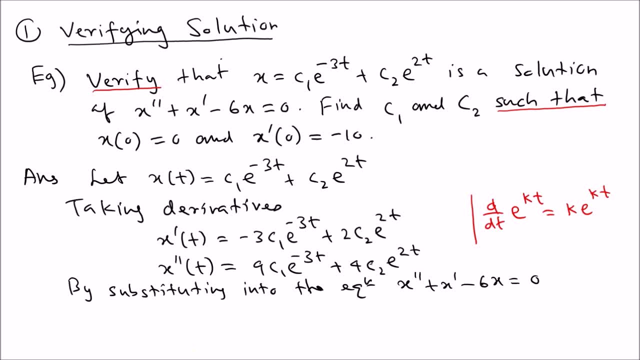 what we're going to do. we can start with the left side and see what's going to happen. so let's start with the left side. so x double prime plus x prime minus six x equal. so let's solve the xp, x double prime, which is 9 c, 1 e to the minus 3 t plus 4. 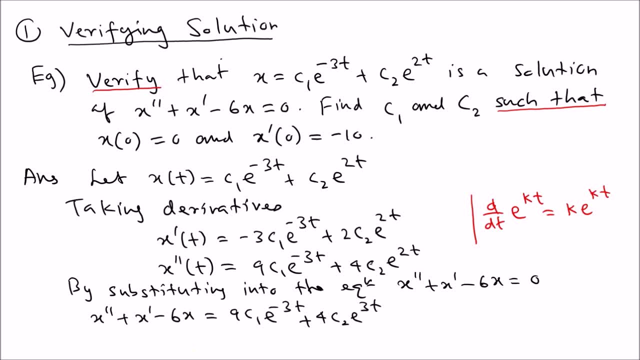 c, 2 e, 3 t, that's x double prime and x prime which is negative: 3 c, 1 e to the minus 3, 3 t plus 2 c, 2 e, 2 t, that's the x prime and then minus 6 x. so that means you have to. 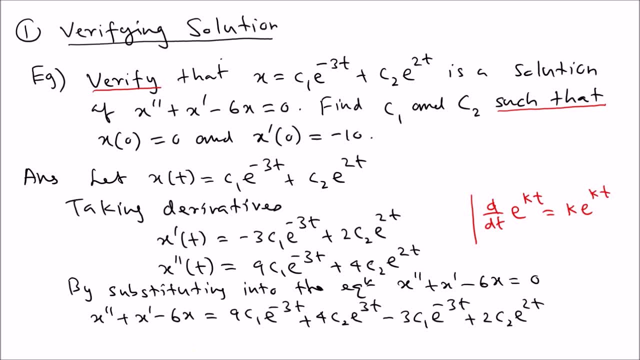 multiply x with the minus sign, so that means a minus. so let's multiply by minus 6, so it's minus 6 c, 1 e to the negative 3 t, and then minus 6 r c, 2 e to the 2 t. now what we can do, we're going to see whether 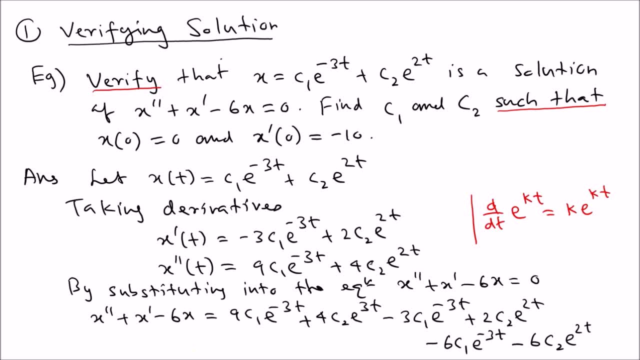 you're going to get c 0, so let's see. so let's go with e to the negative 3 t term. if you look at e to the negative 3 t terms, we have 9 here, we have 9 and we have negative 3 and we have negative 6, and you can see. 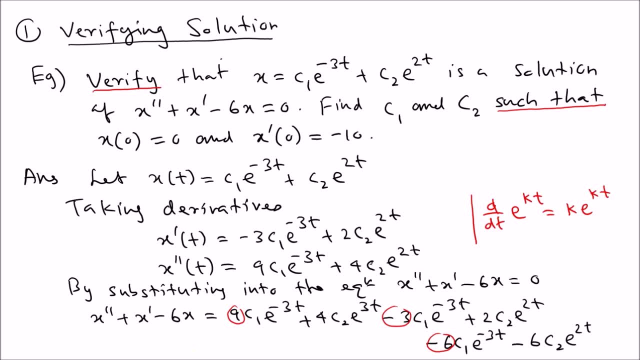 that when you add them, they cancel out. so they all those three- cancel out now. so that's gone, and now i'm going to write this down. actually, that's a small mistake. so this has to be uh two. good, now let's look at the uh 2t terms. so if you look at the 2t terms, 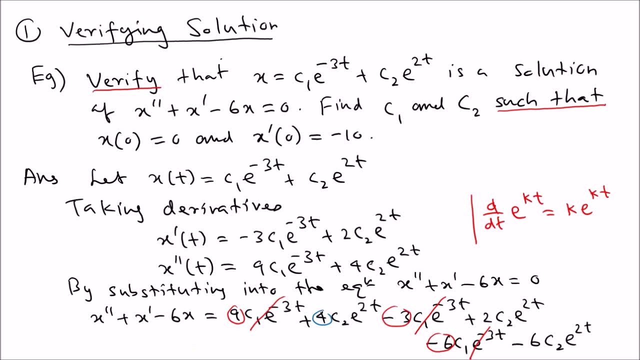 and you can see that we have 4, we have 2 and we have negative 6 and you can see that they all get cancelled out. so that's also cancelled, but i'm going to cancel it in a in the other direction so that you know what you did. so, john, 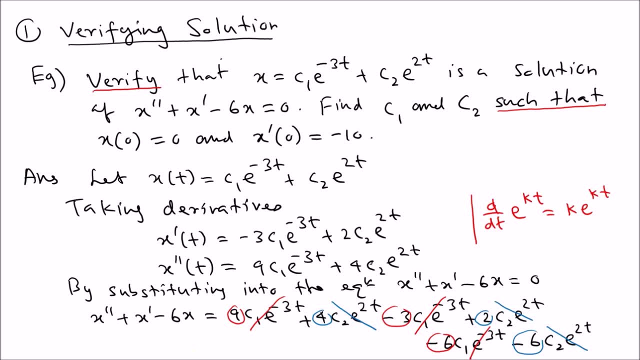 just cancel in the same direction. one, you cancel this positive way. other one cancel the other way, negative, negative, you know with the slam slope. so then you know what you did. uh, so that means they all cancel out. so you will simply get zero. so it simply cancel out and you get zero. that means 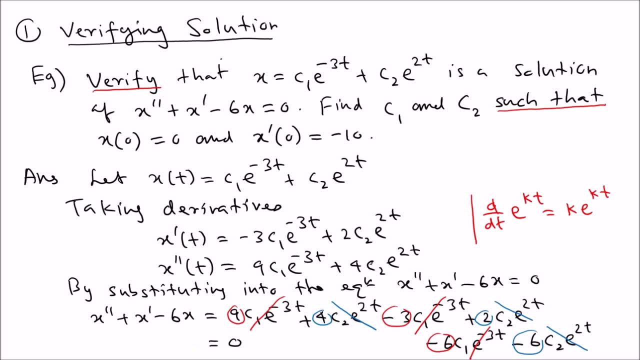 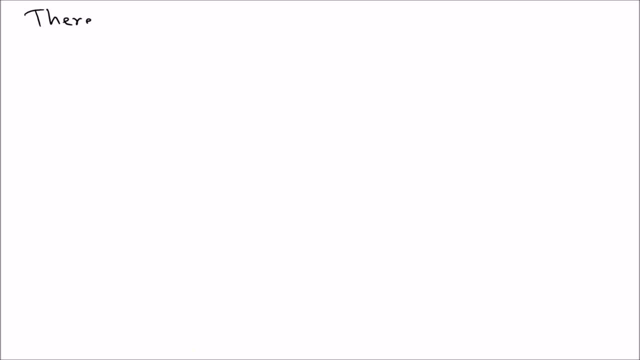 um, your expression is actually a solution of the differential equation, so we can write that. so, therefore, so you can say that, therefore, that's how you're going to complete the argument. so, uh, therefore, it's like we're doing. mathematics means we are making a logical argument, so it's an argument. so, like you, 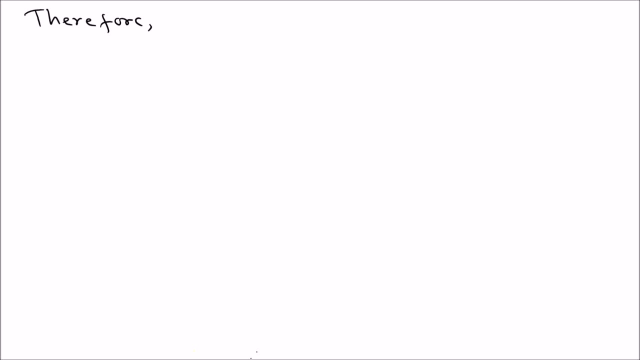 show the reasons and say: conclusion: the reason and the conclusions is like that. so it's a nice argument, okay? um, so let's try to do it like that. it's like much better if you want to do that, right, okay, so therefore, x equal c, 1, e to the minus 3 t. 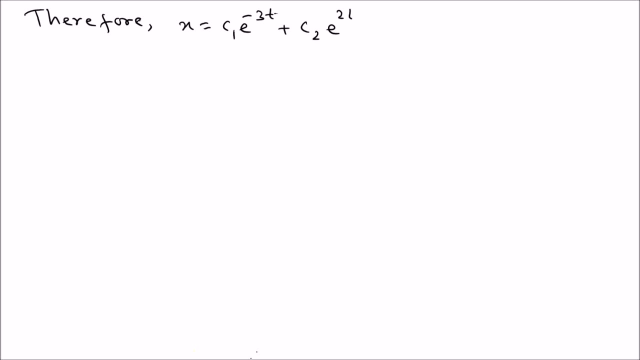 plus c, 2, e, 2, t is a solution, is a solution of the differential equation of x, double prime plus x, prime minus 6 x, equal zero. so we prove that yes, it's a solution. now, what we can do now? we can use the initial conditions to uh find c 1, c 2. 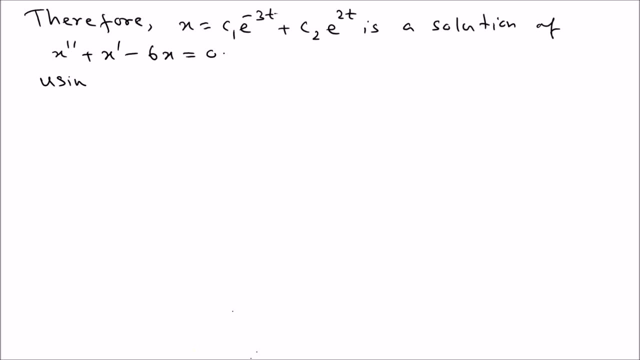 so, using initial conditions. you see initial conditions. using initial conditions. so we have x 0, which is uh, what? what you do is you plug in to the independent variable. you plug in 0, so that means x 0. so wherever you see t, plug in 0. so c 1. 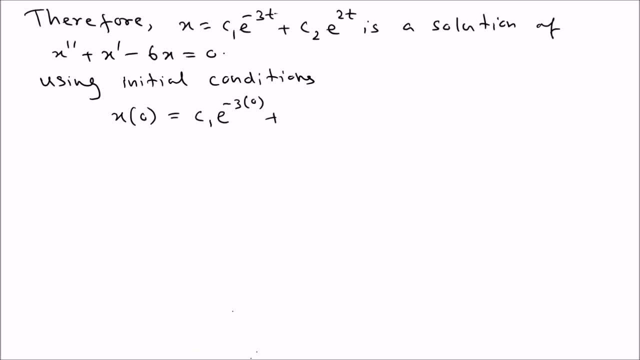 e to the negative: 3, 0 plus c: 2. e to the 2 times 0, so that means we know that e to the 0 is 1, so we know that fact, we know that e to, so we can use that fact. and then that means you simply get c: 1 plus c. 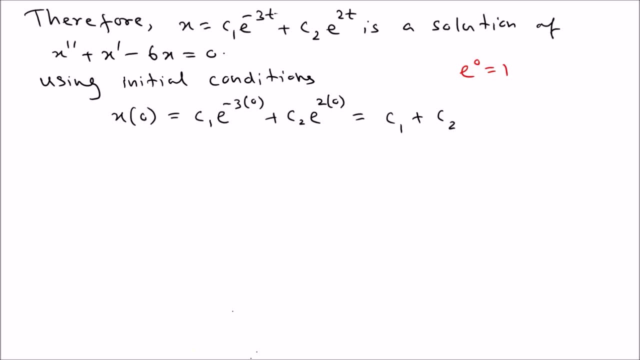 2, but we know that from the condition it is simply 0. it's given that x 0 equal 0, so we we use that condition here. okay, so this is given. this equals 0 is given. now what else we need is we can use derivative condition. so we know that x. 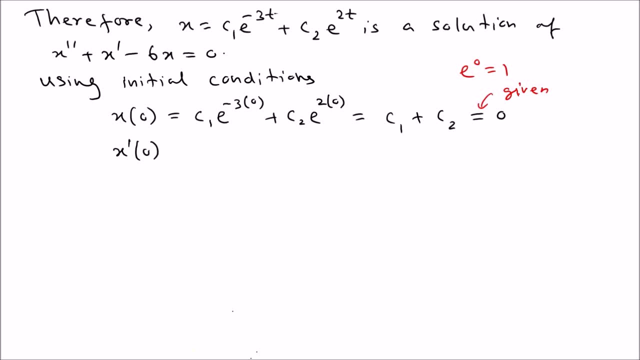 prime 0, which is negative, 3 c 1 e to the negative 3: 0 plus 2 times c 2 e to the 2 0. now again the same argument. so you're going to get negative 3 c 1 plus 2 c 2, but we know that. 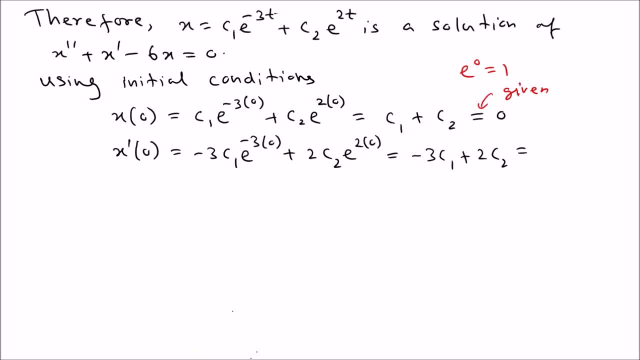 uh is given that this is equals to negative 10.. again, so we know that x is equal to negative. this is given okay, so it's not our choice. it's given okay. now the goal is to solve these two equations. okay, so, uh, so we have these two equations. 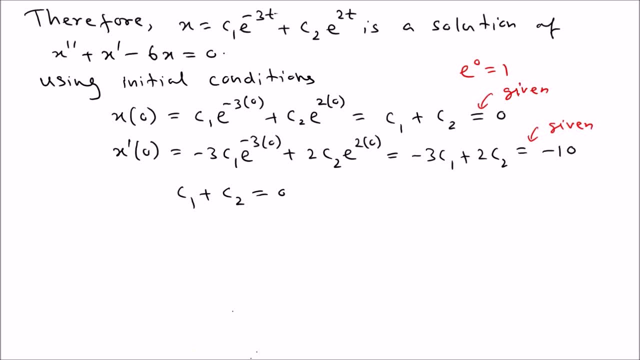 c 1 plus c 2 equals 0 negative. 3 c 1 plus 2 c 2 equal uh, negative 10.. now, uh, i'm going to call these two equations are 1 and 2, because it's going to make it easy. 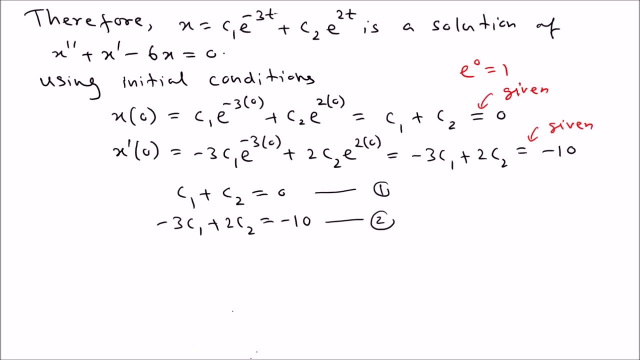 so maybe you learn how to solve these equations when you were in high school or middle school. um, so there are two methods to solve. one is you're going to solve, solve for one and substitute that in the other one. i do not recommend recommend that method, because that's. 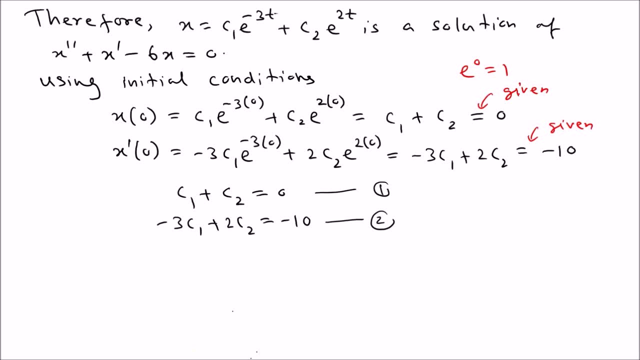 that's long, pretty long, for these kind of things. we are not going to do that. what we can do, we're gonna try to get matching coefficients, but that's much faster and there's a video just to um learn like how to solve these kind of equations and you can learn more about. 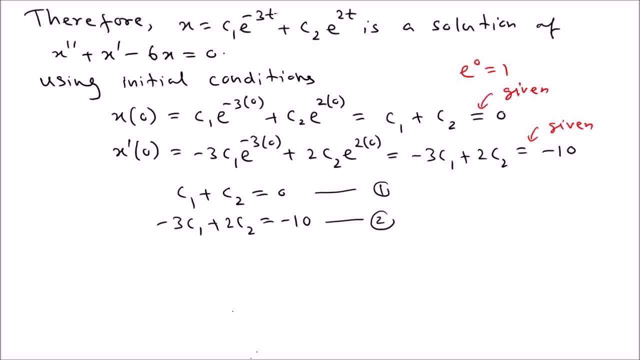 that, if you want to watch that and even like how to go for two, three, four, five, six, seven, eight, nine ten, nine, ten, nine ten, two, three, like that, so we can use that technique here, the matching, matching coefficients technique. so what's the matching coefficients, what we're gonna do? 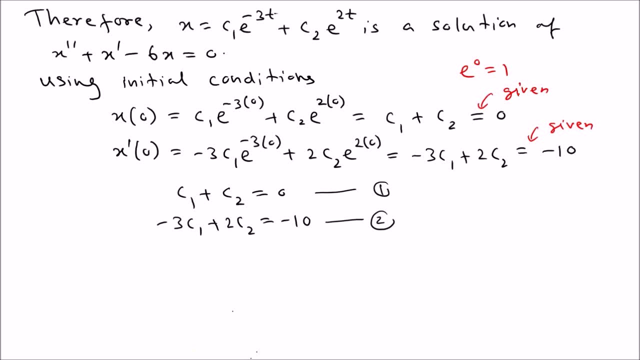 and you can see that, um, especially when you see positive and negative, we try to go for that. it's much quicker. so you can see that in the bottom equations you're gonna see negative three here. so what you're gonna do in the first one also, you try to get a. 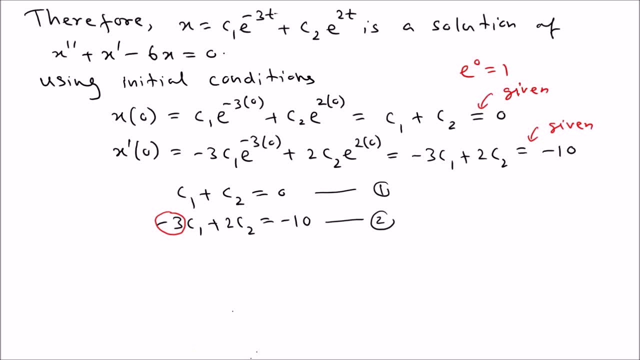 three, uh, but with opposite sign. so, for example, you try to get three c one. so if you get three c one in the top one, now what we can do, we can simply add them. once you add them you can see that c1 term gonna cancel out. so you simply get c2. so that is the. 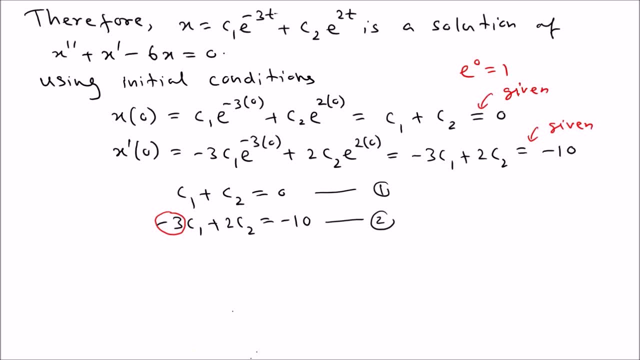 fastest way to solve this one. so that's what we're gonna do, what we call matching coefficient technique. okay, so what we're going to do by, uh, three times the first one plus the second one. if you do that, because if you multiply by three, you get- 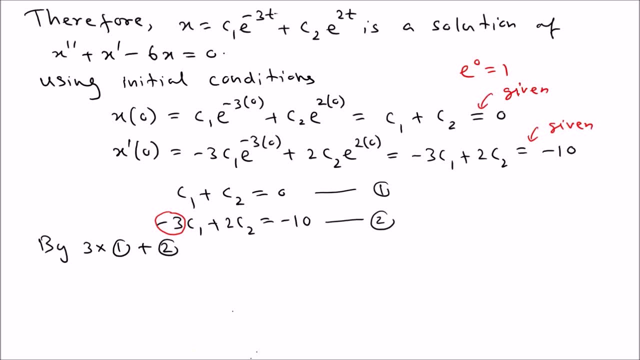 3c1 plus 3c2. when you add c1 get cancelled. you simply get 3c2 plus 2c2. uh, equal negative 10. and then this says that 5 c2 equal negative 10. now what we can do: we can divide both sides. 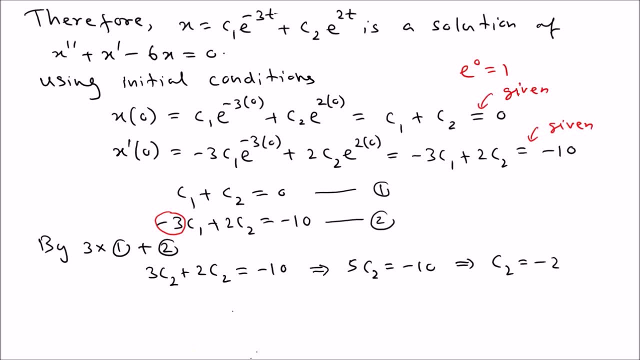 by 5, so you get negative 2. so you can see it's very easy. okay, you get the answer. and then what we can do? you can pick one of the equations by uh, but the first one is easy, so by one you can see that c1 is simply negative, c2: 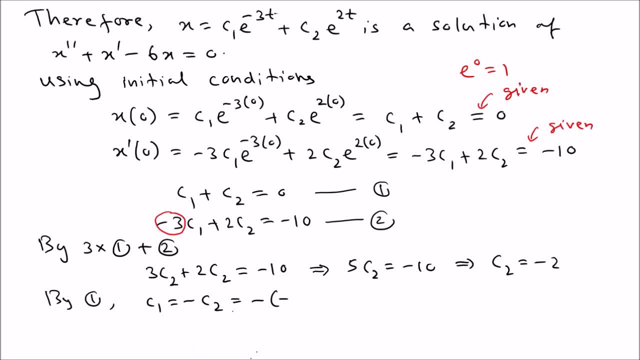 so just plug in the c2 value here so it is negative. negative 2 that means 2.. you don't want to show all these steps, but since this is the first example of this type, i'm showing all these steps, but later we can ignore some of them. some obvious steps. so we're 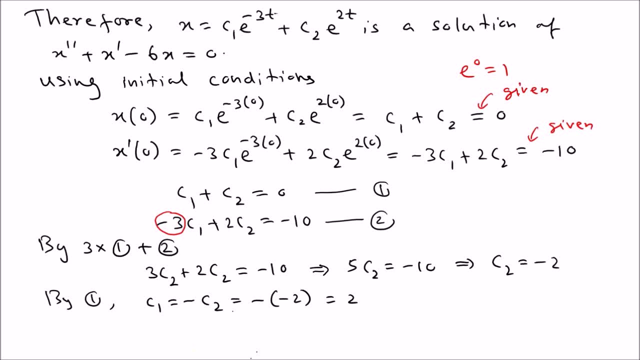 done. now you can complete that, so someone make an order. so you're gonna preserve your uh results in the best possible way. okay, that's how you're trying to do. that's why we're writing all those words. okay, um, to make a good argument. so that's a. 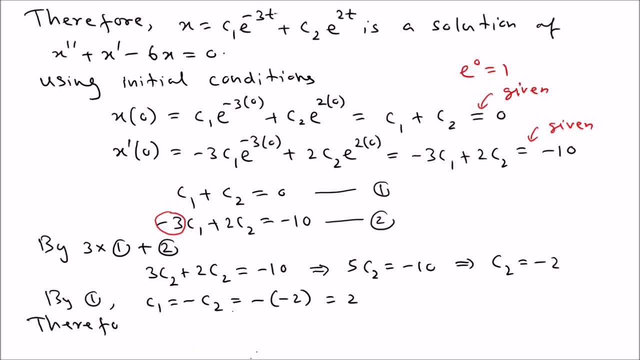 good argument. so therefore, um, therefore, we can say: the solution, the solution to the initial value problem, to the initial value, to the initial a value problem is uh, is we can write that x t which is equals to 2 e, negative 3 t minus 2 e, 2 t, so that is the. 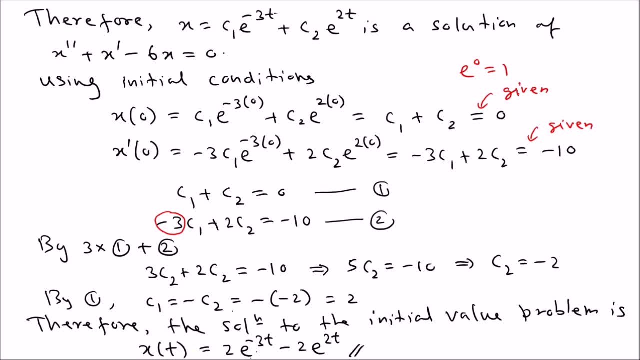 uh, final answer for that problem. so what you can see that you know if you to do this, it doesn't take much time. so it's like maximum it would take like 10 minutes to do all of these. what i'm doing is slowly just to explain everything, but you know when you want to. 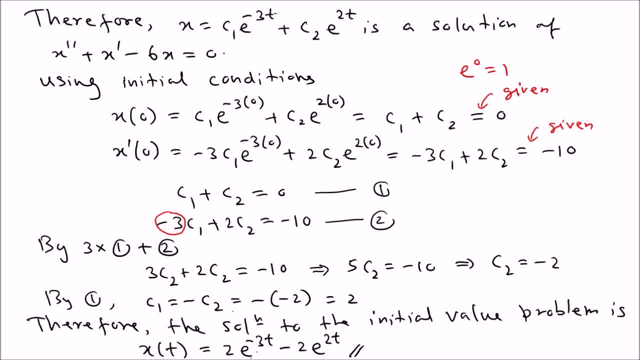 do that in exam or something you don't want to like. we don't explain, like i mean, we we explain, but not like we are not going to take too much time. you just write it fast, okay, so so it won't take too much time. uh, you can see. you can practice and see. 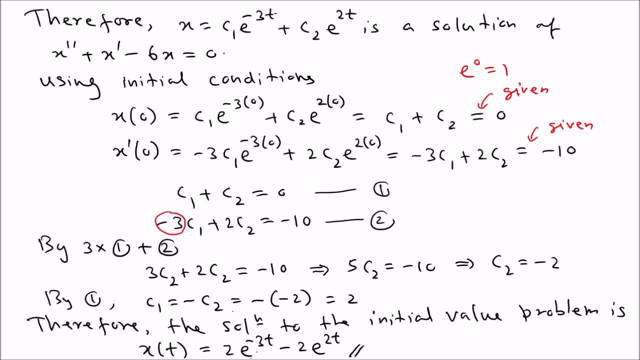 how long it takes for a problem like that. okay, good, so that's the first problem, uh, and if you need more, you can look at the first video about that to find more information and what else we did. okay, good, so let's go to the next topic. 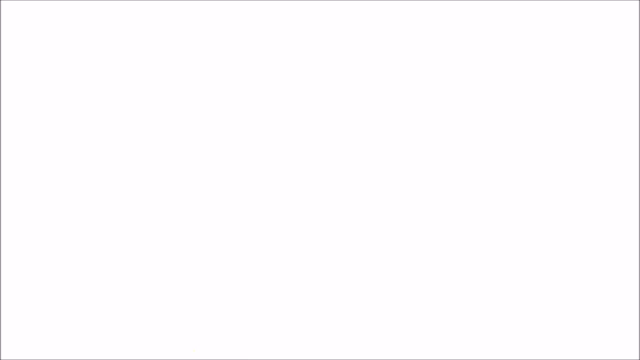 so the next topic is what we call the um four fundamental equations. so when you talk about four fundamental models, so let's talk about that: uh, four fundamental model equations for fundamental, for fundamental model equations. so we talk about, uh, four models. and why we did that? because we know that these models, like appear pretty much. 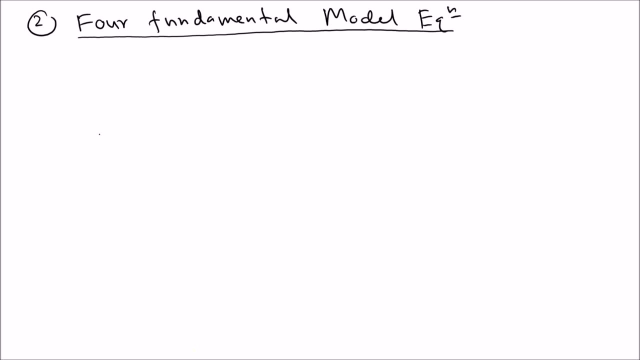 everywhere in sciences. so it's good to know those four separately. uh, okay, so, uh, the first one, uh, what we did was the exponential growth model. that's pretty much everywhere. so exponential growth, so that's pretty much everywhere. it's like you know, bacteria, uh, even like these days, covid- all of them follow the exponential growth model. 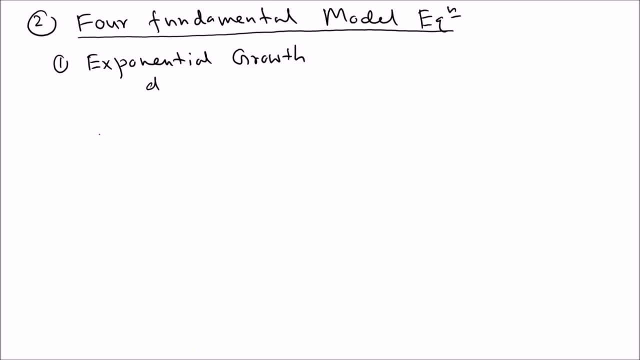 um and then uh. so the differential equation is d y over dt. we can use the t as the uh independent variable is a time, it's my more, it's like kind of makes sense. so k is a constant, we assume k is positive, so and then we know that the exponential 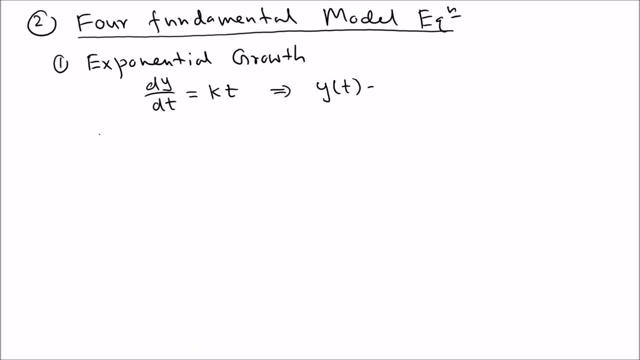 solution of this one is we can write as y t equal a constant times e to the k t. so that's the solution and you can remember, you can use this and you know. you know that even we can. we can solve this very easily. uh, just uh. this is like a separable difference. equations. 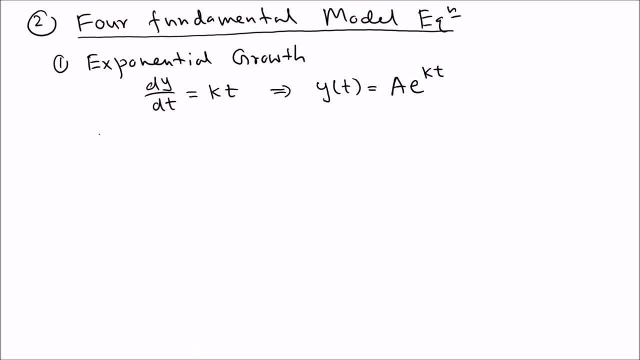 or we can even use a simple calc 1 technique to solve this one. okay, it's not a difficult, difficult problem, okay? so now, if you look at the uh, the solution for the graph of this one. so, uh, what is the graph of this, this exponential growth? 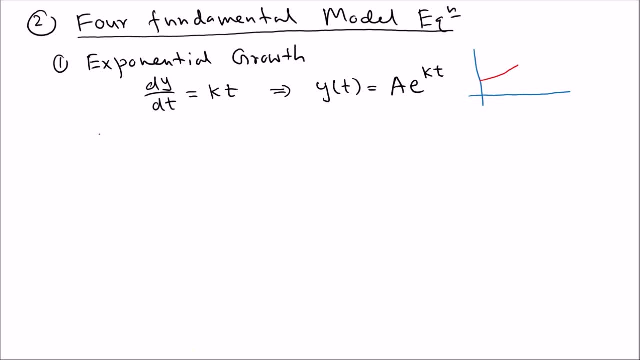 that means you start at a value and it's going to grow, uh, so this is what we call the exponential growth model. that's the starting value, a- okay, and then it's going to grow. so we assume that k is positive, it's a growth, okay. that's the. 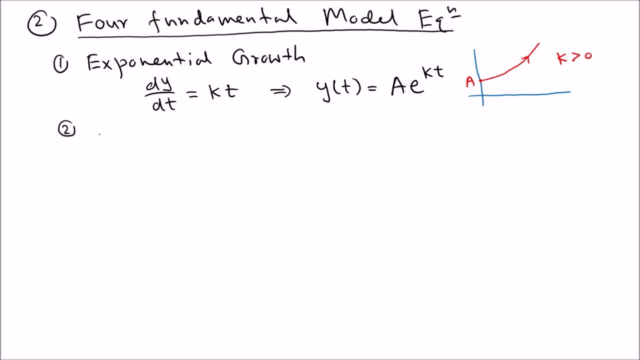 first case. and then we talk about the uh, what you call exponential decay. so exponential decay, exponential decay, model source: exponential decay is very similar: d y over d, t, and then we assume that k is positive but with a negative sign in front, like that. so it's pretty much similar. what's going to happen? 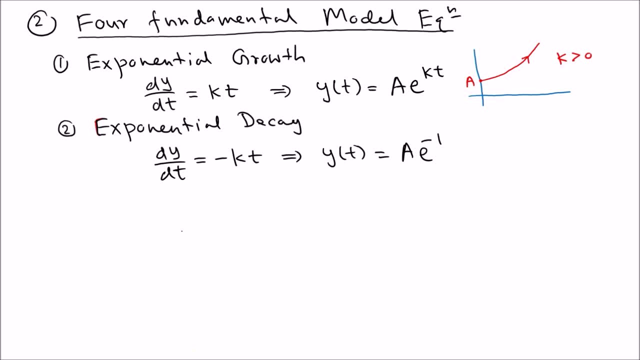 there's a negative sign in front, so the e, negative k, t. so that's what happened and uh, so, if you look at the graph, uh, very similar. but what's going to happen now is it's going to decay. so you can start with the value and go down. 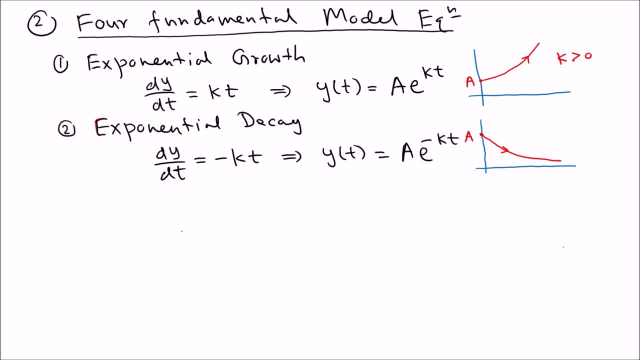 so like that you can see start with the value a and then go down, so you can see this exponential decay. and we assume that k is positive again because that we put a negative sign in the equation. so that's what we call exponential decay. uh, especially like, if you look at uh, radioactive material. 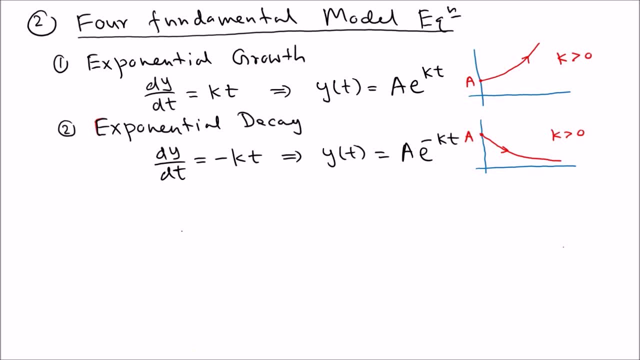 it's going to follow this kind of pattern. uh, there are a lot of other things, like you know: bacteria, if you kind of put like a disinfection there and those bacteria are going to um kill, and then if you look now, if you try to count, so it's going to follow something. 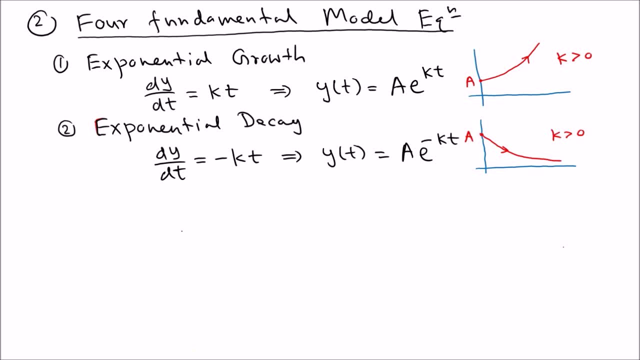 like that, so this, this models are everywhere. like you know, if you get injection, what's going to happen, so, so those are the kind of models for that. so it's very common situation. it's called exponential decay and then, uh, we talk about. the next most common one is what we call the simple harmonic motion. 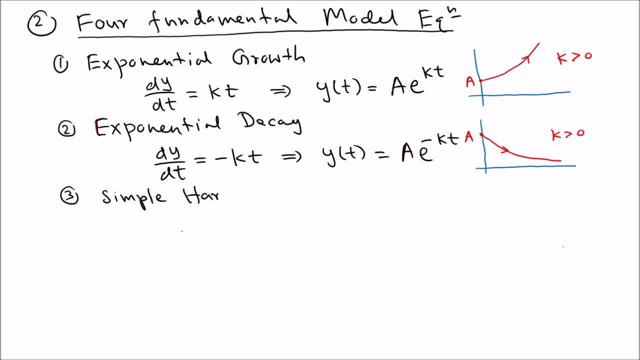 so simple, harmonic, simple harmonic motion. sometime we call shm okay, simple harmonic motion. uh, so it's going to be a difference. now, this is going to be a second order difference equation. we have like d squared, and then we that we're going to use a time variable, let's say time equal um, so we can write negative. there's. 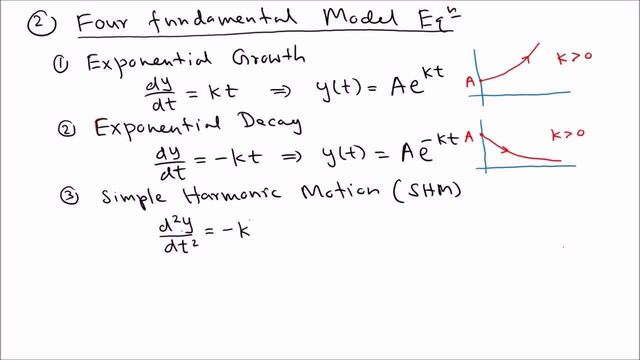 a negative sign and a k squared y. so remember, earlier you had a t, now this is y. so that's the major difference here. that's a dependent variable comes here and then we know the solution. so the solution is with sine cosine, so some number and then we have a cosine. 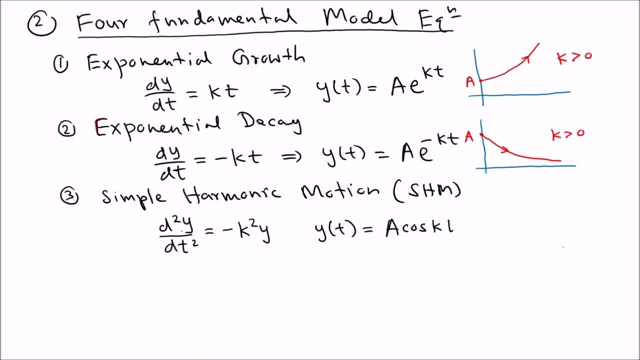 k, t, so k is the square root of that term. so you see, you have to the square root of that. and then another constant uh, sine. so one cosine, it doesn't matter which one we write first. uh, so like that. so that is the solution. so it's a sine cosine. so we have a sine cosine. 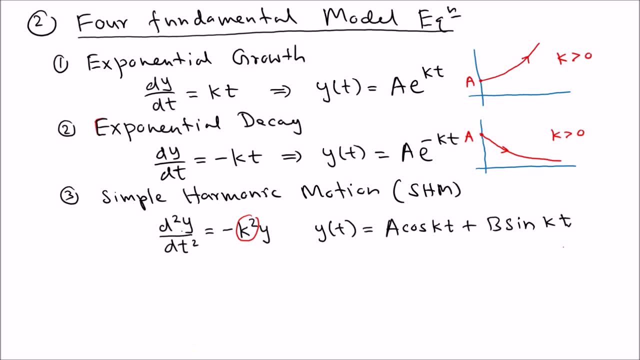 and a periodic functions. so that means if you look at the graph, it has a graph uh like this. so it's gonna be uh periodic and it's gonna fluctuate. it start with some value, depending on the initial condition. that's gonna go in a sine curve or cosine curve. 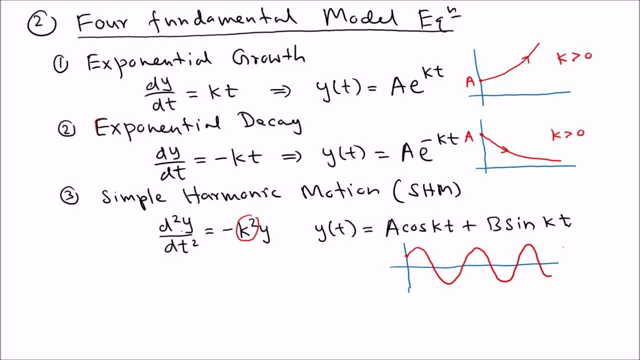 because a mixture of that. so, yeah, so that's what happened. um, so this is what we call a simple how many motion. this is everywhere, like all the atoms, um, in the body. uh, follow these curves, okay, and if you have a mass and a spring, ah, it's going to follow these kind of. 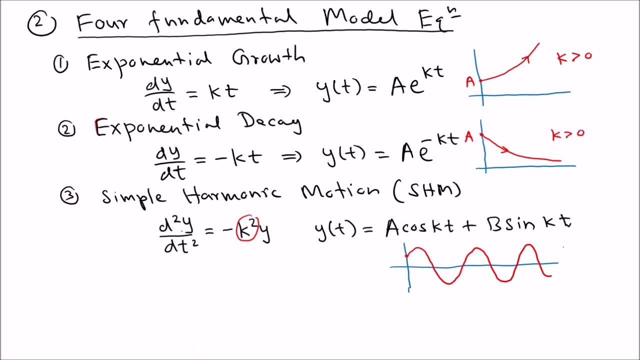 patterns. so this is like kind of very common. so it's called the simple harmonic motion. and then are the fourth one, what we normally call the hybrid model. so we have a hybrid model. what's a hybrid model is we have the exponential growth and the exponential decay. you can combine them. 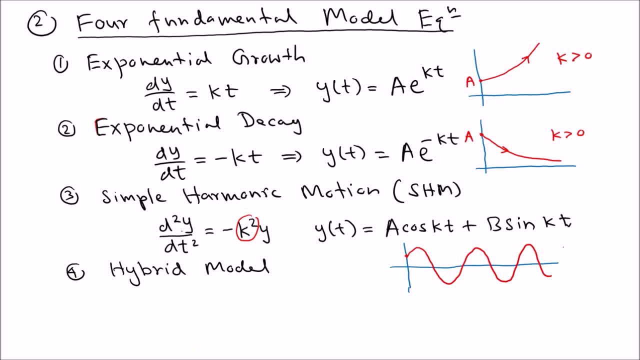 into one. that's a hybrid model and you can see the interesting relation. it is simply the same equation we just write above, but with the plus sign. so that's very interesting. what happened? that's not t here, it's the plus sign, the above one, but with the plus sign. 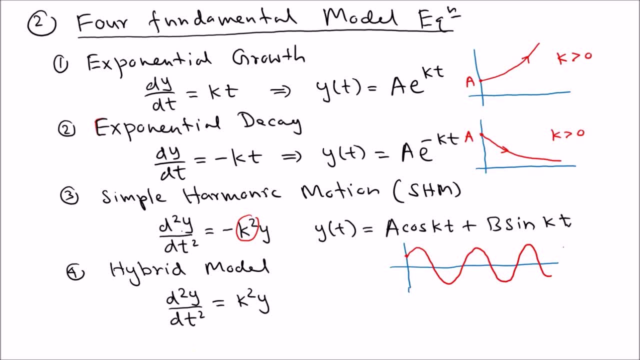 we stupid the k squared. so what's going to happen? we can write the solution of this one in two different ways. uh, the one way is using the hyperbolic cosine and hyperbolic sine function. is a cosine, is a cos, kt plus sin, uh, kt equal h, to mean there's a hyperbolic functions. 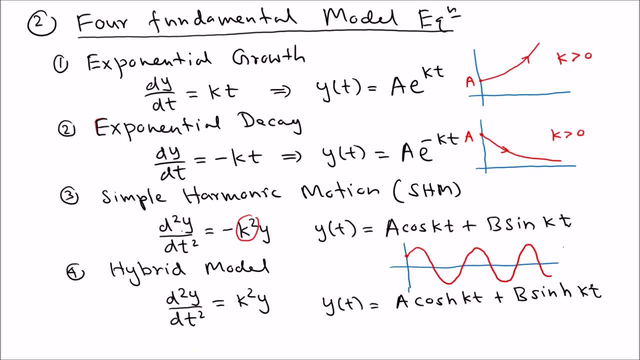 and then uh. if you are not familiar with this, you can look at the uh the video for that. we explain that and we also talk about some other properties, for example derivative. one of the major thing is that when you take the derivative uh, course becomes sin and sin become. 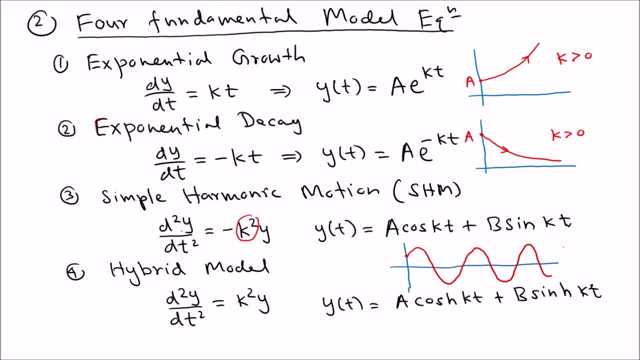 cos there are no negative signs. it's one of the major difference between the regular sign and cosine. also, uh, you can write this solution in different way. uh, i, i'm gonna still use a, b, but those are not simple. a, b, some other constants, but i'm still gonna say a, b. so a, uh, e to the uh. we can write: 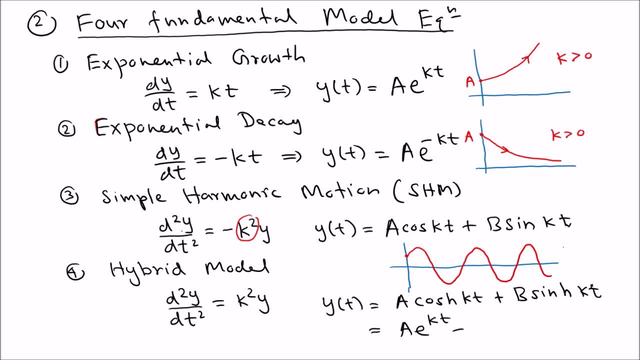 one of them. let's say kt as a kt and then plus b e to the negative kt. that's why you call the hybrid model: uh, this is the exponential um growth model and that's the exponential decay model. so you add the two and you get the hybrid. 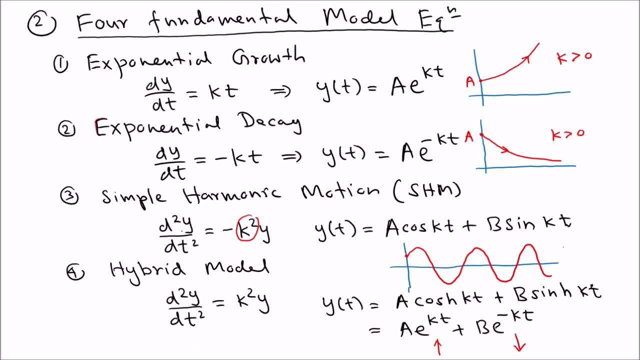 model. so that's the hybrid model for uh, when you have that different sequence, that's hybrid. so those are the four fundamental model equations and if you look at the graph, uh, so you're going to get like graphs, like this, so i'm going to put both together, uh, so 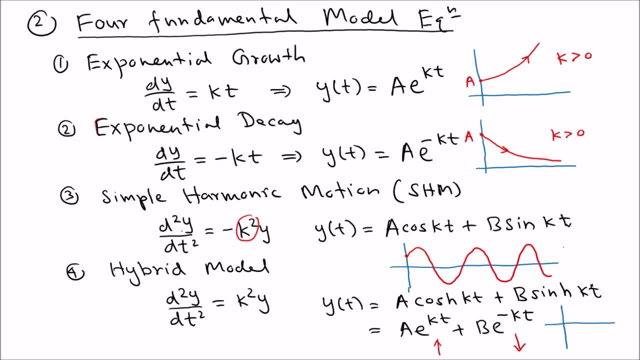 you can get a graph like that. so, because it's part sine part, part of e to the kt, part in the minus kt, so whoever the win gonna get the uh formula. so it's gonna be like that. uh, oh, like you know, it can be like that. okay, because we know that it's going to. 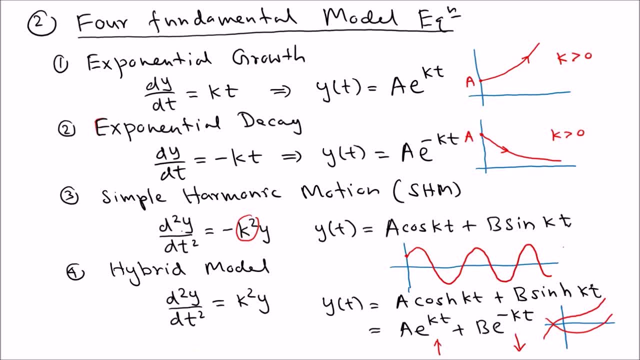 we know that, uh, if you hang a wire, heavy wire, it's gonna go in a uh equation like that: uh so it's like in many situations and uh so, uh, yeah, good, now let's try to see how to solve a problem using, uh, these models. so the goal is, if you see one of them, you can directly write. 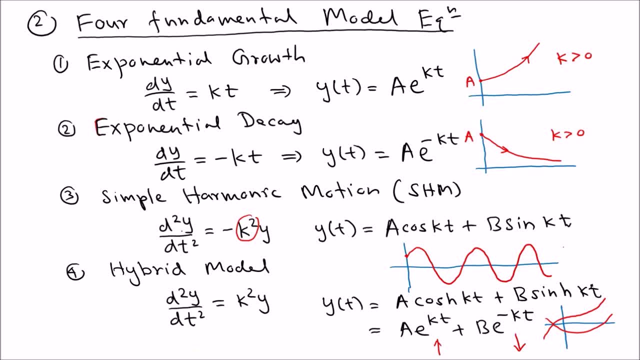 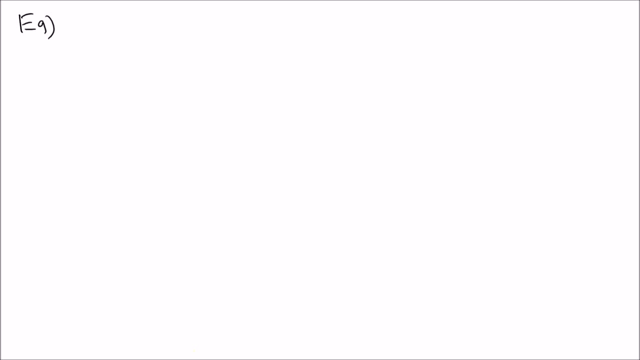 the solution. okay, because these are familiar one. remember this. this is very useful for your other causes, so you can directly use the uh results. uh, so let's look at a problem, so let's solve this problem. uh, so we have, let's say, solve the initial value problem: d squared x over d, t squared. 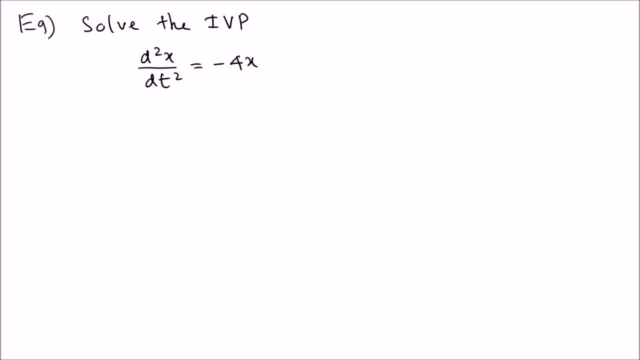 equal minus 4x, along with x 0 equal. let's say, 12 x prime 0 equals 0.. uh, why we need two conditions? because this is a second order difference equation, so you need two conditions. now what we can do, we're going to match this equation with one of those four. 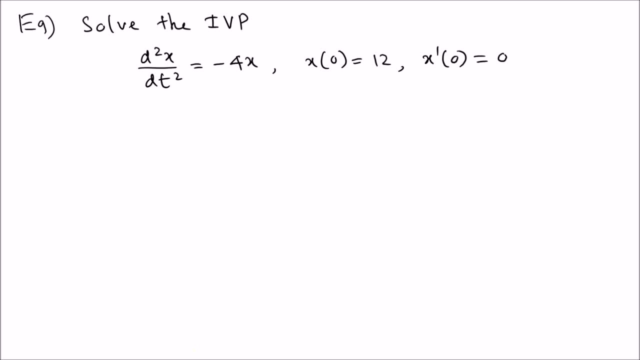 models and you can see that this is the simple harmonic motion situation. and you can see that, uh, in this problem k squared equal 4. this implies k equal to, because we consider only the positive value. now we can write the general solution. so the general solution is: 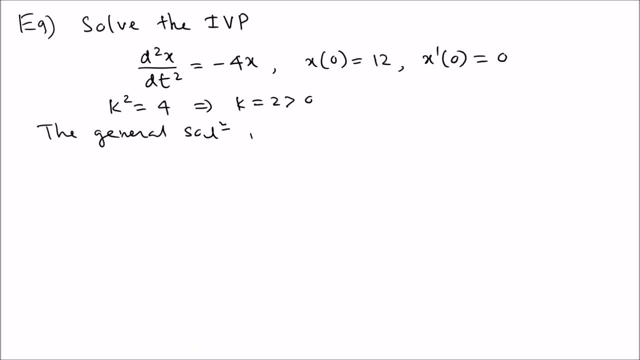 so the general solution is: uh, you can say xt equals, you can directly write it: it is a cos 2 t. but 2 is t is the independent variable. you have to be careful, so the independent variable goes there, okay. and then also uh, this x and this has to be x. 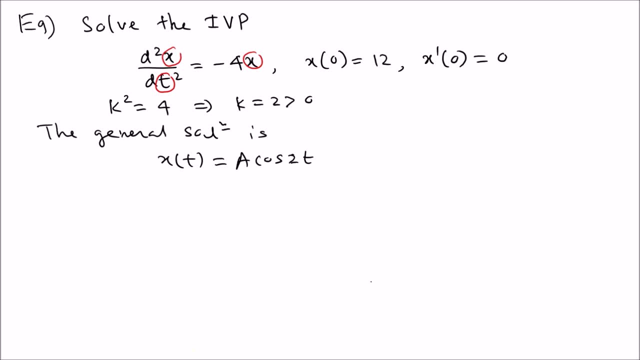 otherwise it is not this type of problem. good, um, and then so we have uh plus plus b, sine 2 t, so we have that. so that's the. this is directly come from the four model equations. now what we can do are we can use the initial conditions. but we can see that when you want to write the 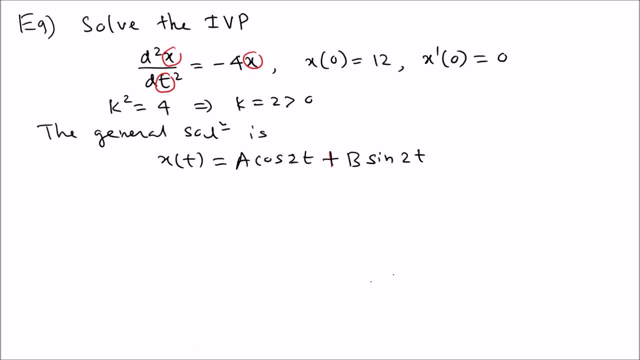 use the initial conditions. there's a prime, so that means let's take the derivative first. so taking derivatives, taking derivative, so we can write x prime, t equal. so what's the derivative of this one? it's a cosine, so derivative means the negative sign. but there's a 2 here, that 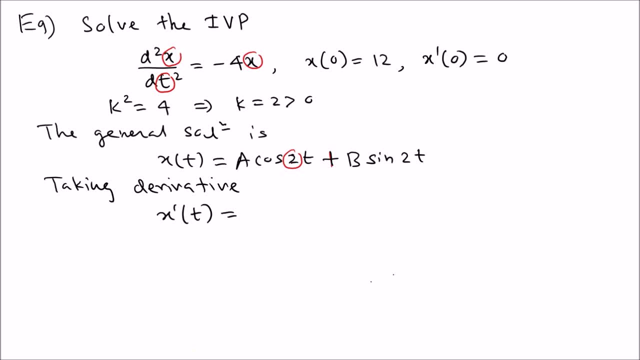 means by the chain rule that 2 comes out, so that's going to be negative 2 a sine, 2 t plus same thing. sine, when you take the derivative is going to be cosine, so it may 2 b cosine, 2 t by the chain rule. now we can use the initial conditions. so 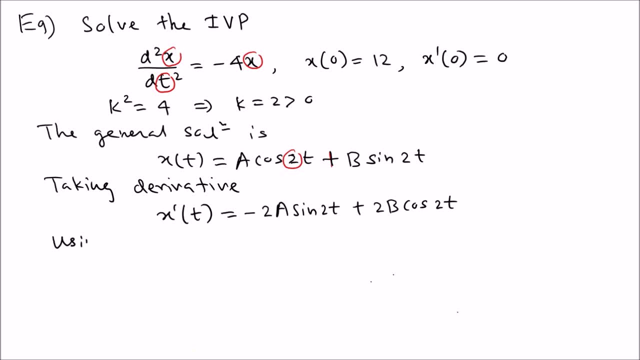 um, using initial conditions. using initial condition, we have x 0, x 0. that means plug in 0 for the t, so you're going to get a cosine 0 plus b sine 0, which is equals to 12.. this is given. now we know that cosine 0 equals to 1, sine 0 equals to 0. so because of that, 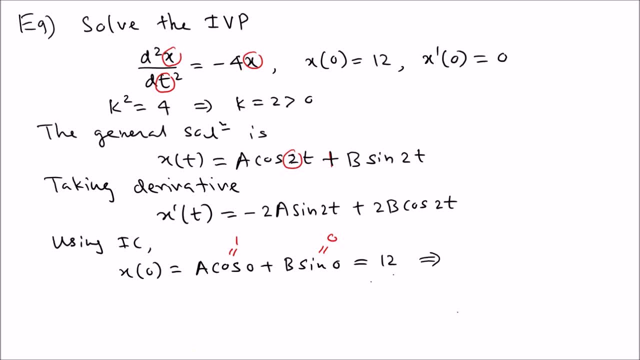 this simply implies that a plus 0 equal 12. that means a equal 12. so we find one value. now, using the other condition, we know that x prime 0, which is, equals to the second one. so negative 2a, you can actually put the value here. so it is. we already know the value. 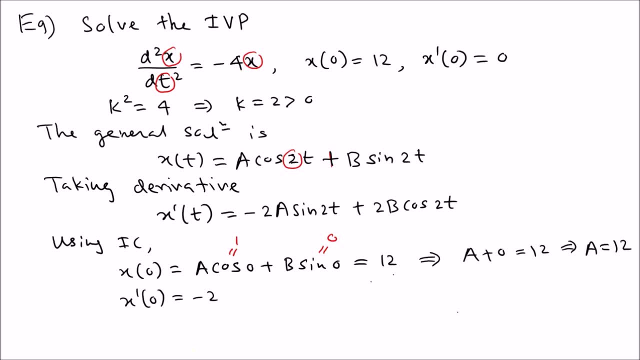 so i'll put the value here just to make the calculation easier. so 12 ah sine 0 plus 2b cosine 0, which is equal to 0. so again we know that the sine 0 equals 0, cosine 0 equals 1. so that means this is that: 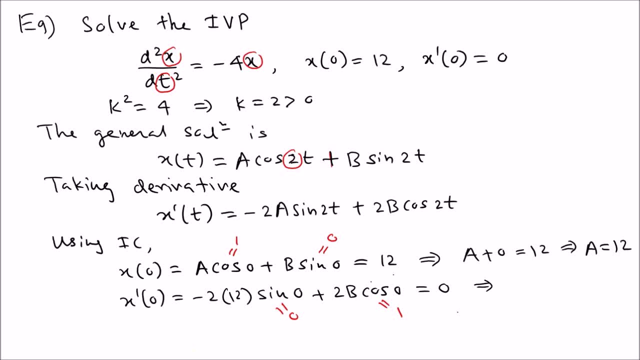 so nothing comes from the first term. this says that 2b equals 0. so this says that b equals 0. that means the beta. i'm going to go away. so that means i'm going to go away from this. so i'm going to go away from this. 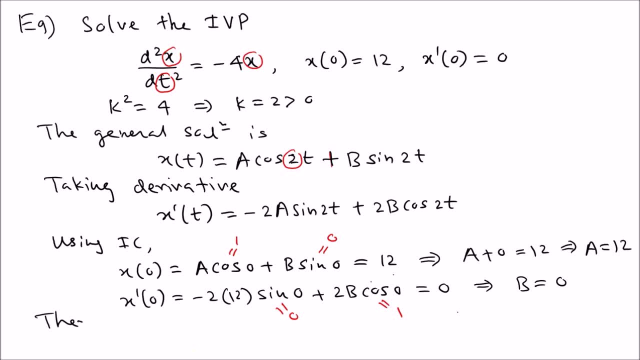 that means, therefore, the solution is therefore, the solution to the initial value problem is simply x t equal to 12 cosine 2 t. so that's the solution of the problem. good, um, so let's go to the uh, the next topic. so what's the next topic? 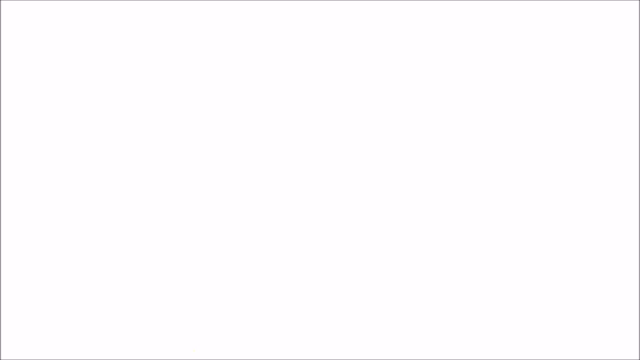 so what's we're going to do? uh, we're going to talk about, uh, the classification of differential equations. so, um. so, number three: the classification of differential equations. classification of differential equations: so we talk about various types. so we've got the, we've got the. so we first start with what we mean by. 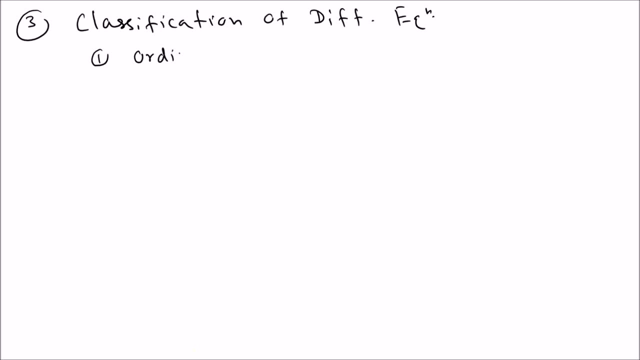 so we first start with what we mean by a ordinary differential equation. ordinary differential equation, differential equation, so we normally call this ode, ah, in this one what we have: one independent variable, one independent, one independent a variable, so we have one independent variable. so, uh, an example would be something like this: 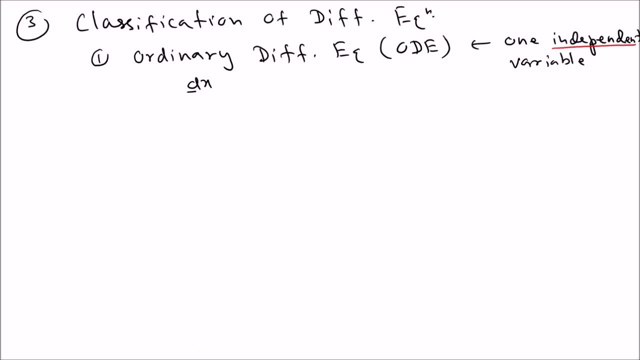 dx over dt. r plus 3, x equal t plus 1. you can see the independent variable is t and thus there are no more independent variables. so it's an ordinary differential equations, or d, e and then the next type. so this is the next type of differential equation. 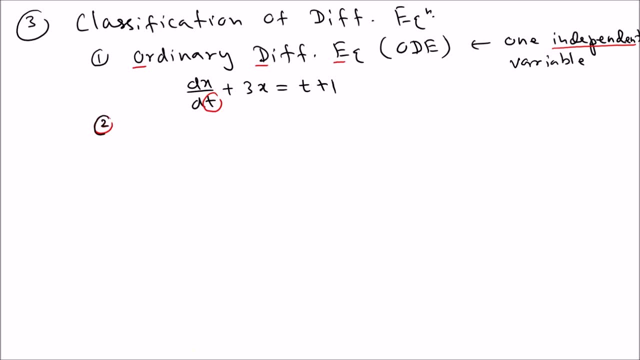 is what we call the partial differential equation. so we have partial differential equations, partial differential equations, partial differential equation, or we call this- is a, p d e. there's a shortened form for that: p d e, partial differential equations. so what we have- more than one, more than one, uh, independent variable. 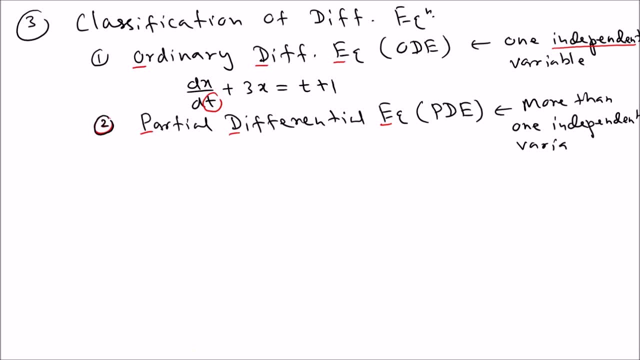 more than one independent variable. so there are more than one independent variable. sometimes the space and time, those are the two in two common independent variables. so, uh, so such a differential equation have a kind of form like this so we can write, let's say, let's say what is the 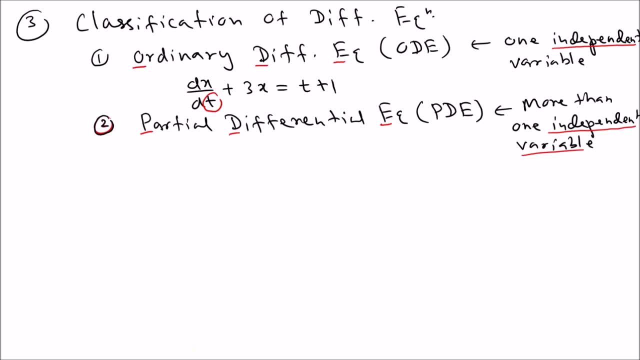 of x and y. so then we can write it like this: so if you use a function of x and y, if u, uh is a function of x and y, so that u is a function of x and y. so that's how we write it, so then you can. 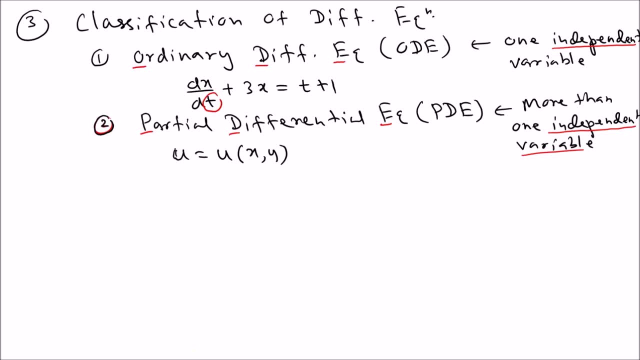 write a differential equation, uh like this: uh, we can say uh, we can use the daba for that. so w over daba x. uh plus three times w over daba t. equal. we can say x, uh plus t. so this is a partial differential equation and you can see that there are 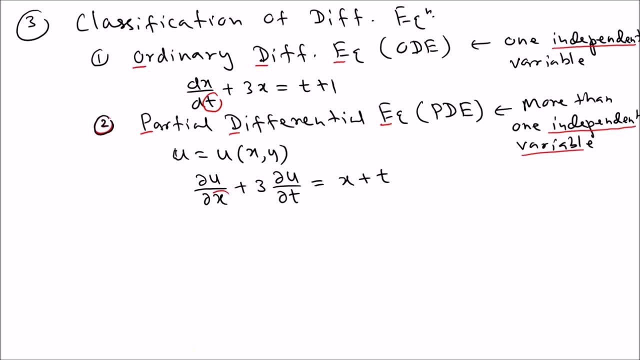 two independent variable, space and time. so x and t are independent variables, but that is a different course and we are not going to focus that in this course. this is only for a partial differential. this is only for ordinary differential equations, so we are not going to focus that in this. 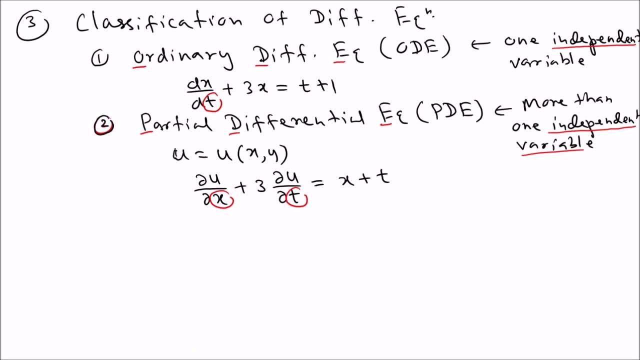 except in few cases, because we need, uh, the idea of partial differential equation in in certain situations, and other than that, we are not going to focus on that. okay, that's about that. so there are two uh independent variables. so these are the uh independent variables independent. okay, so there are two. in the first one, you only have one, okay. 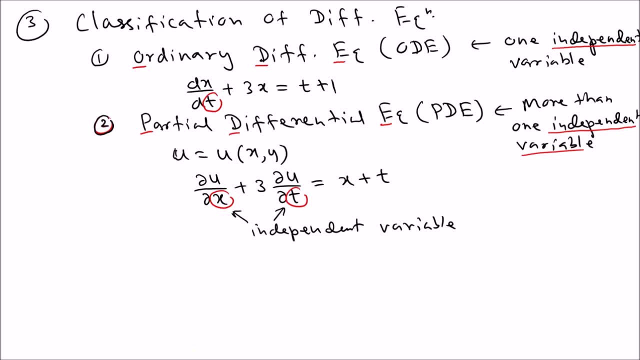 um, and then, uh, we talk about what we mean by independent a, um, order of a differential equation. so that's the next topic. we talk about the order of a differential equation, so order. so order means the highest derivative appear, highest derivative, highest derivative, highest derivative is what we call the order. so, for example, if 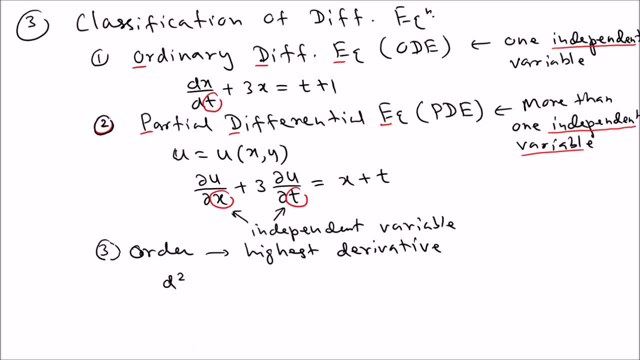 you look at this differential equation: uh, d square d squared y over d, x squared plus x equal 3.. so you can see the highest derivative to appear is 2, so we call this is a second order difference equation. we don't take a two order. 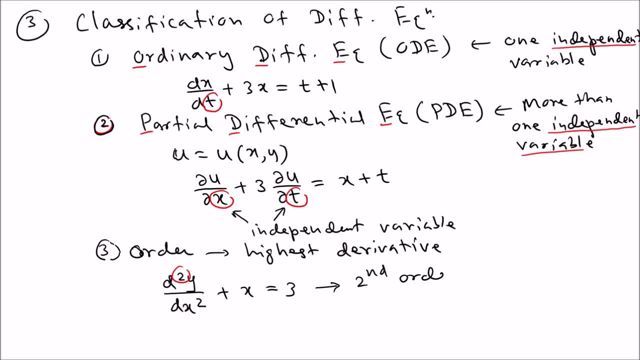 so we say this is a second order, uh ode second order od e. second order od e. so we say this is a second order, uh ode second order od e. good, um, that's the highest they really appear. the question why you do that? because you know that, depending on the order, 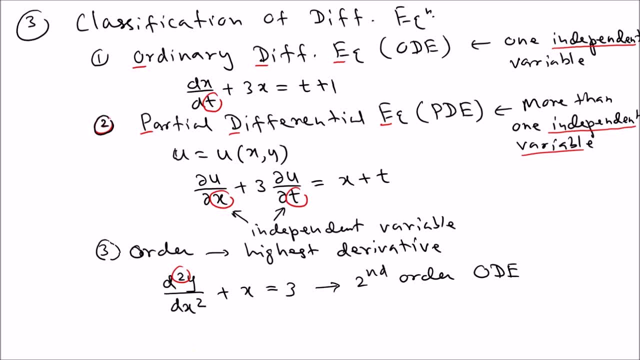 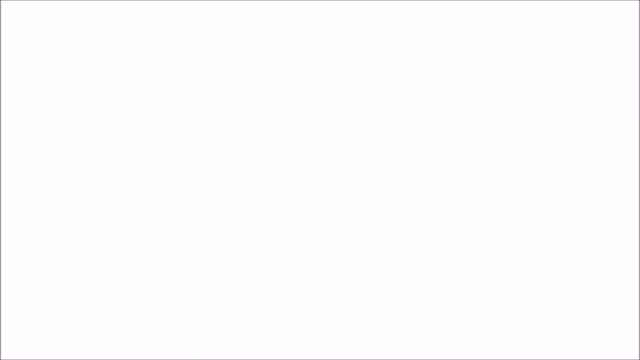 we had to use different techniques. that's, that's the major point here. so the next important topic is what we mean by linear and non-linear equations. so the next one is: uh, before a linear and non-linear, so linear versus non-linear, um, so that means linear means no powers other than 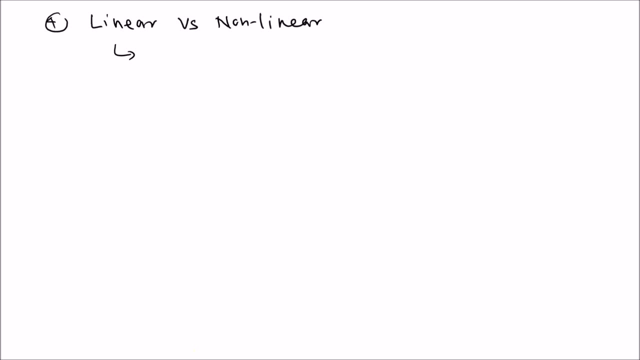 one of the dependent variable. so you're going to see no powers, no powers other than one, other than one. so of the dependent variable, of the dependent variable, so we don't worry about the independent variable. so there can be only powers of one. so that means there are no products. okay. 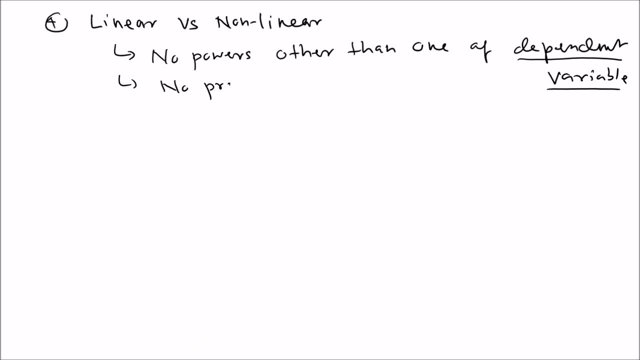 in other words, no products, no products of the dependent variable, dependent variable or its derivatives. so let's talk about uh two examples. so let's talk about uh two examples. if you say x is the dependent variable, so we can write dx over dt plus t, cube x equal t, so you can see that there are no. 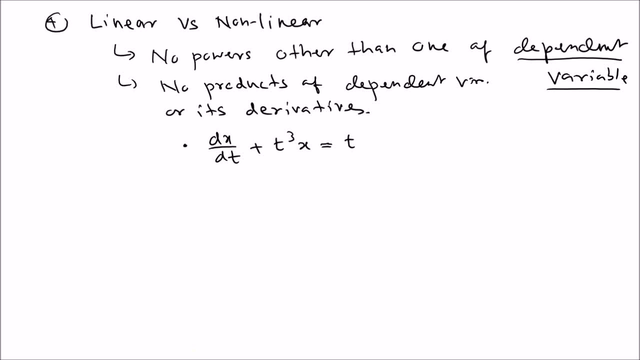 powers other than one present in it. so that means there is no powers of the powers of x other than 1. so this is a linear equation. t, 3, t is the independent value. that's okay. so this is linear. and if you look at this, one x times dx over dt plus, 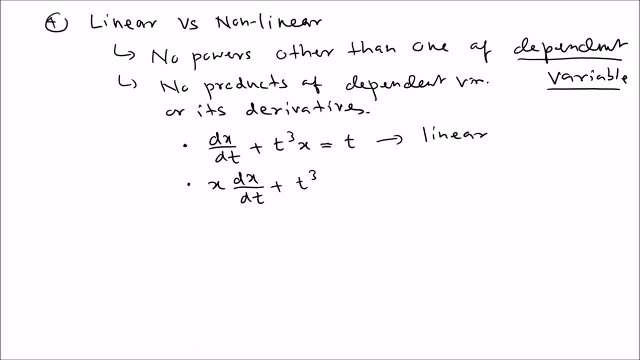 the same thing here: t 3 x equal t. this is non-linear, so those two equations make a big difference when you try to solve. linear equations are easy to solve. any equations are easy to solve, so that's the fact. the linear equations are easy to solve. 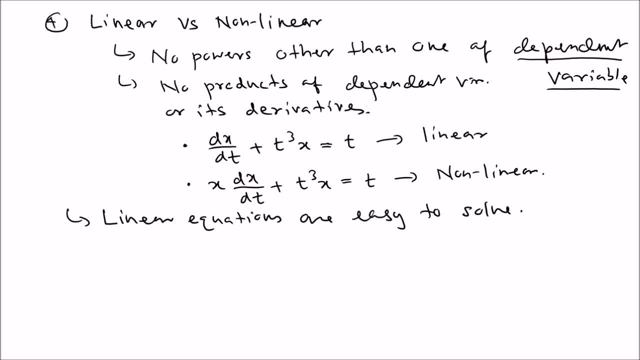 good. ah, so these are linear equations and they are easy to solve, non-linear good. and then talk about what we mean by the constant coefficient. so number five: constant, coefficient, constant, coefficient, constant, coefficient, uh, equations. so that means all the constants are coefficient, all the constants, all the um coefficients. oh, i'm sorry, all the coefficients are constants. 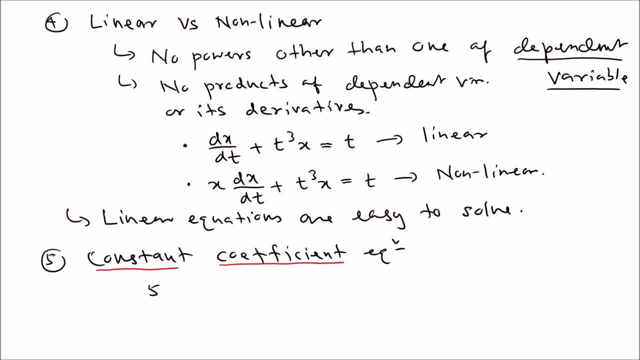 okay, all the coefficients are constant. so, for example, 5 x double prime minus 3 x prime plus x equals 0. so this is a constant coefficient difference equation. you can see that all the coefficients are just numbers. uh, what we normally do is we consider a characteristic equation to solve, okay. 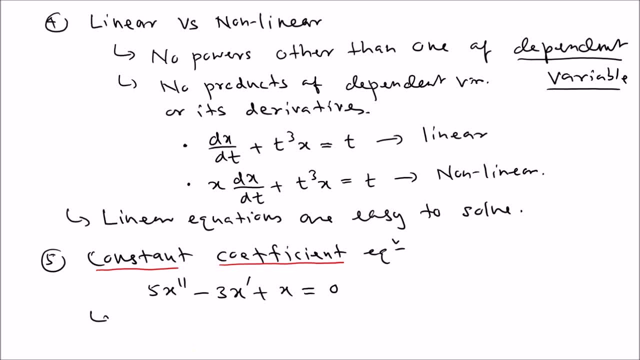 so, uh, so use characteristic equation in lambda. uh, use a characteristic equation to solve uh which remember which uh which is in lambda? so we write a lambda equation, good, um, and there's a characteristic equation for matrices as well. but here, uh, we call the characteristic equation for that, because i can characterize the, the. 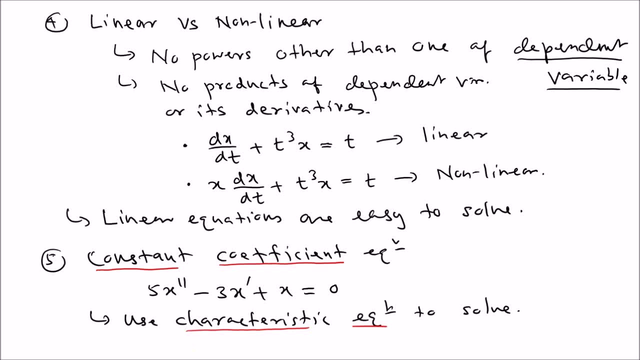 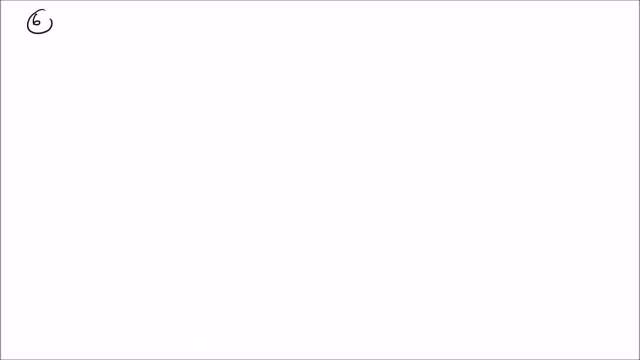 okay, that's a constant coefficient. and then let's talk about homogeneous versus non-homogeneous. so the next one. so we have homogeneous, uh, versus non-homogeneous. so be careful, are the homogeneous and non-homogeneous has a different, two different meaning in differential equations. 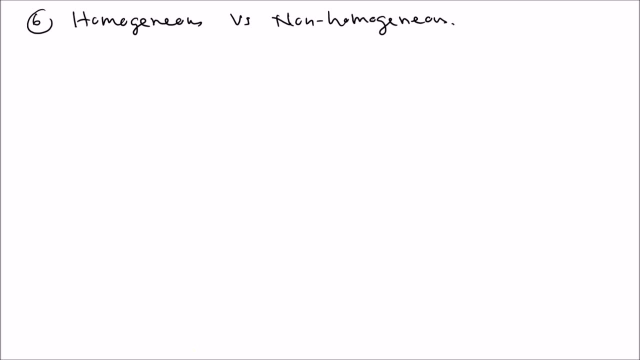 uh, and then we can talk about the homogenous and non-homogeneous again later. so here, um, uh, what we mean by the homogeneous is uh, whether uh the differential equation equals zero or not. so like uh, it will be easier from an example. so, for example, if you have 5 x double prime, 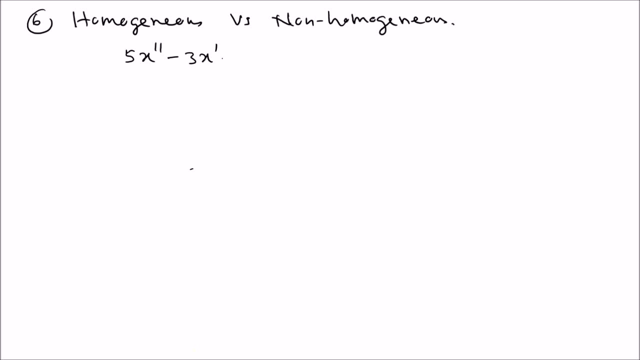 minus 3, x, prime plus x equals 0. you see that uh. so you can see that uh. so you're gonna set the differential equation to zero. that means that side is not a uh, uh function of the independent variable, so all the dependent variable. you can put it one side. 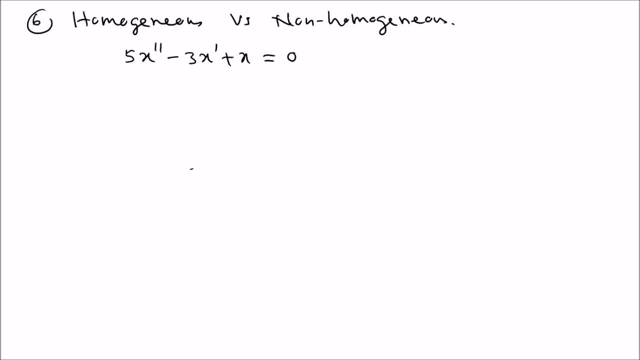 and then you can see that. so we can write this one as a. this is what you call a homogeneous equation. so homogeneous, so no functions of the independent variable. okay, so it's a homogeneous equation, so we can write this one as a. this is what we call a homogeneous equation. now you can say: 5 x double prime. 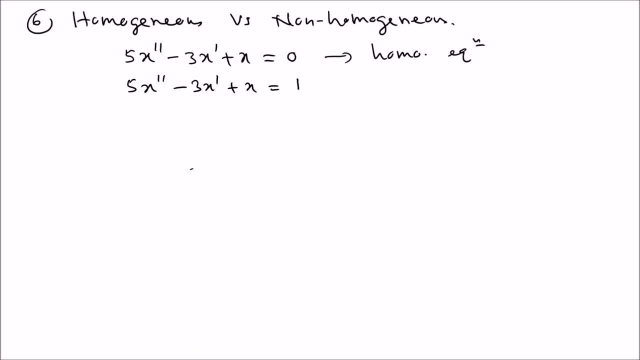 minus 3 x prime plus x equal t. this is non-homogeneous because it's a function of uh, the independent variable. okay, so if you have a function, because you can all always pull, all the uh dependent variable turns to one side, and then if you see a function of the independent variable alone, 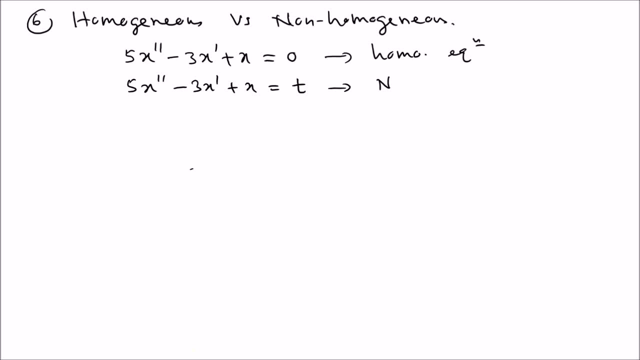 that's going to be non-homogeneous. okay, you see, a function of the independent variable alone, a zero. we just say other than zero. okay, because zero is also function, but other than zero. so this is what we call non-homogeneous because of that t term. so this is, uh, non-homogeneous. 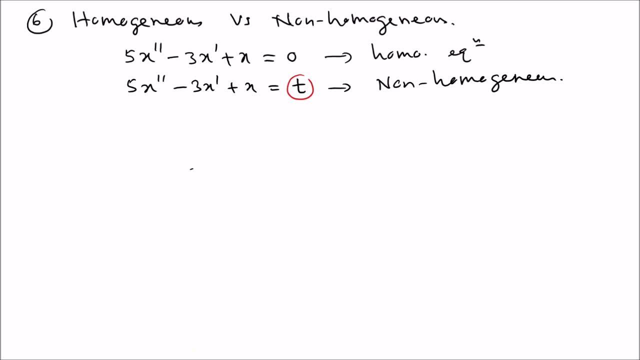 good, a homogeneous and unknown. so there are. there's a function of the independent variable alone. okay, so that means that the independent variable is a function of the independent variable only. so that means let's write that. so there is, there is a function. function of the independent variable. 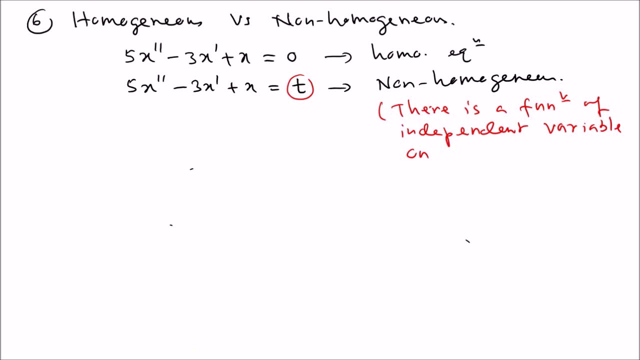 only independent variable only. okay. so if you see a function of independent variable only, it is what we call non-homogeneous. and then we have what we call autonomous, autonomous, autonomous differential equations. so autonomous means, uh, if the differential equation does not depend on the independent variable, we call it the autonomous differential. 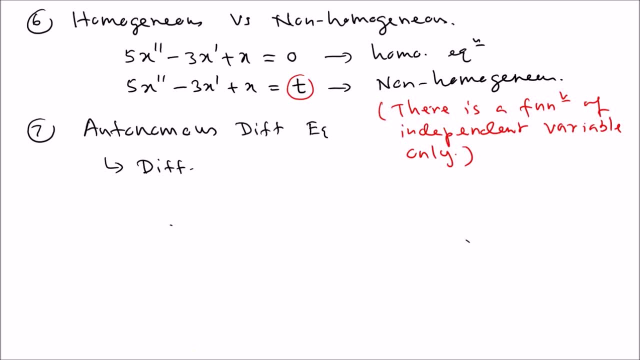 equation, the differential equation, difference equation does not, does not depend on the, does not depend on the independent variable independently. okay, if the decision does not depend on the independent variable we call it is a autonomous differential equations. let's write this one so you can say d x over d t plus x squared. 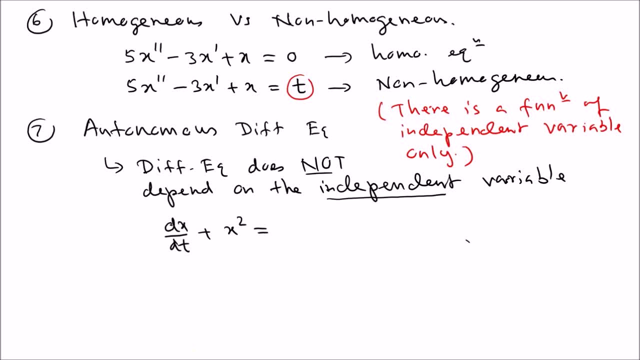 equal uh three. so you can see that this is. this does not depend on the t variable, so this is autonomous one. okay, so this is autonomous. so if you had like a function of t somewhere, so it is, it is non-autonomous, it's autonomous, okay. and then the last one is the. 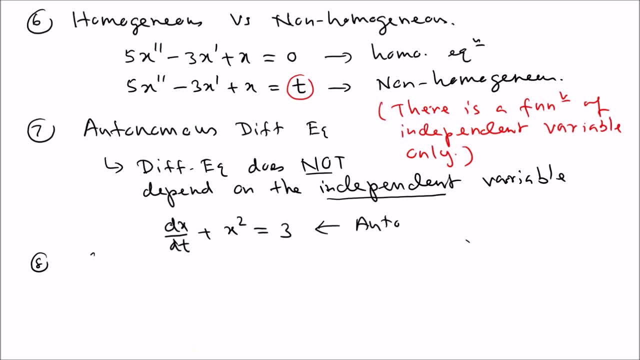 autonomous topic of this is what we call system of ods. system of ods, so a system of od. so not just one equation, but there are many equations, so like, for example, x prime equal to y plus e to the t, y prime equal, let's say, 3x plus y sine t. so this is what we call a. 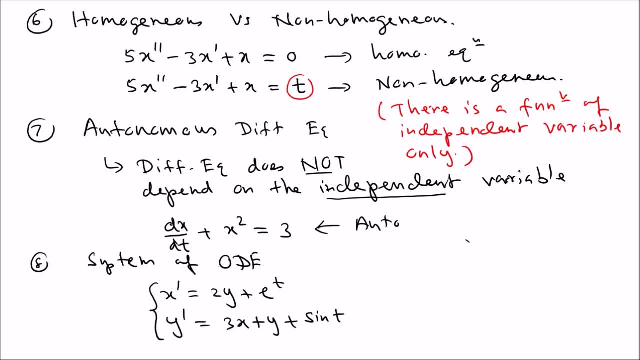 system of od. uh, so we discuss all of these types. good, uh, so that's about that. uh, so i don't discuss any further examples of this one, but if any more example, you can look at the corresponding uh lecture for that. but this is the kind of basic ideas we talk about. 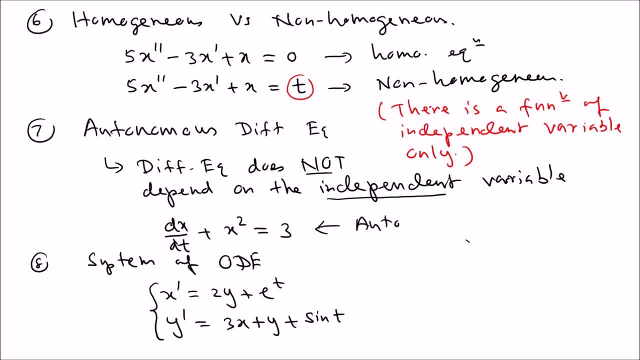 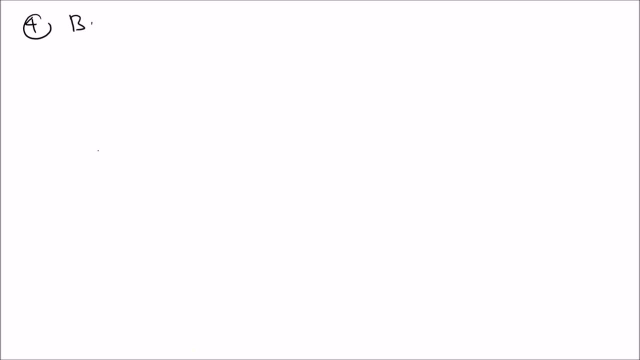 let's go to the next topic. uh, so the next one is what we call the basic integration. so number four: basic integration, basic integration. so this is a very simple thing that we did. we did even this one in calc one. uh, so there are two types, so let's go with the type one. 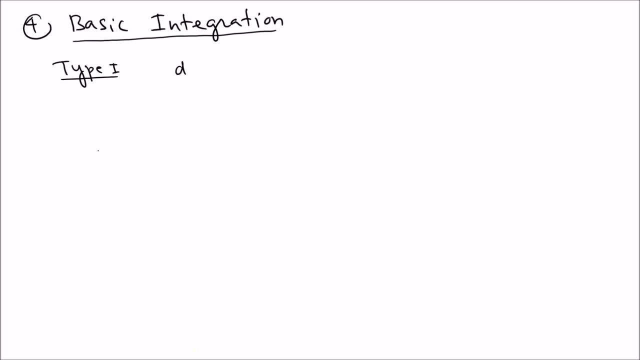 so what's the type one? you have a differential equation which is just on the on the right hand side, the independent variable. so this is a function of the independent variable. so this is a function of the independent variable, only independent variable. so if this is a function of independent variable things, 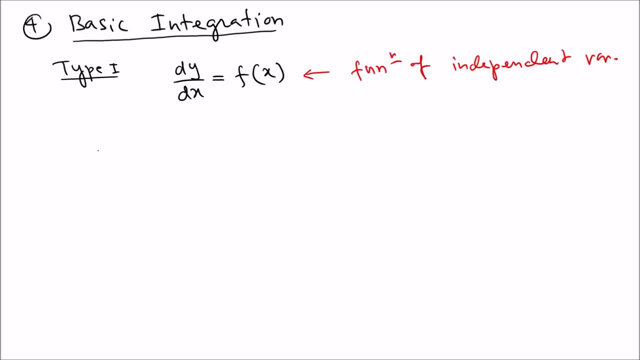 are very easy: just integrate the two sides. so that means y is simply the derivative of a, y simply the integral of the derivative. okay, we're just going to integrate with respect to x so that they cancel each other. so that means simply become the integral of f, x, dx. so it's very simple, just. 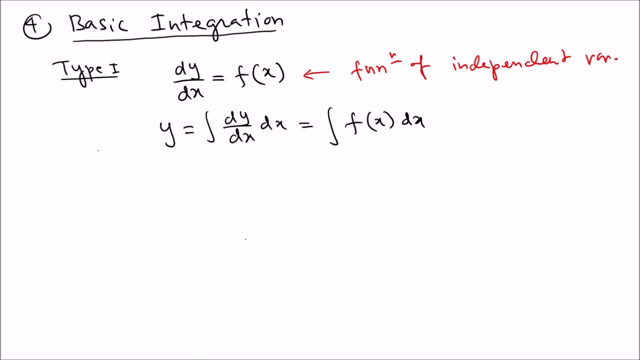 integrate. that's going to happen if the derivative is a function of the independent variable only. so this is the easiest case. you can simply integrate that. you have to be careful, uh, because sometimes, um, it's not the case. okay, so let's talk about type two. so what's the type two is? 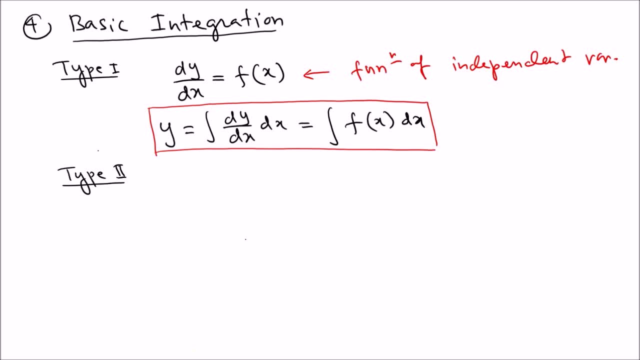 so type two: uh, we have d y over d x, but it is a function of the dependent variable. now, okay, so if you get the function of dependent variable, so let's write. so what happens is that you get the function of the dependent variable. what happened now is is a function of. 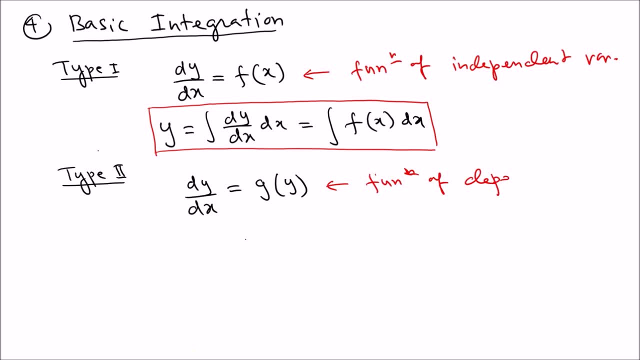 function of the dependent. so what we can do in this case, we can flip the uh equation over, so we can write this one as dx over dy, 1 over gy. now you can see that this came back to the previous case, because you can simply consider y as the dependent variable in this case. 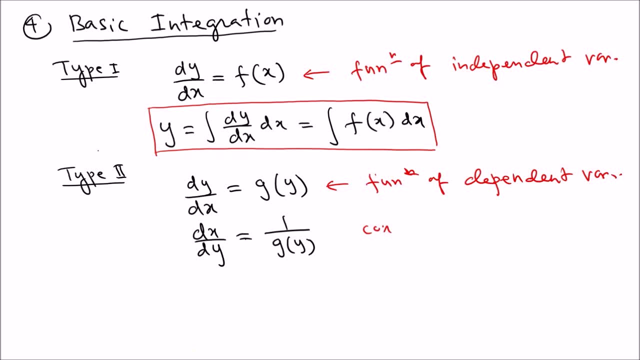 so we can see: consider, consider y as the independent variable, so that's the whole point- and then just indicate the two sides again with respect to y. now, so that means you're going to get x, which is the integral of dx, over dy with respect to y, not x integral of. 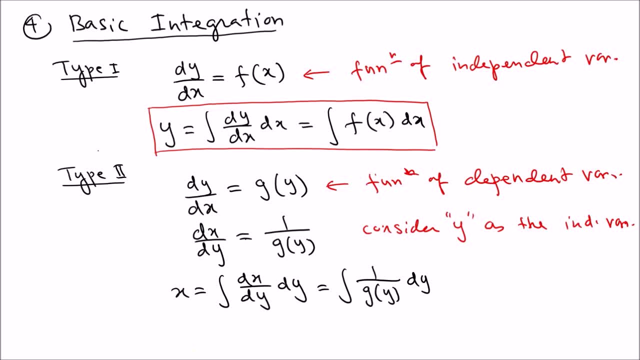 g, y, d, y. so that's what's going to happen in that case. we're going to get, with respect to y, okay, those are the, the first type, what we call the basic integration. so you can just use a table of integrals for that, uh, the common ones, and you can do a lot. 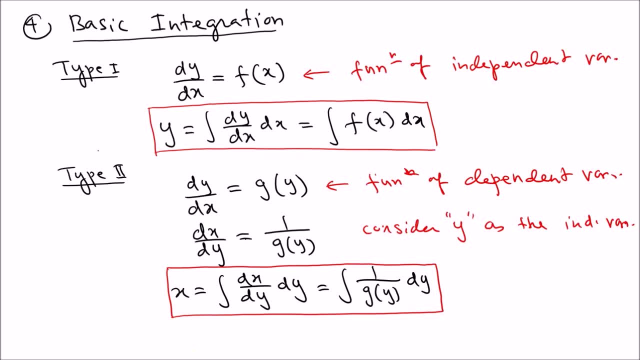 of problems just using this, these two equations. so the first case is the derivative is a function of the independent variable. second one is a derivative of the function of the dependent variable. in the second case we're going to flip the equation over and integrate. so let's do two examples from those two types. 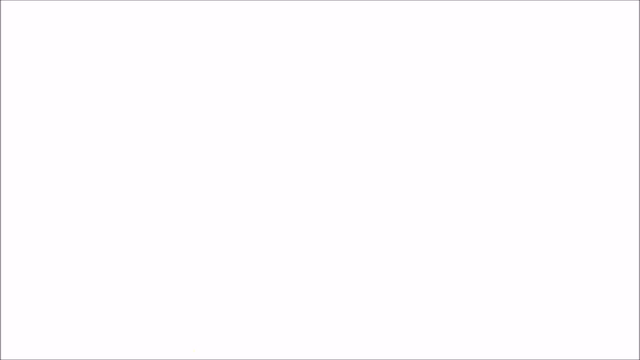 so we have this first example. so let's say um solve the initial value problem. let's say d, y over dx, equal three times cosine, x, three cosine. let's say two x minus 8, e to the negative, 4x plus 5, along with y 0 equal negative 3, something like that. 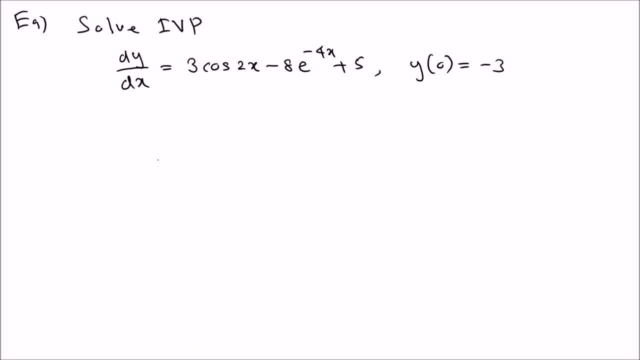 and what you notice. you notice that is the independent variable. this is the independent variable, and you can see that it's only a function of the independent variable. so that means this is the case, one that might be the case here. integrate the two sides, okay. so you can see the function of. 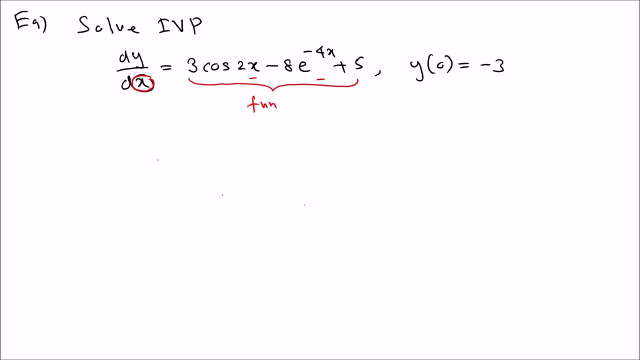 so this is a function of x. okay, x is the independent variable. so that means we can have, we can integrate. so by integrating, just integrate, okay, by integrating y equal, just the integral. so it is 3 cosine 2x minus 8, e to the negative 4x. 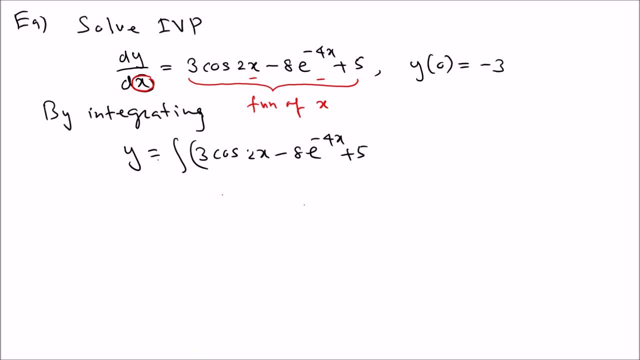 plus 5 dx. so this is just very basic integrals and if you uh forget. so these are the kind of formula that we're going to use here. so if you have e to the k, okay, d, x. the answer is simply 1 over k, e to the k, x plus c. 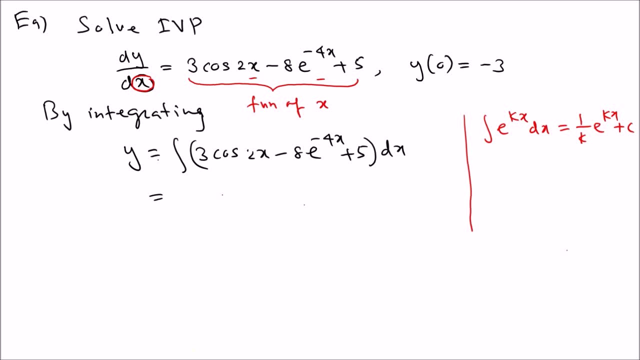 this only works when k is a constant. and the second one: if you have a cosine k, x, d, x, and we know that it is simply 1 over k, sine k, x, so just divide by k. and the other one: if you have a sine k, x, k has to be a constant, so this is simply negative: 1 over k. 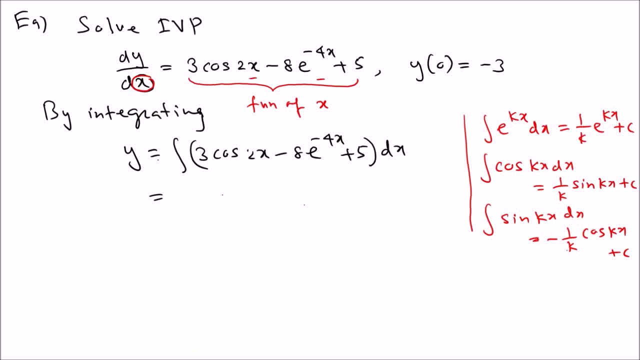 cosine k, x plus c, so those are the kind of three common ones. and then also we have the power rule that everyone know, and so this is what we're going to use now. so that means in this case, k equals 2, so simply divide by 2. it's a cosine that means. 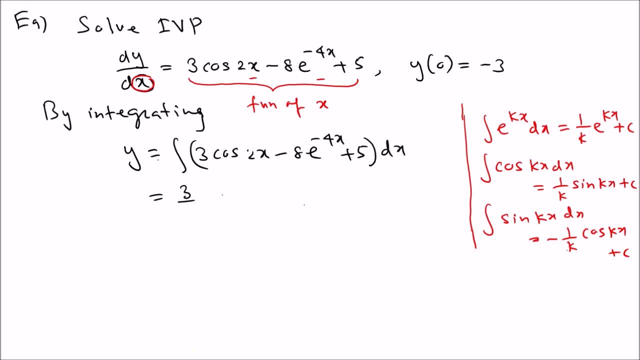 it's a sine 1. so divide by 2, so that means it's going to be 3, halves right. sine 2 x minus, you can see 8. you have to divide by negative 4 e to the negative k. x plus 5 is a constant, so it's a 5x plus c. so that's what you get and you can. 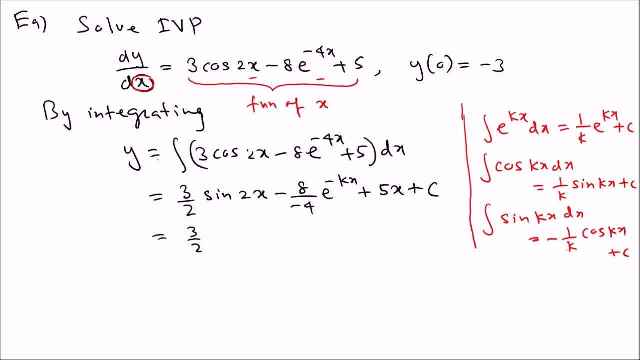 simplify this a little bit. so you're going to get 3 halves assign to x. simplify: you get 2, e to the negative. uh, this, k actually 2.. uh, k actually 4.. so you get 4, uh. so to the 4x. 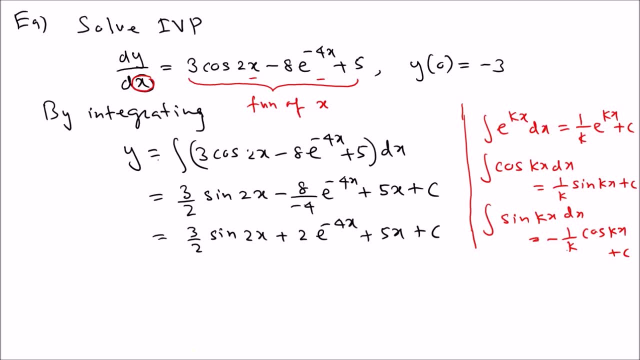 uh plus 5, x plus c. now what we can do is we can use initial con condition. so using the initial condition uh, y 0 equal negative 3, you can see that negative 3 equal y 0. that means, wherever you see the independent variable, plug in 0. you can. 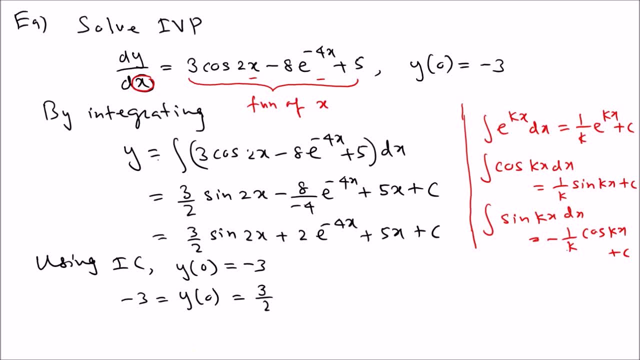 so you're going to get 3 halves sine 0, which is 0 plus 2, e to the 0, which is 1 plus 0 plus c. so you can see that this is 0 and this is 1. so this tells you. this tells you that negative 3 equal. 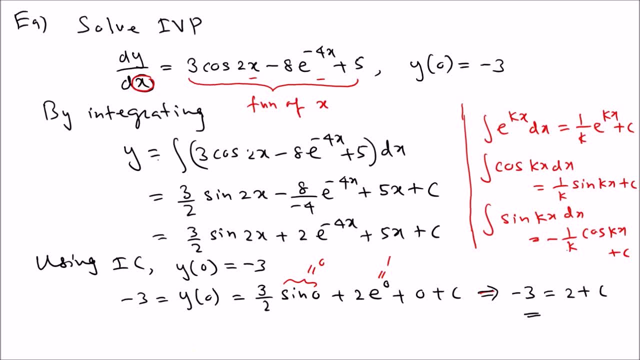 2 plus c, so in other words c equal negative 5. so you can plug in that. so that means the solution is simply: y equal 3 halves sine 2 x plus 2 e to the uh: 4 x plus 5, x minus 5. so that's the solution. 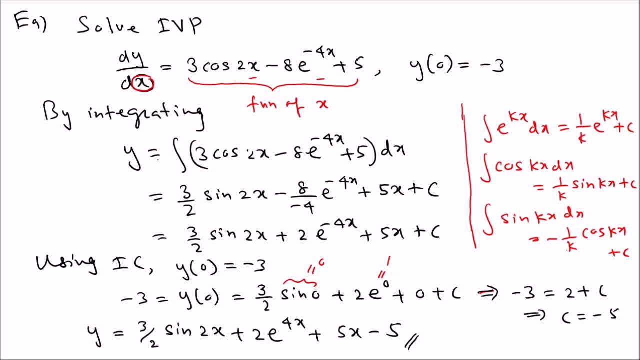 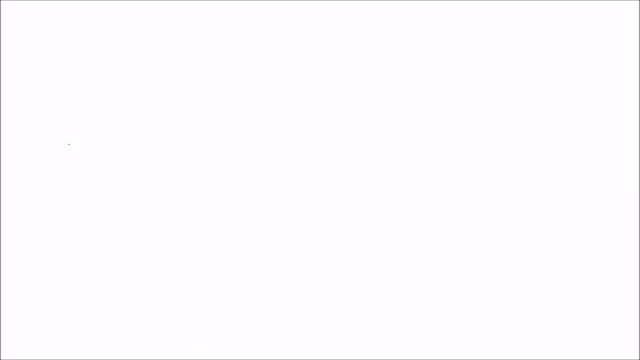 so, so you can see that it's not difficult. uh, we just use the uh basic integration technique because, uh, the right side is just a function of the independent variable. now let's look at the other type. so what's the other one, this example: so we have, let's say, solve the ibp, the initial value problem. 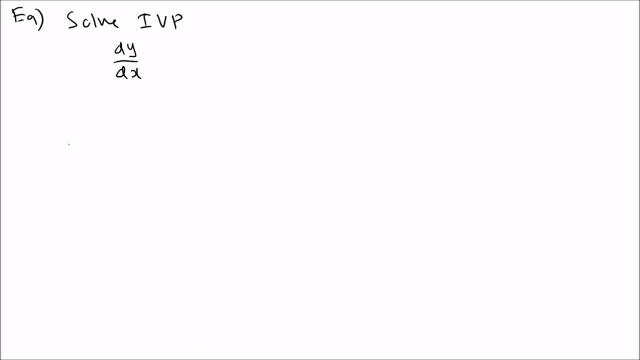 the y over the x, x equal y plus 3, along with y 1 equal negative 2, something like that. so if you see a equation like that, now what we can do, you can see this is a function of the dependent variable. so this is a function of the dependent variable. 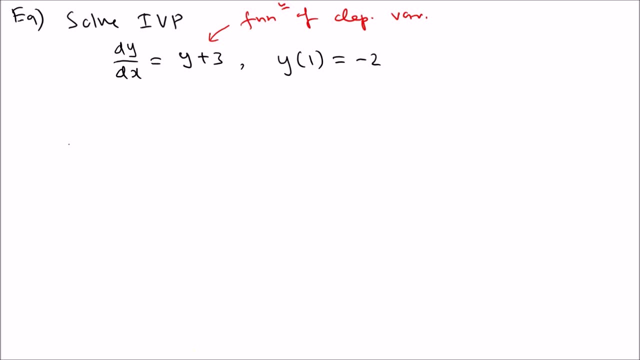 so when you see function dependent variable, what you do, you're going to flip this over. oh, also, you can do, do this problem using the separation of variable. actually, that's the separation of variable, but you can see as a technique, you can remember, like that. so we're going to flip this over, so we 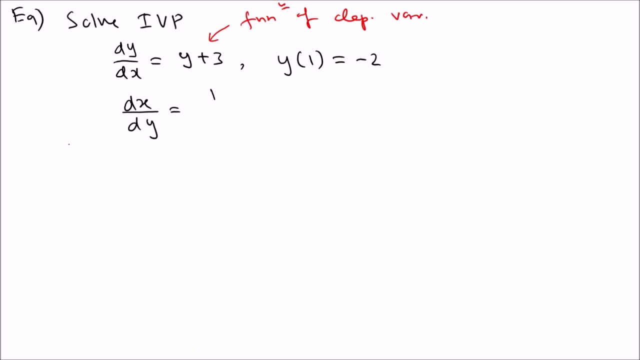 could write this on: dx over dy equal 1 over y plus 3.. now what we can do: integrate with respect to y, so integrate. you can see that we can integrate with respect to y, so integrate with respect to y now. so if you do that, you get x here. 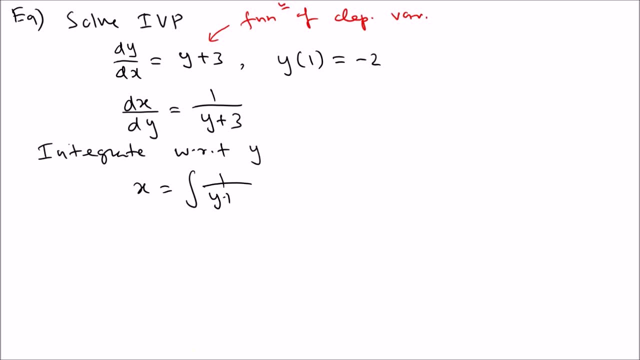 and it's simply the integral of 1 over y plus 3, d, y. so you can see there's a 1 over y plus 3. 3 is just a constant. so this is a log function. so this simply becomes natural log y plus 3.. we are not going to use the substitution here. 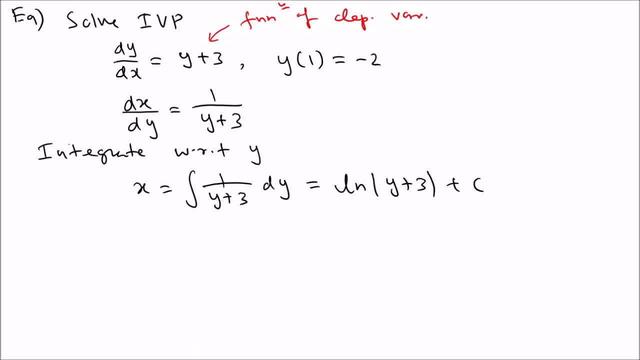 that's like load time ago, okay, so we have the solution now. so we are going to use the substitution here. that's like load time ago, okay, so we have the solution now. so what we're going to do is uh, we can find the uh constant and then uh. so i mean there are two ways to do it. 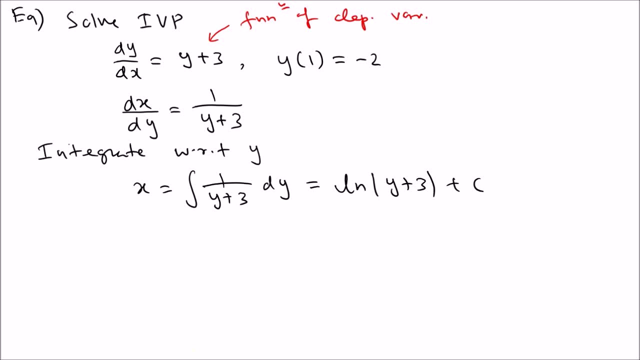 first we can uh solve for y and then plug in the constant, or we can plug in find the constant and then we can solve uh. so so let's do that, so we know the constant, uh, so what it says, that so the using the initial condition, uh. 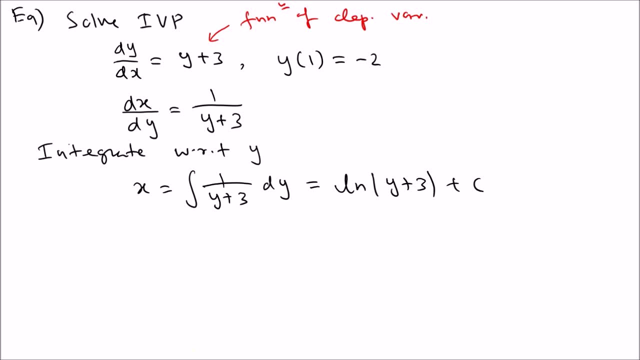 okay. so, uh, there are two ways to do it. either you can use the condition now and then go for the uh, solve for y, or solve for y and then find the constant, so it uh work both. be careful, uh, what do you get? okay, because sometimes, when you try to, 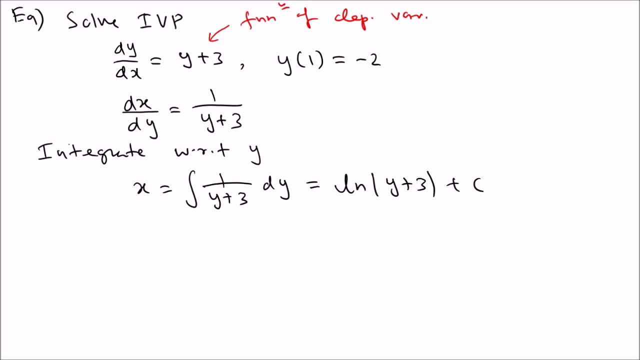 um, write the log form with the exponential form. remember you get plus or minus, so you'll be careful with that, whether, uh, that is the case, so let's solve for y first. remember you get plus or minus, so you'll be careful with that, whether that is the case. 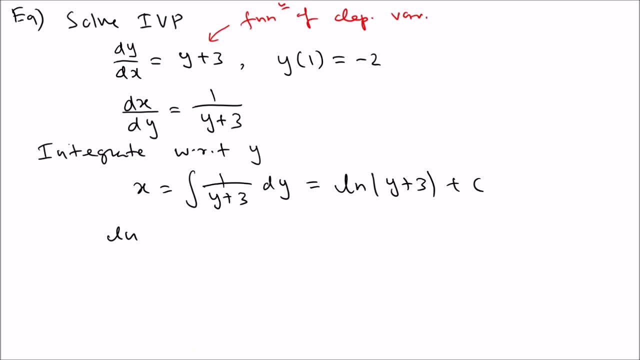 you can write this one as ln. y plus 3, equal x minus c. so this says that y plus 3. we have solved many problems like that, so you can see that this is absolute sign. so that means you're going to get the plus or minus here. so we have. 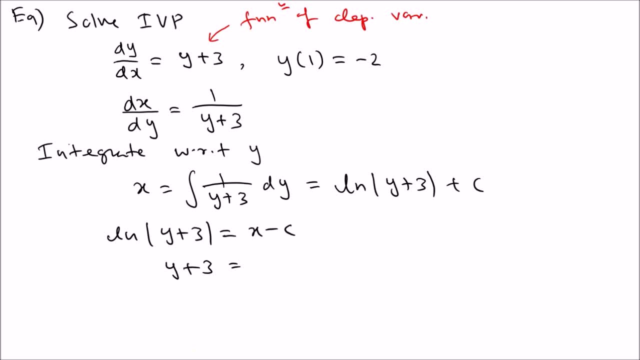 it's a plus or minus. how you can see: uh, e to the x minus c, so uh. so now what we can do, we can write this one as e to the uh, like plus or minus, e to the minus c and then e to the x. what i'm going to do, i'm going to call this whole thing. 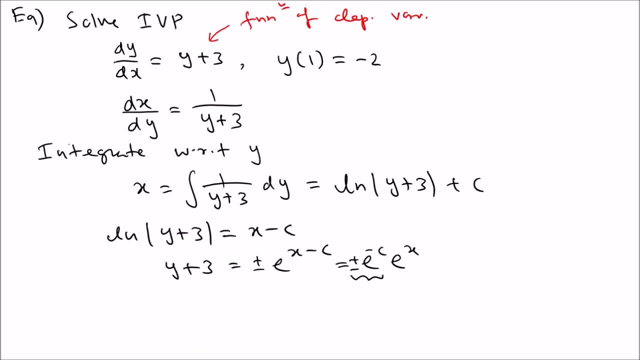 uh e to the x minus c, just a uh c. so if you do that or some other letter, if you want just what we normally call the by abyssal notation, i'm going to call this whole thing just c. not the same c, but another one, okay, like. 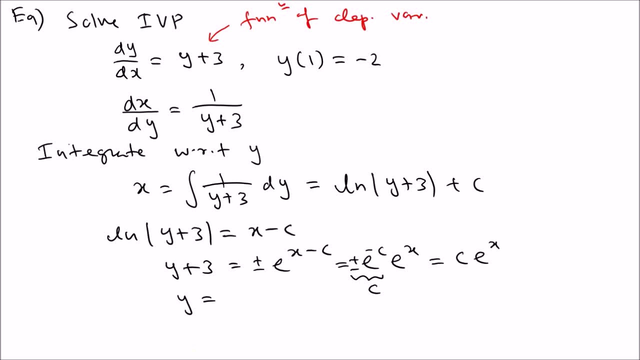 that. so we can write it like that. so, in other words, y equal c, e, x minus 3. now we're going to use the initial condition. so, using the initial condition, we know that, uh, but the initial condition is a negative 2 when you plug in x equal 1.. 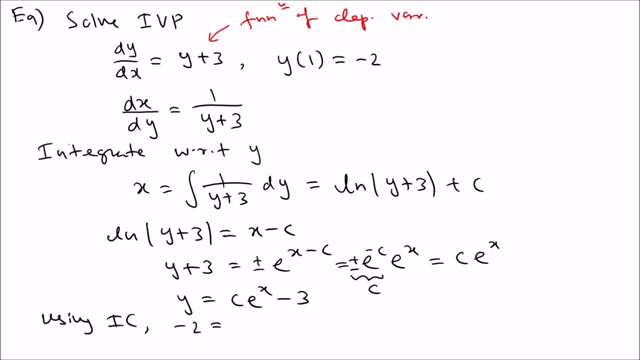 so let's do that. so that means negative 2, y equal, negative 2 equals c, e negative 1, negative 3, and then we can. what we need to do is we need to solve for c. so let's do that. to do that first are: 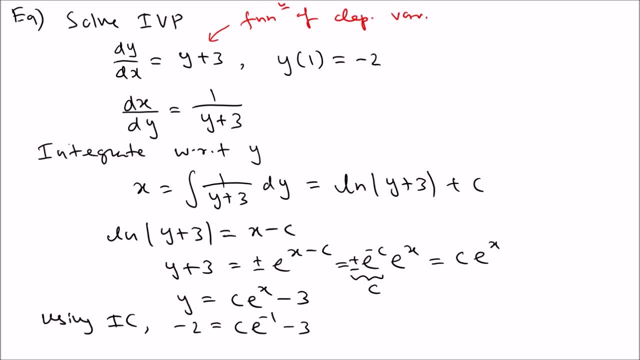 we going to move the number to the other side. that means we're going to add 3 to the both sides. so this says that 1 equal c, e negative 1. in other words, if you multiply both side by e, it says that c equal e. so this is the. 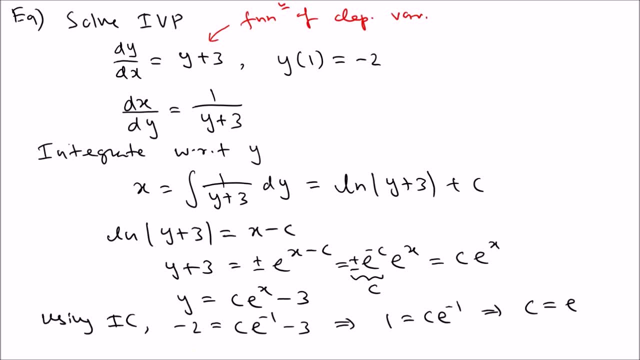 if you plug in c equal e, what's going to happen? y equal e times e to the x minus three. okay, uh, so, and then you can combine them, uh, because e means e to the one. so if you combine that, uh, so you're going to get y equal e, x to the x minus. 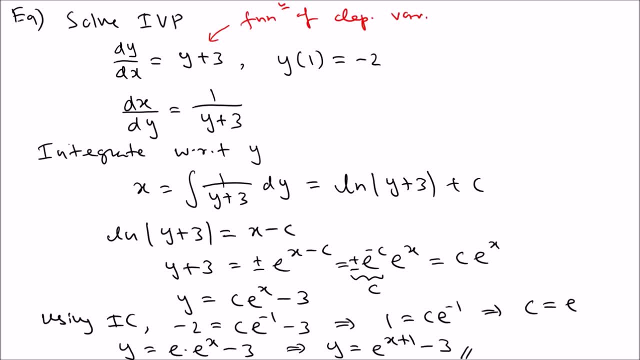 so that is the solution. yeah, i see that there's a small typo here: uh, because uh, we plug in uh negative one, it's not negative, it's positive. so that means there's no negative sign. so that means this is going to be e to the negative 1. so that means this is negative 1. 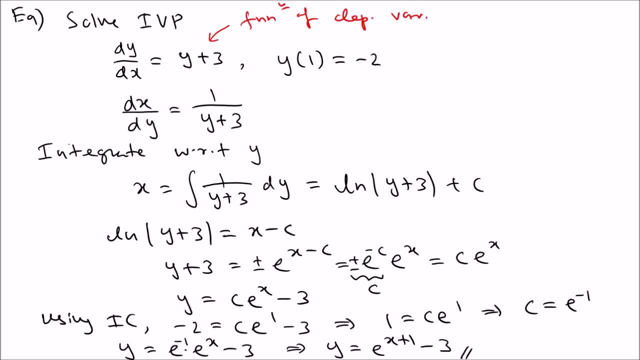 so that means the final answer this is minus 1. good, so that is the solution of the um difference equation, and you can see that that's not that difficult. uh, but there's a process that we need to remember, good, uh. so let's move on. so let's talk about 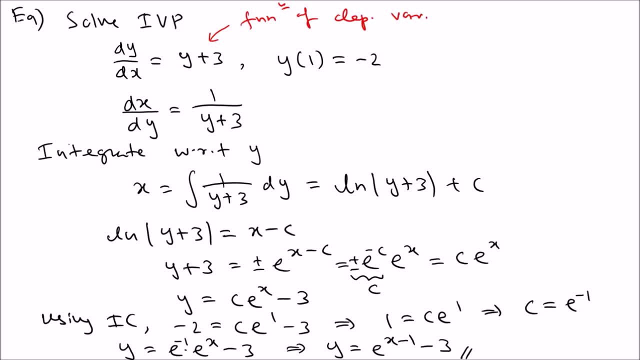 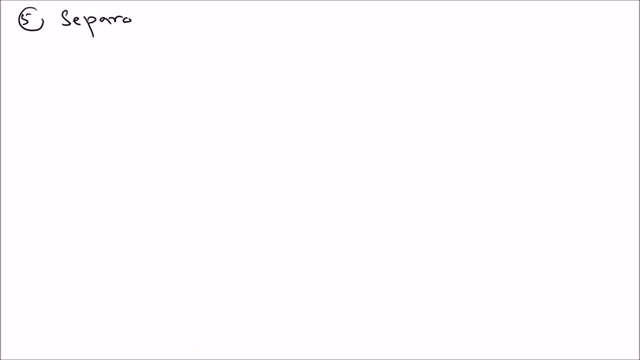 the next major type, uh, so what is the what we call the separable difference equations? so, number five: separable difference. so what is the separable difference equation? separable differential equations. so what's the separable differential equations? so let's look at the differential equation we have: d y over d x. 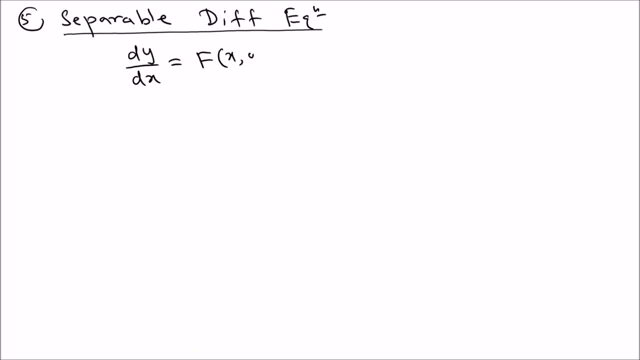 which is a function of x and y. but sometimes what happen? you will be able to separate them into. you will be able to write this fx of functions, a product of function of. so if you can write this one as a product of fx and y, we call it is a separable equation. so this is what we call a. 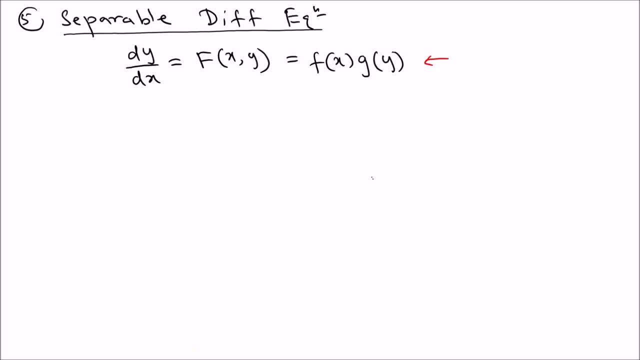 separable difference. if we can do that, we call it a separable differential equation. separable differential equation because you can separate them. okay, and after we do that, what we can do, we can divide both sides by g- y. so if you divide, you can write this one. 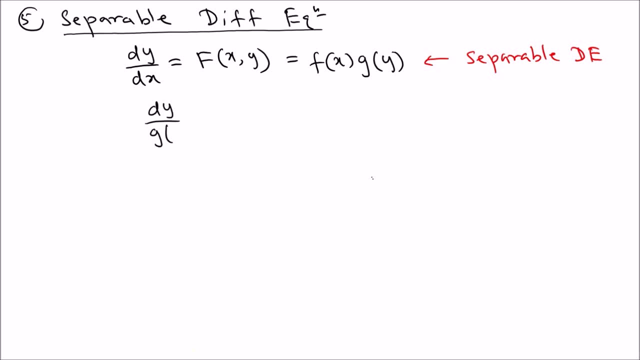 as d y over g y equal. on this side we have fx. we're going to multiply, we're going to bring dx to the other side so we can separate y's and x terms, and then after that, what we can do, we're going to separate, integrate them separately. so that is. 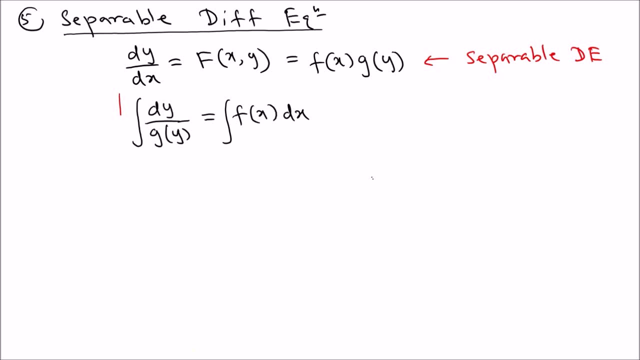 what we call the separable equation formula. okay, so you're going to integrate them separately. okay, very simple argument: we're going to first write as a product, and then we're going to write as a product, and then we're going to move the gy to the other side by dividing. 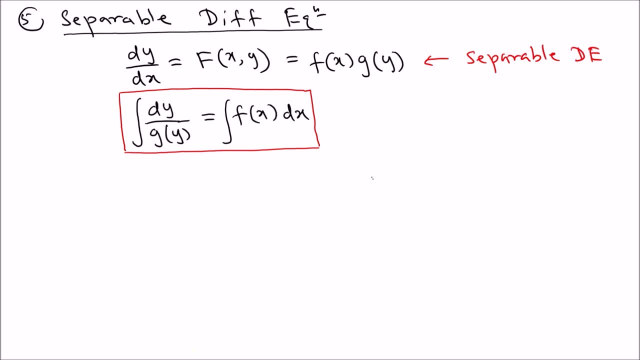 and then integrate the two sides separately. so let's look at some examples. so example: so let's say solve d y over d x doesn't look like x, d y over d x, uh, equal. let's say uh y minus 4 x y. and then we're going to move the 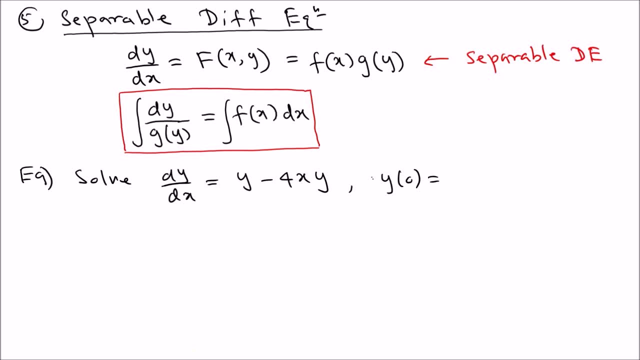 y over d, x, and then y, zero, equal, let's say, e something. so when you get a problem like that, um, you can check whether you can write this as a product of x and y separately. so that's the first step, so the answer, and you can see that yes, you can write. 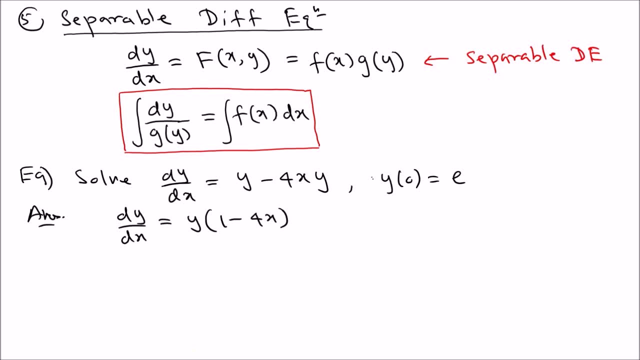 the right hand side. if you pull y out, you can see 1 minus 4x. you can see it's a divide this side by the y function. leave the x function on this side and then integrate with respect to x on that side. integrate this with y on this. 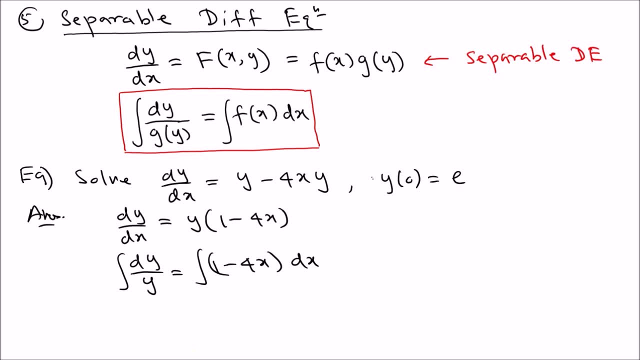 side. so that's the uh magister. now what we're going to do. we're going to integrate the two sides separately, first one with x, right, left side with y, right side with x. so you're going to get ln, uh, absolute y here. this is just a power rule, so you're. 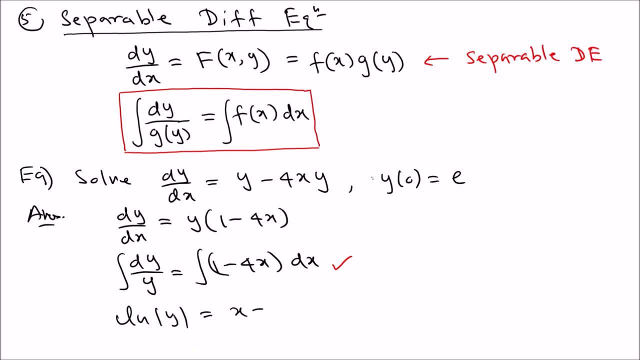 going to get x minus. if you integrate x, you get x squared over 2. so that means we've got 2 x squared plus c. we are not going to add c 1, c 2. we only add 1 c to one side because you. 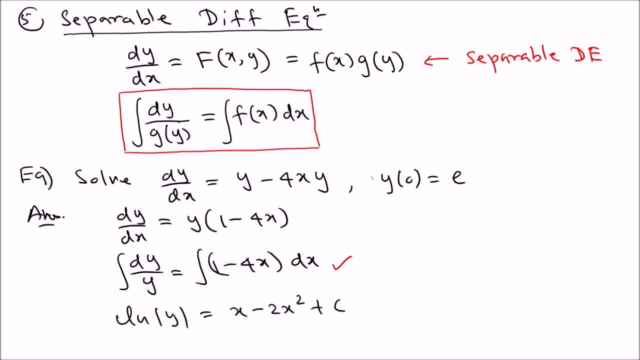 can always simplify. now we can write this one using the exponential form, so so let's do that. so if you write them using the exponential form, i can do it here. then you can see all the work. so if you write the exponential uh form. so what's going to happen is: 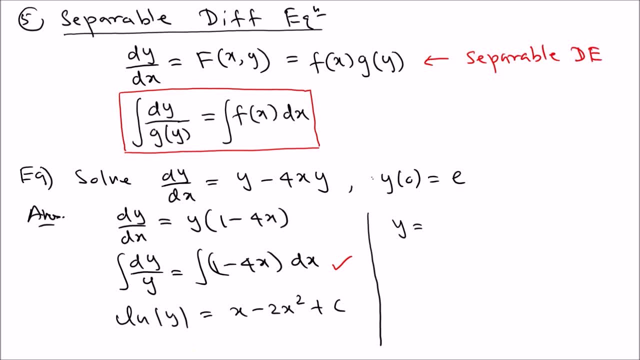 y equal the same thing. we know that's absolute value, so you get plus or minus and then you can just put one constant. so it's the same thing here. so it is. so what happened is plus or minus, and then e to the x is equal to the y to the capital. 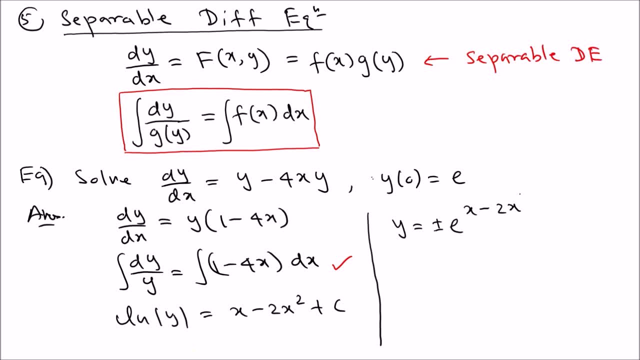 function x squared plus c, and then what we're going to do: the plus or minus, and then e to the c, we're going to combine. so if you, uh, you combine that, let's write that x-ray step. so if you combine that, uh, plus or minus e, and the c, uh, we're going to combine. so that means 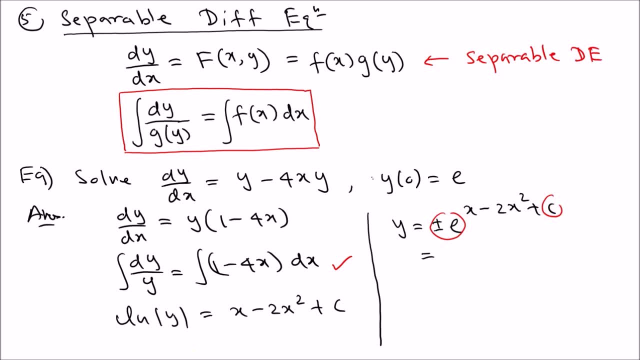 you're gonna, i'm gonna call it a. so if you call that a and then you're gonna get e x minus 2 x squared. we have done this a lot, okay, so that's plus or minus e to the c. you could just call a and we still have e to the x minus 2 x squared. good. 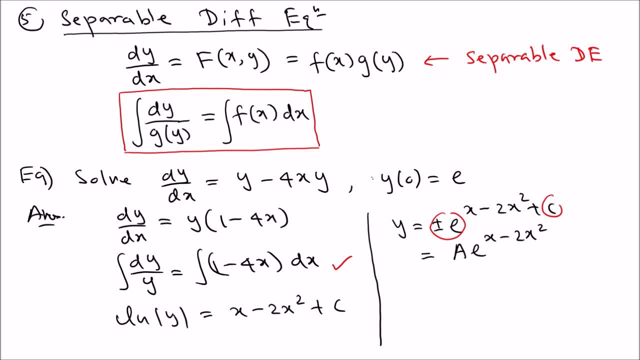 so that's the solution. now, what you can do, we can use initial condition, so the uh, using the initial condition that y 0 equal e, so we're going to get e equal a. so that's the solution. e to the 0, e to the 0 means 1, so that means a. 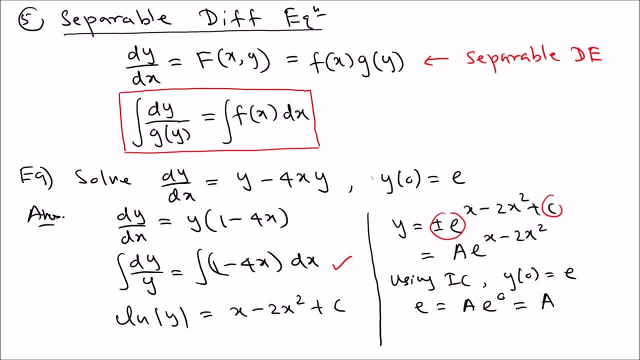 so a equal e. so that means y equal e to the one. ah, we have e x minus 2 x squared. this means thus e to the x minus 2 x squared plus 1. so that is the complete solution. it's not difficult, okay, so that's the solution. 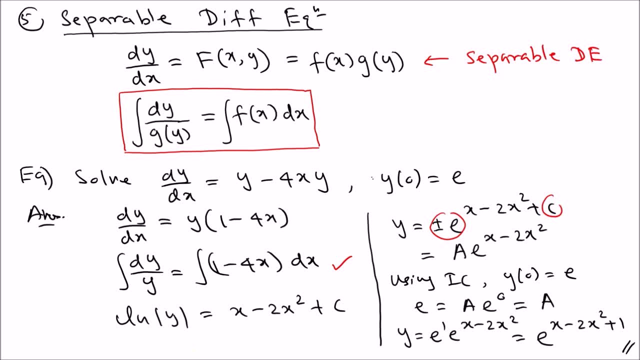 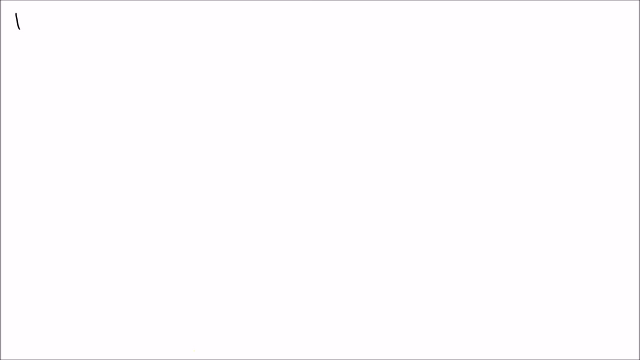 first we find a general solution. that's the general solution, and then we use the initial condition to find the constant. okay, um, let's just do one more example. it is very, very important uh topic. so how about this example? so the next example, let's say solve. 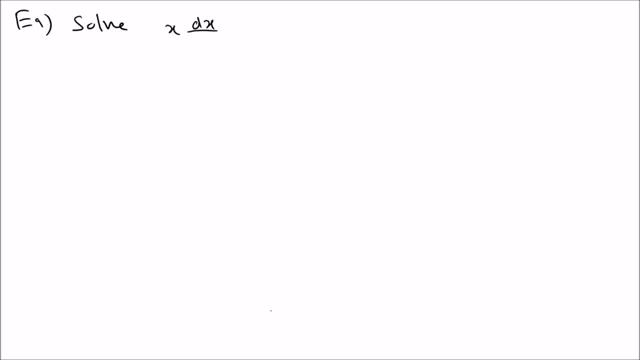 x, dx over dt equal e, 3 e to the t minus x, something like that. so let's try to find the general solution of this one. so what is the independent variable? independent variable is t. you can only switch, uh, flip it and then change that uh, so it doesn't matter. uh, at the end you're gonna get the solution. 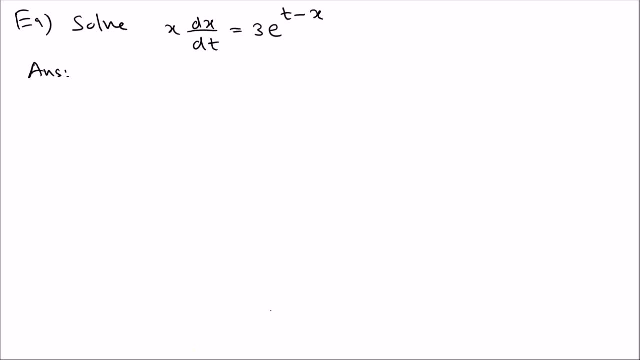 okay, okay, so the answer. so what we're gonna do? uh, we're gonna use a certain algebra here, so we write dx, dx over dt. uh, we can write this one as 3, e to the t times, e to the negative x, so we can do that. 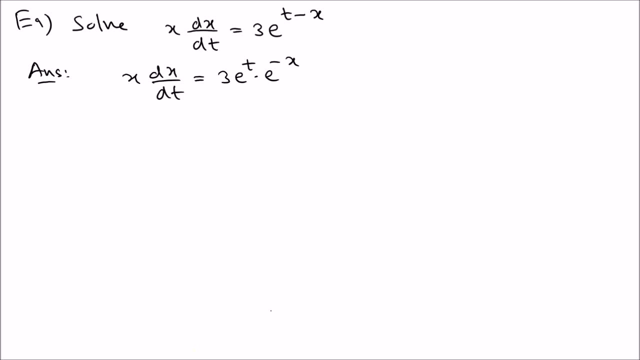 now what we can do. we can multiply. we can see whether we can move x terms to one side, t terms to the other side. actually, we, you can see that, yes, we can do it. if you multiply both sides by e to the x, uh, you're gonna get. 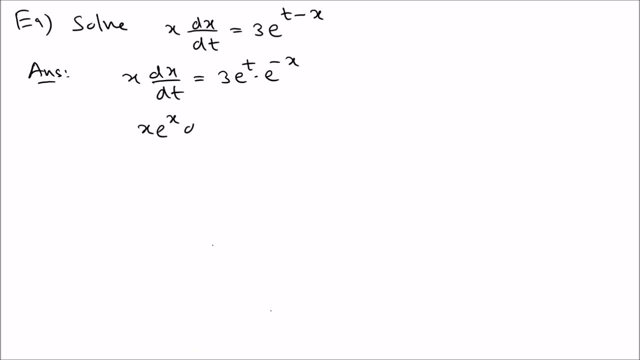 x, e to the x, dx, and then i'm going to leave 3 here, i leave e, t here, and then dt. i'm going to move to the other side so that we can do so. you can see, it is a separable equation now, so we can. 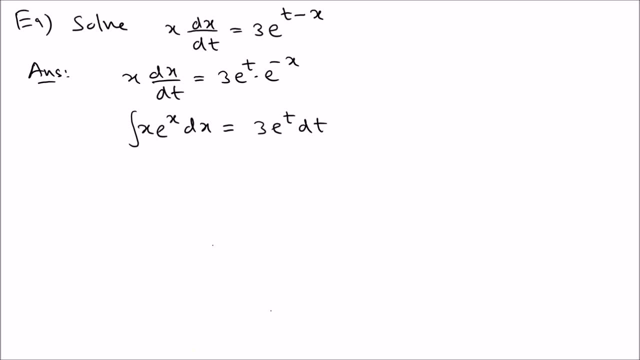 integrate the two sides, uh, separately. uh, right side is okay, how do the left side? for the left side, uh, you have to use the integration by parts, okay, so, uh, so we're gonna make the table, so we're gonna pick u equal x. you can use the shortcut, you can use the. 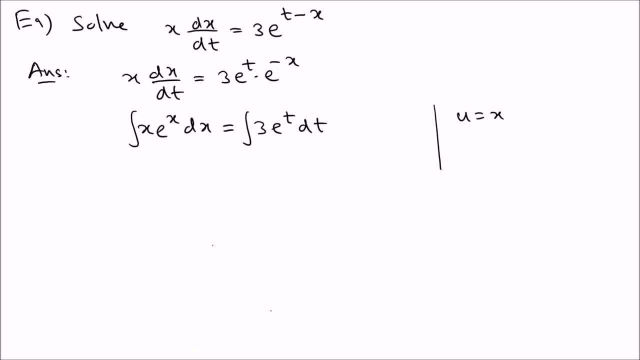 di method. i'm going to just use this regular method, okay, just to make sure that. okay, so dx, dv. so if you are trying to use the shortcut method, the di method makes that you practice that first. okay, so di method and there's a video and that kind of solved many problems there so you can practice. 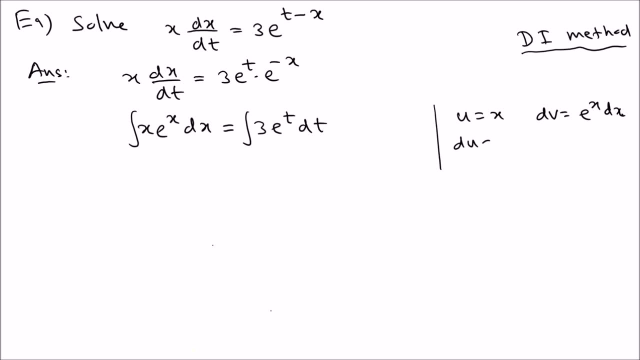 using that, okay. and then we take the derivative here, so it is du equal dx, and then you have the integration by parts formula. so you have to integrate, so you get ex. and then what is the integration by parts formula? it is: udv is simply equals to uv. 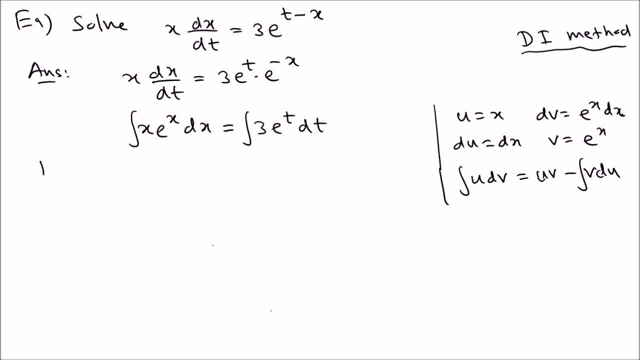 uh minus vdu. so that is the integral by parts formula. so we can use that. so by the integration by parts formula on this side you simply get uh uv. that means x, e, x minus d. u means dx. equal here 3 e to the t plus c we add: 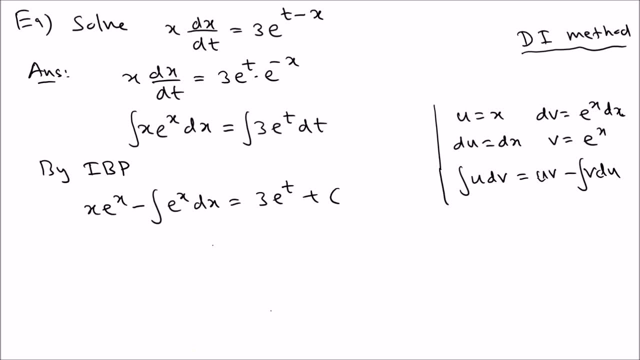 only c, one side, uh. and then we can finish the integral here. so we get x, e, x minus e, x equal 3, e, t plus c, uh. so the question is: can you solve this for x? x is the dependent variable, can you? um, because of that x term we cannot. 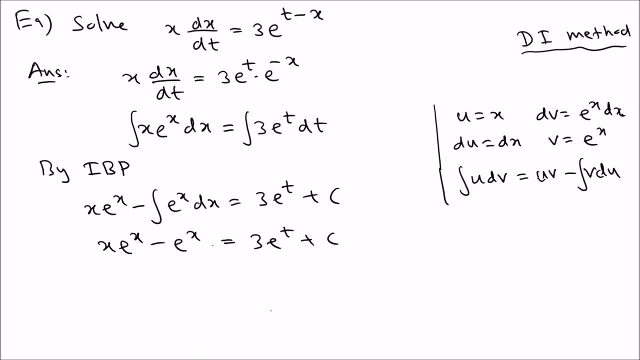 uh, because there's no way you can pull the x term out, because when you have sine cosine exponential log, um like that, there's no way you can pull the x term out. when you have a product like that, it's a non-linear. okay, so this makes it non-linear, so we cannot. so we can leave it like that. 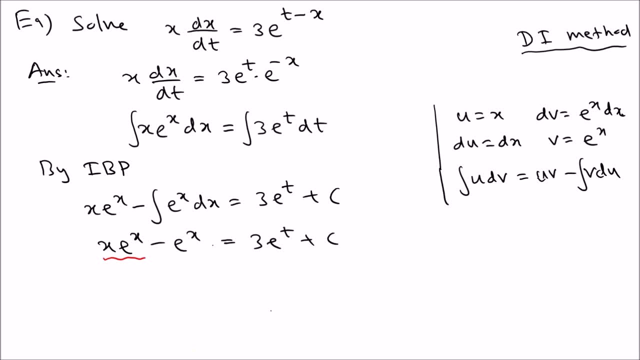 so this implicit solution, so this is the implicit solution, so this is the implicit solution. so implicit solution of x: and if you have initial conditions, what you can do is you can plug in them and then solve for c, but otherwise you just have to leave it like that, because that's not how you can. 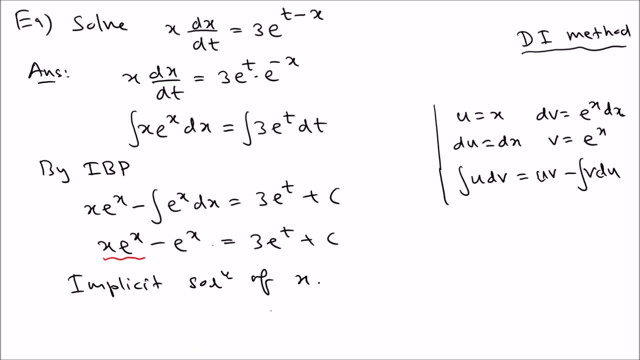 solve this, but that's the implicit solution for the x function. very good, okay. so let's talk about the next important type. uh, that is the first order. uh, linear differential equations and we're gonna use the integral equations. that's the next major topic. okay, you always have questions in the 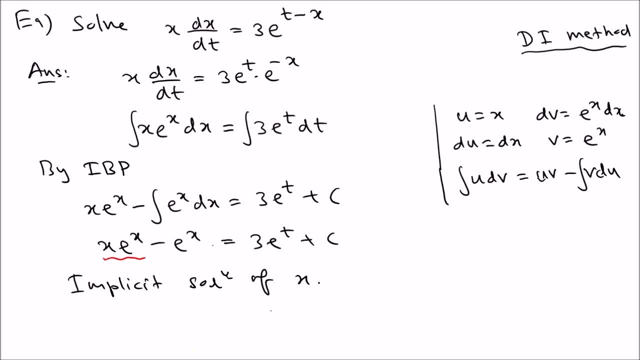 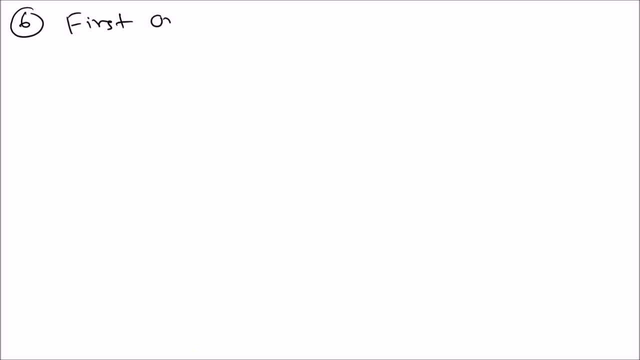 exams. good, uh, so let's talk about that now. uh, so the next topic. this is uh six, number six. so this is first order, first order linear. first order linear: uh, differential equations. you have to remember, like that, first order linear. so we use the integrating factor method. 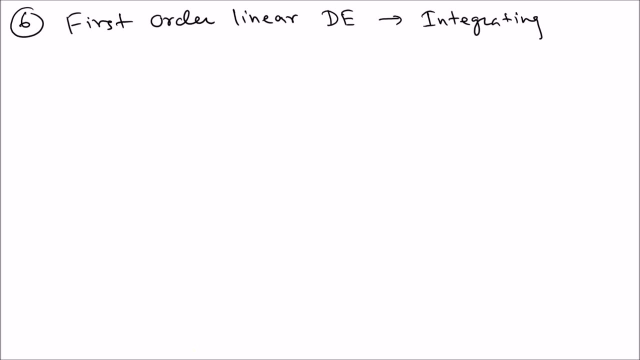 integrating fact indicating factor method, uh. so let's talk about the uh. let's recall what we did. so we write what we call the standard form. so it has to be of this form. if it is not, you have to be of this form. you have to bring it to this form before we do anything. 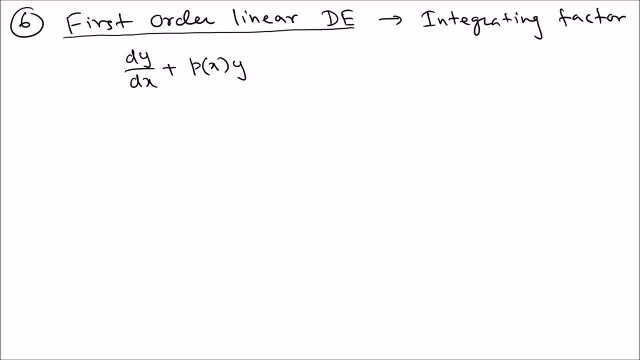 and then dy over dx plus pxy equal qx. so that's the kind of format for the first order, linear. this is what we call the standard form, standard form, standard uh form, uh and then. so if it is not in the standard form you have to bring into the standard form first. okay, 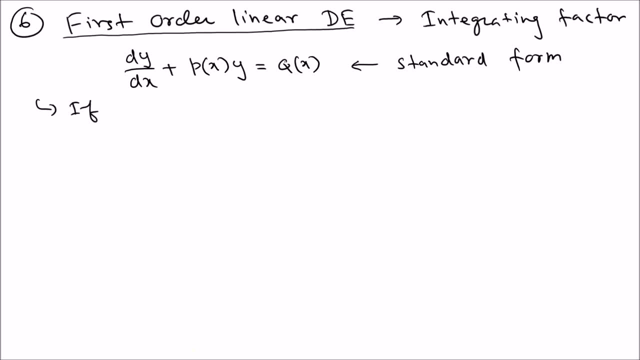 so, if not, if not, uh bring it to standard form. that's the first step. bring it, uh, bring it to, uh, bring it into the standard form, and if you don't do that, your answer is wrong. okay, so it's very careful, you have to bring it to the standard form. 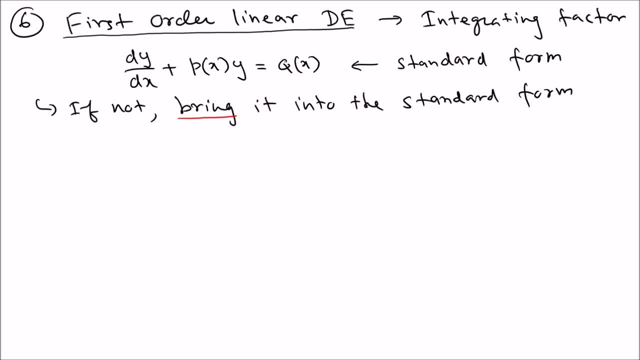 good, so let's talk about the uh standard form, uh, steps, uh, so what are the steps of such a problem? so the first step is: so, so we assume that it's in the standard form. okay, that's the standard form. so we assume, uh, this is the case. uh, now what we can do. 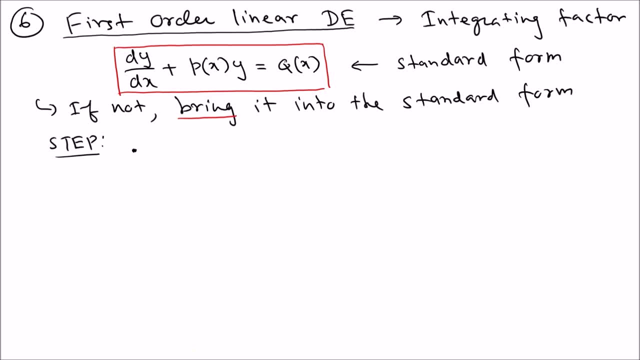 uh, we can find what we call the integrating factor. okay, so, find the integrating factor i, which is always e to the px, dx. p means everything you're gonna with with the sign. so we're gonna uh calculate that. after that, what we're gonna do, are we gonna multiply? 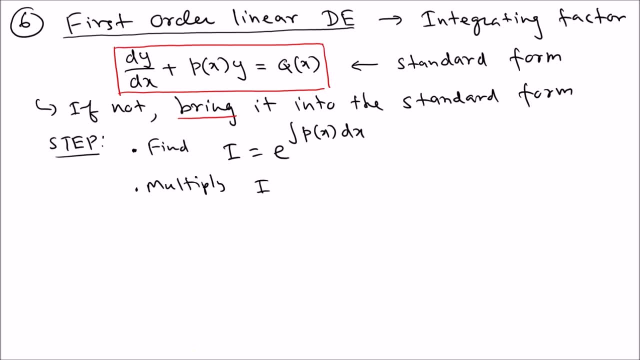 we're gonna multiply the whole equation by that, so we can write i x times the d, y, d, x plus p, x, i x times y. on the other side we have q x times i. now the magic happens. what's the magic? you can see that on the left side. 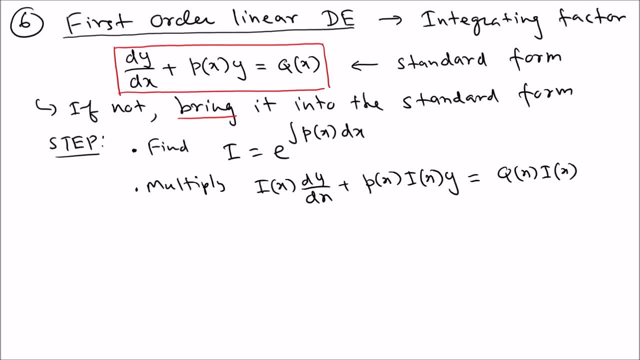 this is automatically the product rule for the product y and i, so we can write the form. that's what what we normally call the form, so what the form here is. automatically this side becomes the product of y and i. that's automatic. that's the product. if you apply the product rule, that's what you get. and on: 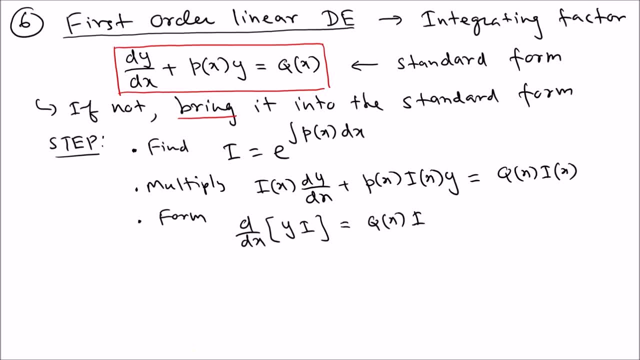 the other side. now we have q, x and i. now what we're going to do is we're going to remove the derivative. we can integrate both sides so you can integrate and once we integrate, what's going to happen? you get y i term on this side. this is just the integral. 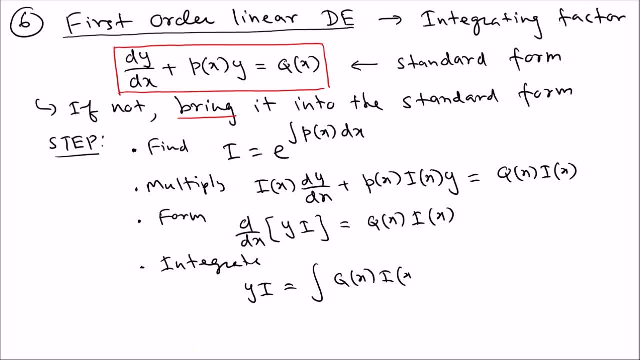 q, x, i, x. so you can see this is a function of x. it may or may not be able to integrate. if you cannot, we leave the with the integral sign dx, and we can exaggerate the plus sign. now what we can do, so you divide by i, so that means y- is simply: you're going to divide by. 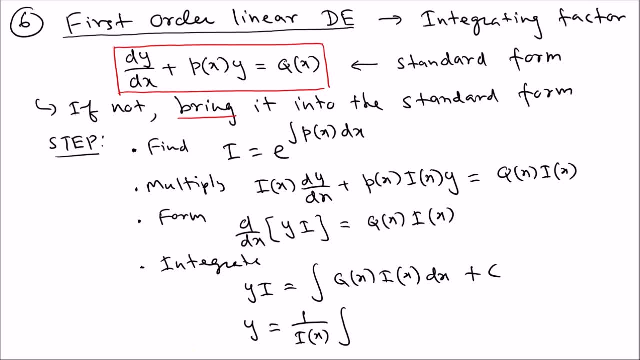 item. so you're going to get the bracket. so so we have inside that we have qx, i, x, d, x plus c. so those are the steps. um, so let's try to don't remember this as a formula, just just because it's much easier to uh, follow these steps and 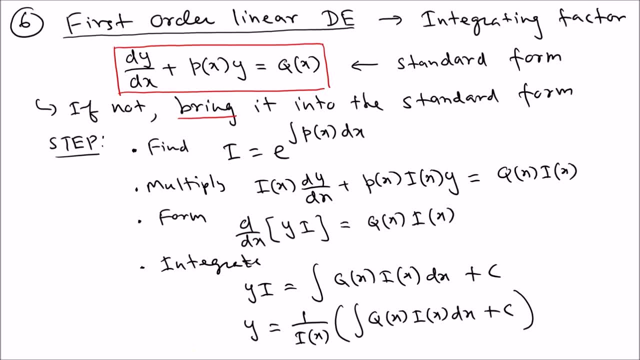 i'll get this uh quickly. uh, that's exactly the whole point of learning these things. okay, plug into equations, anybody can do that uh. so it'd be better to like kind of follow the steps and get that. um good, so let's do uh, maybe two examples from, uh the topic. this is very important, so i'm going to. 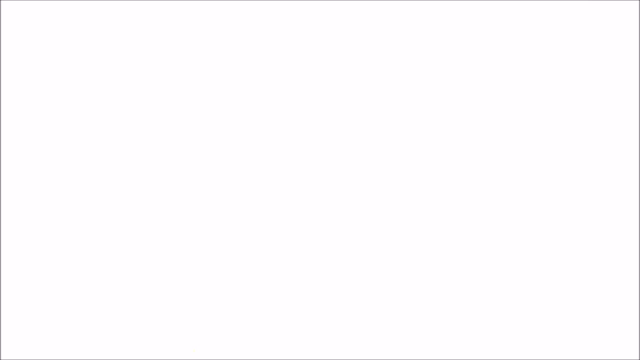 two examples. the first example. so example number one: so let's say we have d y over d x minus 3y, equal e to the 3x sine 4x y, 0, equal negative one-fourth. so the answer. so you can see that this is a first order linear difference. you can see the. 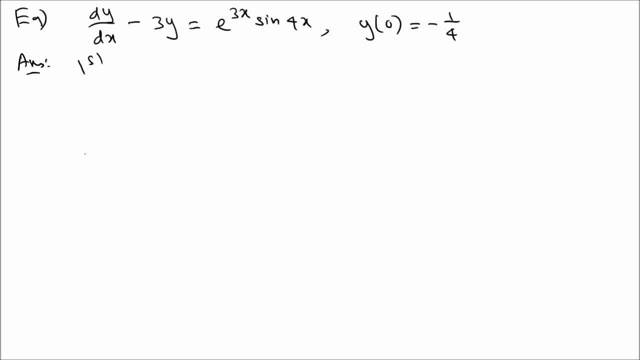 right form. okay, so this is first order. uh, linear, uh equation. so that means we're gonna use the. you can see the original separable equation. you can separate x and y um so we can use the indicating factor method. so let's go step by step. so we're going to find the indicating factor. 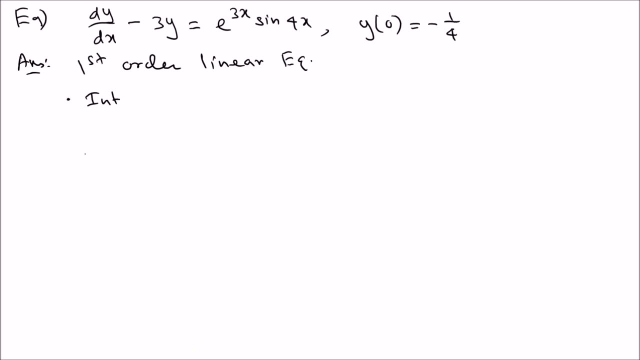 uh, integrating factor. so we're going to say i, which is e to the px, dx. so let's plug in here e to the uh. what is the px? you can see, px is with the sign negative 3. that's the p. so it is negative 3. dx, negative 3. you can pull out so that. 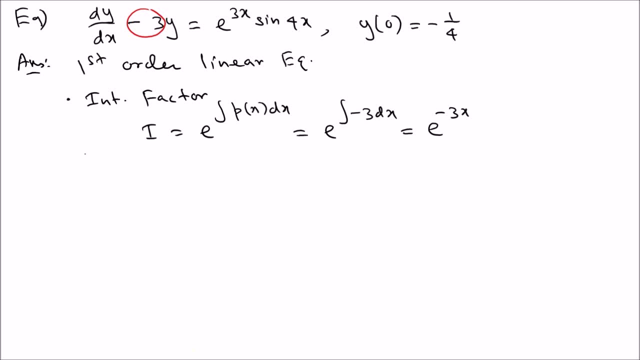 means it's going to be e to the negative 3x. we are not going to at the c, uh, because we are looking for one solution that all this moves. now, what we can do, we can multiply, uh, so so you can multiply the whole equation by that. so it is e to the 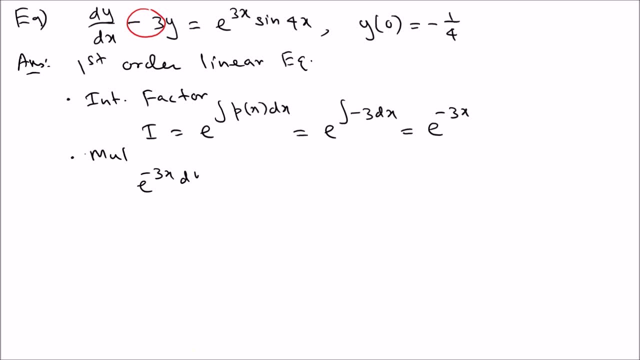 negative 3 x, d y over, dx minus um. you have three e to the negative 3x. what we get from the other side it is e to the negative 3x, e to the 3x sine 4x. you can see it simplifies very well, okay. so that means, if you simplify properly, 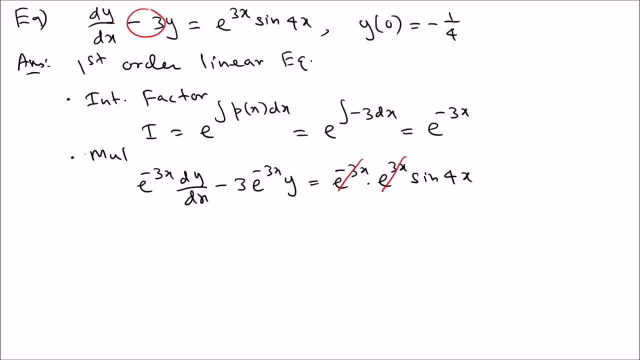 it can work very well. so you're going to get the sine 4x. okay, that's the gift you get if you did that. right, it simplifies very well. good, so that's the gift you get if you did that. now we know that this is automatically. uh, this side is, so we can write the form. 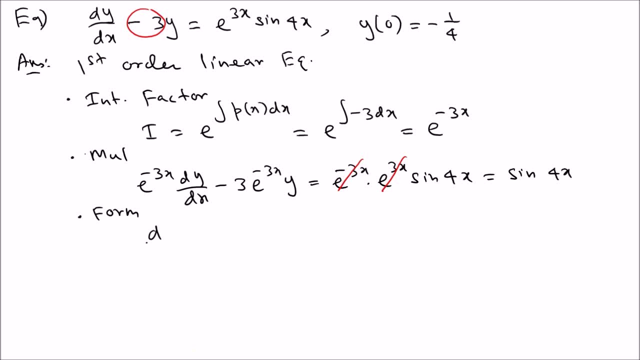 so this is automatically the derivative of the y and the integrating factor. so that is automatic thing. on the other side we have sine 4x to remove the derivative. we can integrate. so integrate with respect to the derivative, with respect to x, x is the independent variable. 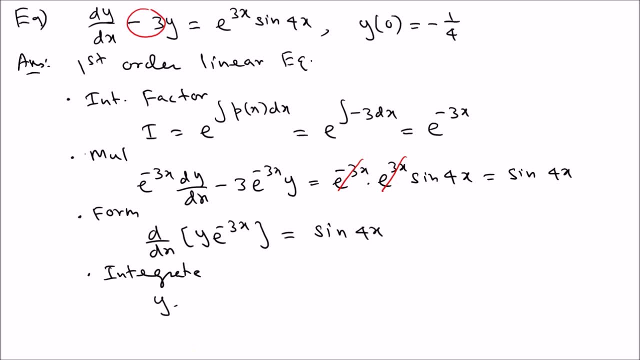 so that's going to cancel out. so you simply get y, e to the negative, 3x, the integral of sine, 4x, dx. this is very easy to integrate. uh, k equal four, so you can divide by that. this is sine, so it's a negative cosine. 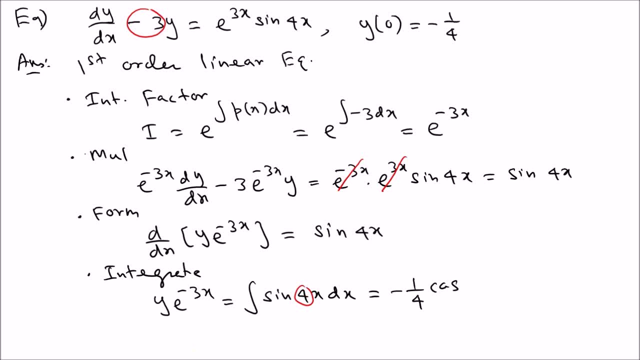 so this can be negative one fourth: cosine 4x plus c. don't forget that you can do. we're going to multiply both sides by e to the three x. so if you multiply by e to the three x, both sides, so you're going to get negative one fourth. 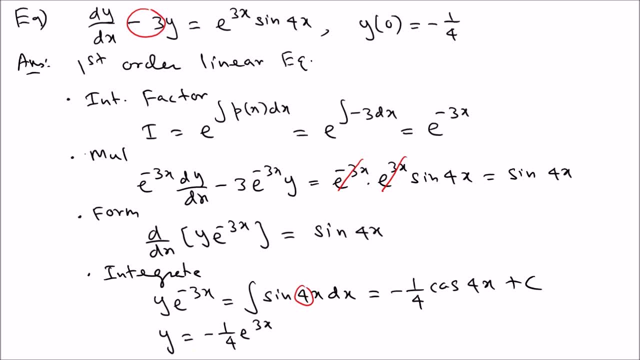 e to the three x. when you multiply e to the three x is the opposite sine. okay, so it's a negative three. you multiply by positive three, so so that they're going to cancel on the left side. on the other side, you multiply by e to the 3x, so you're going to get that. 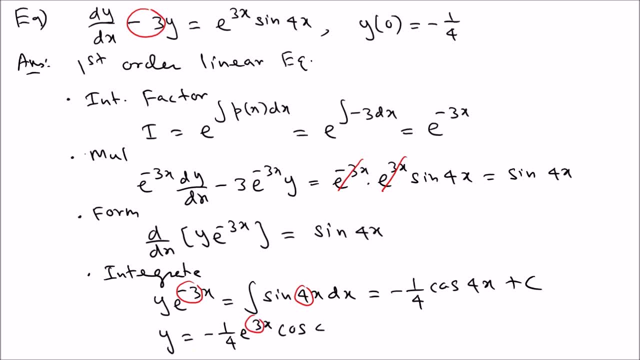 times cosine 4x plus c, e to the e knight plus e sizable. so that is the solution. that's a general solution. okay, so this is the uh general solution. now what we're going to do, since we know the initial condition, uh, let's plug in that and try to find c. otherwise, this is the solution. 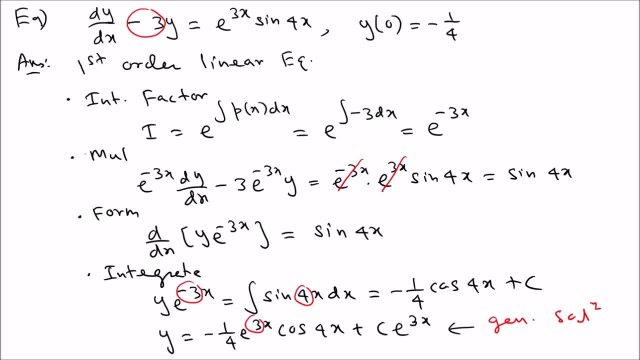 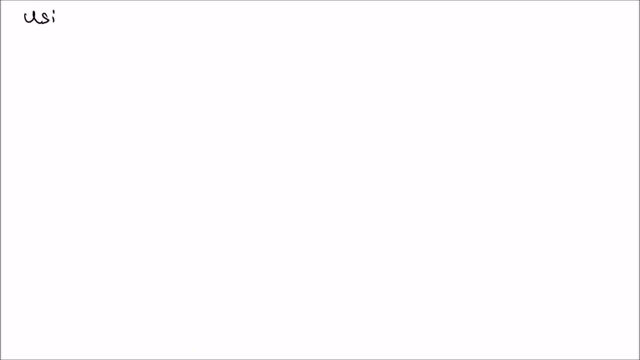 so if i need to find general solution, we done okay. so let's next step is we can use the initial condition and to solve it. so, using the initial condition, using the initial condition, y 0 equal negative 1, 4- you're going to get negative 1: 4, which 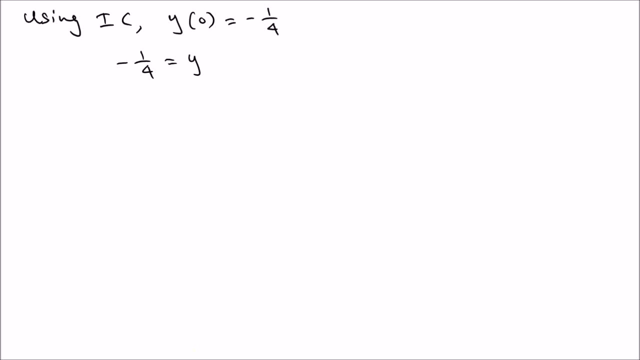 is simply equals to y, 0. this is negative 1. 4, where you see uh, x, put 0, so e to the 0 cosine, 0 plus c, e to the 0, ah, which simplifies to negative one. fourth, because we know that the cosine 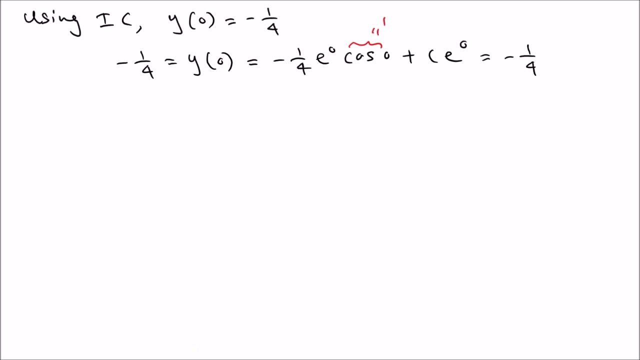 is one, and then we gonna apply the negative. this is also 1, so you're going to get negative 1, 4 plus c. uh, you can see negative plus 1, 4. negative 1, 4, cancel. so this is that c equals 0, so that means that term is gone. 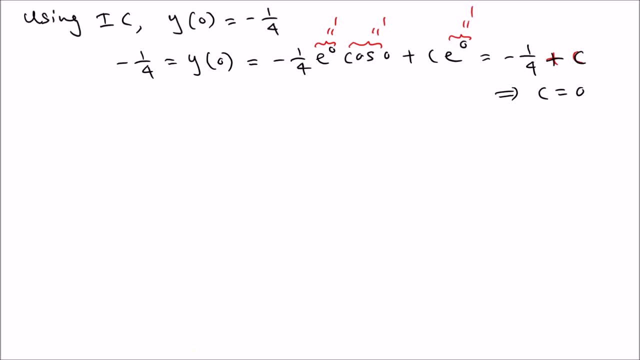 so you simply end up with y equal negative 1, 4 e to the 3x cosine 4x as the solution to the initial value problem. good, uh, so let's try to solve, uh, one more of that, because this is very important. so i'm going to do one more. 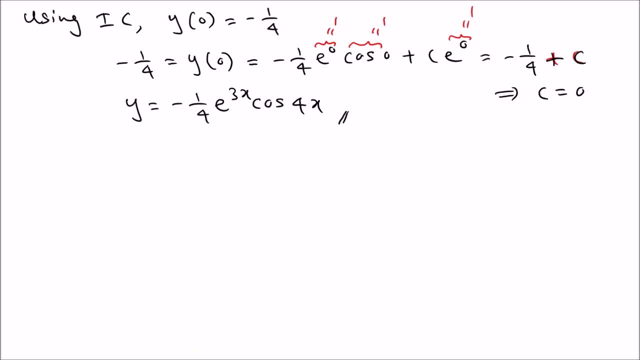 so then, as the next example, let's try this for the example uh, solve. let's say that we have a solution. let's say t d y over d t minus 2 y t, cube e to the negative 2 t. okay, okay, um. is this in the standard form? 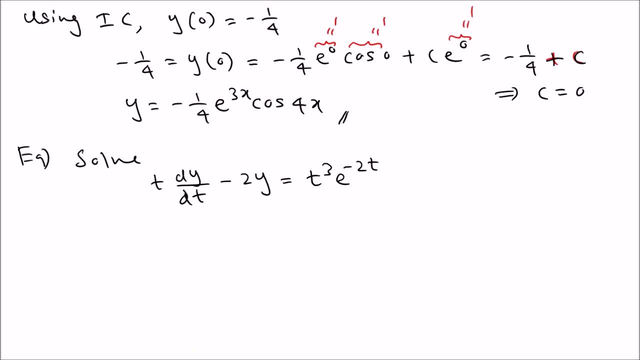 so that's the first question you want to ask. okay, first question: you want to ask whether this is separable. okay, that's much easier. actually, that's not the first. first question is whether this is the basic integration problem. this is like d y over dt: equal function of. 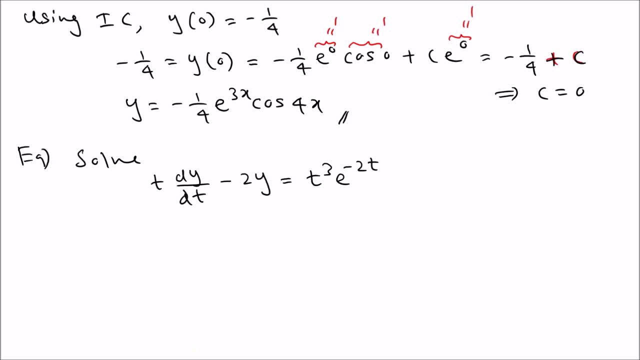 the independent variable only or function of the dependent variable only? and you can see that no, it's none of them, so it's not basic- and then ask whether this is a separable difference equation. can you separate the x term? can you separate the y terms and t terms? 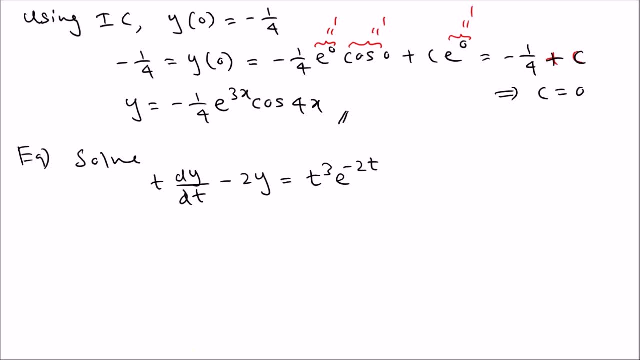 and you can see that there's a sum and also there's a multiplication. there's no common term, so this is not separable. and then we're going to go for the linear. first of all, the integrating factor method. so when you go into any factor method, you ask the question, can you? 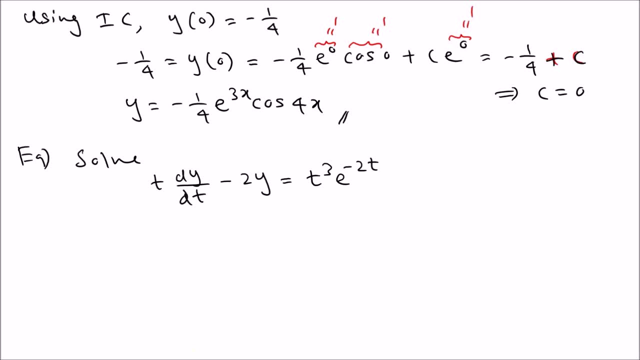 is this in the standard form? and you can see that this is not in the standard form. so what are you going to do? you have to bring it to standard form. so how to do that? you're going to divide by t, so, because you don't need that term. so that's the. 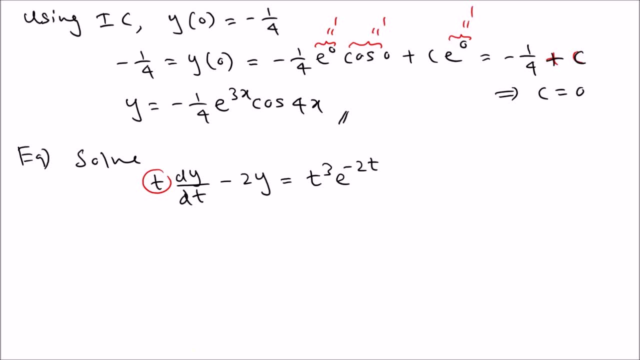 only problem. so we're going to divide the by that first. so let's do it. so we divide the whole equation by t. so that's the first step to do. okay, so we can write: uh, not in standard form, not in standard form, not in standard form. 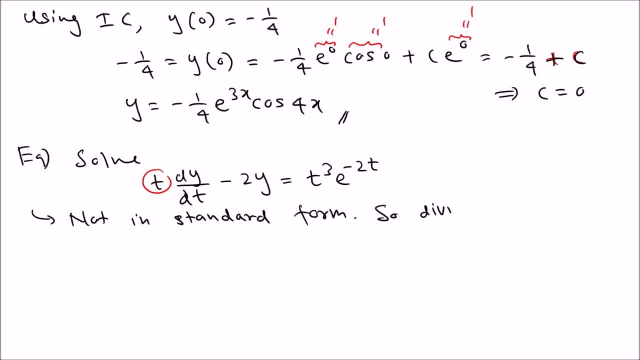 ah, so i divide by by that t term. ah, so you're going to get d y. you're going to get d y over d, t minus 2 over t y equal. this become t squared e to the negative 2t. okay, now, this is standard form. everything looks good. now what do you? 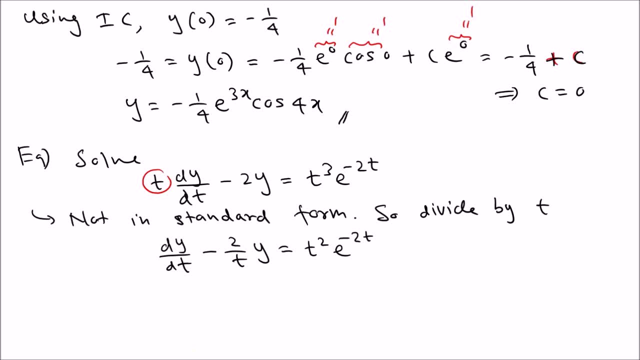 want to do: find the integrating factor. so let's do that. uh. so the first thing we will divide, okay? so, uh, find integrating factor, integrating factor. so which is i equal e to the integral of p t? now, p t d t, so it is e to the integral of p t, which. 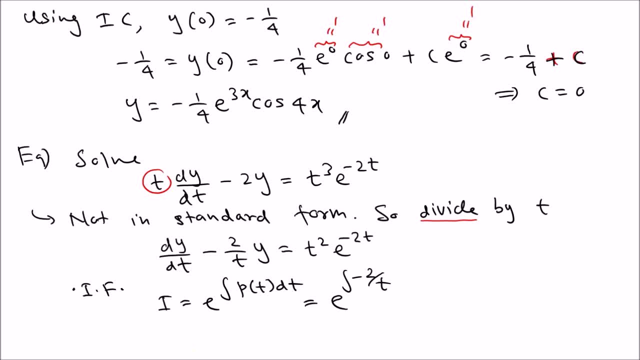 is negative: 2 over t. you have to pick the whole thing, okay. d? t. this is very easy to integrate. we normally do pull the negative t out. this is 1 over t, dt. 1 over t means ln. that means e. to the negative 2, l n. 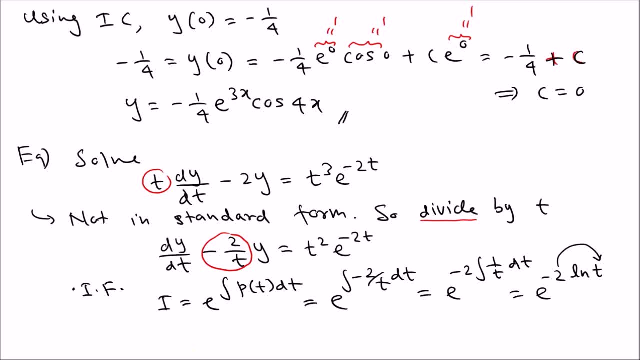 t. we're going to bring this as a power, so that means we can write this one as e to the ln t negative 2. now from algebra, this part get cancelled, okay, so you're gonna get t e to the negative 2, or in other words, one over. 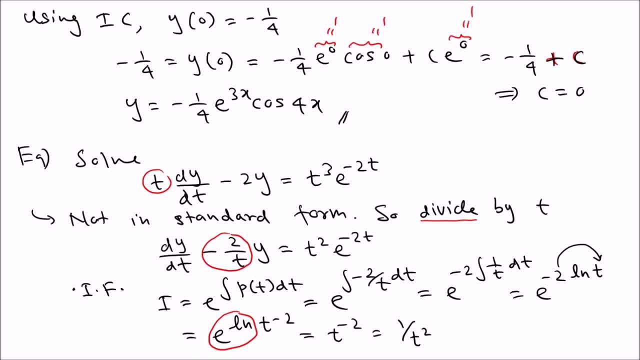 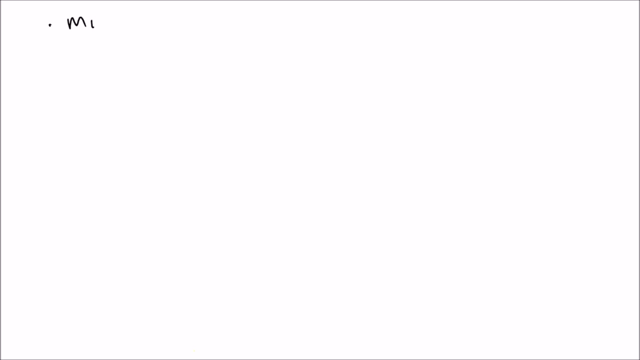 it doesn't matter which formula. so that is the integrating factor. now what we gonna do? we're gonna multiply the, the equation, our standard form equation, using by the integrating factor. so let's do that. ah, so when you do that, so we're gonna multiply by uh 1 over t, squared, the whole equation. 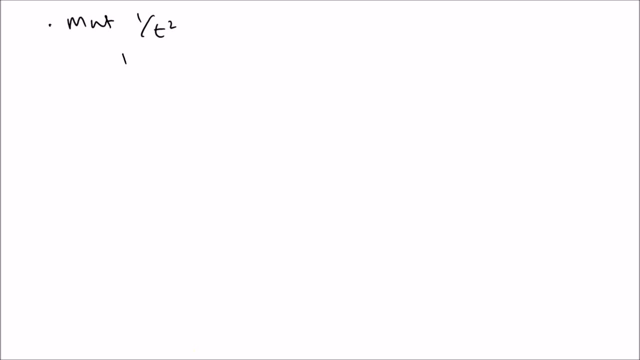 so you're going to get 1 over t squared, dy over dt minus. it's going to be t cube now y equal what happened here? it is 1 over t squared. you what you have here you have t cube e to the negative 2 t, so you can see this get cancels. very well. 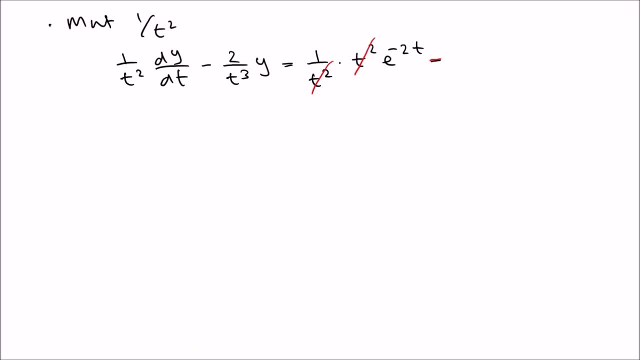 ah, and then you can see that you can get e to the negative 2 t. so then we can write the form so that this side is automatically uh become the uh. so we write the form so this side automatically become d over dt y times the integrating factor. 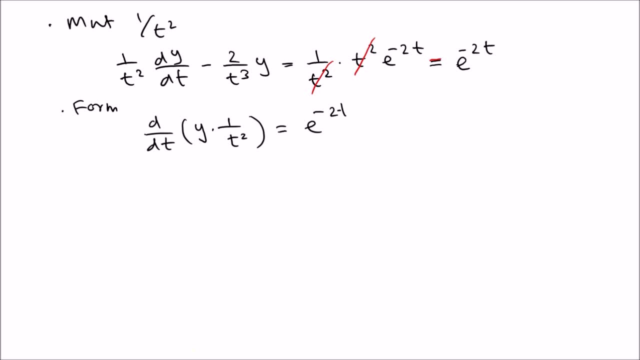 other side is e to the negative 2 t. we can integrate this now. if we integrate, you get y uh times 1 over t squared. this is the integral of e to the negative 2 t, dt. this is a very simple integral. you're going to divide by 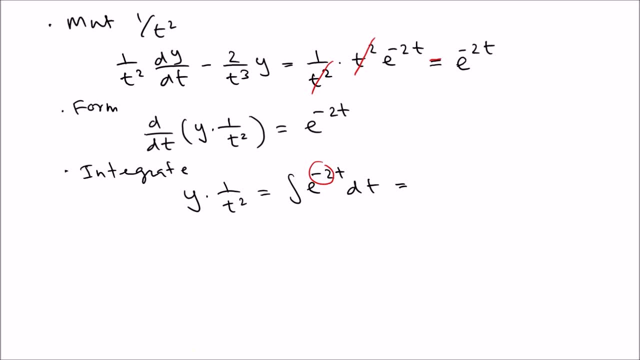 the constant. so that means it is negative one half e to the negative 2 t plus c. now what we're going to do? uh, we're going to multiply both sides by t squared, okay, so multiply 2 t by t squared to cancel that. so we're going to get y. 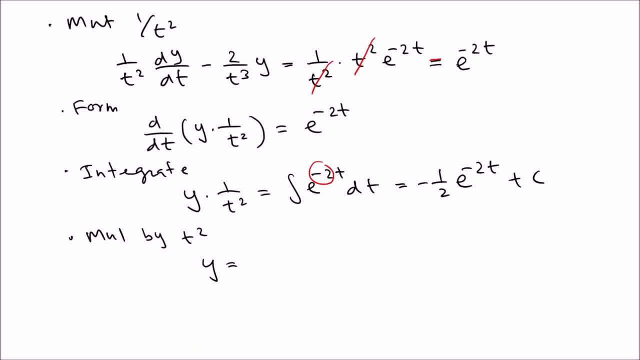 equal. you're simply going to multiply by t squared. so you're going to get negative one, half t squared, e to the negative, 2 t plus c t squared. so if you know the initial conditions, uh, we can find a c okay. so if the initial conditions are the initial conditions, are the initial conditions of. 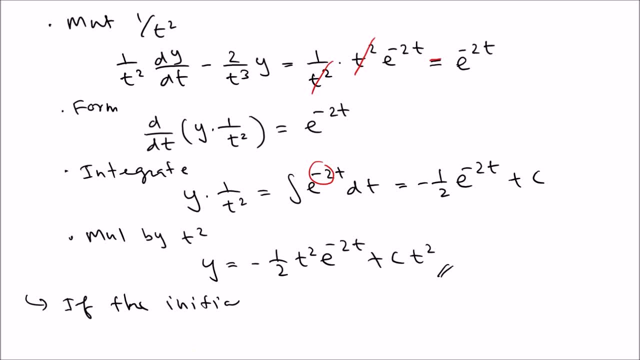 the initial conditions are given. if the initial conditions are given, we can find c. so that's the idea, uh, of using uh the integrated factor method. so you can see that it's not that difficult, but there are certain steps that you need to uh follow. so here, what we did was we: 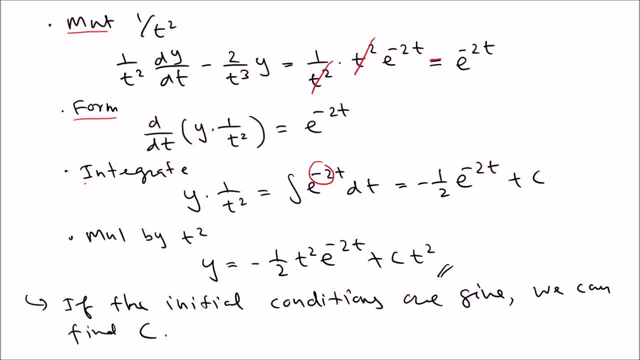 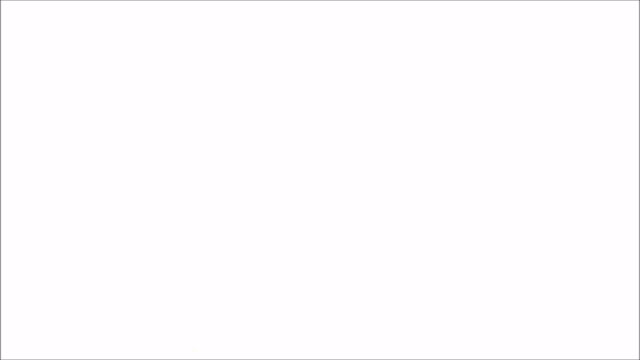 multiplied by 1 or t squared, and we write the form integrate and multiply again by t squared to isolate y. great. so next we can talk about what we call the substitution method. there are three uh, so we're gonna talk about one by one. so let's talk about the uh substitution method. so there are three substitution. 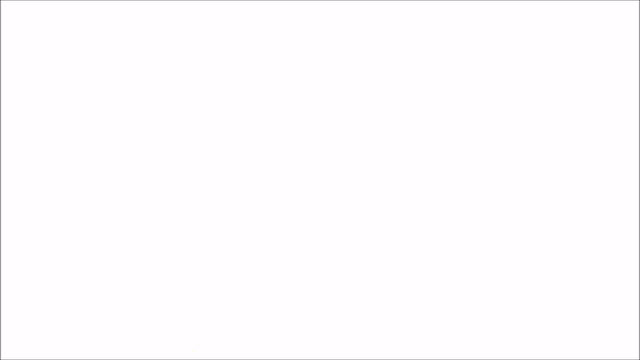 methods. so we're gonna do one by one the substitution methods. so i'm gonna do, uh, so we can talk about three, so let's go with the first one, uh, what we call the direct substitution. direct substitution. so what's the direct substitution list? it will be clear from an example. so what? 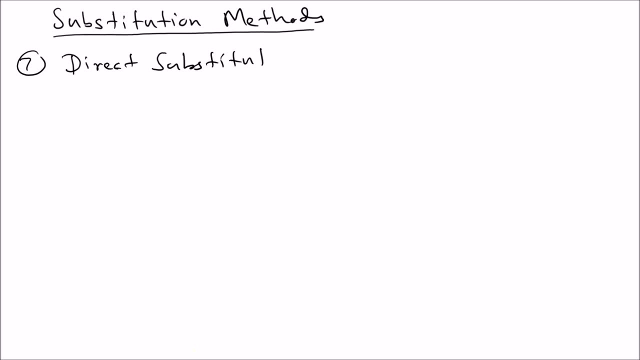 we know is that if we have a direct substitution. so what's the direct substitution list? it will be clear from an example. so what we normally do is let u equal what we call the inside function inside a function. so we're going to put the inside function. 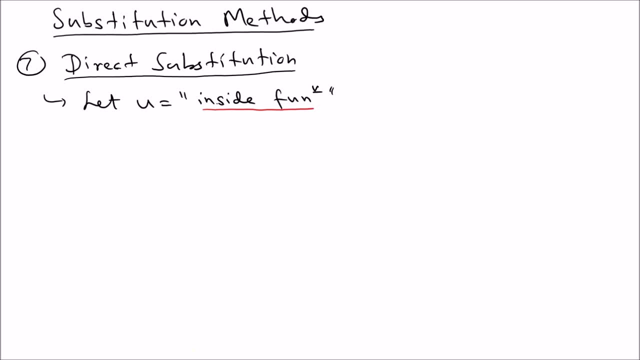 as u, and then we can write the difference equation using the new variable and rewrite, rewrite the differential equation using the new variable, using the new variable. so let's see this in a problem. so how about this one? let's say a: solve d y over dx, equal y plus 4x. 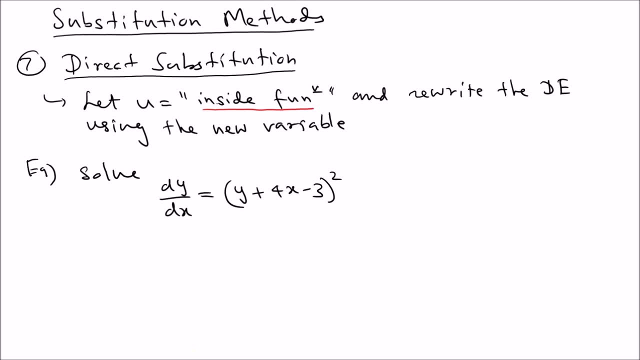 minus 3, refer万 a to the square, maybe something like that. so y0 equal 4. so let's look at this problem and you can see that if you look at this differential equation, um, if you try to expand this one, you're gonna get a lot of terms. 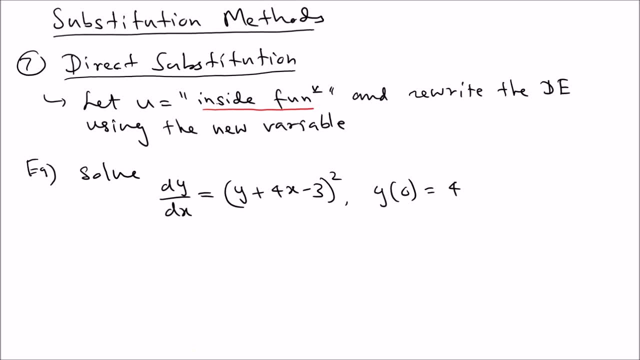 and it would be very difficult to solve, because there are y terms, y squared terms, x, y products and a lot of terms. uh, so, and you can see that, uh, none of the. so we can substitute for this inside function. that's the inside function, so let's so. that's the starting point, so what we're going to do. 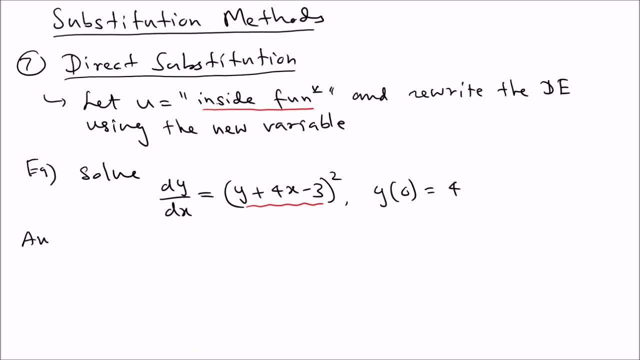 so the answer we're going to just the basic substitution we're going to pick. so let's say, let u equal the inside function y plus 4, x minus 3. so that's the starting point. we're going to pick that inside function and then just take the. 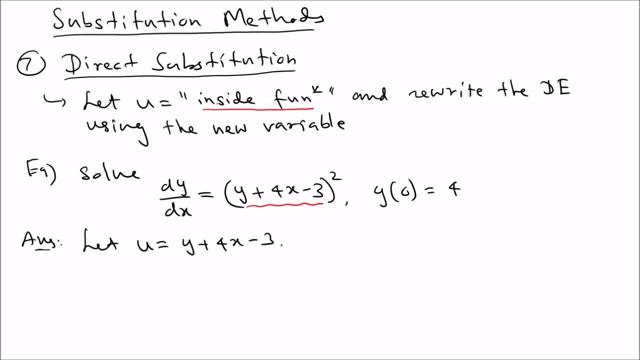 derivative. ah, so if you take the derivative, so taking derivative, so taking derivative. uh, we can write this one as uh y prime, or d by dx, so d u by d x, equal d y by d x on the other side, plus 4 y from here. okay, 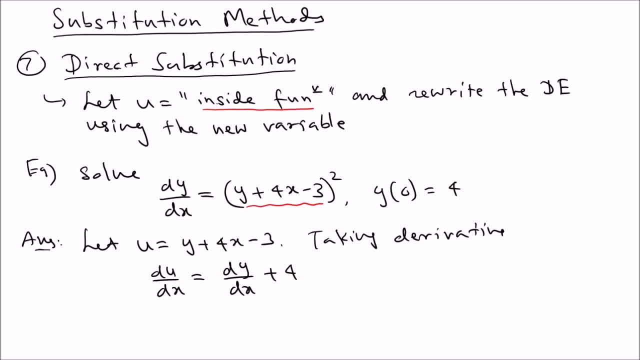 negative, so it's going to go away. so that's what you get, um, and then what you can do is you can solve for d y by d x. so this is the d y by d x equal uh, d u by d x, uh minus four. so we're. 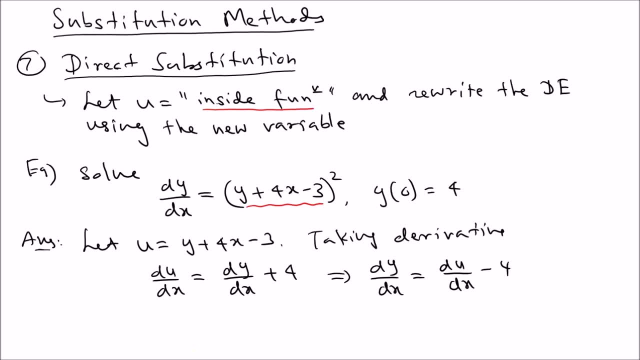 going to plug in that here. so if you plug in that, uh, what will happen to the differential equation? so d, d y by d x, you can replace by that, so it's going to be d? u over d x minus four equal. are we going to put the inside function as u, so it becomes u squared. 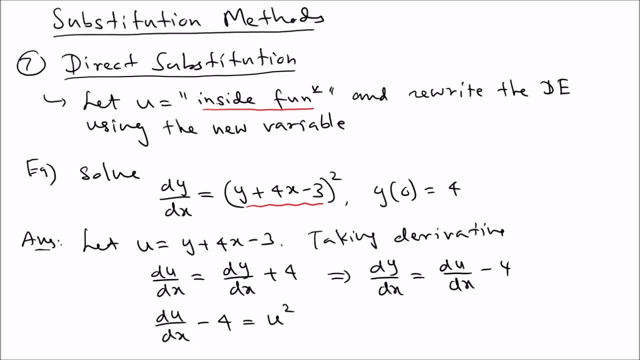 so that means uh. so this is that uh d u over d x is simply u squared plus 4, and you can see that this is a separable equation. this is separable, so we can just use the uh separation of variable method to continue. so we're going to solve for uh. 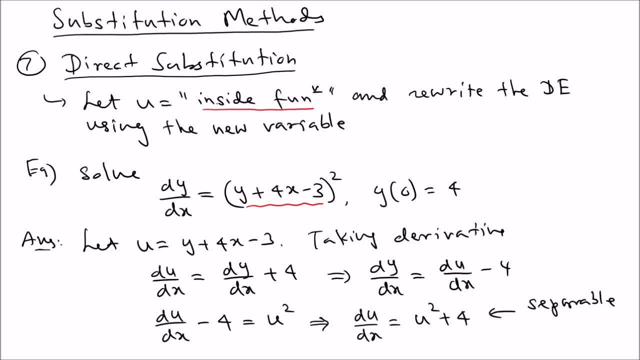 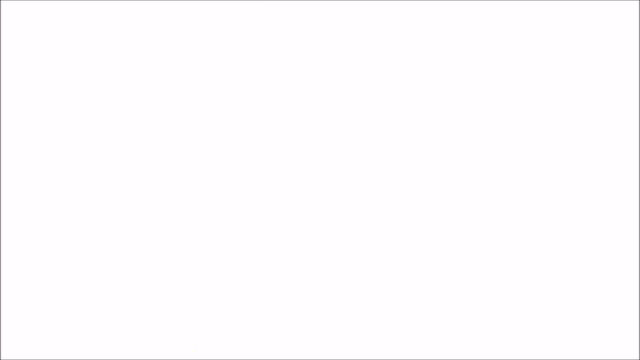 u first, after you solve for u, then you can use the substitution, this substitution, to solve for y. okay, just uh, solve for y, okay. so that's the idea. so let's finish the argument. so we have uh. so what we have, we have d? u over d, x is equal. 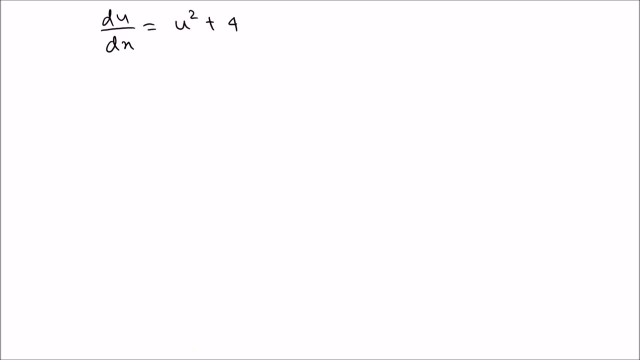 to? u squared plus 4. so you can. you can uh move the? u terms to one side, so we can write this one as d? u over: uh, u squared plus 4. the other side is simply d? x. now what we're going to do? we can. 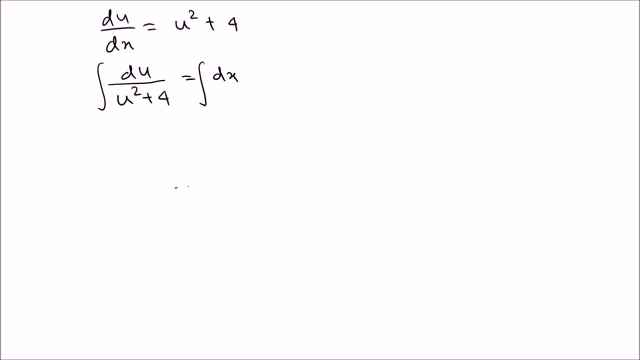 integrate the two sides. so if we integrate uh on this side, this simply going to be tan inverse u, because remember, there's a formula uh. so what the formula says, if you integrate 1 over x, squared u plus a squared uh, so this is simply uh, 1 over a tan. 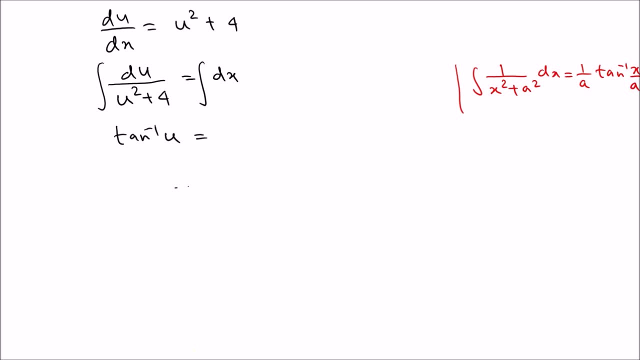 inverse x over a. so that's the formula, says plus c and that's what we can use here. so this is one of the formula. it's a direct formula, so we can use that um, and also you can find all these formulas in another video i put, like you know, all 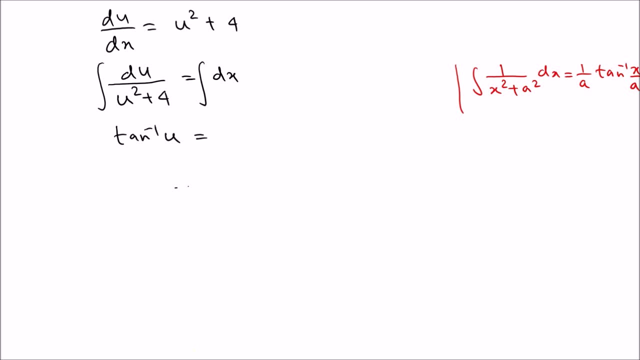 the videos in one, one formula: uh. in one video, uh. so you can see like kind of all the common formulas so you can check the uh, uh, calc 2 uh youtube list for that from that you can find it good. and also put a link, uh, link to uh in the description so you can find that. 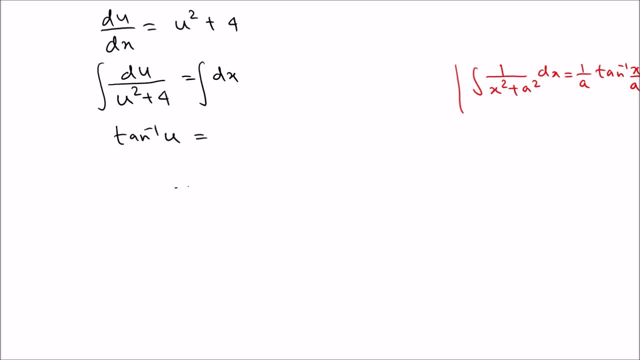 in the description of this video: good, okay, so that's what you get from the left side. from the right side, it is simply x plus c. that's what you get, um. so this means that if you take tan of both sides, uh, so this is that, uh u equal tan. 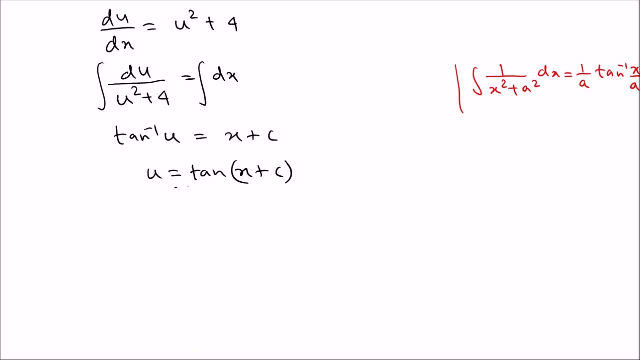 x plus c. uh, and then what is u? uh you equal. now we're gonna substitute it back. okay, so, uh, since uh u equal y plus 4x minus 3, you can put that here: 4x minus 3 equals x plus c. now you can just solve for. solve for y. 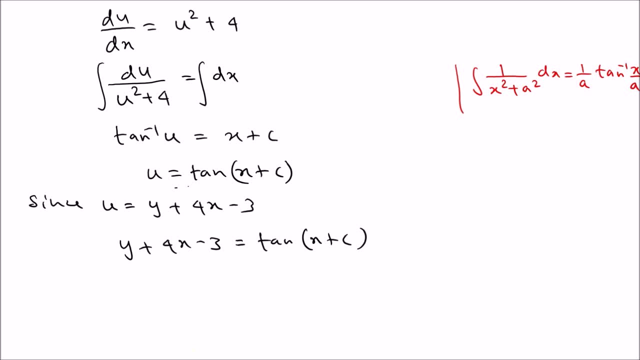 so you can see it's uh very simple. so y equal. if you know, the general solution is 3 minus 4x plus 10, x plus c. so that's the general solution and if you the initial uh, if you want to solve the initial value problem. 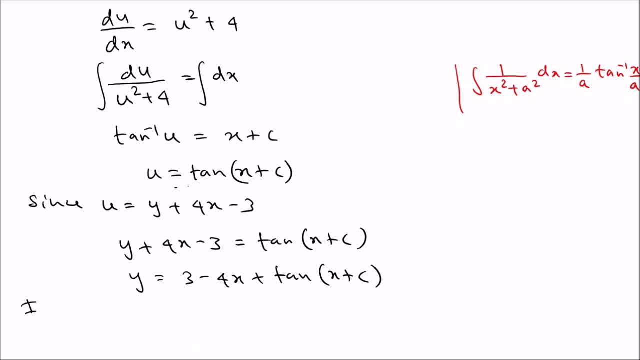 so you can use initial condition. so the initial condition y e, y, 0 equal 4 gives. so we plug in that. so the 4 equal 3, uh minus 0 plus 10 c. so this says that 10 c equal 1, in other words c equal pi over 4, that's: 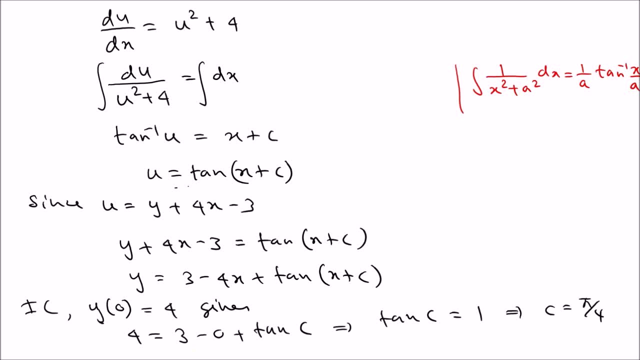 just one value. there are infinitely many values, so that's just one value. there are infinitely many values, so that's just one value. there are infinitely many values, so this is one solution. uh, so so one solution is equal. uh, pi over 4. uh, that means you can plug in that and you can write one solution. 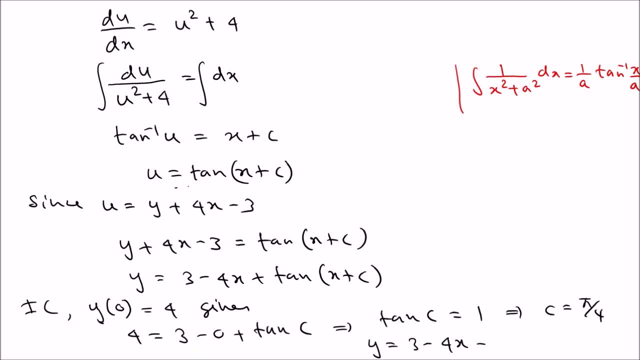 as 3 minus 4x plus 10 x plus pi over 4.. if you know the general solution, we know that for 10 you need to add a k pi, so that's so. that's going to be the same thing. you will have all the possible. 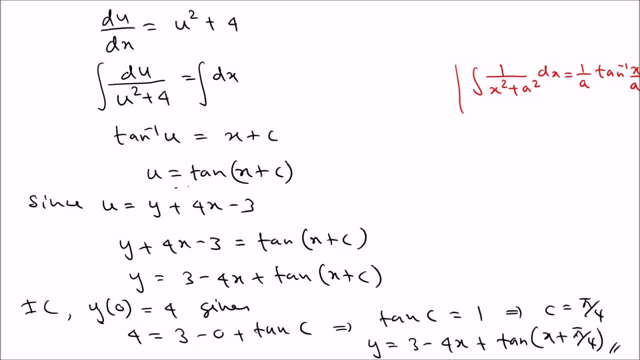 uh solutions, because we know that the tan has the period a pi, so you're going to add multiples of pi. okay, good, so that's the uh solution. but if you need the complete solution, general solution. um, like with all the cases, so this can be negative: 4 pi plus 10, we can do x plus pi over 4. 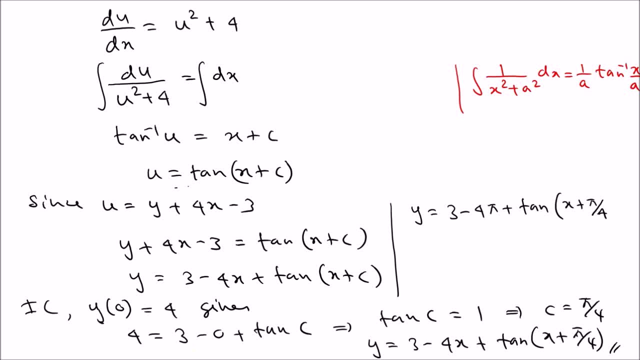 we can do x plus pi over 4, uh plus k, pi, where k is a integer. so that's going to give you, like all the cases, because the pi is the period of tangent function, okay, so, yeah, so you can see that. so the, the basic substitution method, works very well, and then you could solve the. 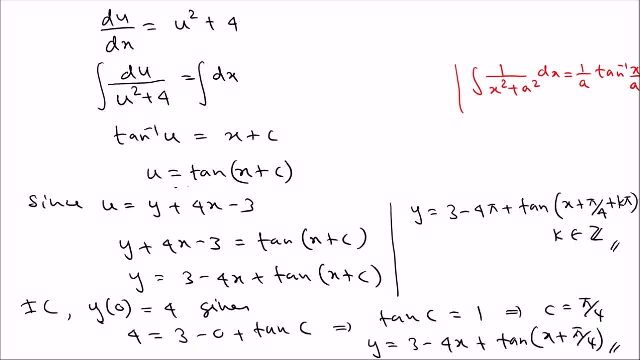 problem, yeah, so again. so, after you solve for u what you're going to? so this is where you solve for u. so you see, solve for u, and then what you do is a substitution, um to solve, to solve for y. good, so that's the b, what we call the basic substitution method. so let's talk. 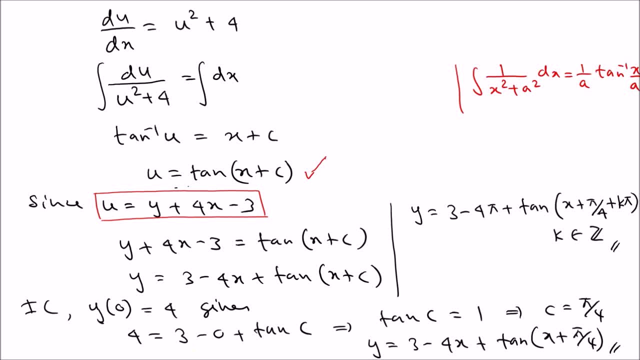 about what we call. the next one is the homogeneous equation. so this is the second meaning of the homogeneous equation. um, here homogeneous means uh, you can write the differential equation in as a function of y over x. so that's the idea here. so let's look at that. 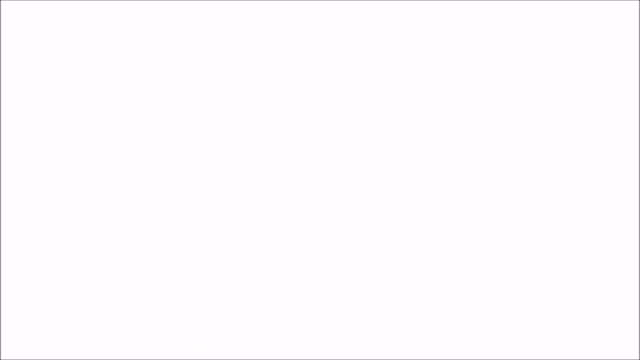 now. so it's number eight: a: homogeneous equations, homogeneous differential equations. um, so what is homogeneous equation? this is one definition of that. a differential equation, a differential equation that can be written as. that can be written as. that can be written as a as dy over dx, a function of 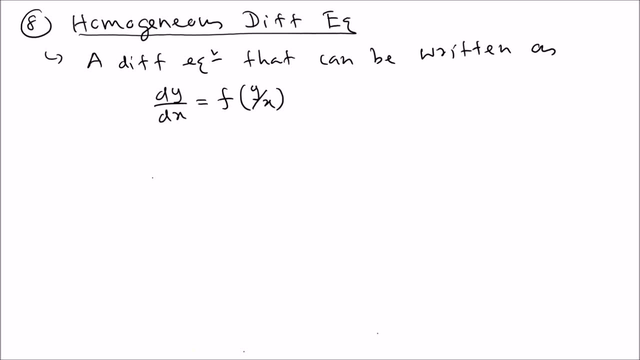 y over x. so if you can write the differential equation in this form, we call it is a homogeneous equation. okay, a differential equation that can be written as dy over dx is called a is called a homogeneous equation, is called a homogeneous equation. so this is like a one definition, it's like the easy definition. 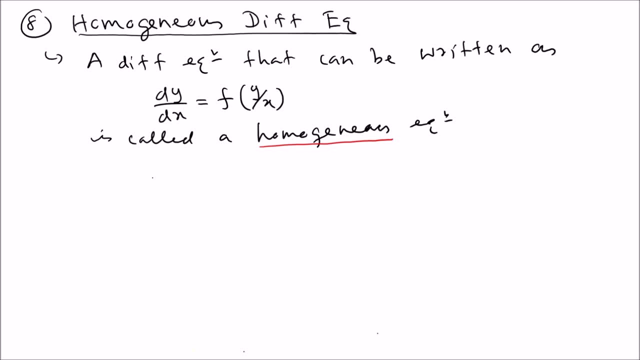 so, in this case, what you're gonna do? uh, since you can write the differential equation as a function of y or x, we're gonna pick that. so. so the solution method is: so: we're gonna let v equal y over x. so that is the um substitution we're gonna pick. therefore, we're gonna write the. 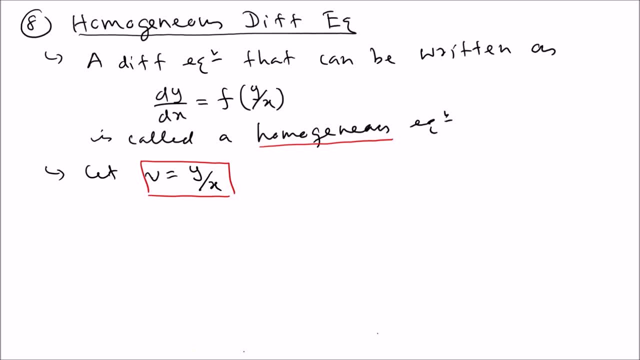 special substitution and then after that we can write this equation as: y equals v of x, and then what we can do is we can take the derivative. so once you take the derivative, what's going to happen? this is y prime: just use the product rule. so you get v plus x v prime just by the product rule. 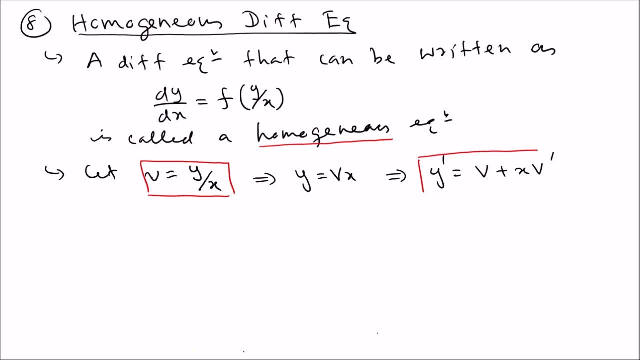 so we can use this as well. so we also need that. so those two are always the case with the homogeneous equation: no changes. so we can use that. and then the next step is: after we do that, then, uh, you can, you can substitute that, and then you get a differential. 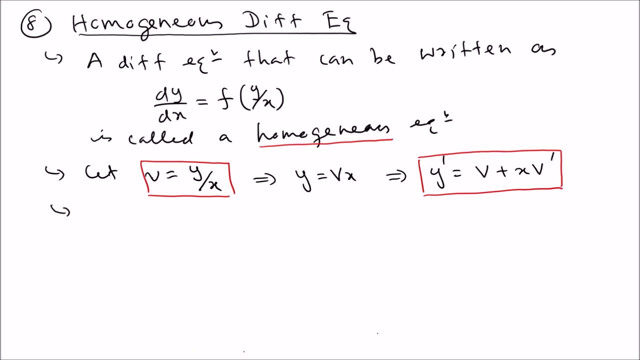 equation in terms of v and x. so solve for v first. so so we can say: rewrite uh, the equation in v and x variables and then solve for v first, and then i use, then use y equal vx. so simply multiply by x to solve for, solve for y. so that's the solution. 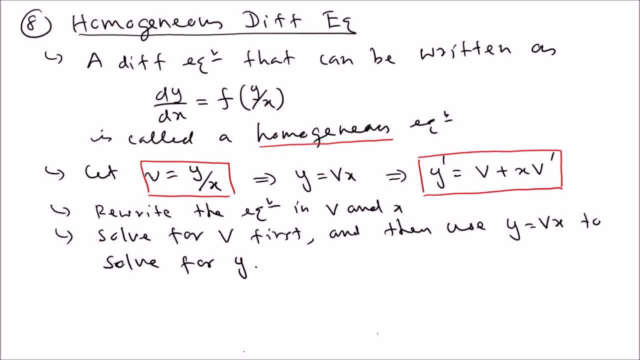 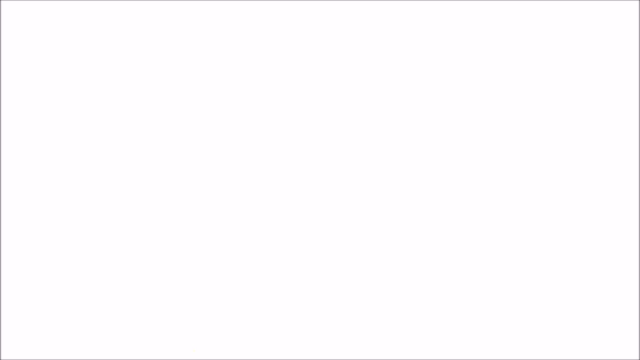 so that's the kind of argument: uh, so, uh, so it's not, it's not that difficult, okay, so, um, so let's look at this in a problem. so, as the first example, let's say this one: solve uh, x, y, d, y over dx. x squared, y squared uh, along with y 1 equal, let's say square root 2, so let's. 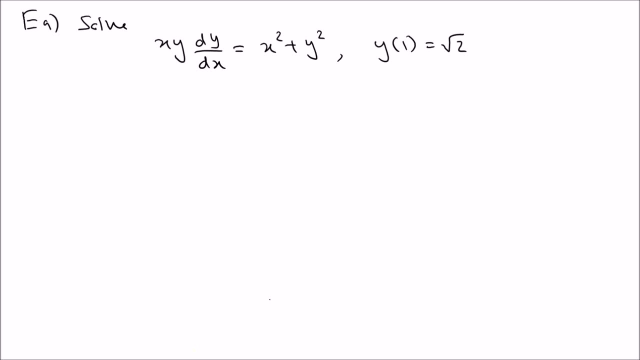 try to solve this equation and you can see that this is: uh, this is not the basic substitution. uh, this is not separable, this is not indicating a factor, so you can't use any of those techniques to do this. so what we're going to do? um, we're going to see this term, so we can. 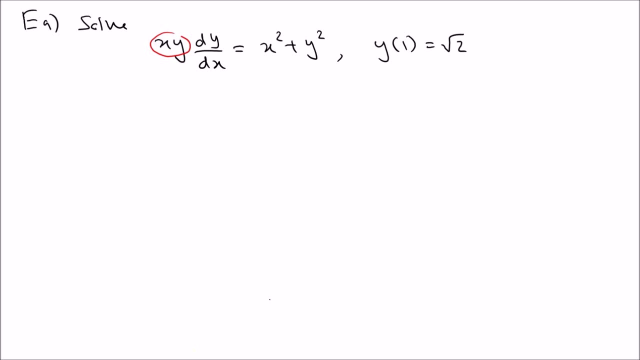 divide by that term both sides. so we're going to divide by that term both sides. so that's the starting point. uh, so the answer: dividing by dividing by x y. so we have d y over dx, which is x squared plus y squared over x y. um, so if you divide x squared, okay, let's. 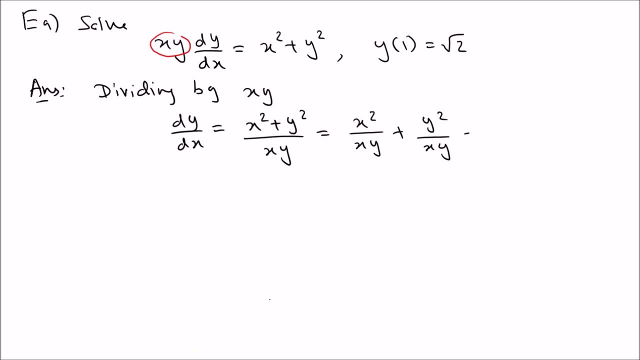 y, you can see x get cancelled. so you're gonna get the first one become x over y, y get cancelled, the second one become y of x. okay, now you can see that it's a function of um y of x, because x over y is 1 over y of x. so that means everything, uh. 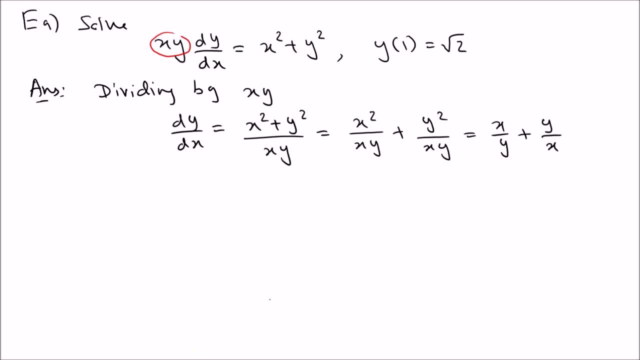 looks good? um, because the first one you can divide by x in the top and bottom, so you can write this one as 1 over y of x, plus the other one is y of x. so that is the function of y of x. now what we can do, we can use a substitution now. 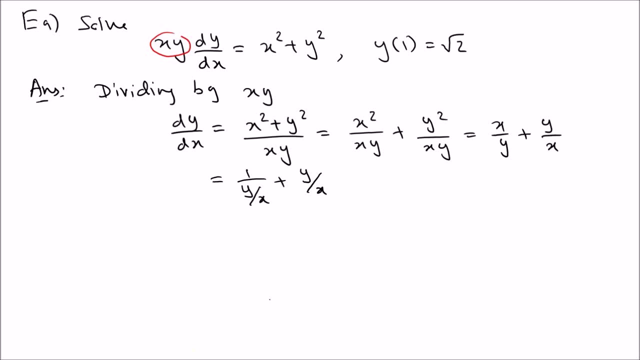 ah, so let v equal y of x, then we know that y prime equal v plus v prime x, so we can write this one as 1 over y of x. so when you substitute uh d y over d, x means y prime, so this side become v. 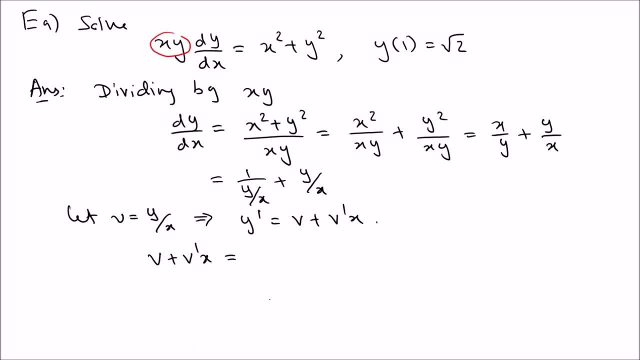 plus v prime x- the other side is 1 over v. plus y of x is v. you can see interesting part: this get cancelled, so that term is going to go away. so you simply have v prime x equal 1 over v, if you write this using derivative. 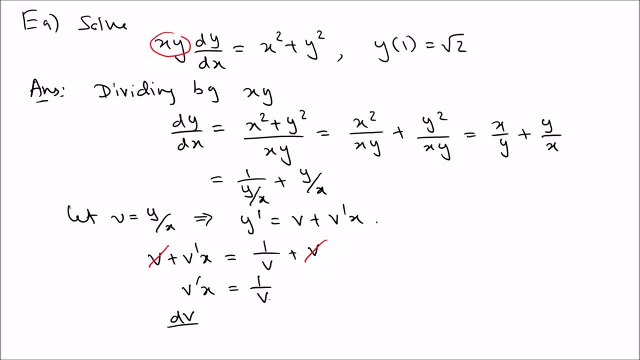 notation: dv over dx, x equal 1 over x. you can see that you can write this as 1 over x. this is a separable equation. so this is separable. so what we can do? uh, we can separate the two variables. so if you separate the two variables, we can write this one as v. 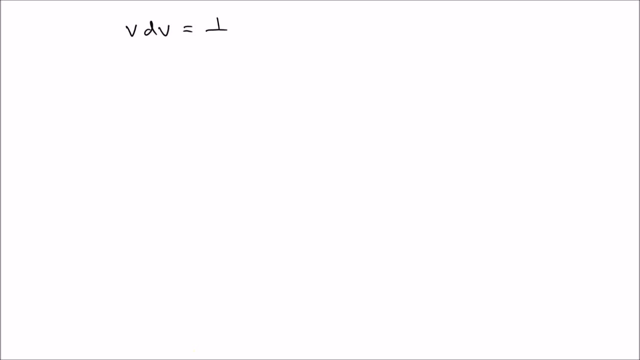 dv on this side, the other side, 1 over x, dx. now we're going to integrate the two sides, so integrate v with respect to v, so it's get v squared over 2. this one, 1 x, means l, n, x, uh plus c. just add c to some one side, uh, so now. so we solve for v. 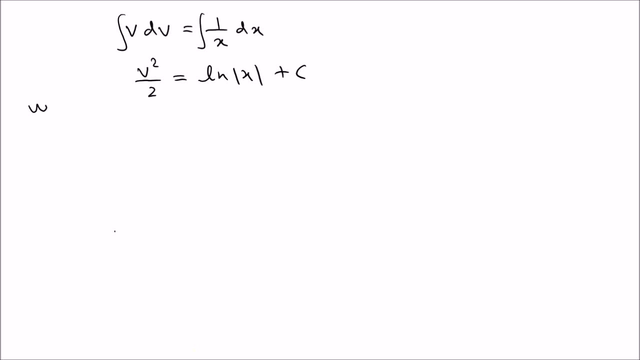 now what we're gonna do. we can do a substitution. so use our y, y equal vx, ah or v equal y of x to write. you can write this one as one: half y over h cross into t plus y of x. here this is ln x plus c. now we can uh multiply both sides by. 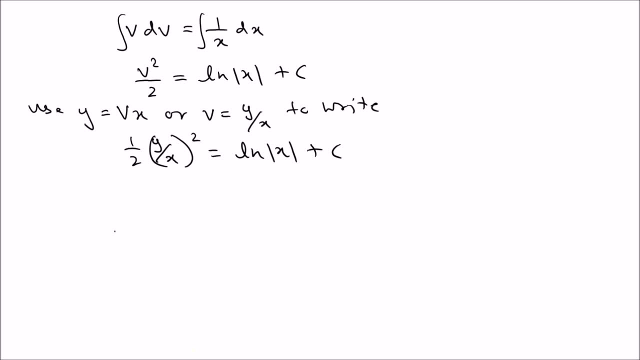 2x squared to isolate y. so this says that y squared equal 2 x squared ln x plus c. uh, now what we can do is we can solve for c. so let's say: uh, using y 1 equal 1, we have action of 1. y 1 equal square root 2. 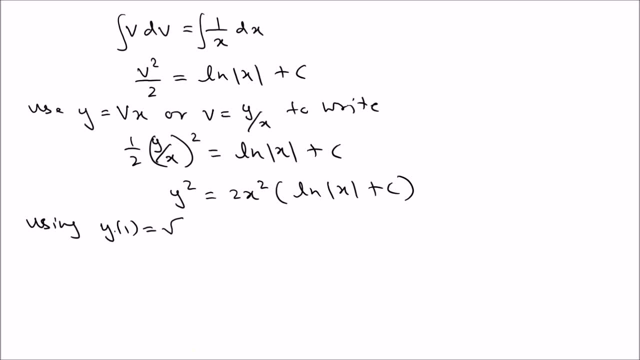 square root 2. we can substitute. so it is square root 2 square. that's the y value, x value is 1 and then we have ln 1 and then we have 1 plus c, but we know that the ln 1 is 0. 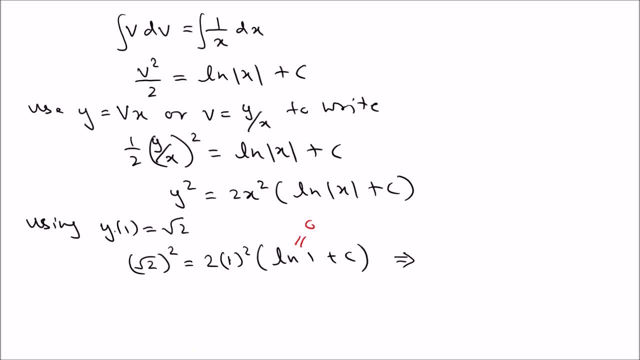 so this says that 2 equal 2. c says that c equal 1. so we can plug in that value back here. so it is 2 x squared ln x plus 1, and now what we can do is we can take the square root, but be careful when you take the square. 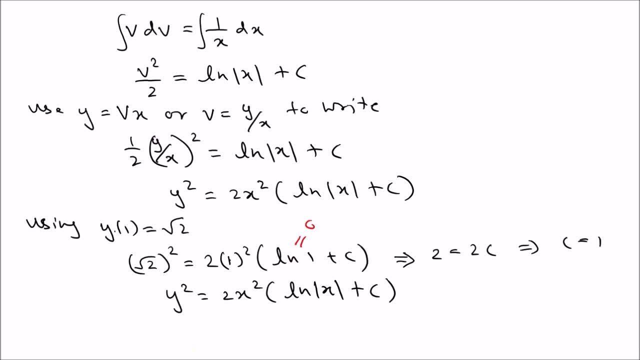 root you get plus or minus. now the question is which one gonna work. but we know that y 1 equal square root. 2, that means which is positive. so that means you have to pick the positive root here. so it is 2, uh, so we have uh. 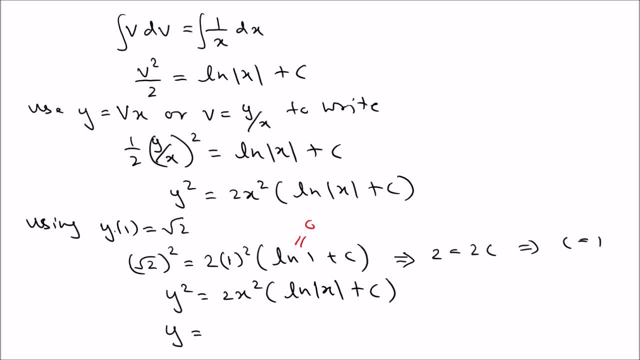 ah, so, uh, yeah, so we have the two there. so that means, uh, actually c equal one, yeah, so let's, let's, so let's write this down, so, let's write this down, so, let's write this down. so c equal one, uh, so, um, now, what we're gonna do, we're gonna do the square root. 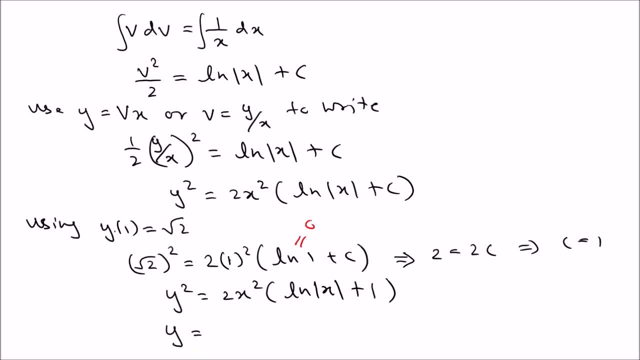 so you only get the positive one. so it is x. so we this is a 2 ln, x plus 2 inside and the square root. so we only pick the positive one. since y is greater than zero, y positive because we know the initial condition is y positive. 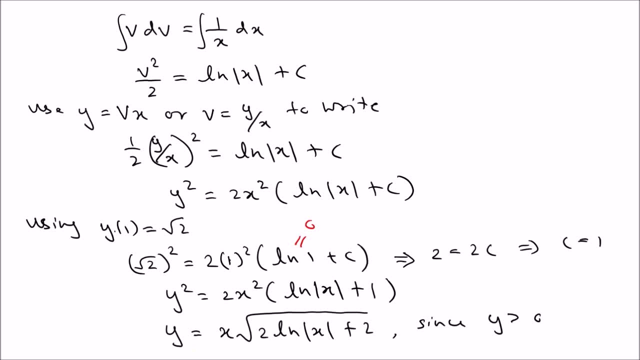 because if we had picked the other one, you get negative answer. so that's not going to work. so, but so that that means, if you are given that, so let's say, if you had, if you had, y1 um equal negative square root 2, if this is given, you can see that c is. 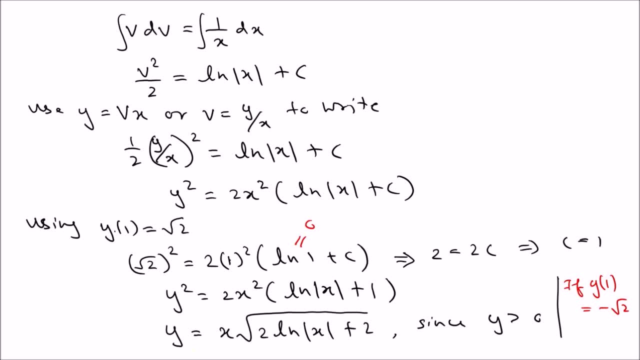 still 1, but you have to pick the negative 1, in this case negative solution, because otherwise it just doesn't work. so you have to pick the negative one, negative one that's not satisfied the condition, because we know that when you try to solve for y, you get plus or minus. okay. so this is. this is what i'm talking. 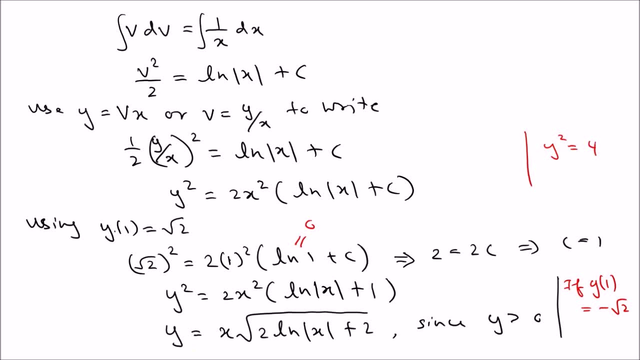 about when you have y squared equal, let's say 4. y can be either plus or minus 2, so which one? it depends on the rest of the problem. so that means if you are given an initial condition like y 1 equal square root 2, you want to make sure i satisfy the 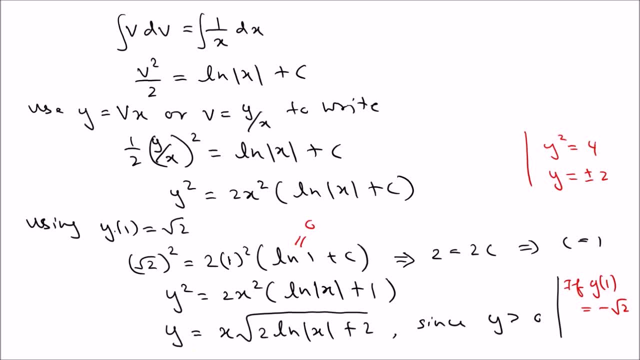 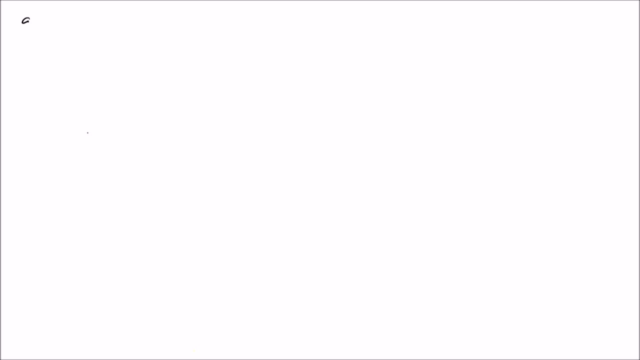 condition. that means you have to be the negative one in that case. so here only the positive one works. okay, i hope you understand the uh argument there. okay, now let's go to this third type of substitution. so the third type is what we call the bernoulli equation. so let's talk about that. 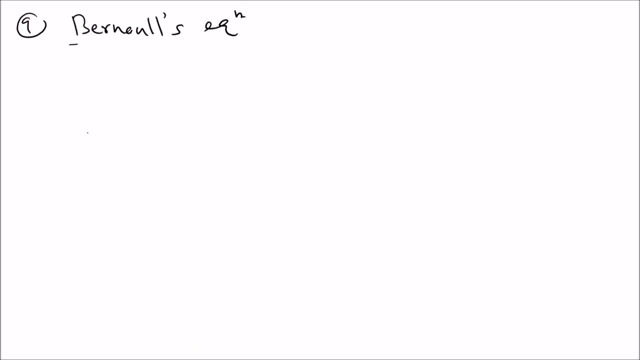 so bernoulli's uh equations, bernoulli equation, uh. so. so what's the bernoulli equation? so this is the extension of the first order linear difference equation. so it is dy over dx plus p, x, y. so we still have that part, but the other side 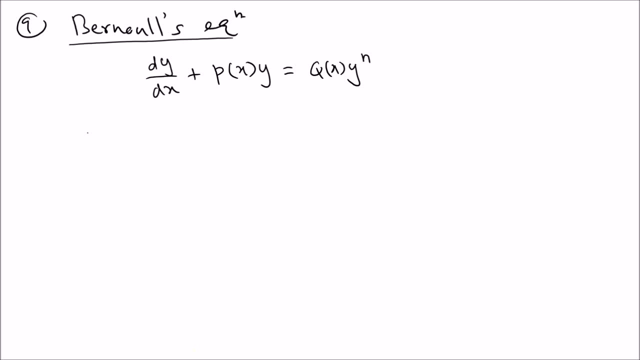 is different. it is y to the n power, so that's a yn term. so that's the difference. we have the extra term on the other side, yn. so there are special cases to consider. so if you get this one, this is a bernoulli differential equation with that y to the n term. but there are. 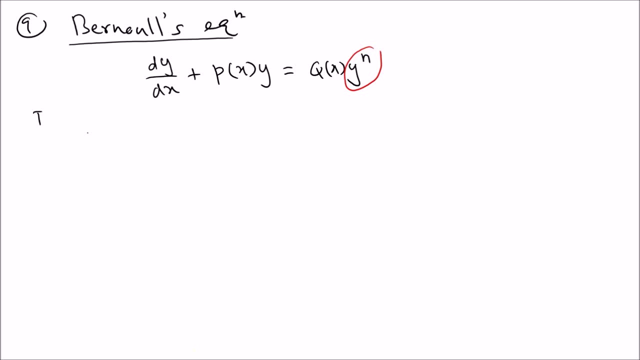 some special cases that we want to consider. what if n equals 0, same time is 0. 0. then you're going to get d y over d x plus p x. y equal q x. so that is our famous one. ah, so this is the uh integrating factor method. 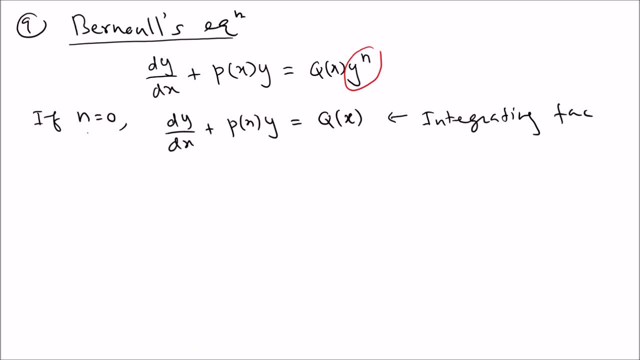 okay, that's the integrating uh factor method. ah, so not very interesting. i mean, we know how to do that. okay, it's interesting, but we know how to do it if we know how to do it, if we know how to do it. so what happened when we say we got n equal 1? 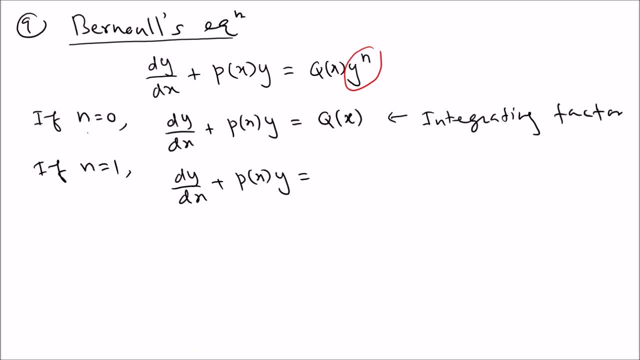 what happened? so d y over d x plus p x y, equal q x y. so if you get that, we have two options. one option is we can bring that this term to the other side. so if you bring this one to the other side. so so there are two ways to do this. 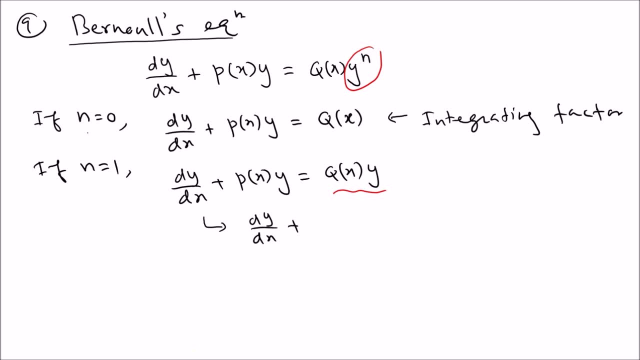 problem. so one way we can bring uh, that term to the other side. and then what happened? y is common, so you can see this again. first order: linear. so this is integrating factors. integrating factors now, if you bring this term the other side, to the left side, so this can be qx minus. 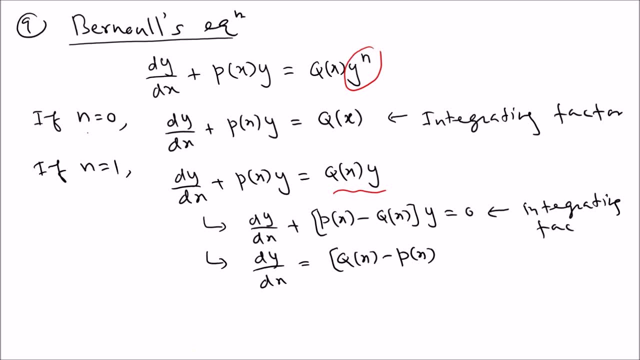 px, y. you can see this is separable. okay, so this is separable. so that means we can solve these two cases. uh n equals zero case. is integrating factor n equal one case. you can solve in two different ways: either integrating factor method or you can use the separation of variable method. 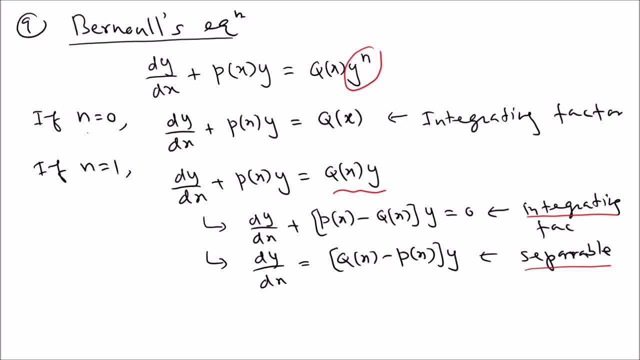 so what we, what we are interested in this one is: we can consider the case we are n naught t equal to n minus px. okay, so that means, if a not equal to zero or one, we have a new case. okay, new situation. so that's the uh bernoulli, uh equation. so we're gonna. 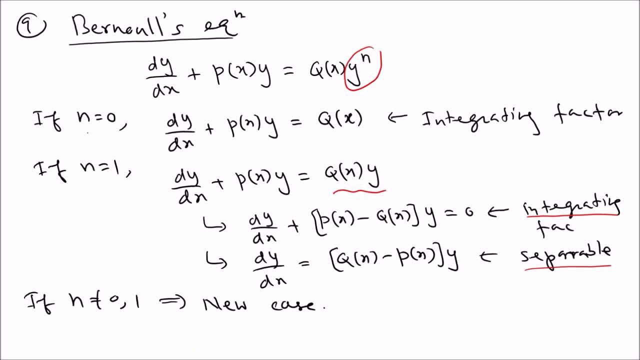 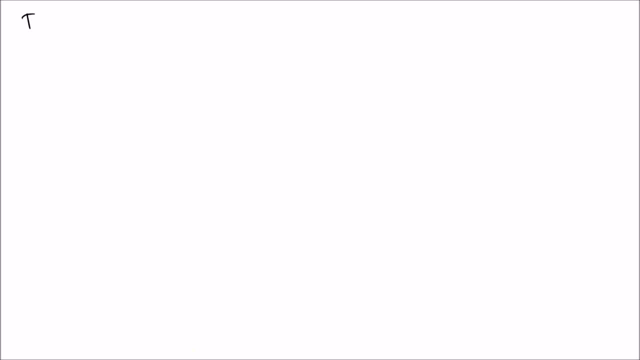 talk about that. so let's talk about that a little bit more. um, so, if n not equal to 0 or 1, so that's the bernoulli equation, right, let's talk about that a little bit more. what we're going to do, we can divide, uh, so dividing by. 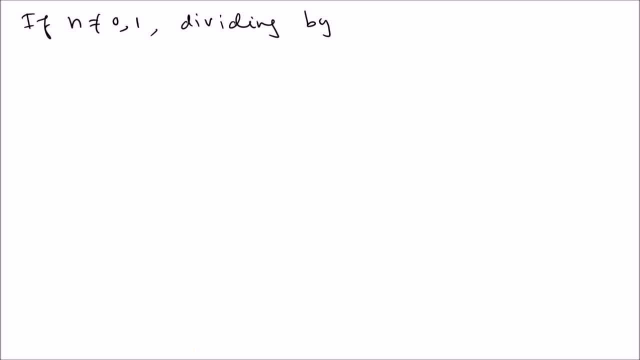 y to the n. we can divide the equation by y to the n term, divided by y to the n term. if you divide the equation by y to the n term, you're going to get 1 over y to the n, d, y over d x, ah, and then here you're going to get p x. 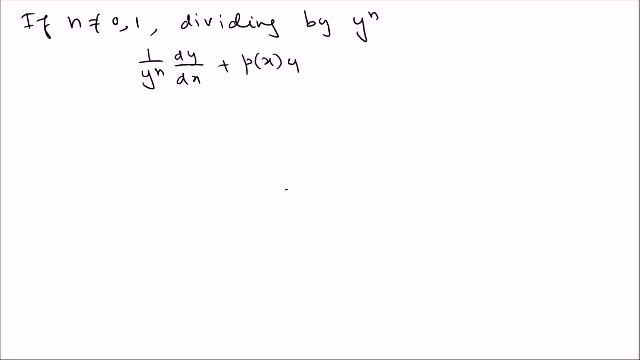 this can be y 1 minus n, because we can divide by y to the n term. we already have one y term, so it's beginning y to the 1 minus n. on the other side you become just q x. okay, now we're going to do a special substitution. 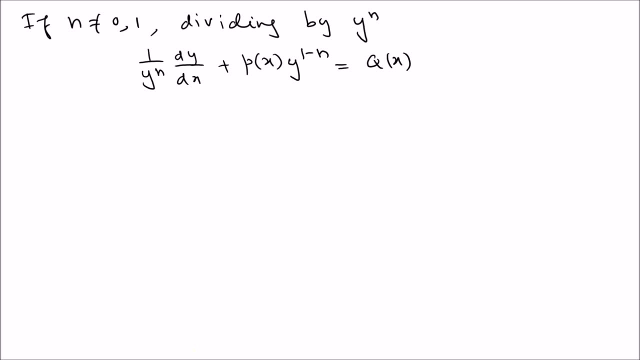 so the substitution is: we're going to substitute for this term, that's how we do, you know, subject for that whole term. so let v equal to y equal y, 1 minus n. so that is the substitution you want to remember. okay, and that's why n cannot be equal to 1, because if n equal 1, 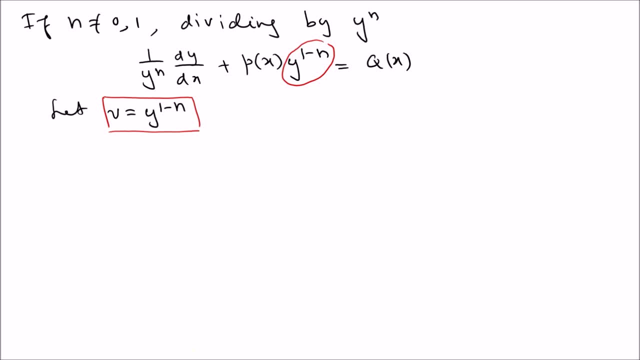 this is just 1.. so it's not going to work. that's not a variable, just a constant. so take the derivative going to be 0.. now what we can do? uh, take the derivative. so taking derivatives, so taking derivatives. we can write this one as: 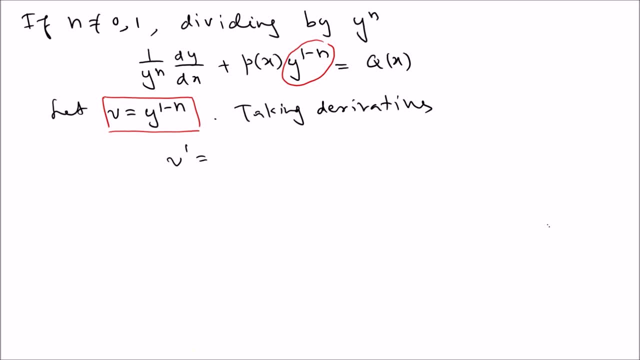 uh v prime. so we can use the chain rule here. it is 1 minus n? y. you subtract one more, so minus n by n? y prime, by the chain rule. so this is the chain rule. good, ah, so that means we can solve for y to the n? y prime term. so this says that y to the n? y prime term. so this says that y to the. 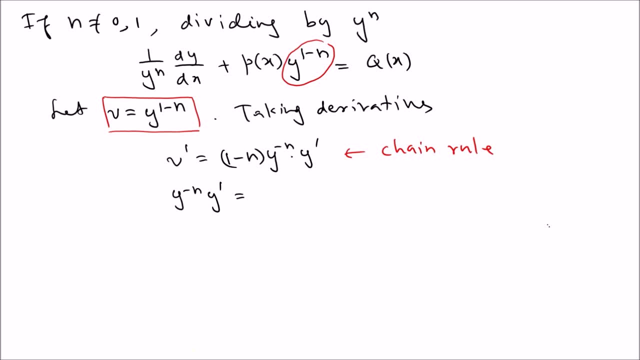 is simply 1 over, 1 minus n times v prime. so that's always the case. now, what we're going to do, we're going to substitute that in the equation. so if you go back and substitute in this form, uh, so you're going to get 1 over, 1 minus. 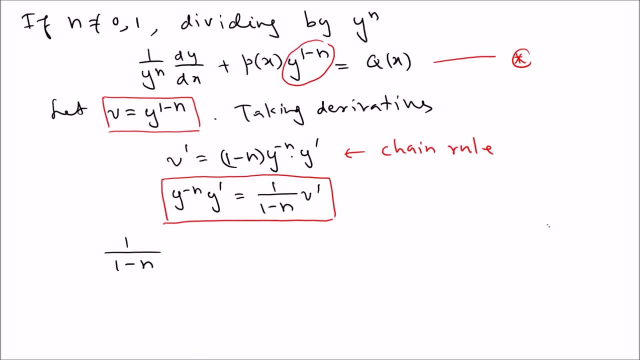 n, v, prime- that's the first term- plus p, x times v, prime, x v equal q, x, and you can see this again: first order linear in v. so this is a first order linear, first order linear in v. that means we can use integrating factors. okay, so use uh, integrating factors. 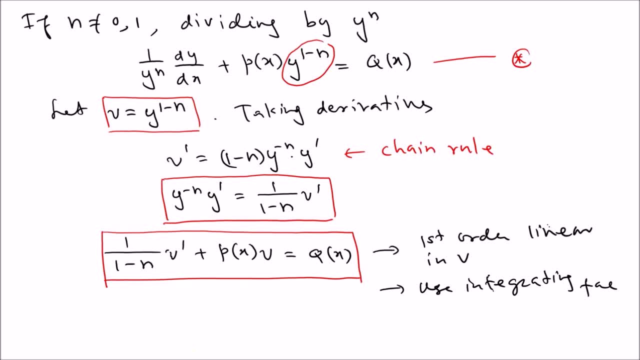 use indicating factors to solve for v, and then i use v equal y to the 1 minus n to find y. so that is the argument. okay, so that's how you solve the bernoulli equation. so let's look at one example to see how it works. 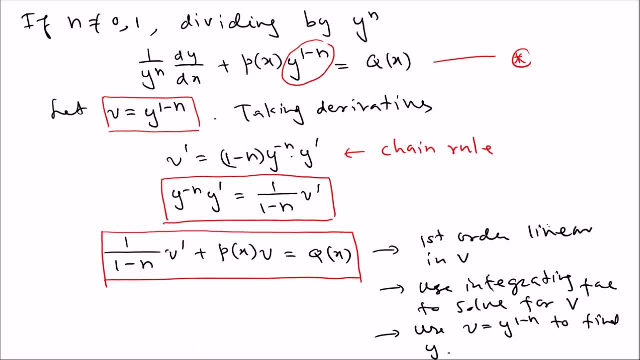 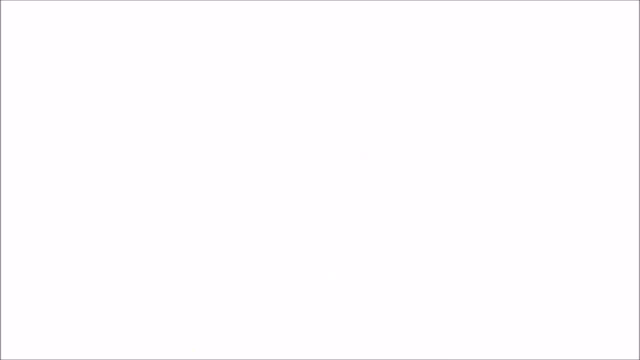 so let's look at the bernoulli equation. so let's look at, uh, one example to see how it works. okay, um, so how about this one solve? let's say, uh, 2x d y over, d x minus y equal 6 x squared y. cube, this one. 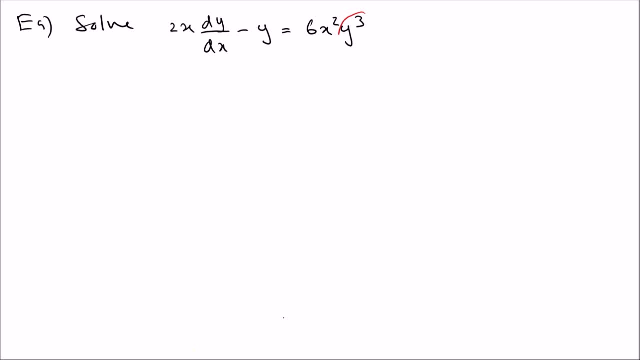 uh, so this is the equation we're going to use to solve the bernoulli equation. so let's look at one example to see how it works. so you can see, we have this term and this is bernoulli. bernoulli is a bernoulli equation. 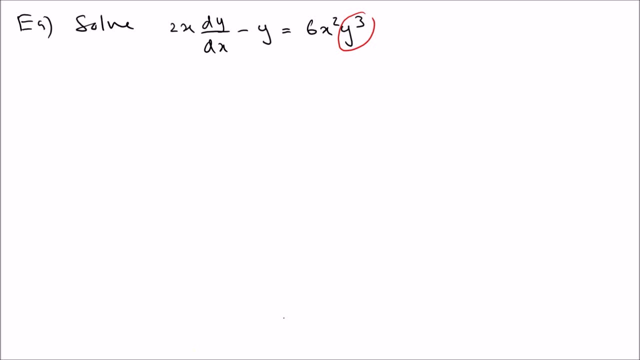 so we divide by that term and also you can see that there's an unnecessary term here. so, uh, what's the term we have here is, and you can see, so, uh, dividing by d, x is the ממ�- north Dollars. we also are going to divide by x also. actually, you can divide by 2 also, but we 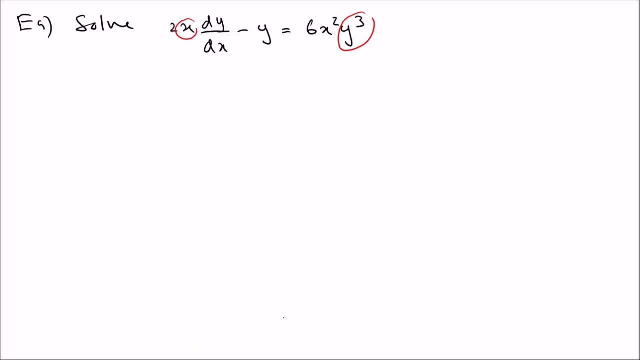 can leave 2 and you can see how it works. so um, so, dividing by dividing by x, y cube. so you're going to get 2 y, q y negative, 3 d y over d, x minus 1 over x y negative 2 equal one of the x terms get cancelled. 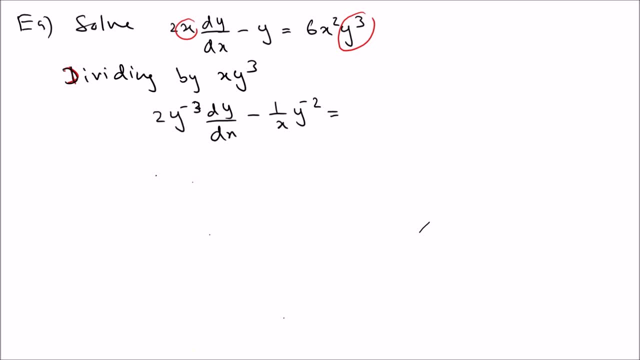 y 3 get cancels. uh, so you're going to get c 6x. that's what they get now the substitution. so we divide. now you can see that you get to the first one form that we want. now we're going to substitute for that. 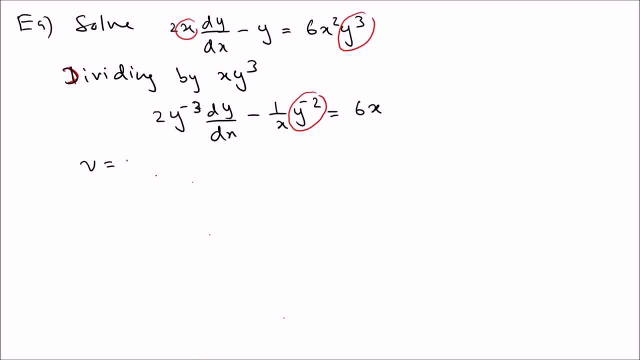 ah. so we're going to say v equal y negative 2. ah, this implies that v prime equal negative 2, y negative 3 y prime, in other words, y negative 3 y prime is negative one half v prime. i mean, that's what we're going to. 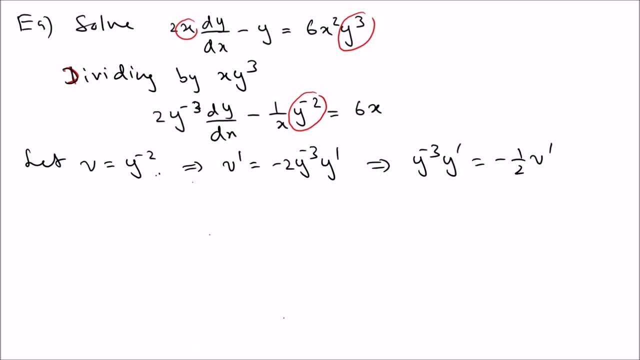 substitute for that. so that's what happens. so we read like that: and now we can substitute that. so if we substitute that, so by substituting, substituting two times, uh, negative one half v, prime substitute for that, and then minus one half v equals 6x. 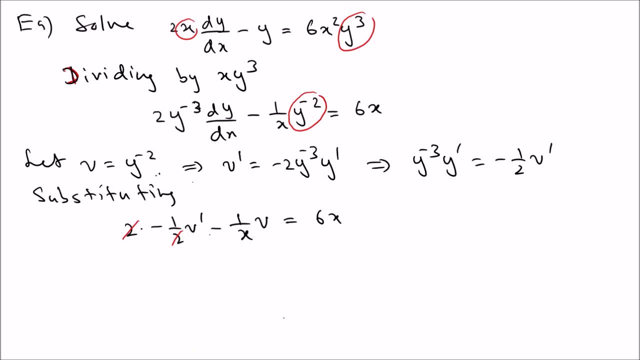 uh, this gets cancelled, and uh, and then you're going to get negative v prime. negative 1 over x v equals 6x. you can multiply by the negative sign, so v prime plus 1 over x v equals 6. you can see, this is first order. 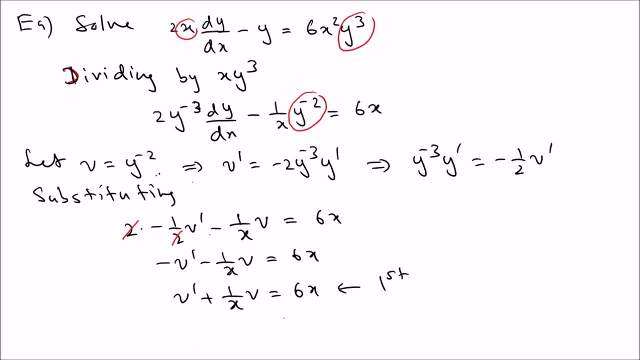 linear in v. that's exactly what we want. first order: linear in v. so let's use the integrating factor method. so the integrating factor, integrating a factor i equal e to the p, x dx, so e to the one over x dx, e to the ln, x, that means x. 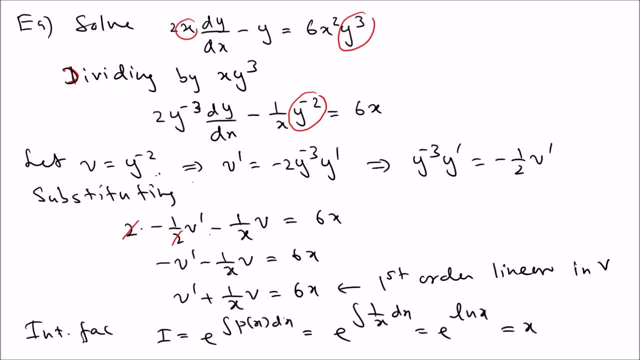 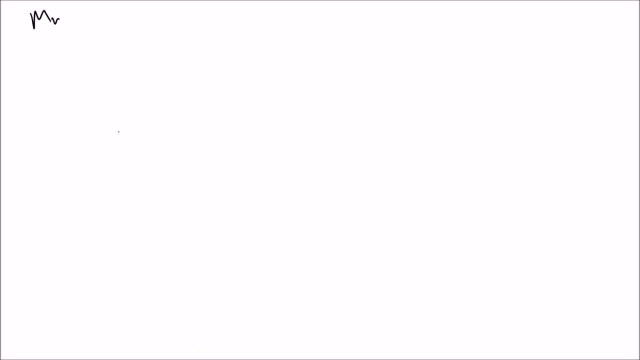 so we get that. now what we can do, we can multiply by that both sides of the vector, so multiplying by x. so we're going to get x v prime minus and a plus v equal negative, 6 x squared. this side is automatically the v and the integrating factor. 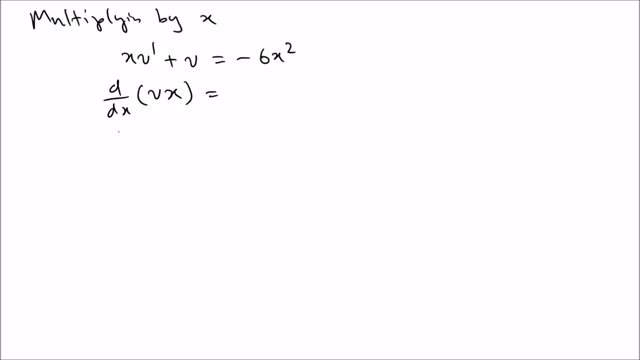 uh, which was x equal, negative 6 x squared. now, integrating those steps are just the integrated factor argument. integrating we're going to get vx equal. if you integrate this one, this can be negative uh, so you're going to divide by 3, so it's 2 x. 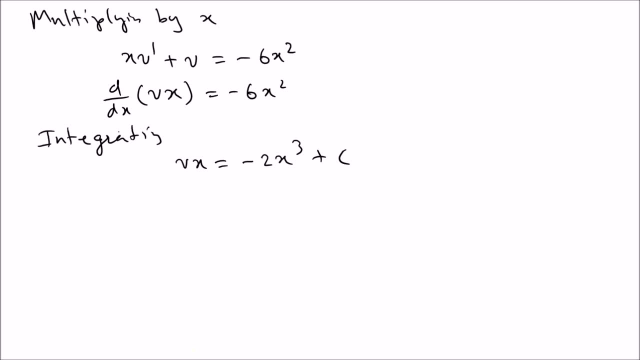 cube plus c. so that means v equal. if you divide by x, so you will u x squared plus c over x. now what we can do, uh, using uh, v equal y to the negative 2. we're going to substitute that, so we have 1 over y squared, which is y. 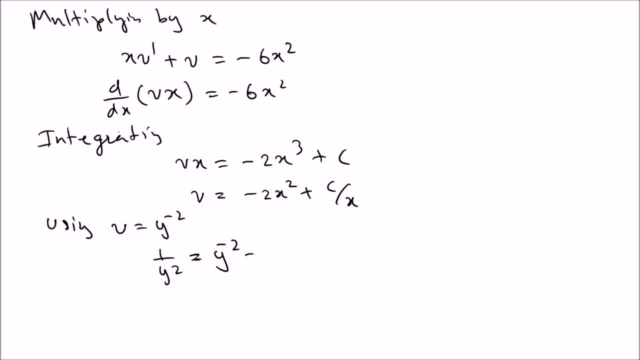 to the negative 2, equal negative 2, x squared plus c over x. so what you want to do now is you want to flip it over. but before you flip, you're going to get the common denominator here. you have to get the general denominator here. you have to do that. so x, so that. 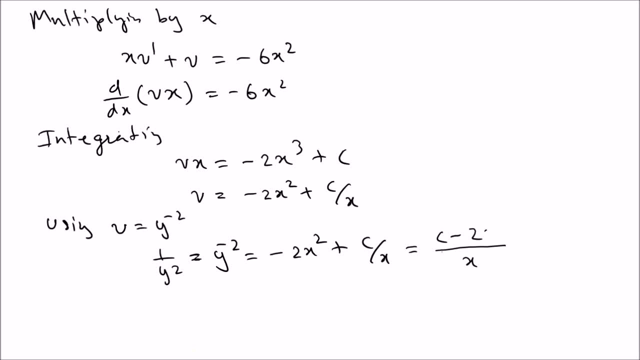 means you're going to multiply by x. you can write this in a: c minus 2 x cube. now you're going to flip it over, so that means y squared is x over c minus 2 x cube. now again, considering our cases, you can say y equal. 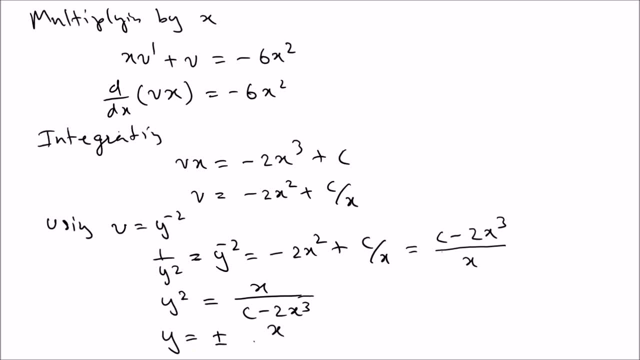 since we don't know, we get a plus oh, minus x over c, minus 2 x to the negative 2. we have the um. we're going to change that so we can add that over all right x cube square root. so those are all the cases, the two cases, and if you 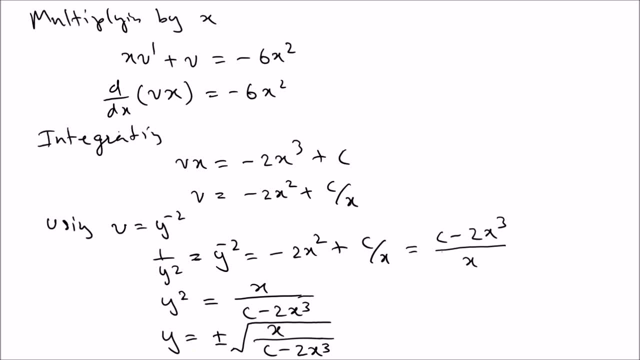 know the initial conditions, we can find them. otherwise, this is the general solution. so this is the general solution, okay. so that's about that. so that's the basic. that's the substitution method. so we talk about the basic substitution: uh, homogeneous equations and then the bernoulli equations. 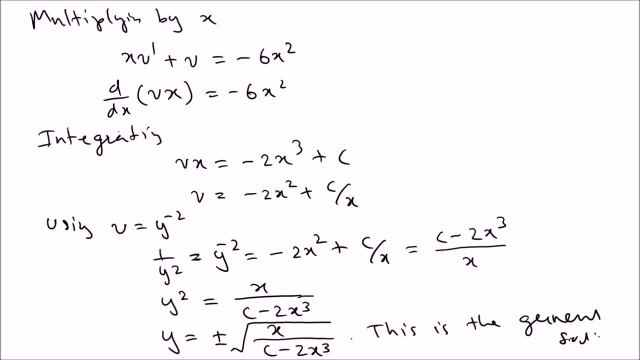 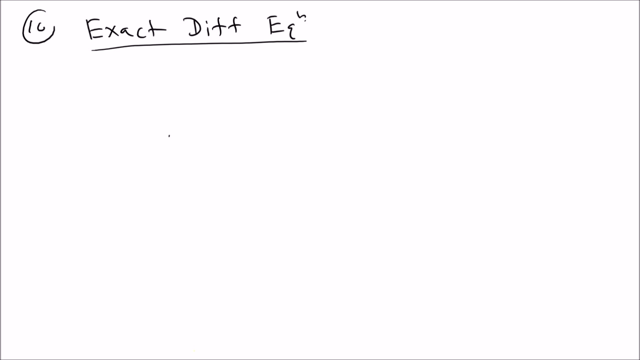 so, and then the uh, the last type of first order differential equations, the exact differential equations. let's talk about that now. ah, so this is the last type. we talk about what we call the exact, uh, differential equations. so what we mean by exact difference? so we can look at the first order differential. 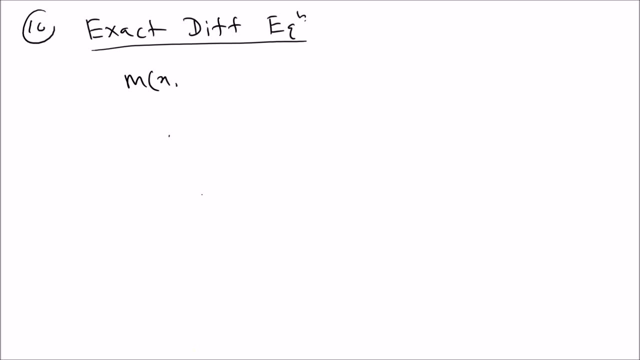 equations, we can look at the standard form, which is m, a function of x, y, d x plus n, a function of x, y, d, y equals zero. so that is the standard form we're going to consider. okay, it has to be d? x plus d? y, but there are other ways to write the. 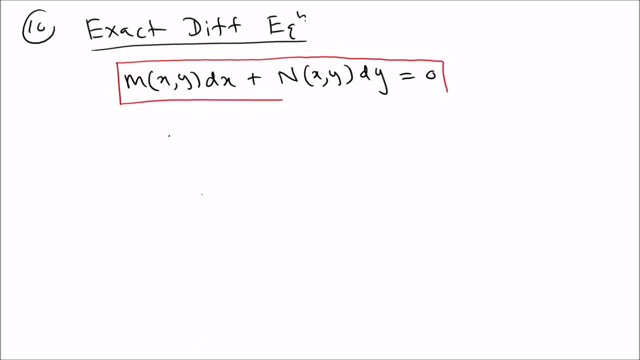 same equation. for example, if you divide the equation by d x, you can write this same equation, this form as well. so you can write this one as uh, for example, d y. yeah, i'm gonna write it uh down here because i need some space. so we can by dividing by d x, we can. 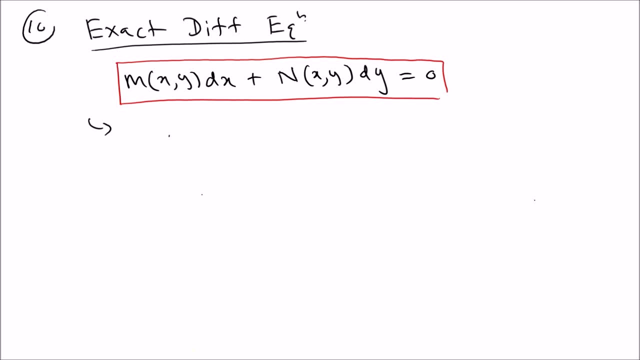 write this one in: uh, for example, d y over d x times times: n x, y, n x y plus m x, just by dividing by d x. but we don't do that because this is really not the right way to do it. uh, we're going to go with the. 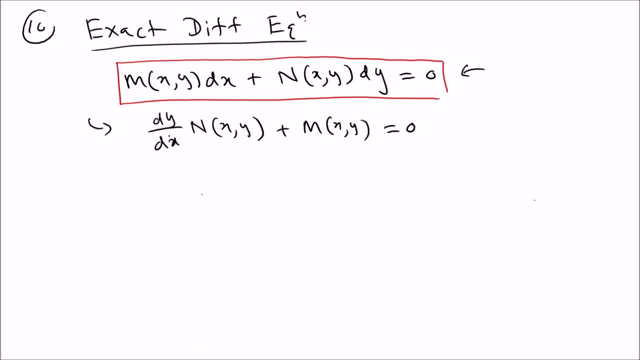 the standard form above. so this is what we call the standard form. we do that for a reason: because there are different equations we're going to come like in physics and mathematical physics come into this form. so that's why we kind of study that. now let's talk about the uh, the theories, uh, that we discuss. 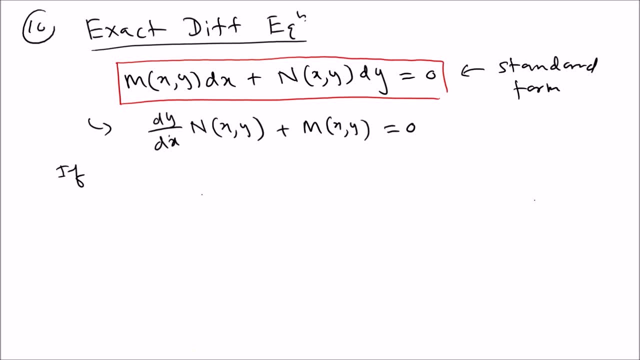 okay, so. so what we call: if the daba m- there's a partial derivative of m with respect to y, equal, the daba uh the partial derivative of n with respect to x, if those two are equal, we call this differential equation, a exact equation. okay, that's the kind of test, uh the equation. 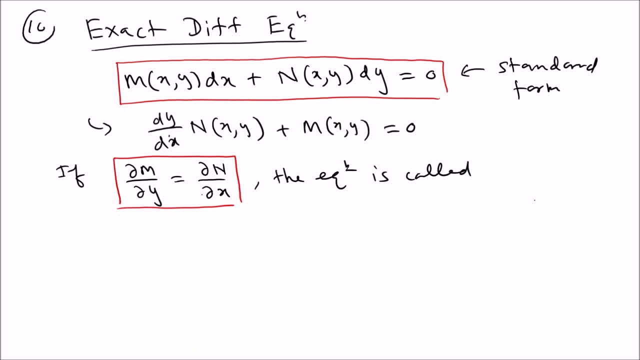 equation is called, uh, exact is called exact differential equation. uh, this is the kind of test we use, uh in that case? and in that case what happens? there is a function, there is a function. there's a function- f, x, y equal a constant. so there's a function. 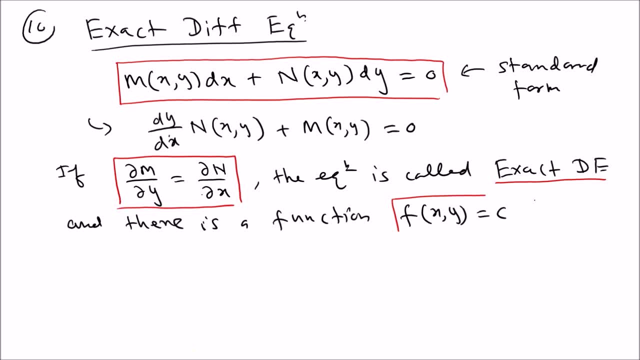 like that, such that, such that that the partial derivative with respect to x equal the m function and the partial derivative with respect to a- y equal the n function. so it says that if that is the case, if this condition satisfies this condition, if this condition satisfies, there is a. 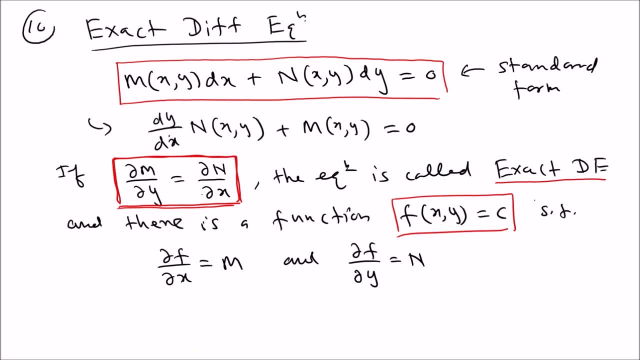 function such that f x y equal constant. c is a constant that can give you double f over x equal m and w for y equal m. okay, and then if you know that function, f x y- what we're going to do, we're going to solve that function. 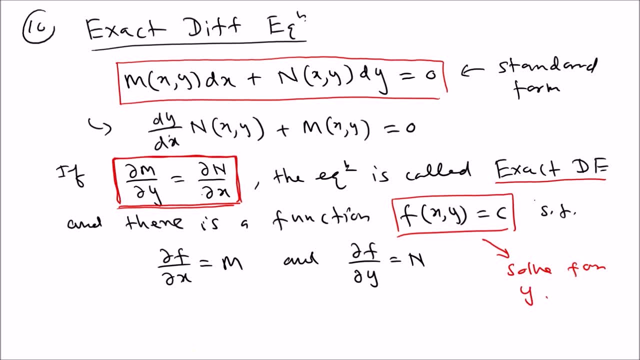 function for y. so that's what we do, and then that y is the solution we are looking for. so let's talk about, let's look at our problem, um, before we do that, actually, let's talk about the solution method. so what we normally do is we're going. 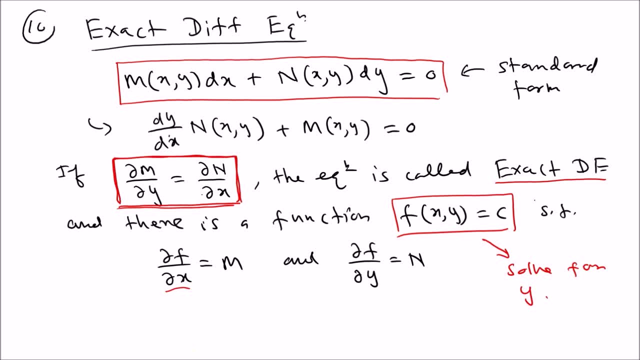 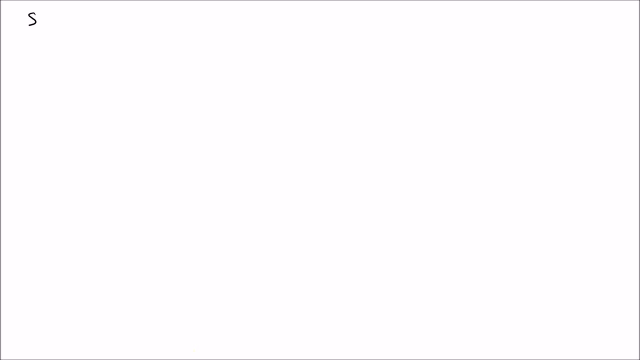 to start with one of those equations- there are two equations- and then take the integral. once you take the integral then you get the function back. so that's the kind of idea. so let's try the steps here. so let's call the solution method solution method. so this is the lendi's argument that we use in differential. 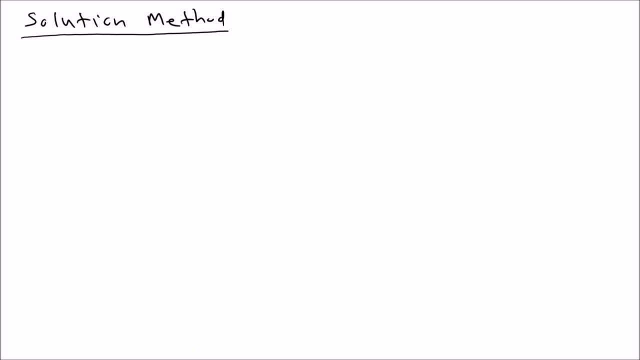 equation: um yeah, so let's say you can pick just one of them. so let's say you uh, you want to use. so let's say you, uh, go with the uh x function, uh x derivative. so let's say you pick that one, so you can just reverse the same. 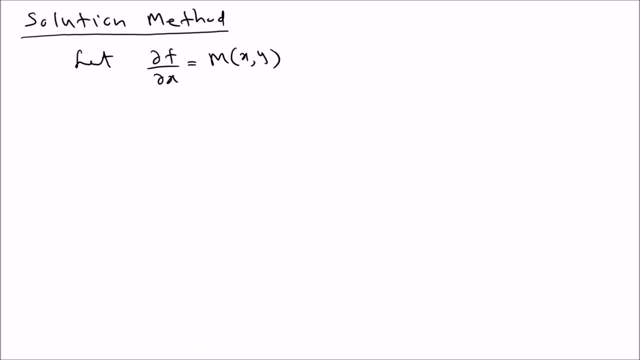 argument. you can just rewrite the argument using the other one if you want, but let's go with this. and then what you're going to do. since this is a partial derivative with respect to x, we integrate with respect to x, so it's very important. so integrate, uh, with respect to x, simply integrate with respect to x. 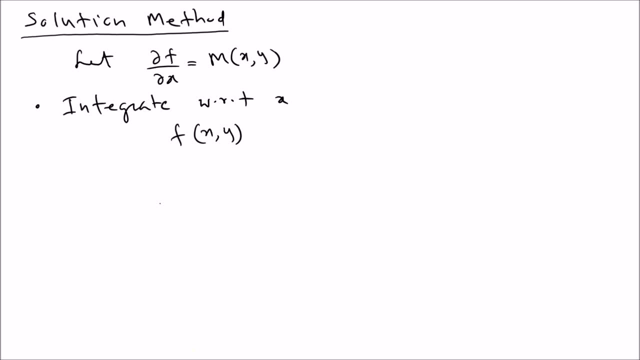 so you can see that you can integrate with respect to x, with respect to x. if you do that, you get the function back. it's a function of x, y is the integral of m, x, y with respect to x. since it's a partial integral, maybe you had a function, only a function of y, because, since you are taking the partial, 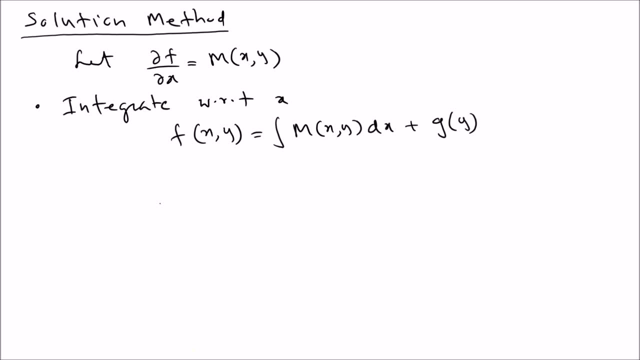 derivative with respect to x to find a double f of a double x. maybe there was a function of y alone. so we just put that back in. so that's a new term. it's not a constant, it's a function of x. so we just put that back in. so that's a new term. it's not a constant, it's a. 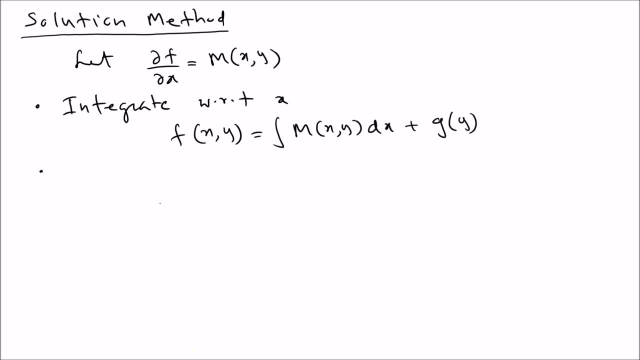 function of y. now what we're going to do? you're going to combine the two, so we're going to differentiate this one, so differentiate with respect to y variable. so if you do that, then you're going to get da by four, by y. that means you're going to integrate, whatever the answer you get. 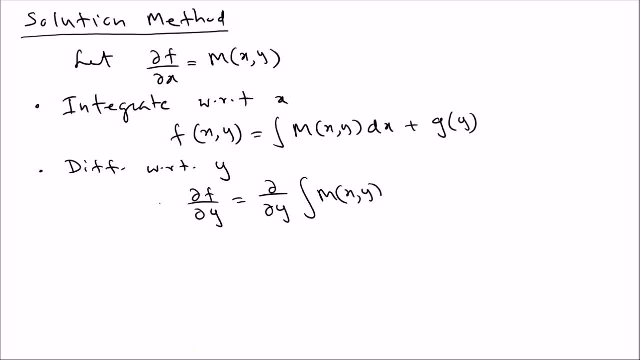 uh, with respect to y, because the function of x and y we want to integrate with respect to x. so what will happen here? it just becomes this regular derivative because the function of y only. we don't need partial derivatives. now, what we can do, we can solve for gy, but the goal is to find this: 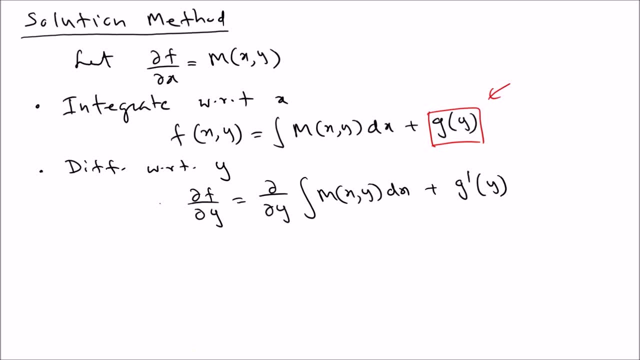 that's the only thing we don't know. so the goal is find. okay, that's the goal: find this. so now what we can do. we know that this should equals the uh, the ny function, because this is the partial derivative with respect to y. this is exactly the n, x, y function, so we: 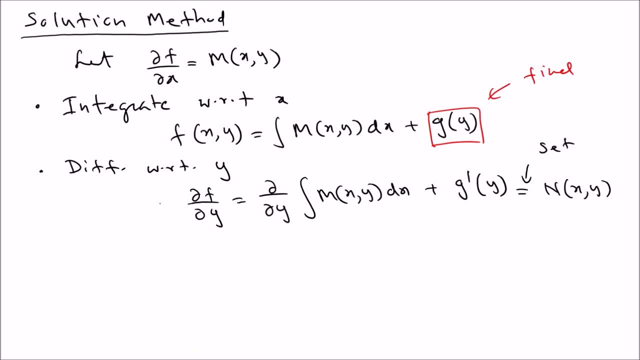 we can set this equal to this, now what we're going to solve for g prime y, okay, or simply solve for g prime y because we can find it, because it could be a match. then you can find g prime y and then integrate and find gy. so the next thing is: 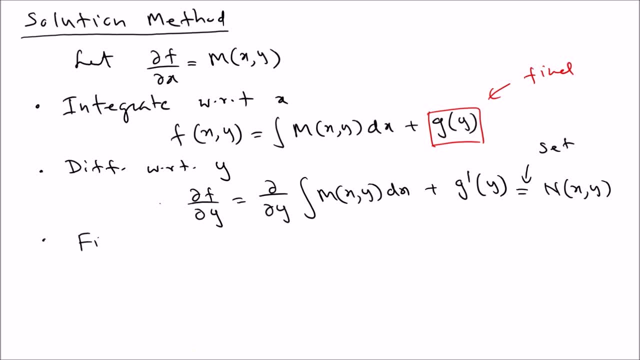 first find g, prime y, and then uh solve for or integrate, and then we can integrate that: first find g, y and or let's. let's write like that: first find gy and and integrate- it's a derivative- integrate to find g y. now what we can do, we can substitute that in the uh. 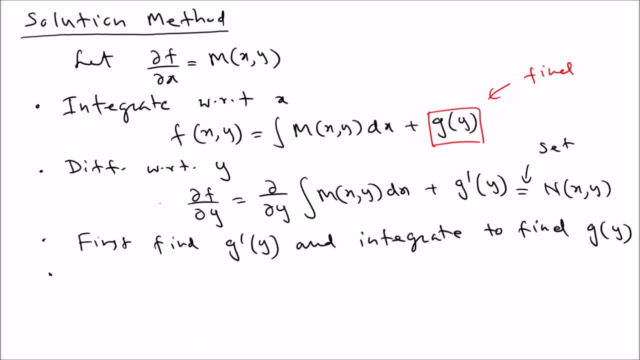 just the function above once you substitute that there. so what we can do, we can substitute the substituting, substituting we have f, x, y function, so we can substitute here. we know this part, plus now we know g y, because we found that above. okay, now we are done yet, but we know that the function, what we're going to do, 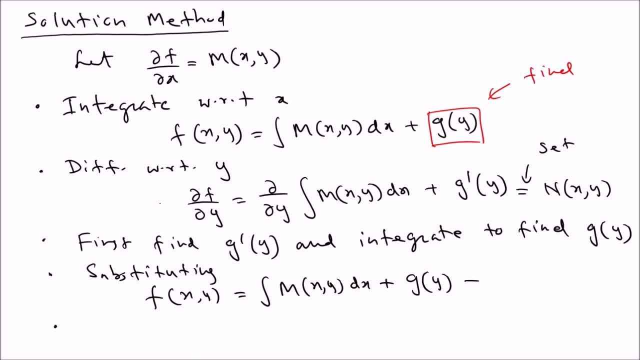 we're going to set this equal to- uh, we can say this- equal to a constant, because that's the function we are looking for. we know that there was a function which is f, x, y is equal to cons, to a constant, so we said that and then solve for. 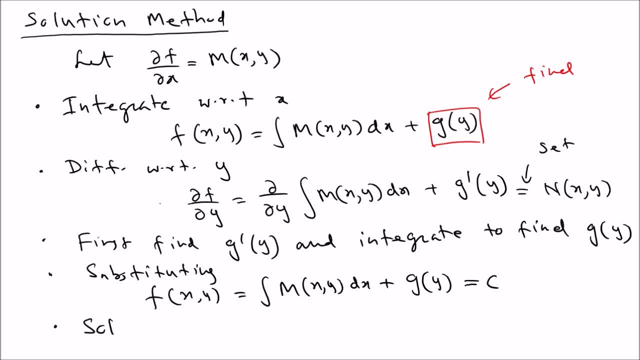 y if possible. after that, what we're going to do? solve. solve for y if possible, because sometimes, uh, we cannot do that, uh, but if you cannot do it, you get a implicit solution for y. so you get implicit uh solution for y, but if you cannot solve, it's an implicit solution. 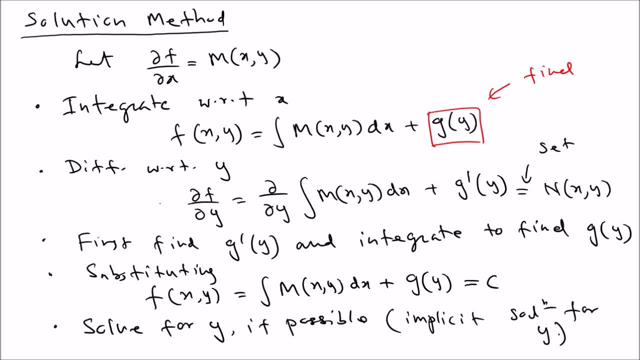 so that is the solution method. i know it's little lengthy, uh, but that's how it works. and then we also talk about the other things. so let's talk about a shortcut method, um, so i'm going to discuss that, so so you can use that if you remember. 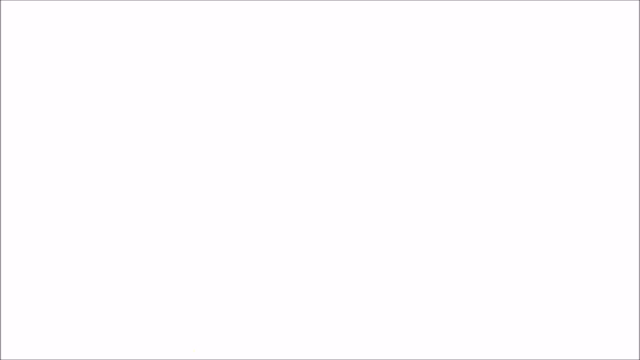 uh, that's, that's not. that is difficult, it's very easy. so let's talk about the shortcut method. uh, so the shortcut method. uh, so what was that? so i'm going to write that you may use, you may also, you may also use the shortcut. uh, so what's the shortcut method? uh, we can start with daba f over daba x. 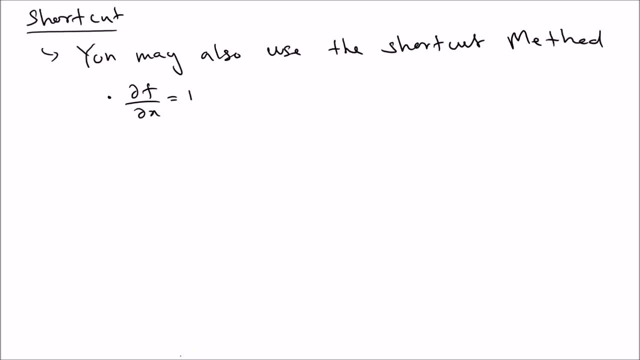 equal m, x, y function, and c is the partial derivative with respect to x. what we can do, we can integrate this one with respect to x. so integrate uh with respect to x. once you do that, you get a function. so what happened when you do that? uh, give me some space here. once you do that, 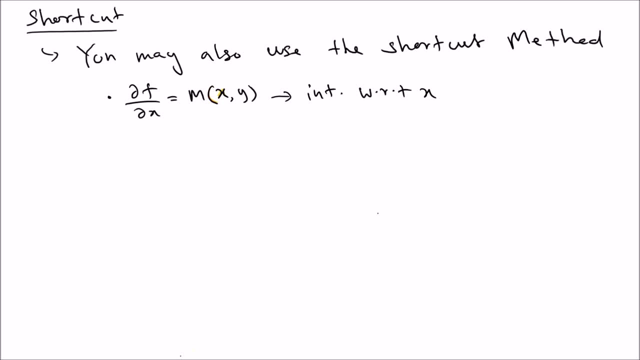 uh, you get a fun. you get the function f x y. so you get the function f x y. so you get a function you just integrate with respect to dx. so when you integrate you can see that. you can see. simply consider: uh, y is a constant, so you get some expression. 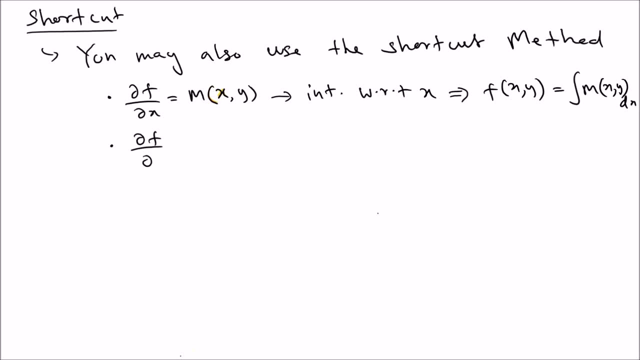 and do the same thing. so what we do, double for double y, which is n, x, y, what we can do with this, you can integrate with respect to y, so you again get the same function in another form. so here what we did, uh, we did the partial integral with respect to y. 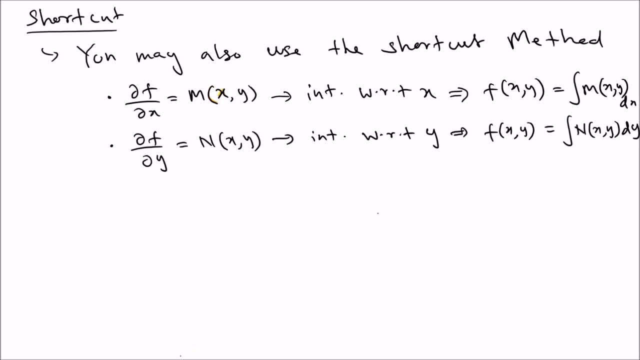 now what we can do. we can write the common terms once, uncommon terms once. so your function f is simply: you write common terms, common terms and uncommon terms once. so that's the uh argument. so after you get that now what we can do, as before, we're gonna set f, x, y to a constant. 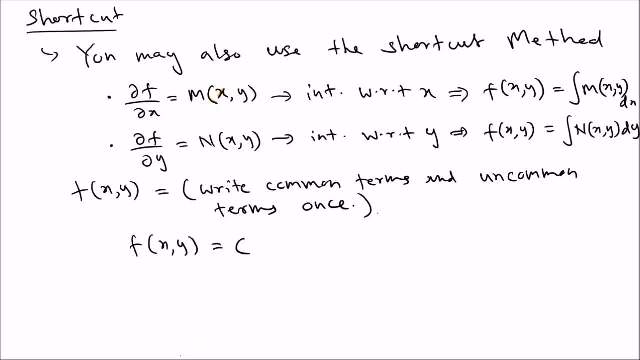 and then, uh, after we do that, after that, what we can do, solve for y, if for super, okay, so that's the, that's a shortcut. um, so you start with w for double x- integrate with respect to x. you go with w for double y- integrate with respect to y, and then you get two expressions: you 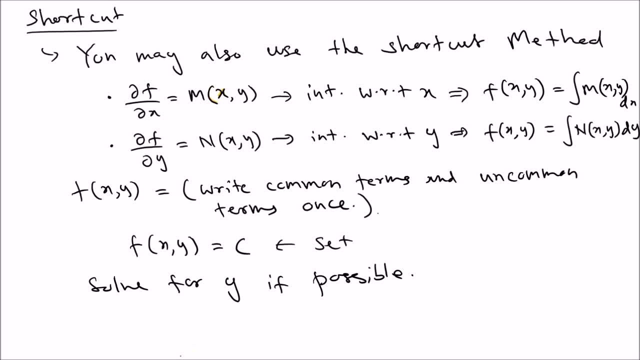 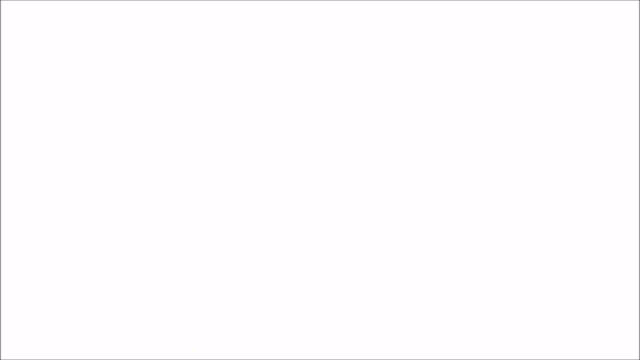 write the common terms once, right the common term, so you can see some common term once an uncommon term. you write the common terms once, an uncommon term once. that's the function f, x, y. you say this: equal to 0, solve for y is possible. so let's look at a problem. 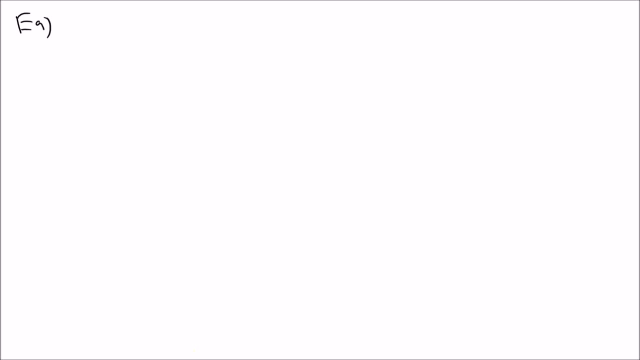 so this is so. let's say, solve 3 e, x minus y, squared dx plus 3 minus 2 x, y plus sine y a d, y equals 0.. so if you get a problem like that, the first thing that we do is we check whether this is exact. so this is the m function. 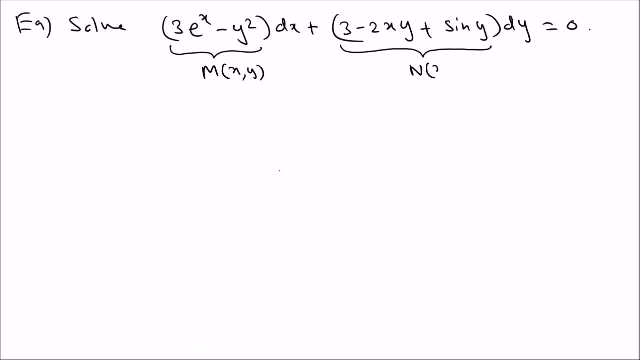 this is the n function. so what we're going to do? ah, we're going to check, we're going to do the test here. so the test is: we can do daba m over daba y. remember the m function, do with respect to the other one. so daba y. 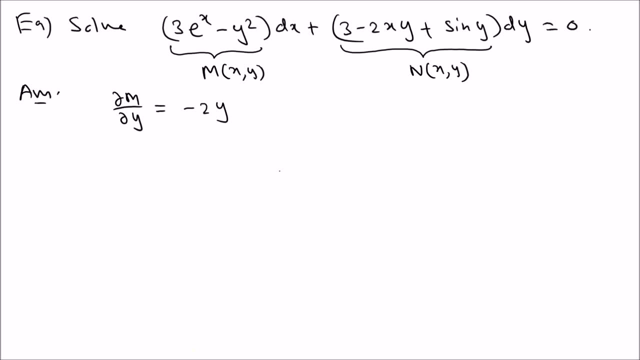 so, which is negative to y, and you can see that that's exactly. equals to daba n over daba x. ah, if you select to x the constant, the sine term goes away because it's a partial derivative. you get negative to y, so they are equal. that means it's a exact equation. 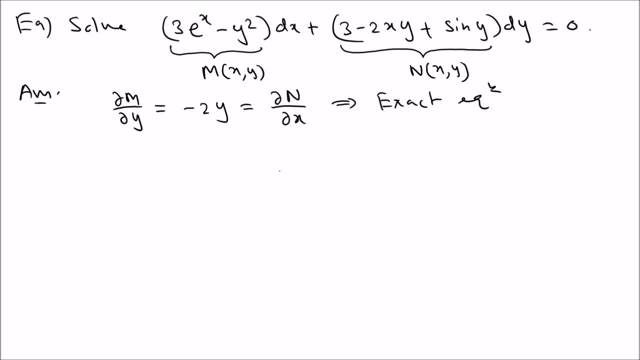 okay, that's an exact equation. so that means um, so, so that's, that means that. so there is, there is a function, there's a function z, f, there's a function z which is simply f, x, y, f, x, y, such that. so there's a function z which is a function of x, y, such that 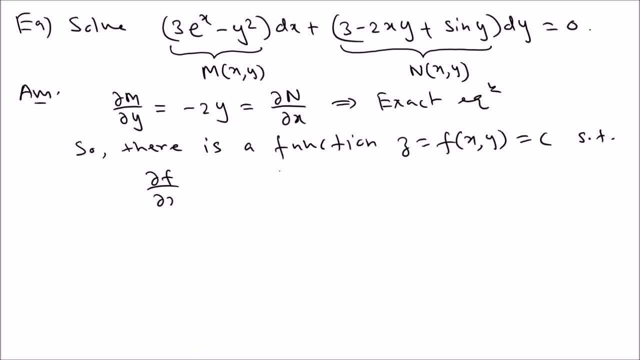 tau by f over daba x equal the m function, which is 3 e x minus y. now what we can do: we can integrate this back to x. so integrate, uh with respect to x. so if you do that, you get f x y. if you integrate with respect to x, it is 3. 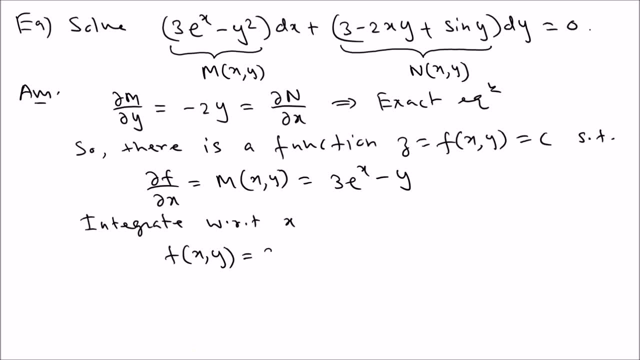 e, x minus um. this is y minus x, y squared plus g y, because we don't know whether there was a function. so i'm going to call this equation number x: 1. now what we can do. we can differentiate this one, differentiate with respect to the other variable. 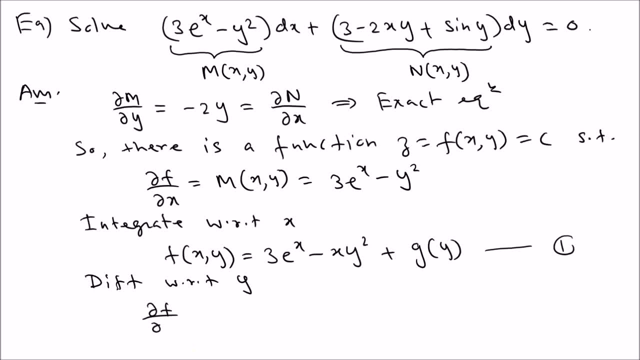 y. so if you do that, you get double f over double y. if you differentiate with respect to y, this is 0 minus 2 x y, because it's a y. so you get 2 y with minus x, you get minus 2 x y, and then um. 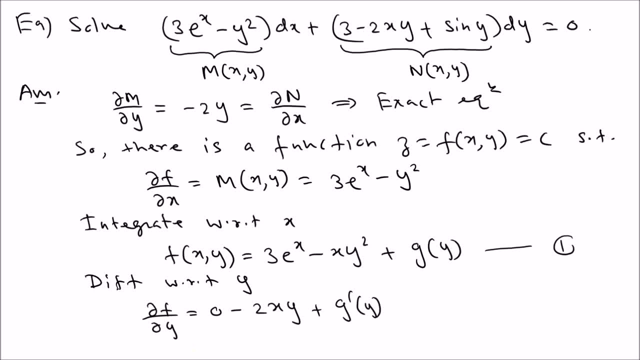 plus g prime y, because it's a function of y only. so it's just the regular derivative. now we're going to set this equal to the nxy function, because we know that by the theory there is a n, x, y function. we can set it uh. 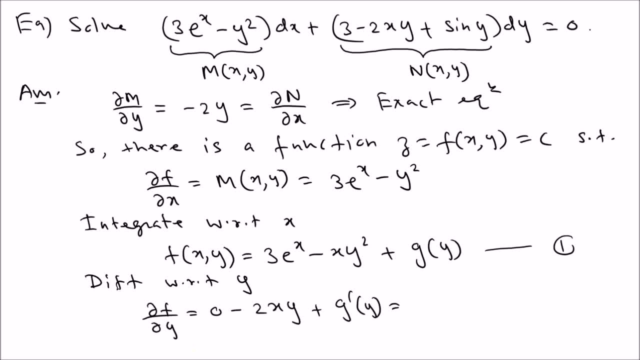 you set to that: ah, so it is 3 minus 2 x, y plus sine y. so it's clearly. you can see that, uh, this function has to be 3 plus sine y, but when you set them equal g prime y has to be 3 minus sine y. 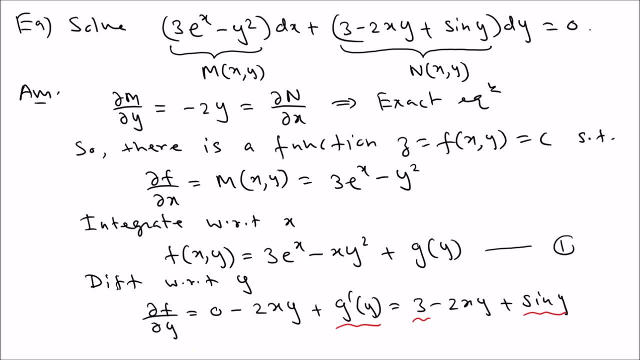 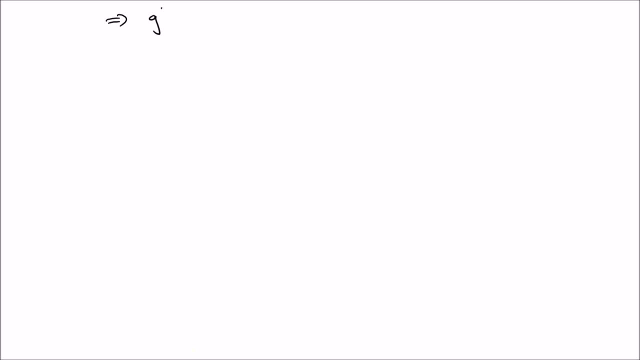 because they are equal to each other. good, okay, so we know that. so that means so this implies that g prime y equals to 3 plus sine y. now, what we're going to do, we can integrate with respect to y, so integrate ah with respect to y, and if you do that, you're going to get g. 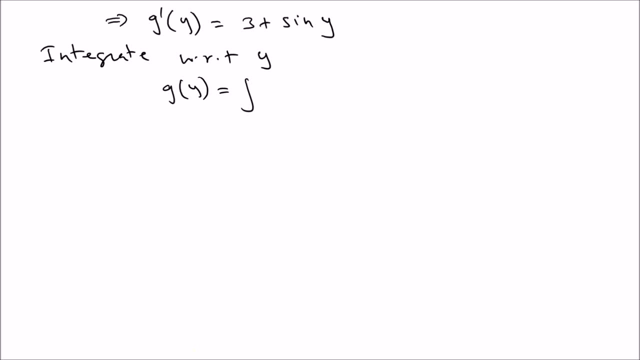 y equals to the integral of g prime, y, d, y, ah. that means if you integrate it's a simple uh integral with respect to y. so you can see that you're going to get 3 y plus. this is sine. so sine means negative cosine, negative cosine y, and we are not adding plus c here. 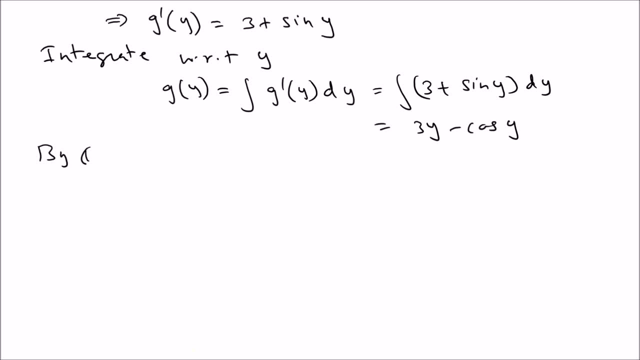 now by equation 1. since we find y, we can substitute by equation 1: f x y equal 3 e x, 3 e x minus y, squared x plus 3 e x, 3 y minus cosine y. so that is the y g y function, that is gy response. 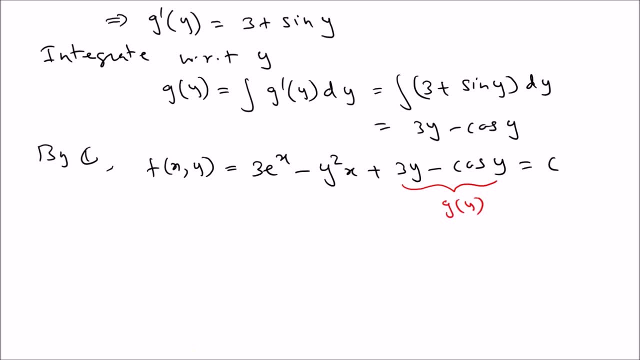 so what we do, are we going to set this equal to c by theory. so that's a constant function- f, x, y that satisfies those conditions. so now what we can see. there's no way you can solve for y, so then the implicit solution is the implicit. solution is given by uh. it is because if f, you see, value of y is labels are equal to right, that's positive, all right. so we find that there's no EST, that again there's no vote in river. so we shall, we solve it. we decide there's no счит Greece, which is 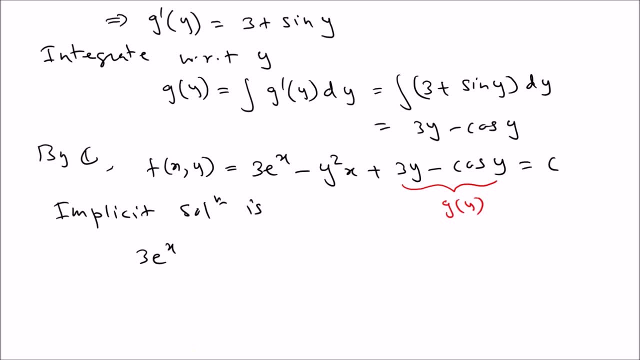 three squared, because c is the root square, which is half square. so if what you 3 e, x minus y squared, x plus 3 y minus cosine y, equal constant. so that is the implicit solution for y. and you can see that, uh, since we have the cosine y term and the y squared, there's no way you can. 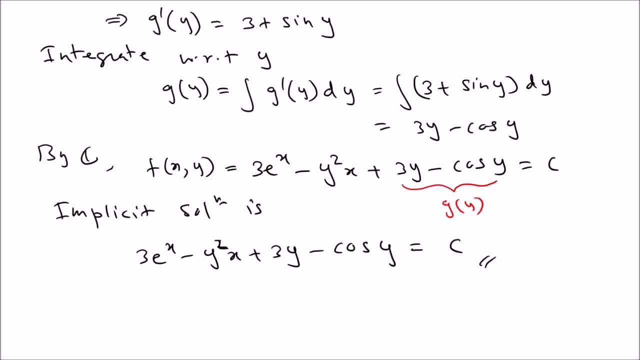 solve this for y, but if you do not have cosine y term, then you can solve this for y, because you can use the quadratic formula um, and then you can solve for y, but since you have the cosine y term, we can solve. good, so this is how this is. 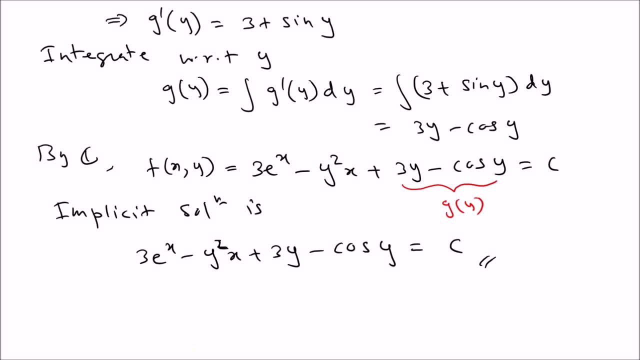 how we solve an exact differential equation. so next we can talk about what, if it is not a exact equation, so what we call the almost exact equation. so we're going to solve that next. so next, next, talk about how to um solve almost exact equations. so almost exact. 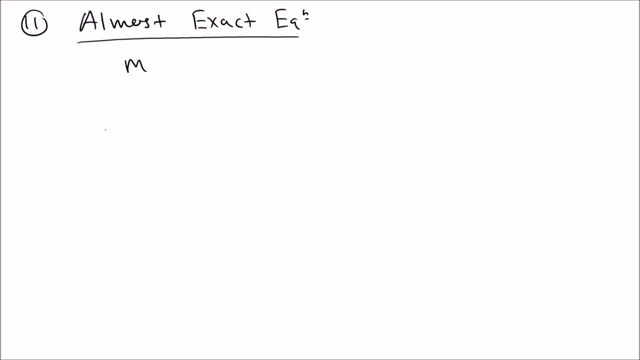 so what's going to happen? uh, if you look at the standard form of the exact equation, m x, y, d x plus n x, y, d, y equals zero. so what can happen? when you take the partial derivative, the first one with respect to y, it does not equal. 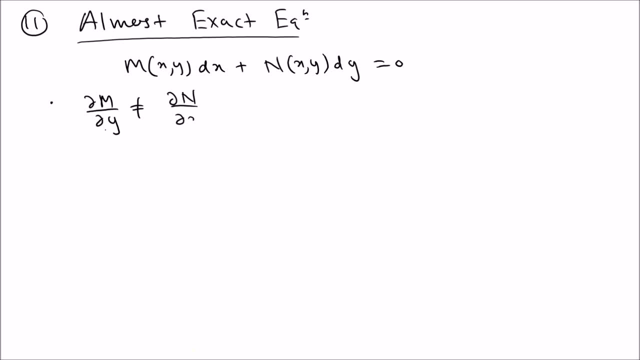 the partial derivative with this of n with respect to x. that's happened. so in this case, you can see that the equation is not exact. uh, it's not exact. so what we're going to do? uh, we're going to use the integrating factor method. so, we're going to use the integrating factor method. 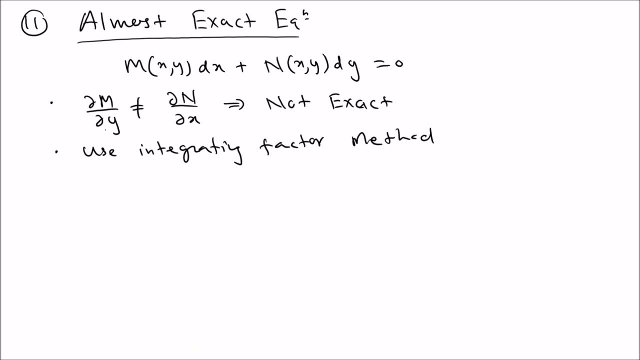 so we're going to integrate the factor method. so there are two cases to consider. we have two cases, so um. so the first one is we're going to calculate m, y minus n, x over n. we calculate that if this is a function of x, only if this: 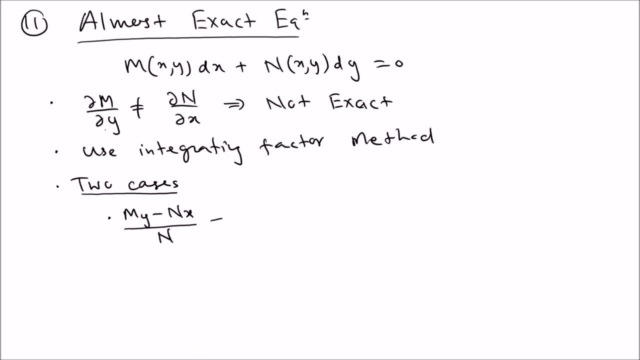 is a function of x only. so let's assume that this is a function of x only. it's a function of x only. in that case we're going to calculate. the integrating factor is also going to be a function of x. uh, which is e to the. we can integrate that expression. 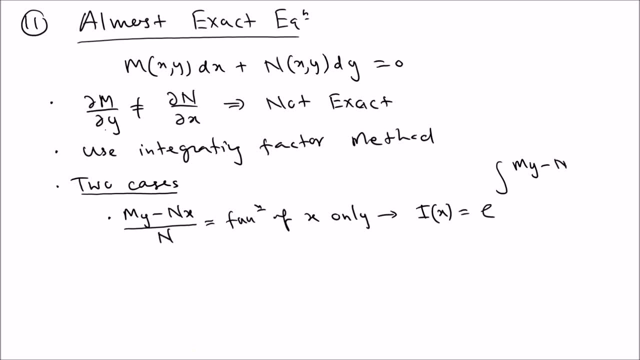 m, y minus n. x over n with respect to x. so that's the integrating factor in that case. the other case is uh n. x minus m. y over m. so this is a function of y. only if this is a function of y, only then you're going to calculate the integrating. 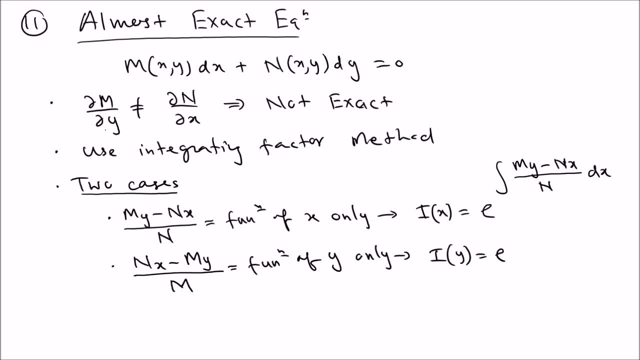 factor i, y, which is e to the. this is e to the y n, x minus m y, over m t y. now, so how you can remember them? um, so you can remember them like this, so you can see: this is uh, uh m n n. the other one is n m m. 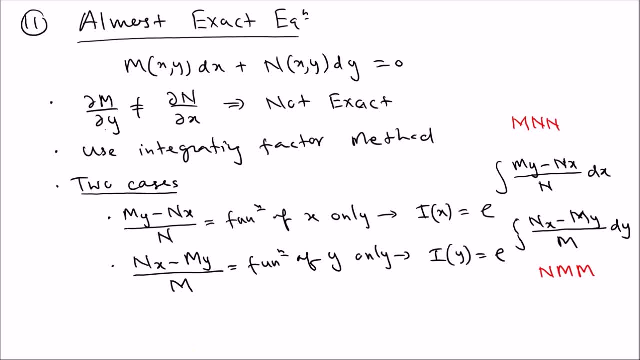 so that's the format of that: m, n, n or n, m, m. um good, and then after we find indicating factor, the, the, the rest of the uh problem is exactly the same as what we normally solve a problem in uh using antigen factor meters. after that, what we can do, then we're going to: 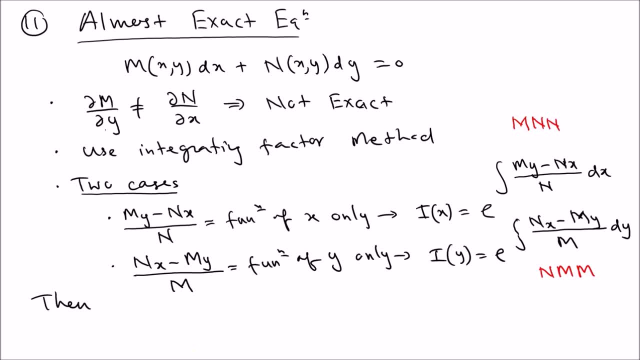 multiply by the indicating factor, then we're going to get i times m? dx plus i times n? dy. so this is m? n, Mn, Nm, NnM, x times Mn. denominated value, building end times m dx plus n- nn. so we're going to follow the exact uh equation argument. this is an exact. 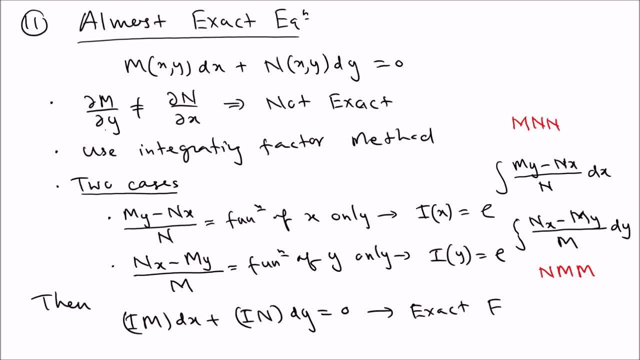 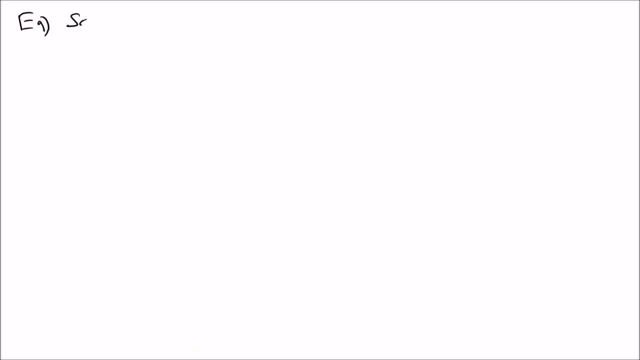 equation. uh, so we're going to follow the exact equation argument. so let's do just one example, just to see how it works. ah, okay, so let's solve this problem. so let's say: solve x, y, d, x plus 2, x squared plus 3, y squared minus 1, d, y equals 0. 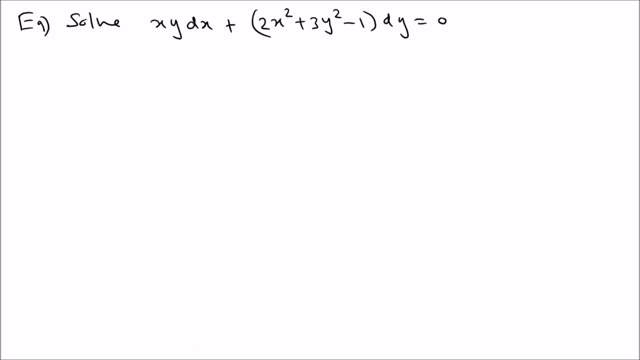 so let's solve that. so, what we are going to do, we're going to pick this as m, we're going to pick this one as n. uh, then you can see that daba m over daba y, which is x, and n over daba y. 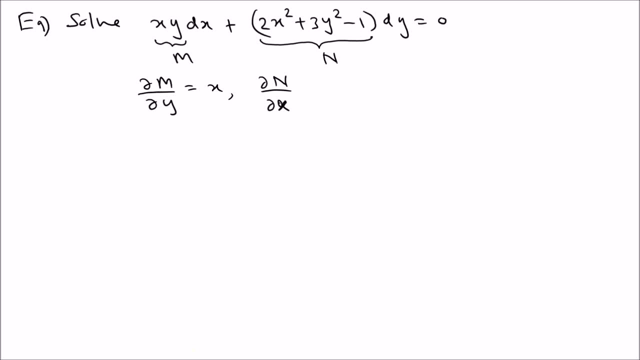 are x, uh, which is 4x, and you can see that they are not equal. uh, so this says that daba m over daba y, not equal to n over daba x. so that means uh, not exact. so not exact also what we're going to do. we're going to see, uh, which one going to work. 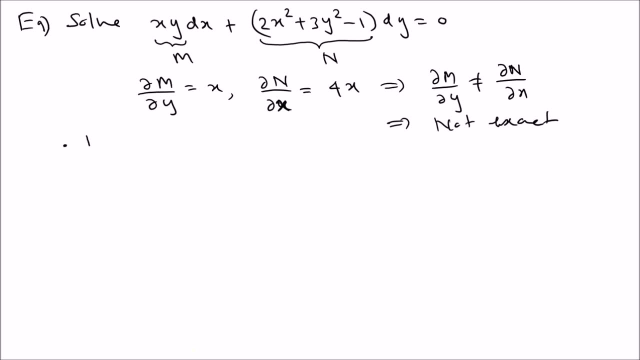 so let's calculate uh, m y minus n, x over n first. so what do you get? what is m y? what is the uh y derivative with respect to y derivative of m, which is x and the minus? let's calculate the x derivative of n, which is 4x divided by n. n means 2 x squared plus. 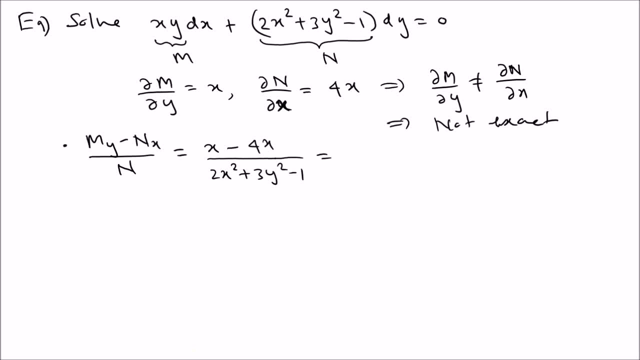 3 y square minus 1, which is: uh, you can see that. uh, this is, this is not a only function of one variable. okay, so you can see that. not a function of one variable, so not a function of one variable. so that means it's not going to work. so let's look at the other one. 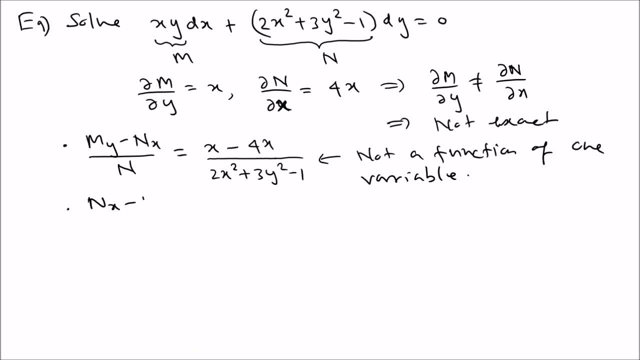 uh, so nx minus my over m. so if you do that, you're going to get nx. that is 4x my. that is x divided by m. now m is x- y. so if you cancel um x, so it's going to be 3x over. 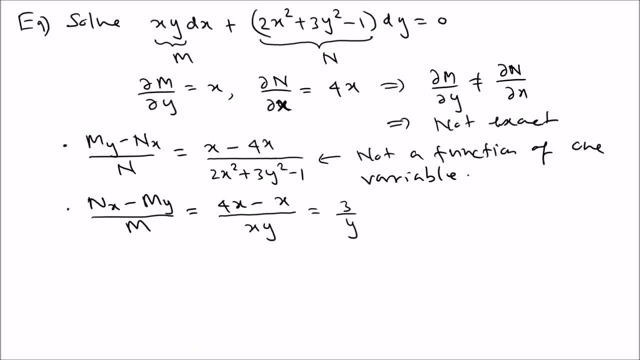 4x a, 3 over y. so you can see that this is a function of um y, only so the function of y, only so. that means we can calculate the, we can find the negative factor. so i y e to the uh, the formula in x minus m y over m d y. 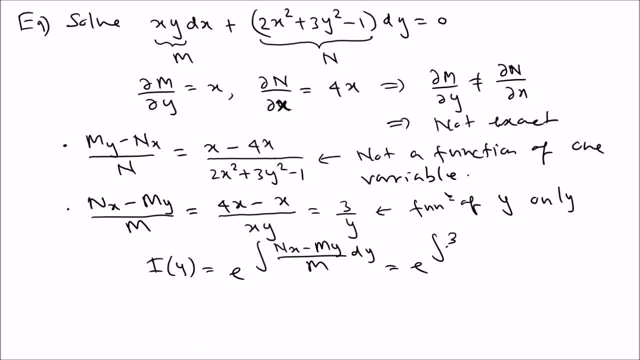 we already calculated that. so it is 3 over y d, y that means 3 l and y. so bring it here. so that means going to be y cube. so y cube is the um indicating factor. so we're going to multiply by that. so multiply by y cube um, the difference will be 3. 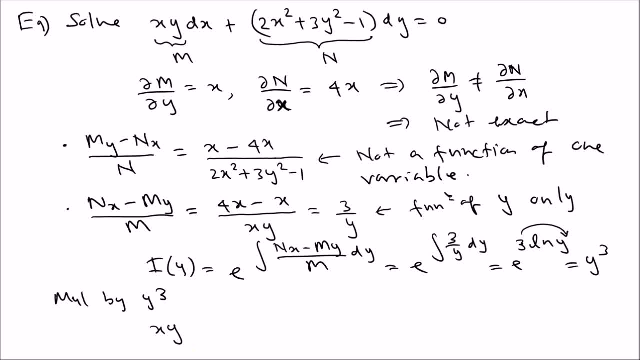 and y will be 4 and y will be 4, and then we're going to get y to the fourth power, d x plus uh, you're going to multiply by y cube, so it is 2 x squared y cube plus 3 y to the fifth power, minus y cube d y. 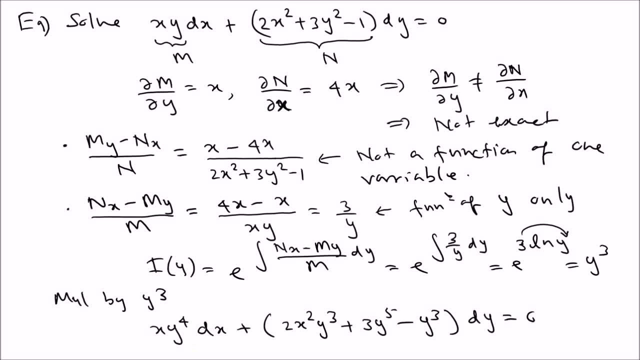 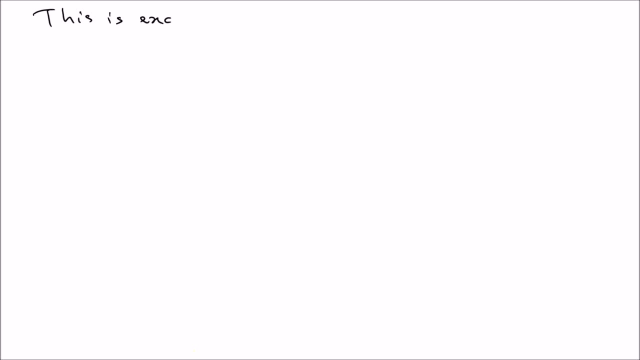 equal 0.. so let's look at and you can see that once you do that, it's going to be exact with us how we pick the numbers. so now, shortcut. let's use a shortcut to get the answer. so this is exact. ah, so we use the shortcut method. so we use 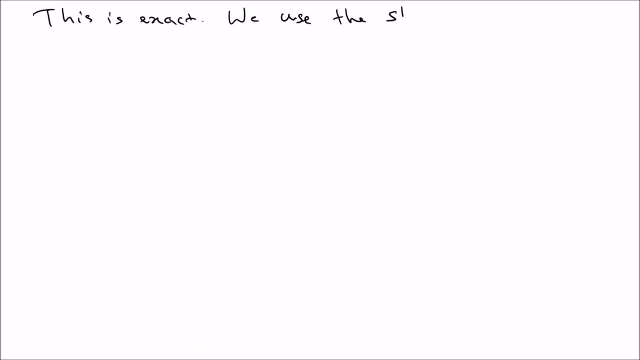 uh, the shortcut method. okay, so let's use the shortcut method. so, if you the shortcut method, uh, what do you get? uh, we're gonna go down by four double x, which is the first function. uh, so we can integrate this one with respect to x. so if you do that, you get f, x, y. 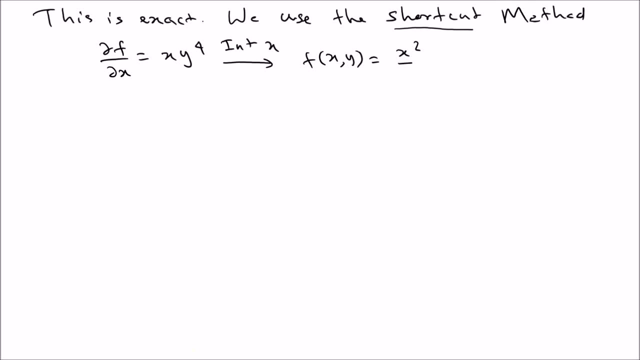 equals to x squared over 2 y to the fourth power. ah, because we integrate with respect to x. so we are not going to add the constants and then go with the other one dot by f over double y, which is the other function, ah, so it is 2 x squared y cube. 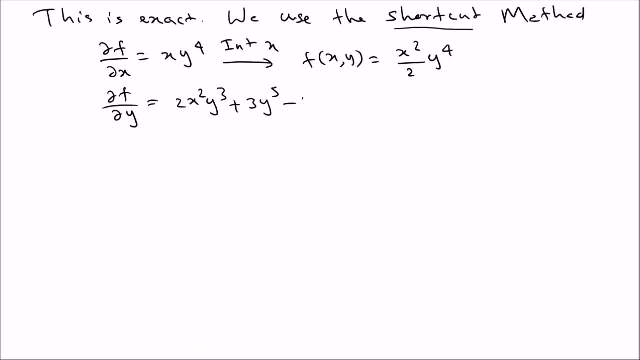 plus 3 y to the fifth, power minus y cube. uh, we're going to integrate this one with respect to y. if you do that, you get f x y. uh, one half x squared y. 4 plus one half y to the sixth, minus one fourth y to the fourth part. uh, now what we can do: your f x y. 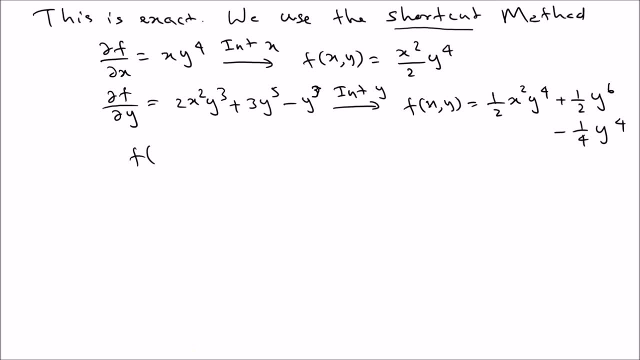 function is we're going to first write the common terms and you can see this is common, so we can write that once. so one half x squared y to the fourth power and they write the uncommon terms. so one half y to the sixth minus one fourth y to the. 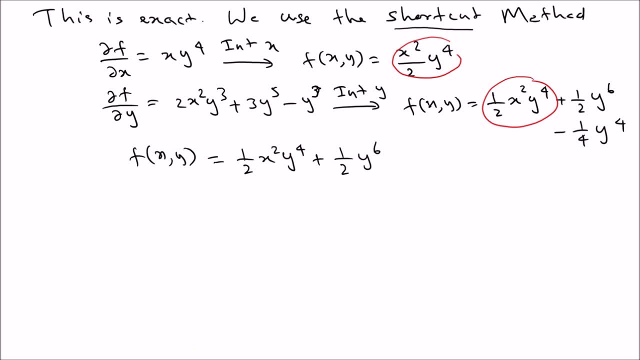 fourth. now what we can do: we set this equal to zero and you can see that, uh, it is not easy to solve this for uh y. so we can write that: one half x squared y to the fourth power. so that means this is the implicit solution. uh, this is the uh implicit. 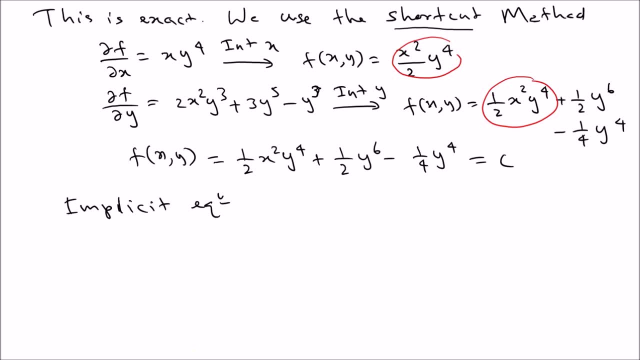 implicit uh equation, implicit solution: the equation for y. so that is the, that is how we solve the uh, almost exact equation and there are, like in our cases, uh, you cannot really solve uh because we only consider two cases: whether m, y over n, x over n, e is a function of x. 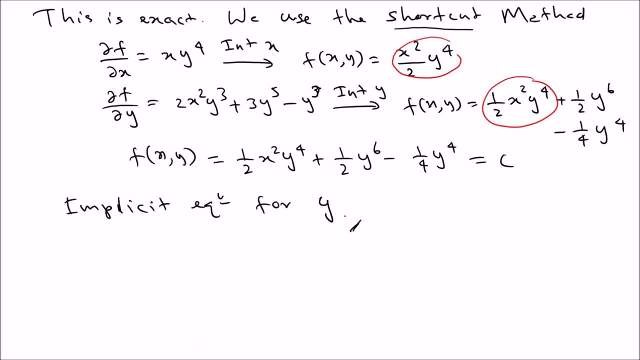 or n, x minus m, y over m is a function of y. what if it is not the case? so that means there are some cases that still give you uh problems, okay, and then there's a video, um, uh, what we normally call it- all in one a video. it's already posted, uh, so so that's the kind of good one that's. 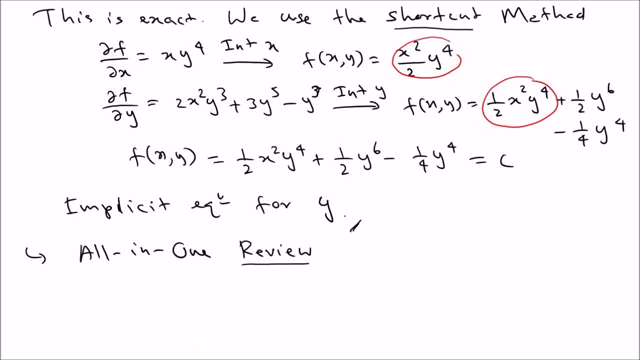 going to give you um kind of all the methods in one video so you can look at. that is in there. I'm going to also put the link to that video all in one review. uh, all in one review for uh, first order equations. okay, so it's going to show you all the uh formulas there. 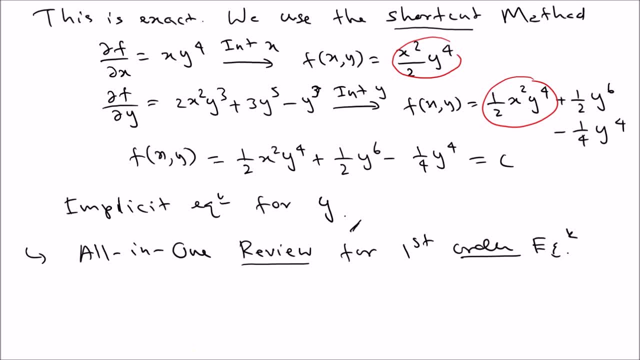 good, uh, now, what we're gonna do? um, we're gonna uh discuss, uh, the numerical solutions, and you can see that there are a lot of equations, uh, that cannot solve. okay, so we're going to do this and we're going to do a lot of just a very small percentage of equation that you can solve. so that means there's. 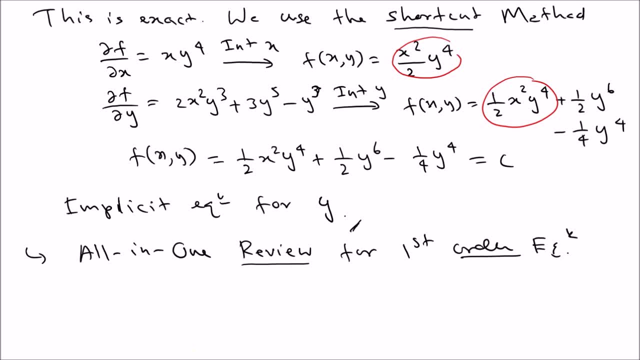 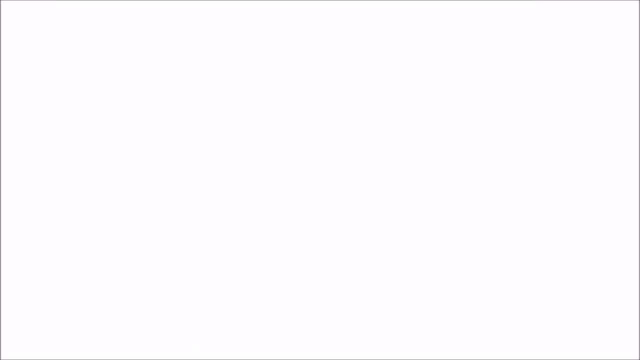 a need to solve, uh, need to find approximate solutions. to find approximate solutions, uh, we're going to use numerical techniques, so let's talk about that. so that is number 12: our numerical methods. uh, numerical methods, uh, in veneto called numerical methods, uh, there are actually. we discussed 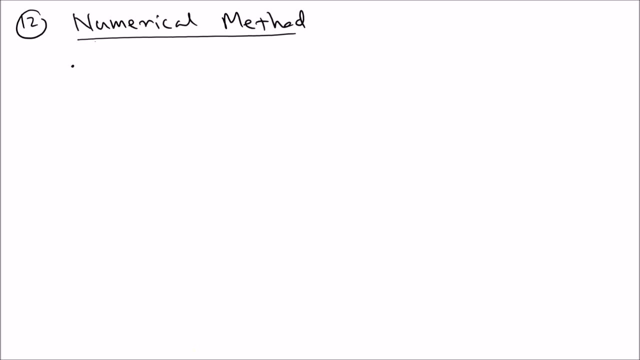 three of them. uh, one is the easiest one, the most obvious one, what we call the euler's method- ah, and then we have improved euler, ah, improved euler's method. and then the very good one, what we call the runge-kutta method. so the runge-kutta method is like very good. it's going to give you answers like: 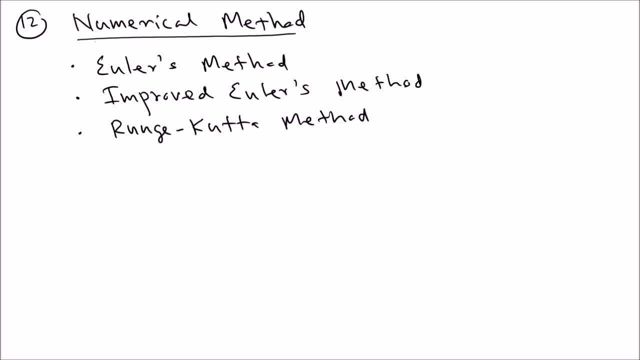 um, excellent uh answers, uh for, uh, certain problems. so let's talk about the uh euler's method. that's the easiest one. euler's method. uh, so how it works. so what's a geometric? uh, geometric method? uh, it's called the euler's method. uh, it's called the euler's method. 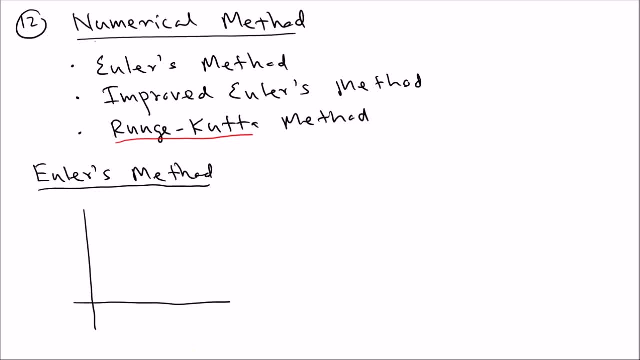 argument for that. so let's say you have a curve, uh, so what's gonna happen? you're gonna. you are given uh, a point and the derivative like the slopes everywhere. so you are given the derivative at each point and a starting point. so that's the only information here. you can find derivative at any point and 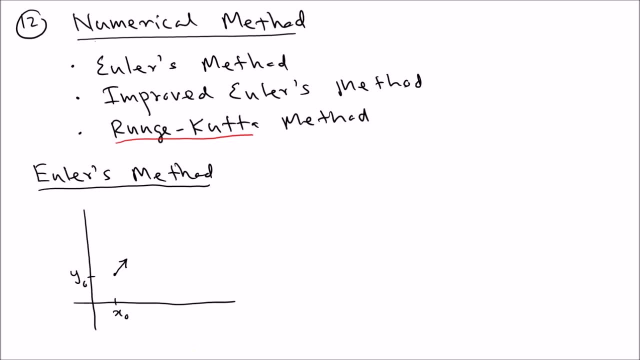 also give you the starting point. so the goal is to find an approximation for another point at some point. so that means um, uh, so the so. so this is the actual curve. so what you try to do, you're going to approximate the value at a certain point. so what we normally do is we're going to 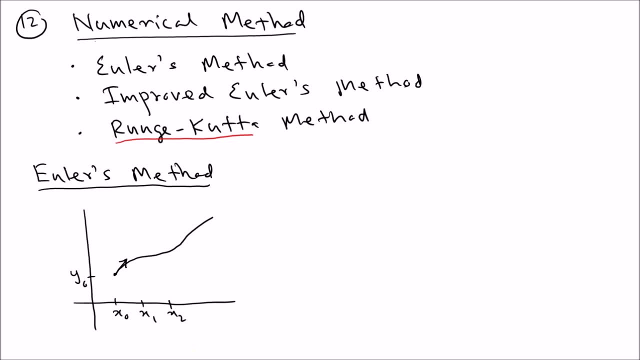 divide this into equal parts, um, and then calculate, approximate the value uh successively. so you're going to calculate y1, uh, that's y1, and then you calculate y2, and then you calculate y3, like that. so, uh. so that's the kind of argument. 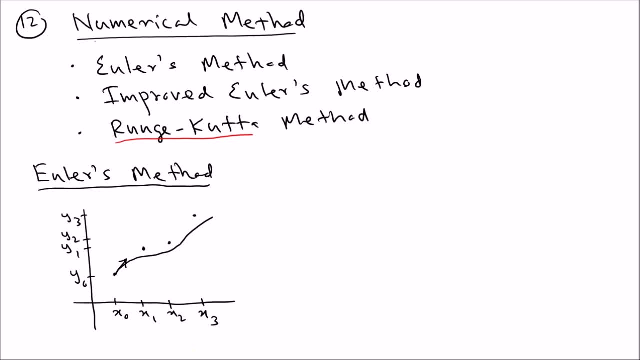 we do, we're going to approximate, uh, one by one, uh, we can look at the tangent line. that's how we do. we can look at the tangent line and then calculate, uh, the next one, uh, so actually, uh, the first one is not exactly correct. so, um, because when you go to the 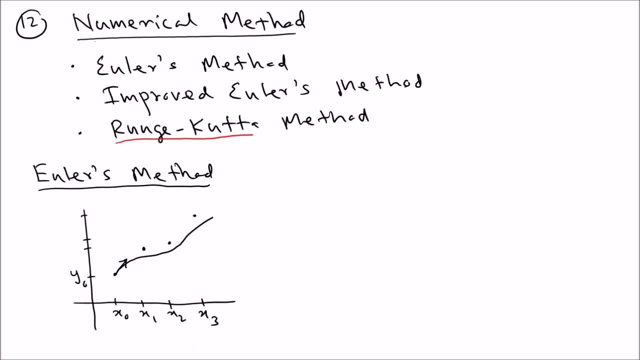 tangent line. uh. so what happened is: let's extend the tangent line. so this is what you get. so that means your first value is here, right here. that's the first one, so that's the first approximation. so that is y1. now we can use that value and also use 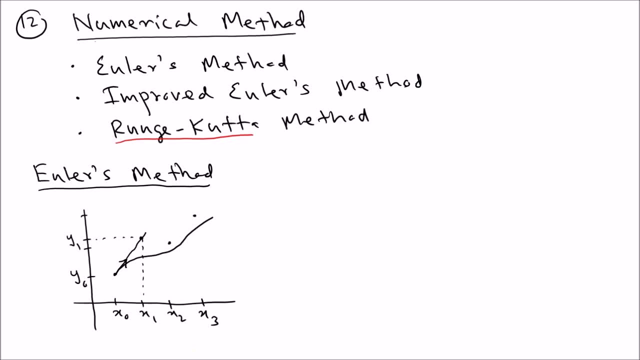 the slope at the point to find the next value. so if you draw the slope at that point, you can see it's going to go like that. so that is y2, that is y2, so like that, uh, we're going to find that's y2. 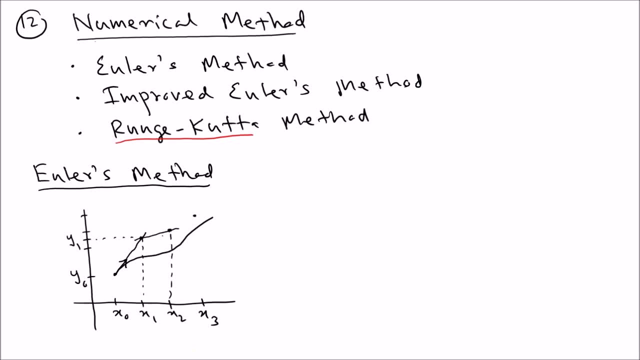 and then we control the slope at that point. so it's going to go right here. that's because i'm going to parallel to that. this is slow, so it's going to give you uh y3. so that's y3. so that's the uh approximate value of y3. 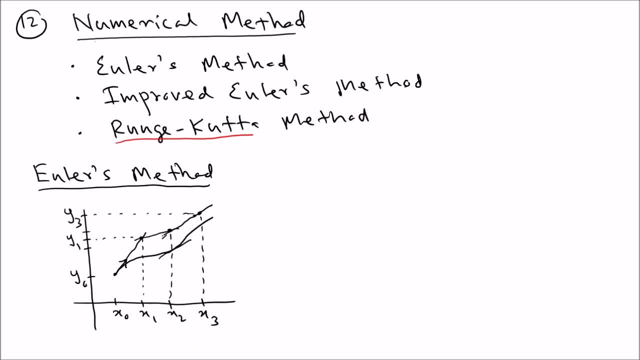 so this is the kind of idea. so you're going to look at the slopes at each point and then use the uh tangent. so the next point. so that's the kind of idea. uh, so what we normally do is we're going to divide this into equal sub intervals: h, h, like that. 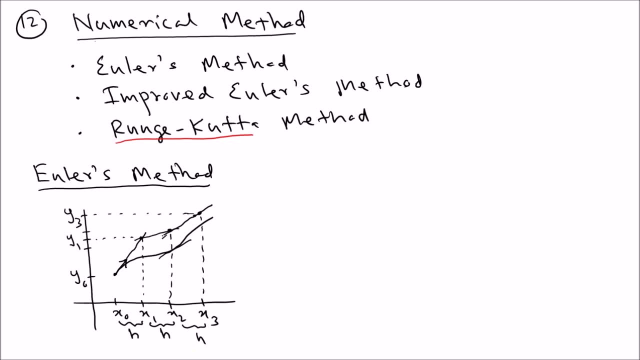 and every time calculate the next point, calculate the next point. so what you are given is simply: you are given d, y by d, x, f, x, y. so that means you know the slope at every point and also you know the star starting point. those are the only things. you are given the slope. 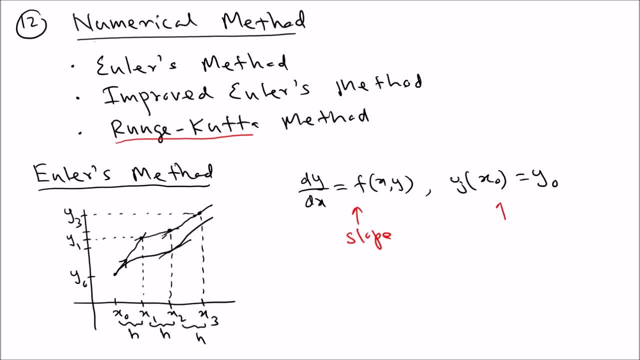 at every point and the starting point. so uh, and then uh, our formula becomes uh, like this: so your n plus 1 node is simply x, n plus the gap, and then your y n plus 1, y current 1 plus h times x n, y n. so that is the scheme for the euler's method. 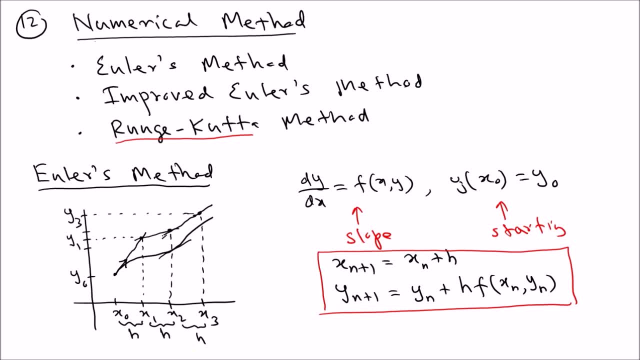 so this is the euler's method, uh formula, and this can work. you can start with: n equals 0. once you plug in 0, you get x 1, and if you plug in 1, you get x 2, 3, like that, depending on what. how many points you need. 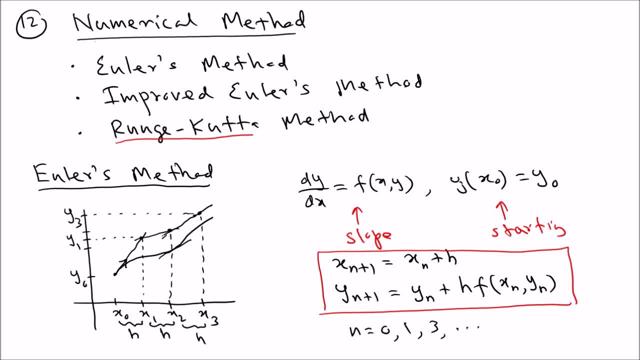 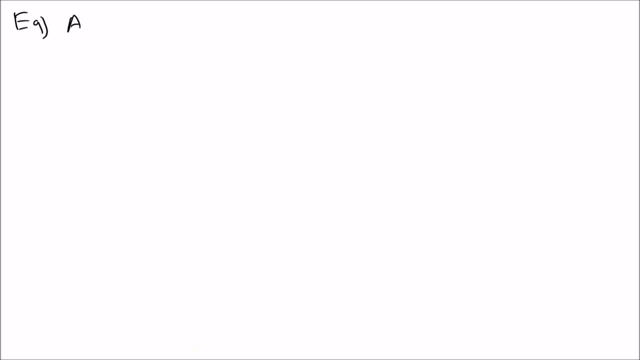 okay, so that's that's it. so that's the euler's method. let's just look at an example, um, and see how it works. so let's look at an example. so let's do this example. let's say approximate, approximate, y2 using euler's method. 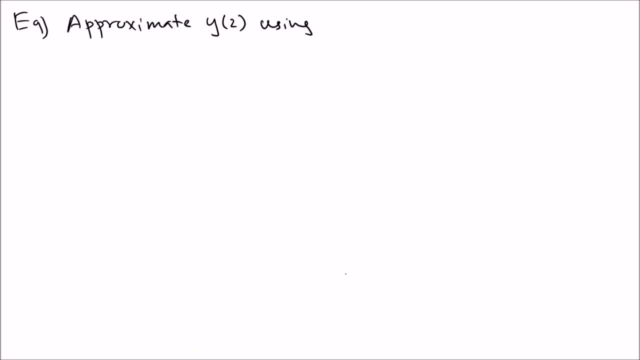 using wireless method. ah, if, given that, if, given the differential equation dy over dx equal, let's say 3, y minus x and y equals 1, equal minus 1 and the gap, the step size, 0.5. so it's a kind of problem that you can get, you can. difference equation initial. 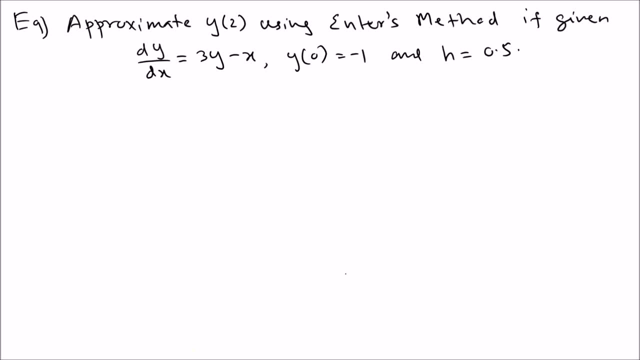 condition, and h. so uh, it is always a good idea to kind of um try to understand what's going on here. so we have x- 0, that is starting value, that is uh 0. and then we have y- 0, that is the y value. so how much value do we have? 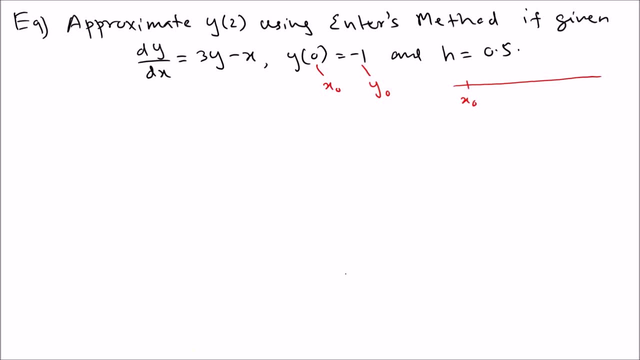 added. so how many we need to calculate so you can see that x: 0 is 0 and then we're going to go in 0.5 steps. so that means we have 0.5 and then 1, 1.5 and 2. so in a couple at 2. so that means 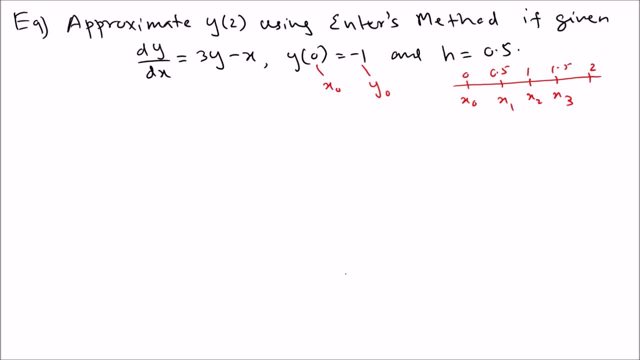 x 1, x 2, x 3 and x 4. so so, knowing x naught and y naught, you want to calculate y 1, y 2, y 3 and y 4 and x uh four more. so let's look at the uh situation here. 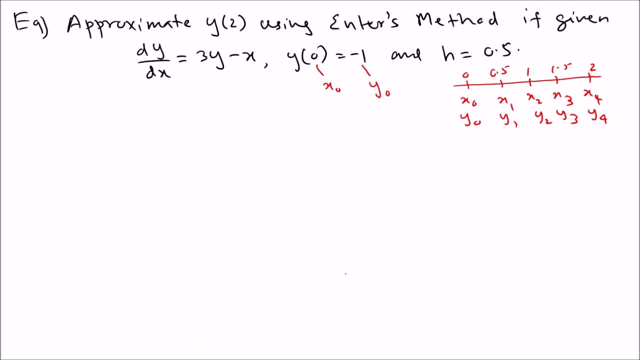 so uh. so what we have is so uh the answer. so what we can do, we're gonna first identify what is the x uh y function. so you can see it is 3y minus x. that's the xor function. now we got a scheme. so what's the scheme? x n plus 1 is x n plus h. 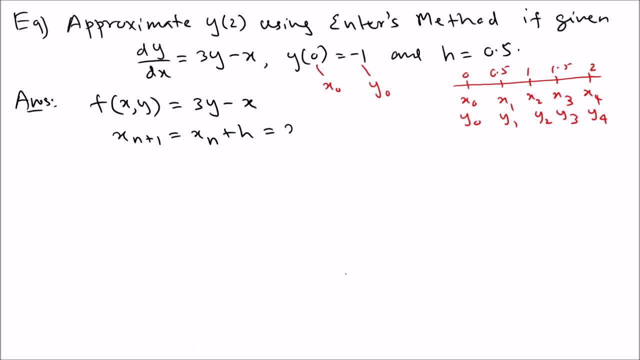 so in this case it is uh, x n plus 0.5. so every time you increase by 0.5 and then y n plus 1, which is y n plus h, ah, f, x, n, y n. so let's plug in and simplify so. 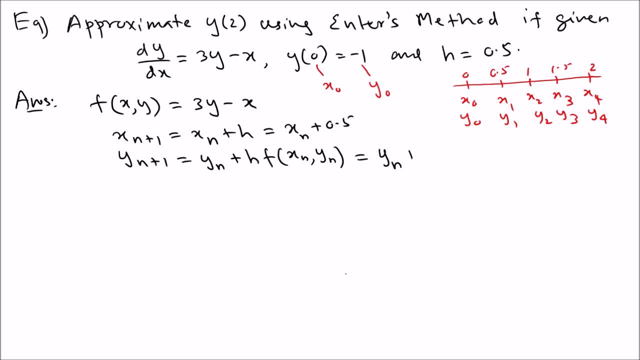 this is y n plus h. n plus h is 0.5. uh, the function is 3 y n minus x n. so you plug into the function because that's a function, so plug in for that. now what we can do is we can simplify. if you simplify this, what do you get? 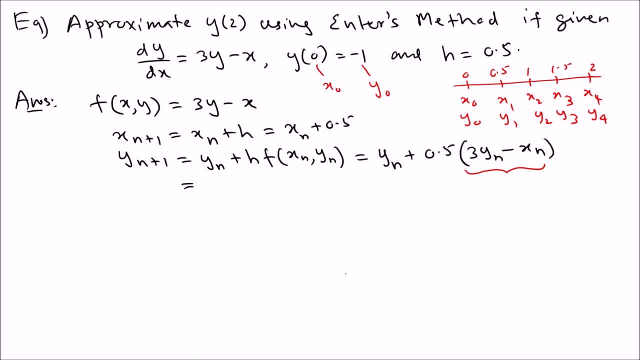 you're going to get. 0.5 times 3 means 1.5 plus 1, so it is 2.5 y n minus 0.5 x n. so that is the formula that we're going to use for each n. so we can start with: uh, we have x naught, which is: 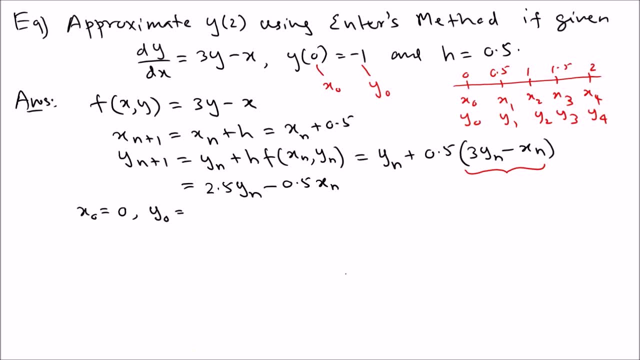 0 and we have y naught, which is negative 1. now we're going to start plugging the value. start: the first value is 0, because when you plug in 0, you get x 1. so when you plug in 0, you get x 1, which? 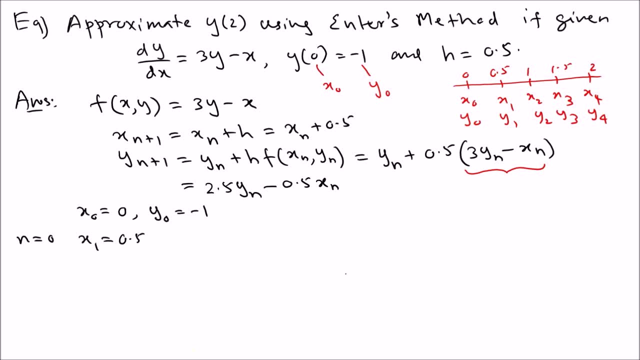 is you add 0.5, so it is 0.5 and y 1. uh, the formula says it is 2.5 y naught minus 0.5. uh x naught. since you know the two values, we can plug in. so it is point: uh, 2.5 y naught is negative 1 and then 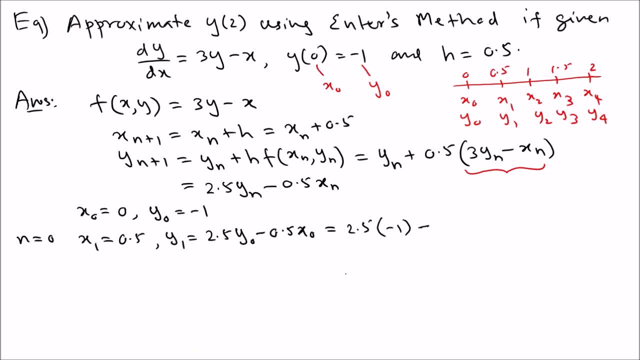 yeah, y naught is negative 1 and then the- uh we have 0.5 times x naught is 0. so if you simplify so you can use a calculator for that, you're gonna get negative two point five. so that is the y one value. so keep doing so. now you plug in equal. 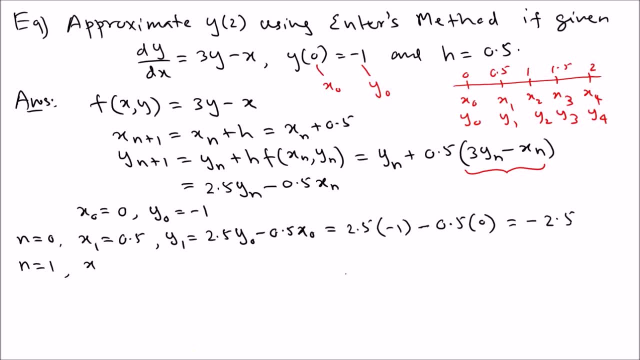 one. if you buy an equal one, you get x 2, which is a 1.0. uh, we have y 2 now, so it is 2.5 y 1 minus 0.5 x 1. since we know um y 1 and x 1, we can plug. that's coming from the. 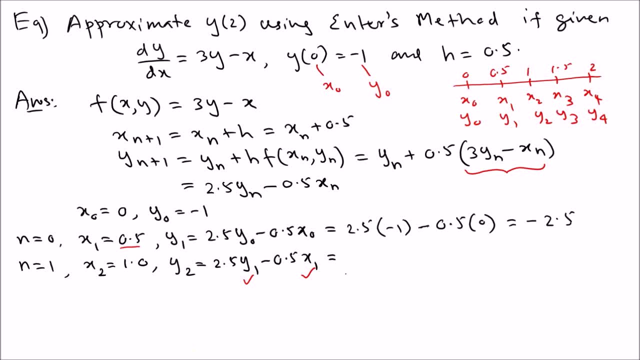 previous table. it's always those two coming from the previous step, so we're going to plug in those two. so you get 2.5 y 1 means negative, 2.5 minus 0.5 x 1 means 0.5, always coming from the previous step. so 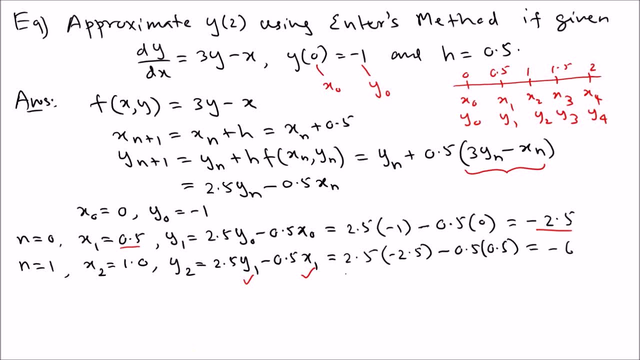 if you use a calculator, you get negative 6.5. go to the next one, n equal 2. so this is going to give you x 3, which is 1.5. this is going to give you y 3 value. according to the formula, it is 2.5. 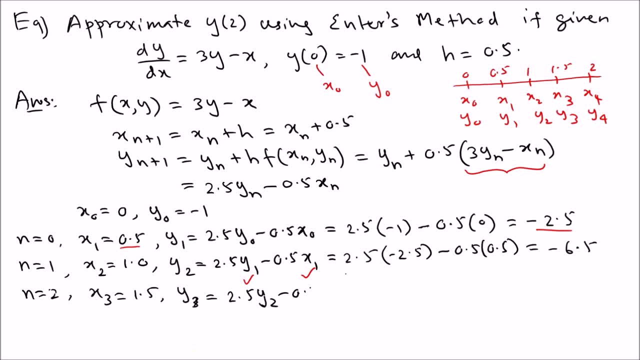 y 2 minus 0.5 x 2. uh, we know all the values from the previous step. so it is 2.5 negative 6.5 minus point uh, five, uh, and then uh, the value of x 2 is 1.0. 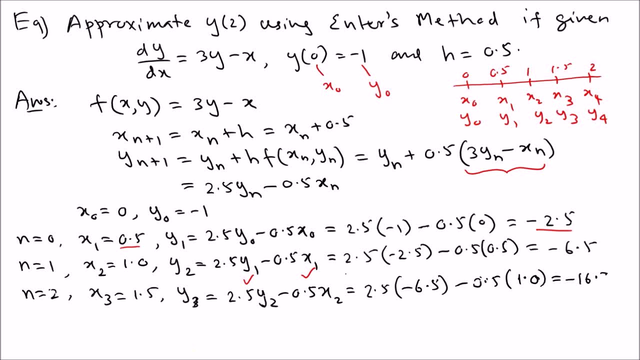 x 2 is 1.0. now what we're gonna do? we're gonna simplify again, so you're gonna get negative 16, 7, 5 is a calculator, and then we can find equal 3. you get x- 4. that means that's exactly the number we want. y. 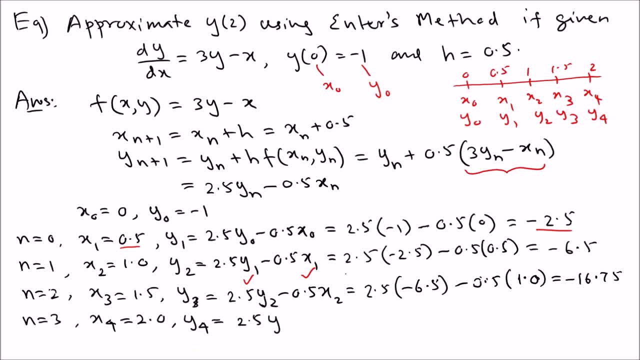 4. that's the value we're looking for. again, it's the same formula- and a 0.5 x 3- we also know that, so let's plug in there. so you get 2.5 negative 1675 minus 0.5 and then 1.5. 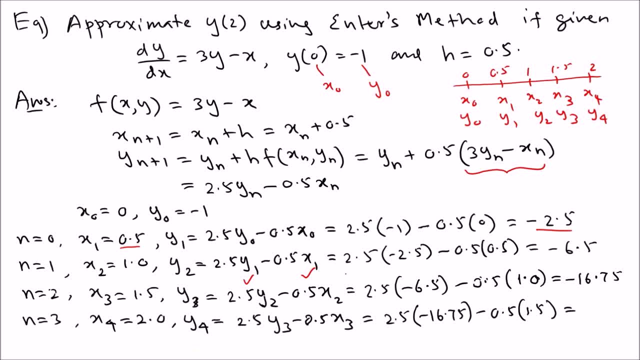 so if it's a calculator, uh, you're gonna get negative 42, 6 to 5, uh. but this method is not very accurate so you don't need this many decimal point. we normally leave like just one decimal point. so that means your y2 value, which is: 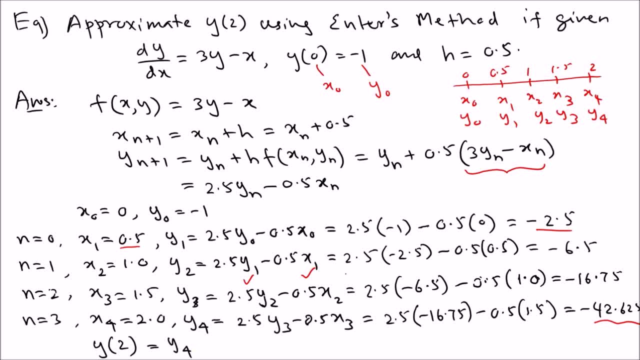 the y. fourth y2 minimum is the y4 uh. it's approximately equal to negative 42.6. okay, so you can see it's not that difficult. so it is always a good idea to uh get this first, uh, because then you can see that you can simply plug in there uh every time, rather than 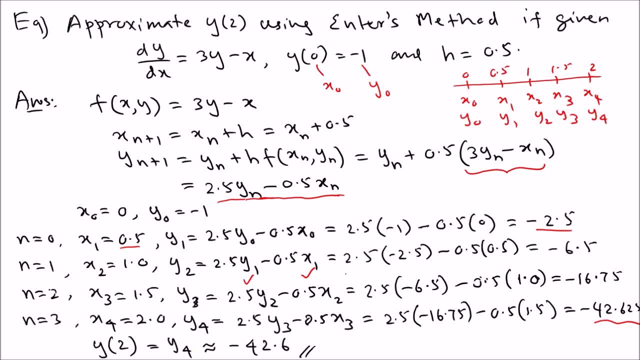 using the original equation every time. so always try to simplify that first and then use that simple equation. this is much, much uh easier, okay, so, uh. so this is how you use the euler's method to solve, uh find the approximate solution. so next what we gonna do is we can discuss the most uh correct version, what we call the. 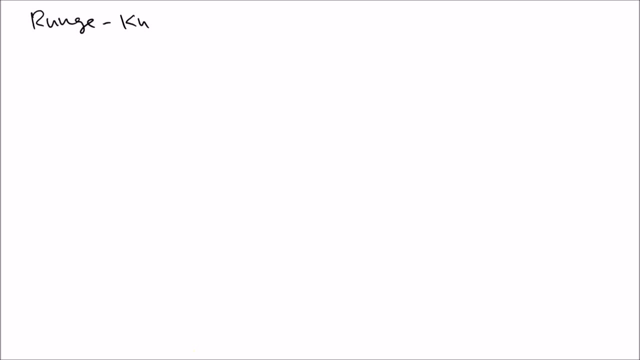 runge-kutta, runge-kutta method. uh, so this is very, very accurate. even the commercial software has used that. uh, so i should say that. so this is uh excellent result. um, uh, like a very similar problem. so you have y prime equal f, x, y, so the slopes are given with a initial condition. 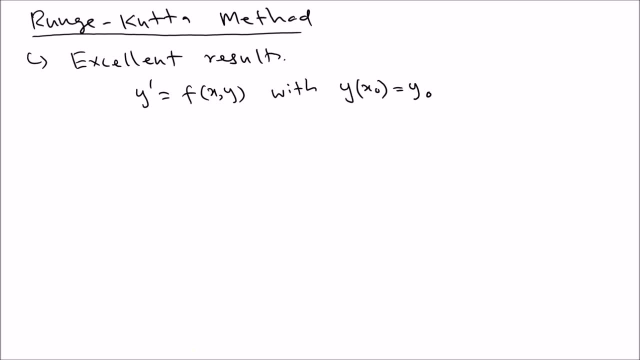 y, x naught, equal y naught. so you have a uh. so you know the starting point and you also know the slope. so then the goal is to approximate the actual curve. the same idea, uh, we're gonna uh split as before, though we're gonna call the gap is h and uh into approximate. 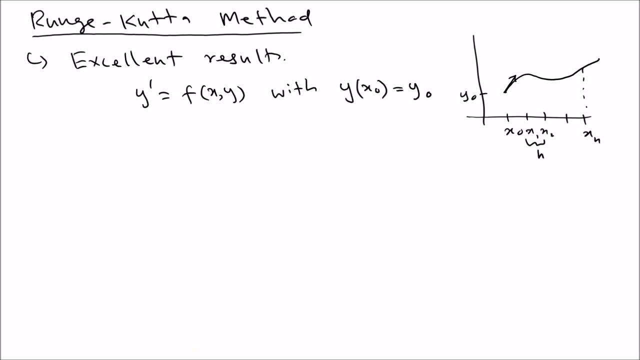 the value at xn, so um. so the scheme is slightly different now. so what we're going to do? we're going to calculate several intermediate values, so we're going to go for n equals 0, 1, 2, like that, depending on how many you need. as before, we're going to calculate the. 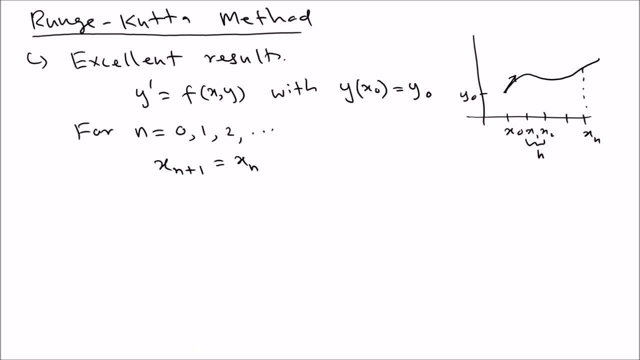 x naught, which is x n plus 1, equal x n plus h. no change. but before we calculate y, we're going to calculate several other slopes. so we can calculate k 1 slope, that is the slope at x, n, y, n. then we're going to calculate k 2 slope. 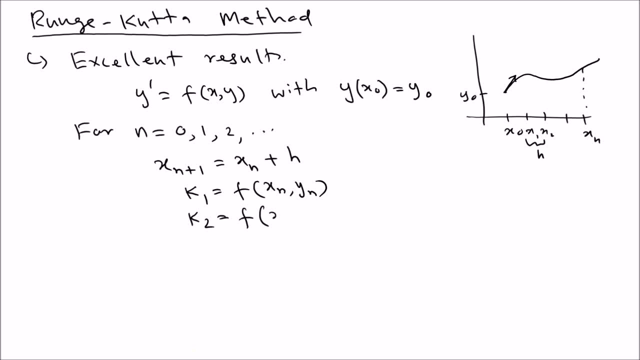 that is a slope, uh halfway in between. so you're going to go x n, you go h over 2 comma, uh y n plus h over 2 times k 1 and then k 2, k 3 slope, which is f again at the halfway point, comma y 1. 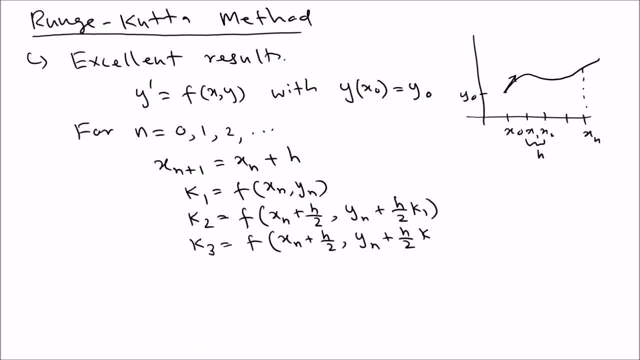 h over 2, k 2 now. so we have k 1, k 1 goes there, and then k 2 goes there, and then we have k 4. so what is k 4, which is f, x, n plus h, y, n plus h times k 3. so we're going to calculate those. 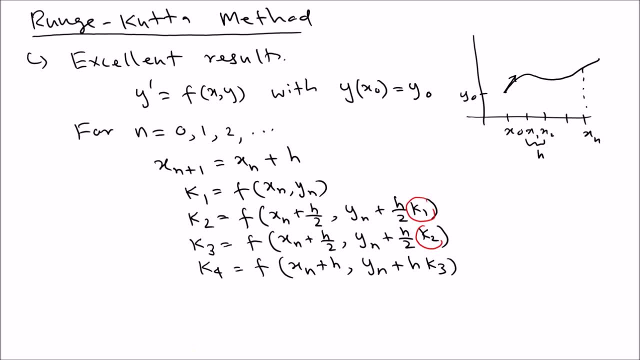 extra slopes, and after you calculate the slopes then you are y n plus 1. the next approximation value is given by y n plus h divided by 6 times k 1 plus 2, k 2 plus 2, k 3 plus k 4. so that is the. 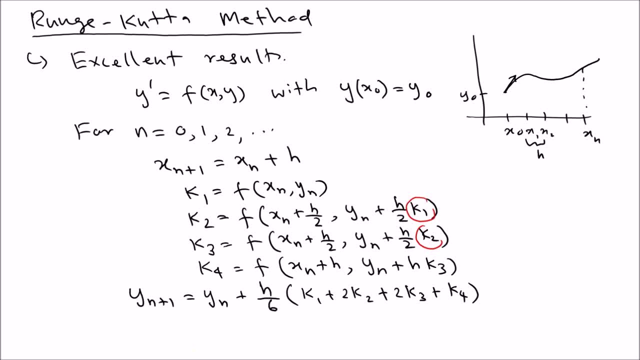 runga kuta scheme is very similar. you are, you know, x naught, y naught, so you're going to calculate x 1 y 1, x 2 y 2, x 3 y 3, like that. so this is what we normally call the fourth. 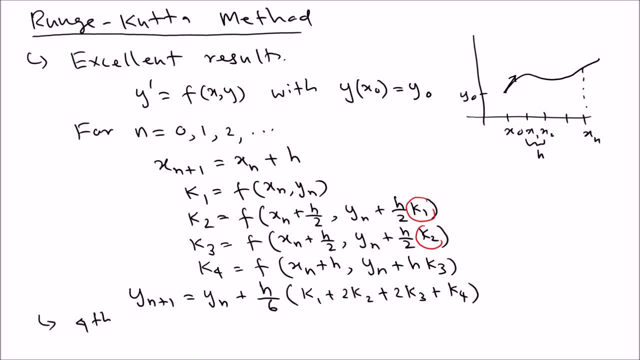 order: runga kuta. so that is the runga kuta scheme. next fourth order: uh runge-kutta method, so normally called rk, with it runge-kutta method. um, these are normally uh used in what we call od45 algorithm in matlab and other softwares. use and improved. use and improved. 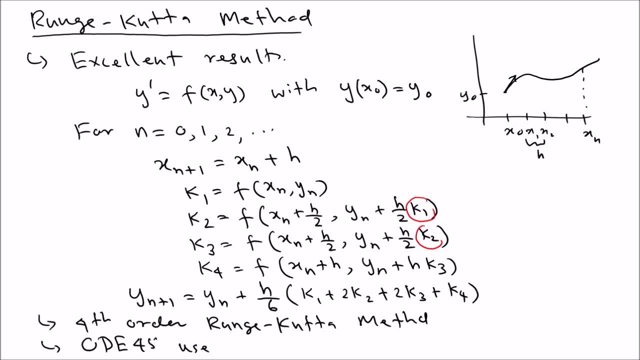 use an improved version. use an improved, improved uh version of this, of this, okay, so so that means it's very accurate, the solutions are very accurate and we solve several problems in the homework. uh, and look at, you can look at that also. we have solved several problems in. 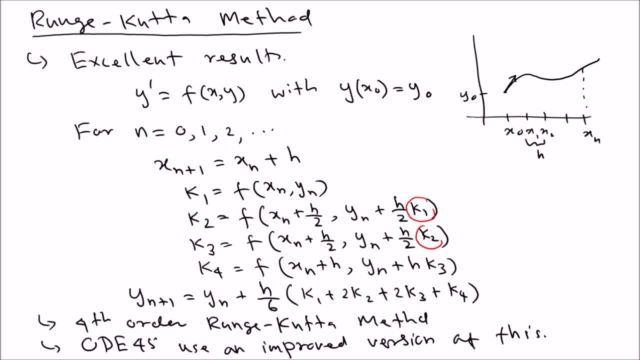 the video as well. so if any more information, uh, you can find them. uh, good, so this is the runge-kutta method and i'm not going to solve the problem from this one because very lengthy. uh, because you know that there are few, many things you need to calculate before we cover the next. 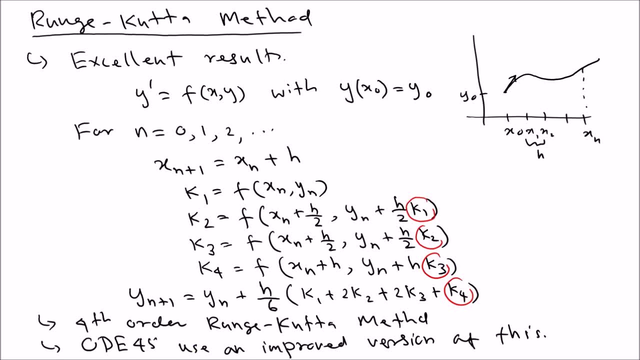 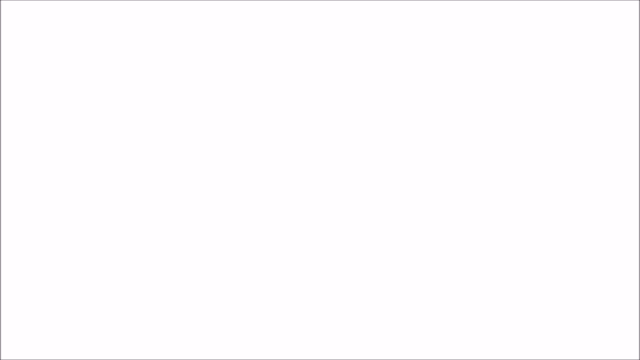 one. okay, so this is a how we gonna solve a. uh, this is the uh. next, uh, good, uh, numerical uh method to solve a first order difference equation. so, okay, so that's the main um point in this java�g. almost all of this java problem is it is called one unit. 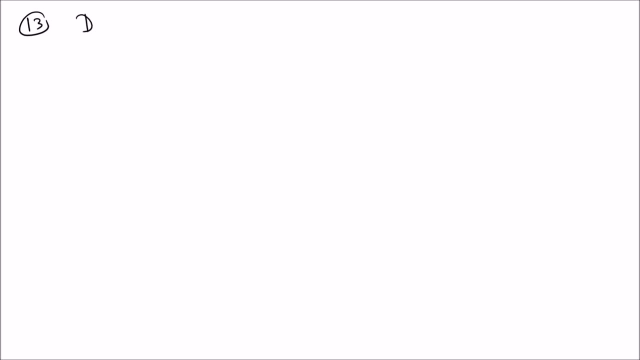 first order difference. so it depends on what it is. so what i showed is a first order random code and it bullet point direction, and when we find a new system it is misplaced. we are actually being made is all that. we are the same. um, we ran the first termに ре jul bejun by java, the first time we have. 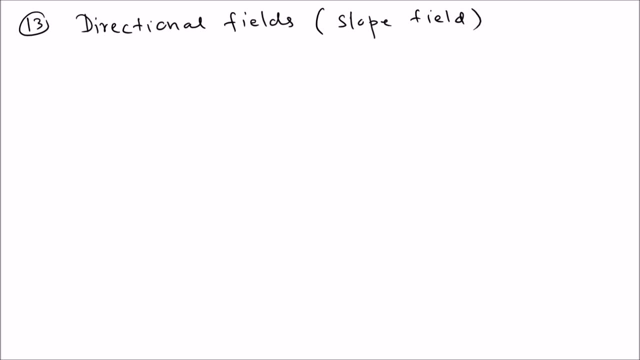 nose clear by java. there we go with that. we had a set logic. we we continue to run with the underlying structure of java. this is um after we are. so what we're going to do? uh, so when we have a differential equation, so let's say you are going to differential equation dy over dx equal fxy. so what we can do is, at each 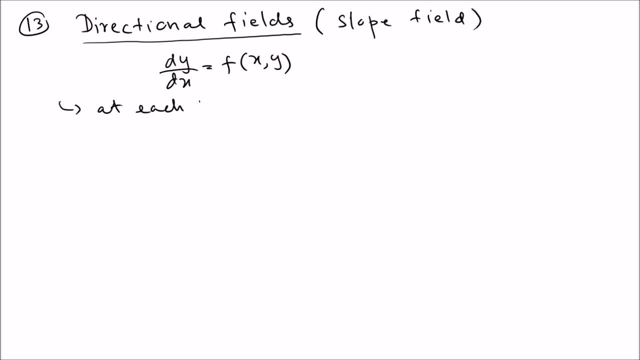 point, at each point in the domain, draw an arrow. draw an arrow indicating the direction of the tangent line, indicating, indicating the direction of the tangent line, the direction of the tangent line, tangent line, so that's what we call the direction of field or the slope. the direction of the line means the slope, so we can do a look at a 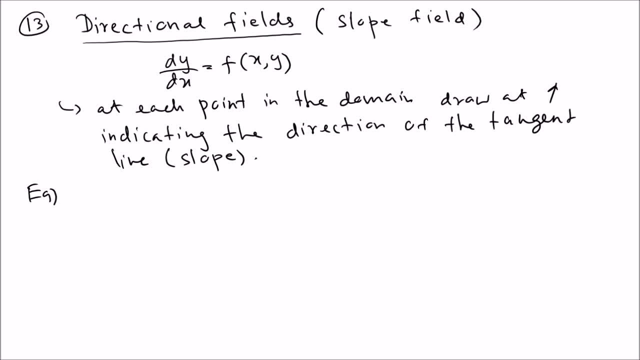 problem. so let's say draw the uh directional field, directional field of, let's say, dy over dx equal to x minus y. so if you get a problem like that, uh, what we're going to do, we're going to draw like a typical grid, uh, you know, with enough points. so let's do that. so this is a grid. 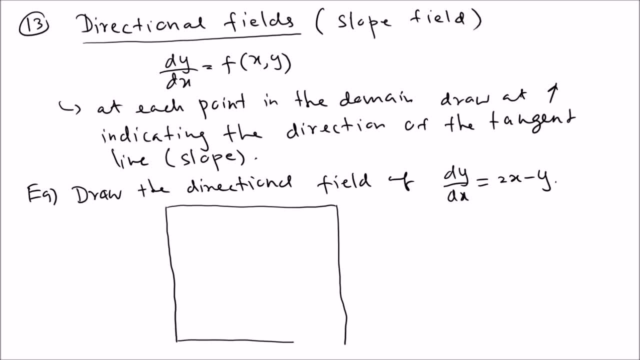 uh with enough number of points, so normally like this will be given. let's divide this into least you know, even s to one uh model. we are defining small radius vectorarium, vectorion, vector i, along with Nagar um. so what we're gonna do? let's say this is zero, and then one, two, three and then negative one. 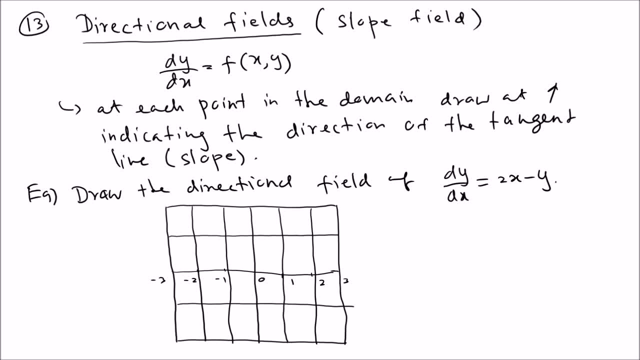 negative, two, negative three, like that. uh, so this is one, two, and then, uh, negative one, negative two. so what we do is, um, so this is the x direction and this is the y direction. so we're gonna, at each point you can evaluate the slope and draw a small line, and we know, uh, if there's a positive slope. so the arrow goes like that: this is: 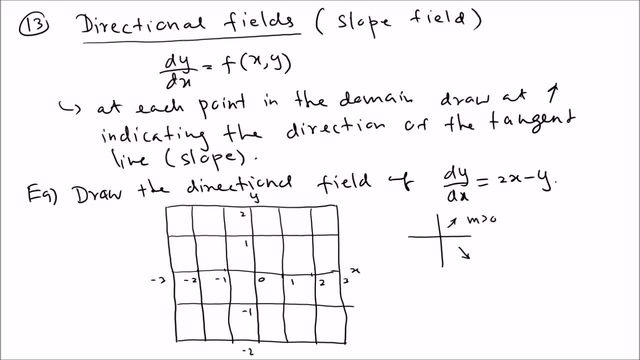 for positive slopes, uh. if you have a negative slopes, that's, the arrow goes down. this is zero slope. uh is horizontal, so we can use those three facts. um, so let's evaluate at zero. so at zero, you can see that if you plug in zero to the uh differential equation, you get dy over dx is. 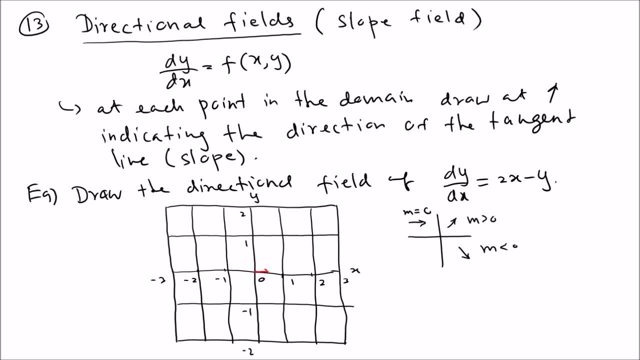 zero, so that means that's at zero, slope is zero. so you draw a line like that with zero slope. and then also you notice that there's a special line. for example, if you look at this line: uh, so you can say on the line, on the line: uh, if you set this equal to zero, so you're gonna get. 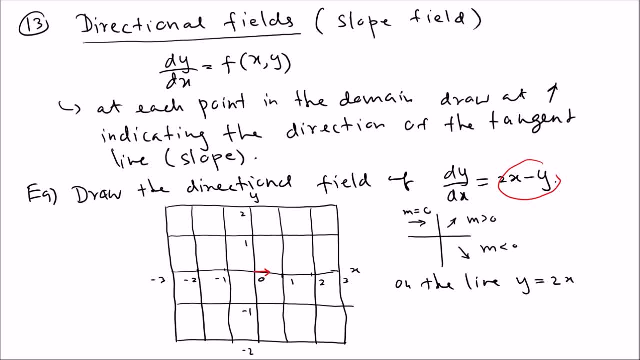 y equal to x. on the line y equal to x, the slope is zero. the slope, the slope is zero, slope is zero. so that means what is this line? uh? so that means at x equal one, y equal two. so that means this is the line, so the line uh passing through, uh, these points. so on this line, the slope is zero. so that. 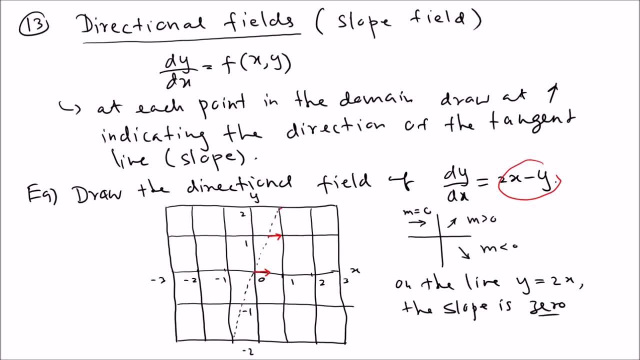 means if you pick any point on that line, you know that the slope has to be zero. so that's one thing. so we know that on that line slope is zero. and also, let's calculate few other uh values, uh. so for example, at this point, if you look at this point, you can see that it is x equal one. 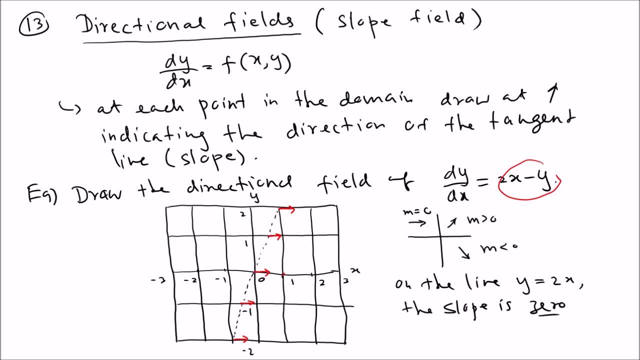 y equals zero, so the slope is two, so it's a line with slope two. and at that point you can see slope is four, so it's more steeper, and here, like, slope is six, so it's much more steep. like that and if you go to the other side you can see at negative one slope is negative two. 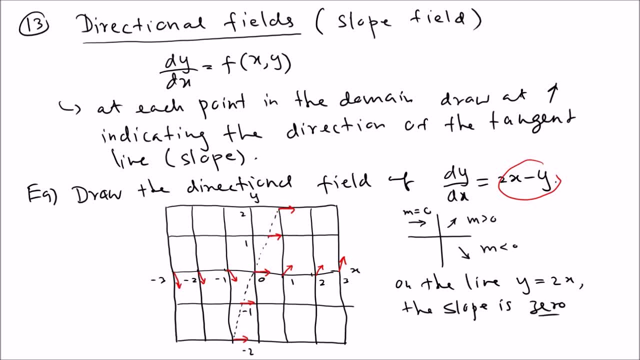 and negative four and negative six, so it's much more steeper. and then, if you go along the y axis, you can see that x coordinate is zero, y coordinates increases, but with the negative sign uh, it's going down. so, for example, at this point the slope is negative. 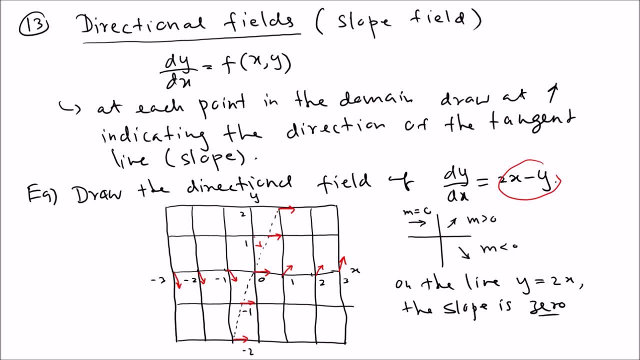 one. so it's going to go like that: the slope is negative one, and if you go up it's negative two, so it's much more steeper, and here at negative one it is one and this is a two, and we can also draw a few more. so, for example, if you add one one, so you're gonna get slope. 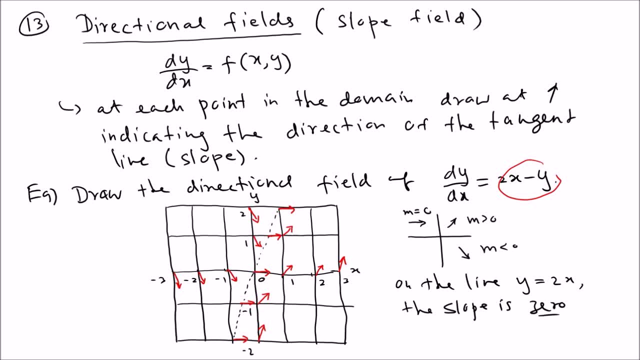 two minus one, so it's one. so slope is exactly one here. and then if you go further, it's the same y coordinate, but x coordinate increases. so we're gonna get more steeper like that. and then here what happened: x is negative one, that means negative two. 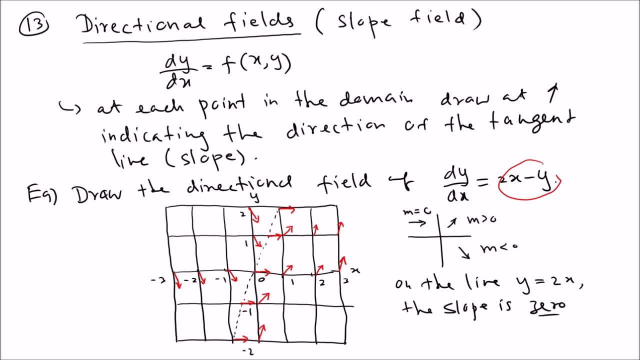 and then y is ah, one. so so at this point what's gonna happen is: uh, let's calculate what you get, so you can see the x equal negative one. that means it's negative two, ah, and one, so negative three. so it's negative three, and when you go up it's get more steeper. 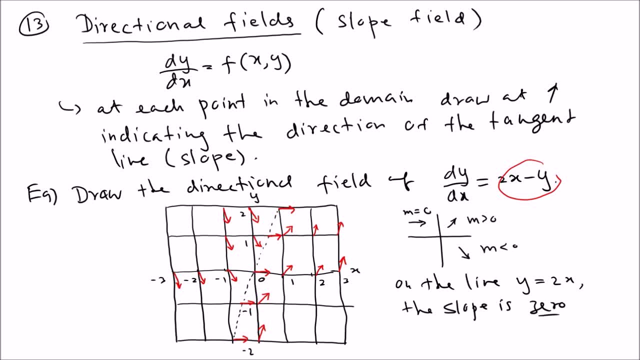 because y code y is sub subtracty. that means get more steeper, and at degree two it's going to be, and so it gets more steeper. you go the same thing. when you go this way, it's going to get much more steeper. and uh, what about? uh, this point? 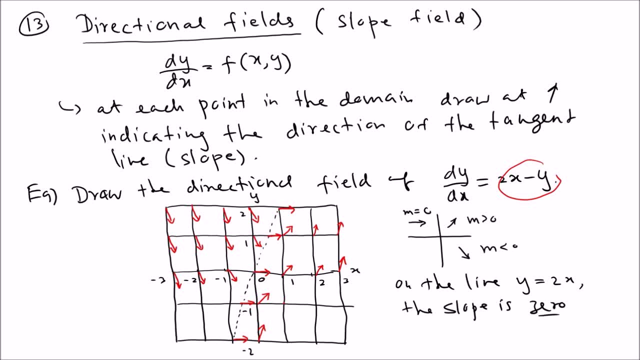 so this point, uh, you can see, x is one, so it's two. and then, uh, minus one says three, because y is negative, this is three, so it's more steeper, the same thing, much more steeper when you go that way. uh, so go down, that means it's gonna get. 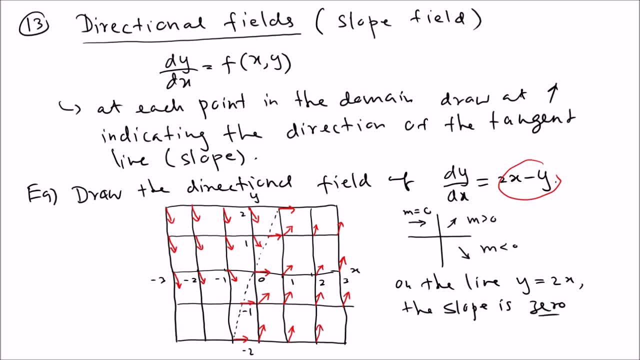 more steeper like that. uh, so we only left these. so let's calculate what happened at this point. so which is negative one? that means negative two, and then uh, and then we have uh, y equal negative one. the negative has become positive, so it become negative one, and then when you go, it's going to get. 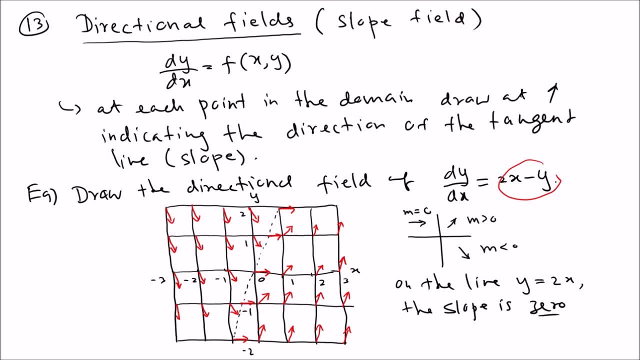 much more negative like that. so those are a few values. okay, so we we see that we have a negative one, we still have just a few more. uh, so at this point, what's gonna happen is it is negative two. that means negative four, and with negative two has become uh. so what happened here? 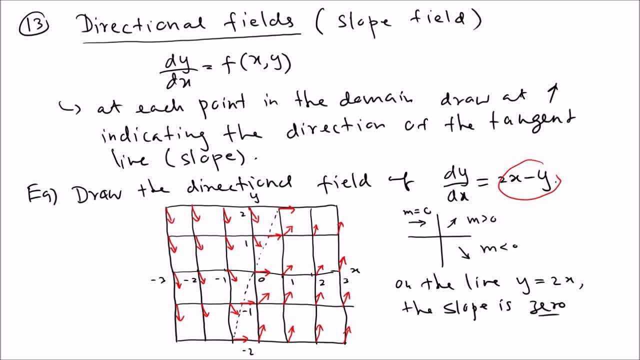 so you can see, when you go down, uh, you subtract negative values, that means gonna get less deeper. so like that: uh, yeah, because, because the negative sign, so it's less deeper. uh, when you go down, so that means this has to be: uh, less deeper than that. good, so when you go down, it's get less. 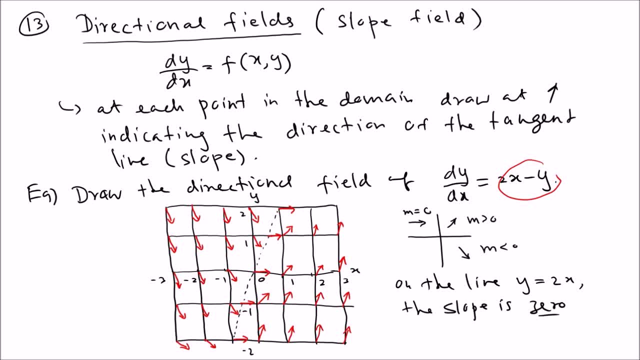 deeper because the negative y sign. okay, so that's the uh directional field. uh, for this one, and good. so now what we can do is we can draw a typical curve, like, for example, if you want to draw a curve that passes through one uh negative one one, so that means the point, this point, that's the negative. 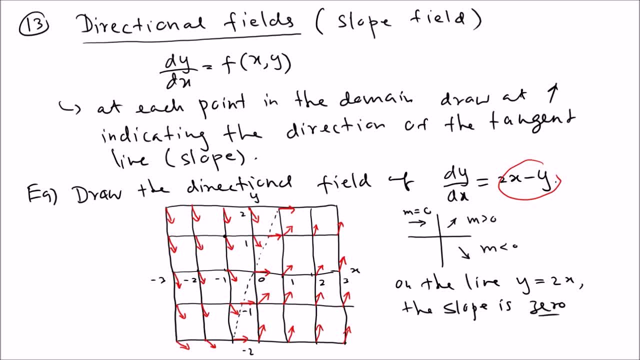 one uh one point. so what's gonna happen? it's gonna follow the uh arrows. so so if you follow the arrows, what's gonna happen? it's gonna go like that, go like this, and i think it's gonna go like that and get zero and then turn and i'm gonna go uh like this. so this is a typical curve. 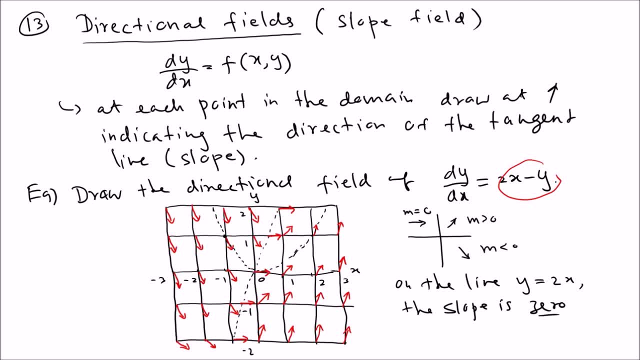 and that passes through, uh, the point one one. so what we're gonna do is simply draw, follow the uh arrows, so like that. so good, okay, so that's what we can do with uh directional fields. and then, uh, what else we had? uh, we talk about uh existence and uniqueness theorem, so let's talk about. 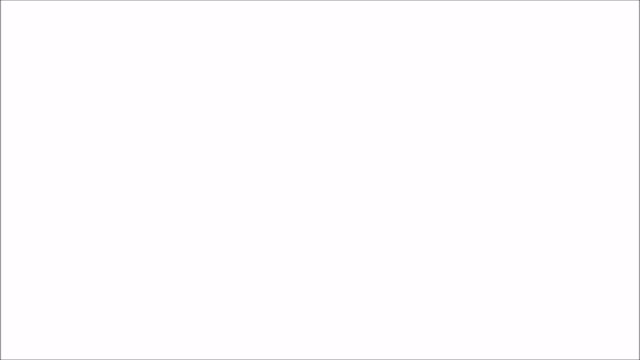 that a little. so we have the existence of the tolerance and the uniqueness. theorem, number 14: existence and the uniqueness, existence or uniqueness. so let's look at the differential equation: d, y over dx, equal f x, y, along with y, x naught. so let's say so there's a region, so there's a point: x naught, y naught. 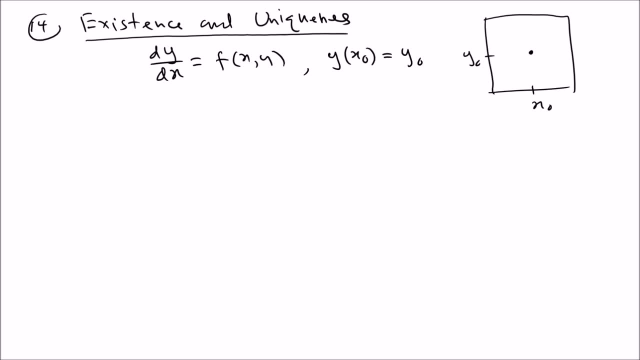 so. so we know that point. now the question is whether there is a unique solution that passes through that point. actually, uh, that depends on certain conditions of the function. so, for example, if the, if the function f is continuous and it's y derivative, y partial derivative, continuous, 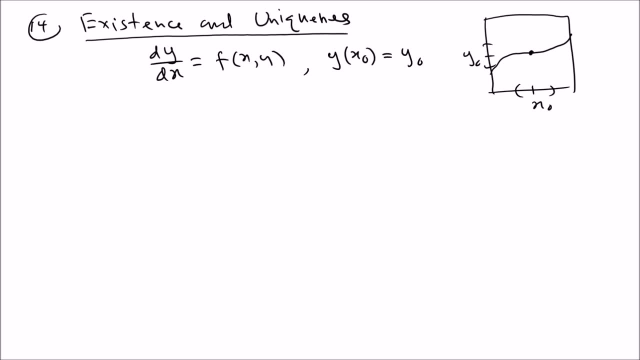 so the answer to that question is yes, there's a unique solution, so let's write that as a result, uh, but in general, uh, a solution, a solution, uh may or may not exist, a or may not exist, but under certain conditions. uh, the answer is yes, so let's uh write the theorem. so this is what we. 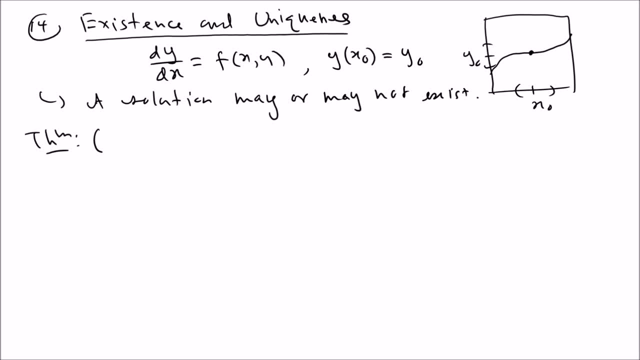 normally call the picard's uh existence and uniqueness theorem. so because existence and uniqueness theorem, so what? it says that for the initial value problem, for initially problem d y over dx equal f x, y, along with y x naught equal y naught, there is a unique solution. 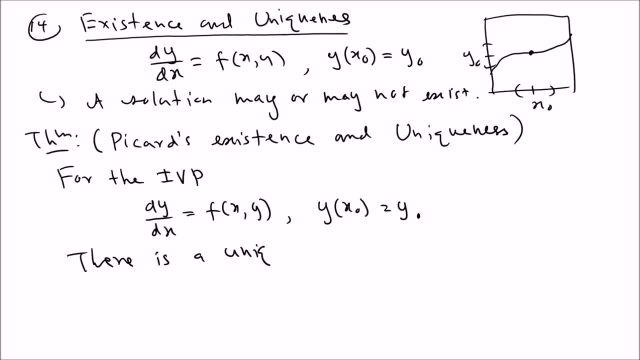 there is a unique solution. this unique solution just in each solution near x, naught, y naught, if the function f, x, y and its partial derivative with respect to y are continuous near x, naught, y, naught. so we check what happened near x from y naught is if the two functions 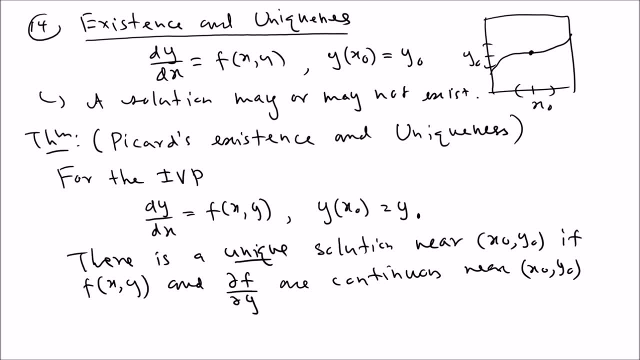 f, x, y and the double x of the double y, the partial with respect to y, continuous, then there is a unique solution around that. so that means if you can extend that interval, along that interval there is a solution, so it can be the whole region, because this interval can be. 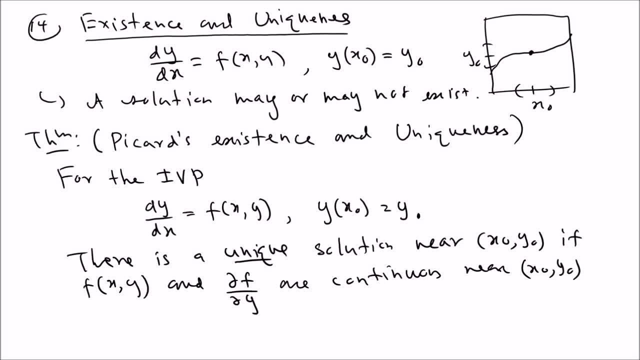 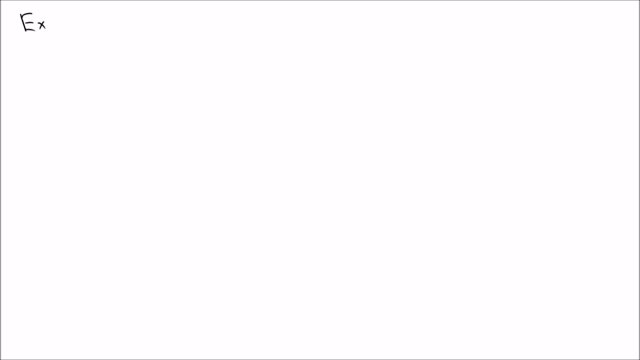 the whole domain. so that's the existence uniqueness theorem. so we only check whether these two functions are continuous. so we can't check continuous near that point. so let's just do one example to see how we can apply that. so for example, something like this for the ivp, for the initial value. 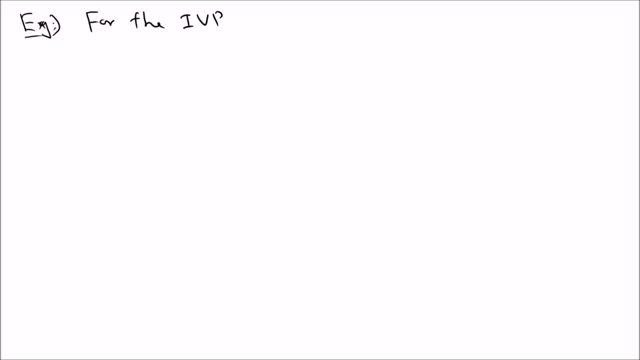 problem: d, y over d, x equal x over y, along with y, 1 equal 2, so that means you can see your region is so, say, 0, so it's a 1 and 2, so there's a point somewhere. so we're going to check what's going to happen near that point. 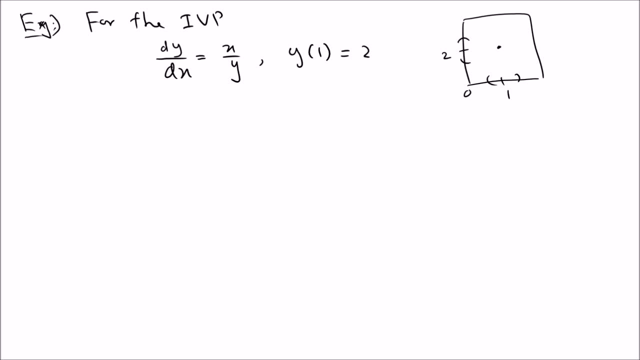 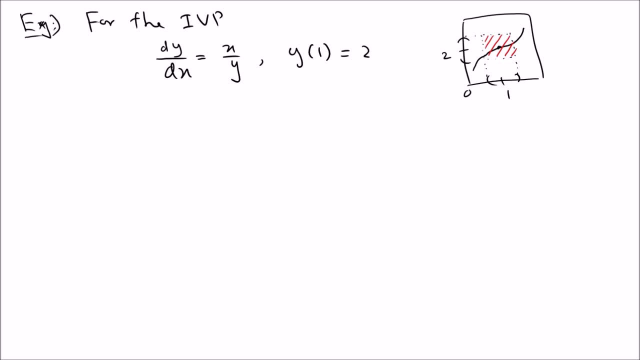 this box can be everything, but we just guarantee in that small one, okay, so then we can see that there is a. there is a unique solution. there's a unique solution. uh, y, equal y, x, so it's a function of x. that's what it means, because in here, 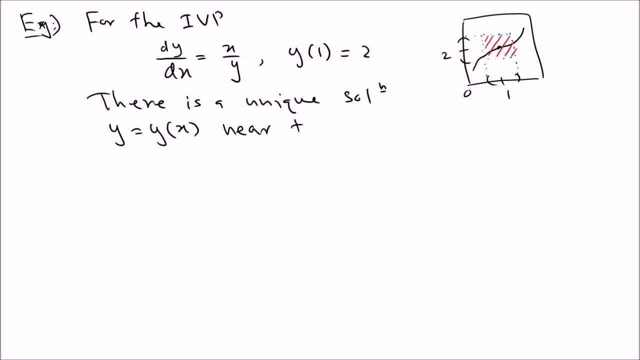 the point near the point one. two, since the function fxy, which is x over y and double f over double y, if you take the positive with respect to y, you're going to get negative x over y squared. that's what you get and you can see that double y is going to be. 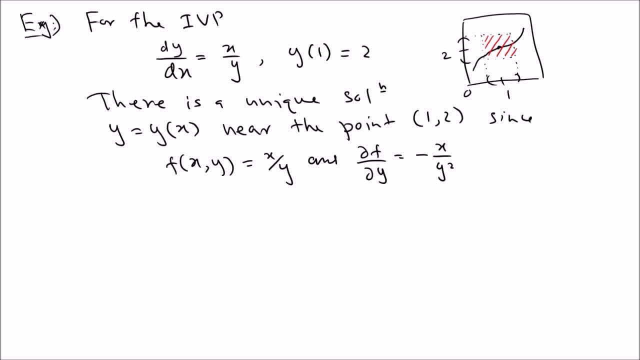 equal to 2, and you can see it just like that. but the whole situation is the same, even if that probable solution, not that you have the same composition now if you look at the fails. so the problem you see is, uh, the DAMM is that it just deletes the function. 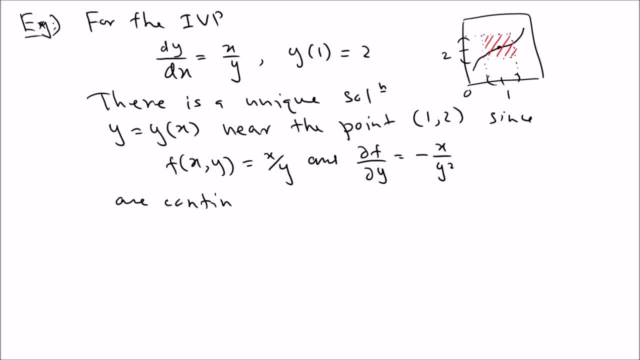 and so we see that for that answer on the что is right we have, z is being continuous here. those are the two PC uh working points right now. so all of these functions are continuous. here, though both functions are continuous, there are no problems with that layer, that region, but you cannot include 0. if you include 0, we get the division by zero situation, but here no, because we only consider near one, two points. so everything, all the functions are continuous. so since the two functions are 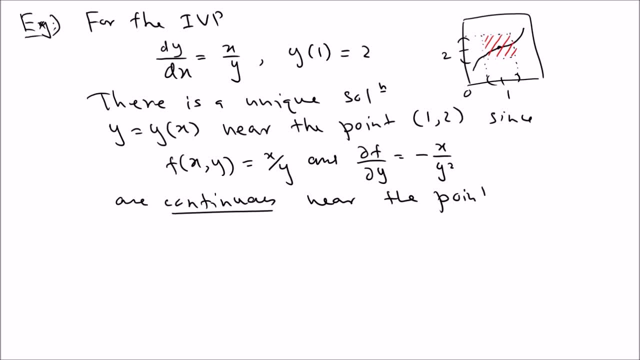 the point one, two. but there are problems. uh, near um here one, near uh one zero. if you have one zero, because at that point the y doesn't exist anymore, okay, so, so we can see, uh, but near one zero, the solution does not exist, since double y over, double, double four, double y, uh, discontinuous. 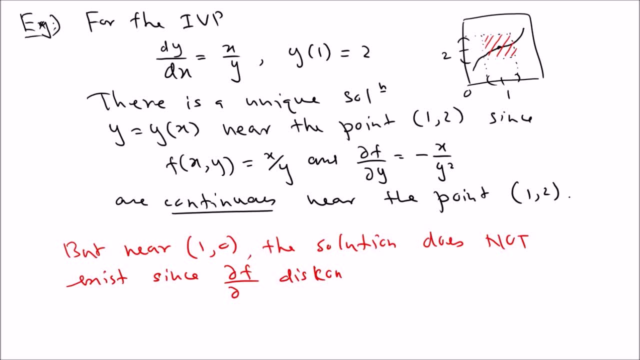 double y, and you see, and ah, f, x, y equal, y over x, discontinuous. this continues at uh, one, zero. so that means there are no solutions for that point, there's no slope at that point. okay, so, and then, uh, uh, we need to talk about the. 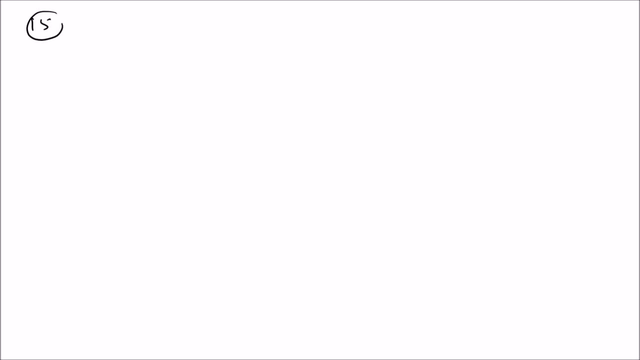 autonomous difference equations, the autonomous differential equations, autonomous differential equations. uh, so you can see an differential equation and this is a translation equation. the translation equation is called is called autonomous. it's called autonomous if it does not depend on the independent way, if it does not depend on the 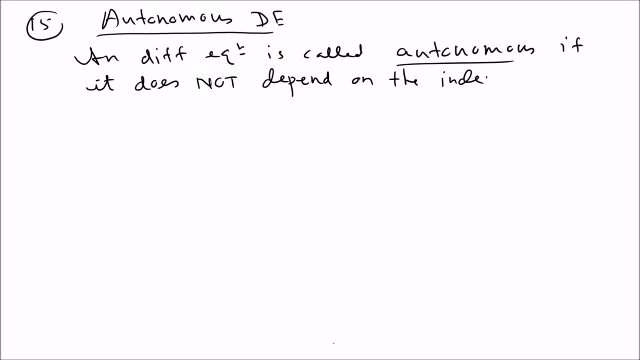 independent variable. independent variable, for example, dx over dt equal minus x, x minus 1 squared, is autonomous, because you can see that it does not change over time. because x, because there's no t term, so it's just fixed. okay, so this represent the, uh, what we normally call the stable solutions. 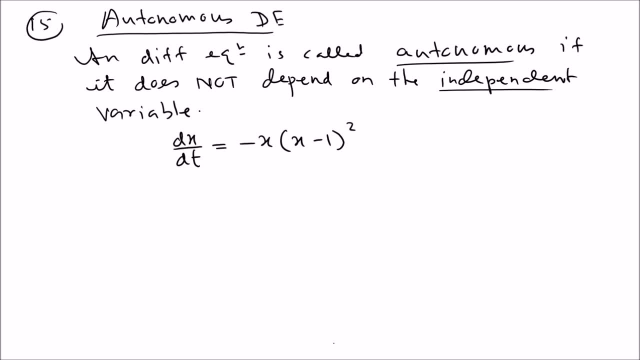 stable situations because it doesn't change, difference equation doesn't change, it can stay there. so uh, so you can see that uh, so the node, so you can see, uh does not change, does not change, does not change as does not change as time. that means in this kt. 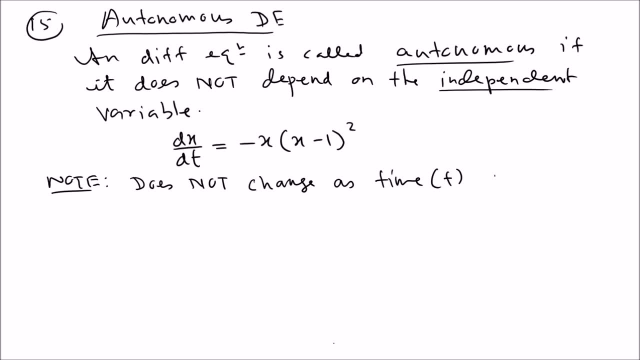 changes. okay, that's very important. uh, and then we define what we call critical points for that. so critical points. so critical point means the particular point of the variable, is the point of the variable which is called a hard side, where the place is where the derivative is zero. so if 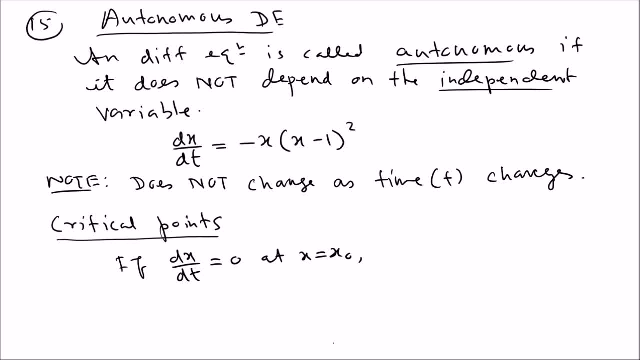 dx over dt equals zero. at x equal x, not x naught is called called a r critical point. it's called a critical point and at the end, where it is zero, if x equals x naught. that's why this is called an speak point. and then after that, what we did was we check whether the critical points are. 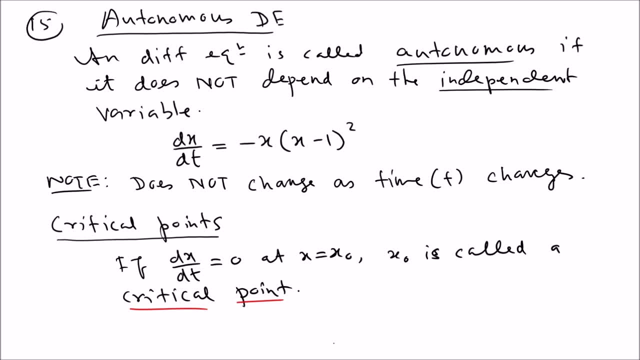 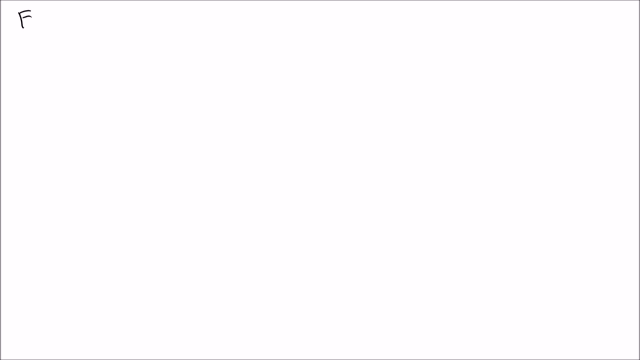 stable, unstable, half stable, so, uh, so we may check. we may check whether the critical points, critical points, are stable. let me check whether the critical points are stable or not. so let's do that, uh, in a problem, so we can do something like this. so the example: 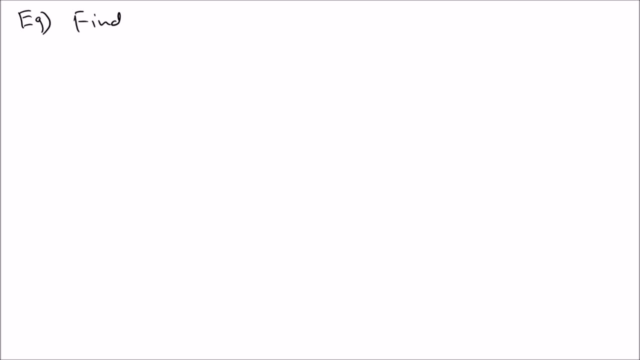 find the critical points and find the critical points. find the critical points and classify. classify them as stable, half stable or unstable. yeah, so there are three types: stable, have stable or unstable. uh, for the differential equation, dx over dt, equal negative x, squared x plus 1, x minus 2, something like that. so what we can do, uh, we're going to first. 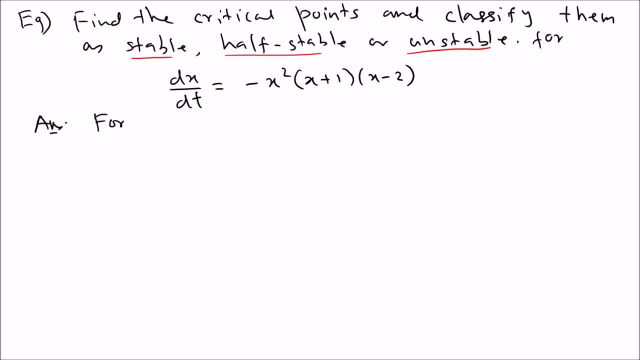 find the critical points. so for critical points, for critical points, what we can do? we can say dx over dt, which is negative. x squared x plus 1, x minus 2 equals 0. this implies that from each factor, the first factor say 0, and then we have negative 1 and 2, so negative 1 comes from here. 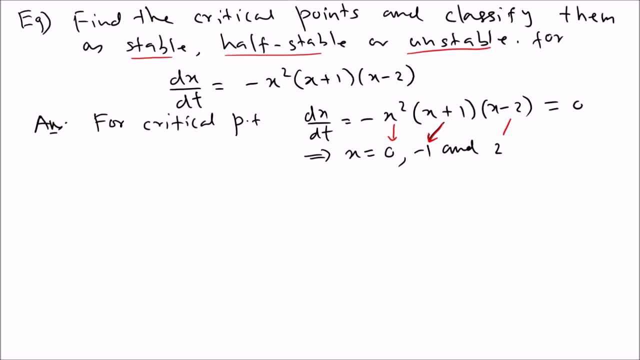 negative 1 comes from here and the 2 comes from here. so those are the three critical points. now, what we're going to do? uh, we're going to draw the face portrait, so it's a vertical line, and we're going to put those numbers in the order. so we're going to go with negative 2 first, and then we have 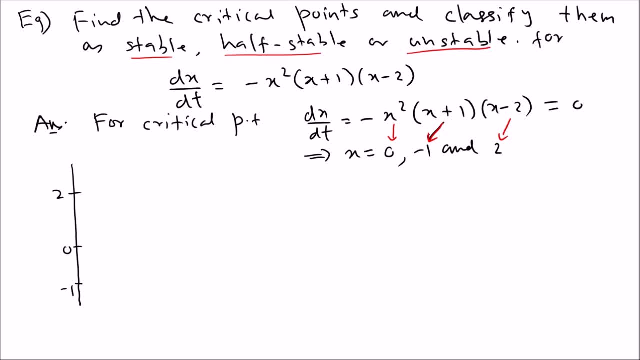 0 and then we have 2. so those are the three points that we have in that order. now what we're going to do? we're going to pick points in those intervals. so we're going to pick a point which is greater than 2, we're going to pick a point between 0 and 2. 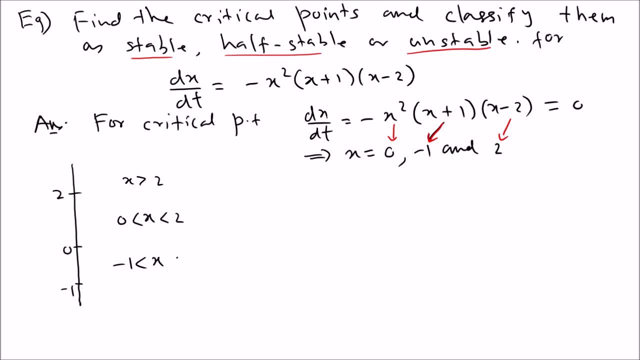 and then pick a point between negative 1 and 2, negative 1 and 0, and then pick a point which is less than negative 1. now what we're going to do, we're going to check the sign of the slope so we can check the sign of the slope, so you can see that. you just plug in a just point. 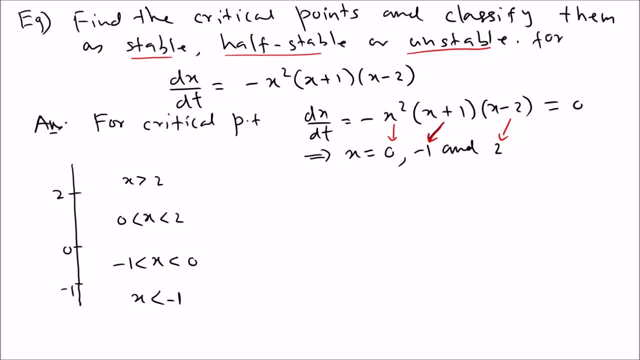 in those region to the equation and you can see that it is if you pick a point like, let's say, 3, so and if you plug in three it is positive, and if you plug in three it is four is positive. if you plug in three, uh is positive. so that means 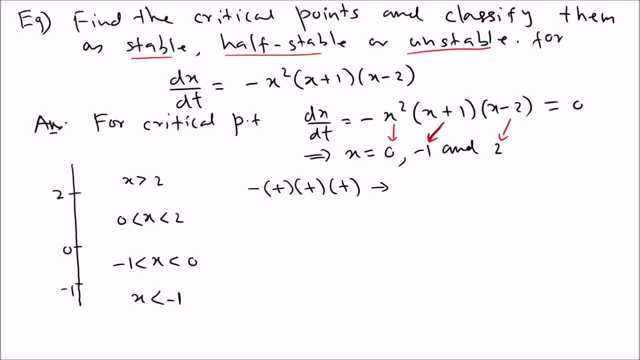 this says that, uh, it's a negative, positive, positive, positive. so it's negative. that means dx over dt is negative. that means it's going to go down. so we're going to put the arrow going down. do the same thing now. we're going to pick a value between 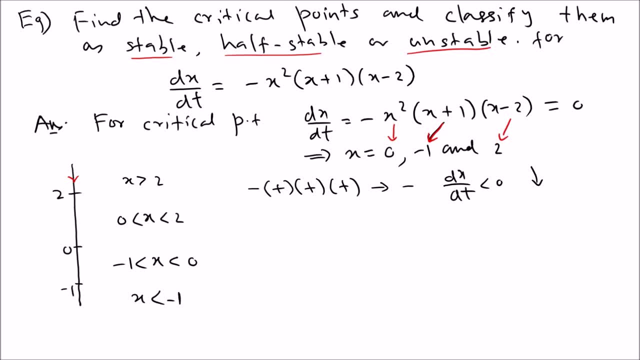 zero and two, so like, for example, one. so if you plug in one, you can see it's negative, positive, this is automatic. and then if you plug in one, you're going to get x plus one means two, so it's positive. and if you plug in one, this is negative, so that means it's. 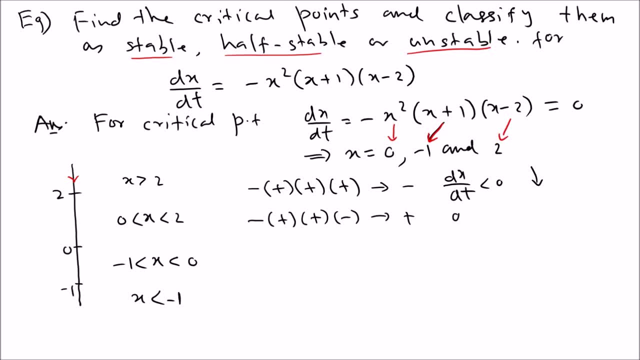 going to give a negative, negative, a positive sign. so that means dx over dt. positive, so that means it's going to increase. so we're going to draw a line like that arrow, like that: now we're going to pick a value between zero and negative, one like a negative. 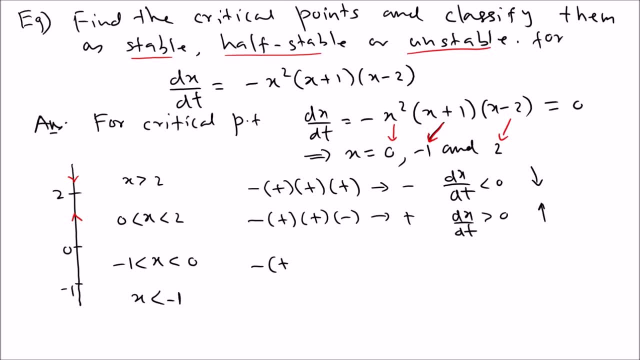 0.5. so if you do that, it's negative, negative, positive, automatic. and if you pick a value between like as like a 0.5, and then you can see this positive and then this is negative. so that means positive, so that means dx over dt, the. this is the slope which is positive. so 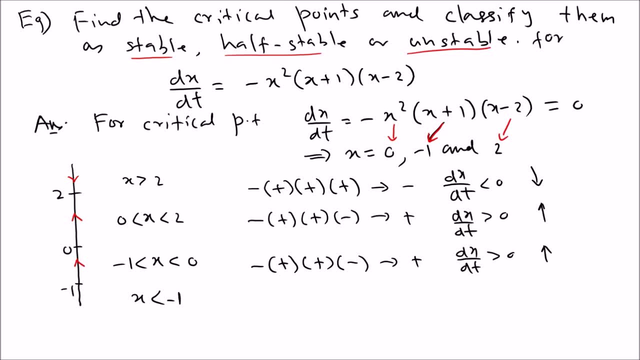 that means going to go up, so that means the arrow going up. now for the last one. we can pick like something like negative two. so if you pick negative two, it's a negative, negative, negative, positive. if you pick negative two, it's going to be negative. this is: 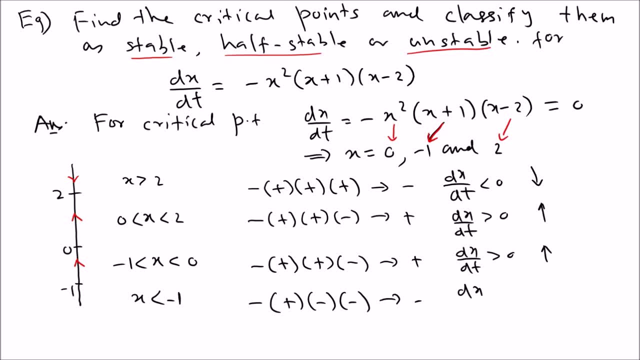 negative. so there are three negative signs. that means negative. so that means dx over dt negative. so it's going to go down. so we will put a down arrow. so now you can see that there are the two arrows converge in the first one. so that means this is stable. 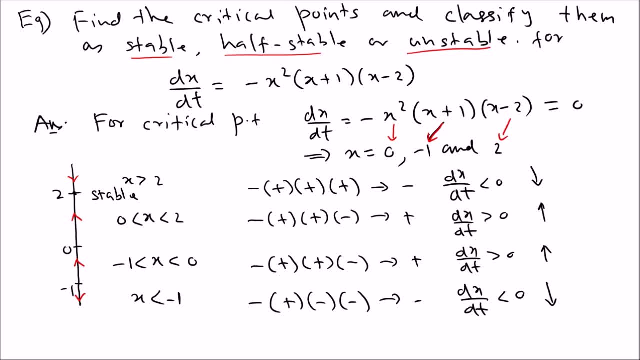 point. at this point it is stable. that means both sides is going to converge, to that. and at 0 you can see that one goes in, one stable and then the last one. you can see that going out. so it is unstable. so we can say that for those critical points. so that's the classification and 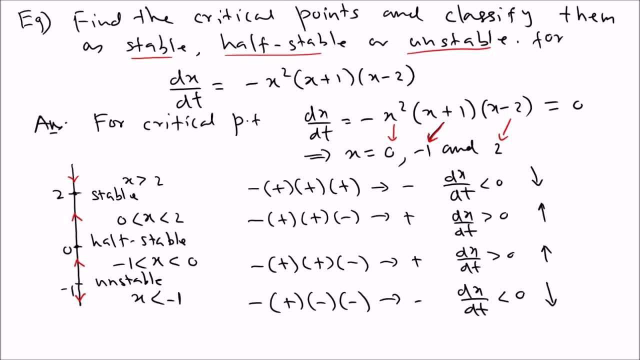 the last thing, what we can do. let's say: um, you start with the point, like at the beginning. you start with a point, so let's say so. the question is, if x, 0, the starting value is, let's say, negative 0.5, so what's going to happen in the long run? so find, 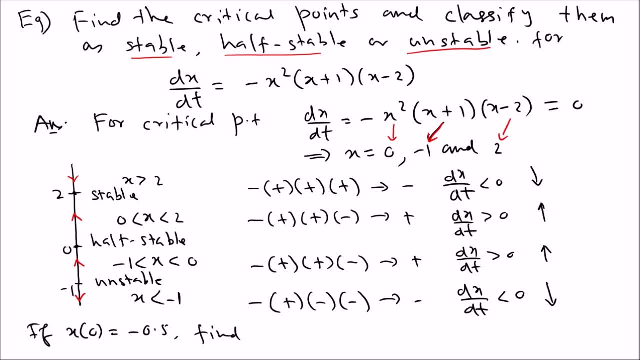 ah, the limit, find the limit. t goes to infinity, x, t. so what's going to happen? you can see that when time goes on, it's going to go up. so that means, uh, it's going to converge to 0. but even though the arrow, all the arrows, 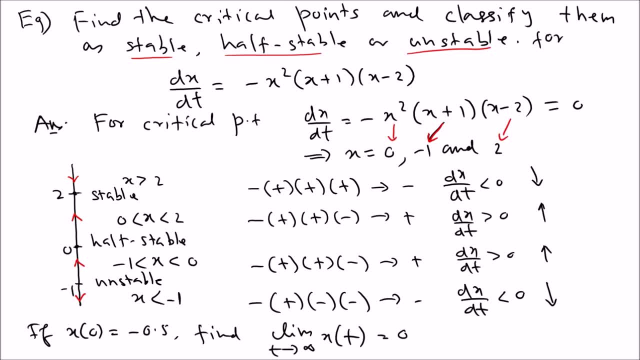 uh, the decimal point is going to go up, so that means the next arrow is also going up. it never go to 2 because it's never past a critical points. that's a very important fact. never cross a critical point, so never cross a critical point. okay, so this is all about first order, differential equation and related topics. 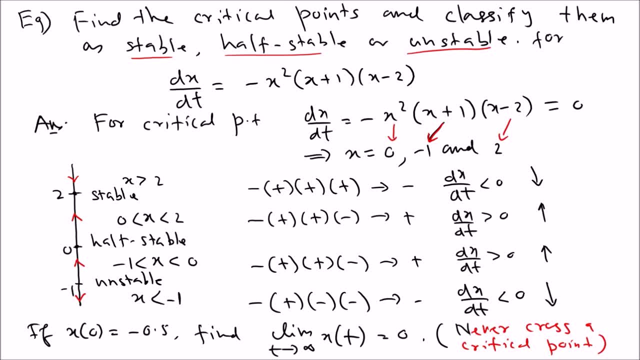 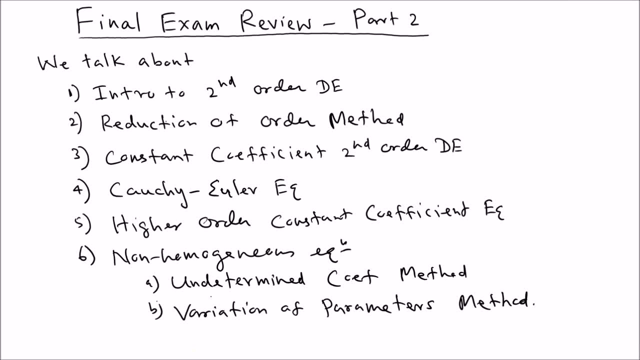 and then we can talk about second order differential equations. so this is the final exam review of part two. in this we are going to talk about introduction to second order linear, ordinary differential equations, in that we can talk about what we mean by general solution and the linear independence. 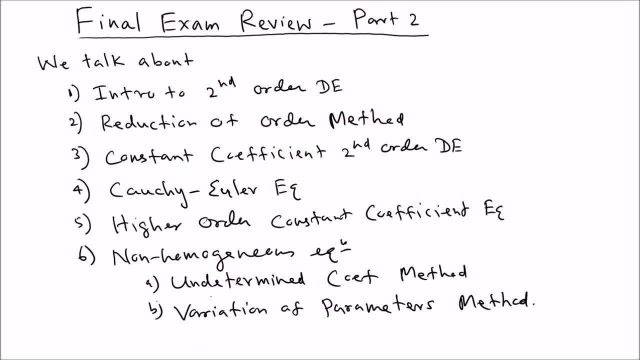 including wronskian test. then we can talk about the reduction of order method. uh, that means uh, we can reduce a certain number of equations. so this was taught in a previous video. how to antithesis under Jeremiah europolalnız, we will look at in that video. 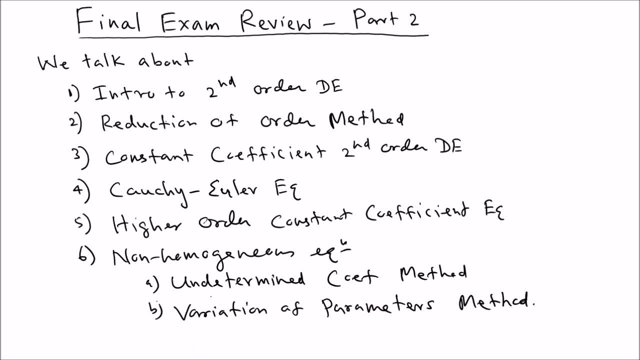 so next exercise we're going to talk about how to point a second order differential equation to a first order differential equation if you know one solution, and then we talk about constant coefficient second order differential equation, then we talk about one of the very special case, what we call the kochi euler. 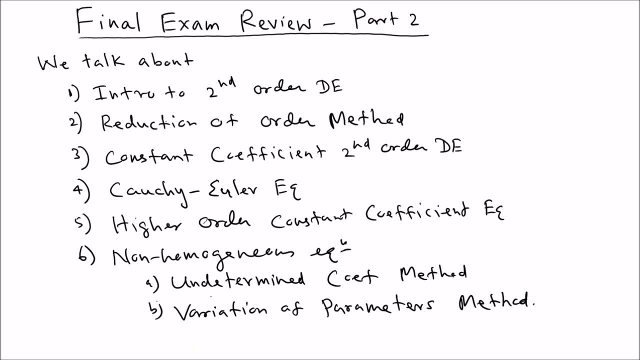 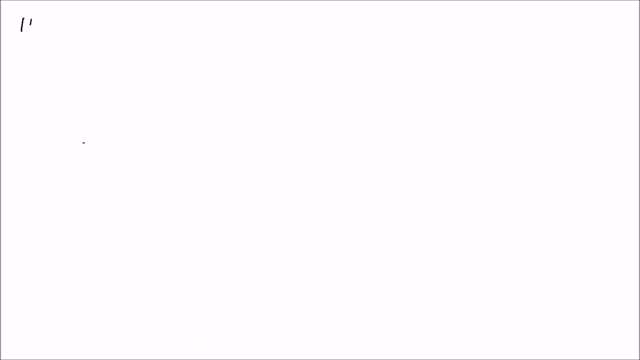 differential equation. then we talk about higher order constant coefficient. under that we're going to talk about undetermined coefficient method and the variation of parameters method. so, uh, let's start with the second order, linear, ordinary differential equations. so this is number 16 according to our list. 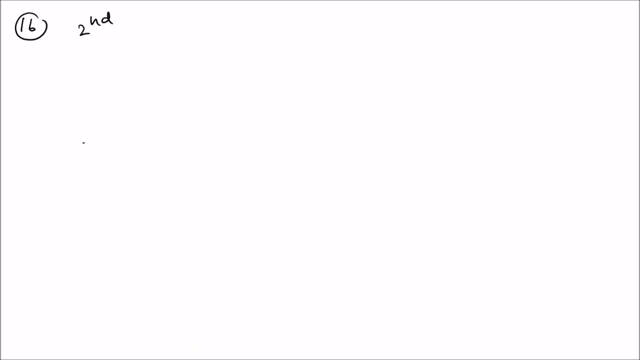 so this is a second order, linear. second order linear, ordinary differential equations. ah, so let a y be the dependent variable dependent variable and x be the dependent variable independent way. here it's always a good idea to check what is the independent variable, um, because sometimes we're going to confuse and write the wrong one and everything is. 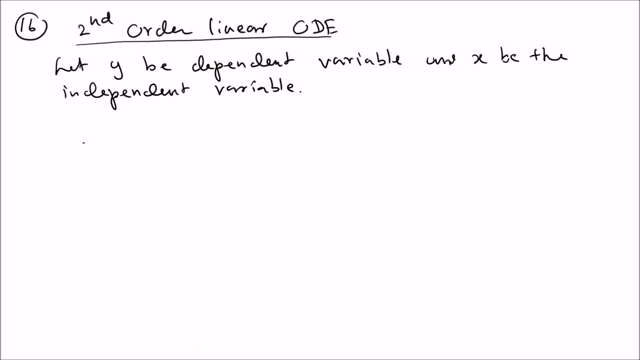 wrong after that. so if you look at a general second order linear differential equation, you can write that in this form. so you can write this as ax. that's the coefficient function of the first, uh, the highest term, and then the, and then we have bx. that is another coefficient function of the second one. 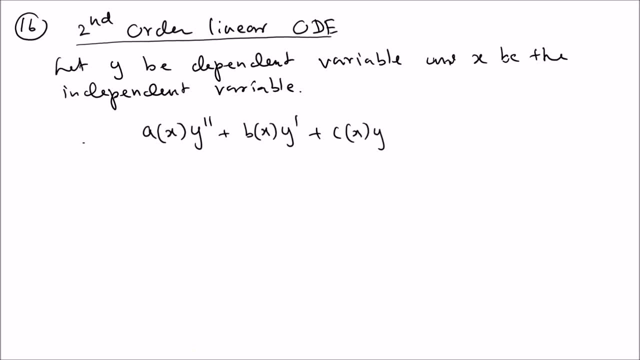 and then plus c, x, y equals dx, because x is the independent variable. so you can write it like that. that is the general second order linear differential equation. now, what we're going to do, we're going to divide by the ax term, just to make it easy and to bring it to the standard form, so we can divide by x. 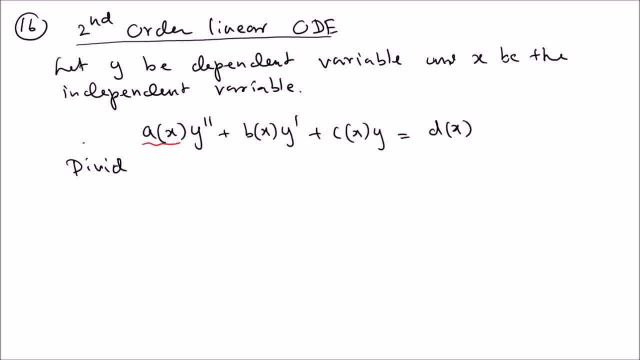 so, dividing by x, we can write this equation as y double prime plus bx over x, bx over a x. later we call the px, and then y prime plus cx over x. y equal d, x over x. so we can write like that: now what we're going to do? um, we're going to call this: uh. 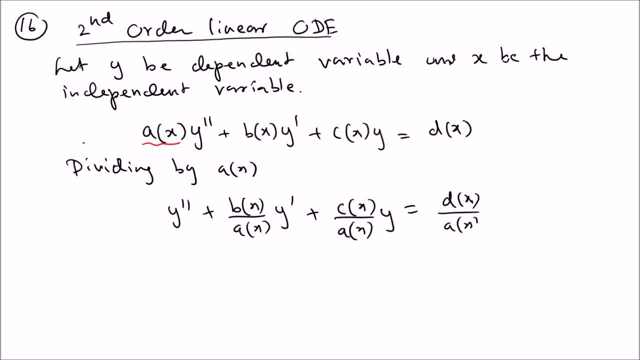 d x over x. so we can write like that: now what we're going to do, uh, we're going to call this uh bx of ax px and this is qx and this is uh fx. so with that we can write the standard form. so we have the standard form. 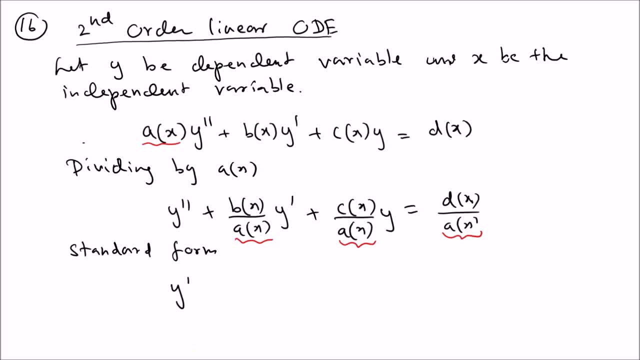 standard form: y double prime plus px, y prime plus qx, y equal fx. so this is what you get and this is what we normally call the standard form. so if the because we know that x is not zero completely, so therefore we can always do that it can be zero. what we can do, we can remove those points. so what we normally 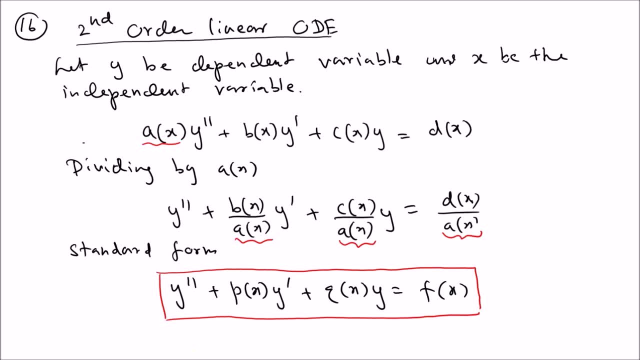 call singular points, so we remove them. um, now what we know, this is a second order differential equation, so there should be uh. so this is second order od. so that means uh. in theory, there should be a second order differential equation, but there are multiple equations, so in this case, uh. 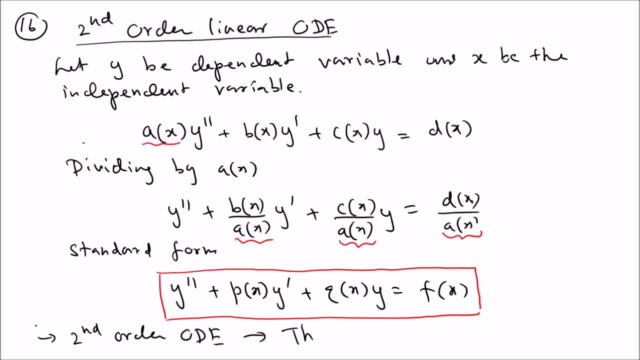 this equation is one. so if i do, x is equal to zero, so if 2 is equal to a. so there are there are two solutions. there are two solutions. why? because this is, uh, second order, so there are two solutions. so let's talk about, uh, the special case first. we're going to consider the case. 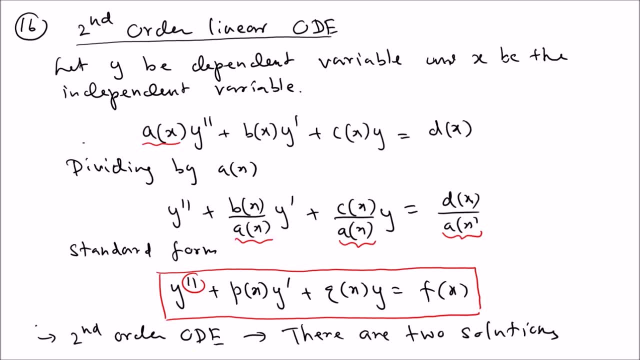 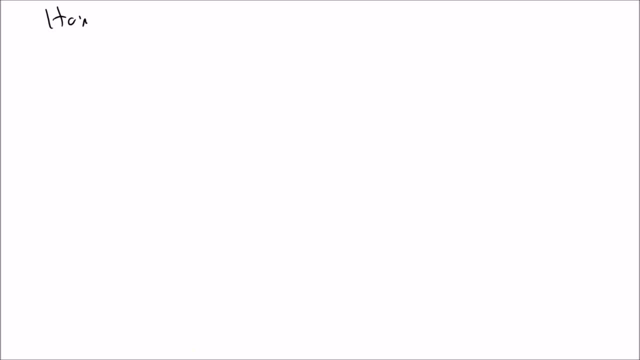 where fx is uh zero. that's the easy one. uh, let's talk about that. so that's what you call the homogeneous second order equation: homogeneous, homogeneous second order- uh differential equation- homogeneous, second order differential equation. so what is that? that is means if fx function is identically zero. 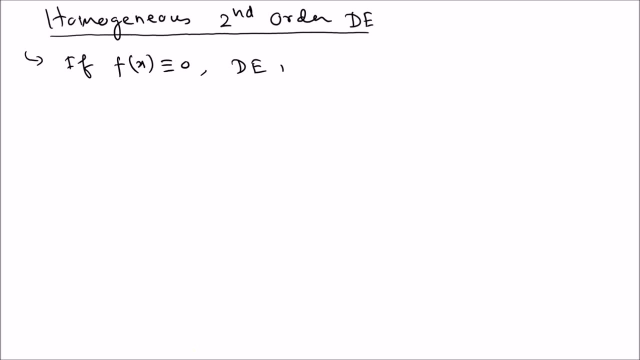 then the differential equation is homogeneous. so it's just a home. that's my homogeneous. okay, that's in short, sometimes, uh, good, now we have this, a very important result, uh, what we call the superposition principle. so what is so? this is what we call the superposition principle, uh, so let's say superposition. 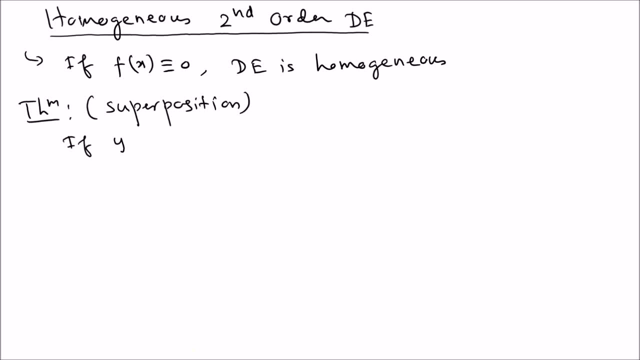 so what? it says that if, if y1x and y2x, if y1x and y2x are two solutions, are two solutions, are two solutions of the homogeneous equation, of the homogeneous equation. uh, if the homogenous equation y double prime plus px, y prime plus qx equals zero, then 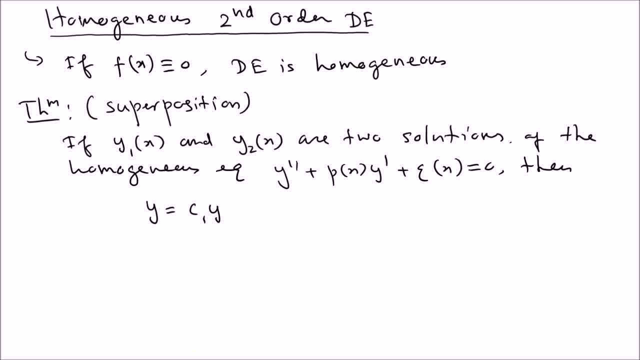 y equal c1, y1 plus c2y2 is also. is also is also a solution. it's also a solution for any, for any c1 and c2. so that's very interesting result. so what it says? that if you know that y1 and y2 are solutions. 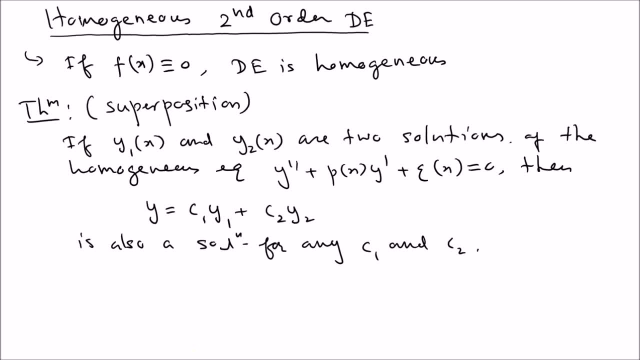 then for any c1 and c2 y equals c1 y1 plus c2 y2 is also a solution, okay, so, um, so this is a very interesting result and let's prove this one. so i'm going to prove this one. so we are not going to prove many in a review, but this is like one of the very 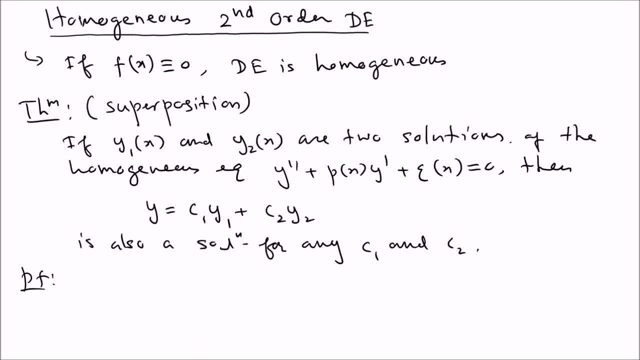 interesting result and you need to know this one. so i'm going to prove this one. so what we normally do is we can write the differential equation of l operator. so, uh, let's say, define l, that's the operator. so that means the second derivative. that means you need d squared, d x squared. 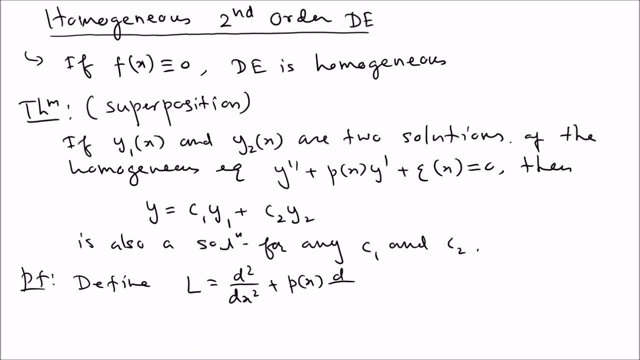 plus this one. we can say px d over dx plus qx, so we can define this operator, so um. and then what can happen? this particular differential operator? we define this difference operator and then we know that this differential operator is a linear operator. so linear operator means if you have a 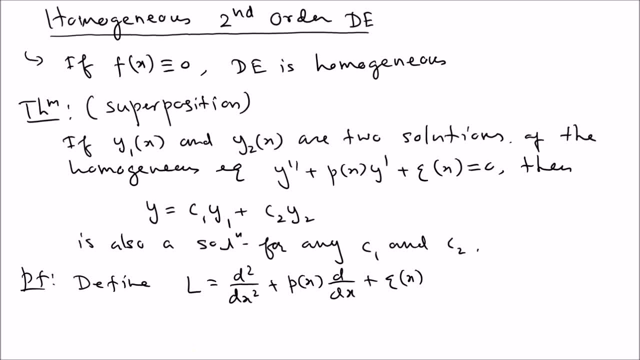 sum, you can write as as 2 and if there's a constant, you can pull it out. that's what we call a differential linear operator. so this is a linear operator. okay, so let's try this. this is a linear operator, so this is a linear operator. now, what we can do, are we gonna act on that? 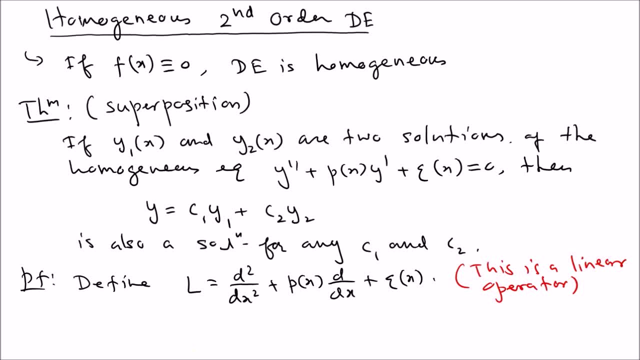 so, uh, so we know that y1 and y2 are solutions. that means if you operate on l, so that'll be ly1 and ly2 are zero, because that's because y1 and y2 are. we're going to operate on that. so, uh, so let's write it like this: 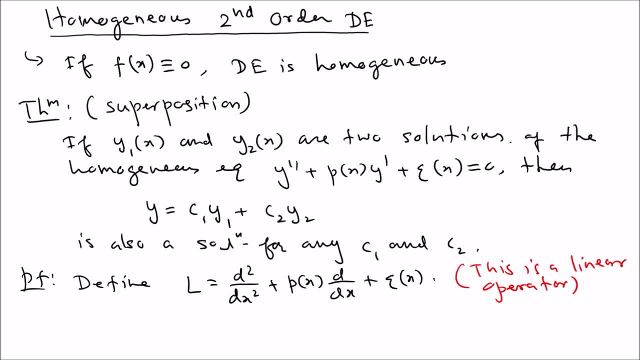 uh, yeah, i'm going to write this extra one. so this operator is linear. there is there are two results. the first one, l y 1 plus y 2, equal l y 1 plus l y 2. that means your sum. you can break it like that. that's the first condition. 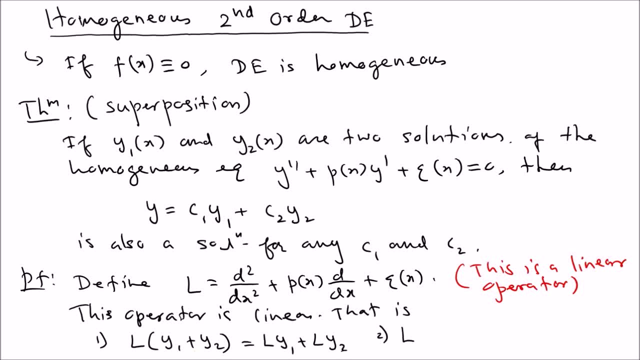 of a linear operator. the second condition is, if there's a constant and y 1, you can pull the constant out. so that's the second operator. so that's what we mean by a linear operator, linear operator. so now let's use that fact. so what we can do, we can consider l, y, which is the 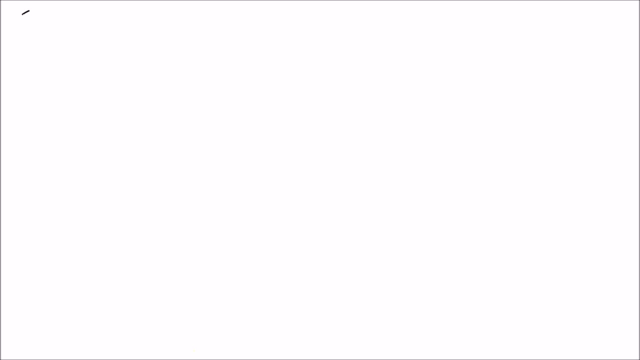 y, we can consider l y. so then, considering considering l y. but what is y? y means c 1 y 1 plus c 2 y 2. now we know that the l is a linear operator, so we're going to break it, so we can write this on l: 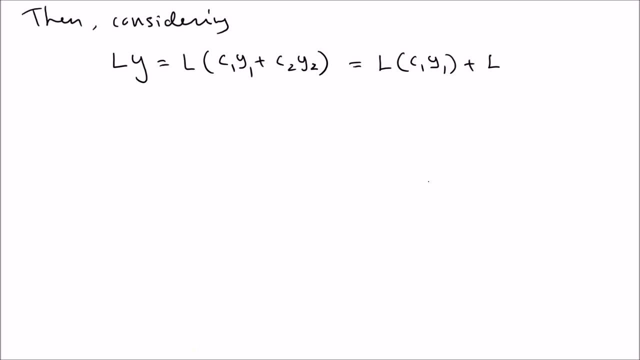 c 1 y 1 plus l c 2 y 2 using the first property. this is from the first property. now we're getting the second property. what is the second property? second property says you can put the c out, so l y 1 plus l y 2. sometimes we just write it like: 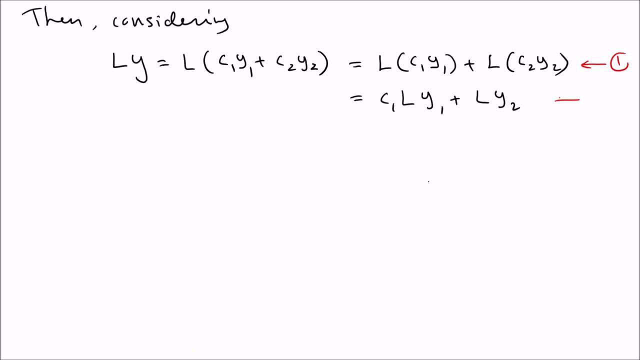 that, without even bracket, this comes from the second property. but what we know now? we know that since y 1 is a solution, this has to be 0.. since y 2 is a solution, this has to be 0 of 0 plus 0. that means the whole thing is. 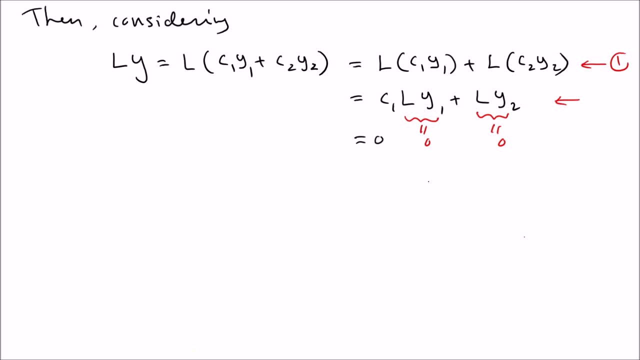 opened. this says that l? y equals zero. that means, so this implies that y is also a solution. so this implies that. so, therefore, therefore, uh, therefore, y is also a solution. so that's the proof. so very simple proof. are using linear operators: uh, so that's. 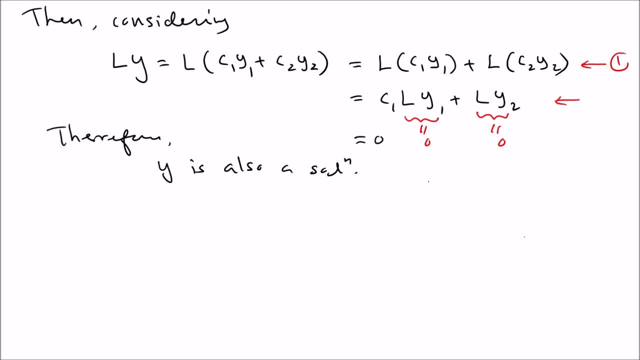 what you call the superperson principle. so let's try to grow to um the linear independence. linear independence, so what's the linear independent means? let's go with the definition. this is a actual definition. so if c 1, y 1- function of y minus the function of x, plus c 2, y 2 equals 0. 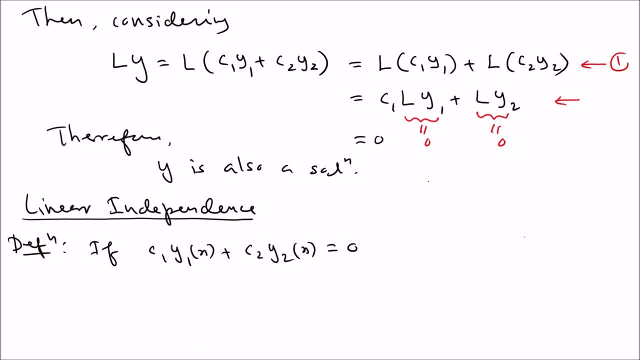 c 1, y 1, 0 for any x for any x implies that implies that this can implies that c 1 and c 2 are 0. that means there's only the trivial solution. if it implies that we call, we call y 1 and y 2 are linearly independent. 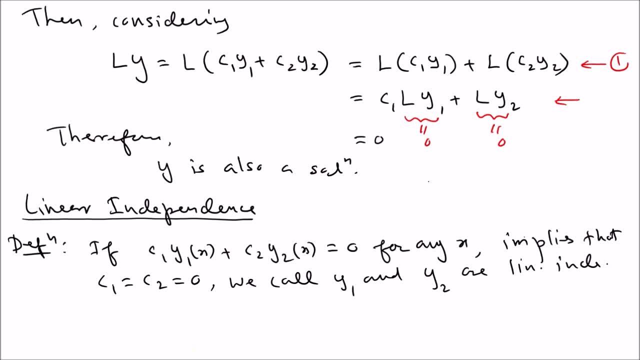 linearly independent. linearly independent. this because we are only considering two solutions, so we are two, but we can just extend this one for three solutions, four solutions like that. i just we just write for two. we are linearly independent if the functions are not linearly. 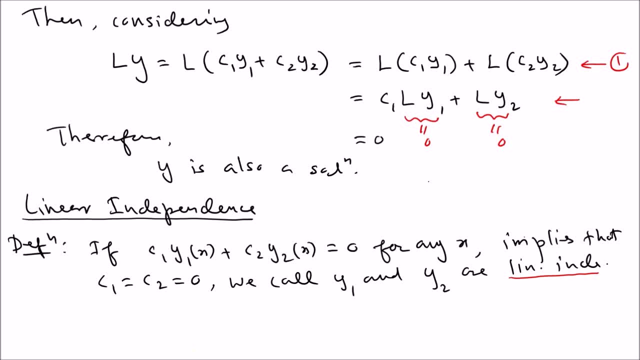 independent if the functions are not linearly independent. if the functions- shortcut fun- if the functions are not not linearly independent, if the function are not. if the function are not linearly independent, ah, they are, they are linearly depend because linearly depend. so what normally happens is we start with a with general set. 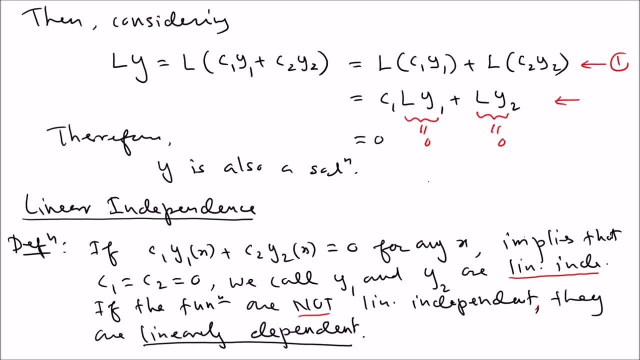 if there's a linearly dependent one, we can remove one. one of the dependent one, one of the dependent one. now, when you consider the new set, see whether this is linearly independent or dependent. if it's dependent, again we remove one linearly dependent one. we keep doing it at. 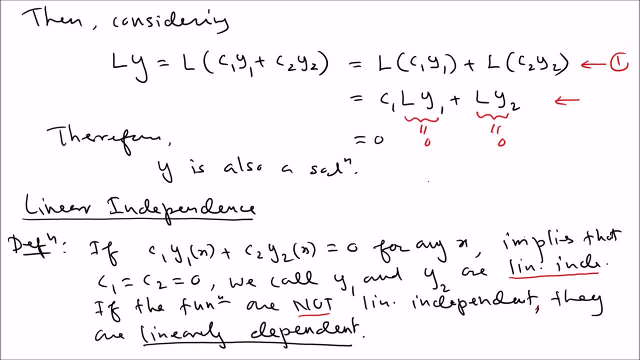 one point. what's going to happen? you get vectors. these are called vectors. actually they're going to be linearly independent, so we can do that like reduction method. we can remove. always try to remove a dependent one, then i we end up the set, which is linearly. 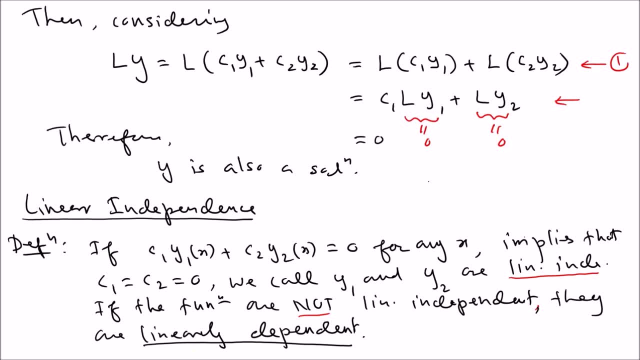 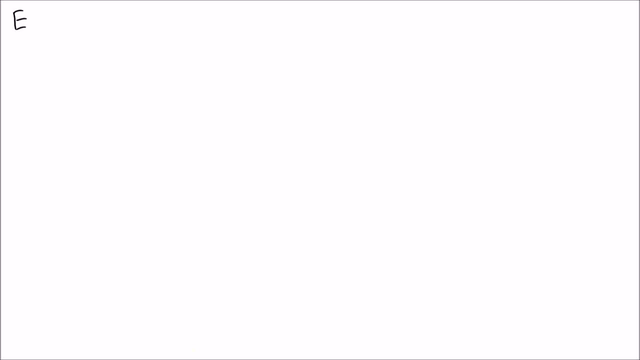 um, independent. that's the kind of criteria. so let's try to do like one example, just to see how things can work so that, so that, uh, y1 x equal x. that's the first function and the second function y2x is, let's say, cosine x. 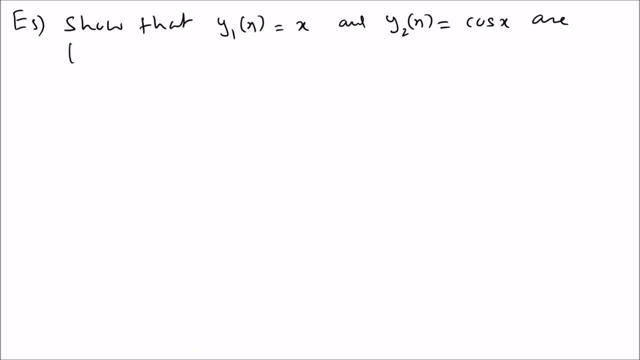 are linearly independent. so that means y1, x is linearly independent. so what we're going to? we're going to use a definition, um. so the answer so this is: suppose we have c1x plus c2, cosine x equals 0 for any x. 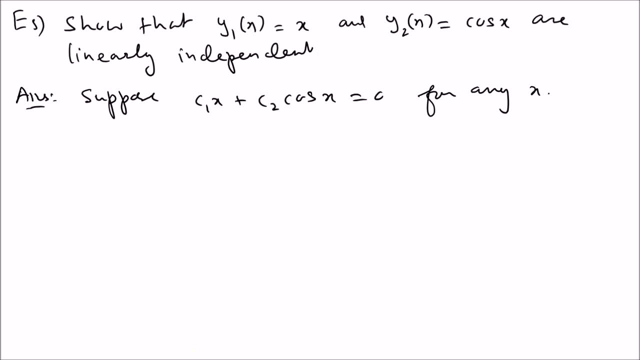 for any x. now what we can do, because this should be true for any x, so we can just pick any value we like. so we can say: x equals zero, uh. so substitute uh. x equals 0. so if you solve x equals 0, what will happen? 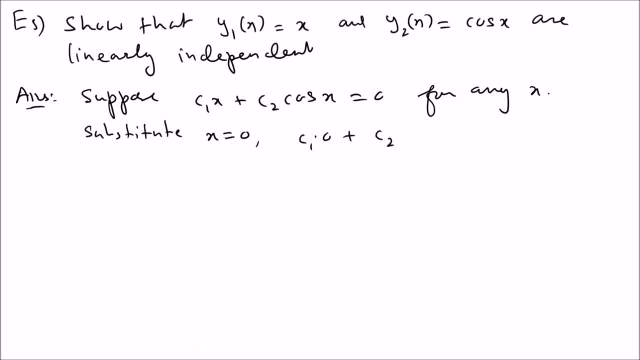 we get c 1 times 0 plus c 2 times cosine: 0 equals 0. should be true for any x. so we put x equal 0, so this is 1. so this says that, uh, c 2 equals 0. so now we prove that c 2 equals 0 now. 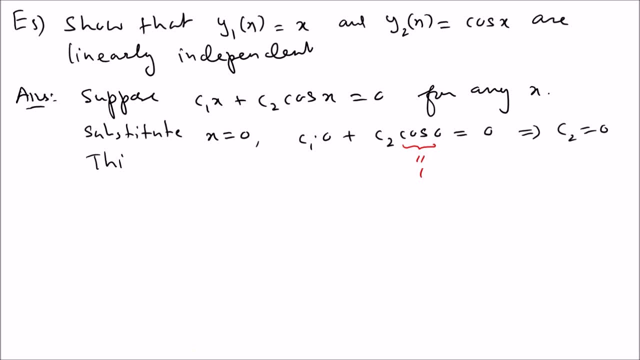 what we can do. so, uh, so that means this implies that solving a math problem is a logical argument. so that's why we write it like that. uh, so what we're gonna. so c 2 equals 0, so we only have c 1 x equals. now what we can do, just put, put any. 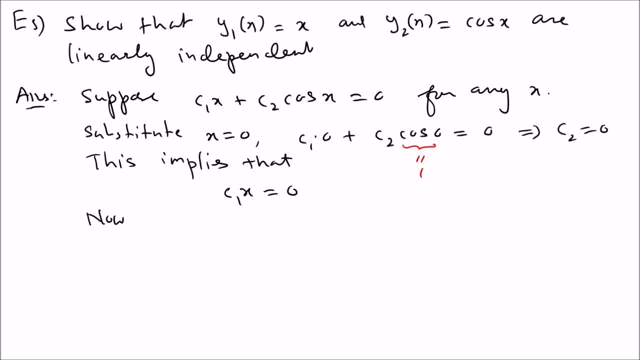 non-zero value. so now let uh x equal one. just pick anything other than zero. so this says that c 1 equals 0.. so what happened now? so so if you start with c 1 x plus c 2 x equals 0. if you start with this, 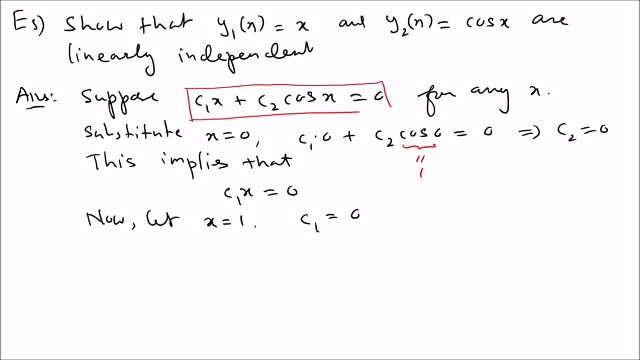 so we start with that. that's the definition- by proving the linear independent. by definition we assume that, and then we this implies that c 1 and c 2 has to be 0. so that means, by the definition, the two functions are linearly independent. okay, um. 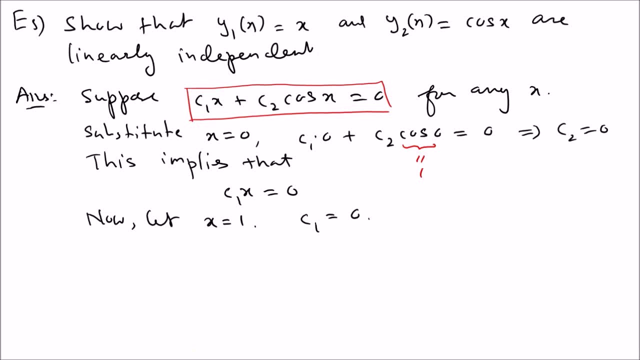 so we can see: uh, thus c 1 equals c 2 equals 0. okay, therefore, by the definition, therefore, therefore, by the definition, therefore, by the definition, y 1 x and y 2 x and y 2 x, and so on, x are linearly independent. 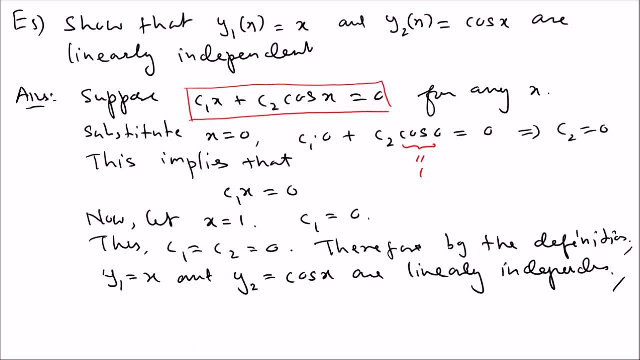 okay, so that's the proof. it's very short proof, but just substitute proper values and we try to prove the c 1 equals c 2 equals 0. so that's how we prove, like something linearly independent. now, uh, so this can be lengthy sometimes, so we have. 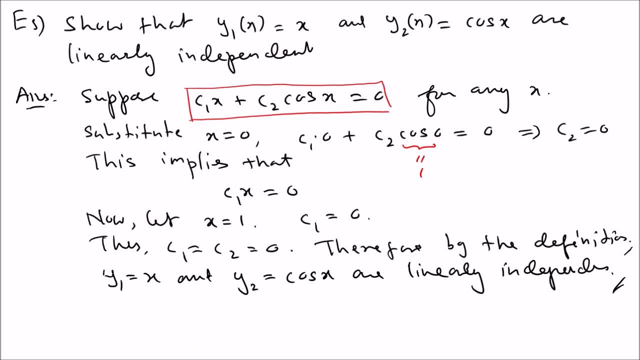 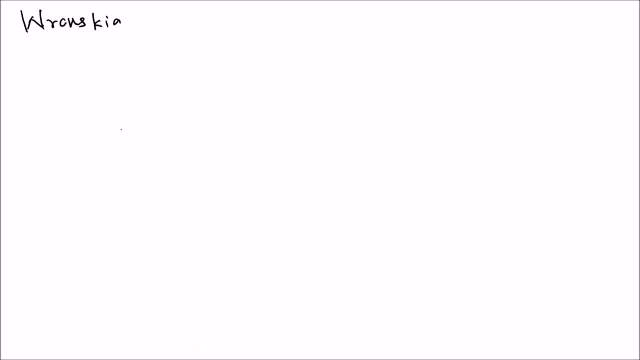 instead the what we call the wronskian test. so let's talk about that wronskian test for a linear independence. wronskian test for linear independence. what it says that we're going to calculate the wronskian. so what's the wronskian of two functions? 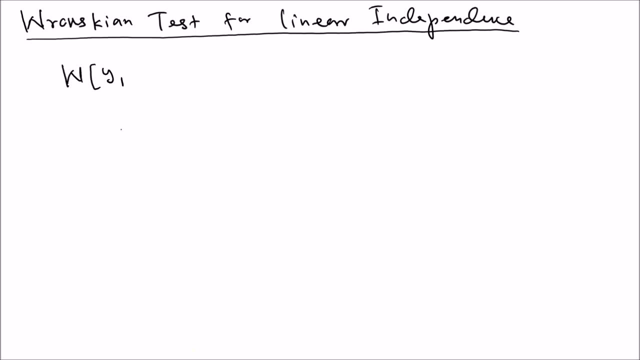 y 1 y 2. so it defined as a 2 by 2 matrix. so this is a two by two matrix. so we're going to calculate the wronskian. it is y 1 y 2, y 1 prime, y 2 prime, that's for 2 by 2. so what? 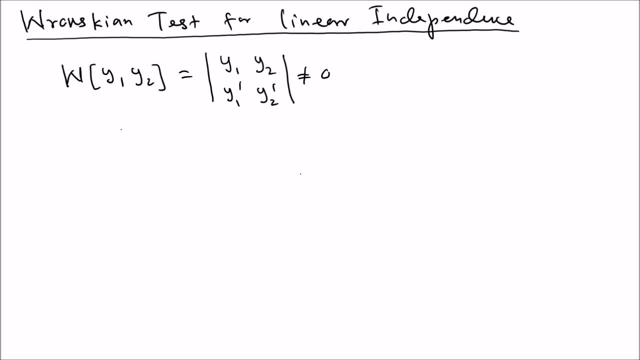 it says that if this is not equal to 0 for some, not all for some, all is good, but we don't need that for some x naught, some x value, then uh, y 1 and y 2 are linearly independent, are linearly independent. 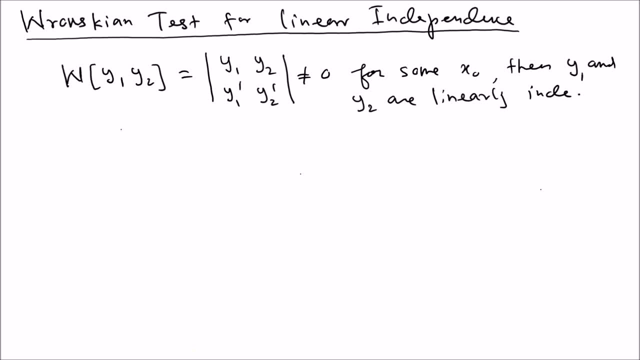 are linearly independent. we prove that where this is coming from. so you can look at the not uh to find out where it's coming from. okay, so let's use this idea to prove this result, just to see how it works, so that so that y 1 equal sine 3x. 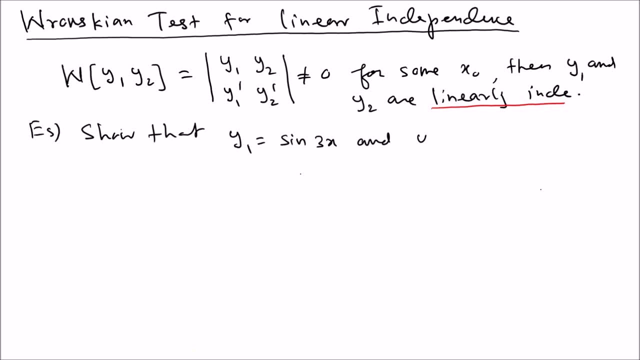 and y 2 equal cosine 3x are linearly independent. are linearly independent short form for the independence ah. so let's do the same thing. so we're going to go with the wranskian y 1 y 2, which is, according to the definition, y 1 y 2. 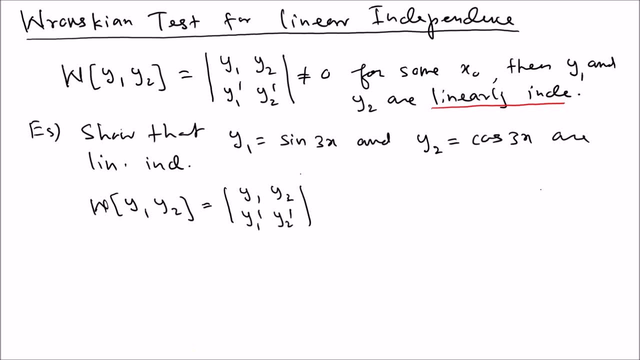 y 1 prime, y 2 prime. the substitute, uh, this is sine 3x. the derivative of sine means cosine 3 comes out by the chain rule. so it's a 3 cosine 3x. this is cosine cosine 3x by the chain rule. it is negative. 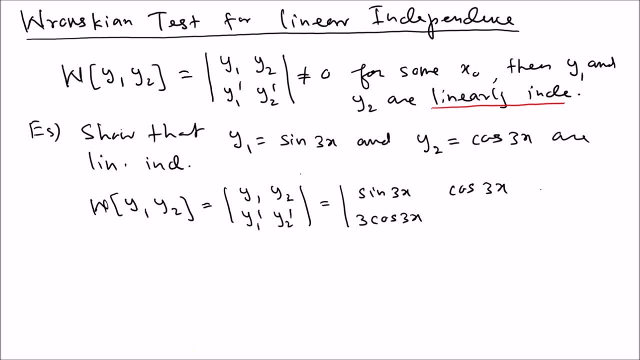 3 sine 3x. now what we're going to be going to find the determinant. this is a 2 by 2 determinant. we multiply the main diagonal and subtract the product of that diagonal, so we get the derivative of sine 3x and we get the derivative of cosine 3x. so we 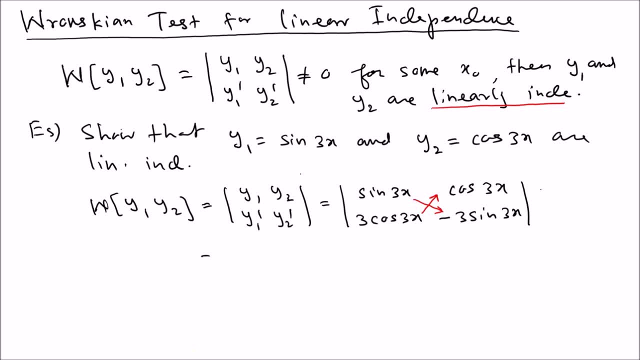 subtract the product of that diagram. so if you want for the main diagonal, you get negative 3 sine squared 3x, minus you multiply the other diagonal, so you get 3 cosine squared 3x. now what happened? you can pull the negative 3 out, so you get. 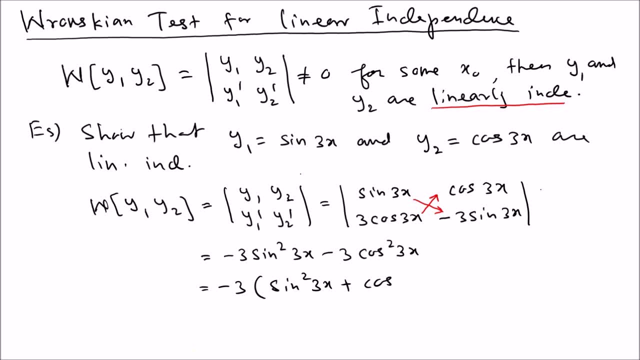 sine squared 3x plus cosine squared 3x squared 3x. we know that by the pythagorean identity. this is 1. you simply end up with negative 3. this is automatically not t equal to 0 for any uh, for any x. why for any x, there's no x. that means independent. 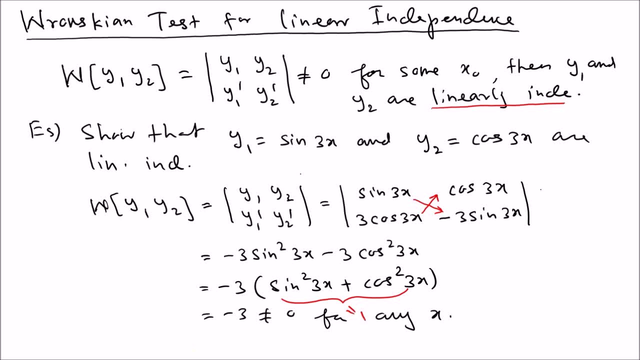 that is, you can say for any x. therefore, those two functions are linearly independent. so therefore, therefore, x, which is sine 3x, and y 2 x, which is cosine 3x, are linearly independent. you can see, that's very simple. uh, just need to. 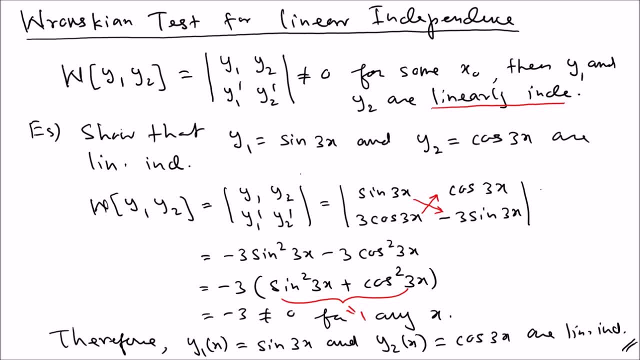 uh use the definition, uh, the definition of the wranskian, and then find the 2 by 2 determinant. if you forget what's the 2 by 2 determinant is, if you have a, b, c, d, the determinant we use the vertical bus is a- d. 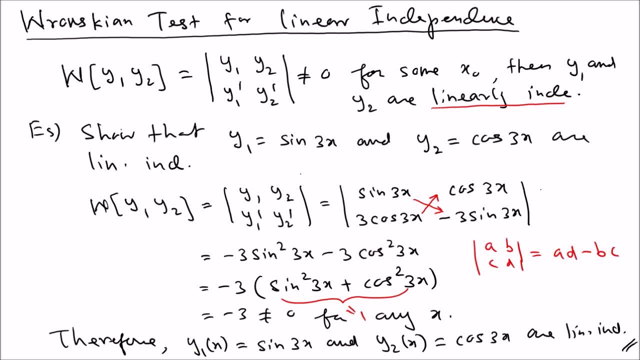 minus b, c, that's the 2 by 2 a determinant. okay, so now we have um. there are like kind of common sets, uh, which are in independent. so i'm going to give you that set because it's it's good to remember that, not just for this class but in general. 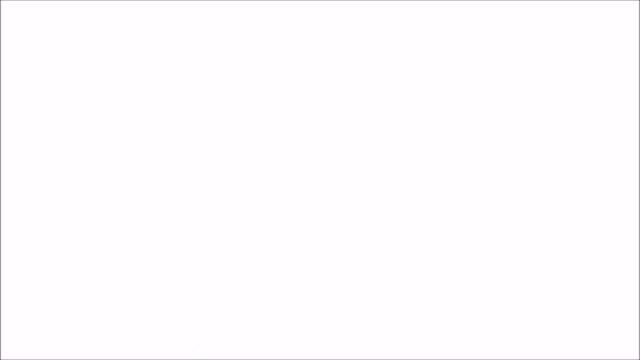 so let's, let's talk about that. um, so, it's a result: the following sets and their subsets. following sets. so if you pick any subset, still work. following sets. following sets and their subset. you can pick any subset and their subsets. we can just put any number of uh, uh. 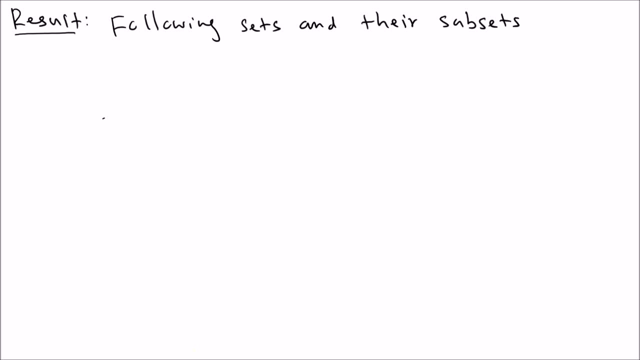 following sets and their subsets are linearly independent. so this is like kind of good uh set to remember. so let's, i'm going to give like about seven of them here, but there are more. so the first one is this: set one x, x squared x cube. 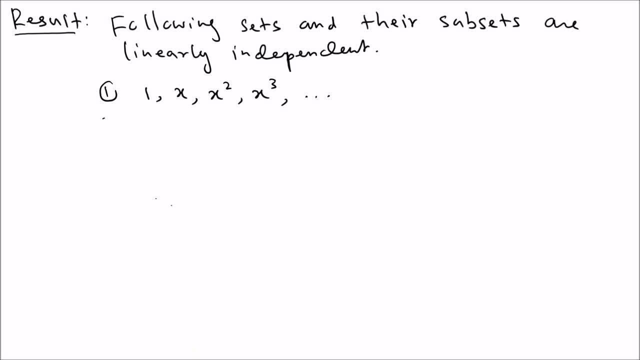 like that. this set is linearly independent. and if you pick any subset, for example one, two, those are linearly independent. let's say, you put one x squared x3, those are independent. that's why i say: any subset you can, this whole set is linearly. 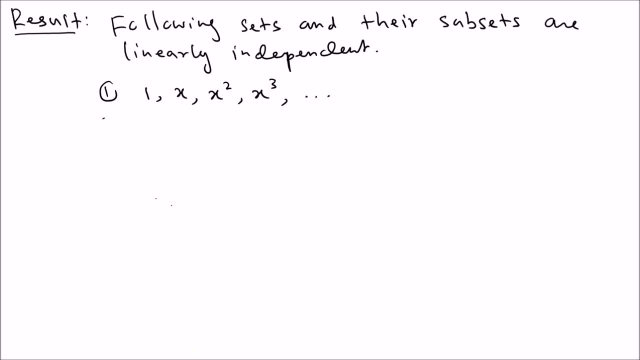 independent and even if you pick any subset of that, still linearly independent, because if you make it small, it's always independent. problem comes when you add more uh. the second one is one, i just add one. so if you make it small to all of them, uh, e, x- then you square this. that means e 2 x. 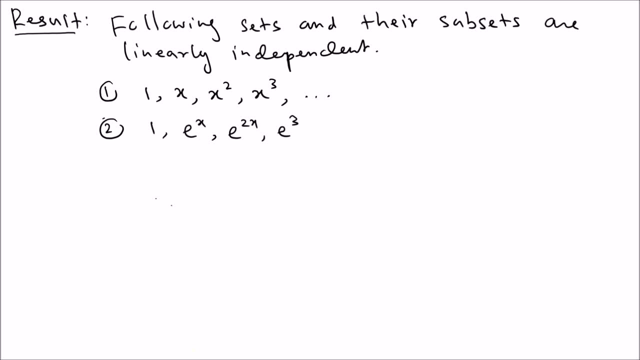 square: this e 3 x, not the square you multiply by another x. so like that. so this set is linearly independent: one e x, e 2 x e 3 x, like that. uh, actually you can just go with any general one. so for example, let's write: 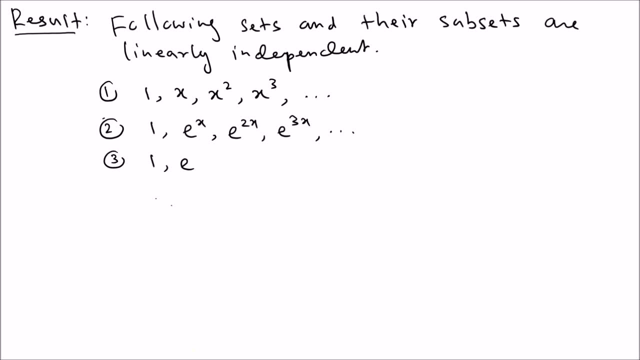 that. so i'm going to add one more, so it's a new one. e alpha, like alpha, is any non-zero number: e 2 and e 3 alpha, e 3 alpha, like that. so this set is linearly independent. number four: uh, how about this one, one x? this is a. 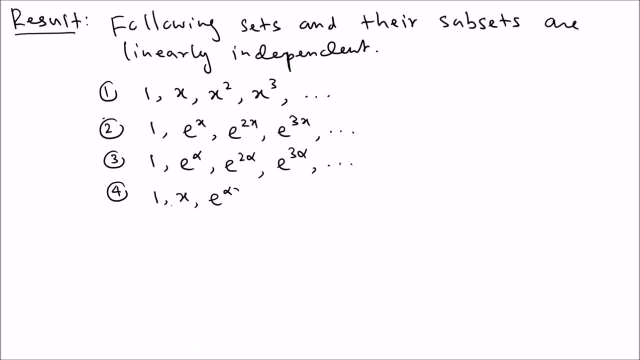 very useful one. we're going to use this a lot: e alpha x, and then we're going to multiply the two, so x e alpha x, and then x squared e alpha x. this set is also independent. you can just multiply by. so uh, so this set is linearly independent and 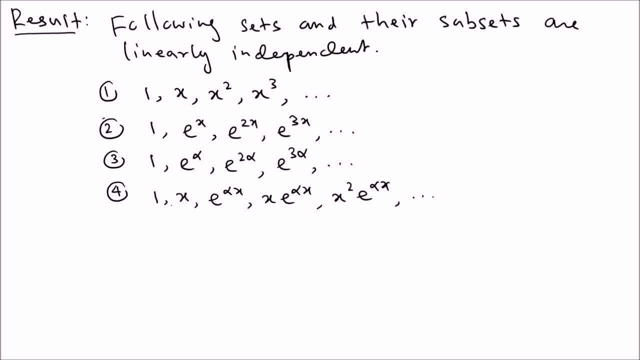 any subset of this is also really independent. that means x. no, for example, you can start with e alpha, x, x, e, alpha. that's like kind of common one, so we need this later. uh, when we talk about repeater roots, so e alpha, x, and then when you multiply by x, it's going to be really 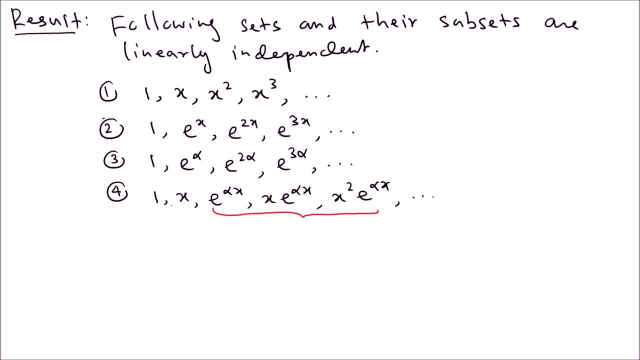 independent. when you have another one independent, this is like useful, very useful. uh, let's go. number five: um, uh, this one e alpha 1 x, e alpha 2, x, like that e alpha 3x. those alphas are different, so alpha 1 does not equal alpha 2 and not equal to any of the other ones. 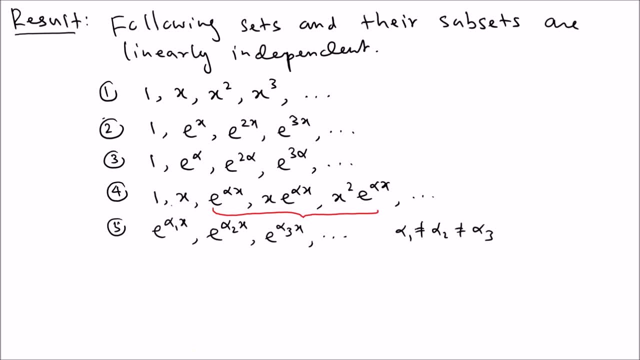 so actually this: this only applies to the other ones, so only says alpha 2, alpha 3, but it's also we have. it's not equal to alpha 1 as well. so if you want to write it like that, you can write it like that actually. so that's the idea. so all the alphas are. 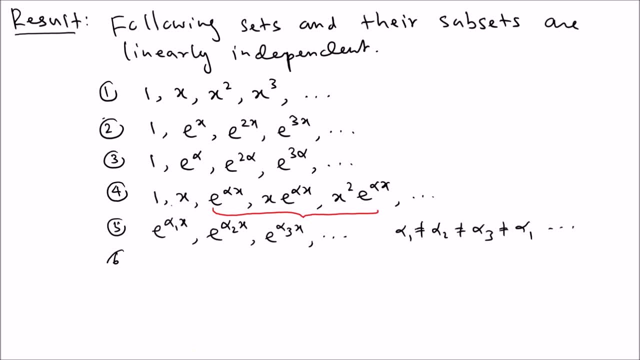 different. and then we have sixth one, uh one, sine x, cosine x, and then we have sine 2x, and then we have cosine 2x, like that. so this is very useful in fourier transform, and that's the fourier transform basis actually. and then we have our number seven. 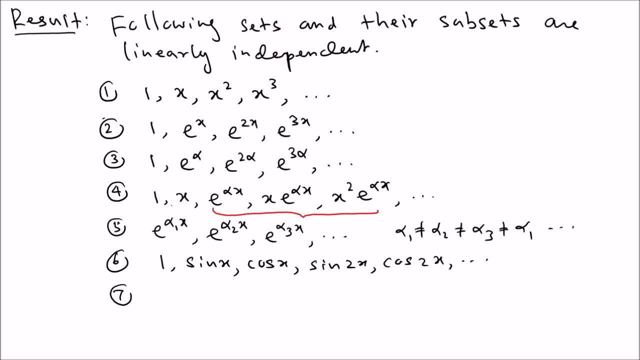 uh, we can square or multiply. we have one and then we have sine x, cosine x, and then we can square them. so sine squared x, cosine squared x, and even you can have any product of the previous ones. for example, you can have sine x, cosine x. these are all linearly. 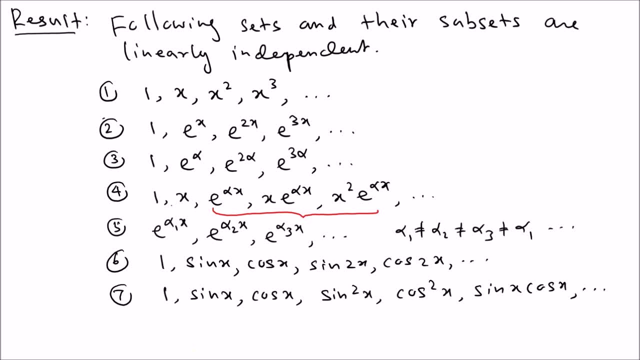 independent and any subset of this is independent. and as the eighth one, uh, i'm gonna write this one: x sine x, and then x sine x, like that. uh, x squared sine x. you get the idea, okay, like that. so those are all these. all those sets are linearly. 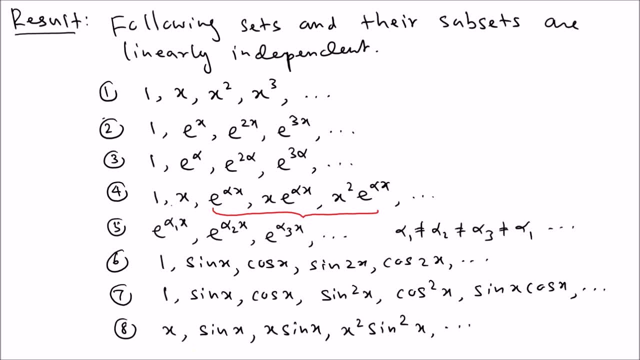 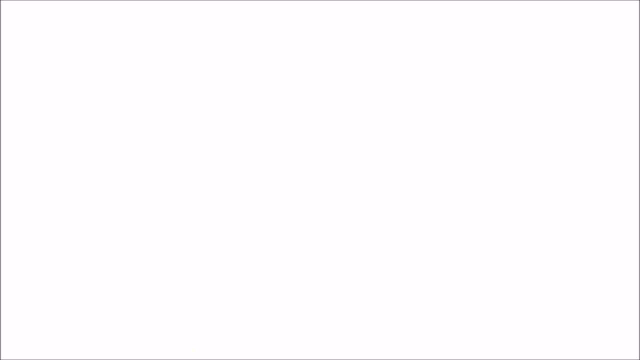 independent. so you can write this one x sine x, independent, and it's good to remember. okay, then we have this major result: um, so let's try this as a theorem uh, what we normally call the existence uh, theorem uh. so we can say: uh, if y1 x. 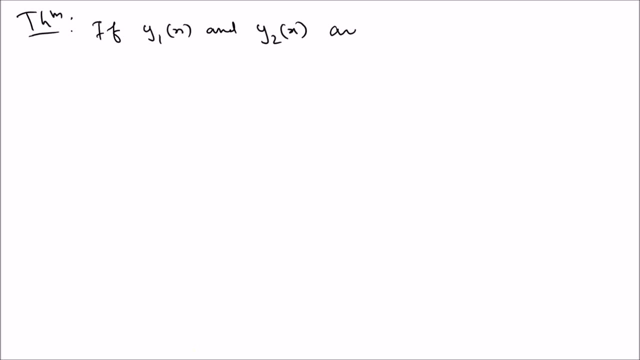 y2 x are two solutions are two linearly independent solutions are two linearly independent. this is very important. it has to be linearly independent. it's not really independent. this result is not true. okay, so if y1 x and y2 x are two linearly independent solutions, 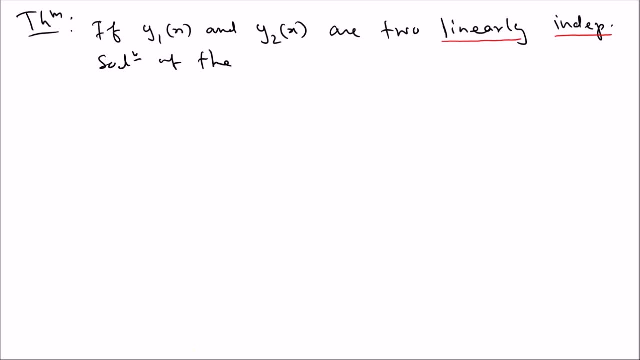 two independent solutions of the uh homogeneous equation. that's the homogeneous equation y double prime plus p, x, y prime plus q, x, y equals zero. the general solution, that means any solution you can write in this form: the general solution. the general solution is given by, is given by: 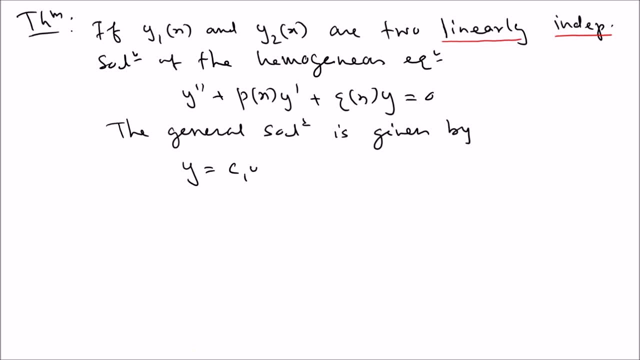 y equal c1, y1 plus c2, y2 um we are c1 and c2. are any constants? okay, these are any constants. so for any constant c1 and c2 um, the general solution is given in this form. for that you can write it like this: 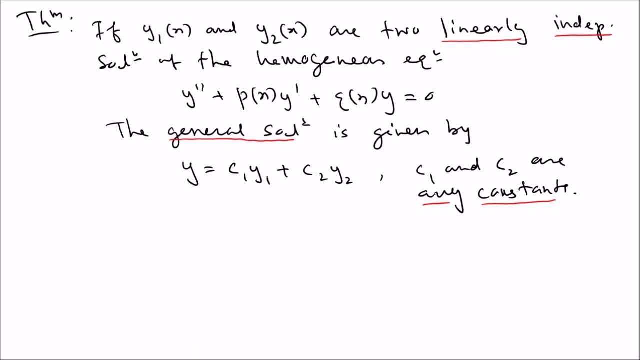 that y1- y2 has to be linearly independent. so that means any solution you can write in this form: y1, c1, y1 plus c2, y2, that's like really powerful result. okay, so that's about the major things. and then uh, so let's talk about the, uh, the non-homogeneous case. so that's uh. 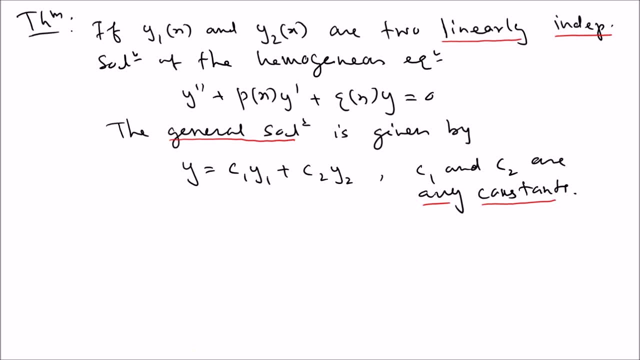 as we each of that topic we can talk about later, but we're going to put it here so that it does like everything is everything together, so none. this is all for homogeneous, but now let's talk about non-homogeneous equation. so the non-homogeneous equation. 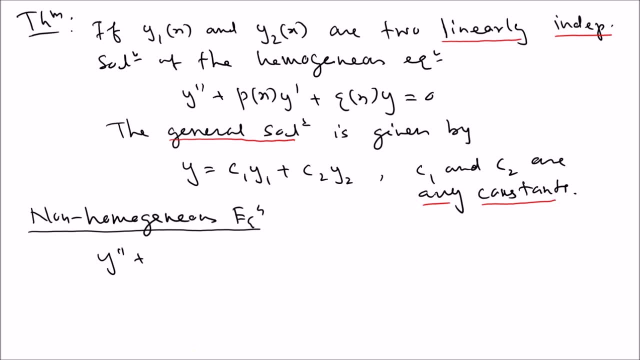 so what's the non-homogeneous equation? we have y double prime plus p x, y prime plus q, x, y, equal f x. so we are f x is not identical. it can be 0 for some values, but not identically 0. so the question is um how to solve it. so that's the question: how to solve. 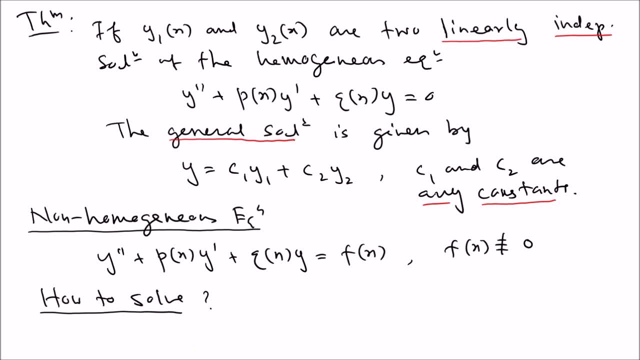 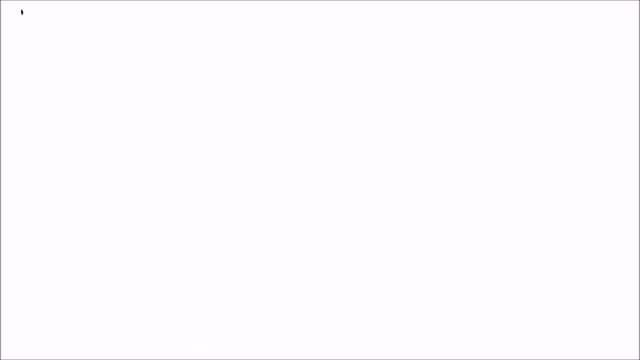 so what we can do, we can split the problem into two parts, okay, so let's talk about that. so what you can do, ah, so again, how to solve. split the problem in two parts. we're going to do: y double prime plus p x, y prime plus q, x equals zero. we're going to get 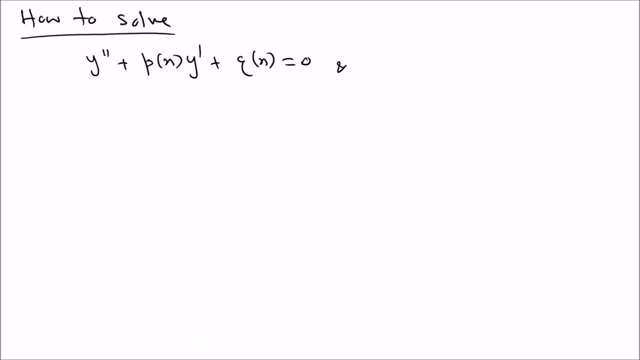 this part and that's what we call the complementary problem. and then we're going to talk about the whole equation again: y prime plus q, x, y equal fx, the whole equation. what we're going to do from the first one, the homogeneous equation, we're going to find the general solution, so find. 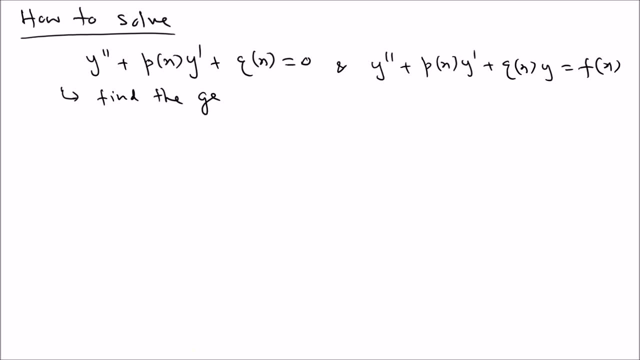 the general solution of the homogeneous equation, find the general solution. we know that this general solution you can write as we're going to call. this is a complementary solution, we're going to call yc. we know that the general solution of this one has the form c 1, y 1 plus c 2 y 2 for 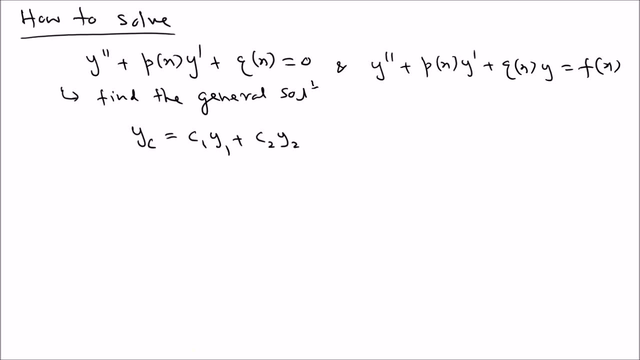 yc 2 solutions. so this one is what we normally call the complementary solution, as i put a, c here- complementary solution, and then from the other one we find one solution, find a particular solution. find a particular solution. here we find a general solution, here we find only one solution. 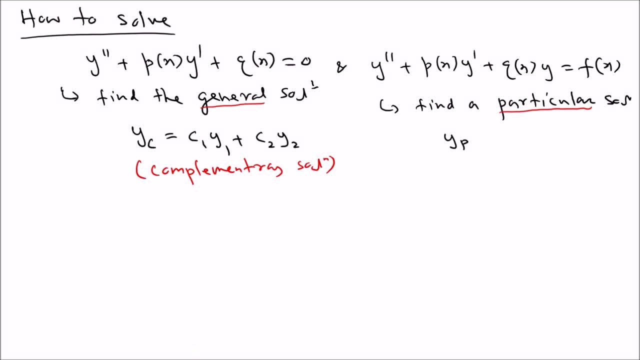 uh, so this solution, what we normally write as yp, because yp, that's the one solution, the particular solution. so this one is what we call the particular solution and then the general solution of the non-homogeneous equation. so the general solution, general solution of the non-homogeneous. 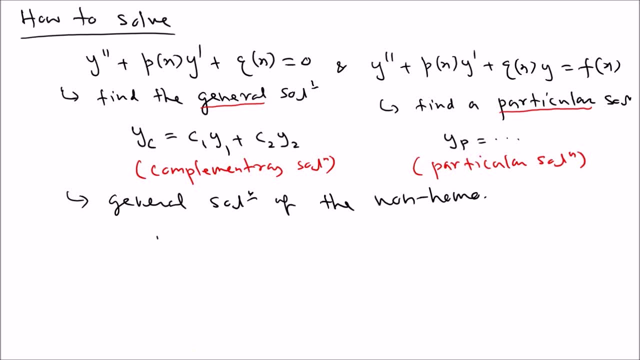 unhomogeneous equation is given by: y is the sum of the two y c plus y p, which is c 1, y 1 plus c, 2, y 2, equal y, p. and we know that. how many conditions, how many unknown we need, how many c's we need because this 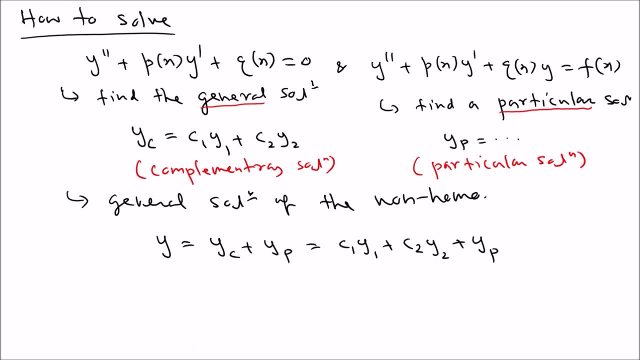 is a second order differential equation. that means we need two, and you can see that those are those two unknown. ah, so this is the general solution with two unknown, and we can find those c1, c2 using the initial conditions. okay, so, uh, so that's the. that's the form of the. 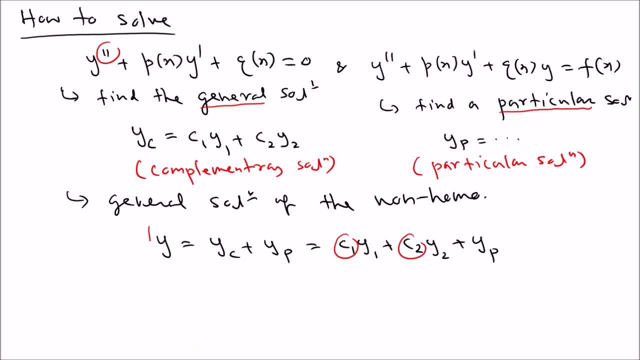 general solution of the. a second order, non-homogeneous equation. okay, uh, to find the non-homogeneous equation, the uh, two methods. so let's talk about write that. to find y p, we use two methods. the first one is the undetermined coefficient method that we discussed later in the discussion, and then we also use the 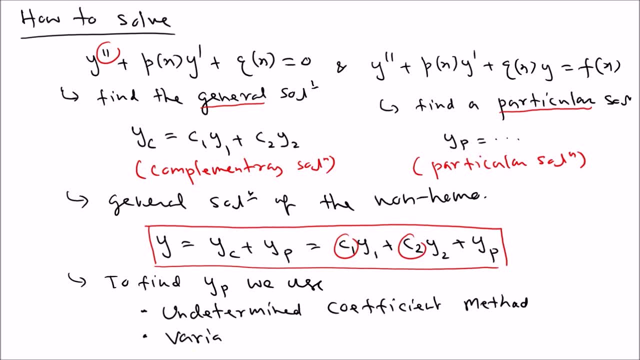 variation of parameters method. uh, the problem is, uh, fused, undetermined coefficient method. there are only three cases that we can do. there are only three cases. we can talk about those three later, but we can use the variation parameters in that case. uh, the only problem is that we can use the. 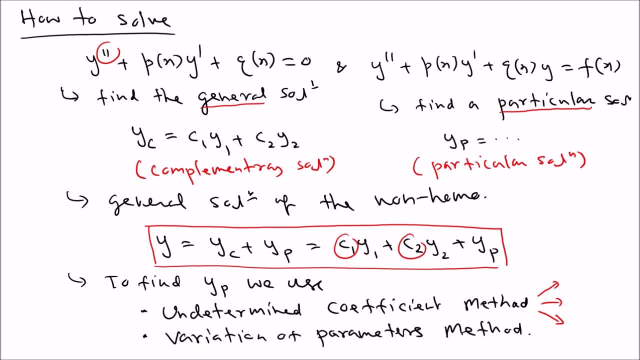 undetermined coefficient method that we can do. so the problem is you might get an integral that you cannot do. then you're going to get stuck again. but otherwise you can use that again to find c1, c2. we use initial conditions- okay, that we normally do at the end to 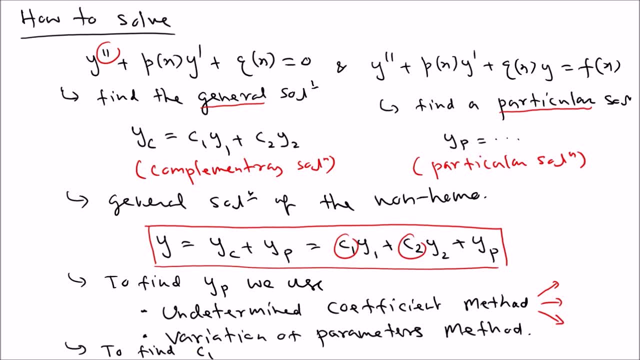 find c1 and c2 use initial conditions. so we use the initial conditions. so we use the initial conditions. so we use the initial conditions at the end. so remember that it's kind of joke, but that that's how you remember initial conditions you use at the. 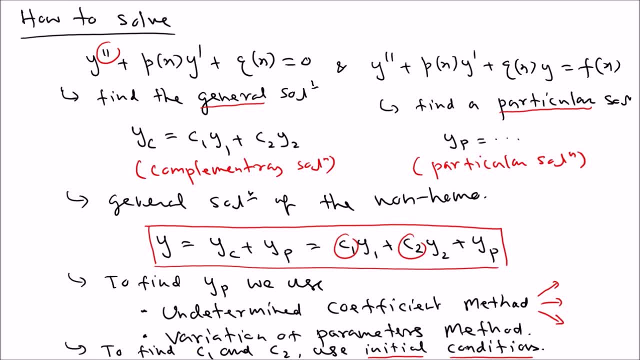 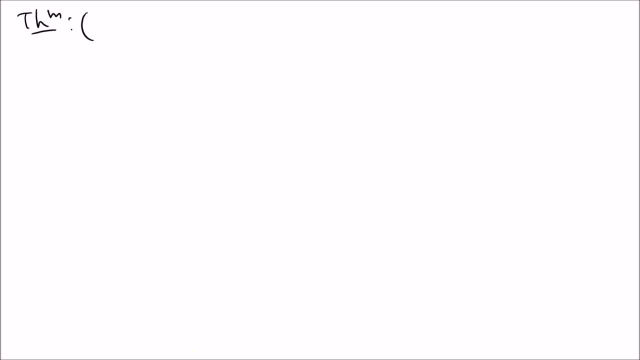 ends. okay, so that's about that, uh. and then we have this, uh, existence theorem for uh, um, second, uh, non-homogeneous equations. let's write that so it's a theorem, existence and uniqueness theorem. so what? it says? that if, if p, q and f are continuous, are continuous. 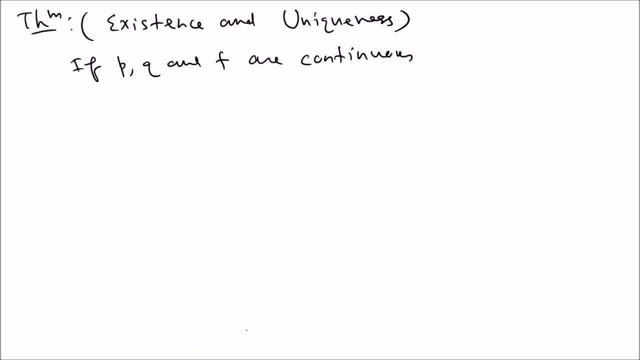 are continuous uh on some interval. so on some interval containing a containing a uh. then then by double prime plus p x, y, prime plus q x, y, equal f, x. has a unique solution. that's very important. has a unique solution. that's very important. has a unique solution. 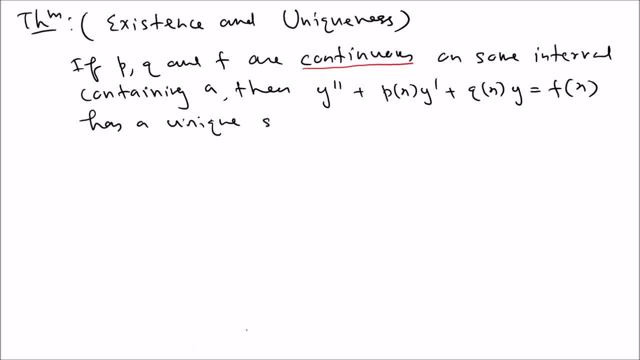 so that we have defined the separation, uh, solution, satisfying. so it's fine. why a equal b and y prime a equal b, 1 on that interval. i so what it says that? ah, if so, on that interval, it says that there's a unique solution because the way i said, interval coming from, because that's where those three 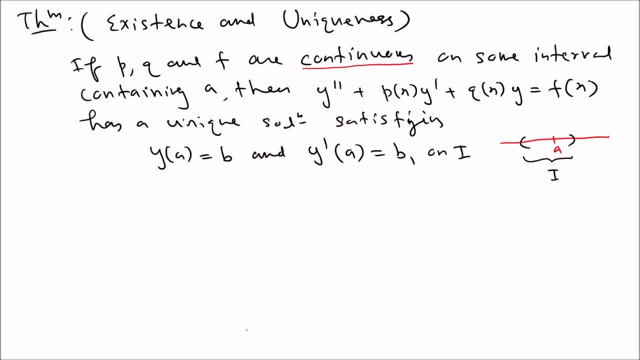 functions are continuous, so in that interval there's a unique solution. so it's very interesting result. okay, so let's just do one last example, um from what we discussed so far. uh, so two solutions, two solutions of x, double prime minus x, prime minus 12 x. 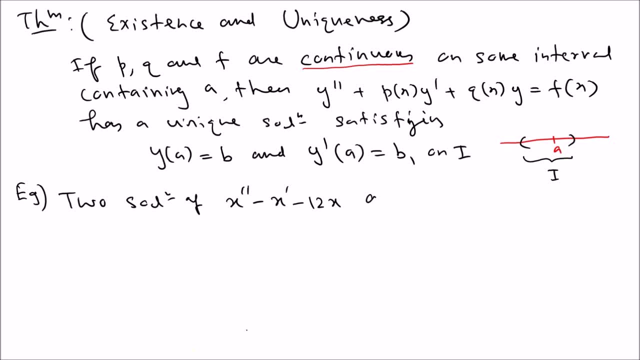 uh are given by that will x equals 0 equal 0 are given by. are given by x 1 equal 2 e negative 3 t and x1 negative 5 e 4 t. so that, so that they are independent, so that they are. 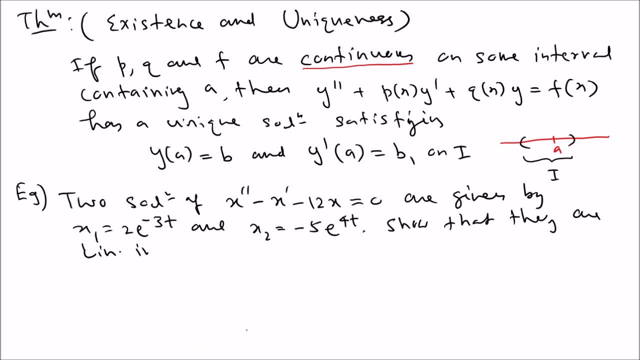 linearly independent. we can use the wronskian test for that. y 1 y 2 ah, not y 1 y 2, is x 1 x 2 ah. so we have x 1 and x 2, so it's x 1 x 2 x 1 prime. 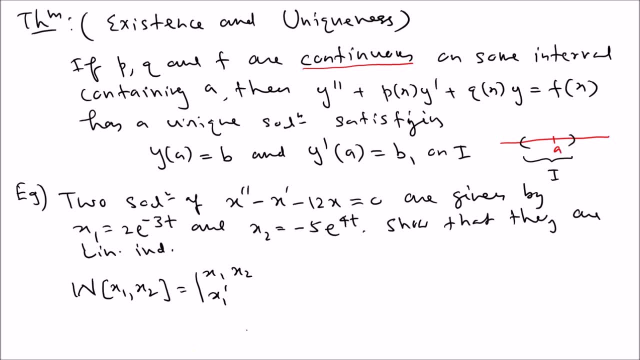 x 2 prime. so if you plug in 2 e negative 3 t, it has a derivative negative 6 e negative 3 t, and then we have negative 5 e 4, negative 6 e negative 3 t, so negative 20 e 4 t. 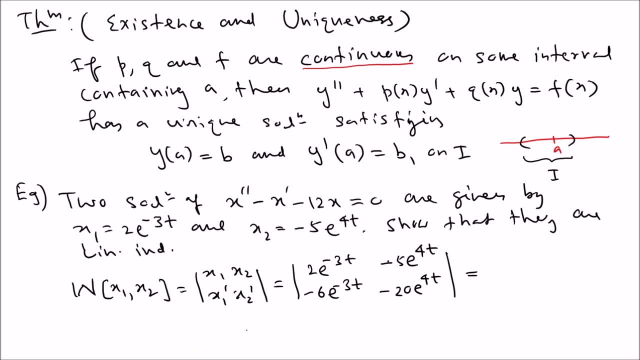 ah, let's take the determinant again, multiply this first and subtract that. so what you get? if you multiply that one, you're going to get negative 4 t e, negative 3 t times e to the 4 t, and when you multiply the other one, you 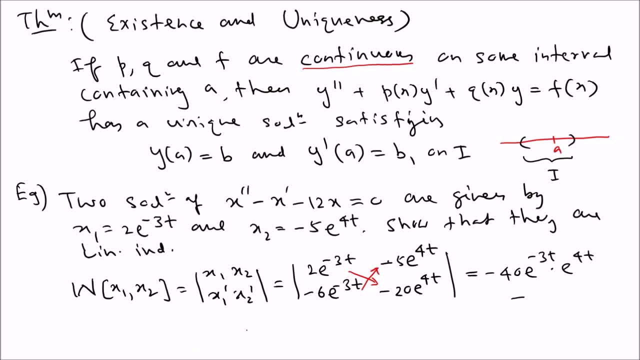 get positive and again minus because of uh. it's a b a d minus b c, so you get 30 uh e to the negative, 3 t times e to the 4 t. when you multiply you get negative 70 e to the t, which is not equal to 0 for any t. 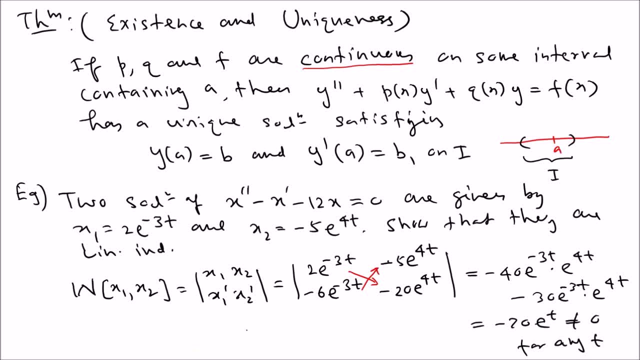 we only need one t, but so for any t doesn't equal zero, so that's the problem. so that's the problem. therefore, therefore, x 1, which is 2 e negative 3 t, and x 2, which is negative 5 e, 4 t. 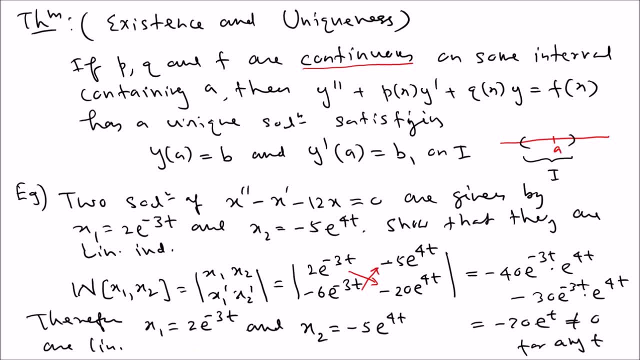 are linearly independent. good, so that's the problem. so that's the problem. so that's the problem, so that's the proof. are very simple, so, uh, so that's the uh, about basics, about the um, second order, difference equations. now let's move on to the reduction order. reduction of order. 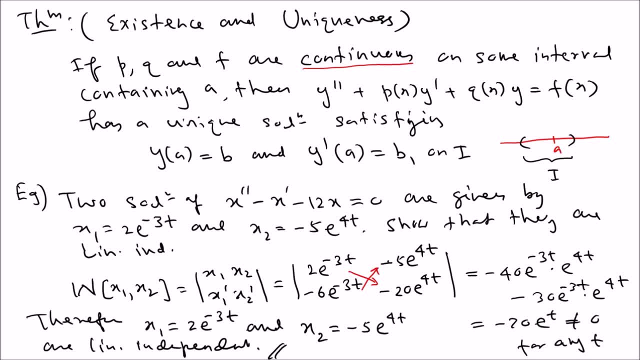 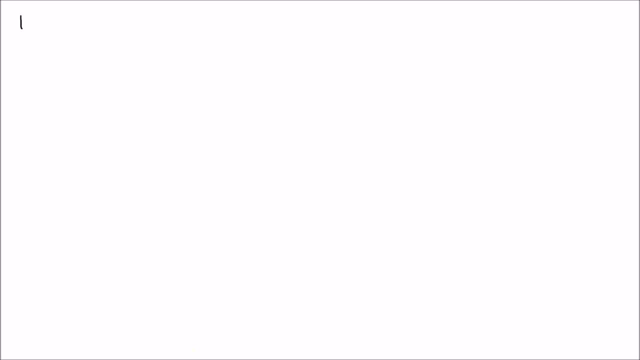 method. so in this uh we can talk about the uh reduction of order method. that's number 17, a reduction of order method. reduction of order method. so what's going to happen? ah, you start with the higher order differential equation and you're going to bring one level down. 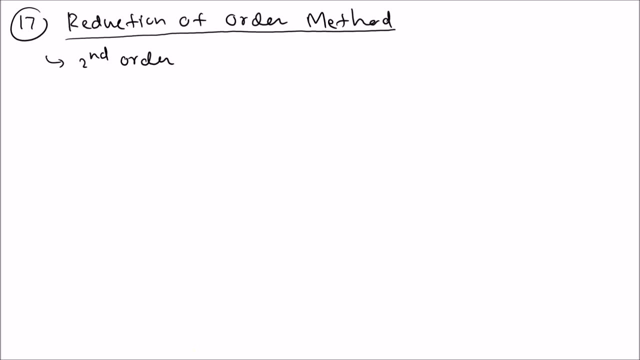 so that means second order differential equation. uh, second order differential equation you can write as a first order differential equation. that's the idea. that's like a reduction of order order. go down so how it works: um, one solution is given. one solution is given. uh, find the other solution. find the other solution. 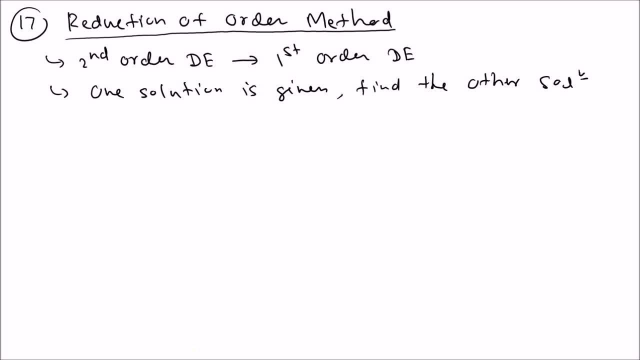 that's the kind of idea: find the other one, find the other one given um. so how it works? so, uh, let y 1, which is not equal to 0, be a solution. okay, that one we know. okay, we know this, so we know this one. now, what we can do, we can assume a solution. 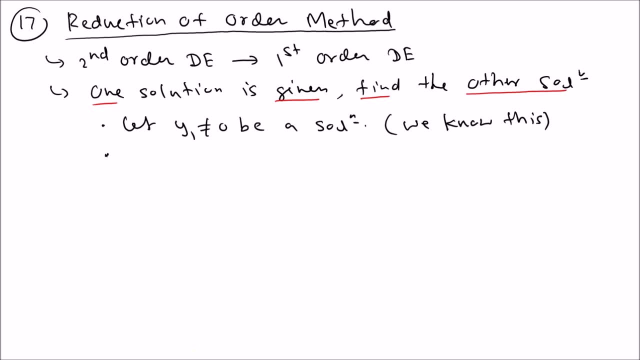 okay, so we can assume, assume a second solution. assume a second solution: uh, of the form, of the form y equal. that's the second solution. let's call it y 2, y 2 equal. the y 1 solution times the solution times u. so u is unknown. that's the way we need to find. 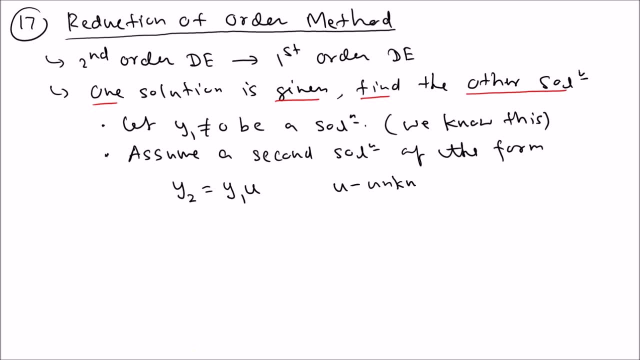 uh, the unknown function. we're going to find that unknown function, so the goal is to find this. okay, that's the starting point. we're going to assume a solution of the form y 1 times u. goal is to find you. okay, goal is to find you, so the goal is: 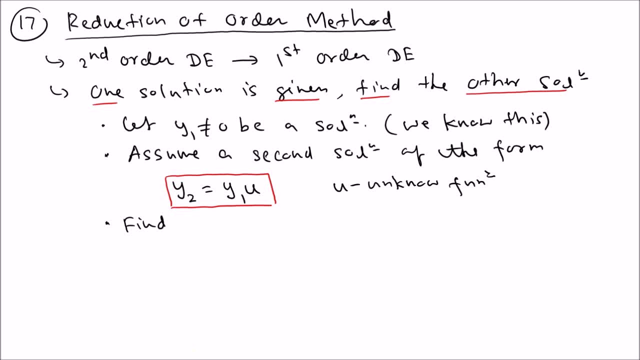 to find you, because after you find you then we know the second solution. okay, but how we do it? we can start taking derivatives and then plug into the equation and then solve. so that's how we do it. um so, uh. so we can start with taking the list, so we have this one and then we can take uh. so, take uh, find you. 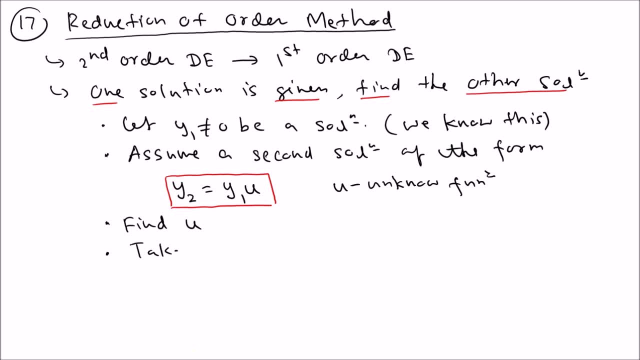 so what? we're going to uh, take derivatives. take derivatives and substitute into our formula. so what is that? so, uh, so difference equation is y double prime, uh plus p, x, y prime plus q x. so we're gonna uh: q x, y equal zero. so we're going to plug in here. so we're gonna take derivatives. 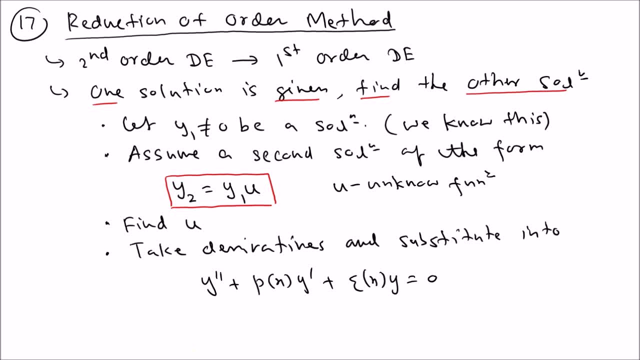 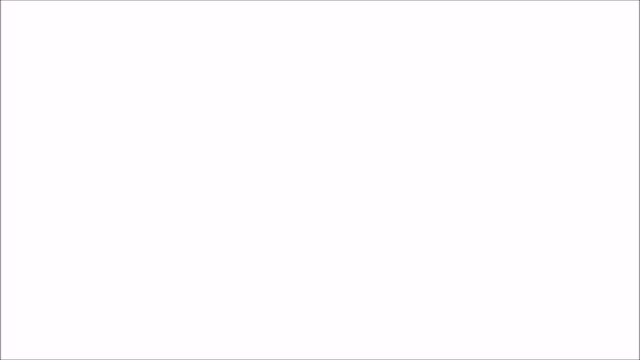 and plug in here. so let's see how it works now. um, so we have y, we have y2 equal y1 u, so take derivatives, so that means y2 equals y1u by the product rule. uh, this can be y 1 prime u plus u prime y 1. that's what you get from the 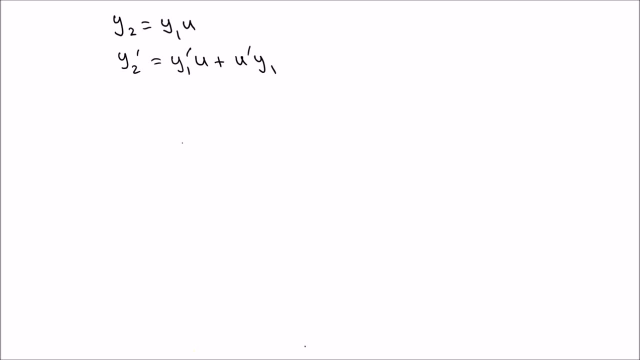 product rule. now: uh, let's take the uh derivative again. so if you take the second derivative, y 2 double prime, now we have two, so you get four terms. so we can take the derivative. so it's a y1 double prime, u plus y1 prime, u prime from the other one, u double prime. 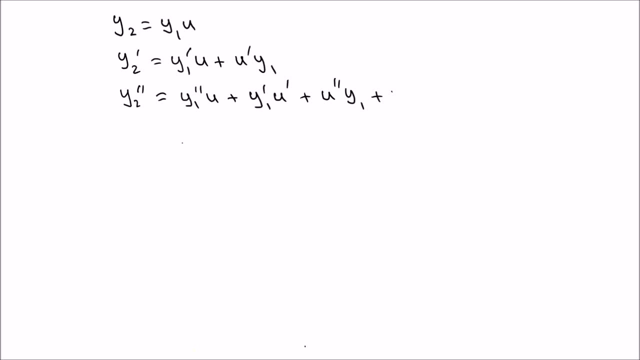 y1 plus u prime y1. now you can see that you can combine these two and write one equation. so you can write this one as y1 double prime, u plus two, using that u prime y 1 prime, and then we have u double prime y 1. 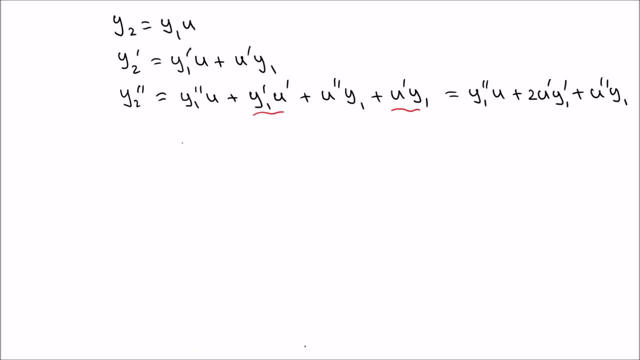 good, now what we're going to do. we're going to substitute this. okay, because we know that this is solution, since y 2 is a solution of y prime p, x, y, double prime plus p, x, y prime plus q x equals 0. we can substitute here, so we're going to get 0 equal. 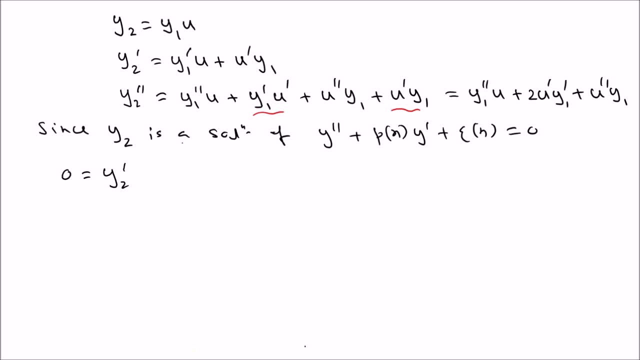 um, we have y 2 double prime plus p x- y 2 prime plus plus q x- y 2, so let's plug in for each term. so what is y 2 double prime? that is y 1 double prime, u plus 2 u prime, y 1 prime. 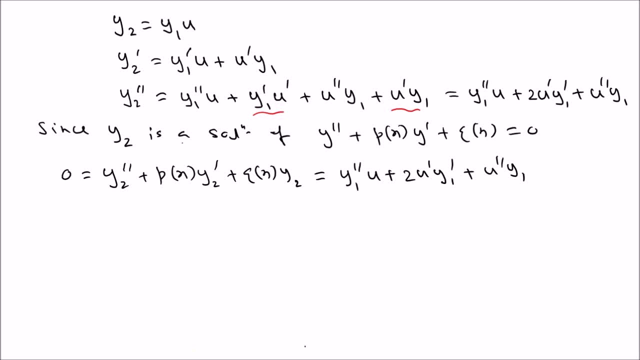 plus u double prime y 1. that's the first one. it's coming from here. now p x times p x times u 2 prime u 2 prime means u 1 y 1 prime. u plus u prime y 1. it's coming from here: 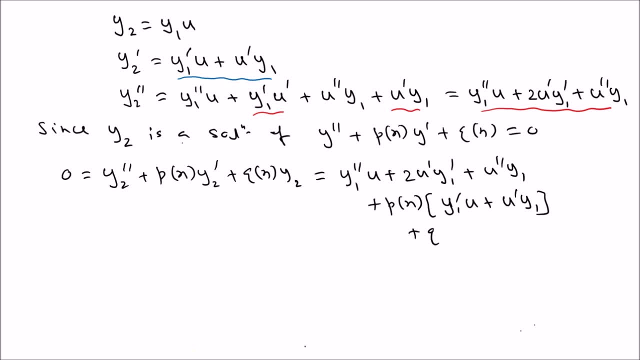 now the other one, which is q x times y 2, which is y 1- u. but we know this whole thing equals here. now what we're going to do, we're going to kind of collect the terms in a different way so that we can use the fact that y 1 equals 0. 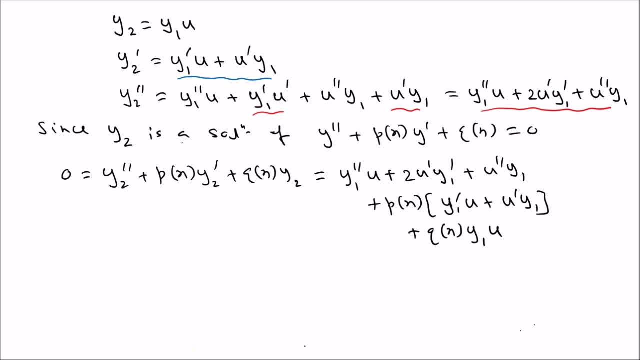 y 1 is the solution. so what we're trying to do, we can isolate the u terms. we're going to. we're going to go with the u double prime terms first. so what are the u double prime terms? uh, u double prime. we have y 1, um u double prime. that means this term. then we're going to. 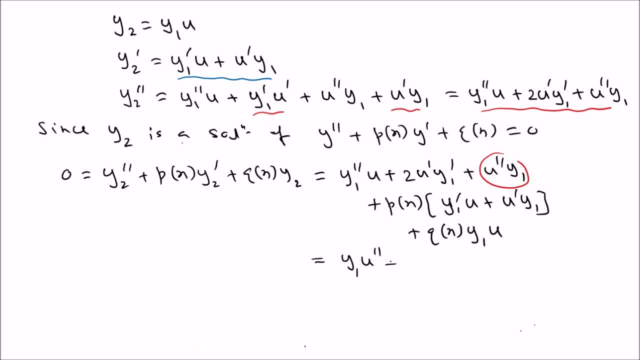 go with the y prime terms for the y prime terms. um, let's collect all the y prime terms. we have two y 1 prime plus that's that term, and then we have the other y prime, so this is another y prime term. so let's collect those two together so we have px. 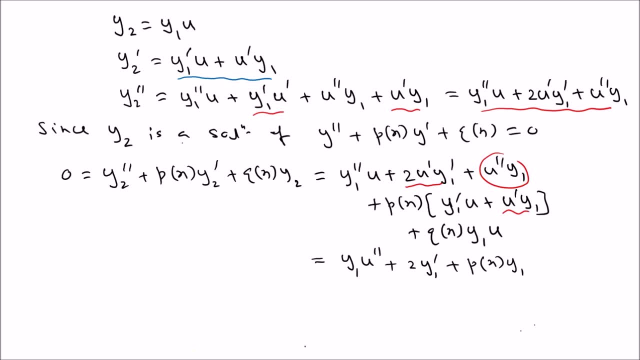 um y 1. so those two have a y prime term plus um u prime terms. and then let's call the u terms or u terms. uh, there's a u term here, there's u term, here, this other u term. let's combine all of them and take you out as a factor. so you're going to get. 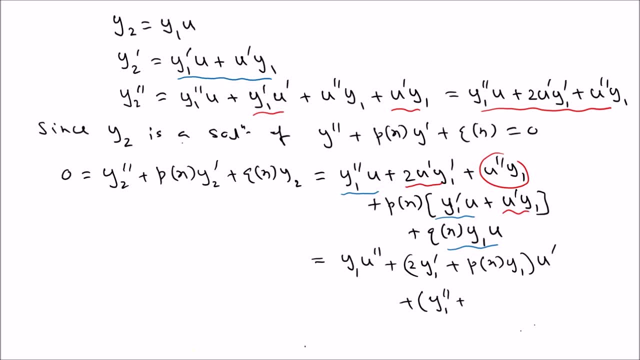 y 1 double prime plus from the second one: p x y 1 prime plus q x y 1. that's what you get from the u terms and then take u out. but we know that y 1 is a solution. that's we know that means this has to be 0 because y 1 is a solution. 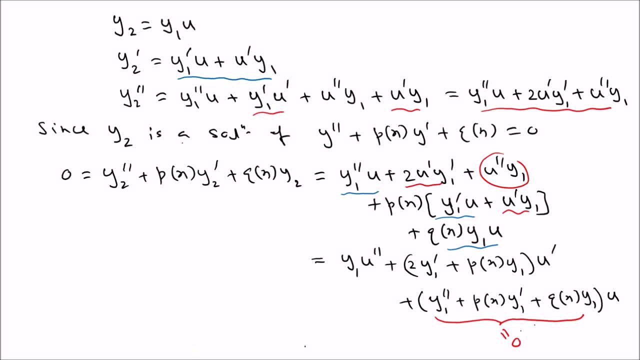 so that means that term going to go away. so you simply end up with this expression: y 1 u double prime, plus two times y 1 prime plus p y 1 u prime. that's what you have. so that means that has to be equal to c, right, because that's. 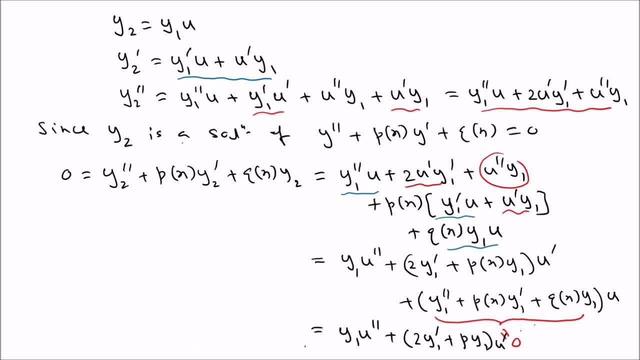 that's the whole argument. that's what we're going to do. you can assume a solution, take derivatives and plug in, and you can see that there's a special term that's going to go away because y1 is a solution, and then you simply end up with a new expression. so what we have now. so this is the. 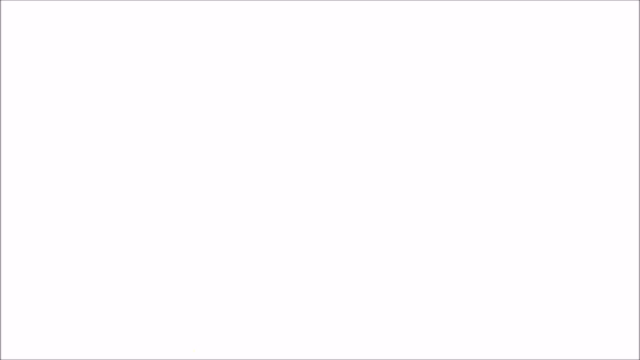 interesting part. so we only have this one. so we have y1 u double prime plus 2 y1 prime plus px. y1 times u prime equals zero. so that is the equation we end up with now. the goal is to solve this for you, solve for u, but you can see that there you. 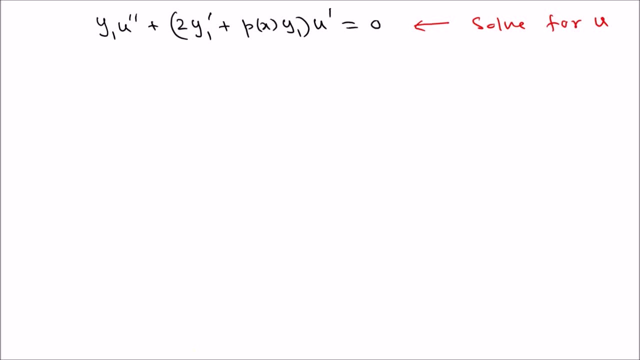 u prime, is there not u u prime? so what we can do, we're going to make a reduction of order here. so what we're going to? this is the whole point. so we're going to say: let v equal u prime, u prime if you say v equal u prime, since there's no u term here. 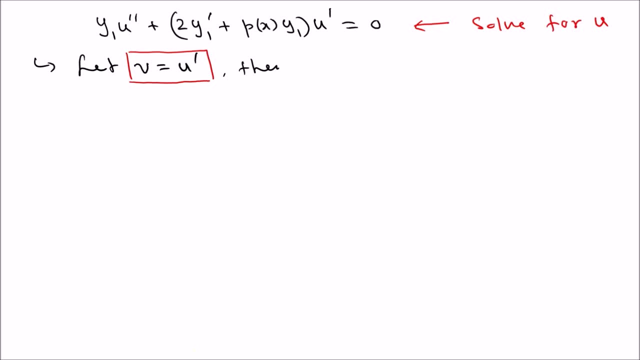 uh. then we have v prime equal u prime, u double prime. so what happened then? we can rewrite the above equation in this form, so we can write the uh the equation like this: we can say: um y1 v prime plus 2 y1 prime, px, y1 u prime means v equals zero. now you can see that this is a first order linear equation. 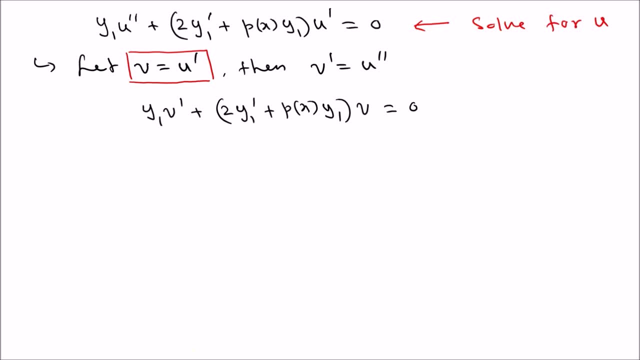 first order linear equation. so first we can do, we can divide by this term if you divide by that term, because that we know that that not equals zero. so v prime plus. if you divide by that, you get: uh, what do you get? you get 2 y1 prime over y1. 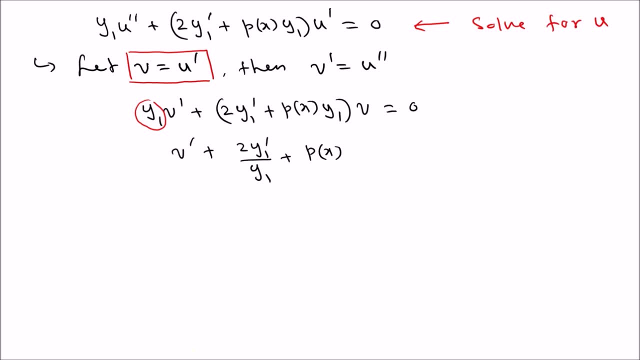 1 plus px. just px times v equals 0.. so this is first order linear in v. this is first order linear in v. now we can solve this. we can use the integrating factor method or some other techniques to solve this one, because this can even be, because you can. 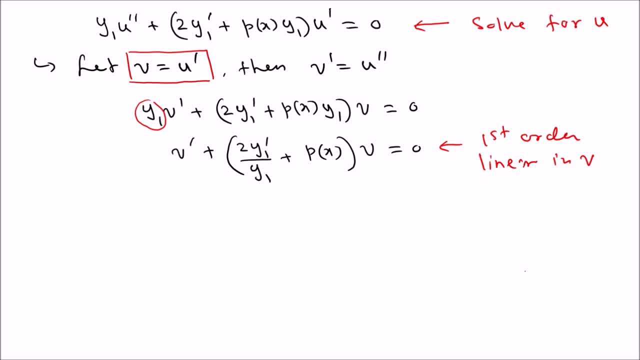 factor. this you can. this can be separable, so depending on what is y1 looks like. so that means uh. so the next step is uh. solve uh for v first and then and then solve for u, because after you solve for v, then we can use the fact that v equal u prime, you integrate one more. 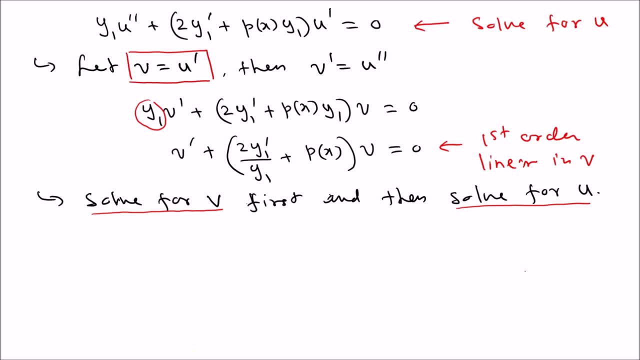 then you integrate, solve for u. so that's the idea. okay, so let's do the actual calculation. uh, in a problem, because what happened when you do a real problem? there are a lot of simplification going on, so it won't be this lengthy. we need to do the actual problem. so let's do a problem. so 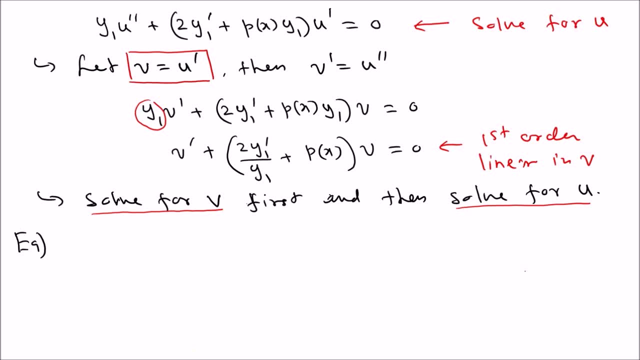 and also i'm going to give you the formula for that, so you can uh use that formula in the exam. but this is just a manual, so that's it. if you want to do something later, okay good, so let's do this one. uh, so it is given that. uh, it is given that. 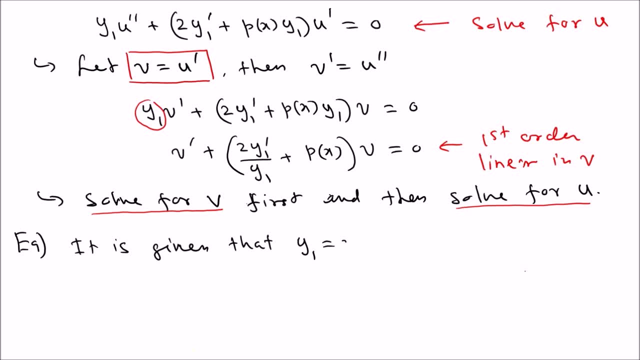 it is given that y 1 equal x squared, is a solution of: is a solution of: x squared, y double prime minus 3, x y prime plus 4. y equals 0.. so we don't know how to solve this equation, but somehow you can use a trial and error. 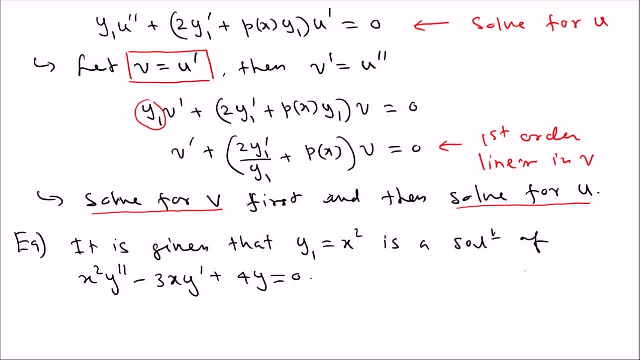 argument or something. we know that this is a solution. the goal is to what are the other solutions? find the other solution, okay, so find the second solution. but there should be two solutions, because it's the second order. find the second solution, so that's the goal, okay. 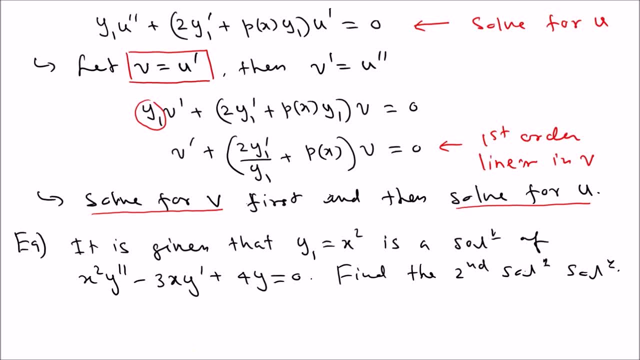 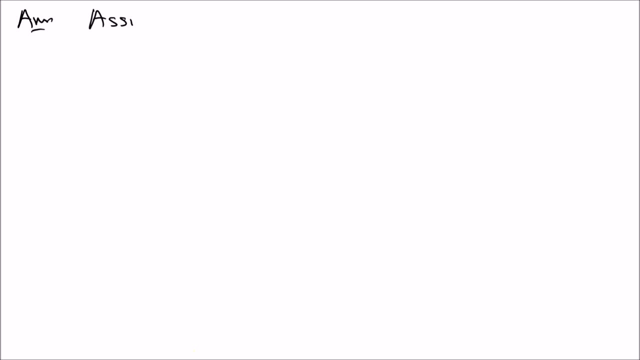 so we can use the reduction forward argument. okay, because we know that that solution. so let's see the argument and completely solve this problem. um good, so the answer: assume a solution of the form. assume a solution of the form. assume a solution of the form y 2. 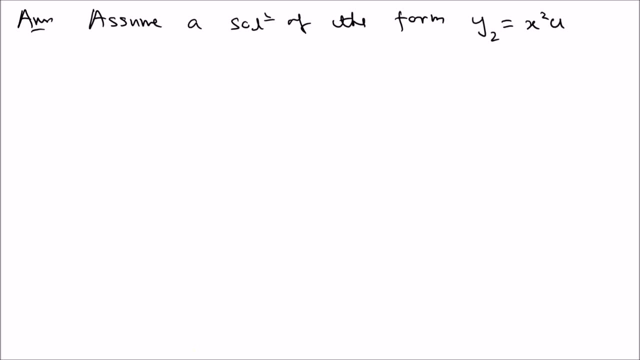 y 2 equals x squared u, because we know that, so we? so we don't write y 1 x square u. now what we do? we could take derivatives. okay, so take in derivatives. we have y prime equal, use the product rule. so it is 2. 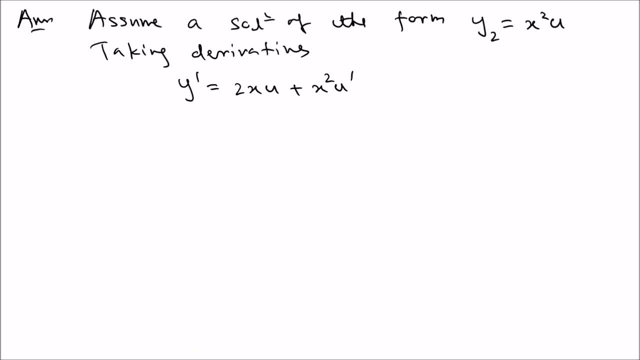 u prime. we have second derivative in the equation, so that means we need the secondary as well here. so if you do the second derivative you get 2 u plus 2 x u prime from the first term. from the second term you get 2x u prime plus x squared u double prime. 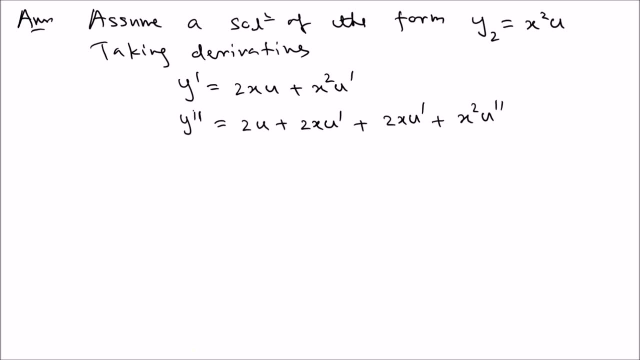 so you can combine this and you can write this one as 2: u plus 4 x: u prime plus x squared u, double prime. we combine these two, okay now, uh, since, um, so actually this is y 2. uh, since y2 is x, so we can substitute that to the equation. 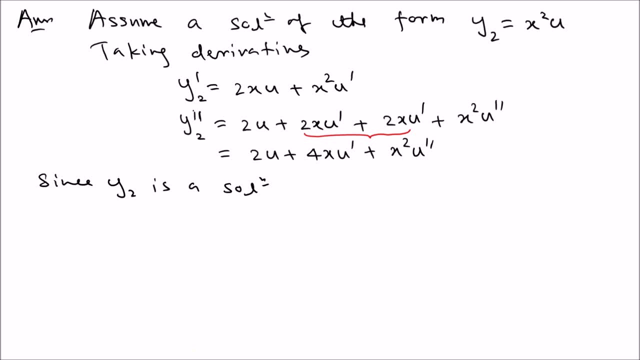 which is write a solution. we can substitute the equation. so we're going to get x squared y 2, double prime minus 3 x. y 2 prime plus 4 y 2 equal x squared times. substitute y 2 prime, it is 2? u plus 4 x? u prime plus x squared. 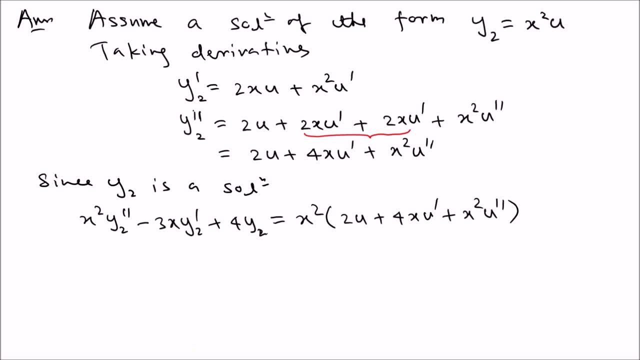 u double prime- this is simply coming from here- minus 3x y prime- y prime means 3 x u plus x squared u prime. plus 4 um y 2. y 2 means x squared u, which is equal to 0, because that's the 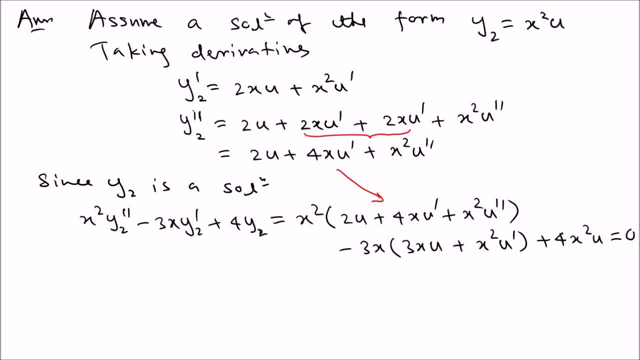 assumption. i'm going to assume there's a solution. now let's see how it's going to simplify. you can see there are a lot of simplification, uh, going on here. there's a type also. this is not three, this is two. uh, you can see that. 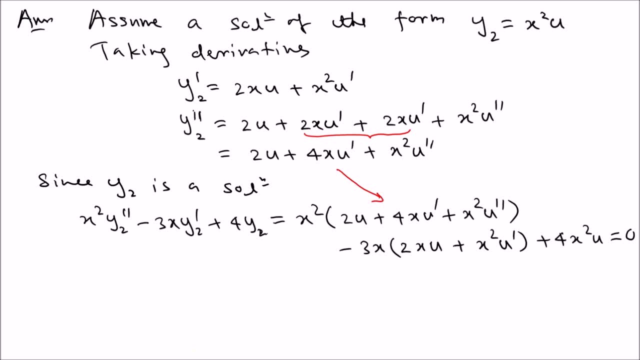 there are a lot of calculation cancellations going on. uh, let's look at the x squared u term. so there's x square u, this is x squared uh u term, and then we also x square u term here, and you can see that those three get cancelled. 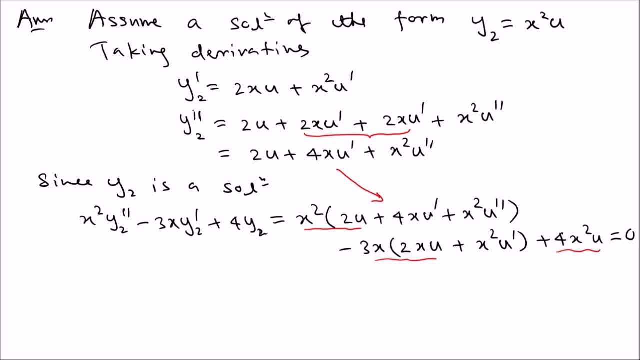 so those three get cancelled out. uh, because we have two, four and negative six. it's gone. so that means you only end up with uh, just a few other terms. so you have, uh, you have, so you're gonna get uh. so what are you gonna get? you're gonna get uh. there's x cube term here. 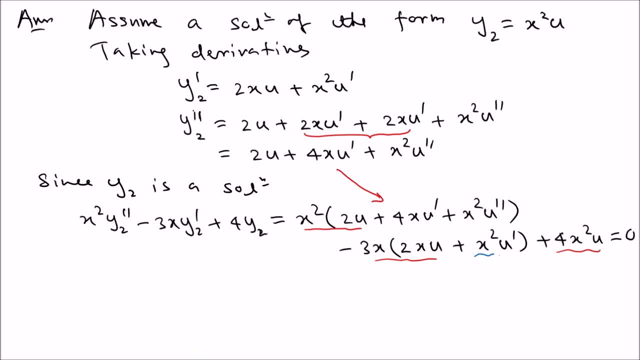 so this is x cube term because that's with x x cube term. there's another x cube term here, so you're going to combine those two x cube term and there's x fourth term. so this is x fourth term because that's x squared, so that means you have x cube term and x. 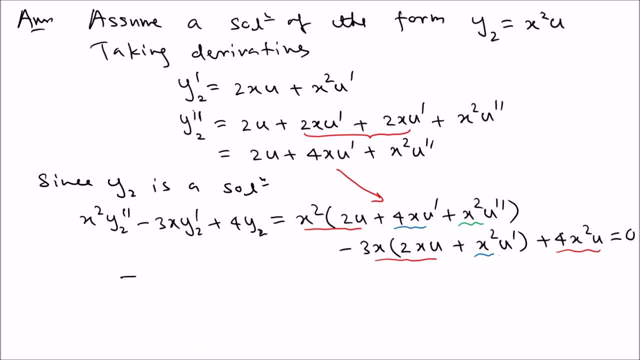 fourth. so this is gonna uh give you that, uh x fourth. u double prime plus x cube. u prime equals zero. so that's what you get. everything else get cancelled. now what we can do is: um, we can divide this by x fourth. so if you divide by x fourth, 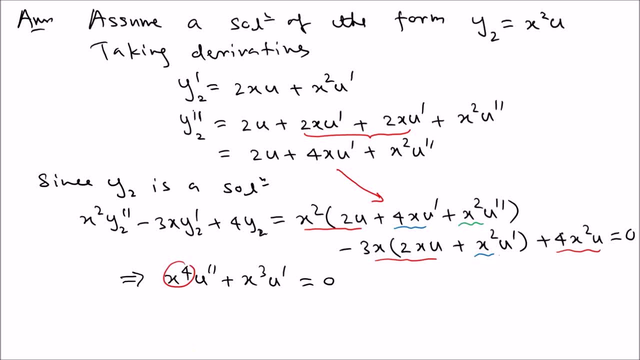 so we can divide by that term. uh. so that means this can be u, this can be u double prime plus one of x, u prime equals zero. now, what we're going to do? we're going to use this formula here, so we're going to use a substitution. so we're going to say: let 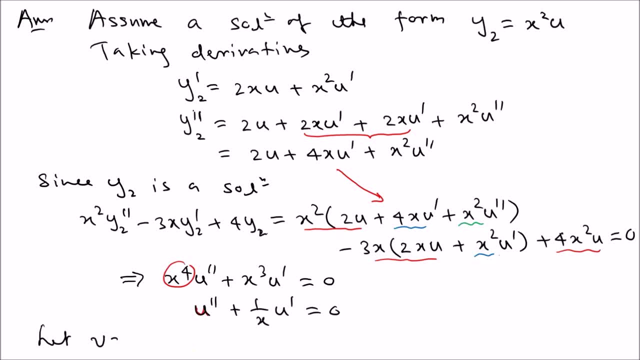 v equal u prime. so let v equal u prime. then we have v prime equal u double prime. so we can plug in. so our equation simply becomes: v prime plus 1 over x, v equals 0. so you can solve this problem using separable method. 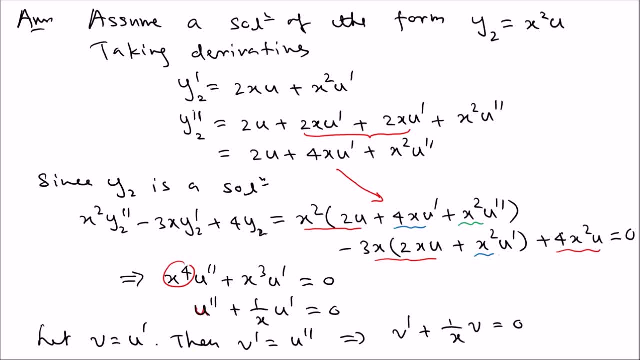 or the integrating factors method, so you can use any method. so it depends on the problem. uh, sometimes you can do that, sometimes you can't do uh, but most of the time, uh, yeah. so it's always like in this problem you can use both of the techniques. so we can use the. 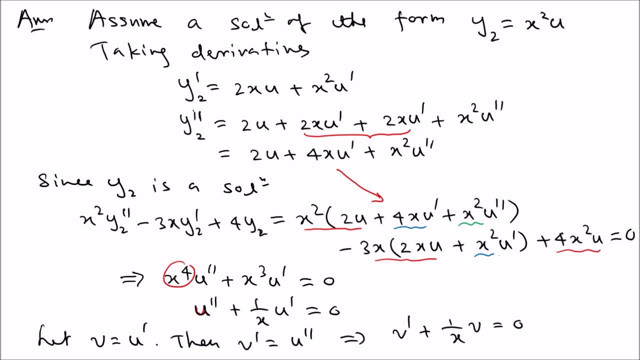 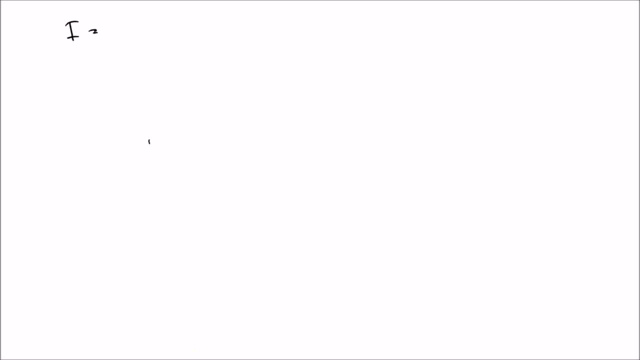 integrating factors. for this one it's kind of straightforward, so let's do that and finish the problem. so we have our integrating factor i, which is the integral of p x d x. so it's integral of p x. p x is 1 of x d x. 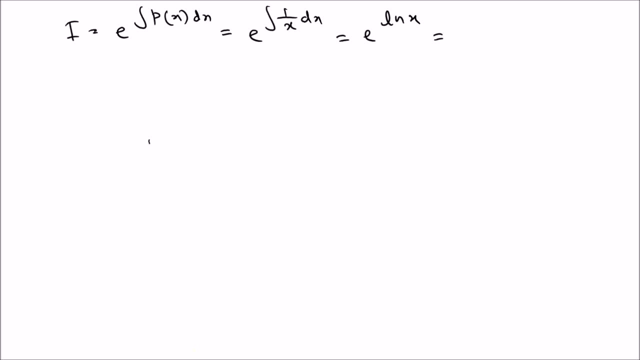 so we have e ln x, and then e ln x, cancel out, so you get x. so that's what you get now. um, from the theory, from the integral theory of integrating factors, we know that this side is simply the derivative, so you're going to get d over dx. 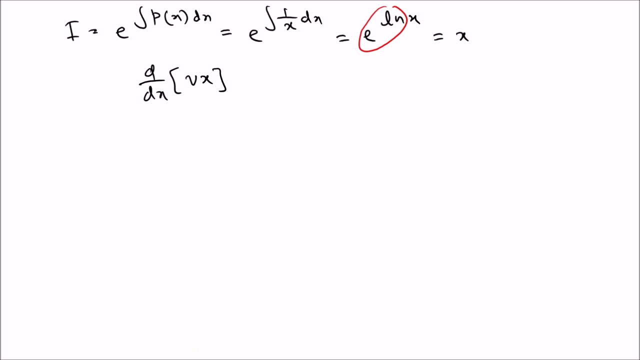 the v times integrating factor equal on the other side is zero. so you're, uh, so integrating, so integrating, integrating. we have vx equal a constant. i'm going to call c1. so this says that v equal c 1 over x, and now we can substitute for a v. 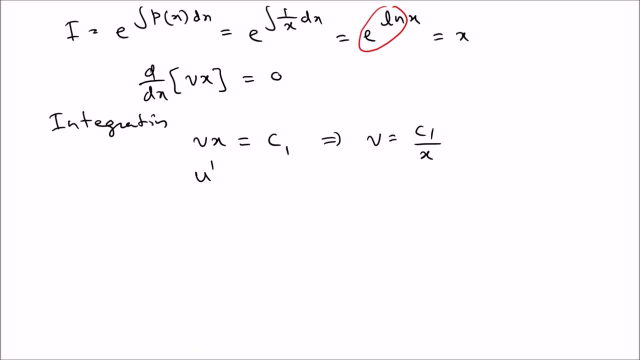 but v means uh, u prime. so this is that u prime equal c 1 of x. to get u we can integrate so u equal the integral of u prime, calc 1 as integral of c 1 out 1 of x dx, that means c 1. 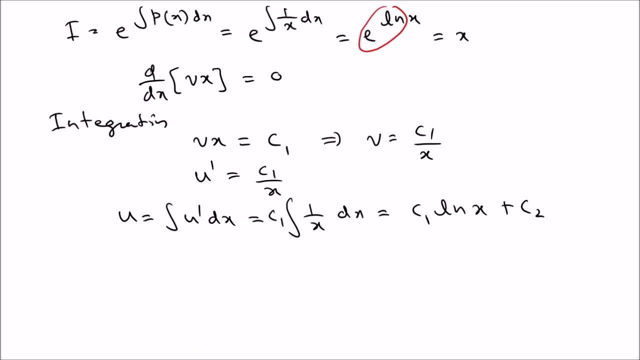 ln x plus c 2. but what you can do, you can ignore c 2, because we are looking for one solution. we can even say c 1 equal 1, so set c 1 equal 1 and c 2 equals 0, because we are looking just one solution. 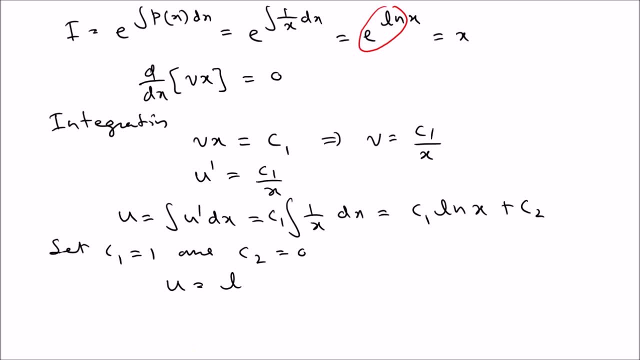 here. so that means you're going to get u equal ln x. uh, so x. actually. here you can say absolute value, because we did not restrict only to positive x, so x can be positive and negative, so you can have ln x. absolutely good, so okay. so that means. 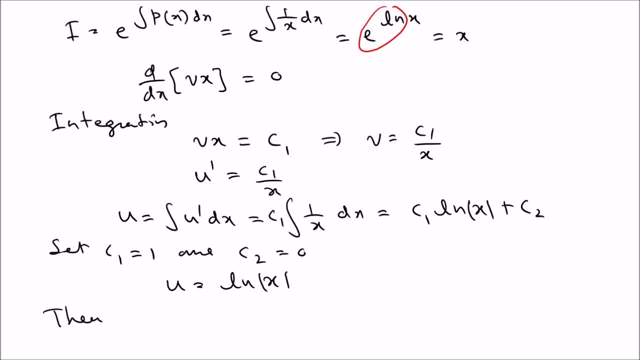 this is a second solution. so then the second solution, y 2, is a equal x squared u, uh, which is x squared ln, x. so that's how you find the second solution, using the reduction of order method. so it's not that difficult, but what we did was we start. we assume a solution of the form y 1. 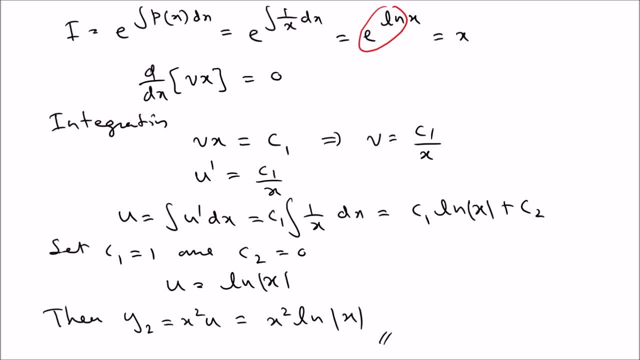 u substitute that, there's a nice simplification. you can see that there's some one. there are a lot of simplifications, a lot of terms get cancelled out, and then you get a simple equation that you can solve using the or integrating factors method. so now i'm going to give you the reduction. 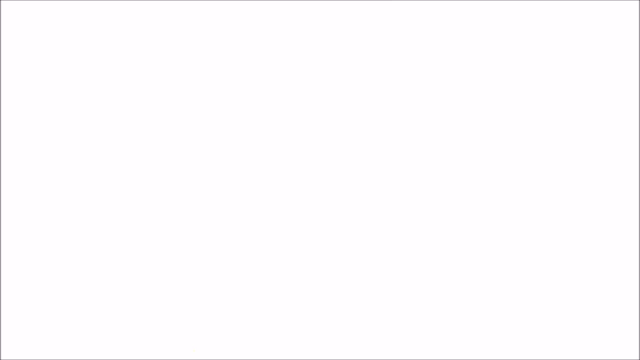 of order formula. so you directly use this formula if you get a problem like that. so the theorem, the reduction of order method, reduction of order formula. so let's say, if y 1 x, y 1 x, not t equal to 0, is a solution, it's a solution of y double prime. 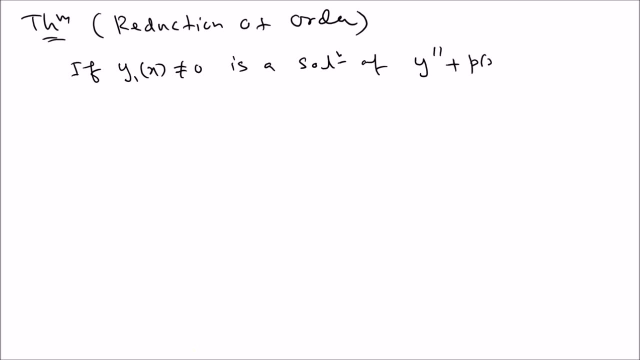 p x y prime plus q x- y equals zero. remember, it has to be of this form. this is not of this form. you have to bring it to this form. okay, we need that. we need to isolate the px term. so sometimes you have something in front, so i have to divide by that first. so you have to isolate the px term. 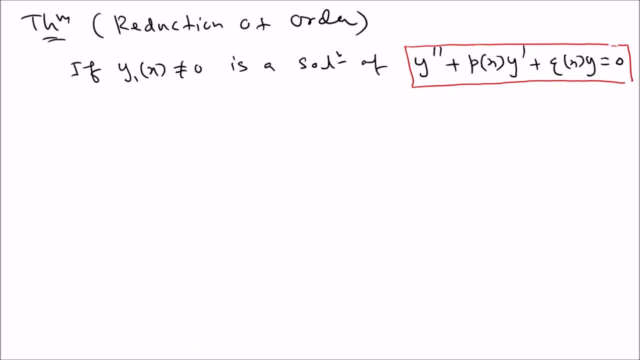 okay, okay. so it's very important, it's a solution of this. then another solution in another, linearly independent. so this automatically linearly independent, another linearly independent. another linearly independent solution is given by: is given by: y 2 x equal, y 1 x, integral of a to the negative, p x, dx. 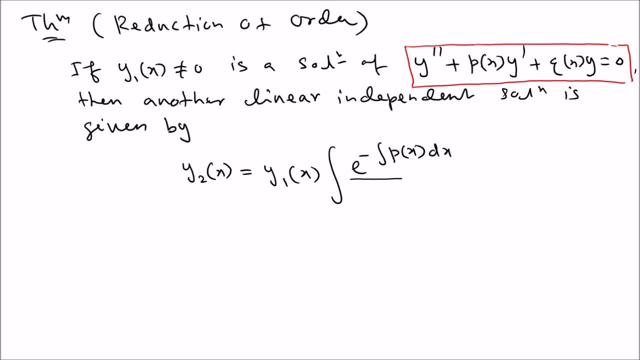 that's why you need to know the px. and divided by y 1 x, whole thing squared: sickness square y 1, tighten minor integral y 1 tx. so that is the formula. that's a reduction of the formula and you can directly use that. do not select normat. 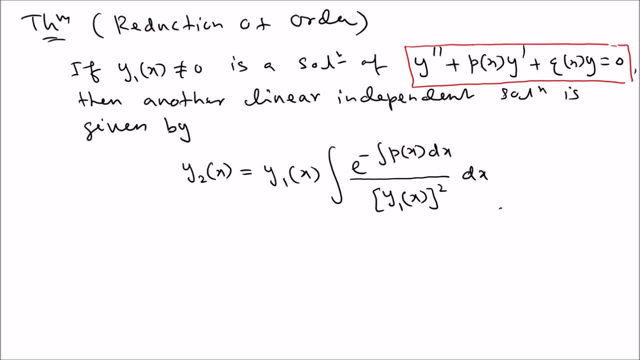 use that. so let's use that in a problem and see how the whole calculation works. so this is a problem of that type. so if it is given that, if it is given that y 1 equal x is a solution, is a solution of x squared y double prime minus x by prime plus. 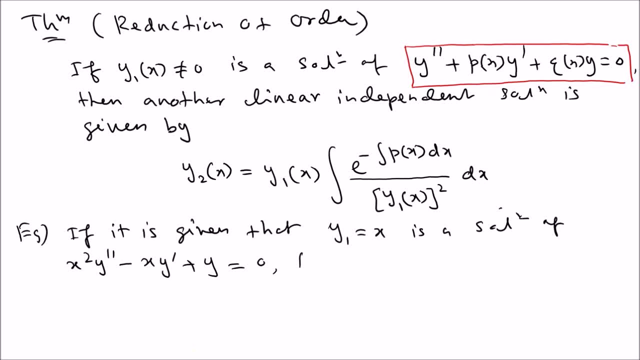 y equals zero. find the general solution. find the general solution. so, uh, so that's the final general solution. that means this is the second order difference, because i mean there's another solution, so we're going to find it other solution using the indicating factor method. so the problem is, when you look at this one, this is not of. 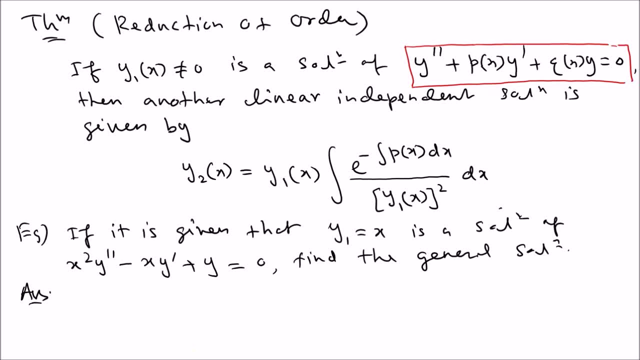 the standard form. there's x squared term, so we'll divide by that. so we have uh, x squared y, double prime minus x, y prime plus y equals zero. so what we can do, we can divide by x squared to bring it to standard form. okay, so the standard form. 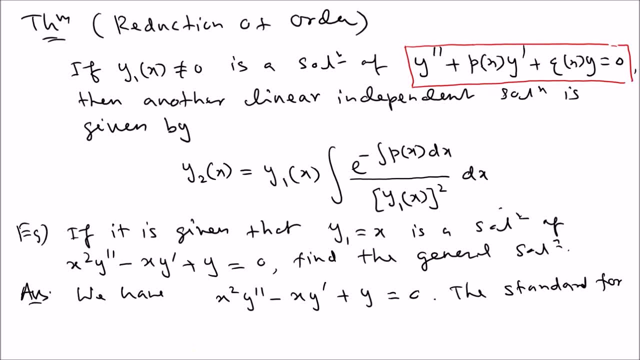 standard form is: if you divide by that, you're going to get y double prime minus a 1 over x. y prime plus 1 over x. squared y are equal zero. so you can see where our px is negative: 1 over x, that's the px2. so you can see where our px is negative. 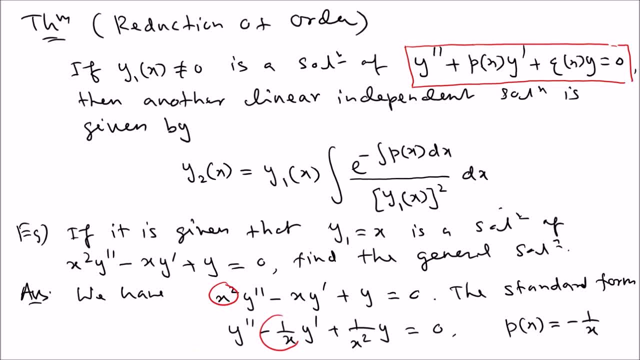 1 over x, that's the px2. so you can see where our px2 is negative: 1 over x, that's the px2. okay, so you have to isolate the px term. uh, good, so, uh, then we can use the formula to find the second solution. 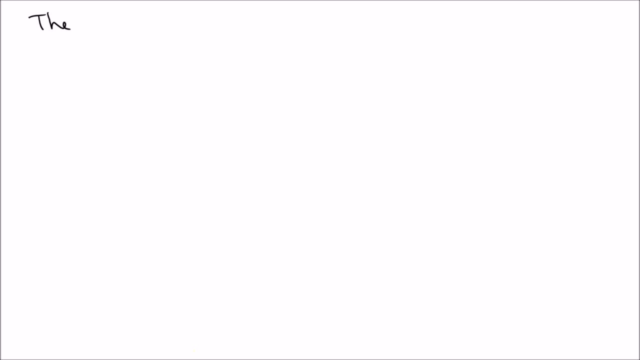 the second solution is: the second solution is given by by the formula: it is y2 times e to the minus px dx over y 1 squared dx. so let's plug in here. we have everything we know. so y 1 is x. the integral of e to the minus px is: 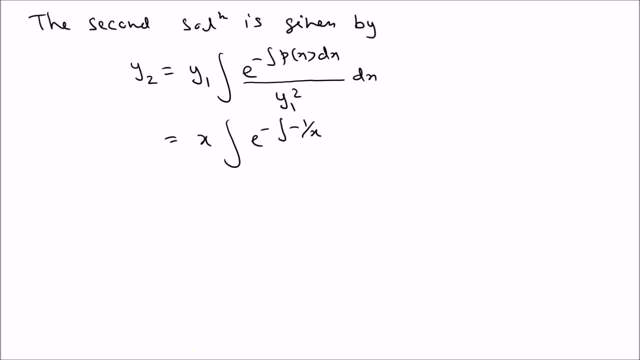 negative: 1 of x dx over x squared dx. this you can simplify a little bit so you get e to the 1 of x dx over x squared and you can see that you cannot bring the x squared out because as you're still integrating inside um. so from that you can see this is x the top. 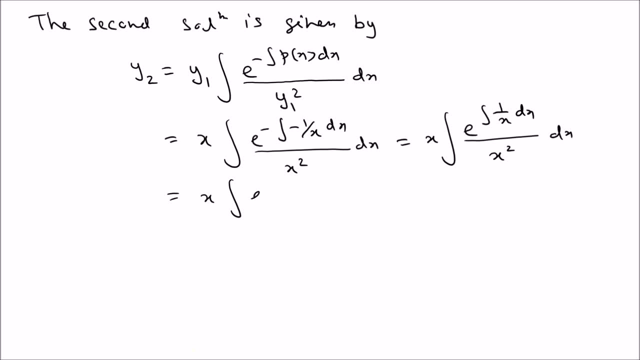 is simply e to the ln x of x squared dx. and then we know that when you have eln x, uh, eln, x, eln, uh, cancel out. so you need x. so this is x times x over x squared dx. this is simply 1: 0 x dx. 1 x means ln x, so we're going to say x. 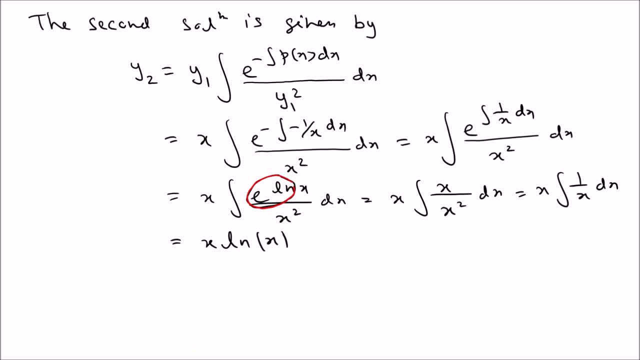 lmx, and we are going to add the c here. ah, the reason is we are looking for one solution. okay, so that's that. uh, now the next step is we need to show that, uh, these two are linearly independent. uh, okay, to show that they are linearly independent, uh, 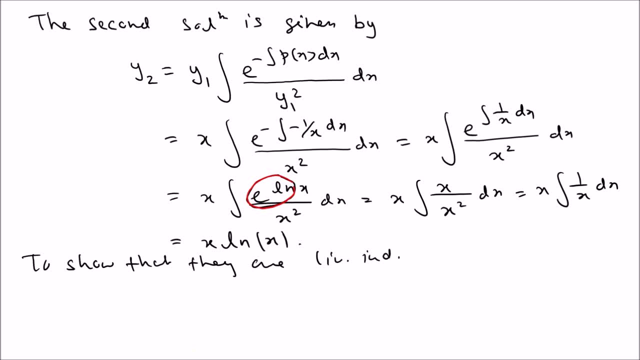 actually, if you remember the theory, it says that these are, say another, linear independent. so at either you say that the independent solution by the theorem or you can just prove this. this is not that difficult. yeah, so the solution is automatically independent, the solution that we get. we can prove that taking a using this formula: 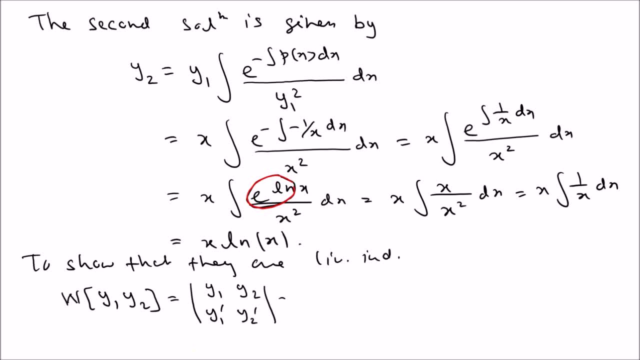 but it's also not that difficult to show that. so let's plug in here and see what happened. this is x, d, dx is 1.. we have x, ln, x, uh derivative, that is, use the product rule so you get ln x plus x times 1 of x, even in this case. 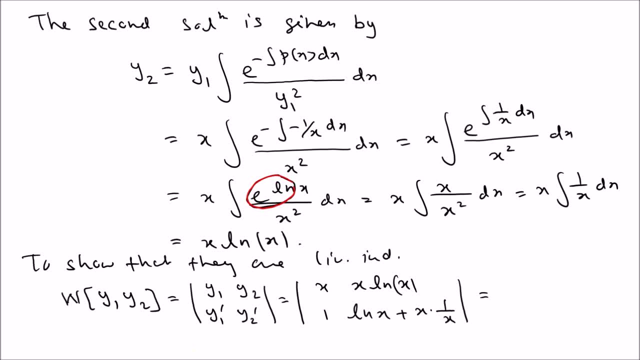 ah. so let's simplify. when you simplify what happened, you're going to multiply, uh. so what do you get here? you get x 1 x ln x, uh, ln x plus 1, that's what you get. so you get x 1 x ln x plus 1, that's what you get. 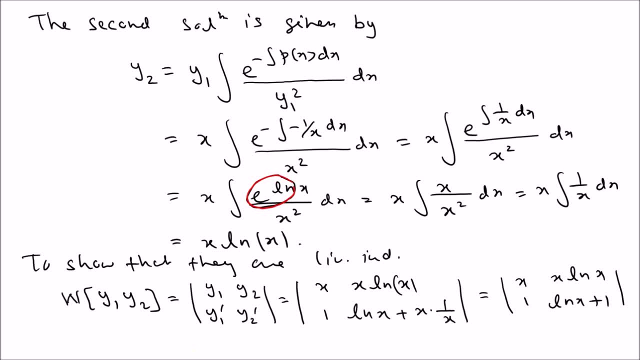 so we can multiply through. when you multiply through what you get, you get x ln x plus x minus x ln x. that's what you get. you can see these two get cancelled so you get x, which is not equal to 0 in general, where x can be anything other than 0. so that means yes. 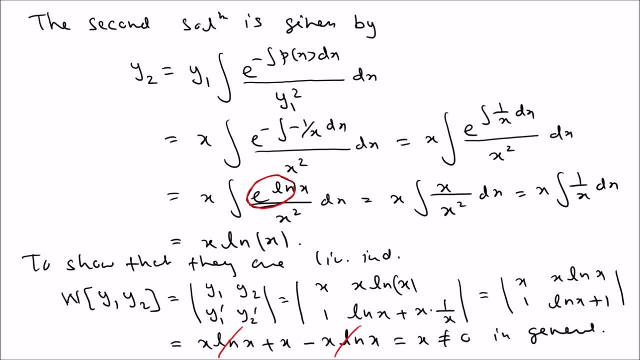 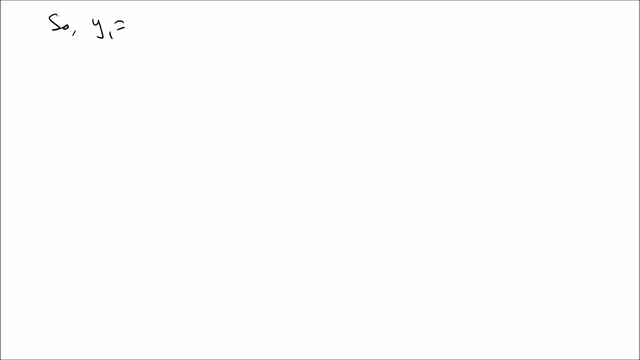 not equal to 0, so they are linearly independent. so, ah, y 1 equal x and y 2 equal x, ln, x are linearly independent. good, uh, therefore the general solution is because in the theory, we know that those two should has to be linearly. 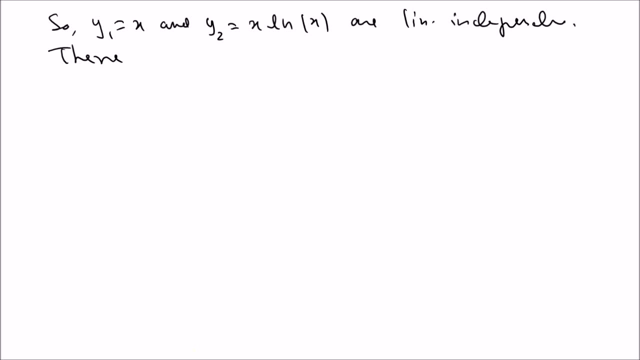 independent to find the general solution. otherwise we can't find the general solution. it's not going to be so. therefore, the general solution is: is given by a y equal c 1 y 1 plus c 2. y 2 equals c 1 x plus c 2 x ln x. 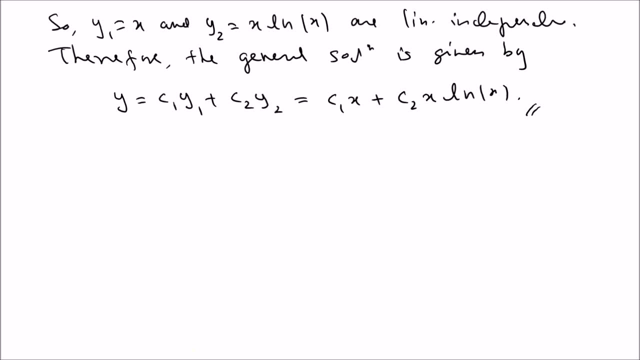 who's general solution. so that's the general solution. so that's how the reduction of order method uh works. so it's uh very interesting and not that bad, okay. so if you have a problem like that, you can directly use the reduction over the formula. okay, let's move on to the most important uh. 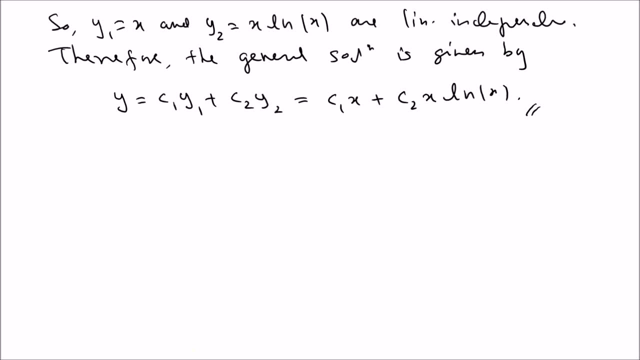 topic. so what's the most important topic? the constant coefficient, differential equations. so number 18 is the most important one: the constant coefficient. constant coefficient, second order, uh, constant coefficient, second order, difference equation- good, uh, so this kind of equation has this form. so it has the form. 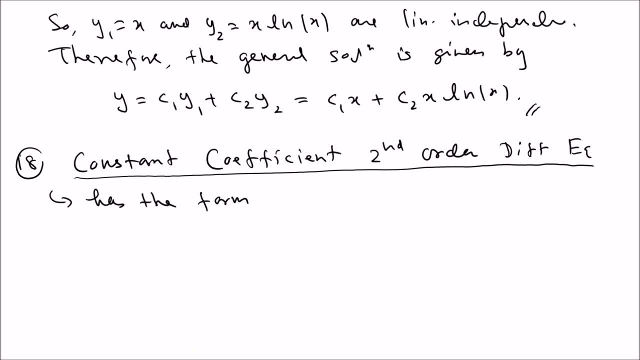 has the form: a constant times, y double prime. another constant time, y prime. another constant time. y equals c, homogenous equation. and then we know that a, b and c are constants. that's the case we trying to um understand. so that is the case, very special case. good, now what we're going to do, how to. 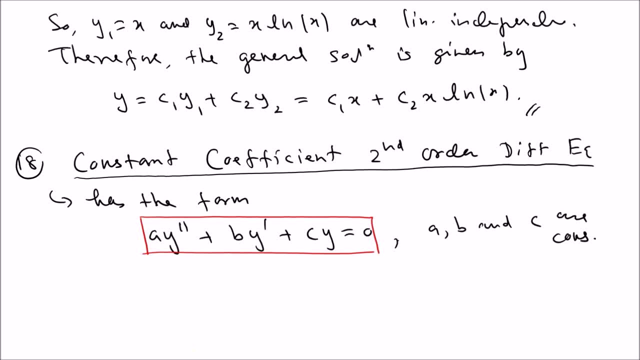 solve this one. uh, what we did? we assume a solution of the form y equal e to the lambda. so that's the. that's how the solution work. so assume a solution of the form of the form y, equal e to the lambda. and then what we can do? we can take the. 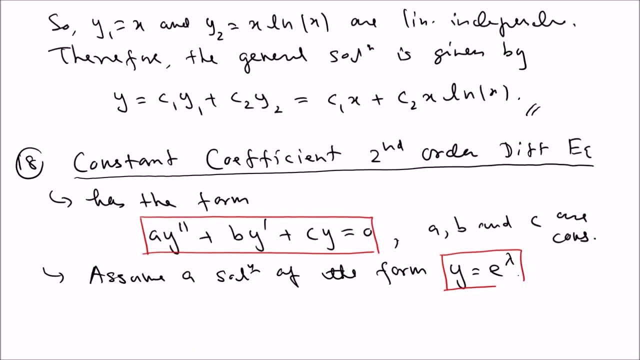 derivatives of that and plug it. we assume a solution of the form and then we can take the derivatives. okay, so take derivatives. so we're going to get y prime, which is lambda, is a constant- this is a lambda e lambda- and then we can take another derivative, double prime. 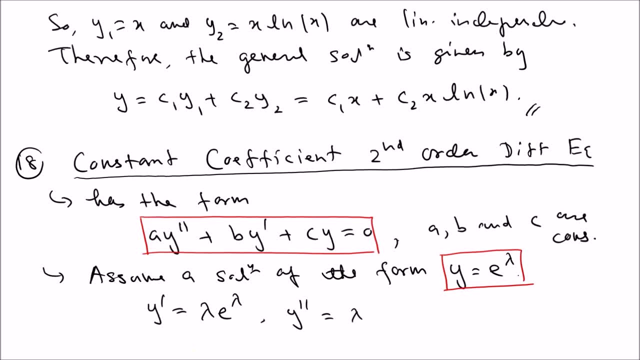 so we're going to take lambda squared e to the lambda, okay, so we know how to take this like that. oh, actually, uh, it's not e to the uh, uh, it's lambda t it's not just lambda. so, uh, we e to the lambda is a constant this. 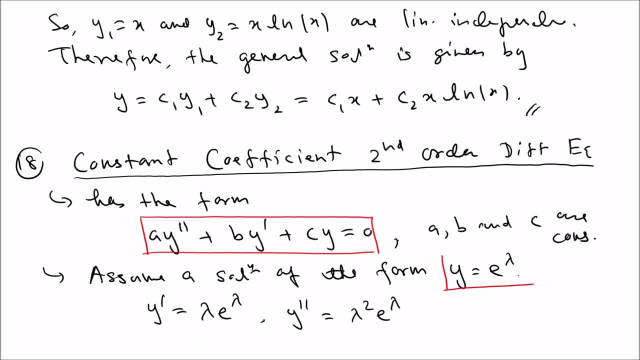 is not a function, it's just fun is a constant for e to the e lambda t, uh, and then also here uh. so t and t, okay, good, um, yeah, so we assume a solution of the form and take the derivatives. so y equal e to the lambda t. 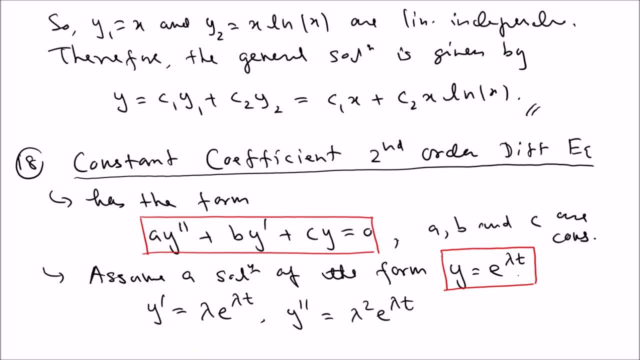 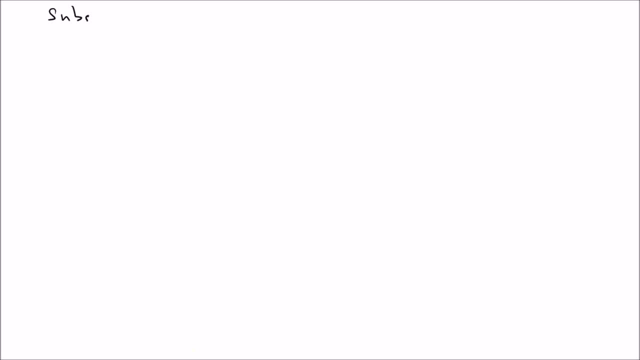 now we're going to substitute this in the equation, so let's do that substitute. so if you substitute, you're going to get a lambda squared e to the lambda t. that's the first one plus the second term b: a lambda e to the lambda t. that's for y prime, because this is y. 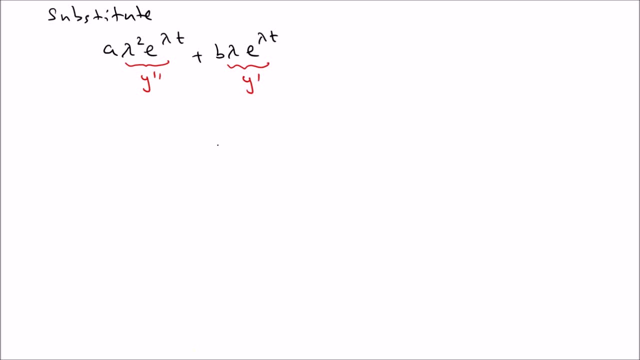 double prime: this is y. prime plus c: e lambda t equals 0, this is y. so we're going to substitute for 3.. now you can see that e lambda t is common, so you can take it out as a factor. so if you take as a factor, 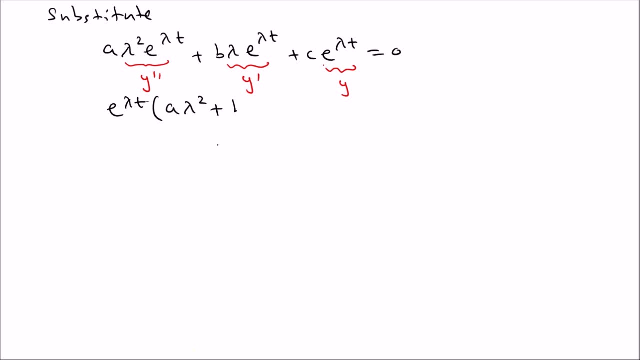 you're going to get a lambda squared plus b lambda plus c equals zero for any t, but we know that e to the lambda t never becomes 0. since e lambda t not equal to 0, the only option that this can be 0 is a lambda. 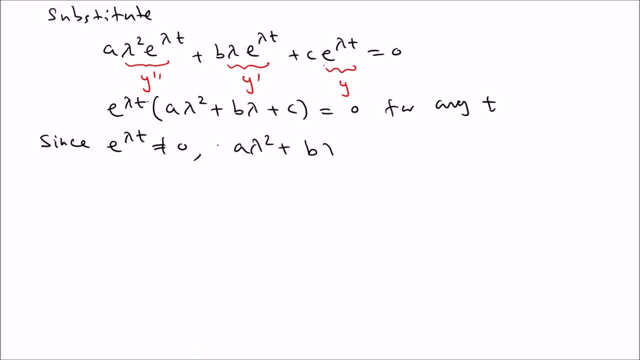 squared plus b, lambda plus c equals 0.. this is what we call the characteristic equation of the differential equation, because this has to be satisfied if e lambda t is a solution. okay. so this is what we call the the characteristic equation. characteristic characteristic equation. good, and you can directly write this: 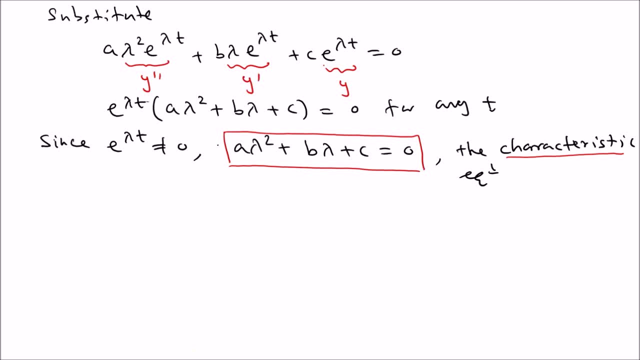 equation. so what happened? when there's a derivative, it's a second derivative. you get lambda square, it's the first derivative. you get lambda 1. there's no derivative, you get lambda 0. that means constant. so you can directly write. you don't want to show this work here. you can directly. 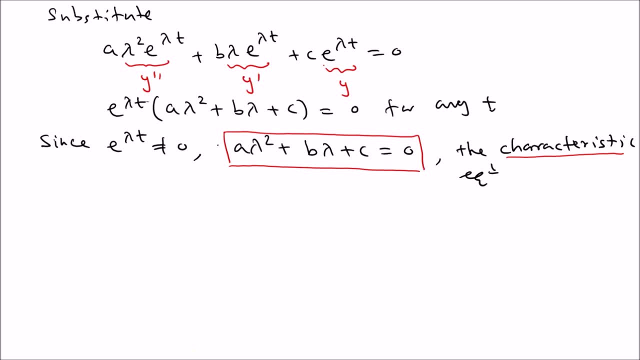 write the characteristic equation. if you have problem like that, okay, then let's try this important theorem: uh, so what? it says that okay so, uh, so the theorem. so consider the differential equation: uh, a, y, double prime plus b, y prime plus c y equals 0. we are 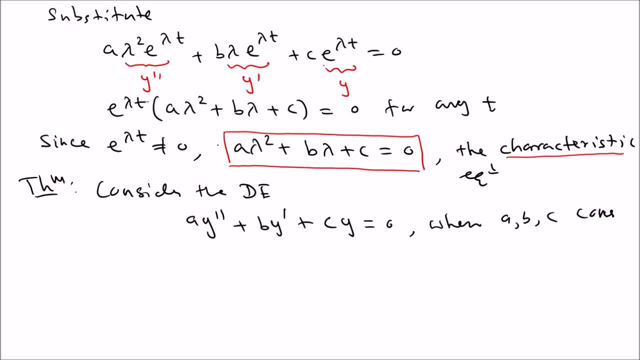 a, b, c, constant, with okay, so yeah, and then. uh, then the characteristic equation. then, don't worry, the characteristic equation we called για equation, characteristic equation is simply a lambda squared plus b. lambda plus c equals 0. so you seem to replace the derivative terms by lambda powers. so see what happens. 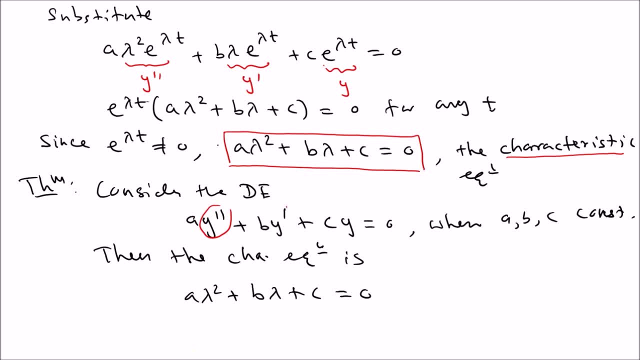 is there a connection? y double prime, lambda square. y 1 prime, lambda, 1 power. there are no derivatives or no lambda powers. it's lambda zero powers. okay, now we can write the general solution three forms, so let's write them separately, so the general solution has the form. 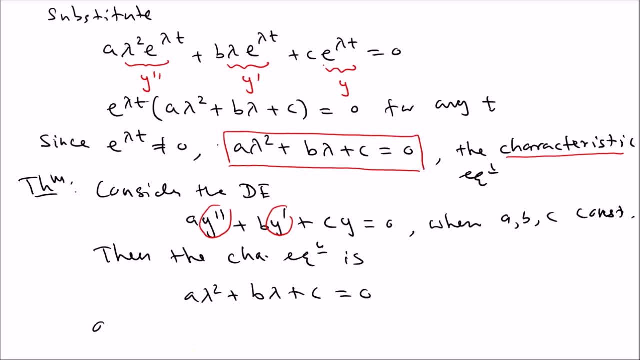 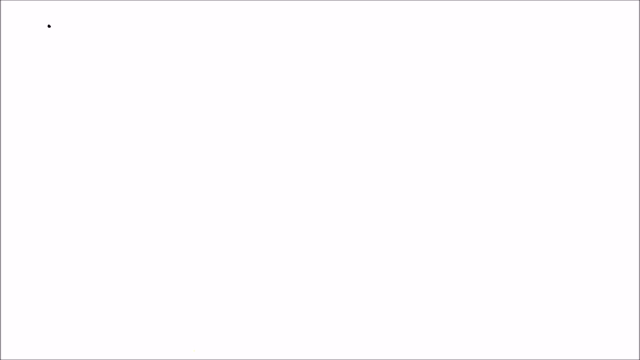 and let's say: and the general solution, and the general solution has the form, let's write one by one: ah, so there are three cases to consider, because this is a quadratic equation. ah, so it can be. uh, so there can be two real roots, distinct real roots, equal real roots or complex roots. 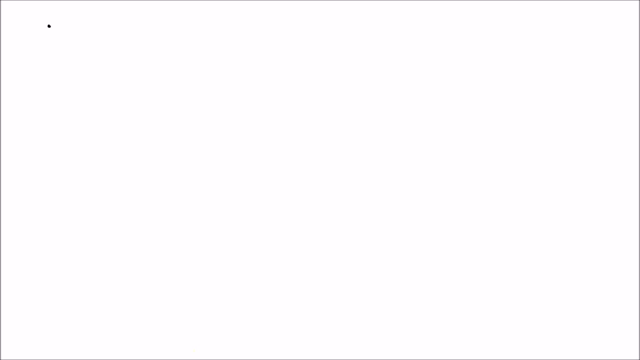 so we have three cases. uh, so if b squared minus 4, a c positive, ah, then what happened? the lambda 1 and lambda 2, ah, real distinct are roots. so the general solution has this form: y equal c 1 e lambda 1 x plus c 2 e lambda 2 x. 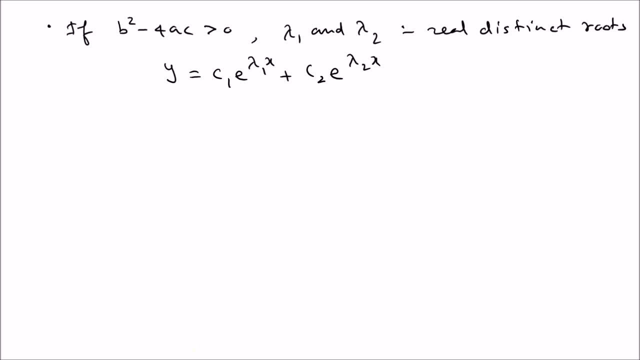 in that case, the second case. the second case: if b squared minus 4, a c equals 0, then what happened? b squared minus 4, a c equals 0, then what happened? lambda 1 equals lambda 2, ah, then what happened? this is a real 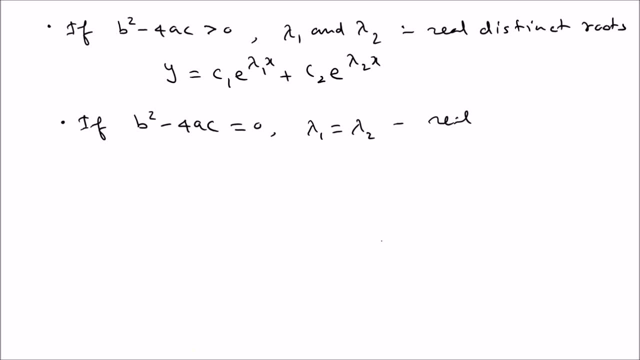 repeated situation: real and repeated, real, repeated. so the solution has the form c 1 plus c, 2 x times one of those terms: ah, lambda 1 x. or you can write it like this: lambda 1 x. or you can write it like this: lambda 1 x. or you can write it like this: 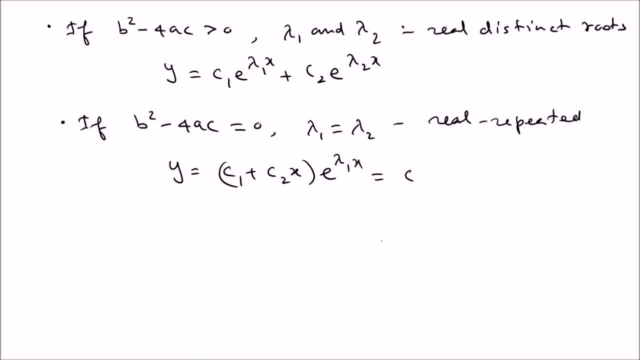 you can expand it and write it like that. you can expand it and write it like that: c 1 e lambda 1 x. c 1 e lambda 1 x. c 1 e lambda 1 x plus c 2 x e plus c 2 x e. 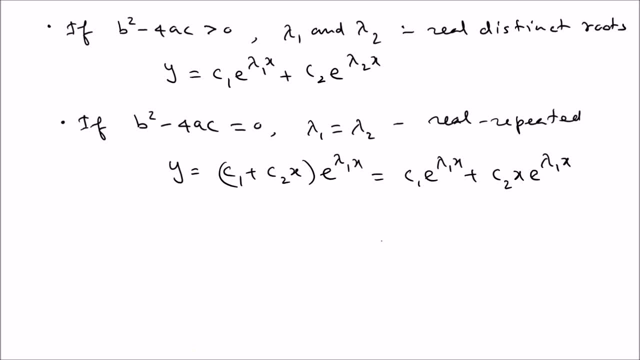 plus c, 2 x, e, lambda 1 x. you can write it like that: lambda 1 x. you can write it like that: lambda 1 x. you can write it like that: it doesn't matter which form okay. and it doesn't matter which form okay. and 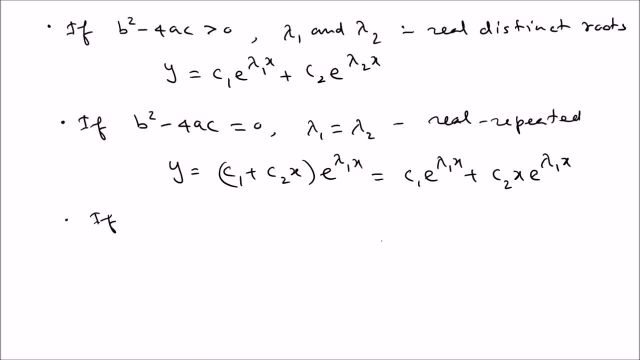 it doesn't matter which form, okay. and third case. third case, third case: if the b squared minus 4 is, if the b squared minus 4 is, if the b squared minus 4 is c, negative, c, negative, c, negative. now what happened? your lambda can be. 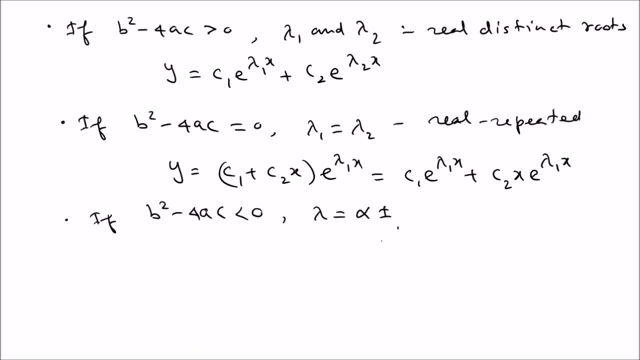 now what happened. your lambda can be now what happened. your lambda can be written as written. as written as alpha plus or minus a beta. i complex alpha plus or minus a beta. i complex. alpha plus or minus a beta. i complex conjugate. this is what we call the. 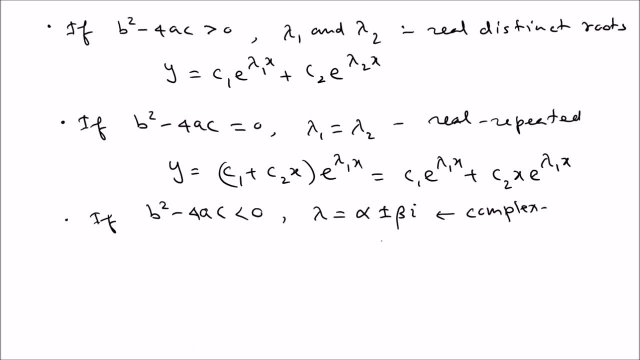 conjugate. this is what we call the conjugate, this is what we call the complex conjugate situation. complex conjugate. so in that case, what complex conjugate? so, in that case, what complex conjugate. so in that case, what will happen? will happen, will happen. your y has the form c 1. 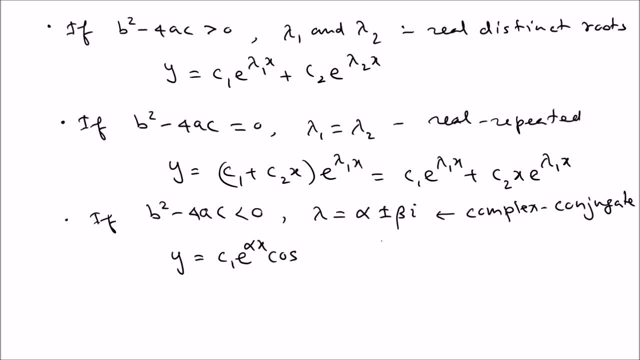 your y has the form c 1. your y has the form c 1 e. alpha x e alpha x e. alpha x. cosine, beta x. cosine. beta x. cosine. beta x plus c 2 e alpha x plus c 2 e alpha x plus c 2 e alpha x sine. 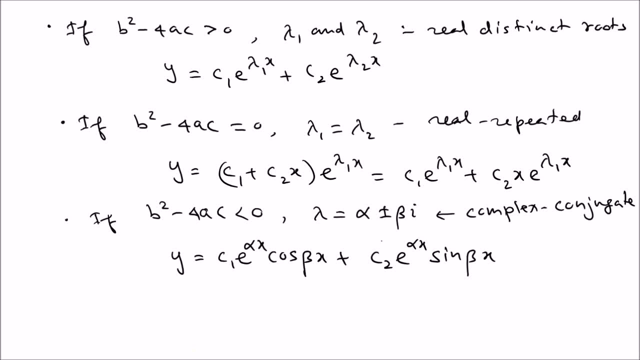 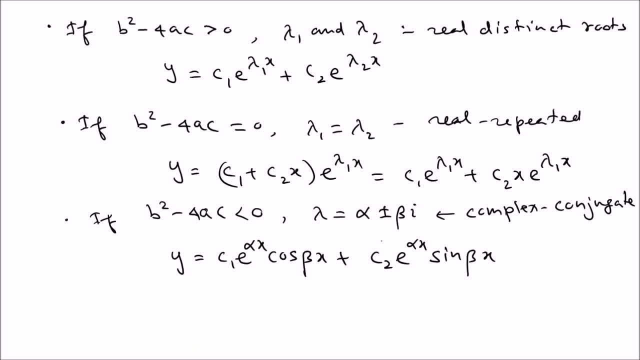 we have a cosine and a sine term. so we have a cosine and a sine term. so those are the, those are the. those are the uh three cases um that we even remember uh three cases um that. we even remember uh three cases um that we even remember. so again, what happened in the first case. 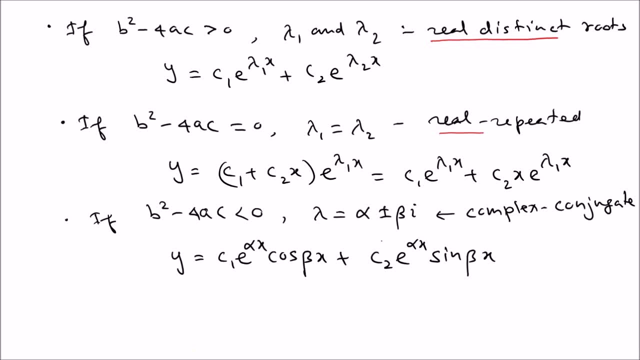 so again what happened in the first case. so again what happened in the first case. you get real distinct, you get real distinct, you get real distinct. real repeated and then complex conjugate. real repeated and then complex conjugate. real repeated and then complex conjugate, and you can directly use the result. 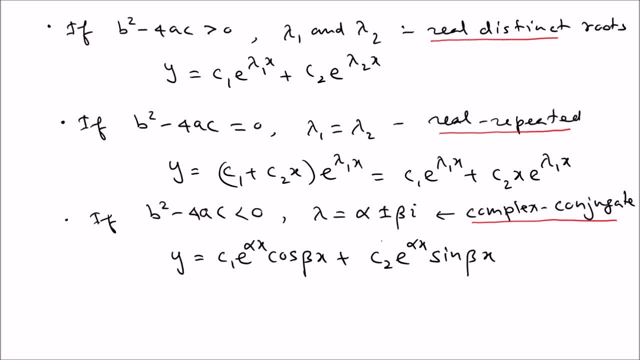 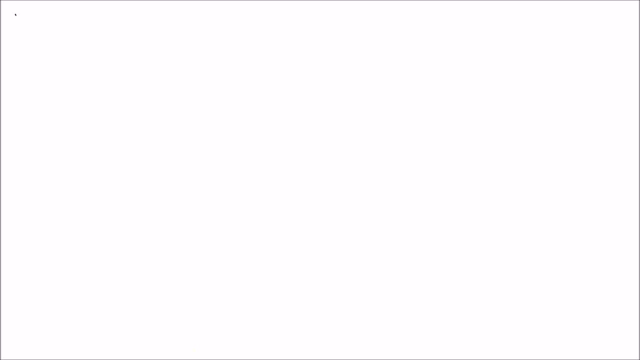 and you can directly use the result: um, so let's uh see this in a problem. or um, so let's uh see this in a problem. or um, so let's uh see this in a problem. or two. so let's look at this problem, find the. so let's look at this problem, find the. 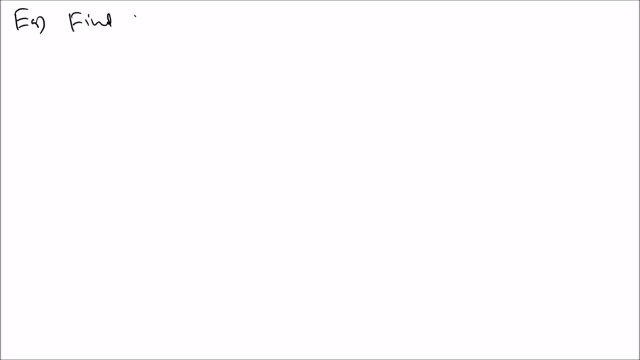 so let's look at this problem, find the general solution of general solution of general solution of. find the general solution of: uh, let's say a 2, uh, let's say a 2, uh, let's say a 2: y double prime minus y prime. y double prime minus y prime. 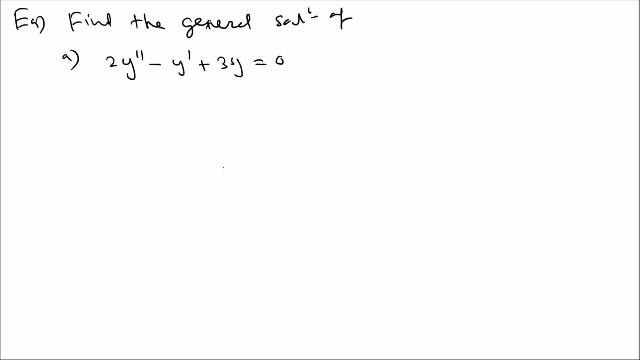 y double prime minus y prime plus a plus a plus a 3 y equals zero. so if you can provide that the first, so if you can provide that the first, so if you can provide that the first thing is we look at the characteristic thing is we look at the characteristic. 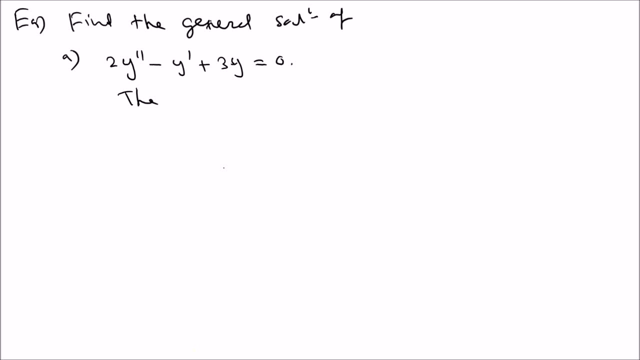 thing is, we look at the characteristic equation, equation, equation. so the characteristic equation equation is: uh, simply, uh. equation is uh, simply, uh. equation is uh, simply uh. two lambda squared minus lambda, two lambda squared minus lambda, two lambda squared minus lambda plus three equals zero. this is very easy. 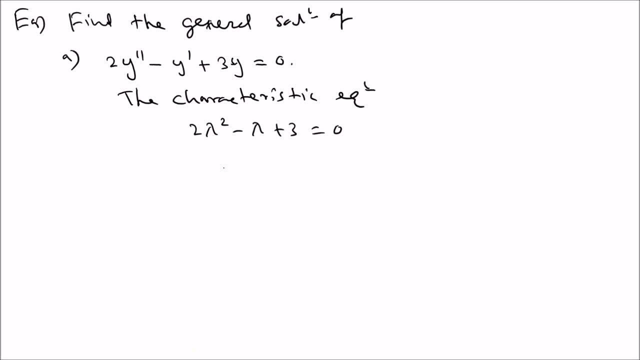 plus three equals zero. this is very easy. plus three equals zero. this is very easy. to find factor, to find factor, to find factor. so what are the factors? uh two times six. so what are the factors? uh two times six. so what are the factors? uh two times six. so you have six. 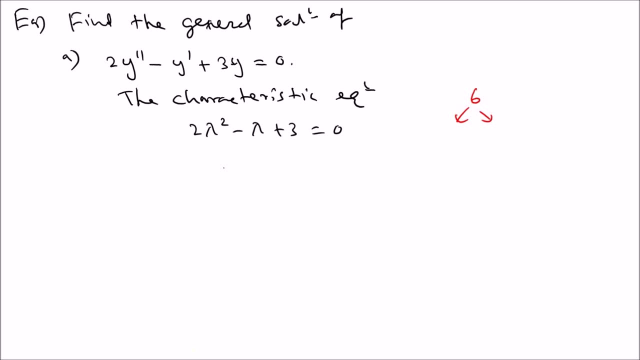 so you have six. so you have six. you're gonna bring uh write this as a uh. you're gonna bring uh write this as a uh. you're gonna bring uh write this as a uh product with the uh product, with the uh product with the uh. when you add the two, you get negative one. 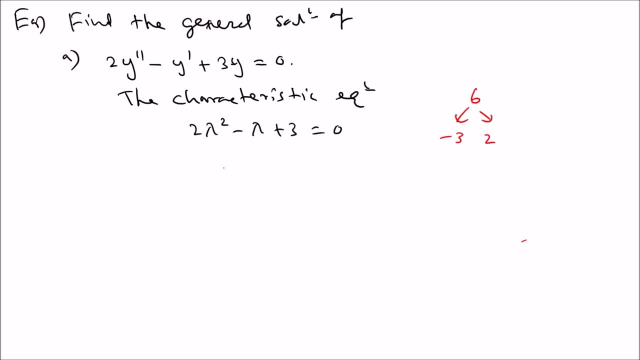 when you add the two, you get negative one. when you add the two, you get negative one. so that means it has to be negative three. so that means it has to be negative three. so that means it has to be negative three and two. so that means your factors are. 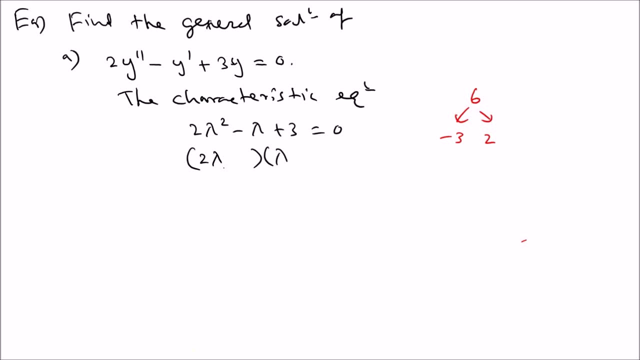 and two, so that means your factors are and two, so that means your factors are: two lambda and lambda, two lambda and lambda. two lambda and lambda. um now to find um. now to find um. now to find the number. so you know that two so the number. so you know that two so 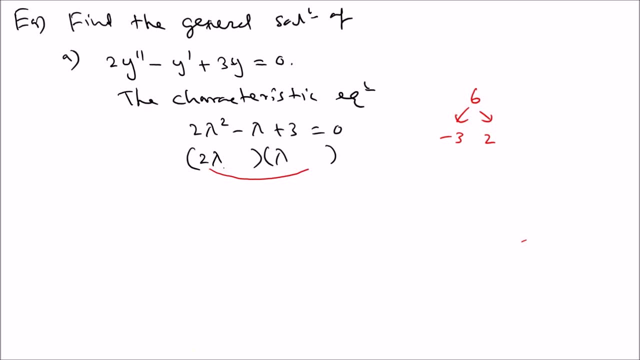 the number. so you know that two. so, uh, how to get this number? you simply, uh, how to get this number? you simply, uh, how to get this number. you simply divide, divide, divide that two by this two. so that means that two by this two. so that means 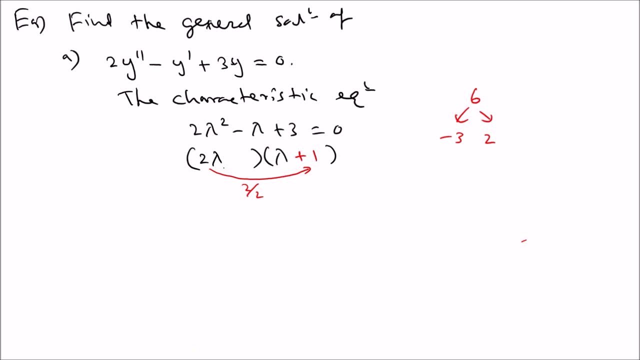 that two by this two, so that means it is plus one. and for the other number it is plus one. and for the other number it is plus one. and for the other number you divide negative three with one. so you divide negative three with one. so you divide negative three with one. so that means uh. 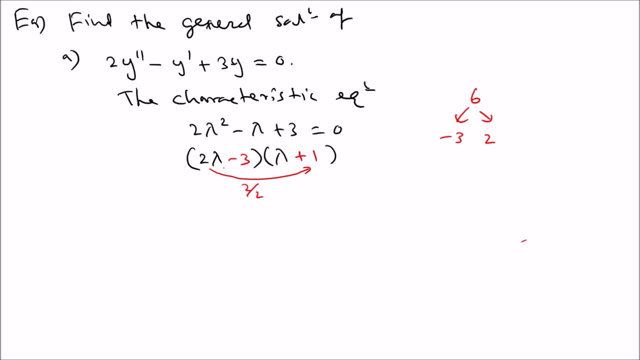 that means uh, that means uh, negative three. so those are the negative three, so those are the negative three. so those are the two numbers you get, and if you don't two numbers you get. and if you don't two numbers you get, and if you don't know how to do that, then you can look. 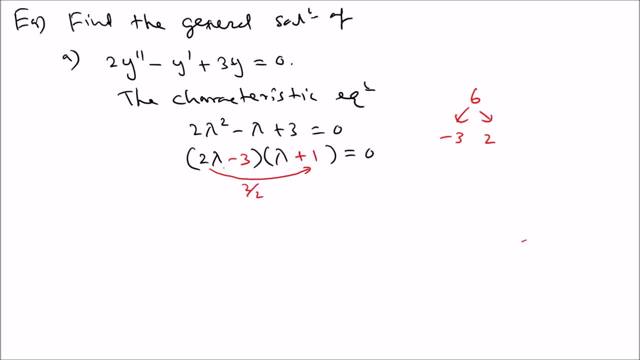 know how to do that, then you can look. know how to do that, then you can look at the, at the, at the effect factor in a polynomial video and effect factor in a polynomial video and effect factor in a polynomial video, and i explain, i explain, i explain all different type of polynomials in. 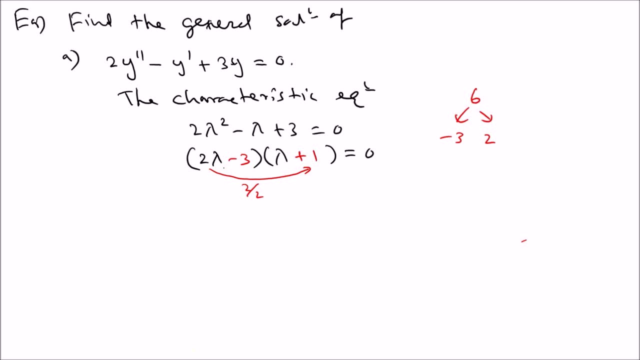 all different type of polynomials, in all different type of polynomials, in there, quadratic cubic, there, quadratic cubic, there, quadratic cubic, quintic quartic, all of them. so that's a quintic quartic, all of them. so that's a quintic quartic, all of them. so that's a video that you can watch. 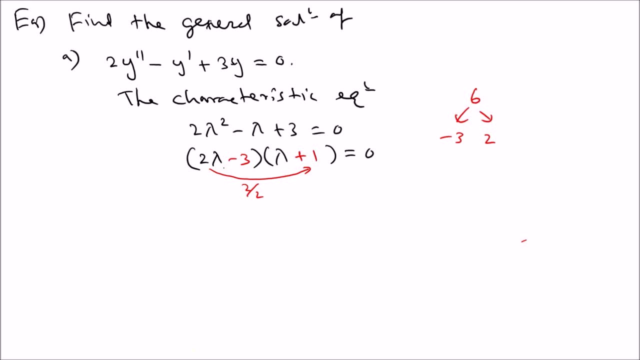 video that you can watch. video that you can watch- okay, good, uh. so then we have the two. okay, good, uh. so then we have the two. okay, good, uh. so then we have the two roots, so roots, so roots. so then you can see, then you can see. 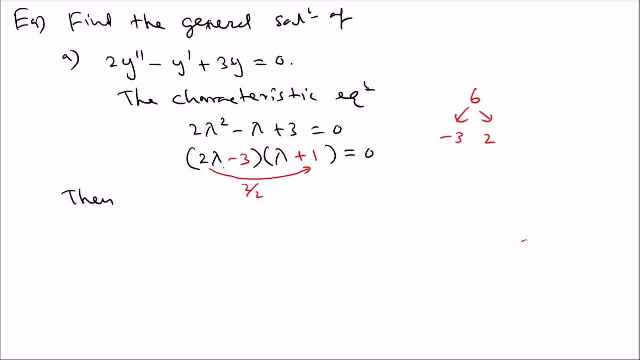 then you can see. so then, uh, you're gonna set them equal. so then, uh, you're gonna set them equal. so then, uh, you're gonna set them equal zero. so you're gonna get zero. so you're gonna get zero, so you're gonna get lambda equal, uh, negative one. 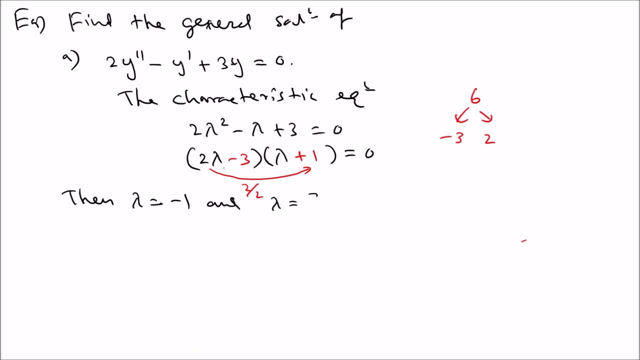 lambda equal, uh, negative one. lambda equal, uh, negative one. and lambda equal and lambda equal and lambda equal three halves. you set them equal to zero. three halves. you set them equal to zero. three halves. you set them equal to zero and get the two values. uh, if you want, i can write that step as: 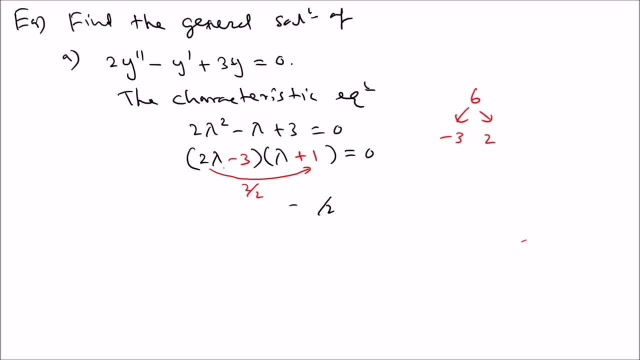 uh, if you want, i can write that step as uh. if you want, i can write that step as well. uh, well, uh, well, uh. so what we normally do is after that. so what we normally do is after that. so what we normally do is after that, uh. 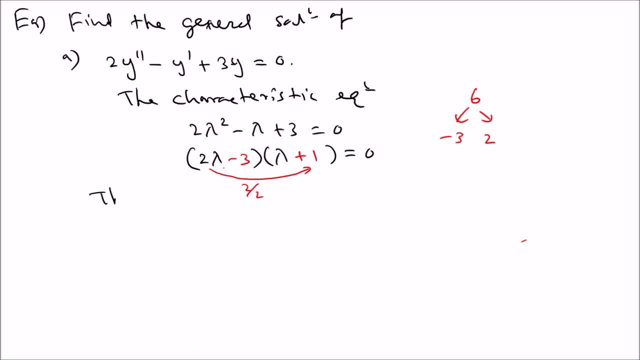 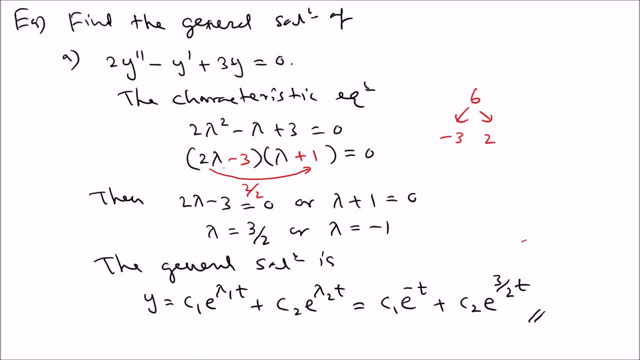 t because i didn't already say anything. okay, good, let's do uh the next example. so problem number b. uh, so we have so problem number b. uh, so we have. so problem number b. uh, so we have four x double prime minus four x prime, four x double prime minus four x prime. 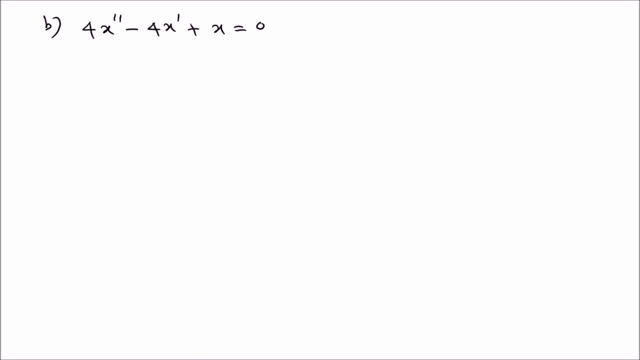 four x double prime minus four x prime plus x equals zero, and you can. plus x equals zero, and you can plus x equals zero and you can definitely pick. cannot pick x as the definitely pick, cannot pick x as the definitely pick, cannot pick x as the independent variable. now, because that is. 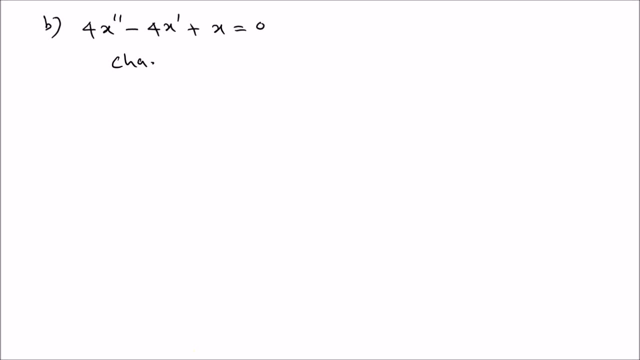 independent variable. now, because that is independent variable. now, because that is the dependent variable, the dependent variable, the dependent variable. okay, so the characteristic equation, okay, so the characteristic equation okay. so the characteristic equation is: is: is four lambda squared minus four lambda, four lambda squared minus four lambda. 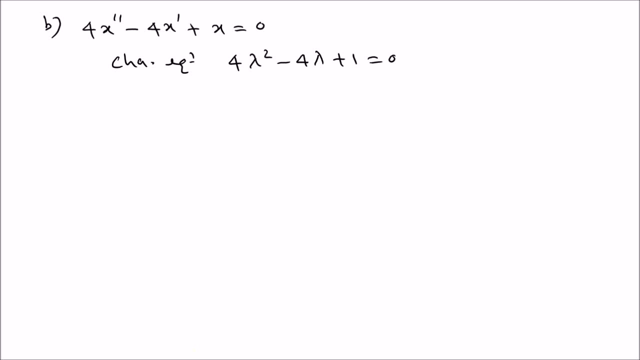 four lambda squared minus four lambda plus one equals zero. our whole factor is, and you can see that our whole factor is, and you can see that our whole factor is, and you can see that this is two. this is two. this is two lambda squared minus two times. 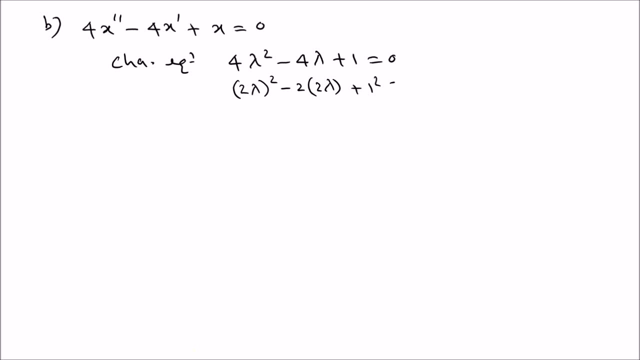 lambda squared minus two times lambda squared minus two times two lambda plus two lambda, plus two lambda plus one squared. so this is a complete one squared. so this is a complete one squared. so this is a complete factorization problem, because we know factorization problem, because we know. 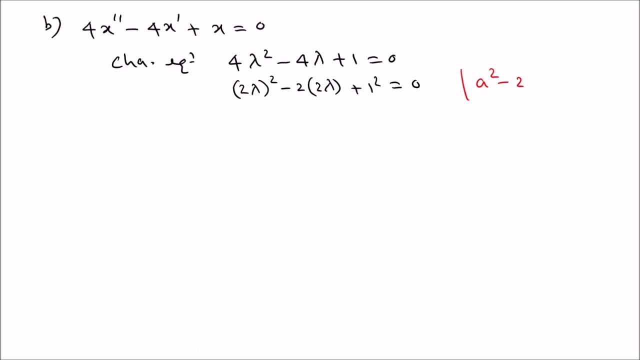 factorization problem, because we know that we have formula, that we have formula, that we have formula: if you're a squared minus two, if you're a squared minus two, if you're a squared minus two, uh, a, b plus b squared. uh, a b plus b squared. 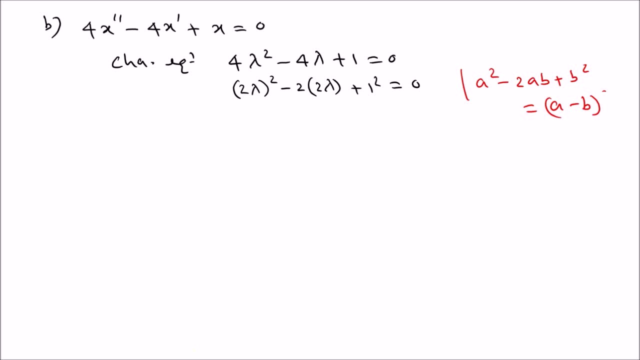 uh, a b plus b squared. this is simply a minus b whole thing. this is simply a minus b whole thing. this is simply a minus b whole thing squared. that's exactly what we have here squared. that's exactly what we have here squared. that's exactly what we have here. uh, so that means this is simply two. 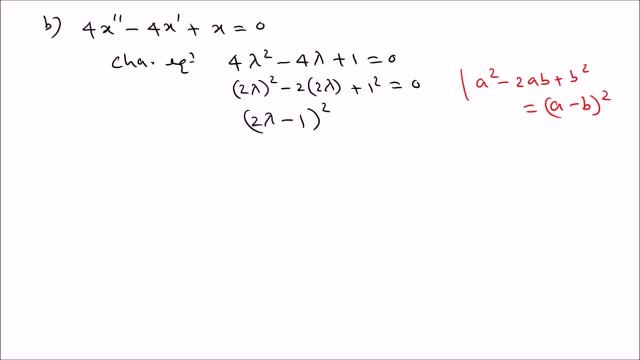 uh, so that means this is simply two. uh, so that means this is simply two. lambda minus one whole thing squared. lambda minus one whole thing squared. lambda minus one whole thing squared. yeah, you can see this again in the uh. yeah, you can see this again in the uh. 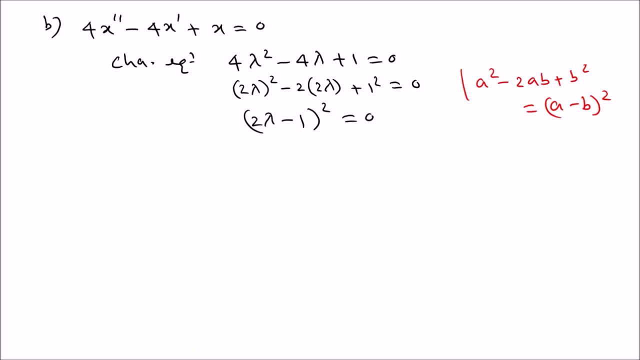 yeah, you can see this again in the uh factor: polynomial video factor. polynomial video factor- polynomial video. good, so we have that now what we can do. good, so we have that now what we can do. good, so we have that now what we can do. we can set this equal to zero. 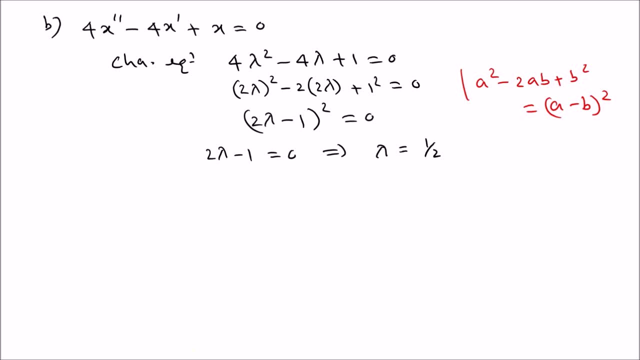 we can set this equal to zero. we can set this equal to zero. half y bring one to other side divided. half y bring one to other side. divided. half y bring one to other side, divided by two, by two, by two. and it also is repeats: uh, because uh. 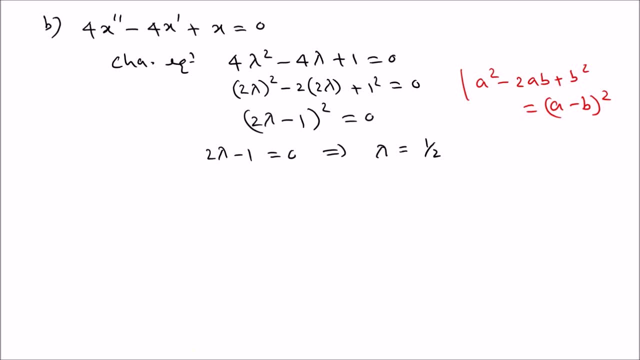 and it also is repeats, uh, because, uh, and it also is repeats, uh because, uh, oh, you can see, with multiplicity two, oh, you can see with multiplicity two, oh, you can see with multiplicity two, uh, with multiplicity a two, because it's a repeat, you can see. 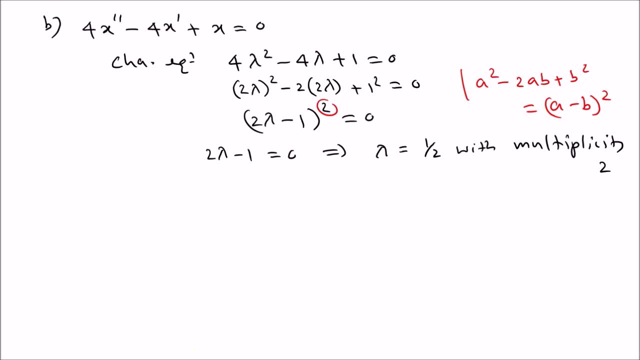 a two because it's a repeat. you can see a two because it's a repeat. you can see square, square, square. good now. uh, so we're gonna get the good now. uh, so we're gonna get the good now. uh, so we're gonna get the solution. 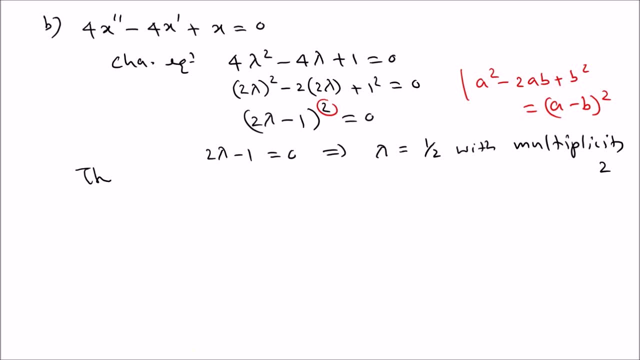 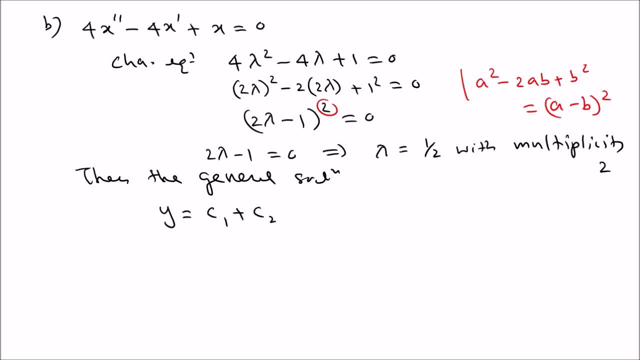 c2, uh, your variable, your independent. c2, uh, your variable, your independent variable. has to be t because you can pick variable. has to be t because you can pick variable. has to be t because you can pick: x there, so t times. x there, so t times. 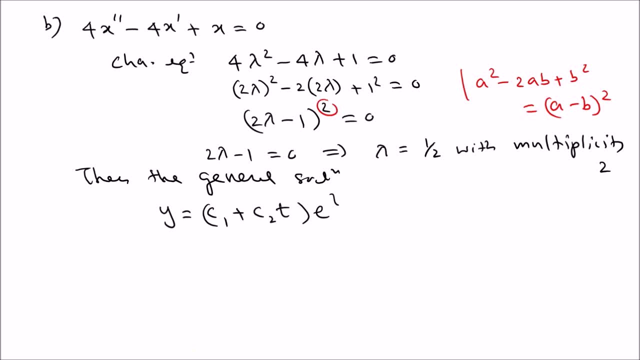 x there. so t times e to the lambda 1 t because it's a e to the lambda 1 t because it's a e to the lambda 1 t because it's a repetition, repetition, repetition. uh, so that means c1 plus c2 e. 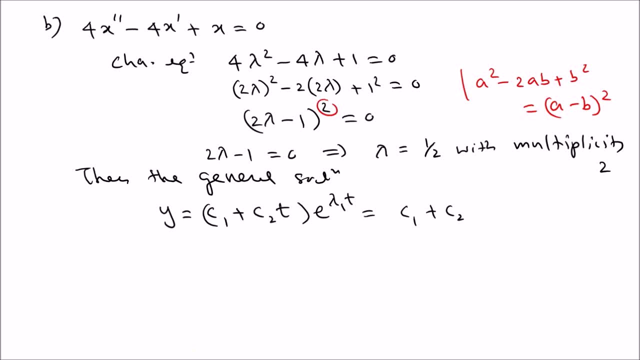 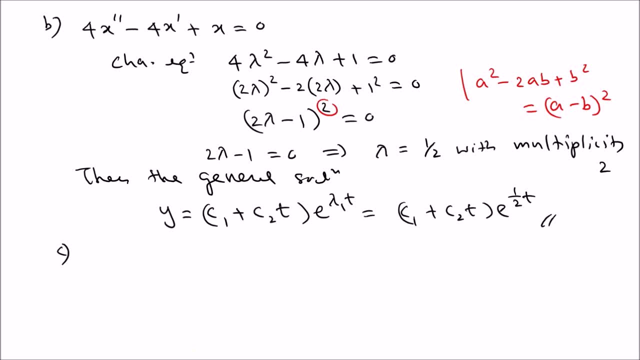 t. so that's the solution: c1, c2- t. so that's the solution: c1- c2- constants, constants, constants. so let's do a last one from the other. so let's do a last one from the other. so let's do a last one from the other type, the complex type. 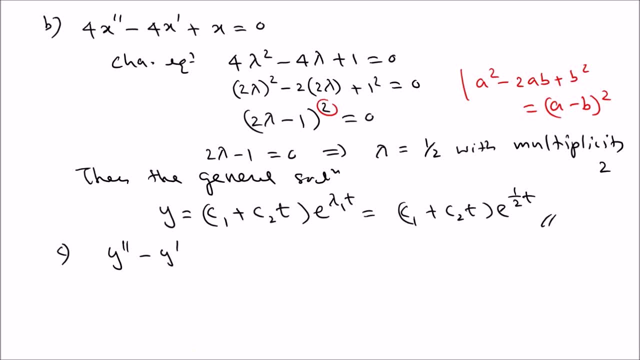 type the complex type, type the complex type. so let's say y double prime minus y. so let's say y double prime minus y. so let's say y double prime minus y prime prime prime: plus y equals zero, again plus y equals zero, again plus y equals zero, again. the characteristic equation is: 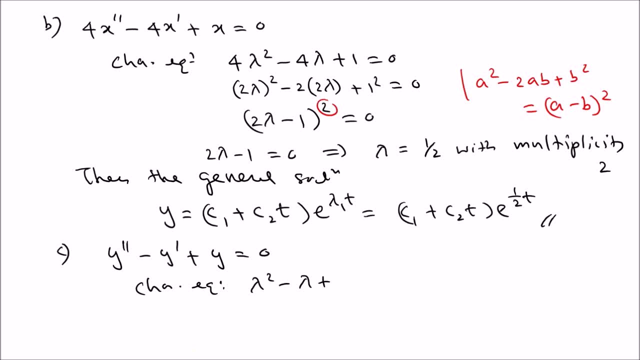 the characteristic equation is: the characteristic equation is: lambda squared minus lambda plus one. lambda squared minus lambda plus one. lambda squared minus lambda plus one equals equals, equals equals zero. you can see that you can find zero. you can see that you can find zero. you can see that you can find factors of this one. so you have to use: 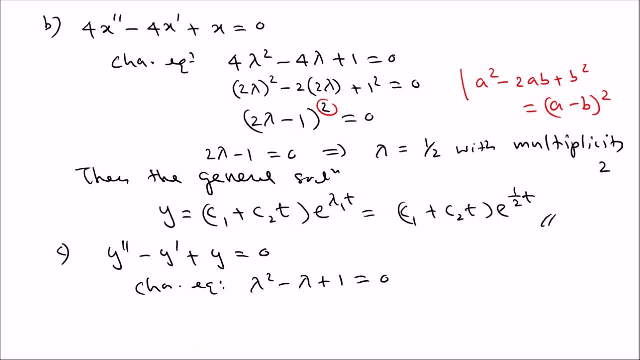 factors of this one. so you have to use factors of this one. so you have to use the uh, the uh, the uh, formula uh, quadratic formula. so which is formula uh, quadratic formula. so which is formula uh, quadratic formula. so which is lambda, lambda lambda? a negative b plus or minus, b squared. 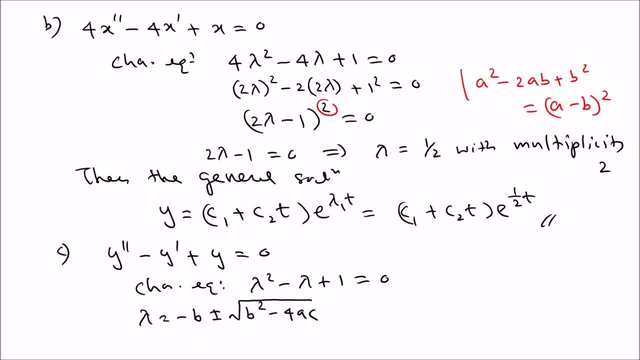 a negative b plus or minus b. squared a negative b plus or minus b. squared minus 4ac, minus 4ac, minus 4ac. square root over 2a. square root over 2a. square root over 2a. so let's plug in here, so you get 1. 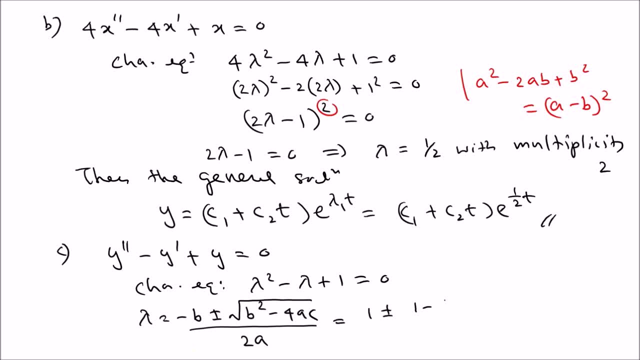 so let's plug in here, so you get 1. so let's plug in here, so you get 1 plus or minus 1 minus 4 plus or minus 1 minus 4 plus or minus 1 minus 4 a c, so you get over. 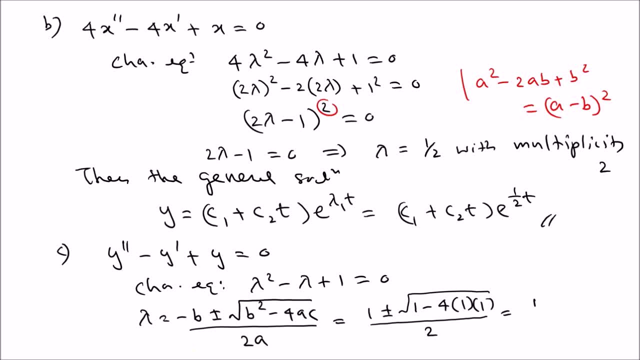 a c, so you get over a c, so you get over. 2a means 2, so which is 2a means 2, so which is 2a means 2, so which is 1 plus or minus negative 3 square root: 1 plus or minus negative 3 square root. 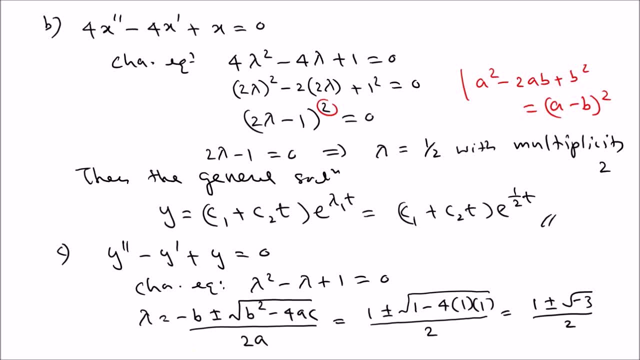 1 plus or minus negative 3 square root over t. you need complex numbers for that over t. you need complex numbers for that over t. you need complex numbers for that. so that's going to square root 3 i so. so that's going to square root 3 i so. 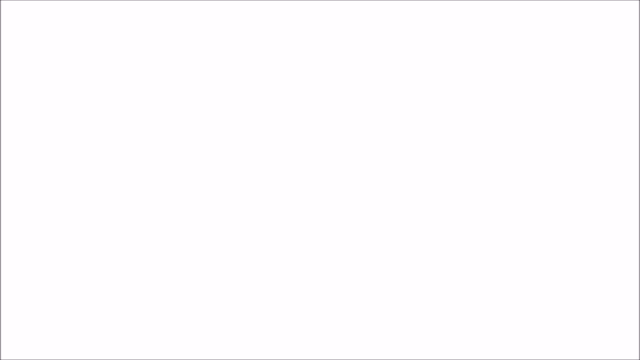 so that's going to square root 3, i. so this says that, this says that, this says that, and so we have lambda equal, and so we have lambda equal, and so we have lambda equal: 1 plus or minus square root 3. 1 plus or minus square root 3. 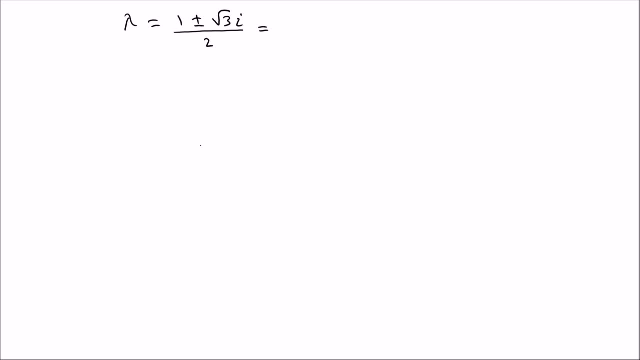 1 plus or minus square root: 3. i over 2. i over 2. i over 2. if you separate this, if you separate this, if you separate this, you can write this one as one half plus. you can write this one as one half plus. 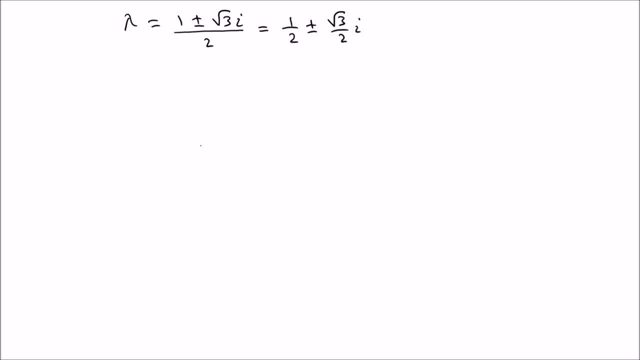 you can write this one as one half plus or minus or minus or minus. square root 3 i over square root 3 over square root 3 i over square root 3 over square root 3 i over square root 3 over 2 i. 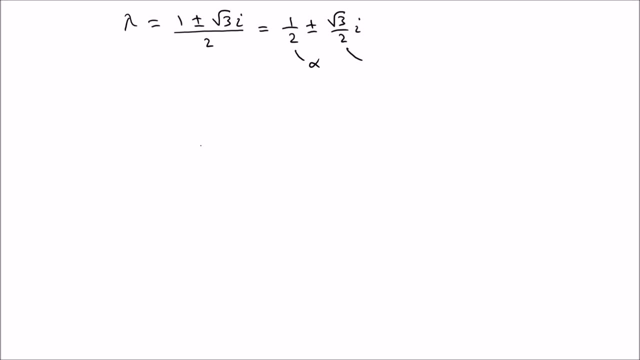 2 i, 2 i. so you can see that that is the alpha. so you can see that that is the alpha. so you can see that that is the alpha value and that is the beta value value and that is the beta value value and that is the beta value. so the general solution is: 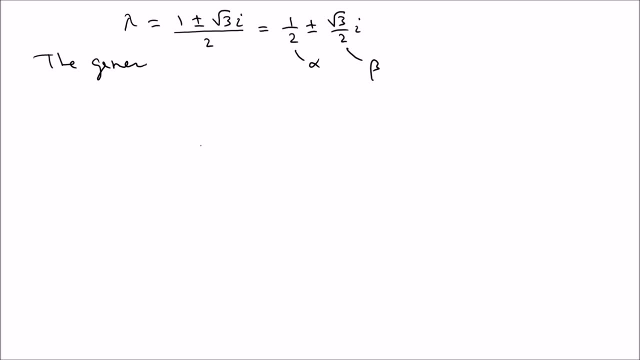 so the general solution, general solution is given by, general solution is given by, general solution is given by y. let's say x is the independent y. let's say x is the independent y. let's say x is the independent variable, variable, variable e, alpha x, e, alpha x. 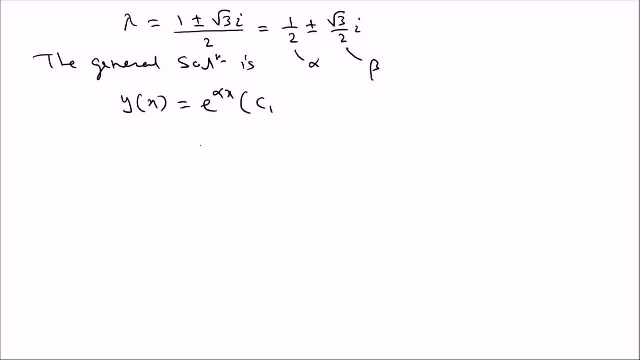 e alpha x times c: 1 cos times c: 1 cos times c 1. cos beta x. beta x. beta x plus c 2 sine plus c 2 sine plus c 2 sine beta x. so that is the format. beta x. so that is the format. 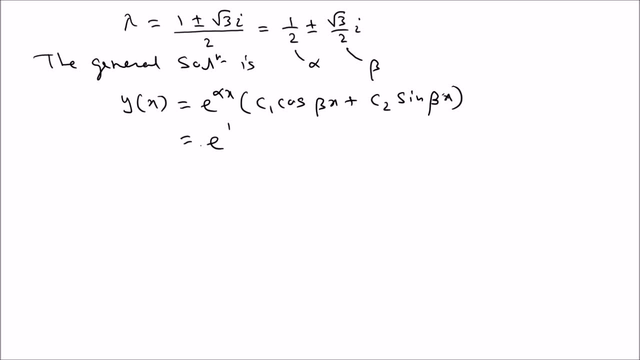 beta x. so that is the format. so we're going to plug in here so it is. so we're going to plug in here so it is. so we're going to plug in here so it is: e, e, e, one half x times one half x times. 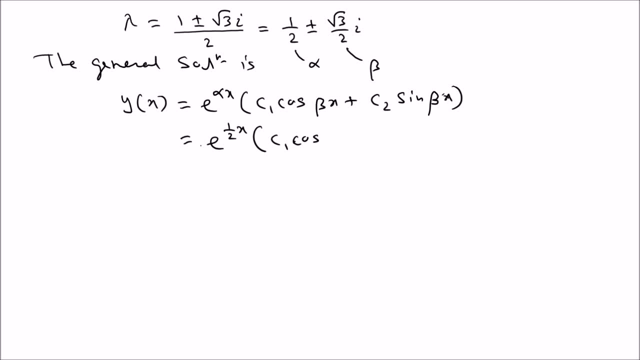 one half x times c1 cos, c1 cos, c1 cos. square root: 3 over 2. square root 3 over 2. square root 3 over 2 x plus c2, x plus c2, x plus c2, sine sine, sine sine square root 3 over. 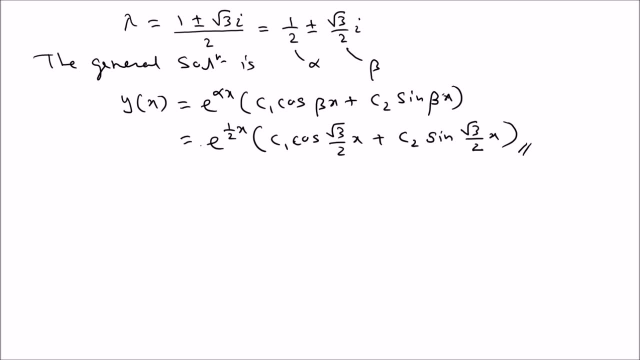 square root 3 over square root, 3 over 2 x. so that is the general solution with 2 x. so that is the general solution with 2 x. so that is the general solution with c1, c2, c1, c2, c1, c2, unknown. and now what we can do is: 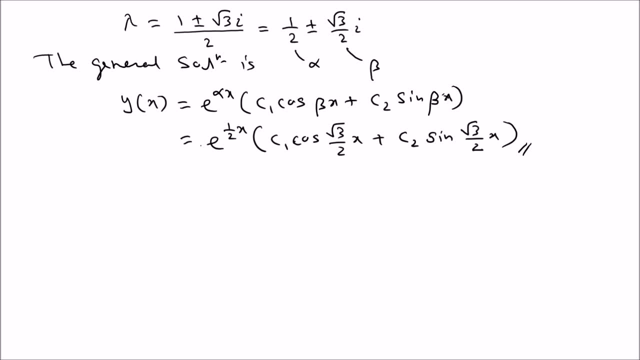 unknown. and now what we can do is unknown. and now what we can do is: we can completely solve a problem with. we can completely solve a problem with. we can completely solve a problem with initial conditions as initial conditions, as initial conditions as well, and to see how it works. as the last, 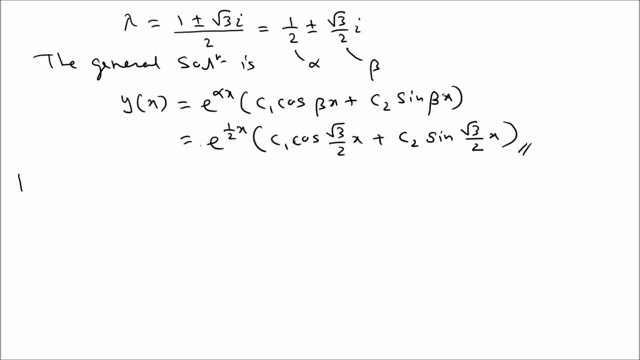 well, and to see how it works as the last well, and to see how it works as the last problem of this type, problem of this type, problem of this type. so let's do that, uh, so, let's do that, uh, so, let's do that, uh, so solve. 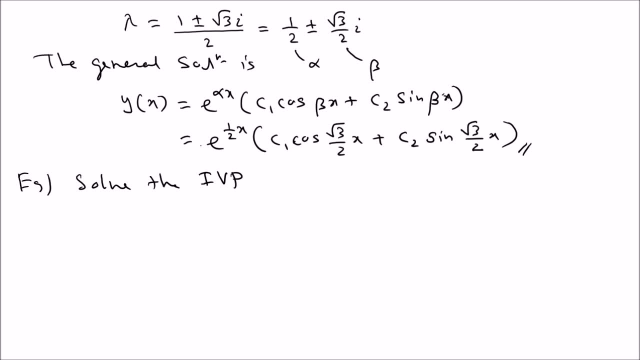 so solve. so solve the initial value problem, the initial value problem, the initial value problem: x double prime plus x double prime plus x double prime plus x prime plus 3x x prime plus 3x x prime plus 3x equals 0 with equals 0 with. 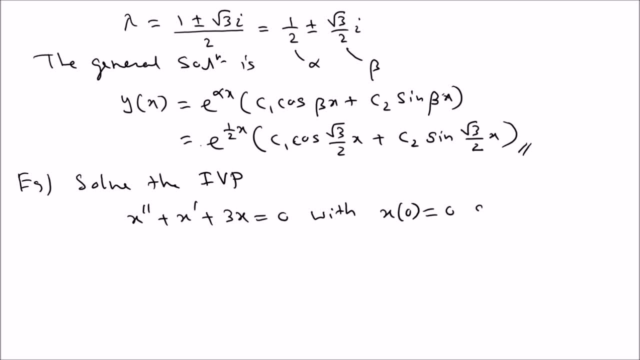 equals 0, with x 0 equals 0, x 0 equals 0 and x prime 0 and x prime 0 and x prime 0 equal 22 and later we can solve this equal 22 and later we can solve this equal 22 and later we can solve this exact same problem using the laplace. 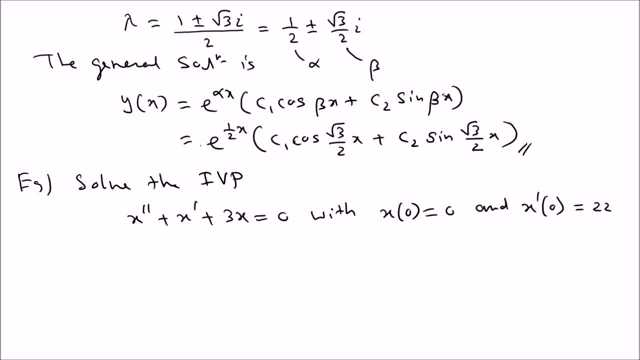 exact same problem using the laplace. exact same problem using the laplace transform method. and you can see transform method and you can see transform method and you can see how it works. okay, but right now we're how it works. okay, but right now we're how it works. okay, but right now we're going to use the. 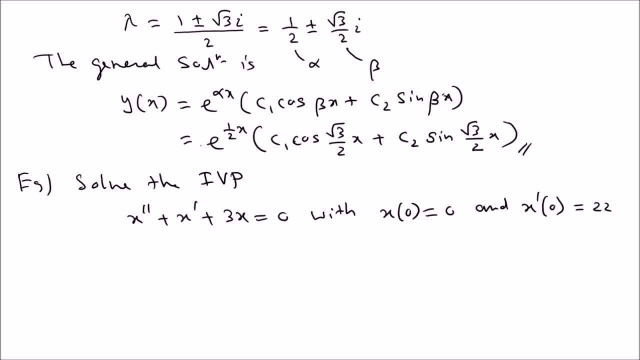 going to use the going to use the constant constant, constant coefficient difference equation. coefficient difference equation, coefficient difference equation. technique, because that's much easier. technique because that's much easier. technique because that's much easier. so let's do that. uh, okay, so the answer. so let's do that. uh okay, so the answer. 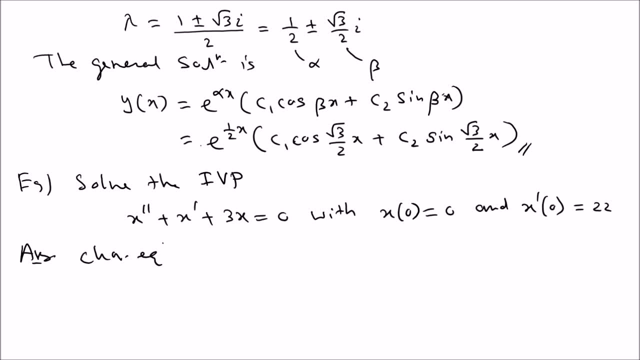 so let's do that. uh, okay, so the answer: we can look at the characteristic. we can look at the characteristic, we can look at the characteristic equation, equation, equation: so which is lambda squared plus lambda, so which is lambda squared plus lambda, so which is lambda squared plus lambda plus 3 equals 0. 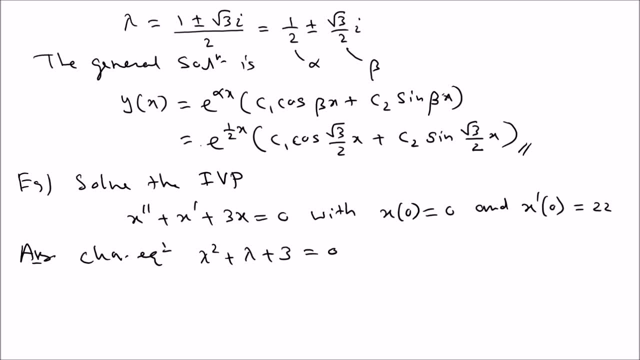 plus 3 equals 0. plus 3 equals 0. and then you can see i it's impossible to. and then you can see i it's impossible to. and then you can see i it's impossible to find the factors. so we're going to go. 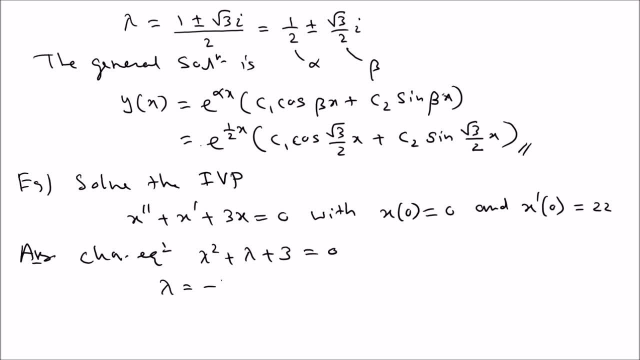 find the factors. so we're going to go find the factors. so we're going to go: with lambda, equal formula negative b. with lambda equal formula negative b. with lambda equal formula negative b. plus or minus b squared minus 4. plus or minus b squared minus 4. 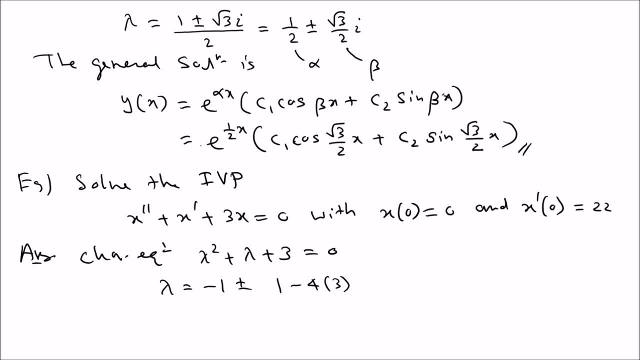 plus or minus. b squared minus 4: uh a is one, so c. uh a is one, so c. uh a is one, so c. over two over two over two. so we can simplify this in negative one. so we can simplify this in negative one. so we can simplify this in negative one, plus or minus. 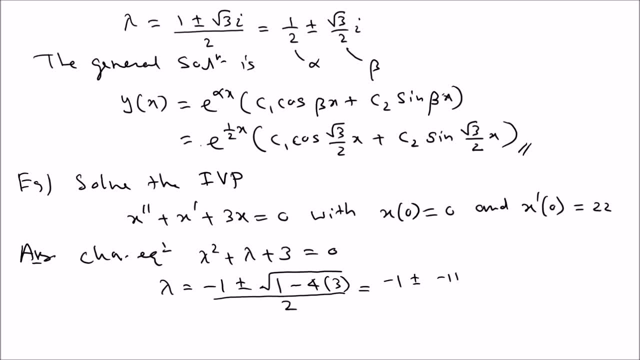 plus or minus, plus or minus. uh, negative 11, so negative 11 square. uh, negative 11, so negative 11 square. uh, negative 11, so negative 11 square. root over two. if you split this, you can. root over two. if you split this, you can. 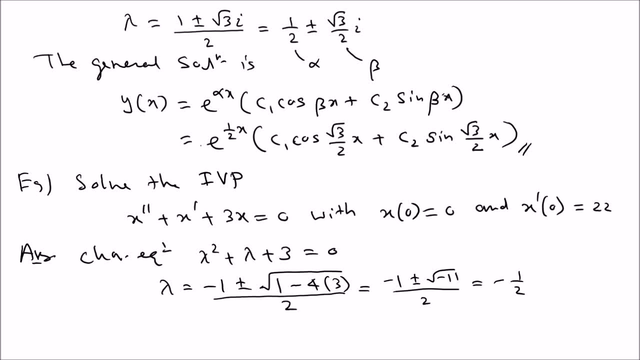 root over two. if you split this, you can write this as negative. one half. write this as negative one half. write this as negative. one half: ah. plus or minus. ah. plus or minus. ah. plus or minus. square root 11 over 2 i. square root 11 over 2: i. 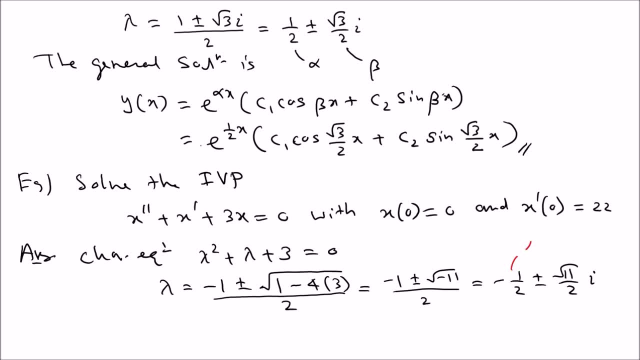 square root: 11 over 2. i. so, uh, so that's the alpha value. so, uh, so that's the alpha value. so, uh, so that's the alpha value. this is the beta value. so you have the. this is the beta value. so you have the. this is the beta value. so you have the alpha value and the beta value. 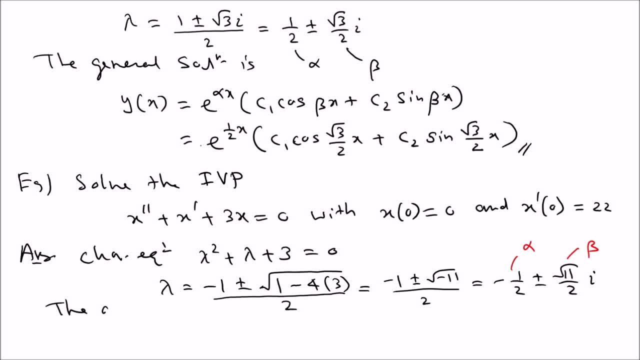 alpha value and the beta value. alpha value and the beta value. so the general solution, so the general solution, so the general solution. so so the general solution, so the general solution. you can write as: so the general solution. you can write as: so the general solution. you can write as: x, t. 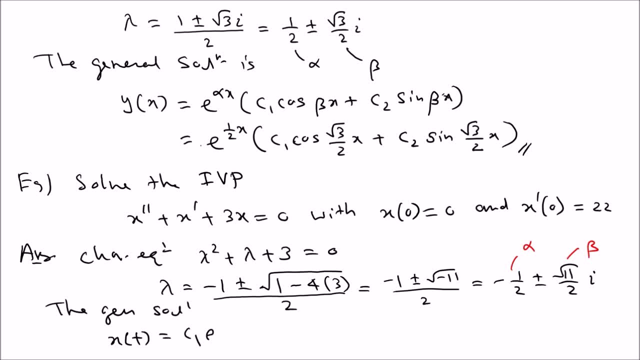 x, t, x, t which is c 1 e to the which is c 1 e to the which is c 1 e to the alpha value. alpha value, alpha value, t. so let's say so, t, so let's say so, t, so let's say so. the function of t, independent variable. 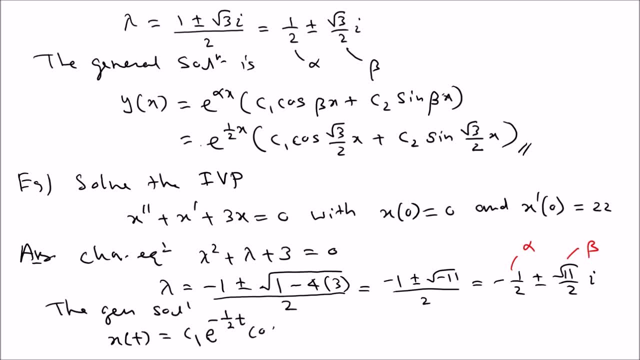 the function of t independent variable. the function of t independent variable is t is t is t. and then we have cosine beta, which is, and then we have cosine beta which is, and then we have cosine beta which is: square root 11 over 2. square root 11 over 2. 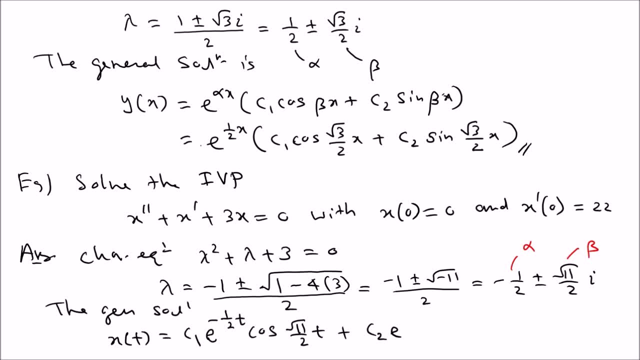 square root: 11 over 2 t plus c 2 e to the negative half t plus c 2 e to the negative half t plus c 2 e to the negative half t sine square root: 11 over 2 t. sine square root. 11 over 2. 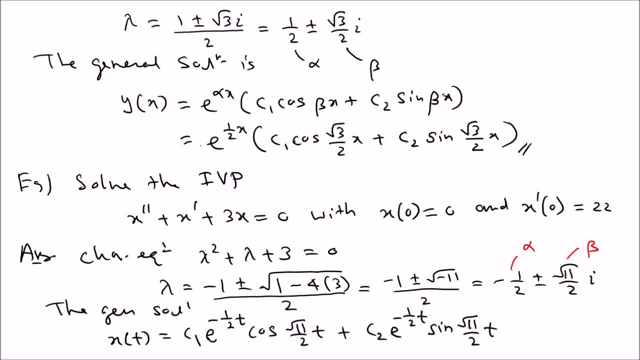 t sine square root 11 over 2 t. so that is the general solution. you t. so that is the general solution. you t. so that is the general solution. you can. general solution, three lines can. general solution, three lines can. general solution, three lines. now, only thing what we have to do is to 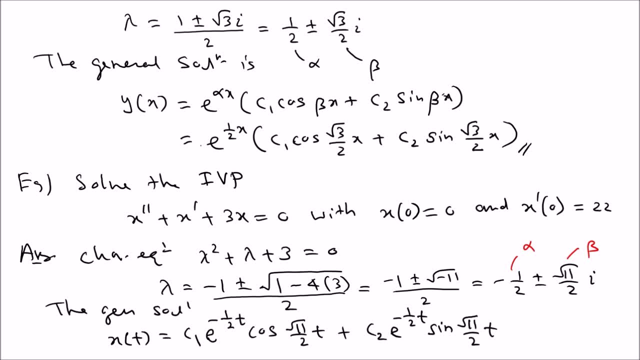 now only thing. what we have to do is to now only thing. what we have to do is to find c1- c2 using the initial conditions. find c1- c2 using the initial conditions. find c1- c2 using the initial conditions. so let's do that so we can use the. 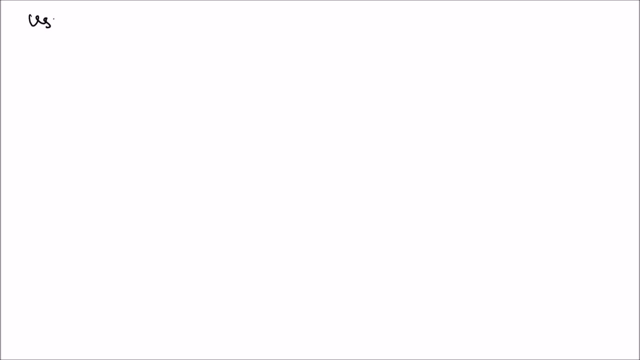 so let's do that, so we can use the. so let's do that, so we can use the initial conditions, initial conditions, initial conditions. so using the initial condition, so using the initial condition, so using the initial condition: first x 0 equal 0. first x 0 equal 0. 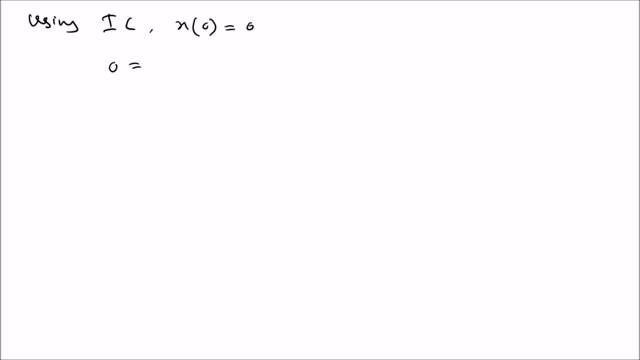 first, x, 0 equal 0. we have a 0 equal. we have a 0 equal. we have a 0 equal x to the zero. that means plug in 0. x to the zero. that means plug in 0, x to the zero. that means plug in 0 wherever you see t, so c1, e to the zero. 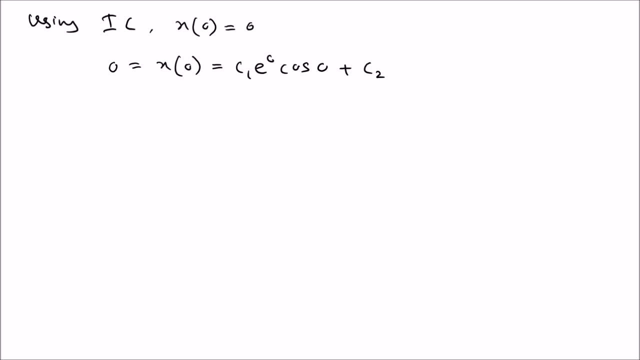 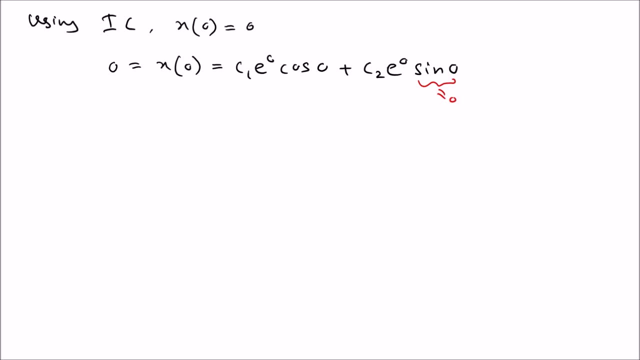 sine zero, sine zero. so this is that this is equal to zero. so this is that this is equal to zero. so this is that this is equal to zero. this is equals to one e this is we know. this is equals to one e this is we know. 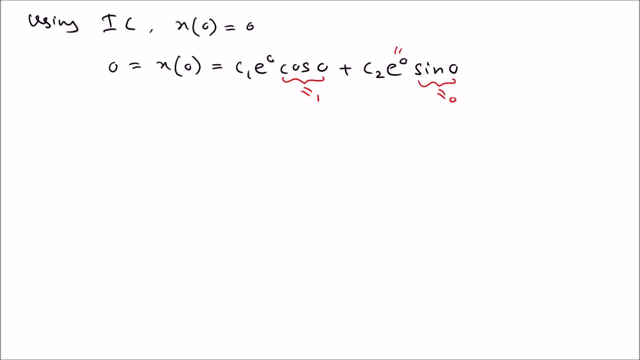 this is equals to one. e this is. we know that this is one, that this is one, that this is one. sorry, this is one. sorry, this is one. sorry, this is one, and this is also uh one, and this is also uh one and this is also uh one. so that means you simply end up with. 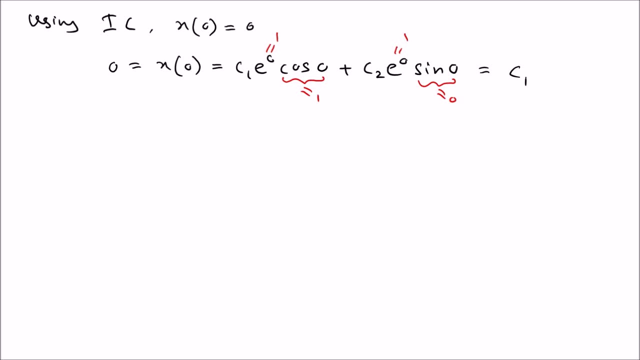 so that means you simply end up with. so that means you simply end up with: pretty good, uh, pretty good, uh, pretty good, uh, c1. so this says that c1 equals c1. so this says that c1 equals c1. so this says that c1 equals zero. so that means your solution. 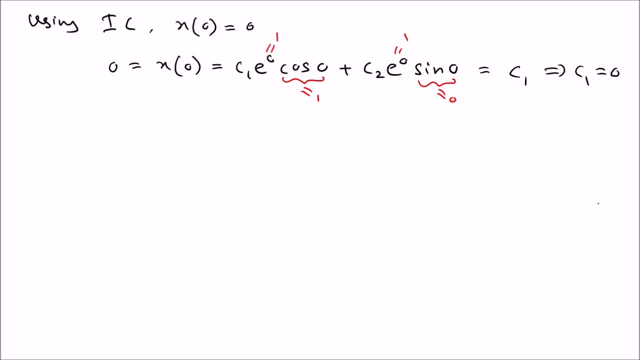 zero. so that means your solution zero. so that means your solution kind of simplified because you don't kind of simplified, because you don't kind of simplified because you don't need the c1 term, need the c1 term, need the c1 term. so that means you have. so thus, 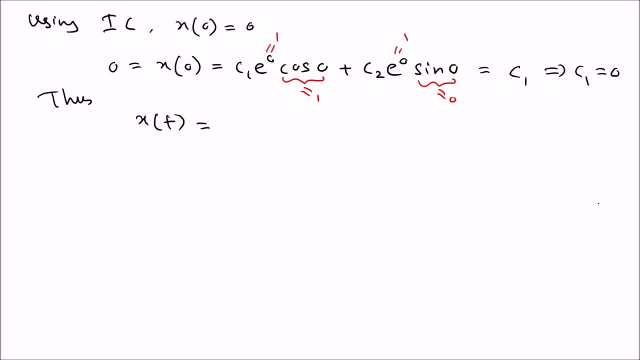 so that means you have so thus. so that means you have so thus. we can write xt like this: it is simply. we can write xt like this. it is simply. we can write xt like this. it is simply: c2 e to the negative, c2 e to the negative. 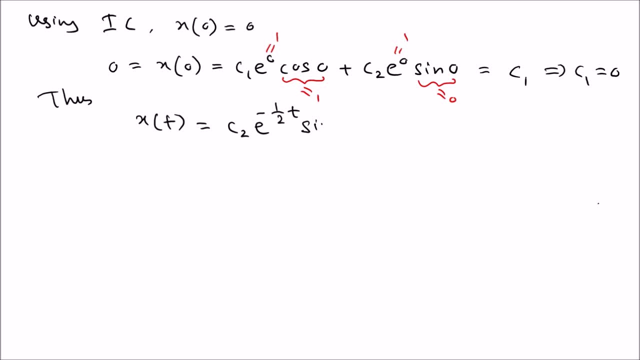 c2 e to the negative one, half t sine square root 13 over 2 t sine square root 13 over 2 t sine square root 13 over 2 t um. so before you create the derivative um, so before you create the derivative um, so before you create the derivative, it's a good idea to do this because then 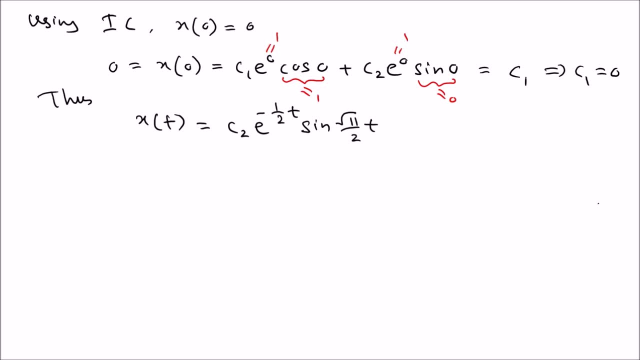 it's a good idea to do this because then it's a good idea to do this, because then you have only one term, you have only one term, you have only one term. otherwise like it to be difficult. so, uh, now what we can do is, uh, we can take the. 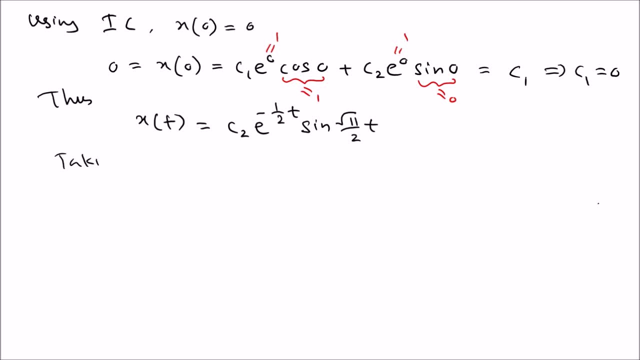 now what we can do is, uh, we can take the. now what we can do is, uh, we can take the derivative, so taking derivatives derivative, so taking derivatives derivative, so taking derivatives, taking a derivative. so we can use a product rule here, so we. so we can use a product rule here, so we. 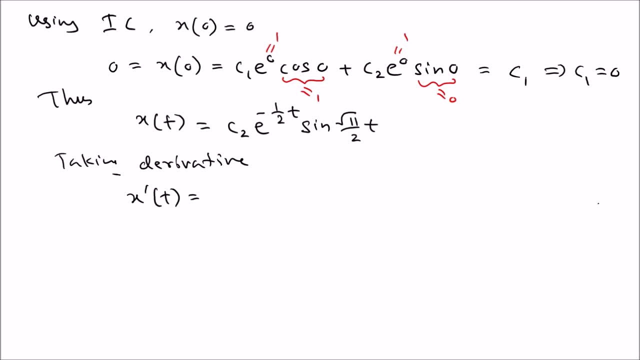 so we can use a product rule here. so we have x prime t, have x prime t, have x prime t, equal, equal, equal, uh, equal, uh. so take the derivative the first term, so take the derivative the first term, so take the derivative the first term, so you get. 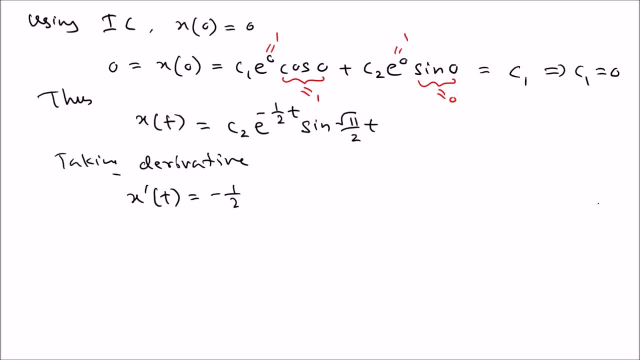 so you get. so you get one half negative, one half, one half negative, one half one half negative, one half c 2 e to the negative, one half t. c 2 e to the negative, one half t. c 2 e to the negative, one half t. no change to this term. 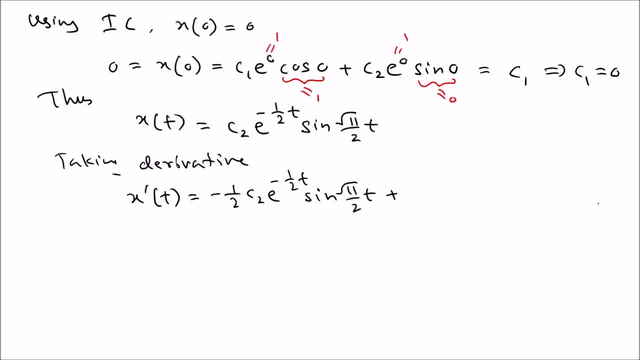 no change to this term. no change to this term. plus now you take the other term, so that, plus now you take the other term, so that, plus now you take the other term, so that means sine, so by the chain rule, means sine, so by the chain rule. 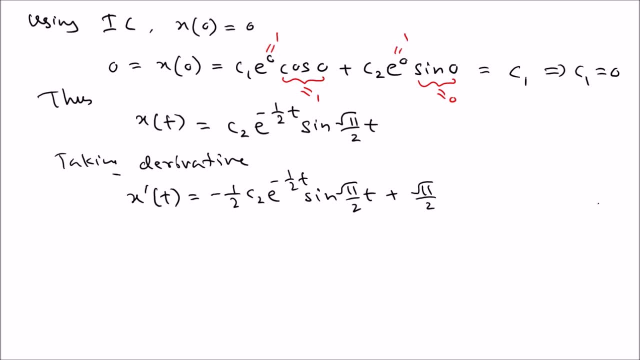 means sine. so by the chain rule: square root 2: square 11 over 2 comes out. square root 2: square 11 over 2 comes out. square root 2: square 11 over 2 comes out. you have c 2 e to the negative one half. 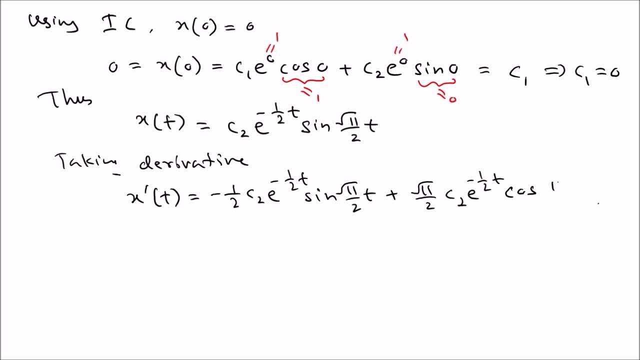 you have c 2 e to the negative one, half. you have c 2 e to the negative one, half. t sine become cosine square root. t sine become cosine square root. t sine become cosine square root 11 over 2 t. that's what you get. 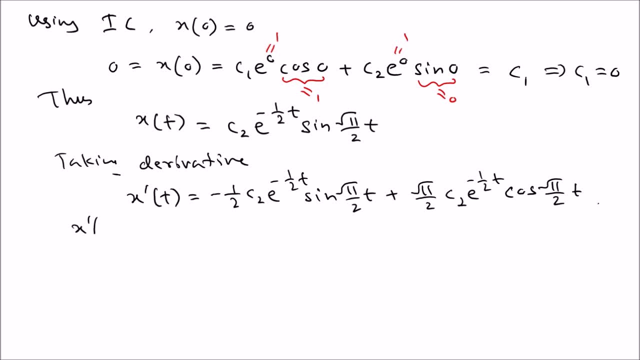 11 over 2 t. that's what you get. 11 over 2 t- that's what you get. now we apply the condition, so x prime. now we apply the condition, so x prime. now we apply the condition, so x prime: 0 equal 22 gives. 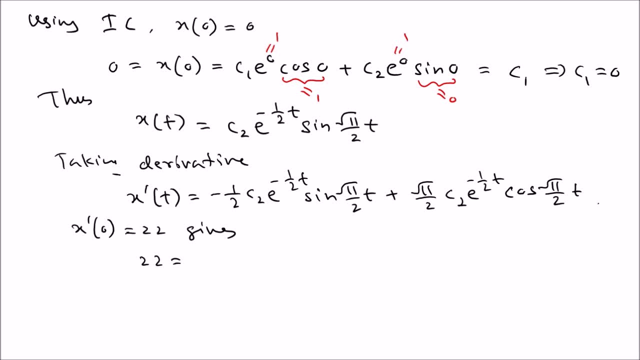 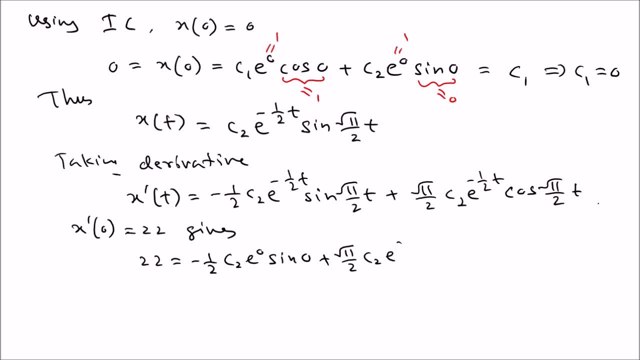 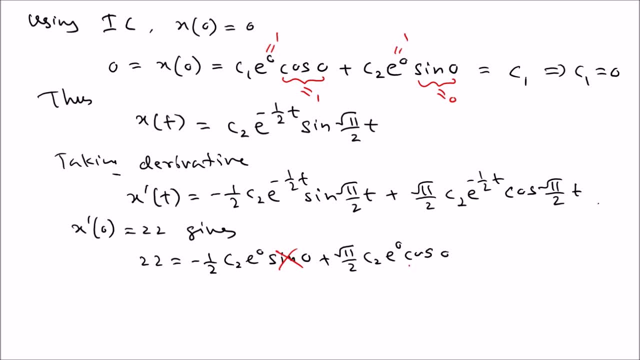 that means as before. that means as before, this is gone. uh, this is this is gone. uh, this is this is gone. uh, this is one. so you're gonna get one. so you're gonna get one. so you're gonna get. what do you get? you're gonna get. 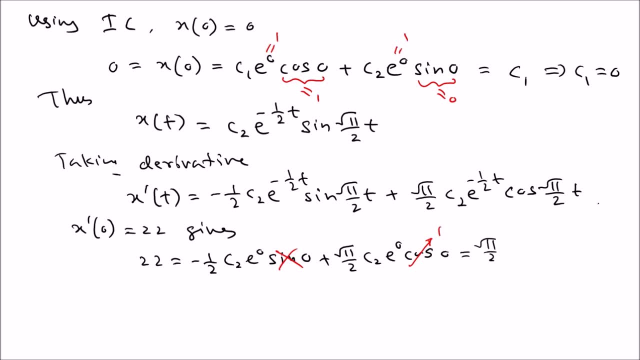 square root: 11 over 2. square root, 11 over 2. square root, 11 over 2: c2. so that's going to give you the c2, c2. so that's going to give you the c2, c2. so that's going to give you the c2 value. so this says: 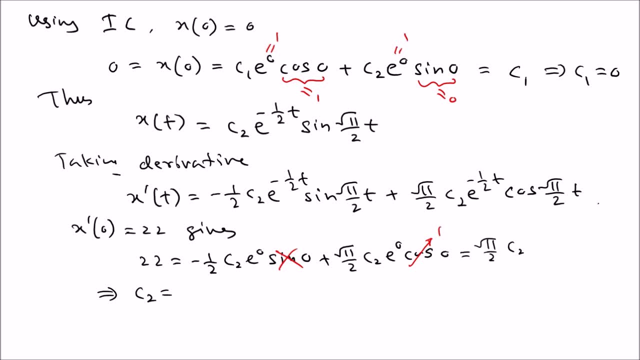 value. so this says value. so this says that that that c2 equal c2 equal c2 equal 4 t 4 over square root 11, in other words, 4 t 4 over square root 11. in other words, 4 t 4 over square root 11, in other words, 4 square root 11. okay, that's c2 value. 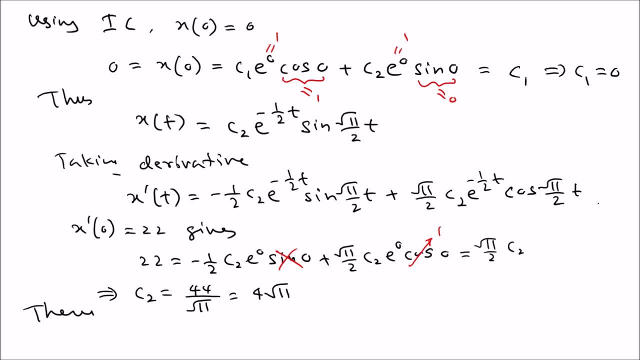 4 square root 11: okay, that's c2 value. 4 square root 11: okay, that's c2 value. so, therefore, we have the solution now. so, therefore, we have the solution now. so, therefore, we have the solution now. we have x t, we have x t. 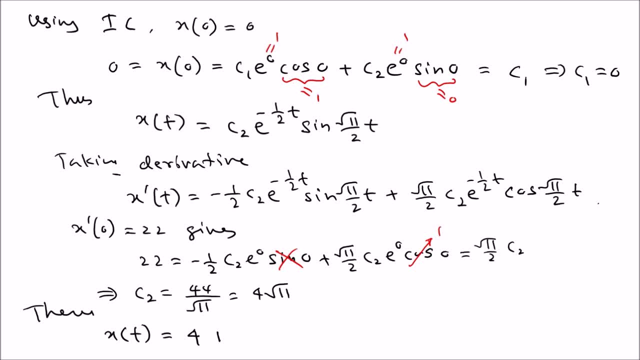 we have x, t, which is, which is: which is 4 square root 11, 4 square root 11, 4 square root 11 e to the negative one, half t e to the negative one, half t e to the negative one, half t sine square root. 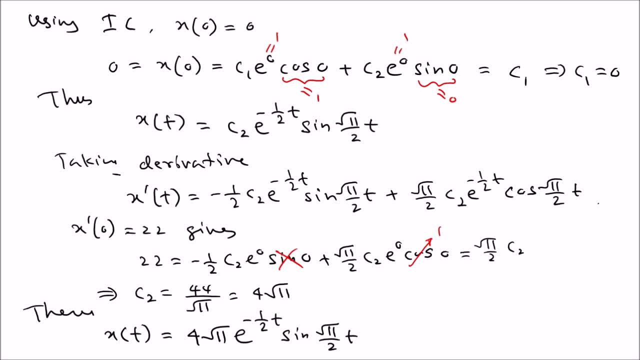 sine square root. sine square root. 11 over 2 t. 11 over 2 t. 11 over 2 t. um, yeah, so that's the solution. so let's um yeah, so that's the solution. so let's um: yeah, so that's the solution. so let's talk about something more about this one. 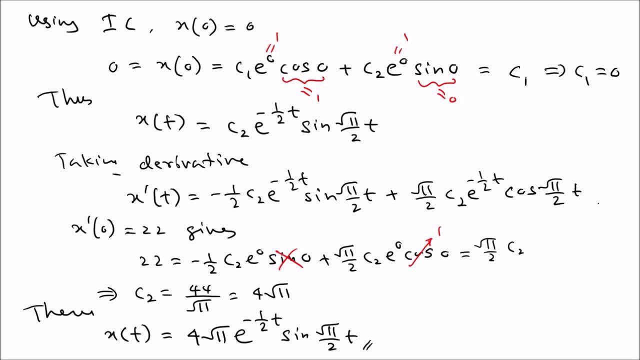 talk about something more about this one. talk about something more about this one. you can see that in this problem, this is. you can see that in this problem, this is. you can see that in this problem, this is a periodic function, we have sine term. a periodic function, we have sine term. 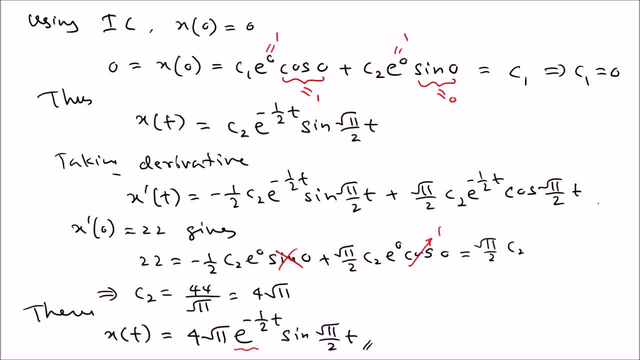 a periodic function. we have sine term. that means the periodic function. but you, that means the periodic function. but you, that means the periodic function. but you can see the amplitude, can see the amplitude, can see the amplitude, that's the amplitude, that's what you got, that's the amplitude, that's what you got. 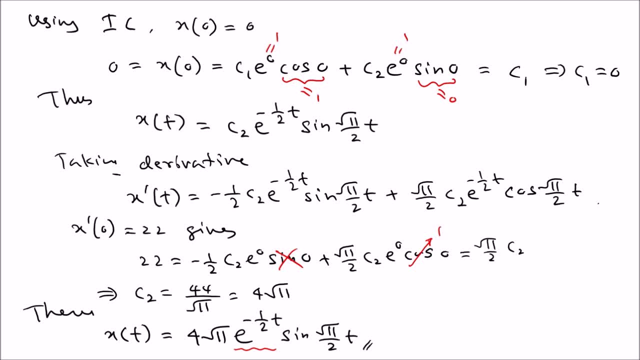 that's the amplitude. that's what you got. envelope, envelope: envelope: that's going to decrease because there's that's going to decrease. because there's that's going to decrease because there's a e, a e, a e. negative term, so that's going to decrease. negative term, so that's going to decrease. 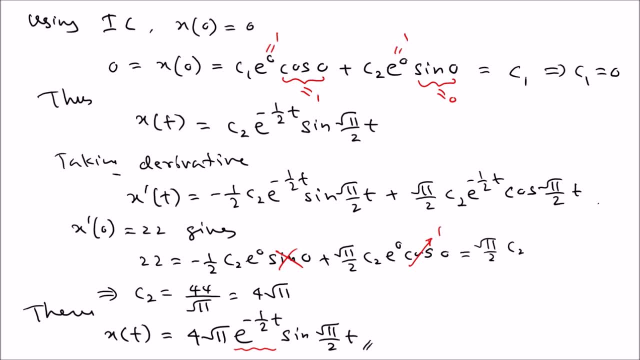 negative term, so that's going to decrease. so that means, if you look at the graph of. so that means, if you look at the graph of, so that means, if you look at the graph of this one, this is very interesting. this one, this is very interesting. this one, this is very interesting. so, uh, so, if you graph this function, 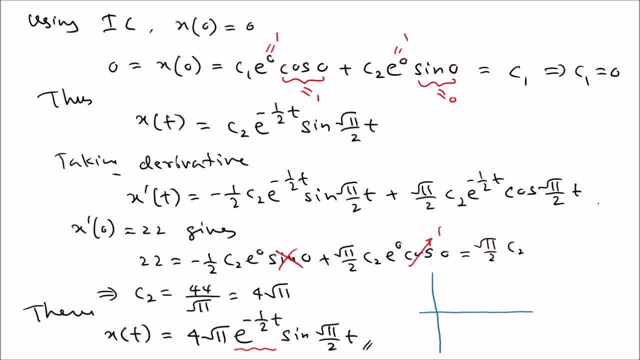 so, uh, so, if you graph this function, so, uh, so, if you graph this function, this is how it looks like. so we have what we call this envelope. so we have what we call this envelope. so we have what we call this envelope. curve e to the negative one: half t. 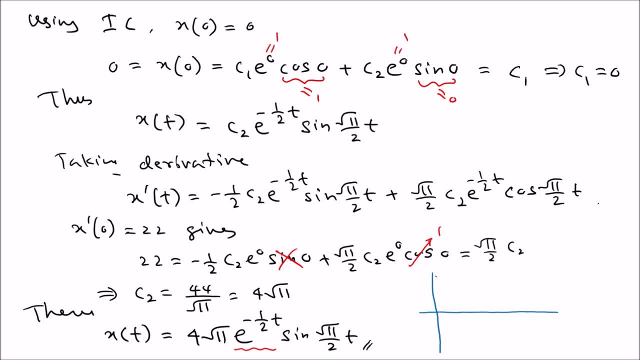 curve e to the negative one half t. curve e to the negative one half t, that's envelope. so that's going to that's envelope. so that's going to that's envelope. so that's going to decrease. so it's going to go like that. and then it's a sign. sign that means the. 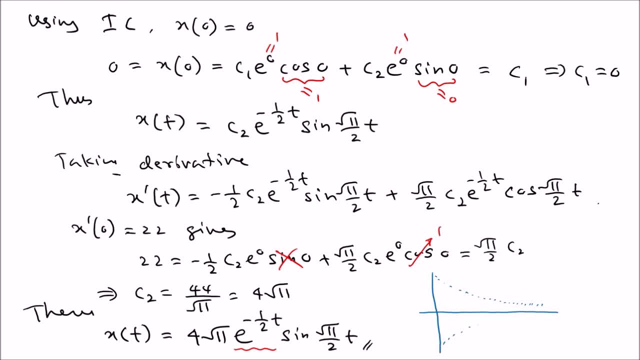 and then it's a sign sign that means the, and then it's a sign sign that means the plus minus. so what we normally do is we plus minus. so what we normally do is we plus minus. so what we normally do is. we can reflect it like that: 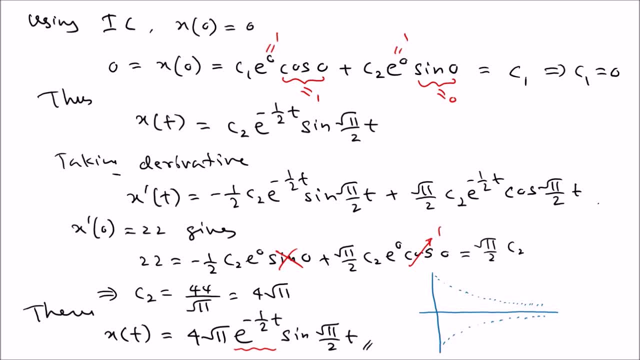 can reflect it like that, can reflect it like that. so what's going to happen now? we're so. what's going to happen now? we're. so. what's going to happen now? we're going to graph the sine function inside. going to graph the sine function inside. 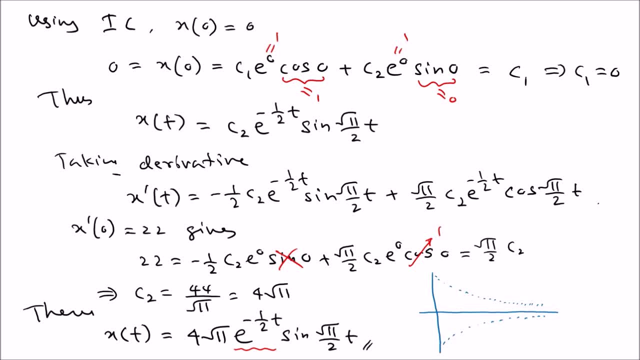 going to graph the sine function inside. because when you have t equals 0, this is because, when you have t equals 0, this is because, when you have t equals 0, this is a zero, a zero, a zero. that's exactly what happened in this. that's exactly what happened in this. 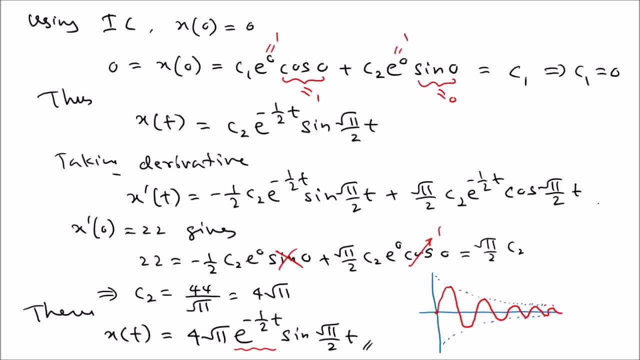 that's exactly what happened in this kind of situations, kind of situations, kind of situations, um. so this is simply this curve is um. so this is simply this curve is um. so this is simply this curve is simply a 4, simply a 4, simply a 4 square root, 11 e to the negative one, half. 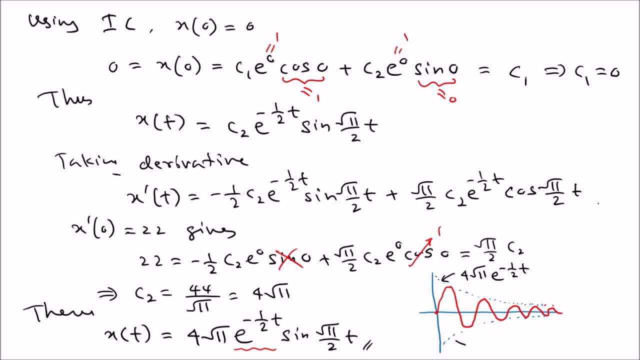 square root: 11 e to the negative one. half square root, 11 e to the negative one: half t. that's that curve. this is exactly the t. that's that curve. this is exactly the t. that's that curve. this is exactly the opposite of that, opposite of that. 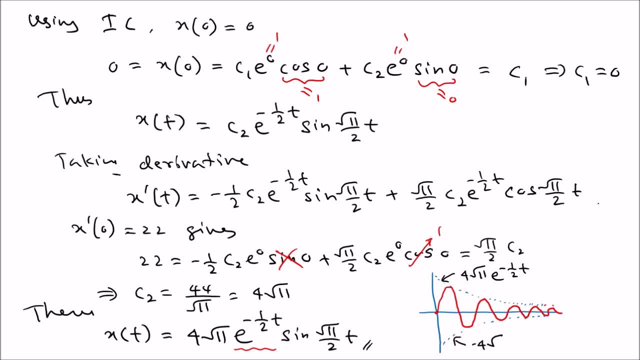 opposite of that. this is the negative 4 square root 11. this is the negative 4 square root 11. this is the negative 4 square root 11. e to the negative one, half t e to the negative one, half t e to the negative one, half t um. so these kind of situations are like: 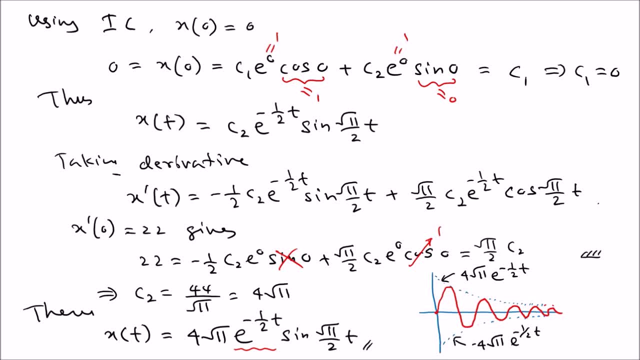 um. so these kind of situations are like um. so these kind of situations are like kind of common, like you know, if you kind of common, like you know, if you kind of common, like you know, if you have like a bob hand like that, have like a bob hand like that. 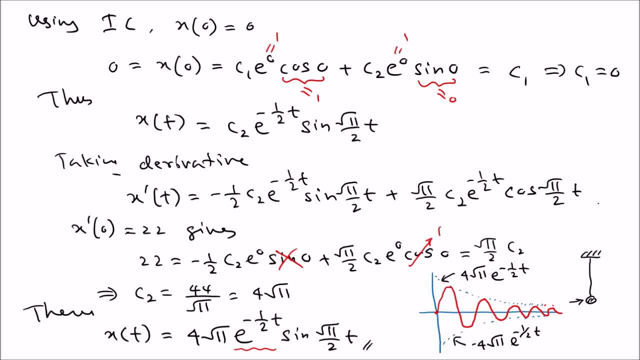 have like a bob hand like that and put like a sudden force like impulse and put like a sudden force like impulse, and put like a sudden force like impulse, then it's gonna go in like a motion like: then it's gonna go in like a motion like: 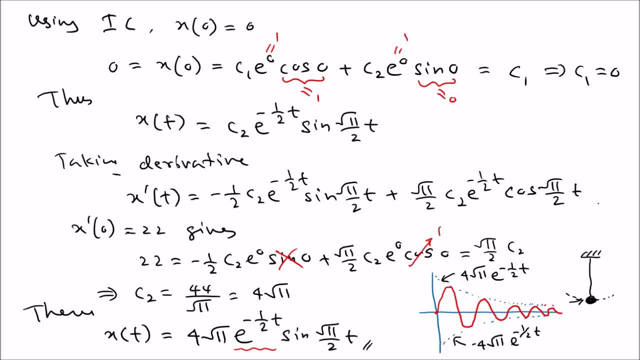 then it's gonna go in like a motion like this, this, this: uh, it's gonna go to this corner and to uh it's gonna go to this corner and to uh it's gonna go to this corner and to that corner, that corner, that corner. so what's gonna happen? because of the air, 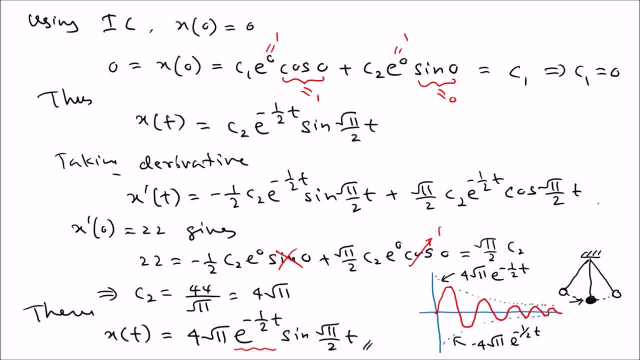 so what's gonna happen because of the air? so what's gonna happen because of the air: resistance, resistance, resistance. the uh, it's gonna slow down. so that the uh, it's gonna slow down. so that the uh, it's gonna slow down. so that means, if you look at the 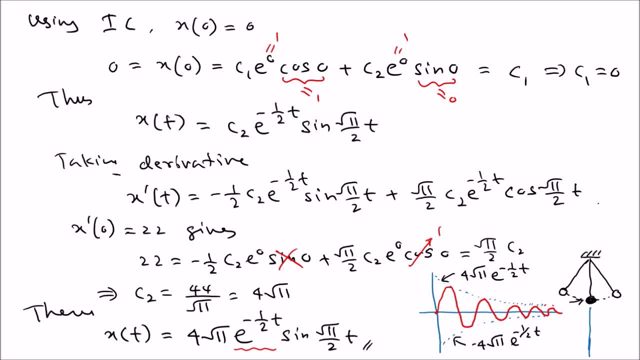 means. if you look at the means, if you look at the graph of this one, if you graph, it is graph of this one. if you graph, it is graph of this one. if you graph, it is exactly what you get. start here. it's exactly what you get. start here. it's. 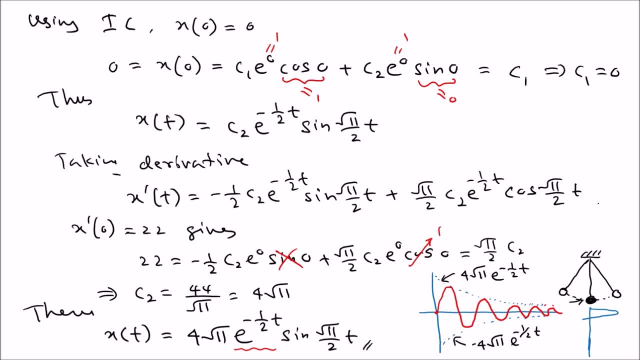 exactly what you get. start here: it's gonna get a sudden, gonna get a sudden, gonna get a sudden jump because the impulse, and then it's jump because the impulse, and then it's jump because the impulse, and then it's gonna slow down, gonna slow down, gonna slow down. i'm gonna go and stop like that. so 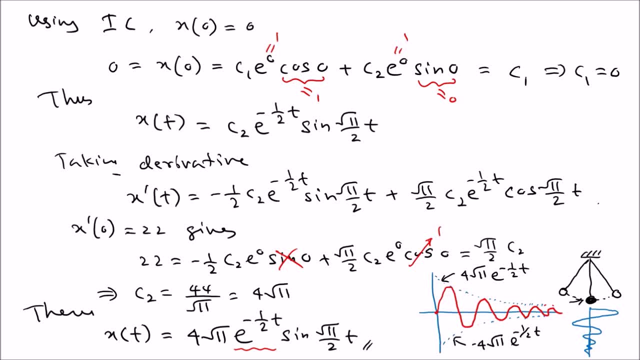 i'm gonna go and stop like that. so i'm gonna go and stop like that. so that's the situation. so this is uh the. that's the situation. so this is uh the. that's the situation. so this is uh the solution you you get using uh. 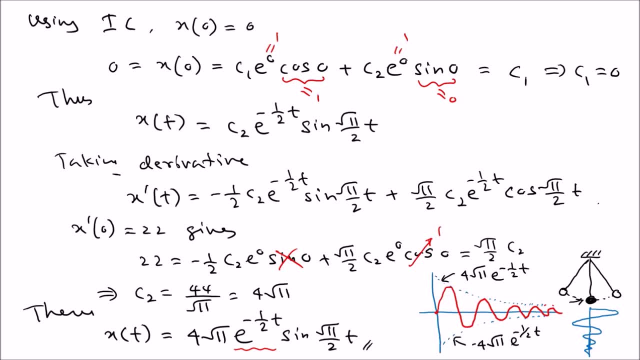 solution. you you get using uh solution. you you get using uh differential equations. that's a kind of differential equations. that's a kind of differential equations. that's a kind of nice, nice, nice idea. okay, so that's about the constant idea. okay, so that's about the constant. 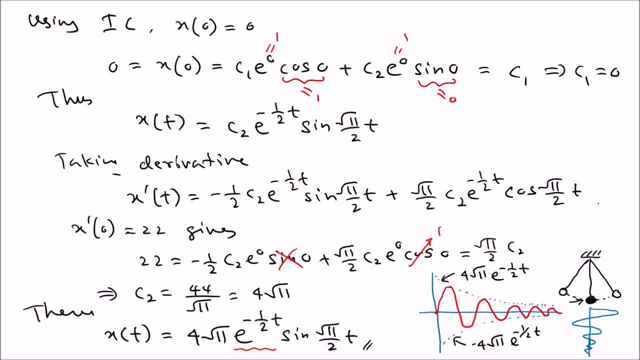 idea. okay, so that's about the constant coefficient differential equations, coefficient differential equations, coefficient differential equations and how to solve it. there are three cases and how to solve it. there are three cases and how to solve it. there are three cases and we talk about those three cases. 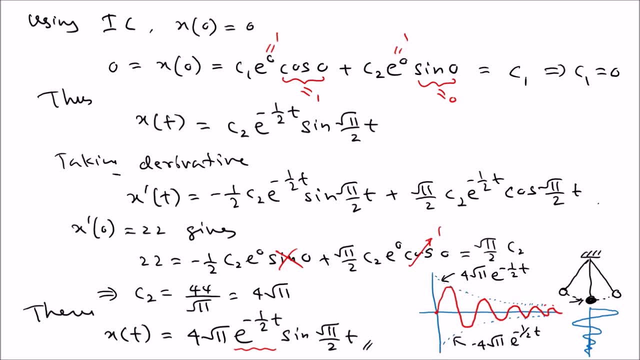 and we talk about those three cases. and we talk about those three cases: uh in the next. we can talk about uh in the next, we can talk about uh in the next, we can talk about another special case, another special case, another special case, what we call the kochi euler. 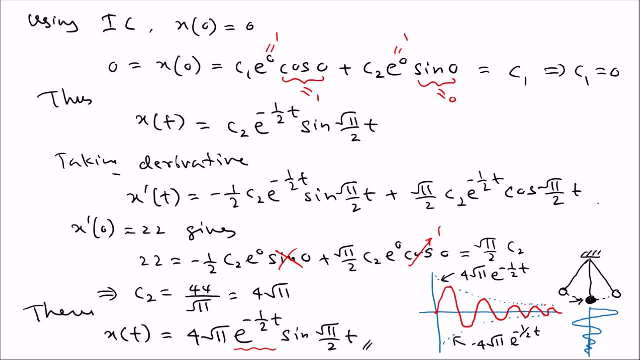 what we call the kochi euler, what we call the kochi euler differential equation. so in this, let's learn how to um, how to. so in this, let's learn how to um, how to. so in this, let's learn how to um, how to solve the kochi. 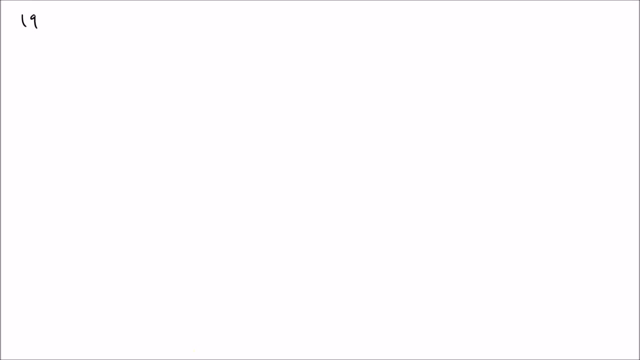 solve the kochi. solve the kochi euler differential equation. so this is euler differential equation. so this is euler differential equation. so this is number 19, number 19, number 19: kochi euler. kochi euler a differential equation- some people. kochi euler, a differential equation, some people. 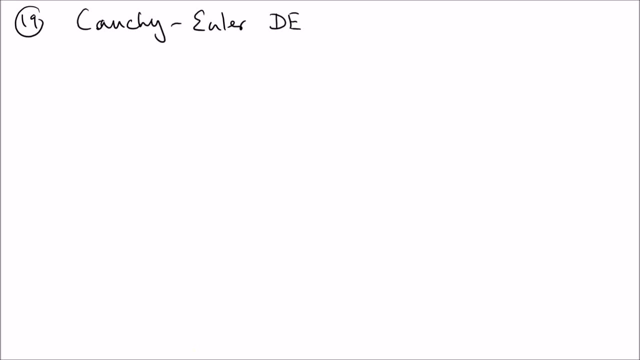 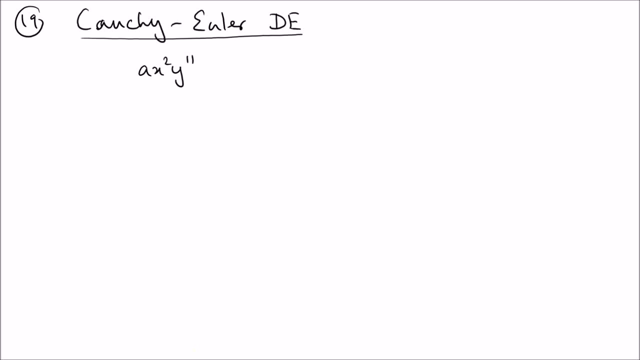 so a kochi euler equation has this form. so a kochi euler equation has this form. so it's a x squared y double prime. so it's a x squared y double prime. so it's a x squared y double prime plus b. x y prime plus c. 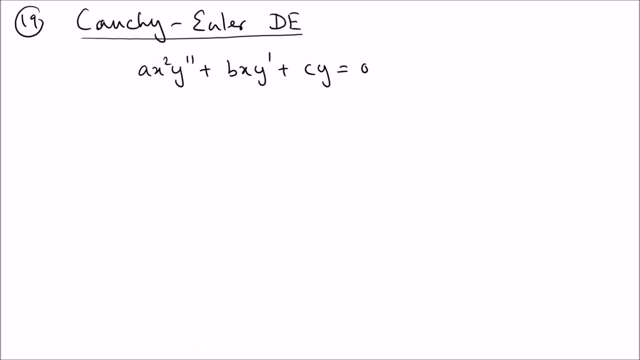 plus b x y prime, plus c, plus b- x y prime, plus c- y equals zero. so that's the format. it's y equals zero. so that's the format. it's y equals zero. so that's the format. it's also second order, also second order, also second order. homogeneous differential equation and also: 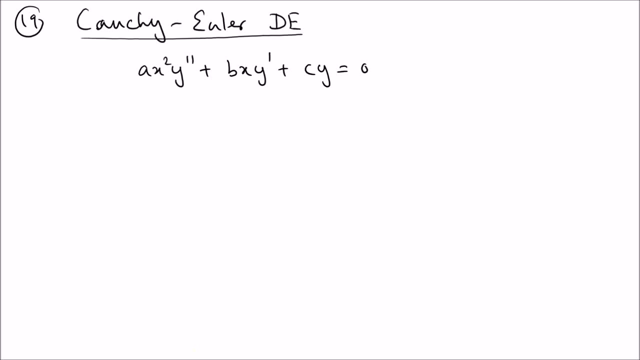 homogeneous differential equation and also homogeneous differential equation and also linear equation. because b- linear equation, because b- linear equation, because b- x is the independent variable, x is the independent variable, x is the independent variable. so that means this is still so, that means this is still so, that means this is still linear. so how to solve it? we can. 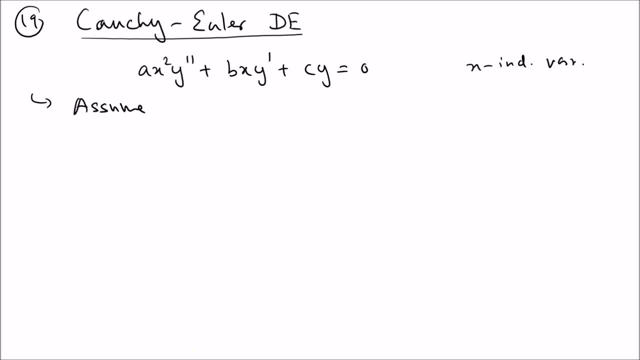 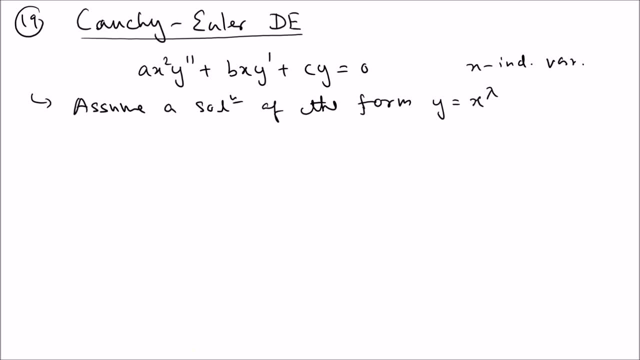 y equal x to the lambda power, y equal x to the lambda power. and then what you try and do we're going, and then what you try and do we're going, and then what you try and do we're going to uh, to uh to uh. take derivative and plug in there and 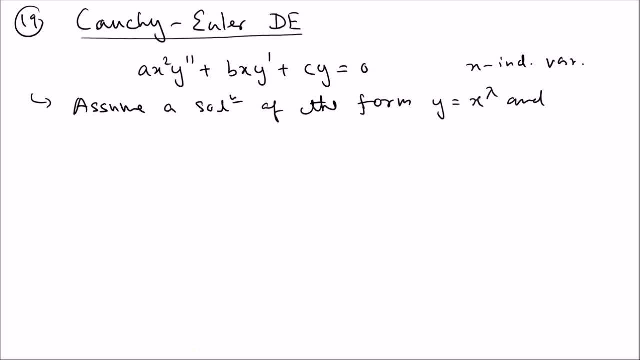 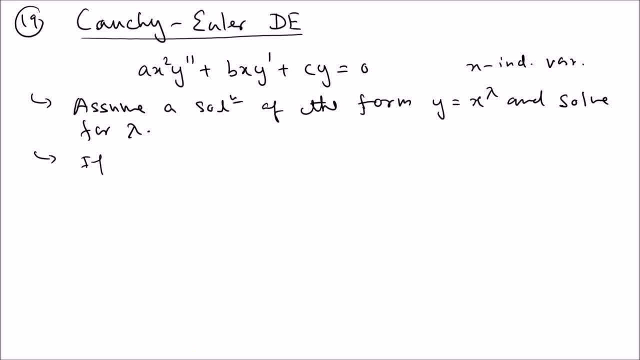 solve for lambda, so that's the kind of idea. solve for lambda, so that's the kind of idea. so, uh, if so, uh, if so, uh, if so. once you do that, what's going to so? once you do that, what's going to so, once you do that, what's going to happen? 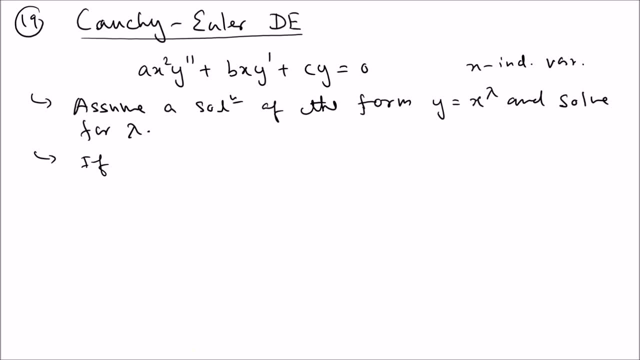 happen, happen. uh, because we're looking for two. uh, because we're looking for two. uh, because we're looking for two. solutions, solutions, solutions. so let's say uh. if they are, so, let's say uh. if they are, so, let's say uh if they are. if they are lambda. 1, which is not equal to. 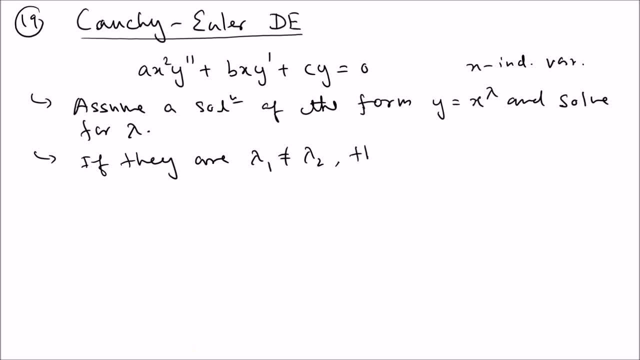 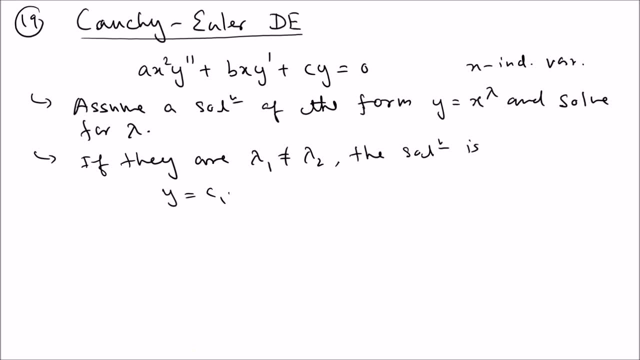 the solution is: simply y equal c1, simply y equal c1, simply y equal c1 x lambda 1 plus c x lambda 1 plus c. x lambda 1 plus c. 2 x lambda 2, so that's the kind of 2 x lambda 2, so that's the kind of. 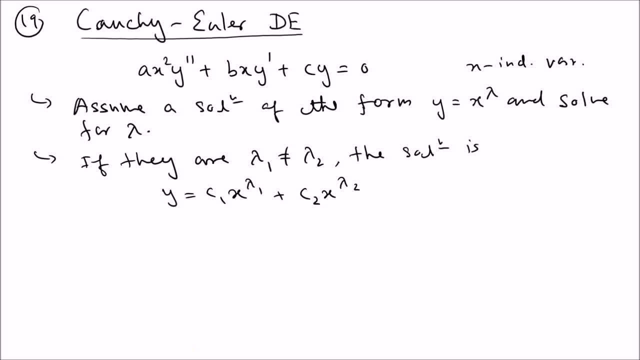 2 x lambda 2. so that's the kind of idea, idea, idea. so let's look at the problem and see. so let's look at the problem and see. so let's look at the problem and see how it works, how it works, how it works, uh. so example: 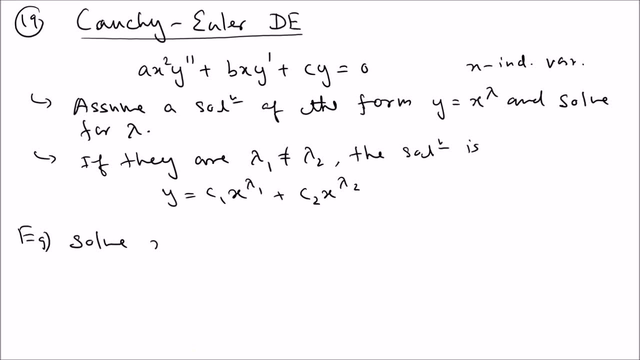 so example. so example: sol sol, sol, sol sol sol x. double prime x squared y. double x. double prime x squared y. double x. double prime x squared y. double prime minus 3 prime minus 3 prime minus 3 x y prime minus 5 y x y prime minus 5 y. 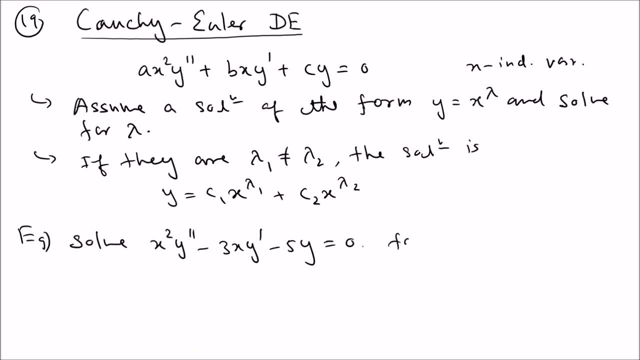 x y prime minus 5 y equals 0. uh for equals 0. uh for equals 0. uh for x positive. let's say x positive, x positive. let's say x positive, x positive. let's say x positive. so how we, how it works, so we're going. 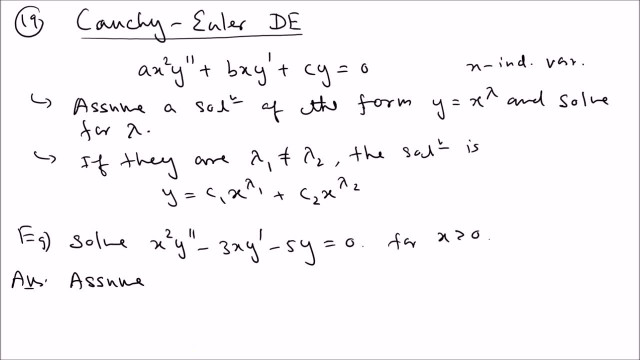 so how we how it works, so we're going so how we how it works, so we're going to assume a solution, to assume a solution, to assume a solution. so assume, uh, a solution, uh, a solution, uh, a solution. assume a solution of the form, of the form. 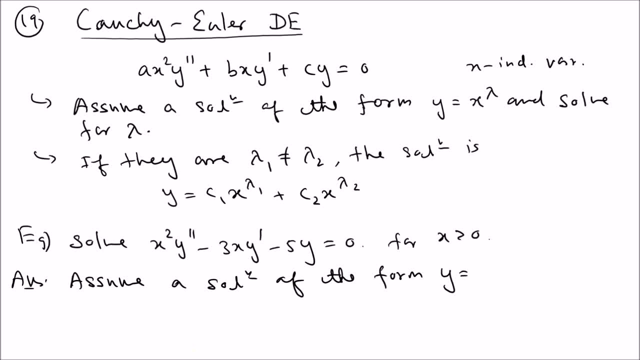 of the form: y equal x lambda, y equal x lambda, y equal x lambda. then what happened then? what happened then? what happened? we take the derivative so y prime. we take the derivative so y prime. we take the derivative so y prime, which is, uh, if you take the derivatives. 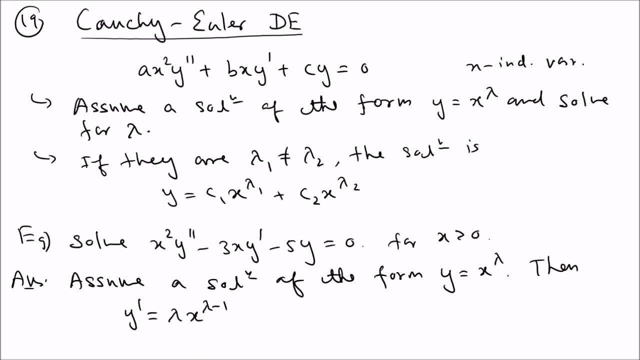 which is uh. if you take the derivatives, which is uh. if you take the derivatives lambda x- lambda x, lambda x- lambda minus 1, just by the power rule. lambda x- lambda minus 1, just by the power rule. lambda x- lambda minus 1, just by the power rule. and then y, double prime, we take one. 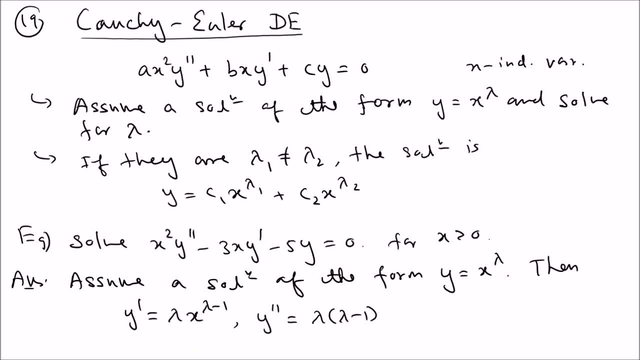 and then y double prime, we take one, and then y double prime, we take one more. so it is lambda, more so it is lambda, more so it is lambda. lambda minus 1 x to the lambda minus 2. lambda minus 1 x to the lambda minus 2. 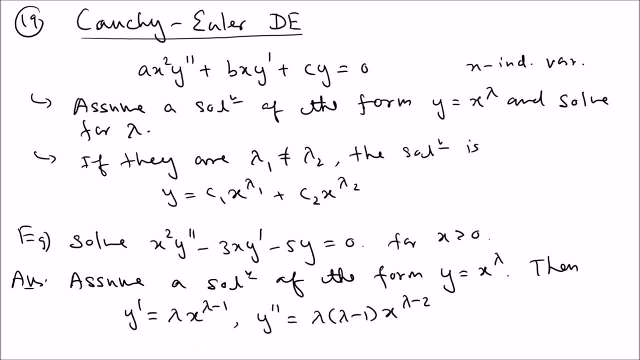 lambda minus 1 x to the lambda minus 2. now, what we're going to do? we're going now what we're going to do. we're going now what we're going to do. we're going to substitute that, to substitute that, to substitute that. okay, so we substitute that. 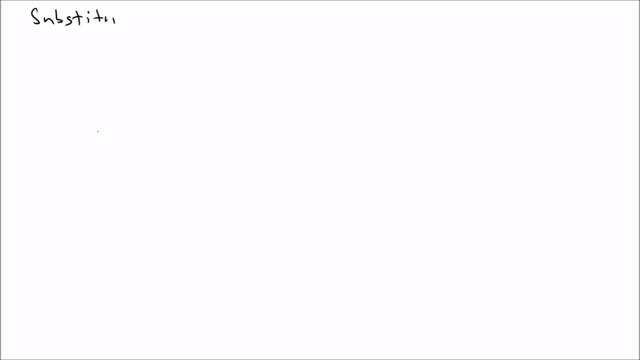 substitute. so once you substitute what happened. so once you substitute what happened. so once you substitute what happened, you have x squared, and then y prime y, you have x squared, and then y prime y, you have x squared, and then y prime y, double prime, which is lambda. 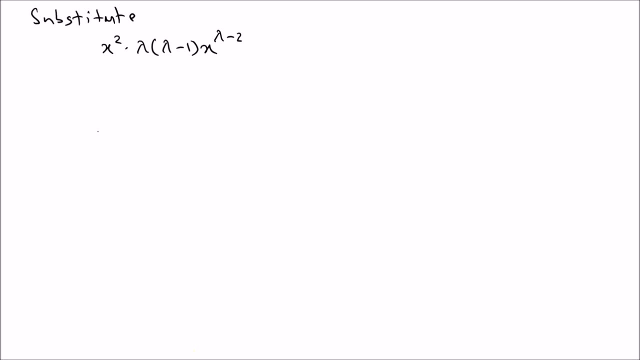 double prime which is lambda. double prime which is lambda. lambda minus 1 x lambda minus 2. lambda minus 1 x. lambda minus 2. lambda minus 1 x. lambda minus 2 minus 3 x. minus 3 x minus 3 x. uh, lambda prime term y, prime term which. 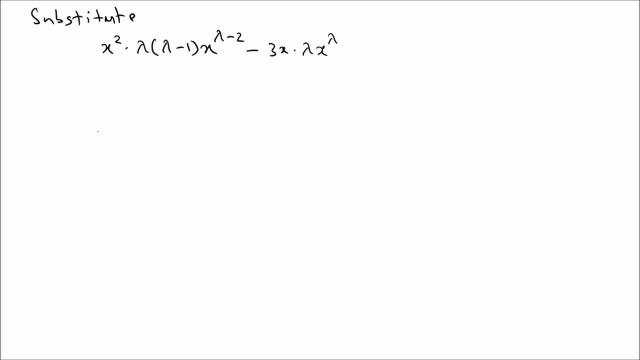 uh lambda prime term, y prime term which uh lambda prime term, y prime term which is x, is x is x, and a lambda x lambda and a lambda x lambda and a lambda x lambda minus 1, minus 1. minus 1 and then minus 5, y term. 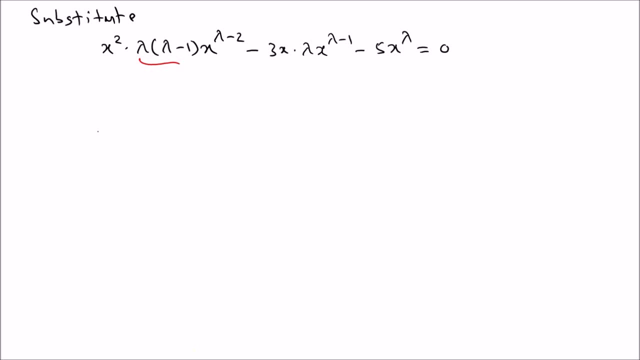 and then minus 5 y term, and then minus 5 y term. so those are the three terms. so again, so. so, those are the three terms, so again, so. so those are the three terms. so again. so this is the y double prime term. this is the y double prime term. 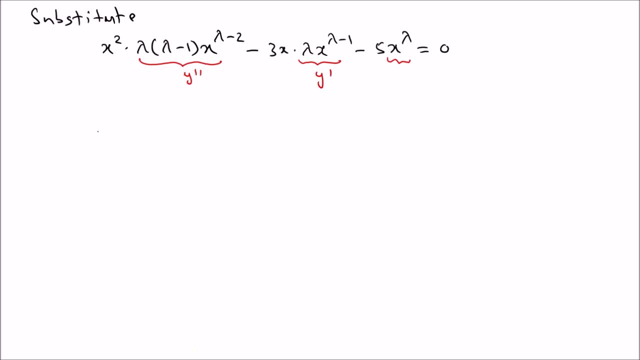 this is the y double prime term, this is y prime term. this is y prime term, this is y prime term and this is the y term. so those are three and this is the y term. so those are three and this is the y term. so those are three terms. 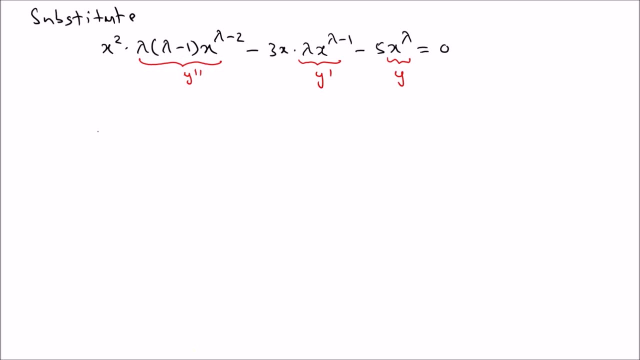 terms, terms, and you can see that, uh, you can simplify. and you can see that, uh, you can simplify. and you can see that, uh, you can simplify this. you get x to the lambda in each this. you get x to the lambda in each this. you get x to the lambda in each term. so we can take it out, so you're. 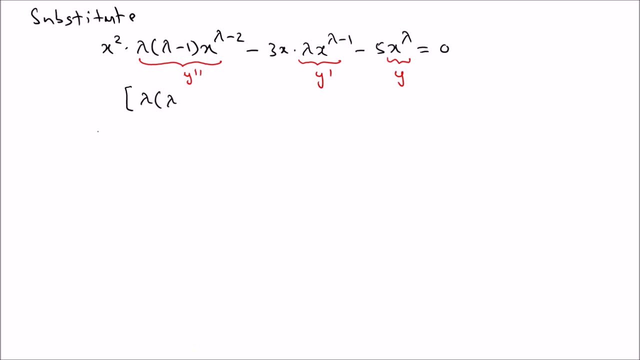 term, so we can take it out. so you're term, so we can take it out. so you're gonna get gonna get. gonna get a lambda times lambda minus one. a lambda times lambda minus one. a lambda times lambda minus one minus three. lambda minus five minus three. lambda minus five. 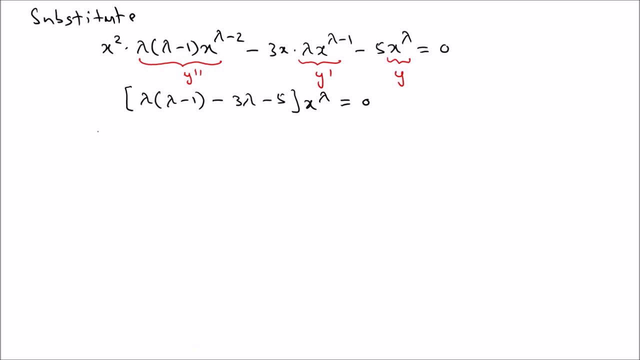 minus three lambda minus five. x to the lambda equals zero. x to the lambda equals zero. x to the lambda equals zero, but we know that x to the lambda is, but we know that x to the lambda is, but we know that x to the lambda is never zero. 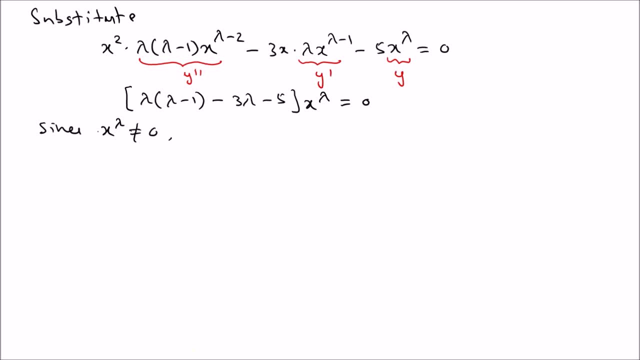 because x not equals zero, so that means because x not equals zero, so that means because x not equals zero, so that means only thing should happen, is only thing should happen, is only thing should happen is the whatever inside the bracket has to, the whatever inside the bracket has to. 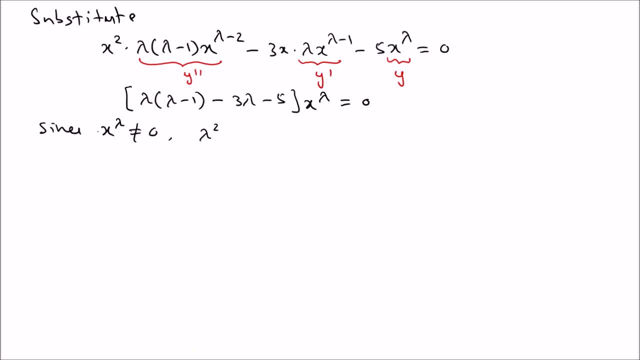 the whatever inside the bracket has to be zero. but you can see if you simplify, be zero. but you can see if you simplify, be zero. but you can see if you simplify that you're going to get lambda squared, that you're going to get lambda squared, that you're going to get lambda squared. you get minus, lambda minus or minus four. 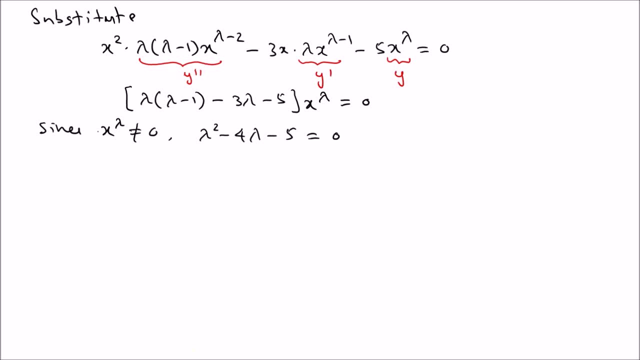 you get minus, lambda, minus or minus four. you get minus, lambda, minus or minus four, lambda, lambda, lambda. minus five, equal to zero. that's what you minus five, equal to zero. that's what you minus five, equal to zero. that's what you get, get, get. so this is very easy to solve. so we're. 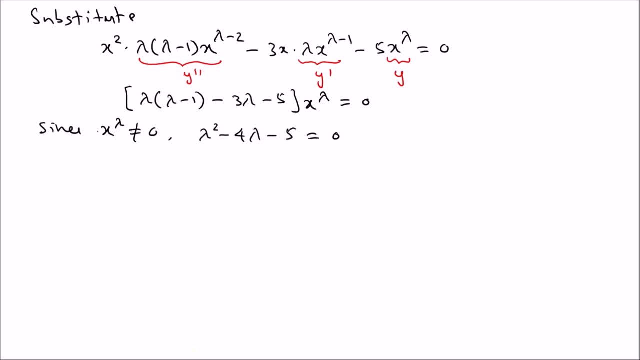 so this is very easy to solve, so we're so this is very easy to solve, so we're gonna uh look at the factors uh, so what are the factors? uh, you can see uh, so what are the factors? uh, you can see uh, so what are the factors? uh, you can see lambda minus five and lambda plus one. 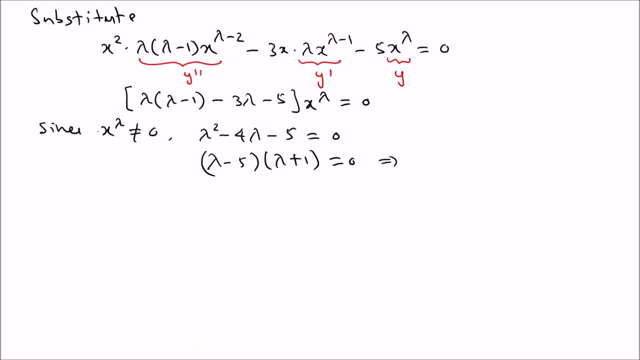 lambda minus five and lambda plus one. lambda minus five and lambda plus one. other factors, other factors, other factors. so this can give you a lambda equal. so this can give you a lambda equal. so this can give you a lambda equal minus one, minus one, minus one and five. so the general solution: 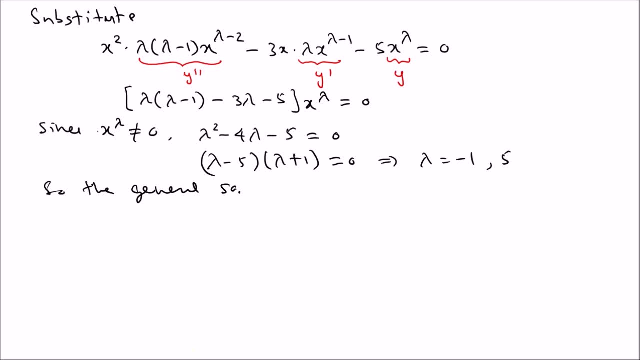 and five so the general solution and five so the general solution. so so so general solution is general solution is general solution. is: y equal c 1 x to the lambda 1. y equal c 1 x to the lambda 1. y equal c 1 x to the lambda 1 x. lambda 1, not x. 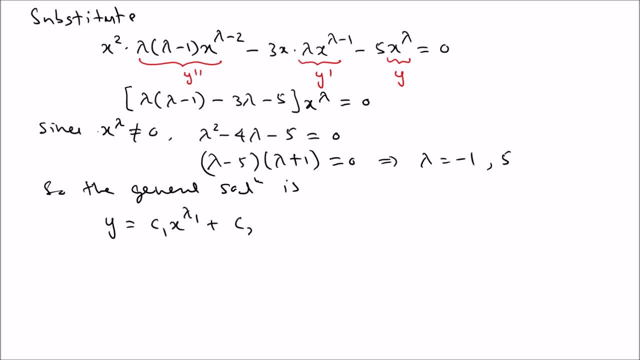 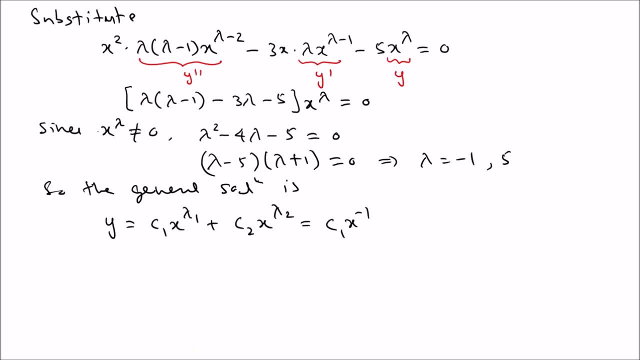 plus c 2 x to the lambda 2. so we're going to plug in that. so the c. so we're going to plug in that. so the c. so we're going to plug in that. so the c 1 x to the minus 1. 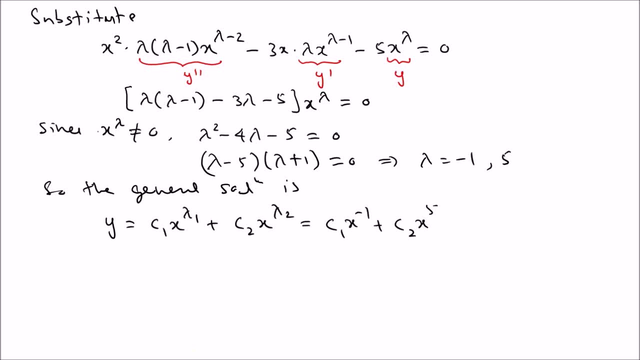 1 x to the minus 1. 1 x to the minus 1 plus c. 2 x to the phi plus c. 2 x to the phi plus c. 2 x to the phi. if you rewrite it um, we bring x down. if you rewrite it um, we bring x down. 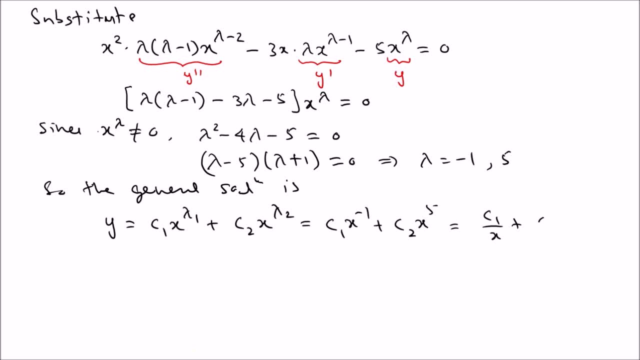 if you rewrite it, um, we bring x down. so you can write this one as c 1 over x. so you can write this one as c 1 over x. so you can write this one as c 1 over x, plus c 2 x to the phi, this is 4x. 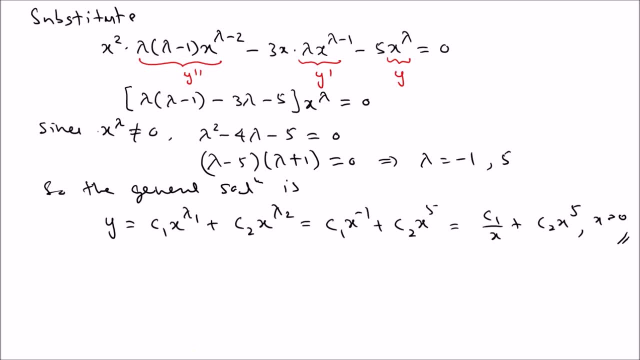 plus c 2 x to the phi: this is 4x. plus c 2 x to the phi: this is 4x. pass it good. so that's the solution. so pass it good. so that's the solution. so pass it good. so that's the solution. so it's not that difficult. 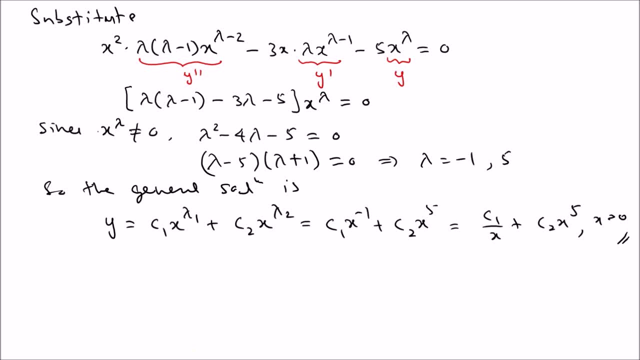 it's not that difficult. it's not that difficult. uh, so you solve for we assume our uh, so you solve for we assume our uh, so you solve, for we assume our solution of x to the lambda. solution of x to the lambda. solution of x to the lambda. take derivation plug-in: solve for lambda. 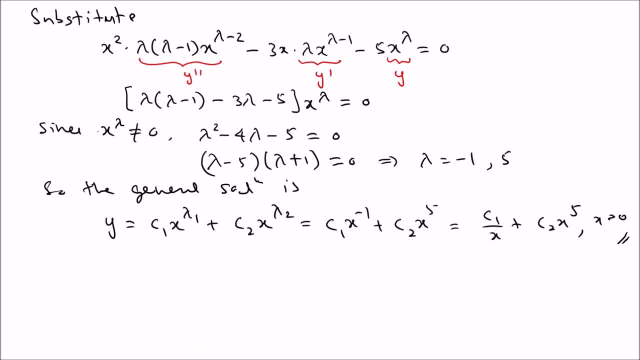 take derivation plug-in: solve for lambda. take derivation plug-in: solve for lambda. so let's discuss another method. what we so, let's discuss another method. what we so, let's discuss another method. what we trying to do here is we can transform. trying to do here is we can transform. 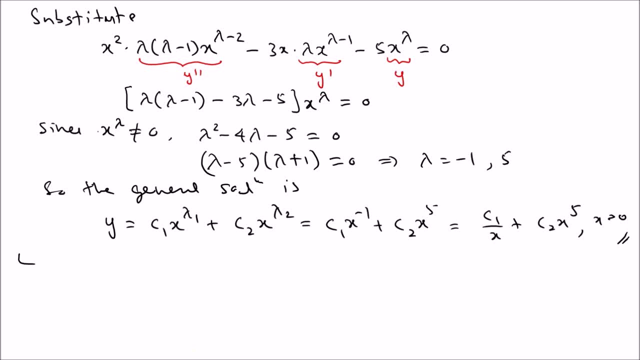 trying to do here is: we can transform the problem to another domain, another, the problem to another domain, another, the problem to another domain, another variable, so another method, another method, so we can transform the problem. another method, so we can transform the problem, another method, so we can transform the problem. uh, so let's say for: 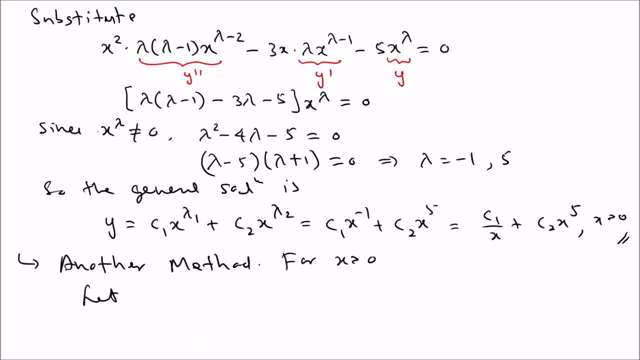 uh. so let's say for uh. so let's say for x positive what we're going to do, we x positive what we're going to do, we x positive what we're going to do, we can let, can, let, can let. x equal e to the t. 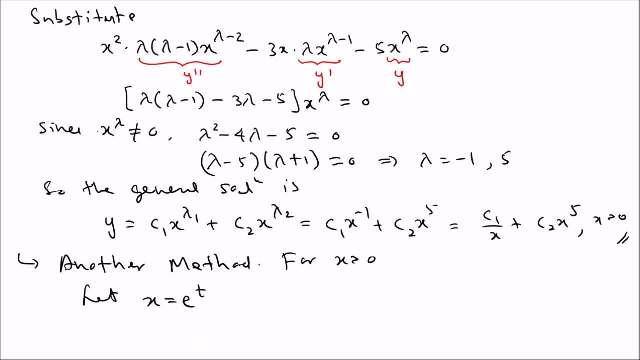 x equal e to the t. x equal e to the t. so we can transform the problem to the. so we can transform the problem to the. so we can transform the problem to the t variable. t variable, t variable, uh, uh, uh. now what's going to happen? you can show. now what's going to happen. you can show now what's going to happen. you can show that. so i'm going to skip that. so i'm going to skip that. so i'm going to skip that. the how it works, you can look at that. the how it works, you can look at. 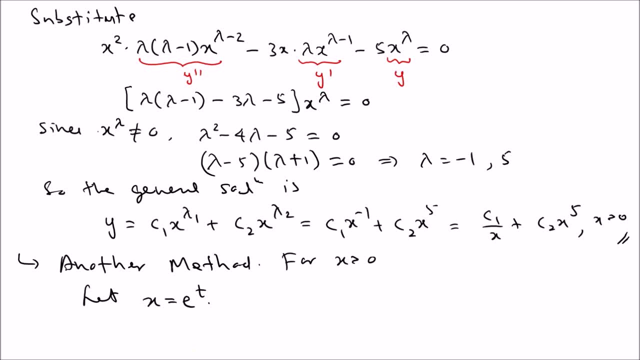 that the how it works. you can look at the video general video for that. the video general video for that. the video general video for that. uh, so then, what happened once you do uh? so then, what happened once you do uh? so then, what happened once you do that, you can transform the variable x to: 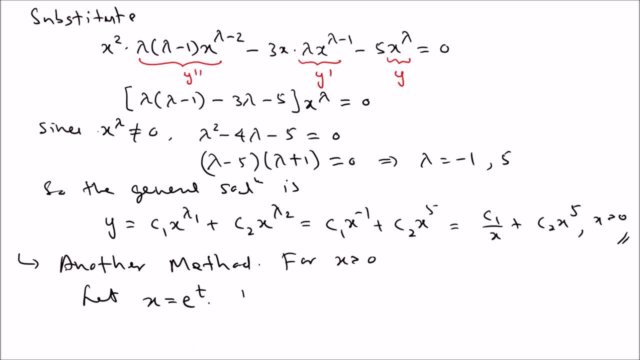 that you can transform the variable x to that you can transform the variable x to t variable. okay, so what happened now in t variable? okay, so what happened now in t variable? okay, so what happened now in variable t? in variable t: the differential equation. in variable t: the differential equation. 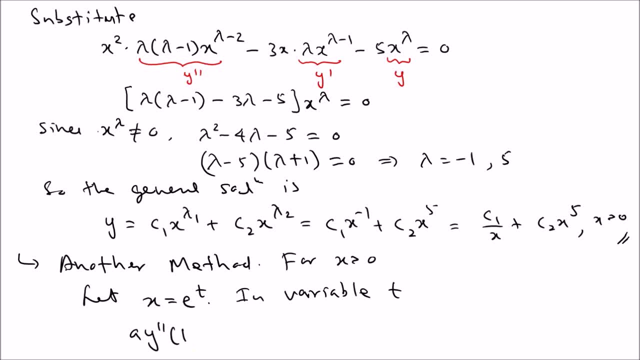 in variable t, the differential equation becomes: becomes: becomes: a y double prime t: a y double prime t. a y double prime t. plus b minus a, plus b. minus a. plus b minus a y prime: again the variable t. plus b. minus a y prime: again the variable t. 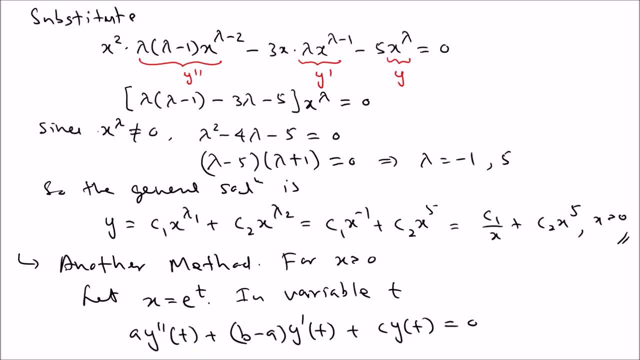 plus b minus a y prime. again the variable t plus c plus c plus c, y t equals zero. you can see that this is y t equals zero. you can see that this is y t equals zero. you can see that this is a constant coefficient differential. a constant coefficient differential. 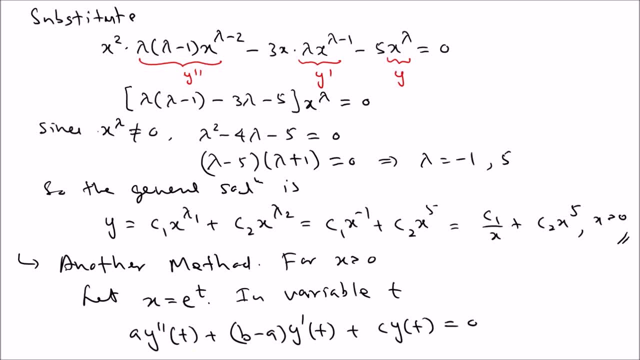 a constant coefficient differential equation, and we know how to solve this equation, and we know how to solve this equation, and we know how to solve this. uh, so that's the idea. so we transform. uh, so that's the idea, so we transform. uh, so that's the idea. so we transform the euler coach equation to a constant. 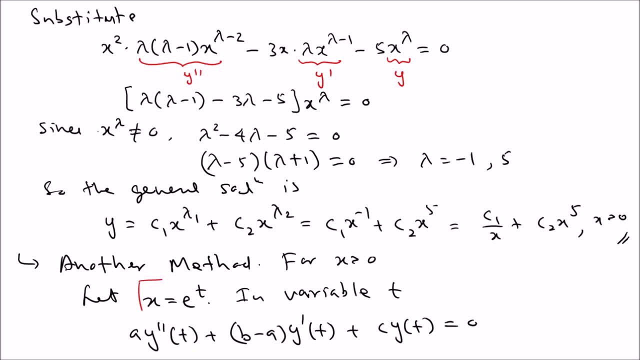 the euler coach equation to a constant. the euler coach equation to a constant: coefficient differential equation, coefficient differential equation, coefficient differential equation by this special transformation, uh, so by this special transformation, uh, so by this special transformation, uh. so this is for x, this is for x, this is for x positive. if we x negative, we can say x. 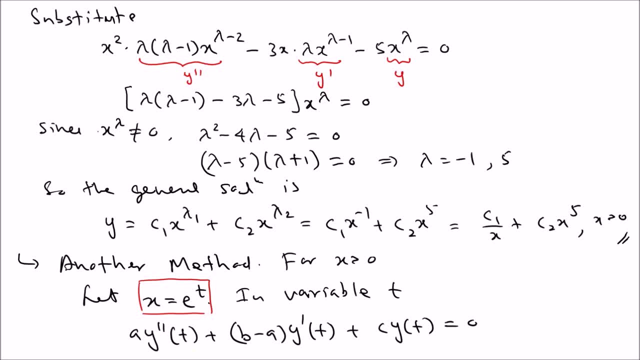 positive. if we x negative, we can say x positive. if we x negative, we can say x. equals negative. e to the t equals negative e to the t. equals negative e to the t. the interesting thing is you get the. the interesting thing is you get the. the interesting thing is you get the exact same equation even in that case. 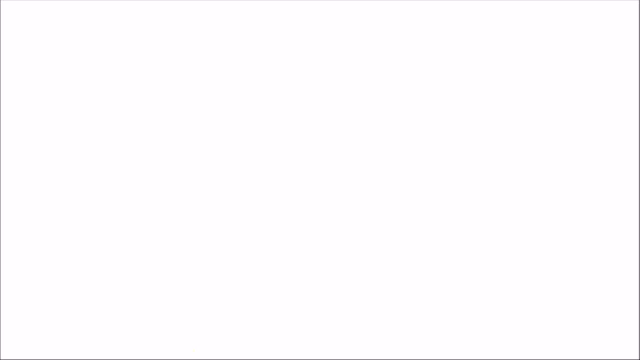 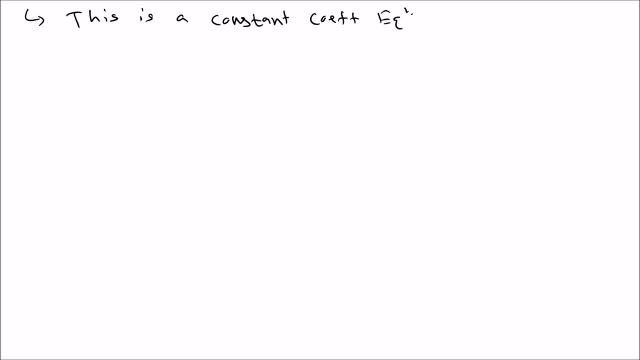 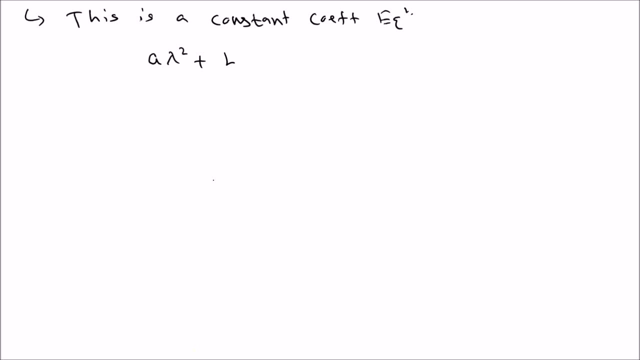 so we can look at the characteristic equation a lambda squared plus b. equation a lambda squared plus b. equation a lambda squared plus b. minus a lambda plus c. minus a lambda plus c. minus a lambda plus c. equals here. that's what you get so. equals here, that's what you get so. 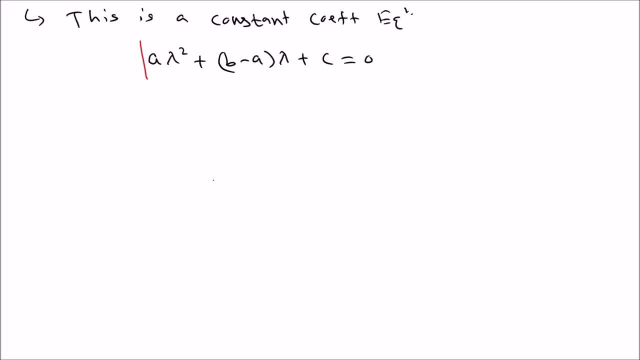 equals here. that's what you get. so that's the, that's the, that's the characteristic equation for the coach. characteristic equation for the coach. characteristic equation for the coach: euler under the new transformation. euler under the new transformation. euler under the new transformation. now, if you know these values, then we. 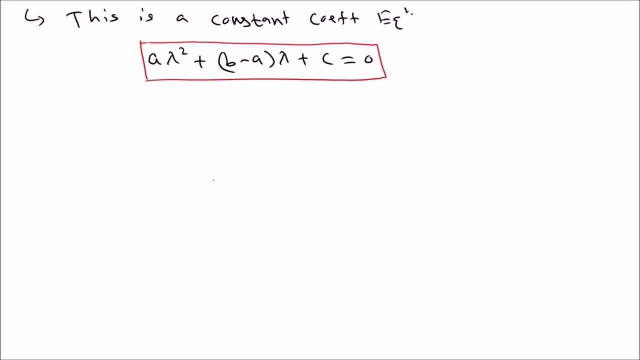 now, if you know these values, then we now. if you know these values, then we know the um, know the um, know the um, the solutions because in in the t variable, the solutions because in in the t variable, the solutions because in in the t variable. what you want to do is you can. 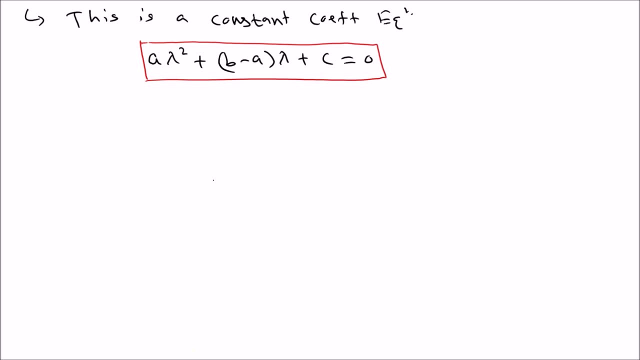 what you want to do is you can. what you want to do is you can transform the variable back, transform the variable back, transform the variable back. so ah, so this is the characteristic, so ah, so this is the characteristic, so ah, so this is the characteristic equation, and you can see, this is: 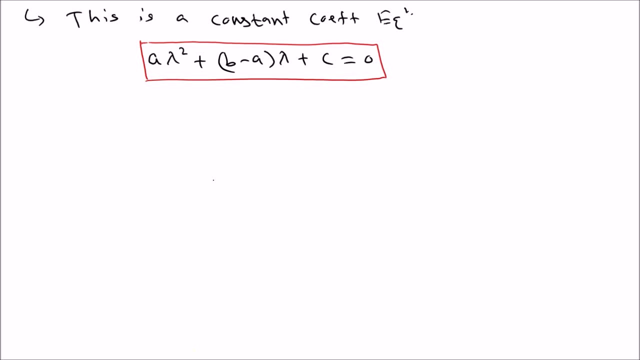 equation and you can see this is equation and you can see this is quadratic in lambda, quadratic in lambda, quadratic in lambda, ah. so so this is quadratic in lambda. again, this is quadratic in lambda. that means ah, ah, ah. there are two solutions. there are two solutions. there are two solutions. okay, so let's talk about the uh. 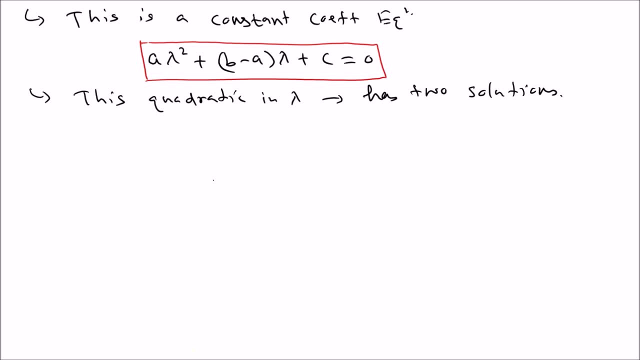 okay, so let's talk about the uh. okay, so let's talk about the uh- separate cases and also separate cases and also separate cases. and also you can see how the how the transformation. you can see how the how the transformation. you can see how the how the transformation works. 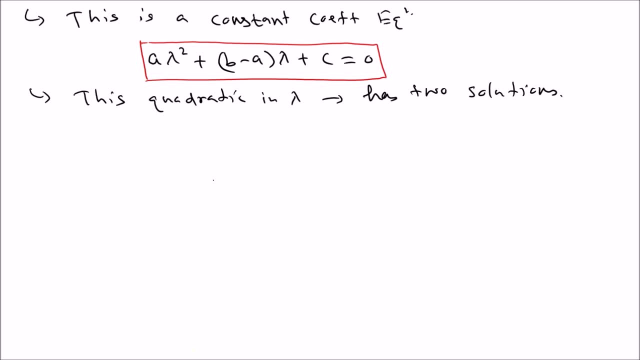 works. works. so we can talk about that. so let's go one by one. if b minus a squared b minus a squared b minus a squared minus 4 ac, that's the minus 4 ac. that's the minus 4 ac. that's the discriminant for this. if it is positive, 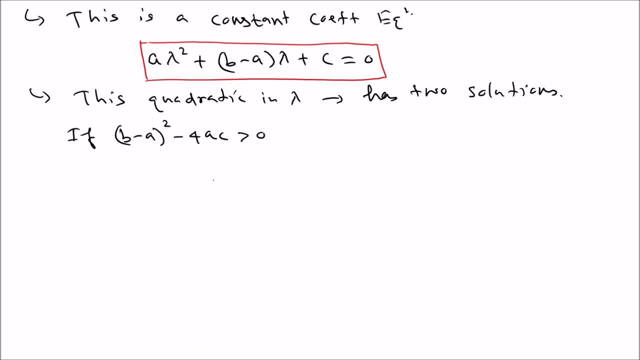 discriminant for this, if it is positive. discriminant for this: if it is positive. there are two solutions. so this have two solutions. so if you call them r1, r2, so this have two solutions. so if you call them r1, r2, so this have two solutions. so if you call them r1, r2, r1 and r2, those are two numbers. 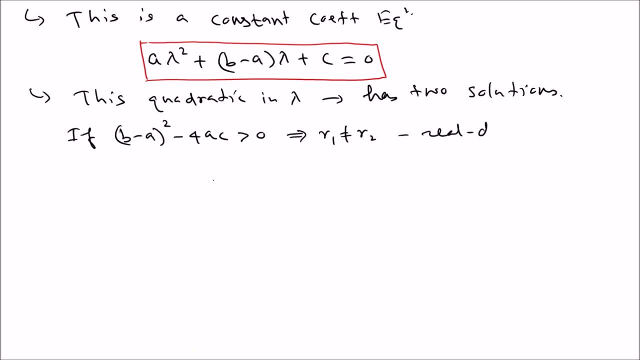 r1 and r2. those are two numbers, r1 and r2, those are two numbers you get. so this is real, you get. so this is real, you get. so this is real. distinct situation. so your solution: y equal. so your solution y equal. so your solution y equal. in the t variable it is c1 e. 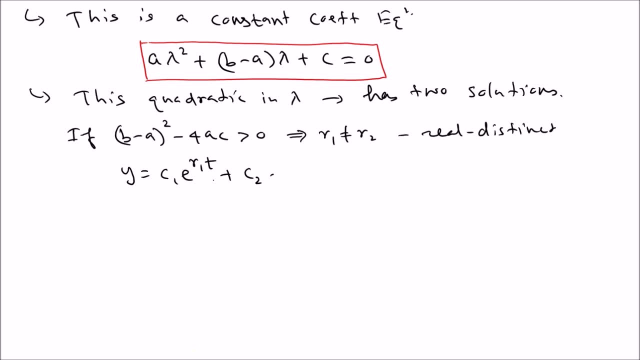 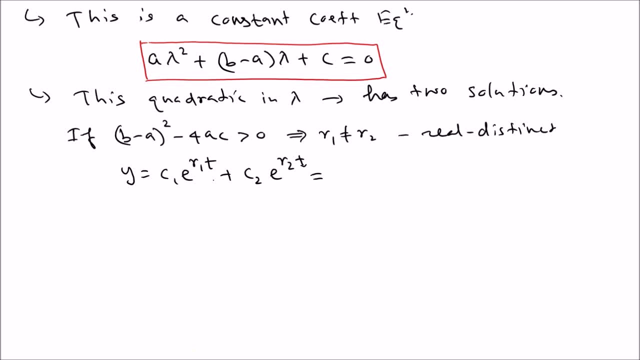 r1 t plus c2 e. r1 t plus c2 e r2 t. now what we're going to do. we r2 t. now what we're going to do. we r2 t. now what we're going to do. we don't transform this. 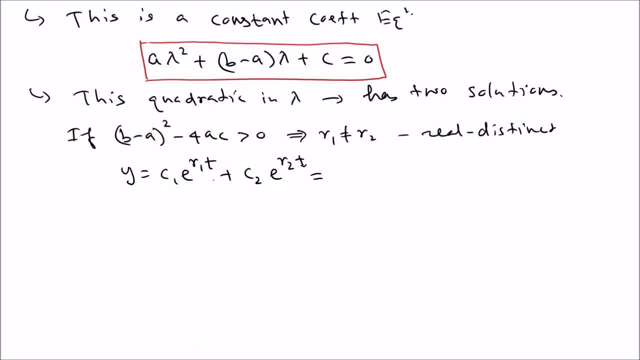 don't transform this, don't transform this to uh x, but we know this to uh x, but we know this to uh x, but we know this transformation in the equivalent transformation, in the equivalent transformation, in the equivalent transformation, transformation, transformation, uh. so what we have? we have x equal. 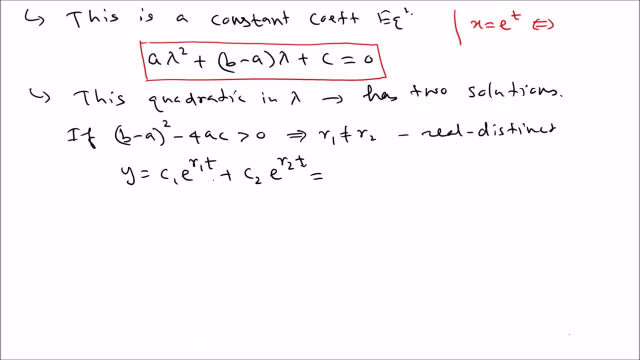 uh. so what we have? we have x equal. uh. so what we have? we have x equal e to the t, if and only if, e to the t, if and only if e to the t, if and only if. t is simply ln x, t is simply ln x. 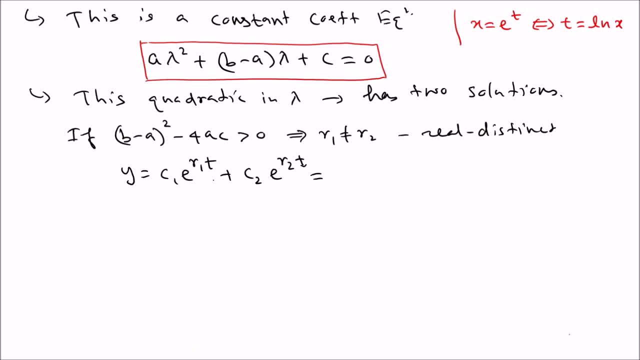 t is simply ln, x. so that's the transformation that we can. so that's the transformation that we can, so that's the transformation that we can use, because use, because use, because e is simply x. so if you replace that, e is simply x. so if you replace that, 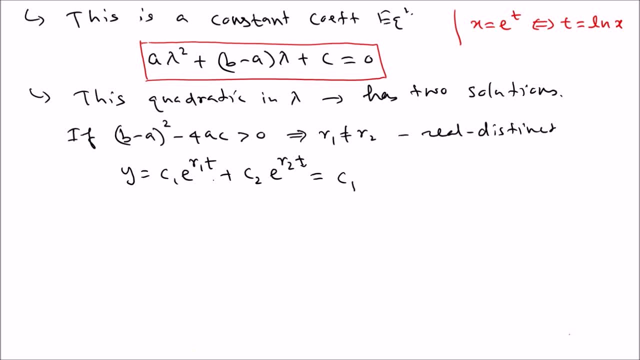 e is simply x. so if you replace that, then this: simply you can write this one, then this: simply you can write this one, then this: simply you can write this one as c1 e to the t is as c1 e to the t is as c1 e to the t is x, so it's become x to the r1. 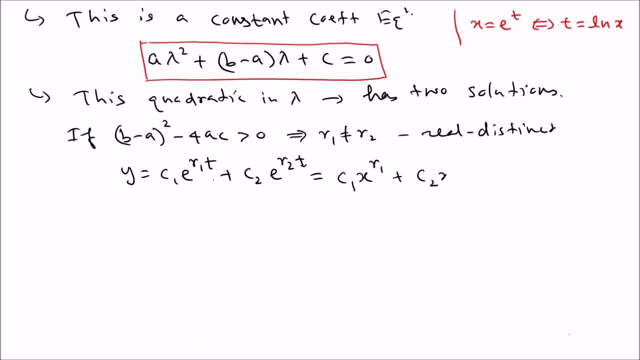 x, so it's become x to the r1. x, so it's become x to the r1. same thing e to the t is x, so this same thing e to the t is x, so this same thing e to the t is x, so this becomes c2. 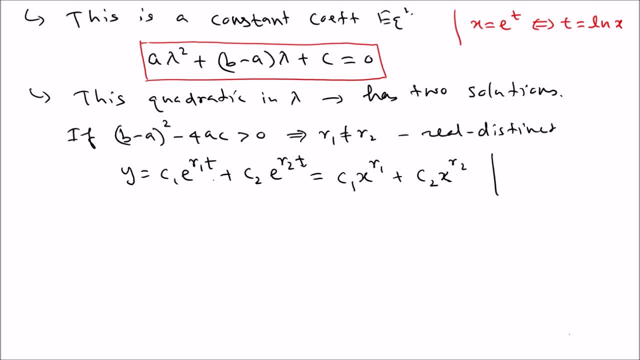 becomes c2, becomes c2. x to the r2. so that's the idea and why x to the r2? so that's the idea and why x to the r2? so that's the idea and why this is algebra. because if you have e, this is algebra, because if you have e, 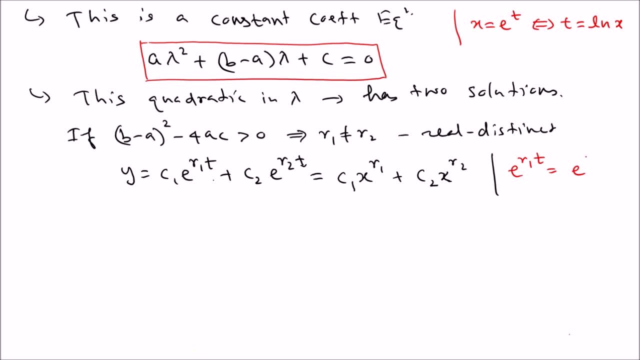 this is algebra, because if you have e r1 t, you can write as e to the t r1 t. you can write as e to the t r1 t. you can write as e to the t r1. that means x r1. so that that's what. 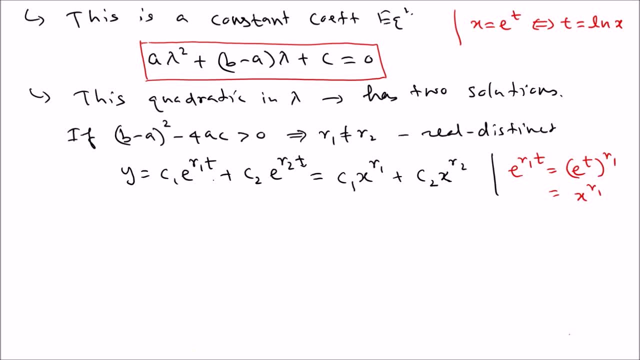 r1, that means x r1, so that that's what r1, that means x r1, so that that's what happened, happened, happened. just basic algebra, so that. so you get just basic algebra, so that. so you get just basic algebra, so that, so you get the solution. 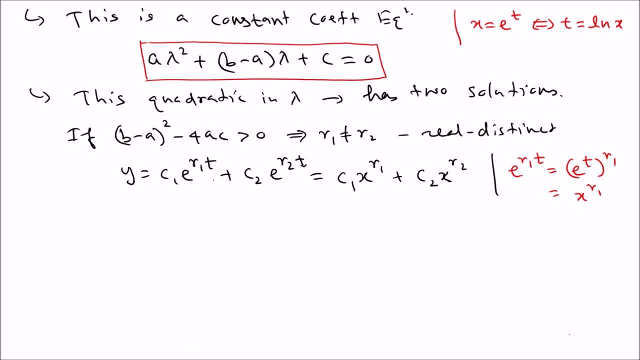 the solution, the solution in x. okay, so that means you. you solve in x. okay, so that means you. you solve in x. okay, so that means you. you solve the new characteristic equation. this is the new characteristic equation. this is the new characteristic equation. this is the characteristic equation for: 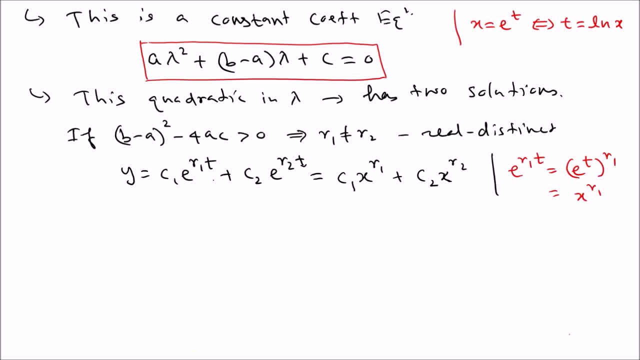 the characteristic equation for the characteristic equation for the uh coach oil equation, and then, after you get that, those, those, and then, after you get that, those, those, and then, after you get that, those, those values, whatever the values, values, whatever the values, values, whatever the values simply going to go, uh here, r1 and as: 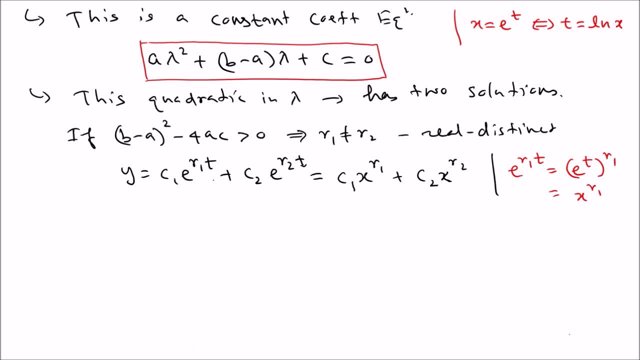 simply going to go uh here, r1 and as simply going to go uh here, r1 and as r1- r2, so very simple. but you have a r1- r2, so very simple. but you have a r1- r2, so very simple. but you have a new characteristic equation. that's the. 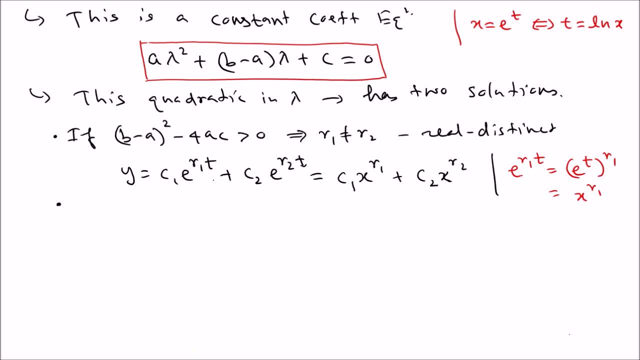 new characteristic equation. that's the new characteristic equation, that's the only thing you remember, only thing you remember, only thing you remember. that's the first case and the second case. that's the first case and the second case. that's the first case and the second case. if 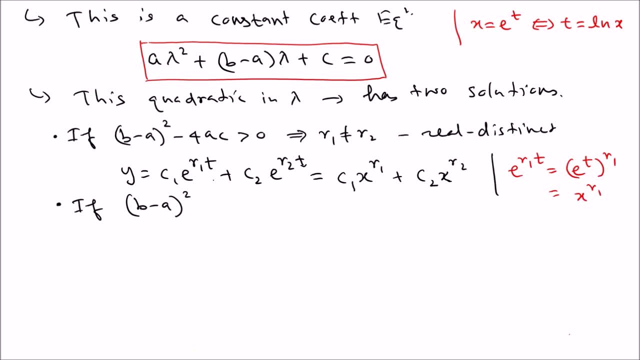 if: if b minus a squared b minus a squared b minus a squared minus four, a c equals zero, uh, what's gonna happen? you're gonna get. uh. uh, what's gonna happen, you're gonna get. uh. uh, what's gonna happen, you're gonna get uh, two equal. 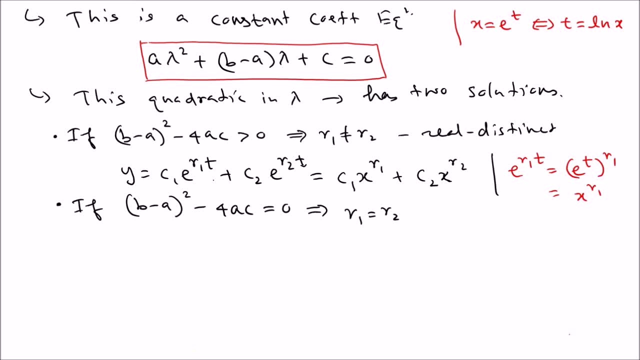 two equal, two equal. so you're going to get r1 equal r2. so you're going to get r1 equal r2. so you're going to get r1 equal r2- a real, a real, a real repeated. in this case, we know how the solution. 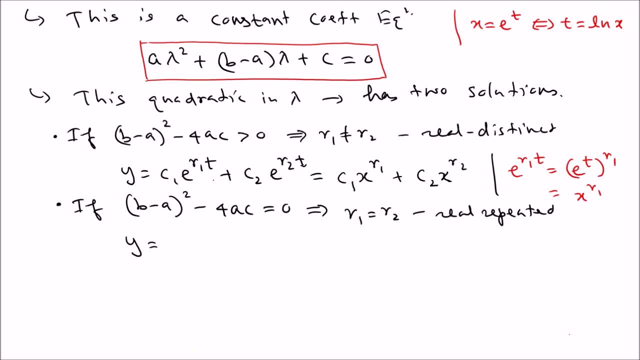 in this case, we know how the solution. in this case, we know how the solution: uh in the t variable, uh in the t variable. uh in the t variable, it has to be uh, it has to be uh, it has to be uh. c1 plus c2 t. 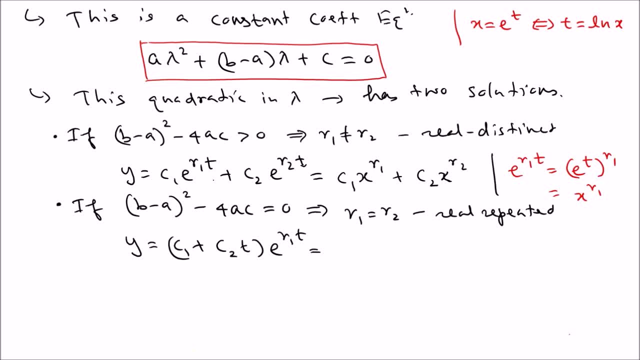 c1 plus c2 t, c1 plus c2 t. e to the r1 t, now again the same e to the r1 t. now again the same e to the r1 t. now again the same argument. argument argument: c1 plus c2, what is t? 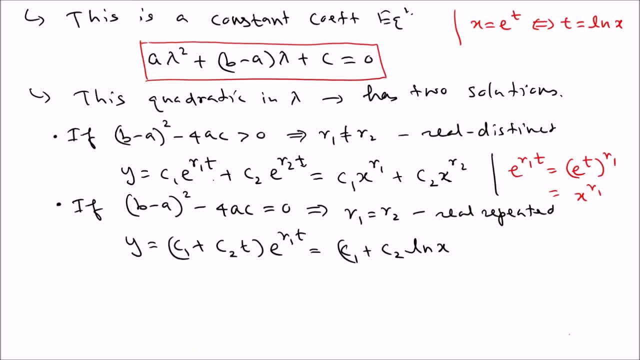 c1 plus c2. what is t? c1 plus c2? what is t? t equal ln x. so now put the ln x- t equal ln x. so now put the ln x- t equal ln x. and then e. this is again as before, and then e. this is again as before. 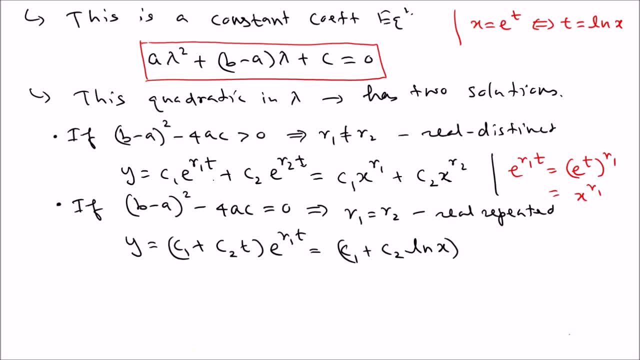 and then e. this is again as before. x to the. this simply become x to the. x to the. this simply become x to the. x to the. this simply become x to the r1, as before. that's the second case and the third case. that's the second case and the third case. 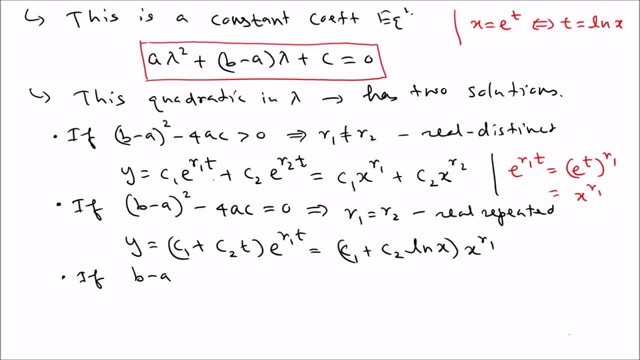 that's the second case. and the third case: if, if, if b minus a squared minus 4ac, if b minus a squared minus 4ac, if b minus a squared minus 4ac, negative, negative, negative, then we have as before. r is, then we have as before, r is. 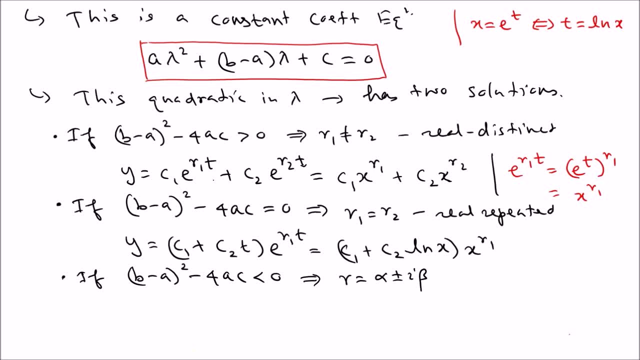 then we have as before: r is complex, so alpha plus or minus, i beta complex. so alpha plus or minus, i beta complex, so alpha plus or minus, i beta. then we can write so as a complex, then we can write so as a complex, then we can write so as a complex conjugate situation. 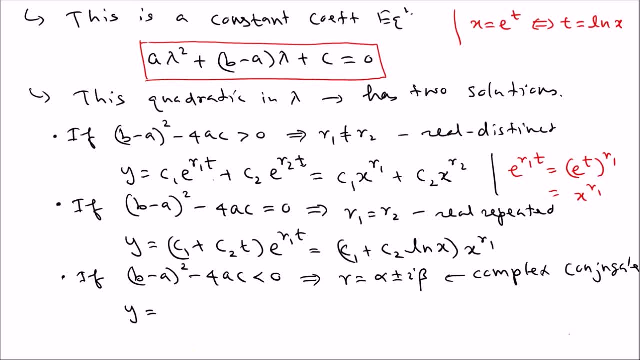 so we can write the solution in the new. so we can write the solution in the new. so we can write the solution in the new t variable, t variable, t variable. so the t variable solution looks like e. so the t variable solution looks like e. so the t variable solution looks like e, alpha t. 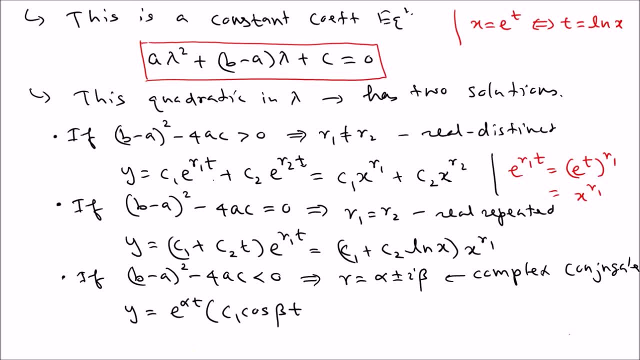 alpha t, alpha t, c1 cosine b, c1 cosine b, c1 cosine b, theta t, theta t, theta t plus c2 sine, plus c2 sine, plus c2 sine, beta t. but what you want to do is you beta t, but what you want to do is you. 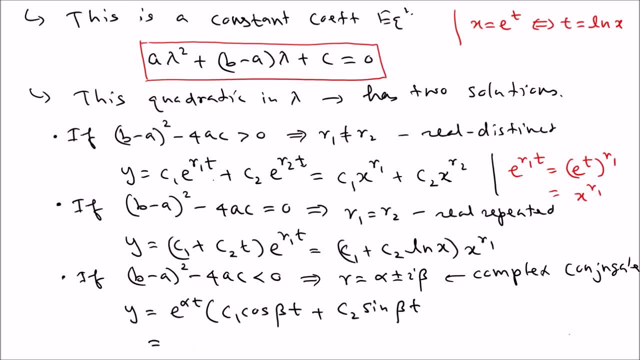 beta t. but what you want to do is, you know, write this one using the know, write this one using the know, write this one using the new variable. so with the new variable, new variable, so with the new variable, new variable, so with the new variable, are you going to get? 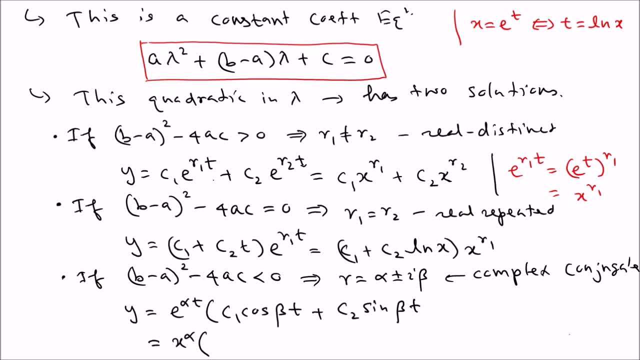 are you going to get? are you going to get? e t is x as x to the alpha as before. e t is x as x to the alpha as before. e t is x as x to the alpha as before. c1 cosine- no change. c1 cosine- no change. 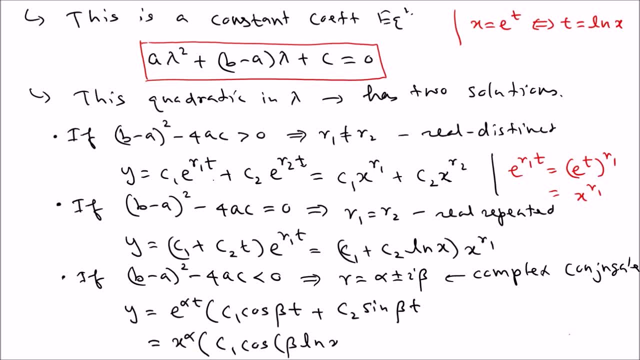 c1 cosine: no change. beta t is l and x- x is positive. so you beta t is l and x- x is positive. so you beta t is l and x- x is positive. so you don't need the absolute sign here. don't need the absolute sign here. 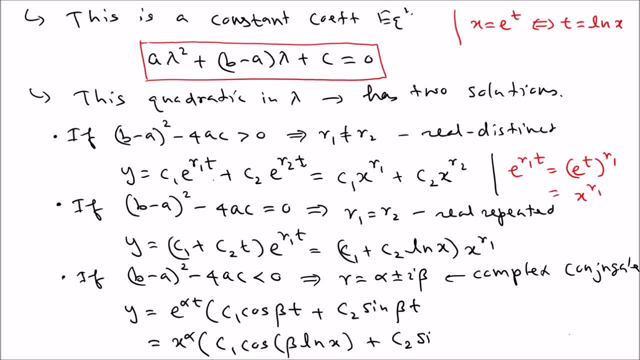 don't need the absolute sign here. plus the same thing: c2. plus the same thing: c2. plus the same thing: c2, sine, sine, sine, beta, beta, beta, ln x, ln x, ln x. so that's the uh. those are three solutions. so that's the uh, those are three solutions. 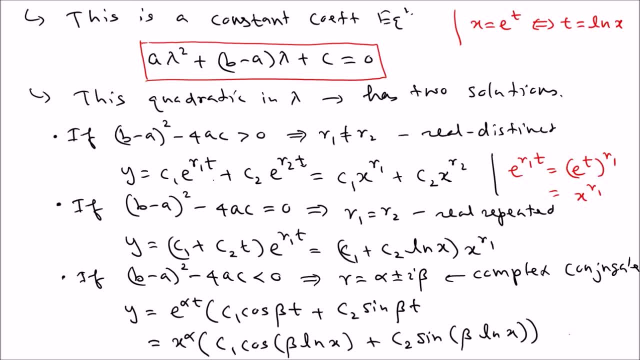 so that's the. uh, those are three solutions. so what do you want to do once you get the? so what do you want to do once you get the? so what do you want to do once you get the? coachwell equation, coachwell equation, coachwell equation. ah, look at the new characteristic. 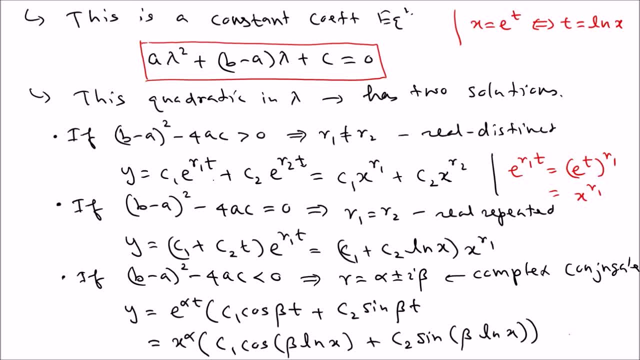 ah. look at the new characteristic ah. look at the new characteristic equation. equation equation: find the values: the lambda values. find the values: the lambda values. find the values, the lambda values: lambda 1, lambda 2. we just call it r because just to remember. we just call it r because just to remember. 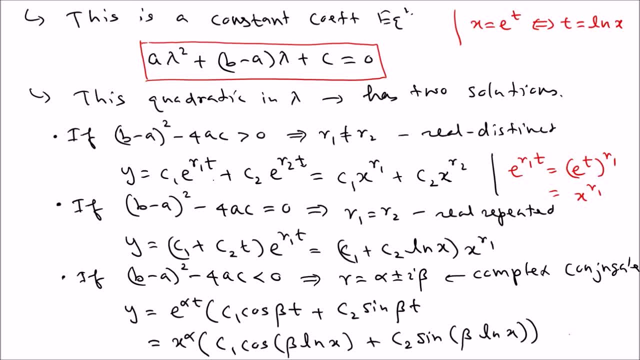 we just call it r, because, just to remember the difference, the difference, the difference, and after you get that, uh, you simply. and after you get that, uh, you simply. and after you get that, uh, you simply get the three solutions. get the three solutions, get the three solutions. okay, so that's the first solution, just. 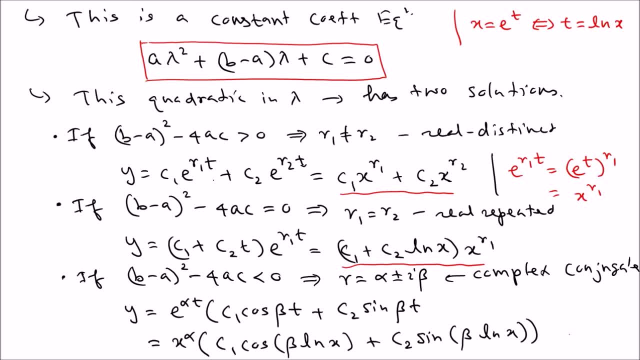 okay, so that's the first solution. just okay, so that's the first solution. just put the new values there, put the new values there, put the new values there, new values there, and the new values in new values there, and the new values in new values there and the new values in the. 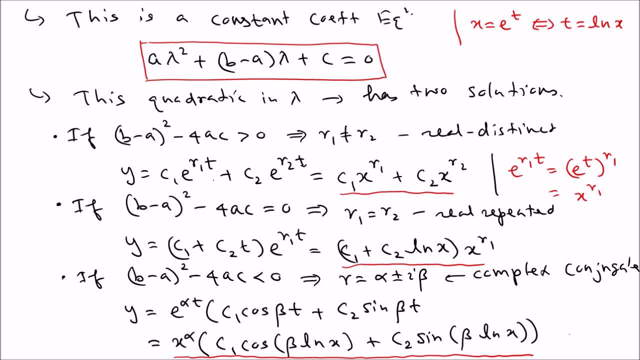 the, the last equation, which is a little long. last equation, which is a little long. last equation, which is a little long: good, so those are three cases. so this is good. so those are three cases. so this is good. so those are three cases. so this is for x, x positive, but we can show that 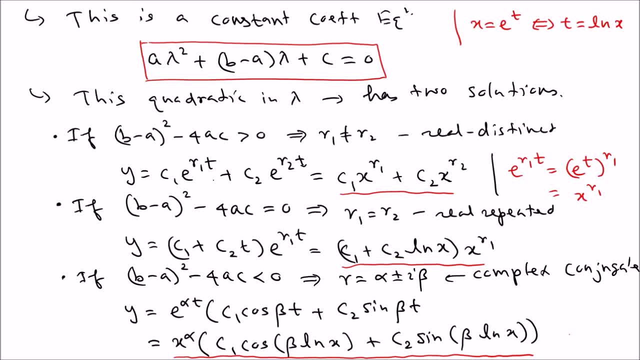 for x, x positive, but we can show that. for x, x positive, but we can show that. so i will write that just for your. so i will write that just for your. so i will write that just for your knowledge and for the future. knowledge and for the future. 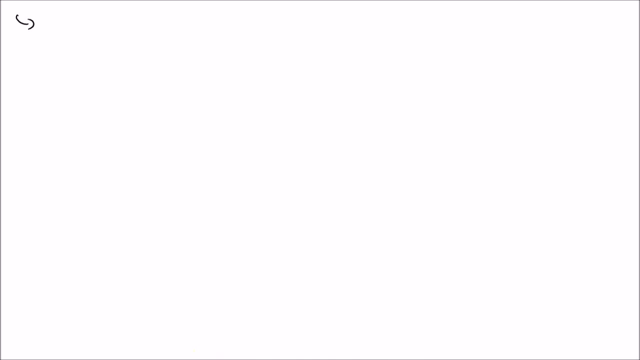 knowledge and for the future. for the exam: uh, we can say for the exam. uh, we can say for the exam, uh, we can say in k um, so we can see, in k um, so we can see, in k um, so we can see. it can be shown that, let's write it can. 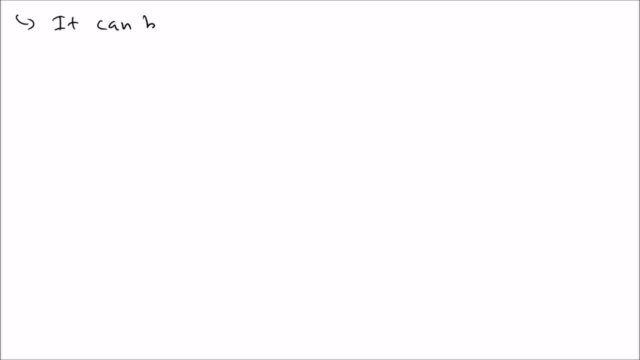 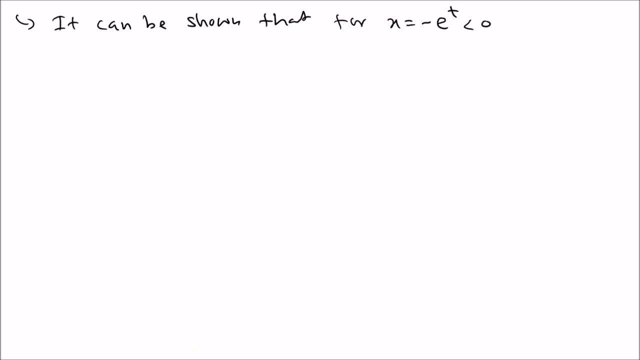 equal negative e to the t. that's the equal negative e to the t. that's the other case. other case, other case. that means x is negative. we get the that means x is negative. we get the that means x is negative. we get the exact same characteristic equation. 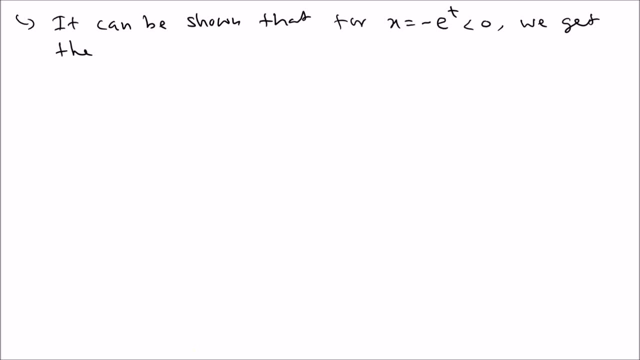 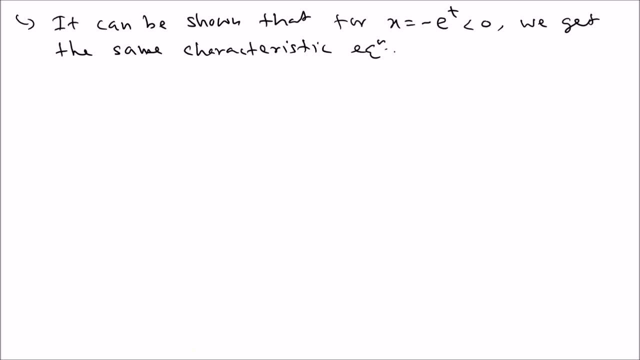 we get the same characteristic equation. we get the same characteristic equation. we get the same characteristic equation: ah. so the generational ah, so the generational ah, so the generational solution. so the general solution, so the general solution, so the general solution for x, not t equal to zero. 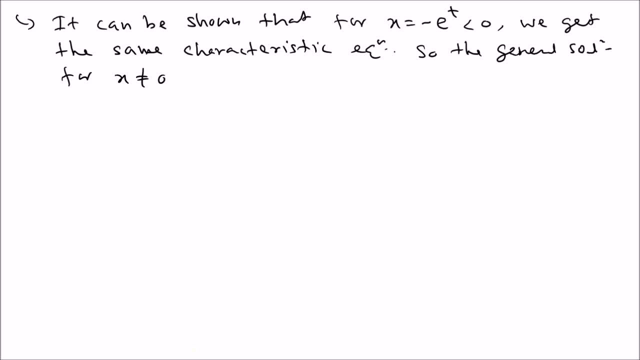 for x not t equal to zero, for x, not t equal to zero. so what you want to do, we want to consider. so what you want to do, we want to consider. so what you want to do, we want to consider the positive case and the negative case. 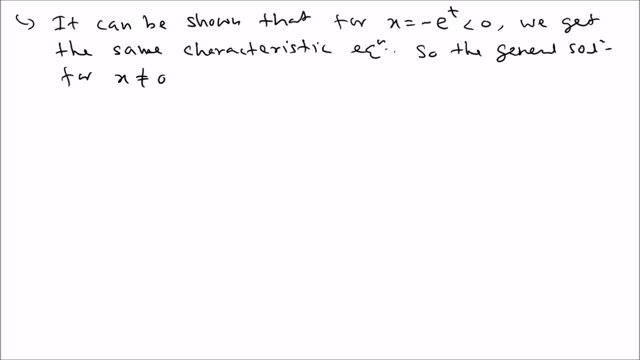 the positive case and the negative case, the positive case and the negative case. so instead of x we put absolute value. so so instead of x we put absolute value. so so instead of x we put absolute value. so that means the three cases are. that means the three cases are. 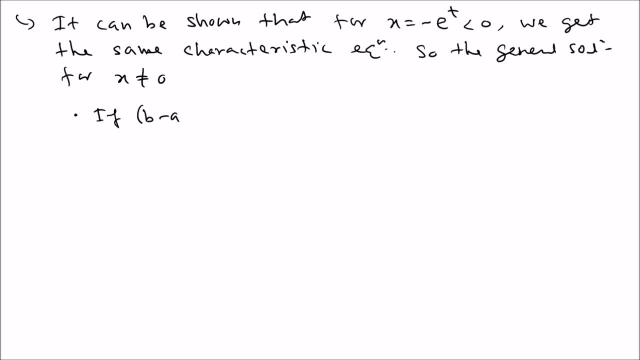 that means the three cases are: if t minus a, if t minus a, if t minus a squared minus 4 a, c squared minus 4 a. c squared minus 4 a. c positive, positive, positive, then the solution is y, then the solution is y, then the solution is y, c1, not just x, the absolute x, because it 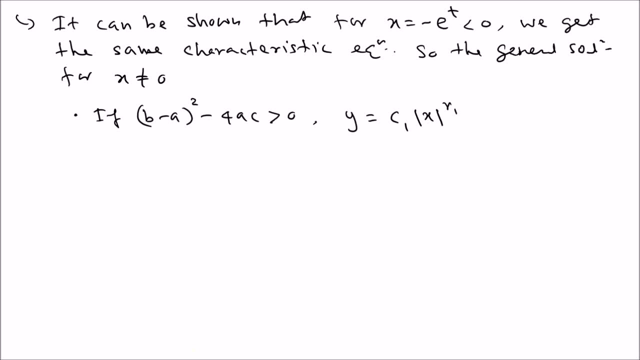 c1, not just x, the absolute x because it c1, not just x, the absolute x because it it can be positive or negative, it can be positive or negative, it can be positive or negative. r1 because we don't know whether those. r1. because we don't know whether those. 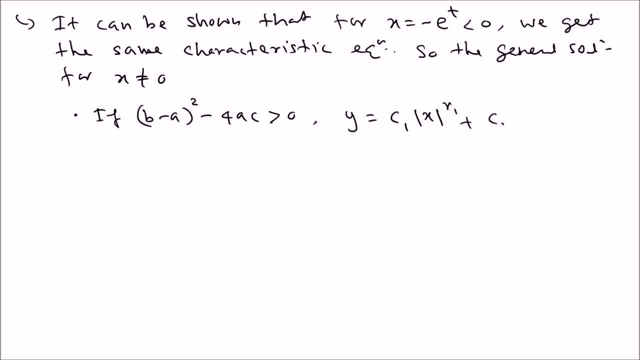 r1, because we don't know whether those are integers. are integers, are integers, so be careful. and then c2, so be careful. and then c2, so be careful. and then c2, x r2, so it has the both positive, and x? r2, so it has the both positive and. 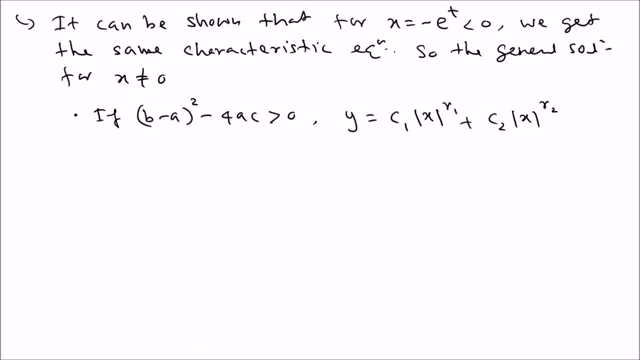 x r2, so it has the both positive and negative case. only thing is you include negative case. only thing is you include negative case. only thing is you include absolute sign, absolute sign, absolute sign, and the next one is if, and the next one is if, and the next one is if: b minus a squared. 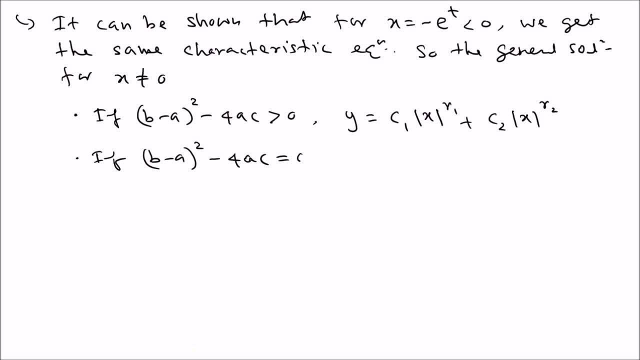 b minus a squared, b minus a squared minus 4ac- exactly equal to 0 minus 4ac. exactly equal to 0 minus 4ac, exactly equal to 0. in that case, y equal c1. in that case, y equal c1. in that case, y equal c1 plus c2. ln absolute value of x. 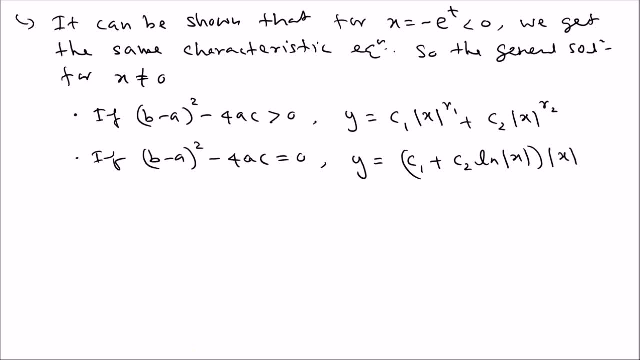 plus c2 ln: absolute value of x plus c2 ln: absolute value of x times absolute value of x times absolute value of x times absolute value of x. r1: that's the common r1 solution. r1: that's the common r1 solution. r1: that's the common r1 solution. the third case is if: 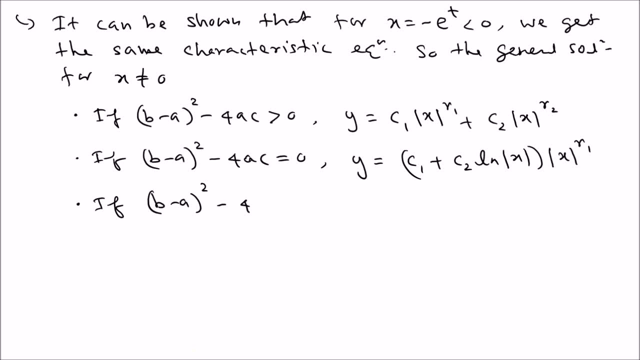 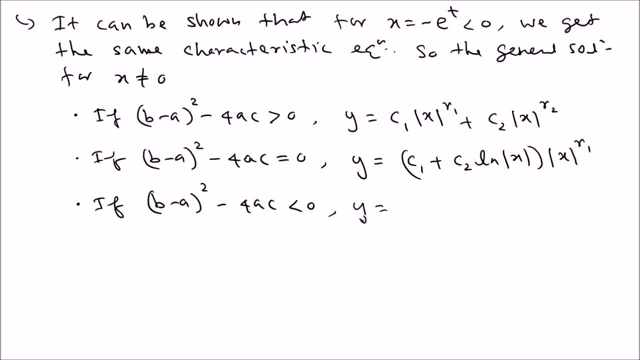 uh, what happened? we have alpha beta. uh, what happened? we have alpha beta. so that means your solution is simply so. that means your solution is simply so. that means your solution is simply: uh, i don't think i have enough space. uh, i don't think i have enough space. 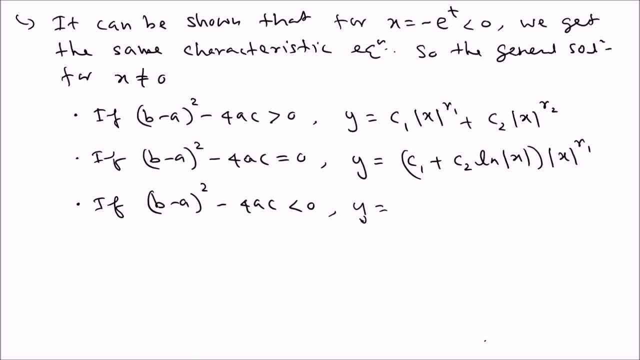 uh, i don't think i have enough space here. yeah, that's right, uh. so it is x to the. yeah, that's right, uh. so it is x to the. yeah, that's right, uh. so it is x to the alpha times, alpha times, alpha times. c1 cosine. 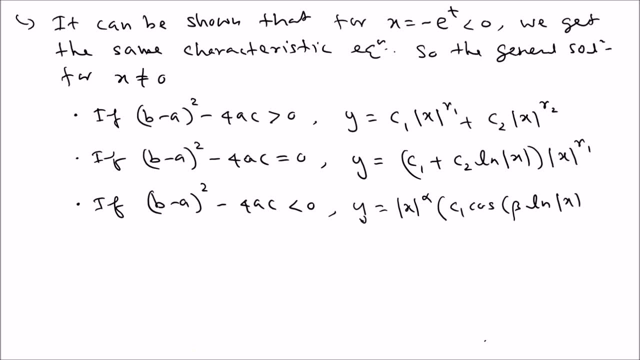 c1 cosine, c1 cosine beta beta beta ln x plus c2 x plus c2 x plus c2 sine beta sin beta, sin beta ln x. so that's the ln x, so that's the ln x, so that's the general case for any x other than zero. 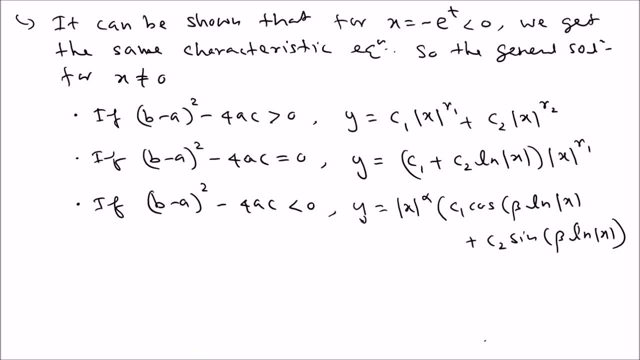 general case for any x other than zero, general case for any x other than zero. so, let's just so, let's just so, let's just solve one equation. one problem to see. solve one equation, one problem to see. solve one equation, one problem to see how it works. 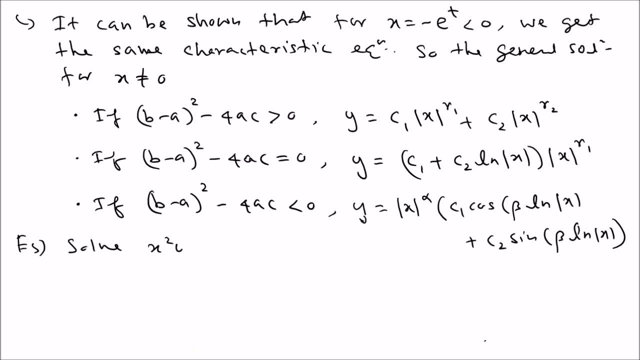 so say: solve x double. so say solve x double. so say solve x double prime x x squared y. double prime minus prime x squared y. double prime minus prime x squared y. double prime minus two x y prime minus four y two x y prime minus four y. 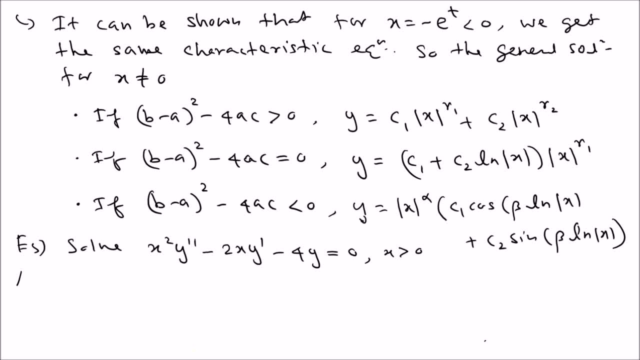 two x y prime minus four y equals zero for positive x equals zero for positive x, equals zero for positive x. so the answer, so the answer, so the answer. the characteristic equation, the characteristic equation, the characteristic equation is: uh, so in this case a equal one. uh, so, in this case, a equal one. 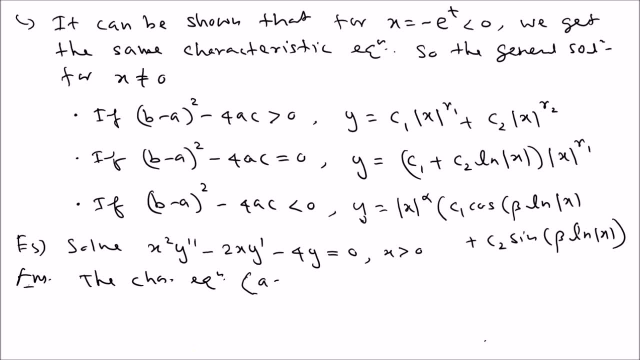 uh, so in this case a equal one, so we can see and write, so we can see and write, so we can see and write. a equal one b equal negative. two a equal one, b equal negative. two a equal one b equal negative. two c equal negative, four. so the characteristic. 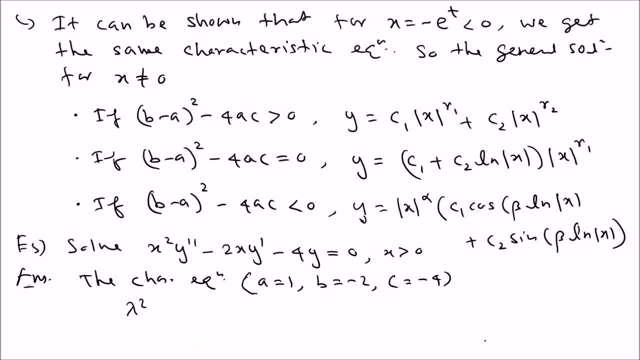 c equal negative four. so the characteristic c equal negative four. so the characteristic equation is simply equation, is simply equation, is simply a lambda squared plus a lambda squared plus a lambda squared plus minus b, minus one lambda, minus b, minus one lambda, minus b minus one lambda, minus four equals zero. 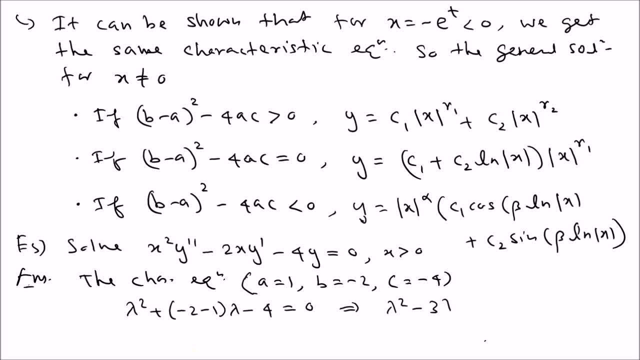 minus four equals zero. minus four equals zero. and so this says that lambda is squared. and so this says that lambda is squared. and so this says that lambda is squared minus three. lambda minus four equals zero. minus three lambda minus four equals zero. minus three lambda minus four equals zero. so the uh. 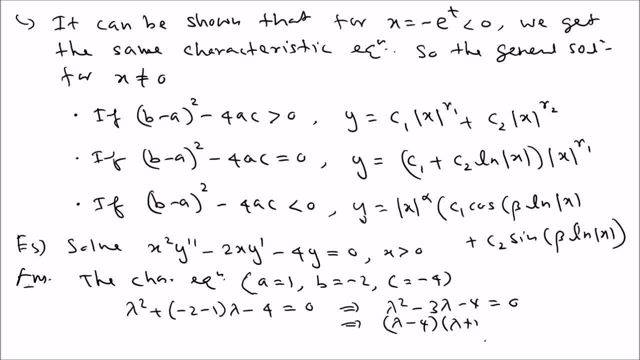 so the uh, so the uh. you get negative four and one, you get negative four and one, you get negative four and one. so this says that, so this says that. so this says that: lambda equal uh negative one. lambda equal, uh negative one. lambda equal uh negative one and four. 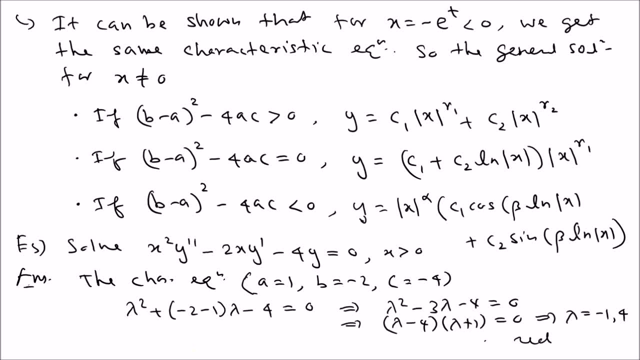 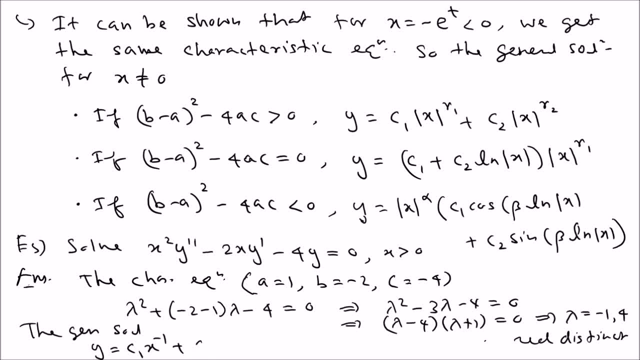 y equal c1. y equal c1 x negative: 1 plus c x negative 1 plus c2 x negative: 1 plus c2 x 4, or if you divide x 4, or if you divide x 4, or if you divide c1 over x plus. 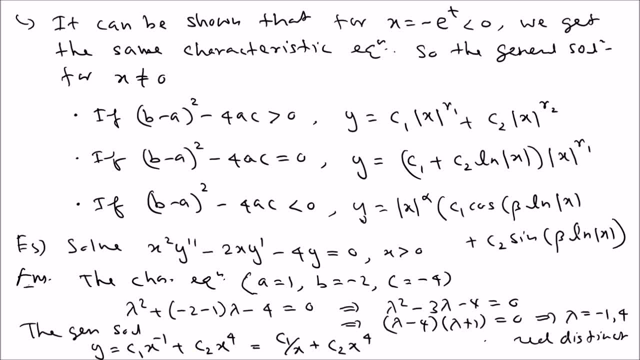 c1 over x plus c1 over x plus c2 x to the fourth power. so that is the c2 x to the fourth power. so that is the c2 x to the fourth power. so that is the complete solution. so you can see it's. 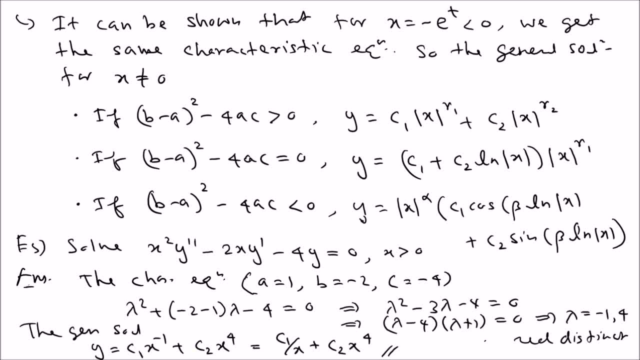 complete solution. so you can see it's complete solution. so you can see, it's not that difficult, but you have a new, not that difficult, but you have a new, not that difficult, but you have a new characteristic equation, characteristic equation, characteristic equation. so it is not: uh, lambda squared a lambda. 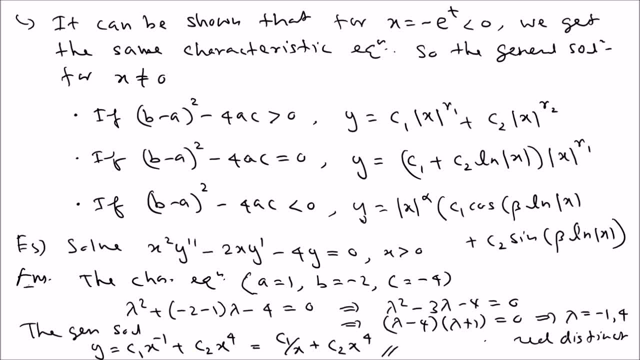 so it is not uh lambda squared a lambda. so it is not uh lambda squared a lambda squared plus b lambda plus c. it is squared plus b lambda plus c. it is squared plus b lambda plus c. it is a lambda squared b minus a, b minus a lambda. 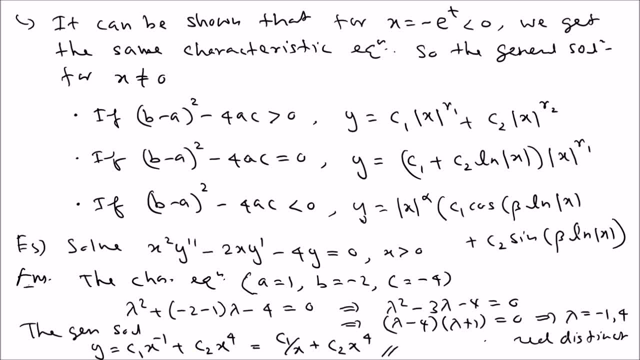 uh plus c. okay good, so that's the uh uh plus c. okay good, so that's the uh uh plus c. okay good, so that's the uh. that's about the characteristic. that's about the characteristic. that's about the characteristic kochi euler equations. so let's move on. 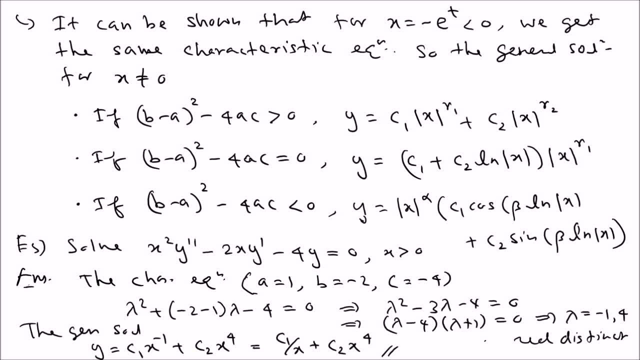 kochi euler equations. so let's move on kochi euler equations. so let's move on to the higher order differential, to the higher order differential, to the higher order differential equations. we just talk about the basics equations, we just talk about the basics equations, we just talk about the basics of that, and then we're going to move on. 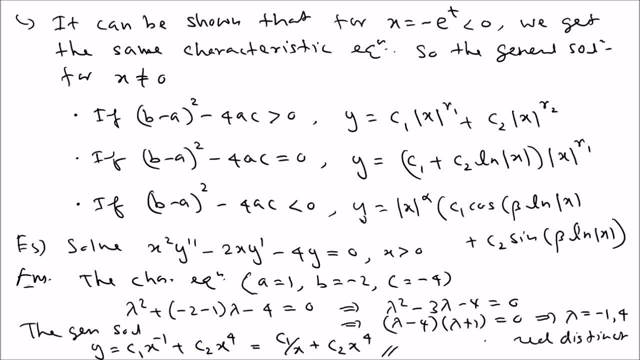 of that, and then we're going to move on of that, and then we're going to move on to the non-homogeneous equation and to the non-homogeneous equation and to the non-homogeneous equation and undetermined coefficient method. undetermined coefficient method. 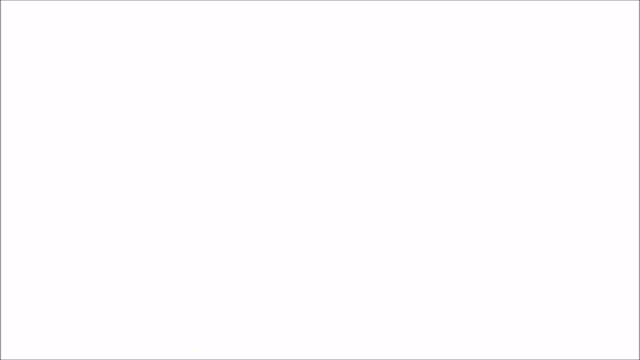 undetermined coefficient method. so let's talk about a little bit about, so, let's talk about a little bit about, so let's talk about a little bit about the uh, the uh, the uh. higher order difference equation. so this higher order difference equation, so this higher order difference equation. so this is topic 20. 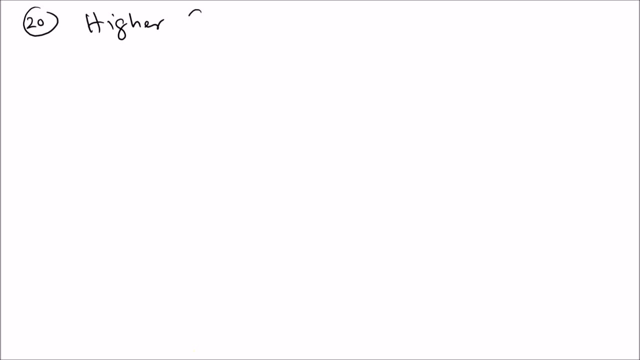 is topic 20. is topic 20: higher order: higher order: uh constant coefficient. higher order: uh constant coefficient. higher order, uh constant coefficient, constant, constant, constant, coefficient, differential equations. so it's coefficient differential equations, so it's coefficient differential equations. so it's very important we do the constant. 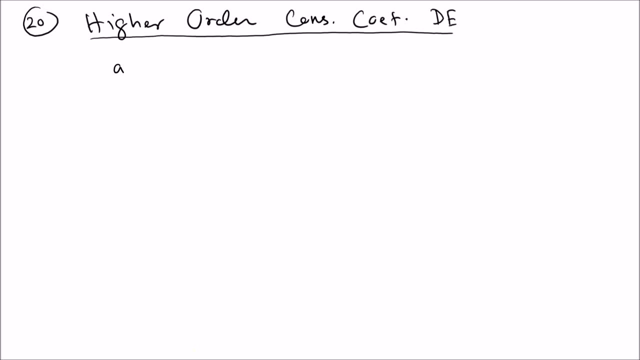 very important. we do the constant. very important, we do the constant. coefficient only in this one. coefficient only in this one, coefficient only in this one. uh. so those equations have this form a. uh. so those equations have this form a. uh. so those equations have this form a. y n, power, b, y. 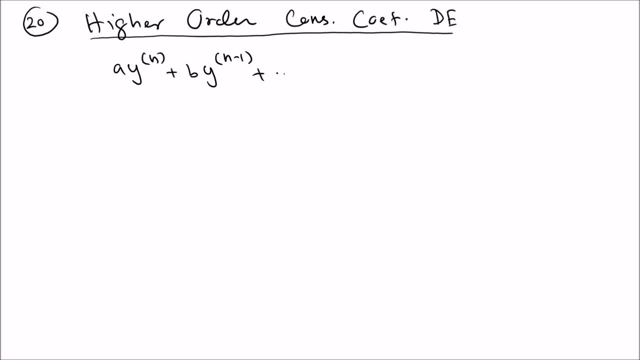 y n power, b, y in minus first derivative. like that we have a first derivative and a constant term, not a constant term. d y term is equal to zero, it's a homogeneous. so we can look at the homogeneous case. good, same idea. you can assume a solution of the form. assume a solution. 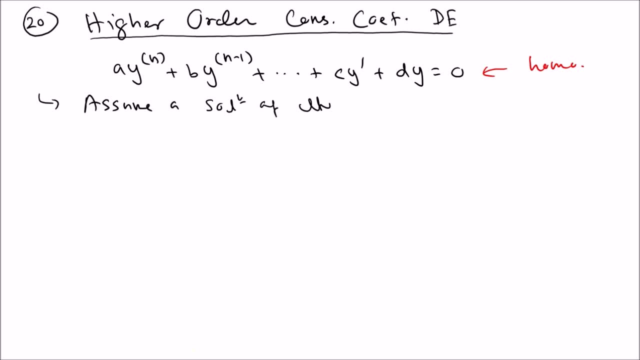 of the form y equal e lambda t, then we get the characteristic equation as before. so the characteristic, the characteristic equation is a lambda n, power is b lambda n minus first power, like that. so you get c lambda plus d equals zero. so that's the characteristic equation. 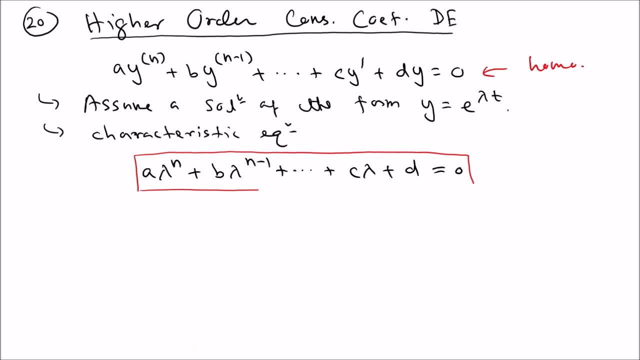 now what we're going to do. we're going to factor this, get the numbers and plug. so, uh, we're going to factor this. okay, so you can factor this. so there are a few cases. so let's go case by case. so we have cases. so the first one is: if 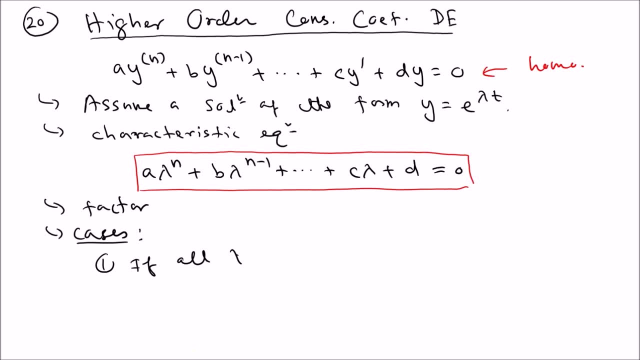 all lambdas are real and distinct. that's the most common case. so what's happened? just the extension of what we learn. so the c 1 e lambda 1. if you use the x as the independent variable, like that, c 2 e lambda 2 x. like that c n e lambda n x. 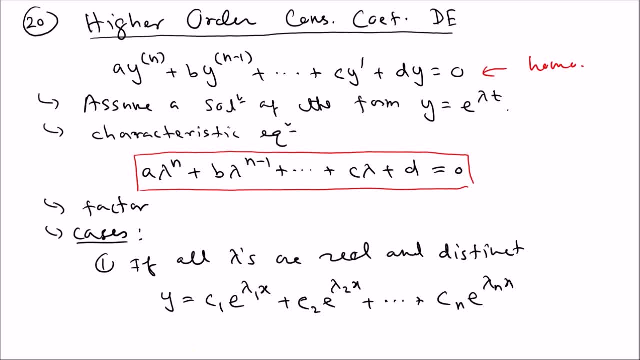 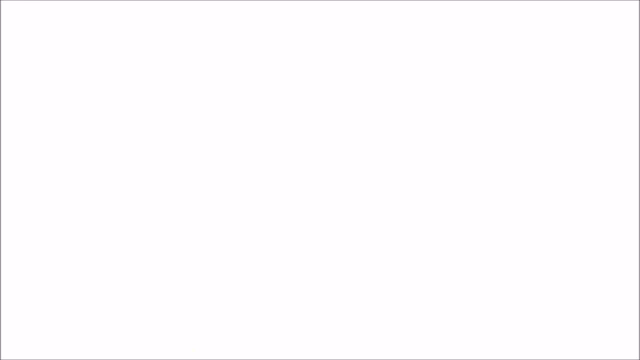 so that's what happened in the uh distinct case. so let's look at the uh repeated case- very similar. so the case 2: uh, let's say, if lambda 1, uh repeats m times and the rest are distinct, the others are distinct, uh, if that is the case uh, then what happened? 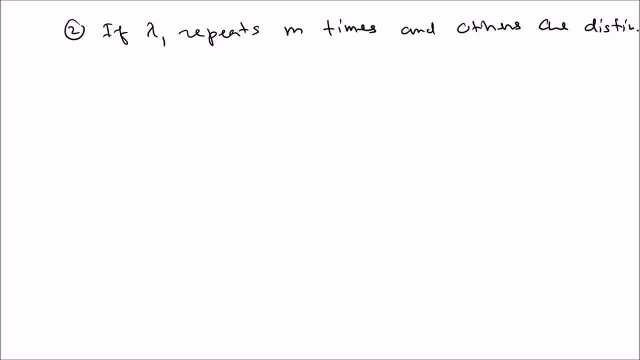 why? so this is just extension of what we have, because when we have two, we have c 1 plus c 2 x. so this is the extension of what we have, because when we have 2, we have c 1 plus c 2 x. so we have c 1 plus c 2 x. so this is the. 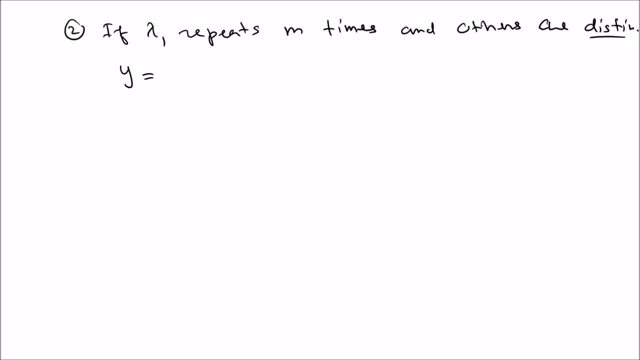 extension of what we have: c 2 x. so if you're m, you're going to go m minus 1. okay, that's idea. so that means c 1, c 2 x, like that. we'll continue that and then we have c m. m term has the. 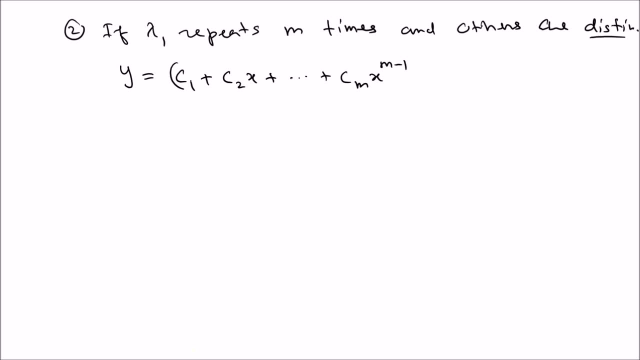 power m minus 1, and then we have: this is similar. so l lambda 1, x plus the rest. we know i just put some numbers, so let's say d, uh, e to the next lambda value, just repeat, and then the last lambda value, lambda n, x, like that, okay. so the 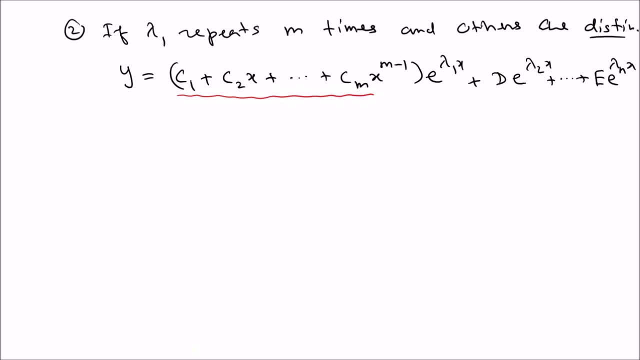 interesting part is here how we can write that term. you can see if it is a m repeats, you're going to see m minus 1, which is 2. you're going to see x. it's like that, okay. and then the last case is the complex case. so let's say: if uh, 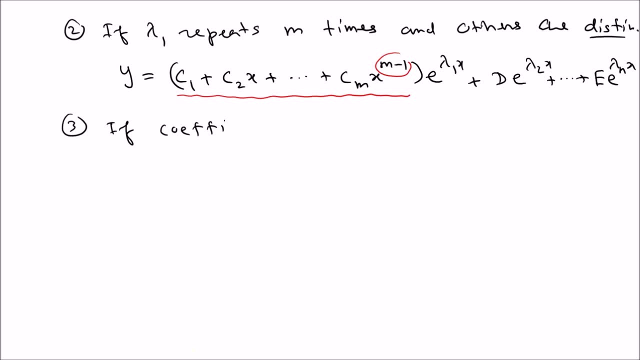 uh coefficients are real. so it's very important: coefficients are real. if the questions are real, then uh, then we have complex conjugate roots, then we have complex conjugates, always complex conjugate uh roots. if the if the coefficients are real, uh, the solution has to be complex. 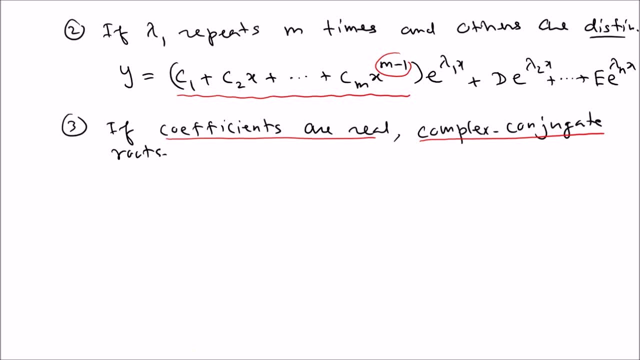 conjugate. that's like theory we prove in algebra. uh, complex conjugate, let's say complex conjugate pairs, that's right, complex conjugate pairs. so let's say: uh, lambda, equal alpha plus, so minus. i beta the whole thing, we will go with pairs, okay, repeats. 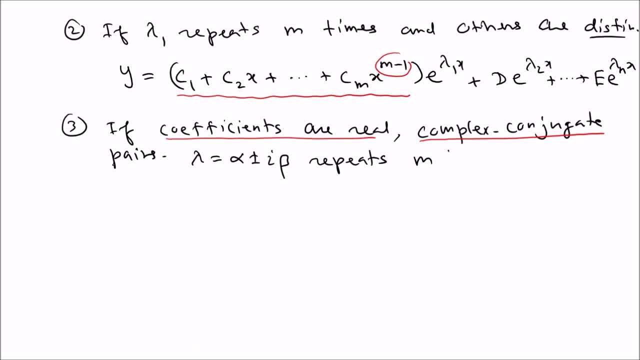 uh, repeats m times. this thing can repeat m times, and others are distinct, others are distinct. so in that case, what's going to happen? y is simply c1 plus same thing again. so we have c, m, x, m minus one. that's the coefficient of e, alpha, x, cosine, beta, x plus. 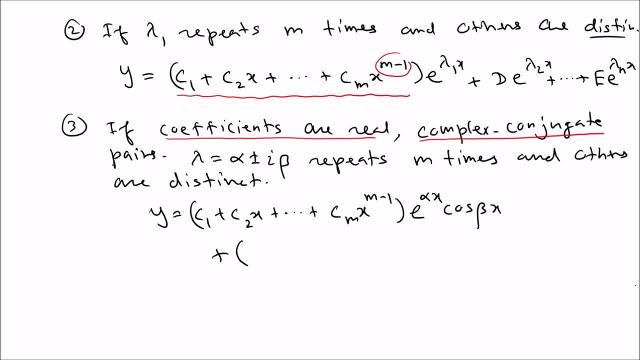 a similar term for our course. as a sine we have d 1 plus d 2 x, like that: d m, x, m minus 1, e, alpha x, sine, beta x and then plus are the other terms. all the uh non-equals, but see the format. so we. 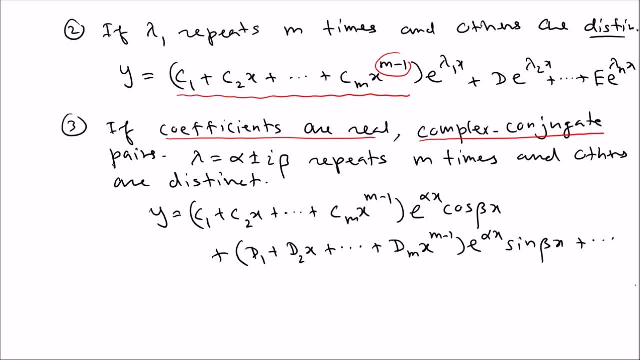 we have two there, so that means we already have two m off. okay, because there are two m many terms and then the rest. rest is n minus 2 m many terms are there, and that's going to follow the other pattern. okay, so that's, that's the idea. 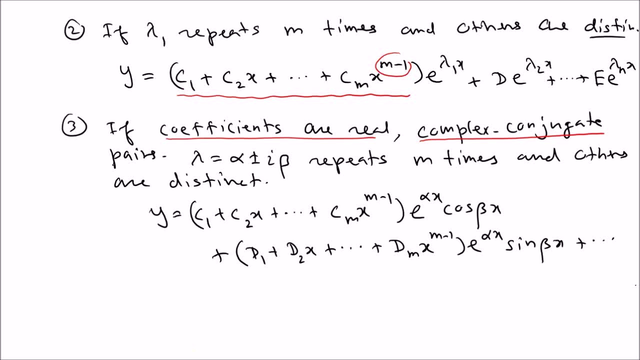 okay, so that's the idea. and then, uh, let's talk about the linear independence. linear, uh, independence, uh, it's very similar, so we can write the wranskian. uh, so, for example, if we have three functions, so we can extend that to many, but let's just for three, so we have the wranskian, so it's going to be. 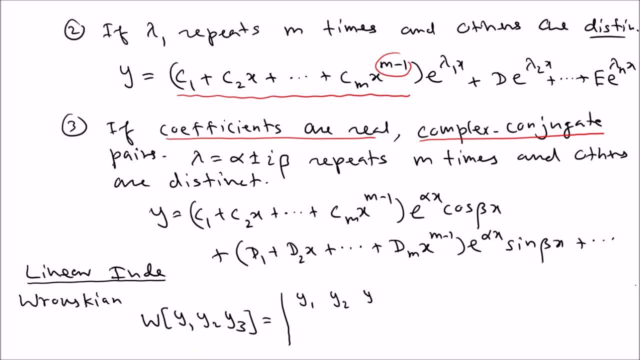 y, y 1, y 2, y 3. take the first derivative, ah, so this is 3, take the first derivative and take the second derivative, so that's the wranskian. and then, if this is not t equal to 0 in general- for some x naught, the functions are that this implies that y 1. 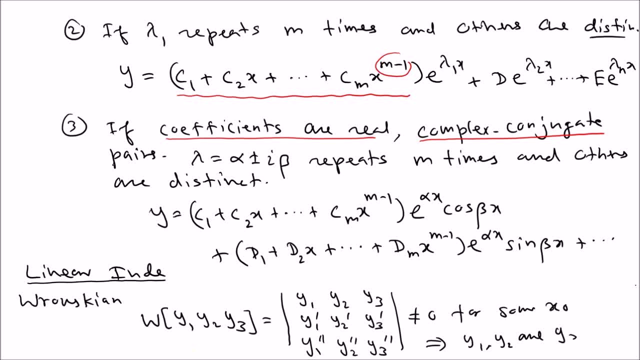 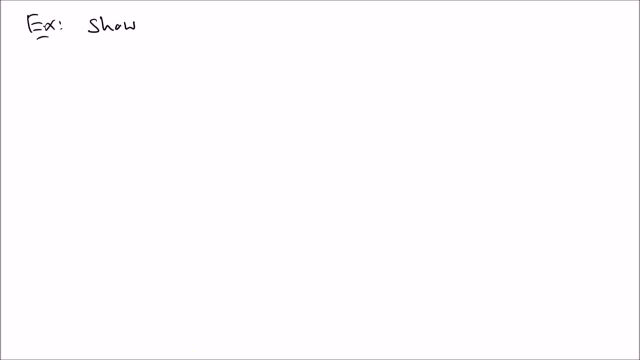 y 2 and y 3 are linearly independent. okay, so that's the kind of idea. so very similar, ah. so as an exercise you can try this. um, you can see the detail in the uh actual lecture example show that so that one sine x, cosine x, these three functions. 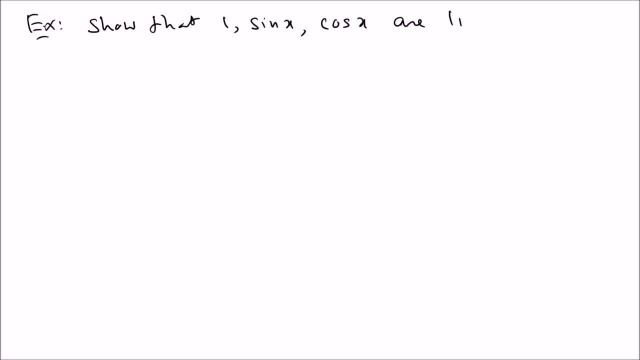 are linearly independent and we already know that this is a one of the uh common linear independent set. we discussed that earlier. so just prove it. and you consider this very easy because one is there once you take: the first derivative is zero, secondary is also zero, so that means the. 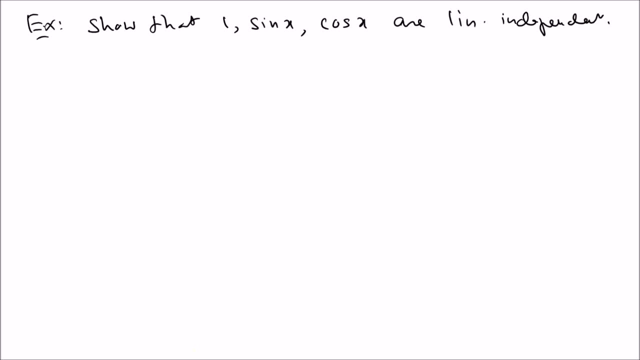 determinant of the three by three matrix is very easy. if you write the cofactor expansion, you only need one times a two by two. so so just one term. so it's very easy. okay, so you can try that. um, let's, let's do it like a regular problem. 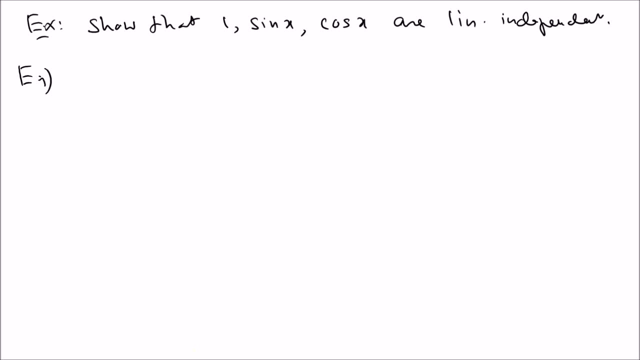 so how about this one? uh, find the general solution of find the general solution of uh, two y, triple prime plus y, double prime plus y equals zero, something like that. so it's a third order differential equation. uh, now what we can do. same argument: we can look at the characteristic. 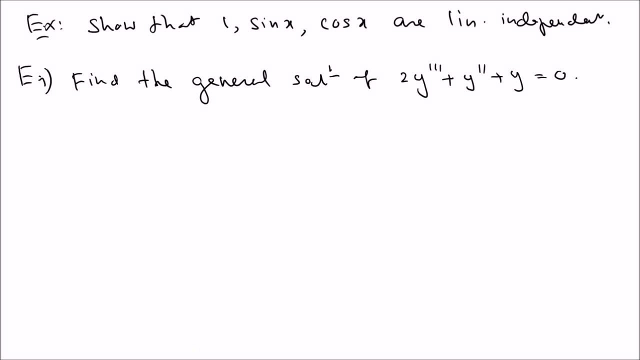 equation? uh, so the answer, we can look at the characteristic equation. uh, equation is going to be: 2 lambda cube plus lambda, squared plus 1, equals 0.. so this is what we get. so it's a cubic equation and you can see that there are no four terms. that means: 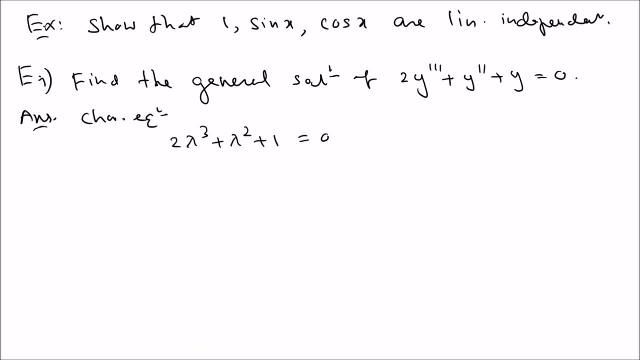 grouping doesn't work for this problem. what we can do, we can use the factor theorem for that. okay, so, uh, select f lambda equal to lambda cube lambda squared plus. and if you are not familiar with how to find factors of the things like that, please look at the factor theorem video. 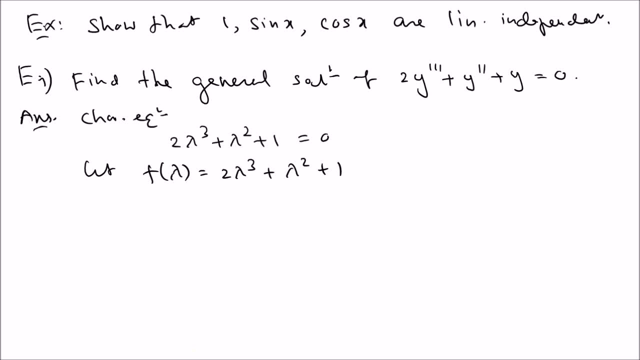 and there i explained: like many different type of problems, like in a quadratic cubic uh quality, like in order four and a quintic, order five, and even like order eight, nine, ten, like larger ones also, we basically use the factor theorem and and then the long division of the synthetic division we normally we go for. 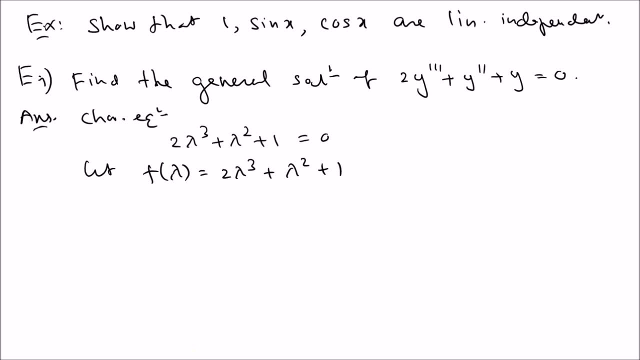 the synthetic division. we first use the factor theorem and then use the synthetic division. that's how we normally do it. so let's, let's see how it works here. after you get that, now we can notice, notice that, uh, and then let's say, not that now what we're going to do is we're going to try these values. 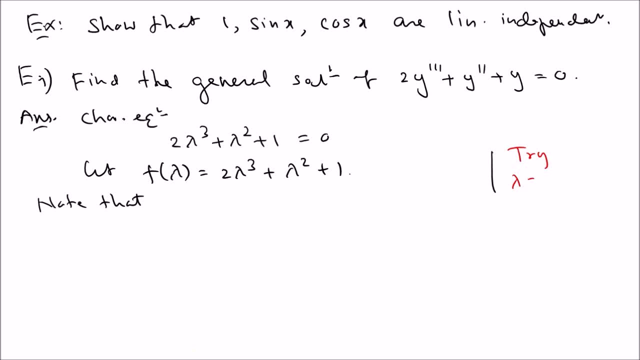 we're going to try: lambda equals zero plus or minus one, and plus so minus two we, until you get a quadratic. that means you only need to find one value, because after that you can divide, then you can get the quadratic. so use the quadratic formula or factor. 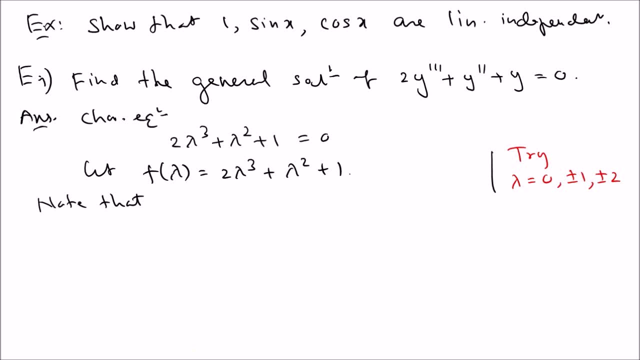 so we just need one value to find. so note that if negative one, if you plug in the negative one, what can happen to negative one cube? negative one cube plus negative 1 squared plus 1, how much you get? you get negative 2 plus 1 plus 1, which is 0. what does that mean by the factor theorem? 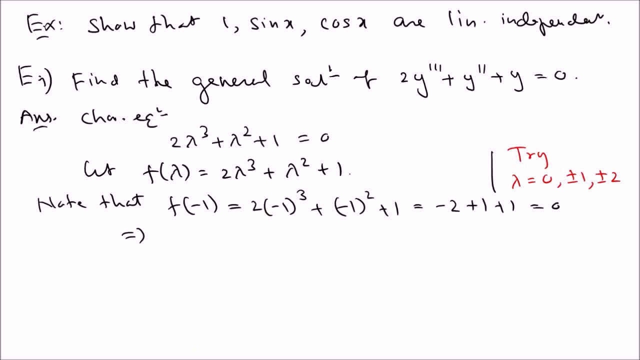 this means that. so this means that lambda plus 1, y plus 1, because it is minus minus 1, because minus we put here in the minus 1, so it's a factor theorem. so lambda plus 1 is a factor, or in other words, negative 1 is a 0. so now what we can. 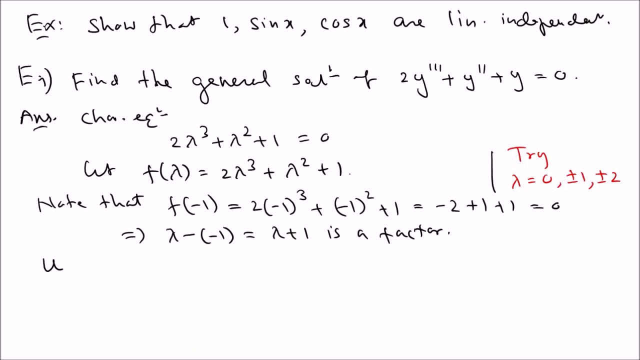 do? we can use synthetic division to find the other one. so use synthetic division to find the other factor, to find other fact. so let's see how it works. in the synthetic division we only uh use the coefficients. so the coefficients are 2 of the original polynomial. 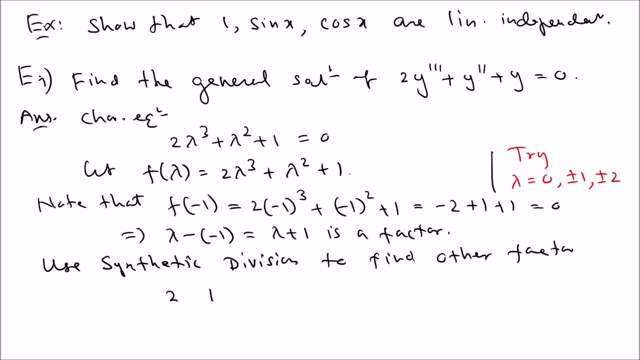 and then x squared, x cube plus 2 and then 1. there's no lambda term. so that means you'll put a 0 there and then 1. so those are the coefficients. so we check negative 1, whether negative 1 is. no, what we are doing is we. we want to get. 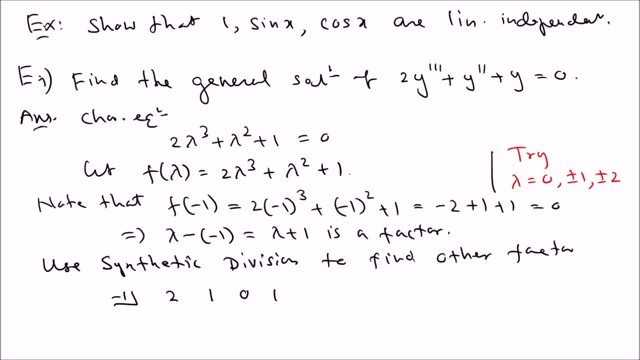 the quotient when you divide by lambda plus 1. so what we put here is the 0 corresponding 0, and you can see the lambda 1. lambda plus 1 means the 0 is negative 1, so that's the 0, so that's the one we're going to use there. 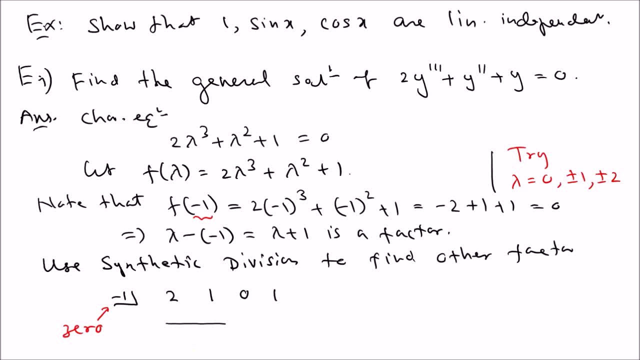 what we normally do is- uh, it's a very simple one. we copy that number first and then multiply and add. you're going to multiply negative 1 with 2 so you get negative 2 with there, and add so you can negative 1, then multiply again with negative 1 and negative 1, and then 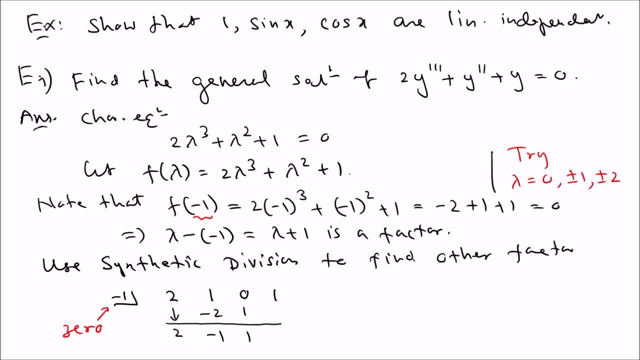 negative 1 and negative 1, so you get 1 and add. so you get there. just add, multiply, add and then negative 1, negative, negative 1 with 1, so you get negative 1, add, you get 0. that means good, that means it's completely divided. if you get a 0. 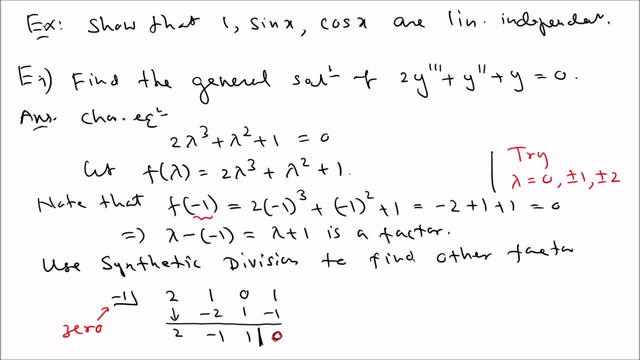 that means it's completely divided. so that's the quotient. so we have the other factor right here: 2 minus 1, 1. those are the coefficients. so that means the other factor are the factors. is 2 lambda squared? why? there are three terms: minus lambda plus 1, so we get that. so that's the other factor. 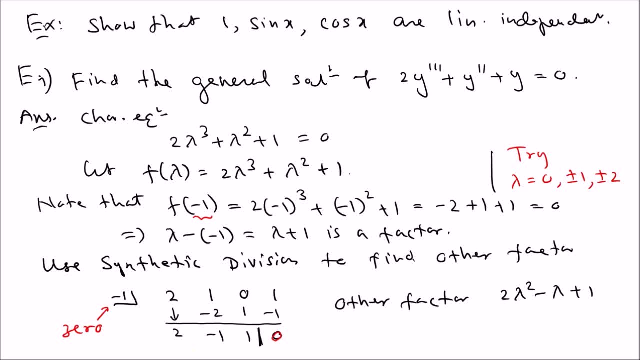 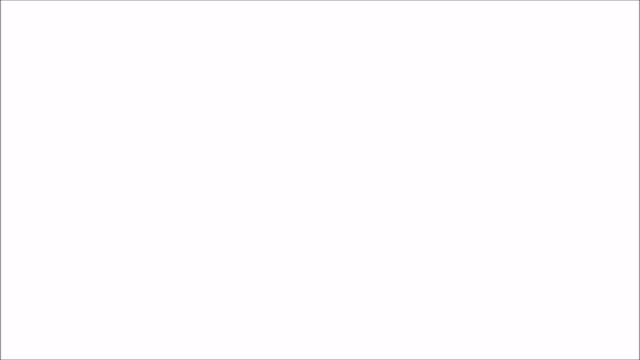 now what we can do. uh, so we can say that equals 0 because we looking for that, so we use. you can see whether you can factor. or you can see that it's not easy to find factor, so we can use the quadratic formula. so let's use the quadratic formula. 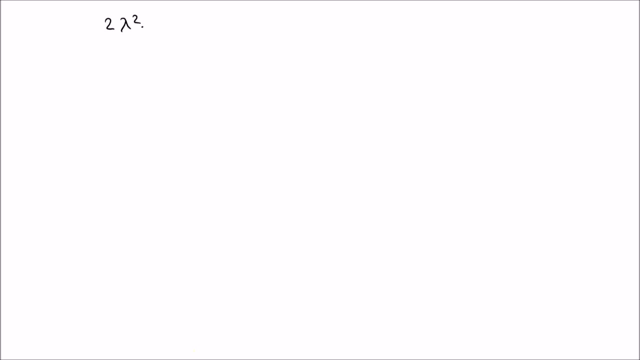 so we have 2 lambda squared minus. lambda plus 1 equals 0 lambda equal minus 1 plus plus or minus 1 minus 4. a c square root over 2a, that means 4. so let's simplify: you get plus 1 plus or minus. you get 1 minus 8. so that means negative 7 square root. 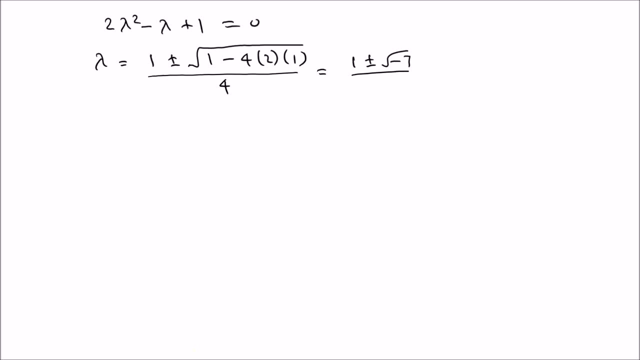 over 4, using complete equations. so you get 1 minus 8. so that means negative 7 square root over 4 plus 1 minus 2 square root 7 over 4. i so, uh, that is the alpha, that is the beta. so we have alpha and beta. now we can. it's a complex, so the complex conjugate. 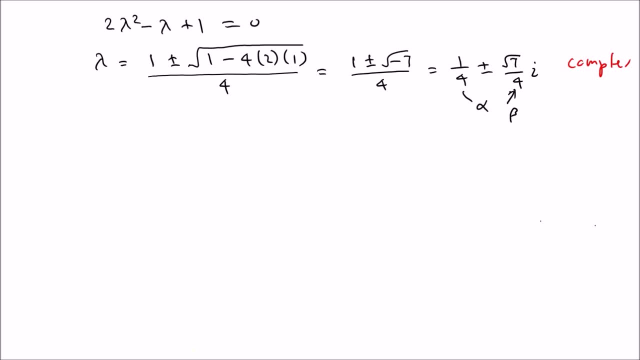 complex conjugate. so complex conjugate means we can use the complex form, so we can use the complex form. so the three roots are uh. so we can see thus: the three roots are lambda, one is negative one and the other one is one fourth plus or minus. 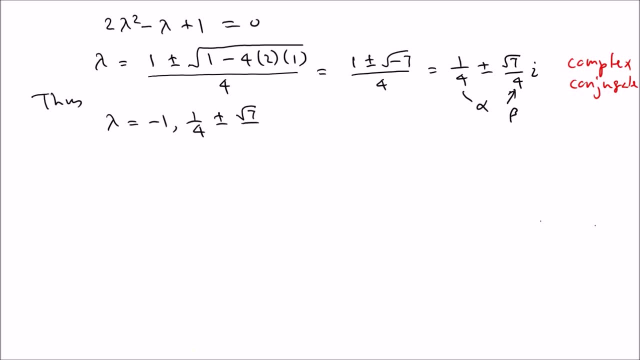 square root, 7 over 4, i, uh, and, as before, the alpha and beta. so we write general solution. so the general solution. so the general solution we can write, which is y equal to y equal c, 1, e to the negative t plus. let's write the form first. so what is the form actually? 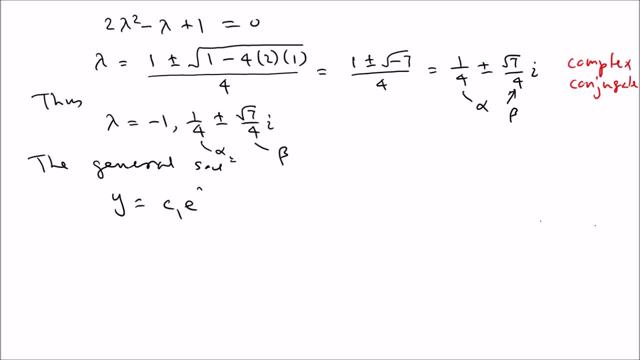 uh, because this there's a one real uh and then uh, complex. so let us see, we can write this one as c 2 e to the alpha t- cosine beta t, plus c 3 e to the alpha t- sine beta t, and if you plug in that, 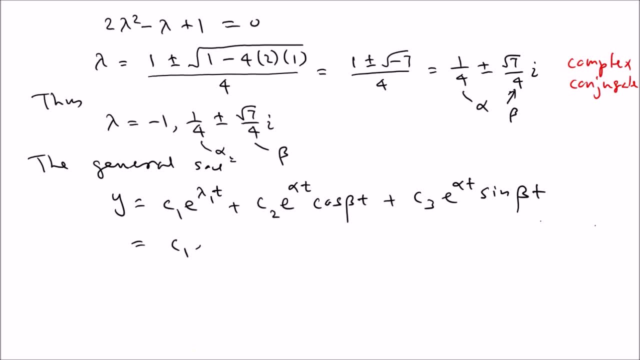 here you're going to get c 1 e to the minus t plus c 2 e to the. uh, what's the alpha? one fourth. so one fourth t cosine square root 7 over 4 t, plus c 3 e to the one fourth t sine square root 7 of 4 t. 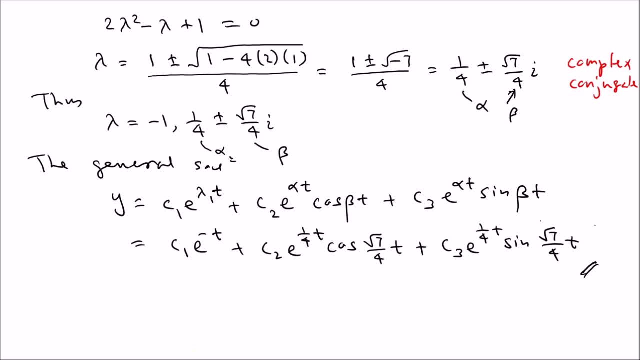 so that is the solution of the third order differential equation. so we use um quadratic equation, sin 3, division factor theorem. so it's like nice problem, okay, so this is the uh end of homogeneous equation. now let's discuss how to solve the non-homogeneous. 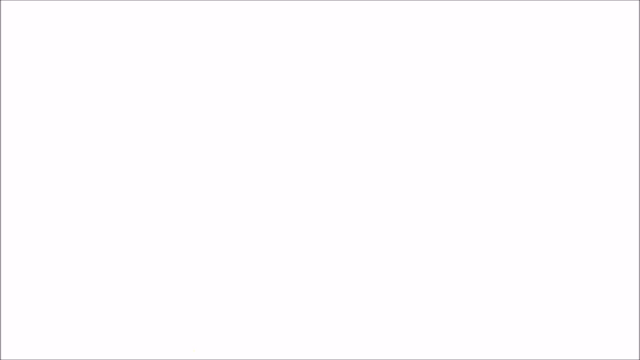 equation. so let's talk about the next, uh, very important type. so, uh, this is the how to solve a non-homogeneous equation. so this is topic 21: solving non-homogeneous equation. solving a non-homogeneous. so we can start with a problem like this: a y squared plus b y prime. 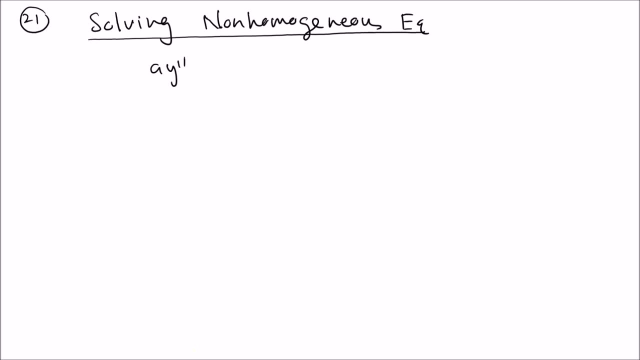 plus c, y, equal fx. this is again a constant coefficient situation. so, with a constant a coefficient, how we do, like this, so we have a constant coefficient, so we have a constant coefficient how we do like we didn't get a problem like that, we're going to split the. 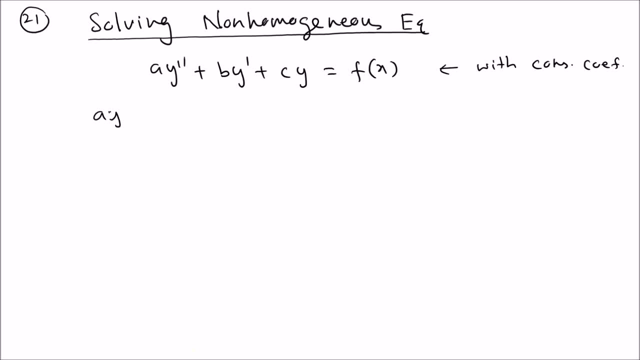 problem. are we going to consider the homogeneous part and the non-homogeneous part separately, like this. so from the homogeneous one we find a general solution. so find the general solution, general solution, what we normally call the complementary solution. so this has the format yc as a complementary solution: c 1 y 1 plus c 2 y 2. 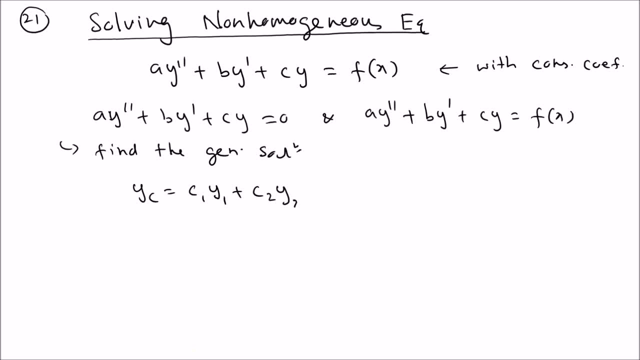 c 1, y 1, c 2, y 2. so that's the general solution, and for the other one we find one solution. so find a particular solution. we're going to call this y p ah. so just one solution, one solution, just one solution. so we don't mean only one solution. now what we can do: 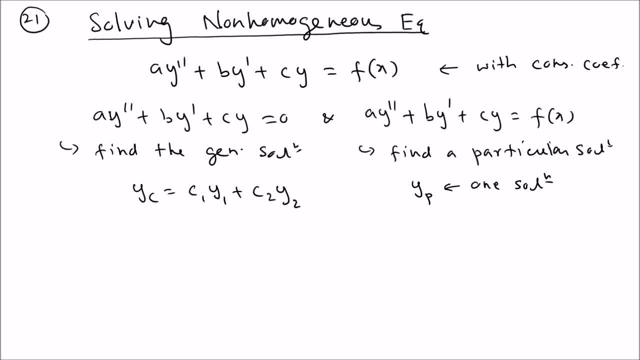 after we know the particular, this is what we call the complementary solution. so this is called the complementary solution to find the particular solution and this is the particular solution, particular solutions- and then we can have the general solution. so the general solution is general solution to the non-homogeneous. 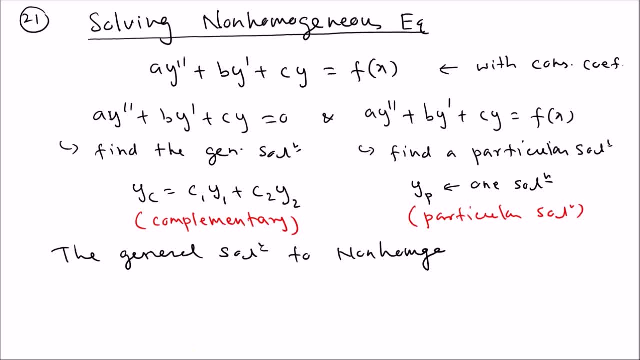 is given by y equal. we just add the two y c plus y p, so you're going to get c 1 y 1 plus c 2 y 2, plus that one solution that you find. so this is what we do. we just need one solution and we add that to the. 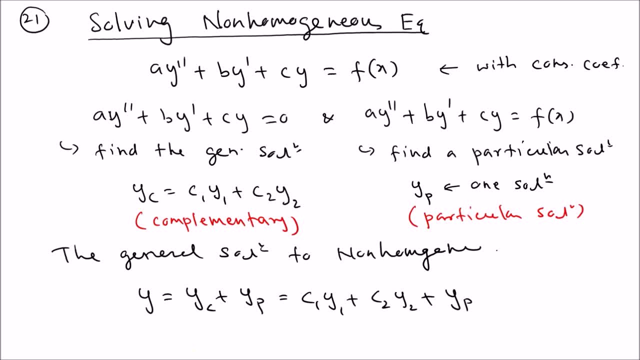 general solution. now the argument is: you know that the non-homogeneous equation is the same as the general solution. so we just add the two y c plus y p. so you're going to get the non-homogeneous equation and you can see that the 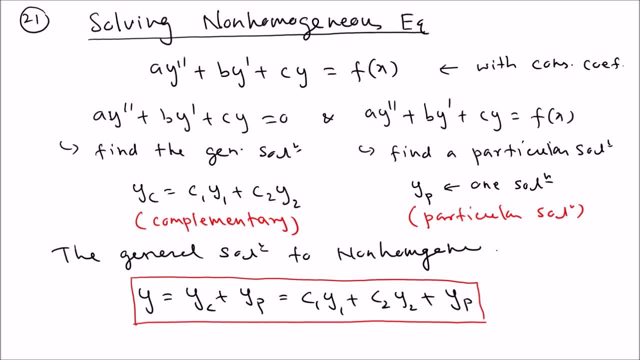 non-homogeneous equation is the second order, differential equation. that means, if you find the general solution, you need two constants. you can see these are the two constants, so everything looks good. so in the second order, you need two unknown, uh, two arbitrary constants. we have two arbitrary constraints, c1 and c2. okay, but yp is only one solution. 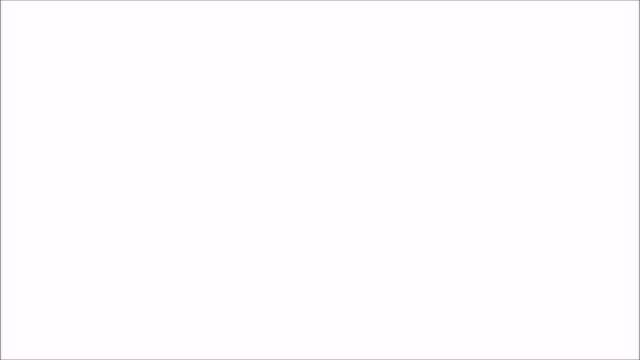 called the particular solution, now how to do this in reality. so what we do is that, uh, we use, uh, use two methods. two methods, uh, to find yp, because we only know how to find yc. uh, so the two methods are: first, one is what we call the undetermined. 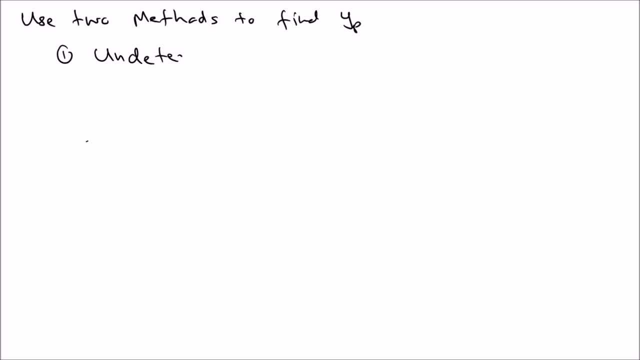 coefficient method, undetermined, undetermined coefficient. and we also use the variation of parameters: variation of a parameters method, variation parameters method. so the problem with the undetermined coefficient is you can only solve three type of problems. okay, so problem with like a exponential function, like that, and then sine cosine and then the polynomials. 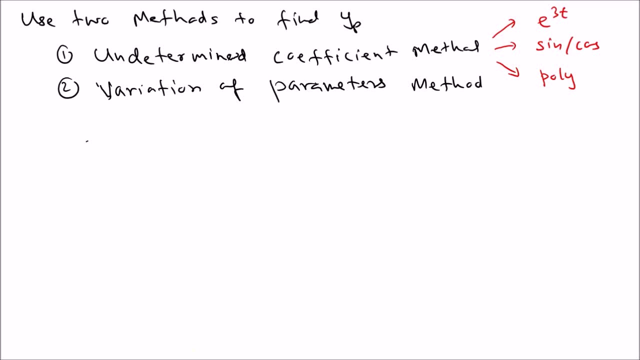 so polynomial. those are the only three types that you can solve using the undetermined coefficient method. so if you get something like secant, you cannot do using this method. uh, like natural log, you can't do, they're using this method, so that's a problem. so we need new. 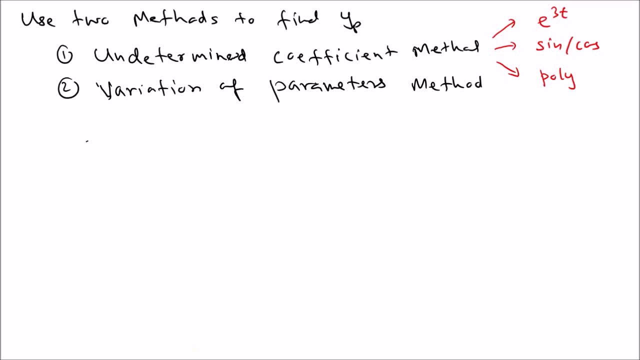 techniques to solve them. that's what we call the variation of parameters method. um, if you have something like that, okay, so let's first talk about the undetermined coefficient method. this is a very powerful technique, uh, so let's talk about that first. undetermined coefficient method. 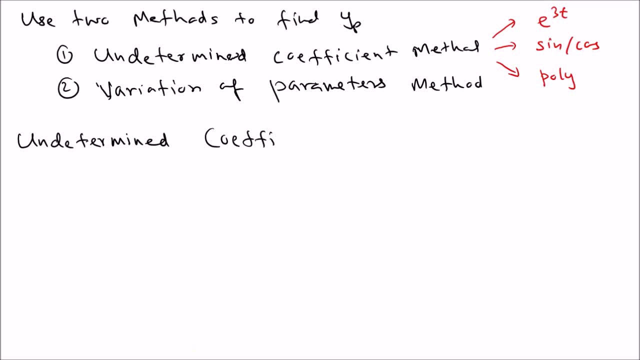 undetermined coefficient. so this is like simple idea. we kind of guess the solution and plug in and try to find those undetermined coefficients. um, so again, work for three cases only. work for three cases only. that's the major problem. so we have a y double prime plus the first and the second case of the 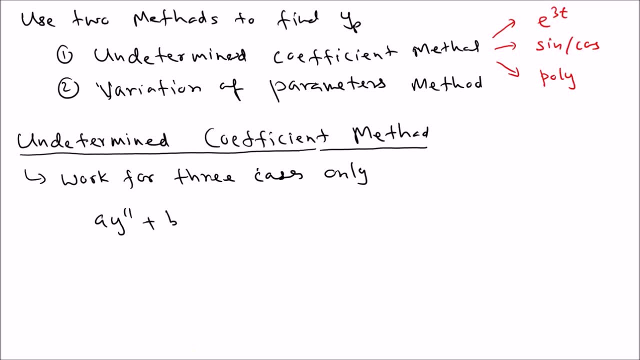 undetermined coefficient method: okay, prime plus b y, prime plus c, y equal. let's say: f, x, x is independent variable, so it can be exponential function. that means, if you have like 5 e to the 3x, we can handle that. then we have the sine and cosine functions, for example. 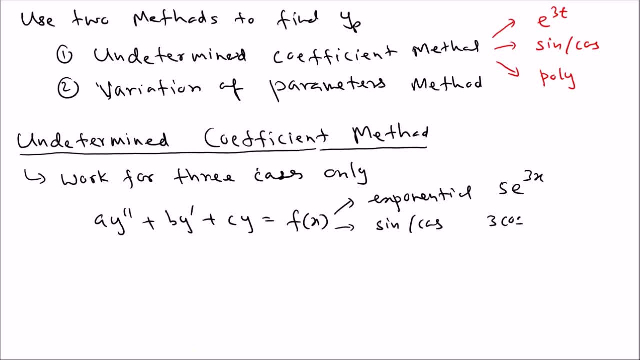 if we have 3 cosine, 2x minus 4, sine x, we can do that and you can see that this is 2, this is 1, that's okay, you can still do it. and the third case is the polynomials. so like a 2 x cube minus x plus 1, we can also. 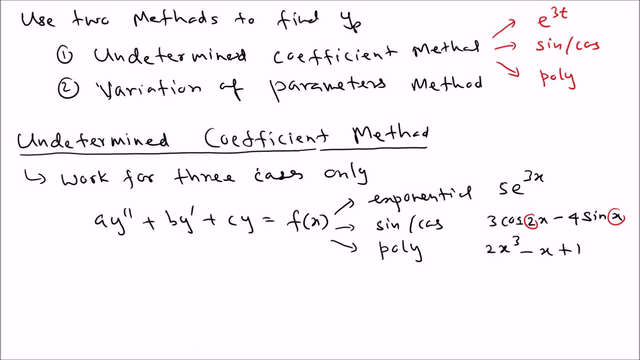 do that one. so those are three types that we can do. exponential: you can also do that one. so those are three types that we can do. exponential, sine cos and polynomials. so what we normally do is, uh, the first step is guess the particular solution, guess the form. 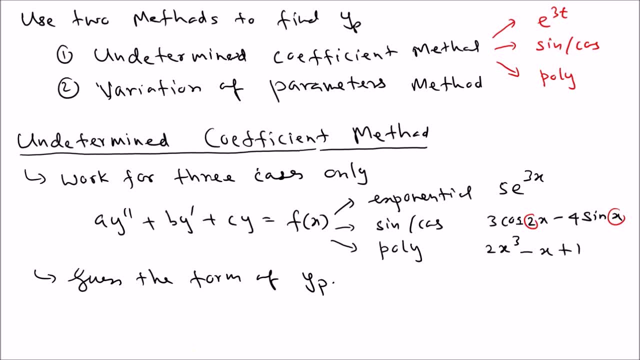 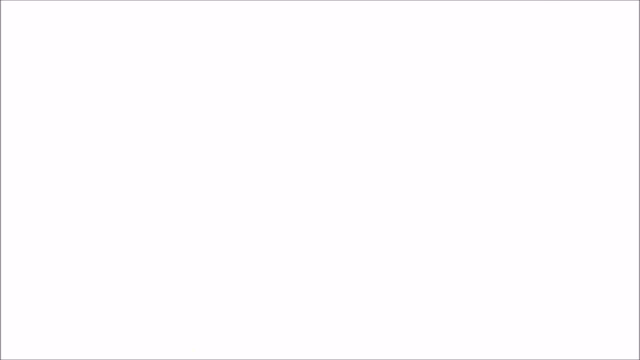 of yp. so that's what we we're going to guess. we guess the form of yp, uh so, but there are certain criteria for that, so let's talk about that. we have uh, so guess uh form of yp. so we're going to follow this table the first time. 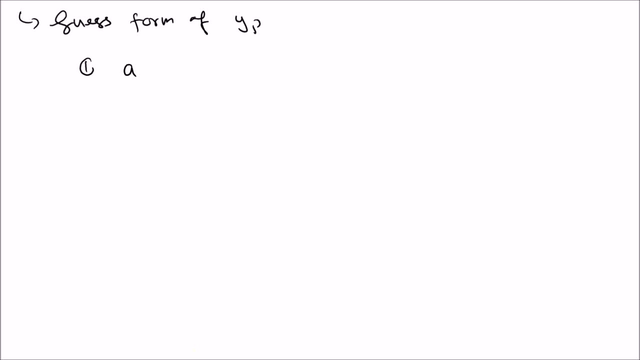 if we have a number times e to the beta x. beta is another number, so your yp. so it's a form of yp, uh gonna be a e to the beta x. the goal is to get the number of times e to the beta x. so that's the first step. 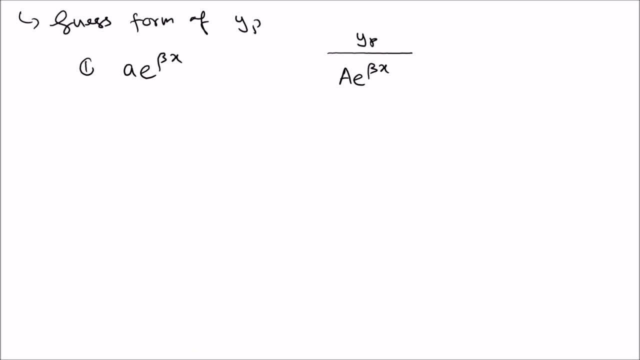 so what we're going to do is this time we're going to base an inverse on a number of times c and we have to find, and we are going to compose that somer sine four times e to the beta x dot into any beaten on, e to the beta x dot into any target was going to be gives outside 투 select the. 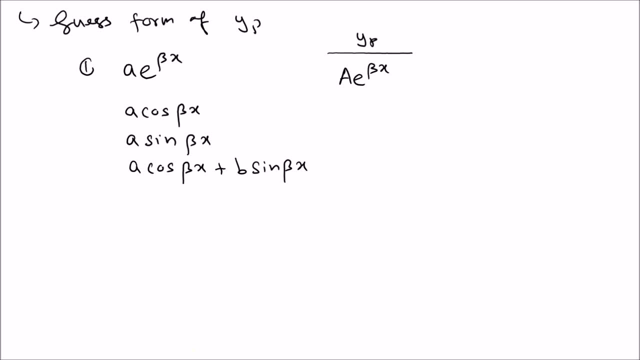 beta x. so here you see that the beta beta. so in this case, all these three has only one form. all these three, if you see any of them, it's going to be simply a cosine beta x plus b sine beta x, even if we have only one, like just cosine. 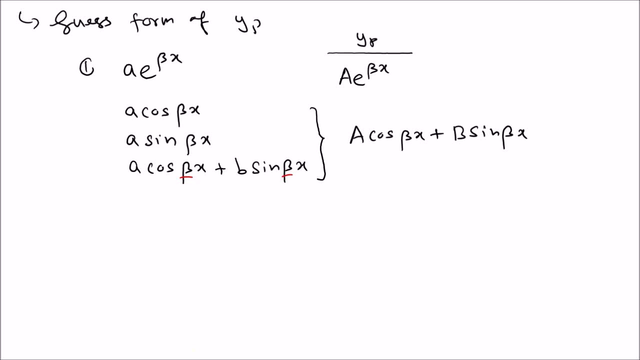 sine, we still need to have two. the reason is, when you take the derivative, it's going to change sine to cosine, so that's why we need to add both. so that's the second type. the third type is a polynomial type, so it is like nth uh degree polynomial. 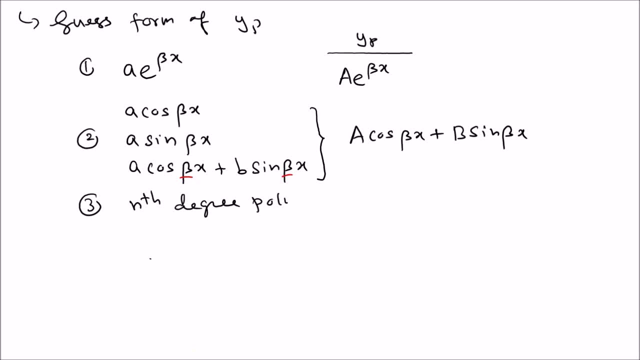 nth degree of polynomial, so you're gonna guess the form as a, say, nth degree. so say a n, x, n, and then, uh, a n minus 1, x, n minus 1. write all the terms and see until a constant. so write all the terms, okay, all term. you cannot miss anything. 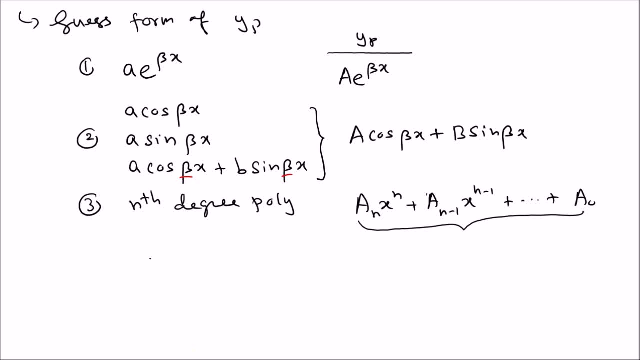 okay, uh, even though the actual function fx doesn't have that, we have, write all of them here, so write all of them. it's very important, good, so that's the kind of idea, so, uh, so let's talk about some special cases, so not, there are some special situations, for example, 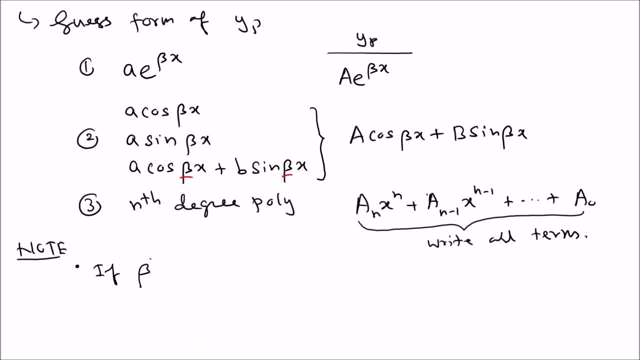 if beta, the rubber, beta, is a root, it's the root of the characteristic equation, characteristic equation of yc, the complementary uh solution, then then yp has to be, then yp has to be a. you have to add extra x in front. so that's very important, because if you do not add extra, 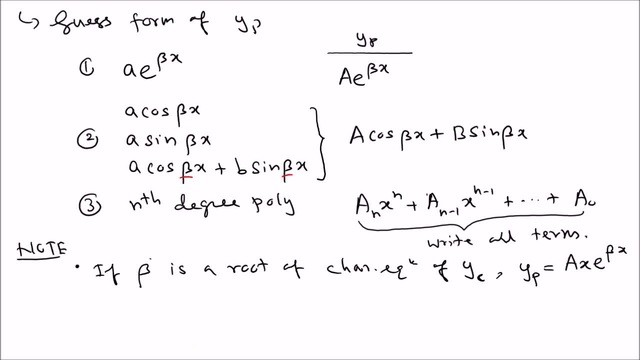 uh x in front. if beta is a solution, what will happen? a e, beta x is a solution, so it just disappears, it becomes zero, so you do not get anything. so that means you have to add a extra x okay together to get to get a uh independent solution. 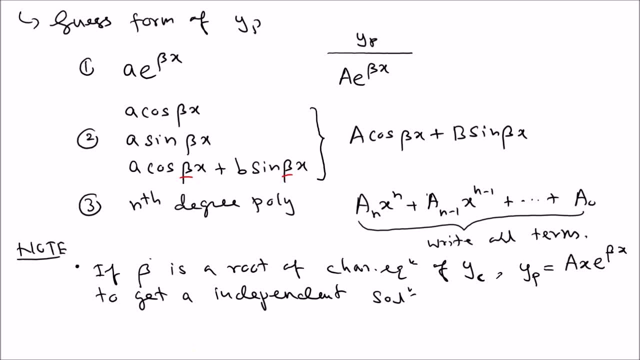 to get an independent solution. it's very important you need that extra x there to get a independence. that happen when beta is a root, ah. and then if beta is a repeater root, if let's say beta is a repeated root, repeated root of the characteristic equation, then you need 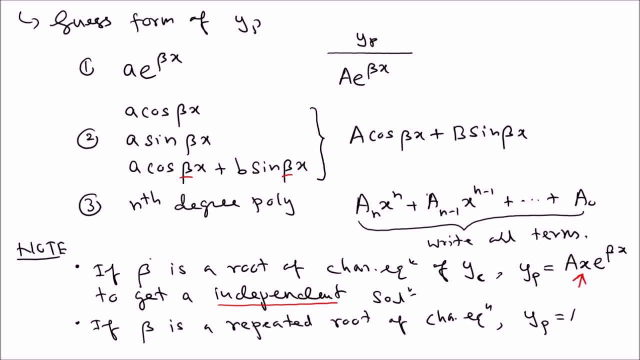 to have another x. so that means there will be a, not just one x. you have one more x or a x squared e beta x. so that's what happens if it's a repeater root, so that means it's a to get an independent solution um. 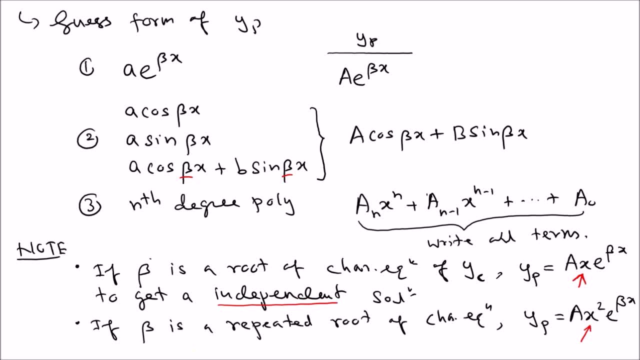 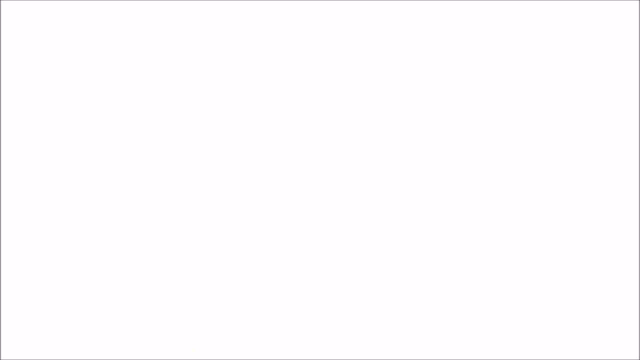 and then the next one is: uh, how about? you're gonna see a combination of the two or three, so let's talk about that. so the next one is: if there's a combination, if there is a combination, if there's a combination of them, write, write a yp for each and combine right yp. 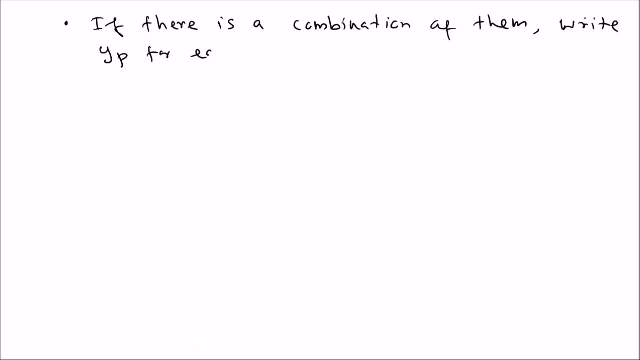 for each and combine. so, for example, let's look at some example of a combination of two cidae, some examples. so let's say, your fx looks like this: uh, 3x minus 2 e 4x like that. so what you can do, you can see that there are two, there's a polynomial. 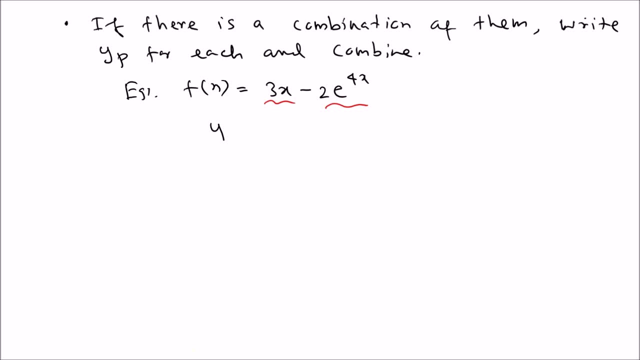 and exponential function. what we can do, we're gonna have both in there. so because of the first degree polynomial, you need a term like ax plus b is the first degree polynomial. that's 4, 3x one. you have c, e, 4x, so we're gonna write for each and combine like that. so 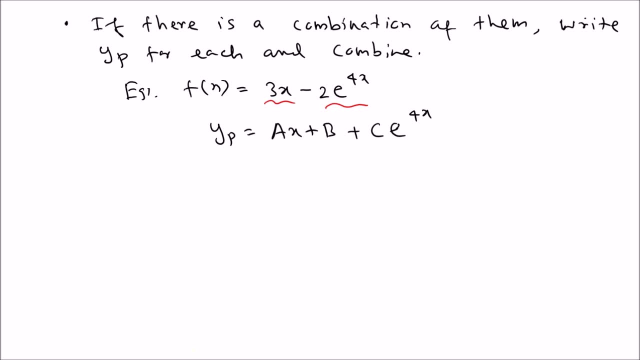 you just write one expression combining both. so that's the idea. it's very simple, uh. the next one is: how about we're gonna see product and like all of them, for example, x, e to the 4x plus sine 3x. so if you get something like that, now the yp. 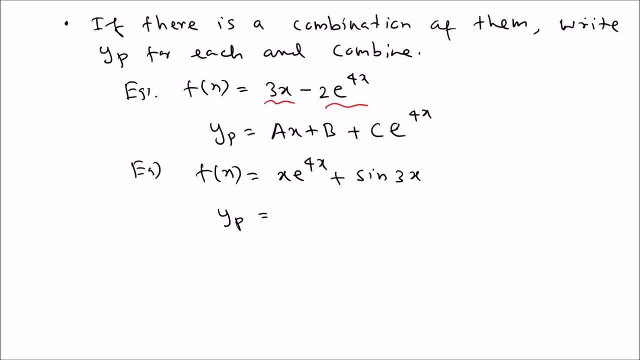 looks like this: so we have x. that means a polynomial, so we write a x plus b for that. and then we have e to the 4x. but for e to the 4x the general term look like c, e, 4x. but there is something here, because a and b already contained c as a. 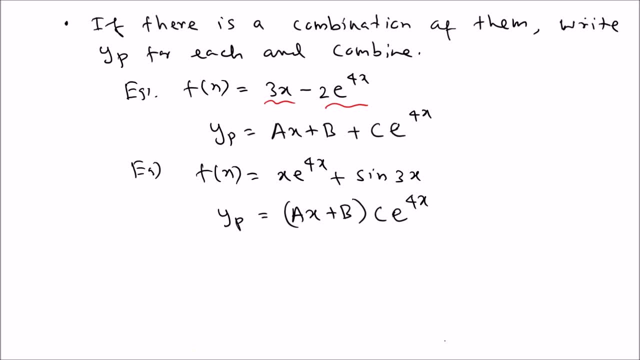 factor. so that means we are write that c here, so we don't write that. we don't include that there because c already containing a and b. so if you add a c, that's extra unknown. so that's going to make it difficult. so we are not going to write that, so we 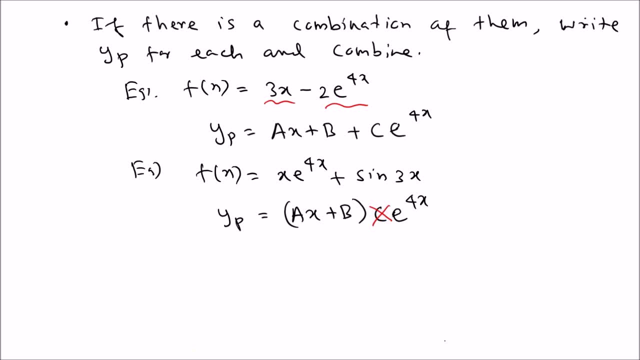 can remove that. that means we, without that. we can write like this: just uh a x plus b e to the 4x, like that, so that that argument always there. if it is already inside as a product, we don't need that extra one. so so that's the first two. 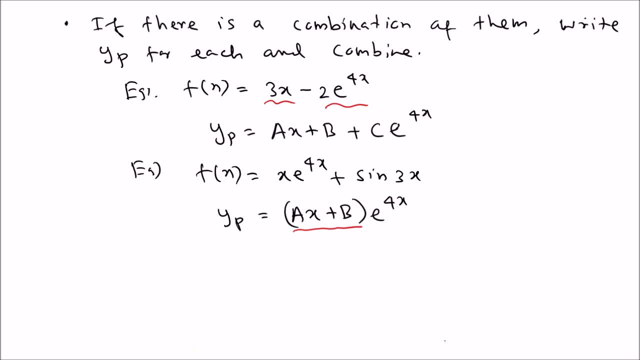 so it's going to take care of x and the e to the 4x. now, sine, the sine is a one term, but we know that you have sine and cosine both. so that means it's a c sine 3x plus d cosine 3x, because if you see one of them, 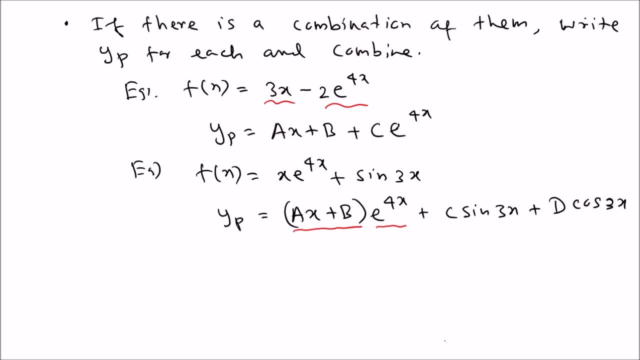 you need to write both. okay, so this automatically come everything good. so that's the kind of idea. so, and then also, let's say you also have an extra term like minus a cosine x. so that means this also going to introduce another two. so that means if you, if you have that, then what's going to happen? it is e. 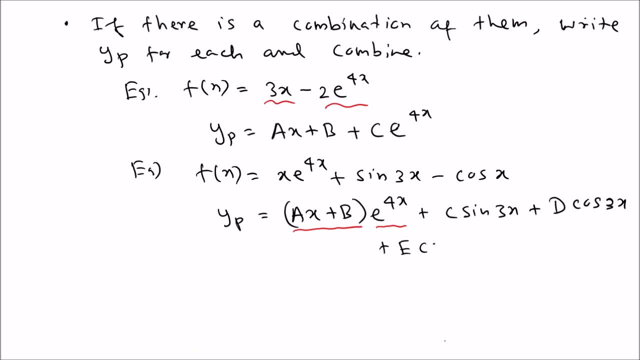 again: uh, sine cosine, it doesn't matter. so write cosine, and also the sine version, f sine. so always go as pairs, okay, so it's it's very important. good, uh, so that means uh, so this is go with that. so that's, that's the first one. 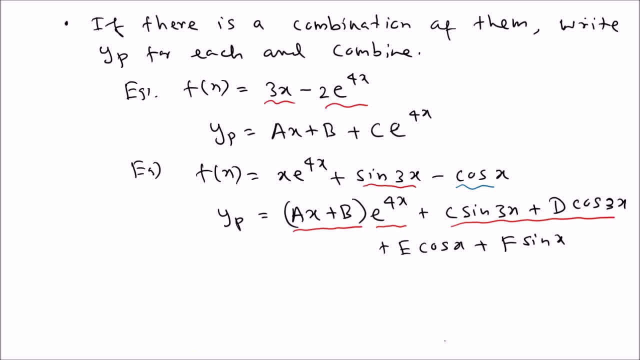 and this one go with that. so that's the uh idea. okay, so i hope it's clear now what happened. uh, the other one that we just discussed before. so let's say, if you, if you have a difference equation like this, let's say you have y double prime minus y prime minus 2. 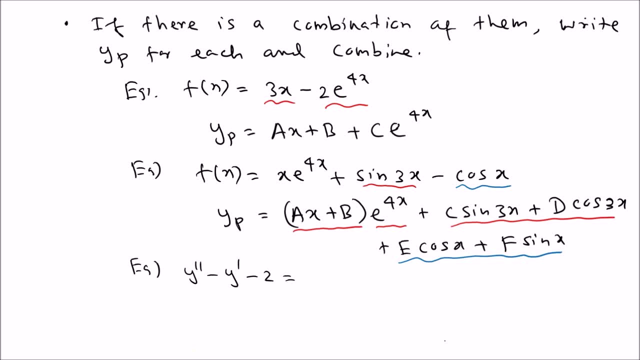 equal uh 3 e 2 x. so if you look at this problem, so if you want to write the form for yp, let's look at their. it's always a good idea to look at the characteristic equation first. if you look at, the characteristic equation is lambda squared. 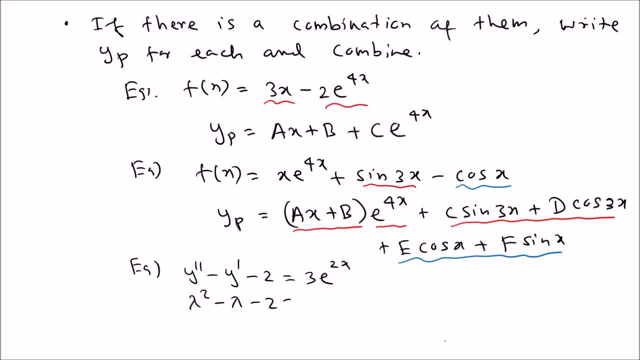 minus lambda minus 2 equal 0. the factors are lambda minus 2 and lambda plus 1.. so this says that lambda equal 2 and minus 1. you don't need to this exactly match with that. so in that case, what's going to happen? 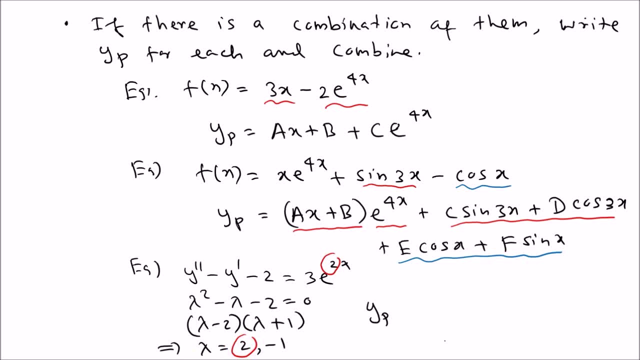 uh, your yp has to include an extra x, so it is a x, e 2 x. the reason is lambda, already appear in the characteristic equation, because if you just have a e 2 x, it's not going to work. the reason is: it's a solution, since the 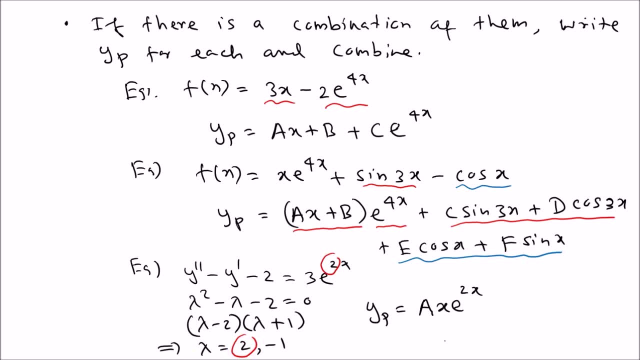 solution. once you plug into the left side, it just gets zero. so you get zero equal something on non-zero. that's not possible. you can have zero equal to non-zero. so because of that, to avoid that, we introduce that extra x to get an independent solution. okay, so to get an independent solution, because we 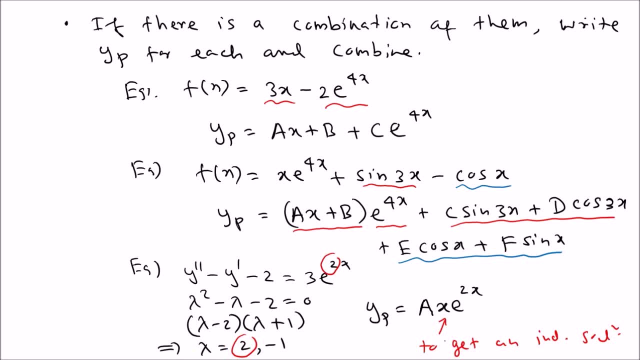 discuss that, because if you multiply by x, it's going to create a new independent solution. so you get an independent solution, okay, okay, so that's the idea. uh, so what we can do now is: uh, let's talk about the, the steps to solve a problem like that. so these: 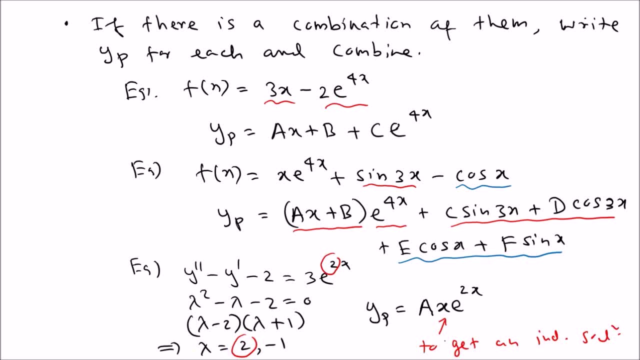 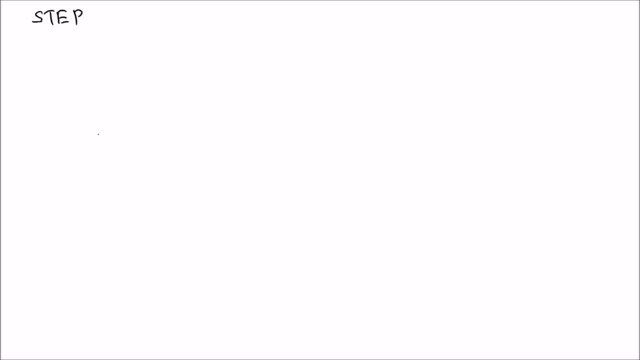 are the steps to solve the problem using undetermined coefficient method. so steps, uh, so the first is: the first step is always going to be fine, yc. the reason is then: it's going to tell you whether the lambda is appeared in the characteristic equation. so we find yc first. 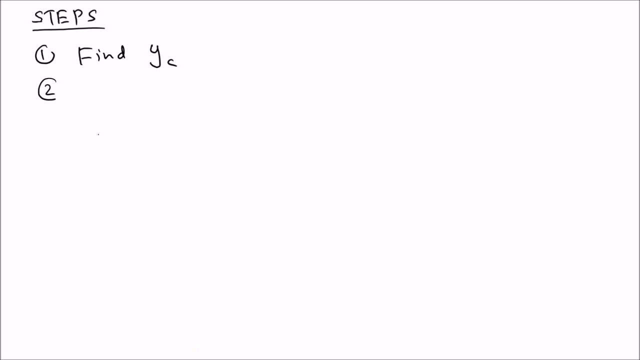 at least the lambda values. that's the first. second step is guessing. why so you're going to guess uh, so guess yp, you guess yp. that's the second step. third step: uh, you can take derivatives. take, uh, enough, uh, derivatives. what does that mean? if it's a second order differential equation, you need two. 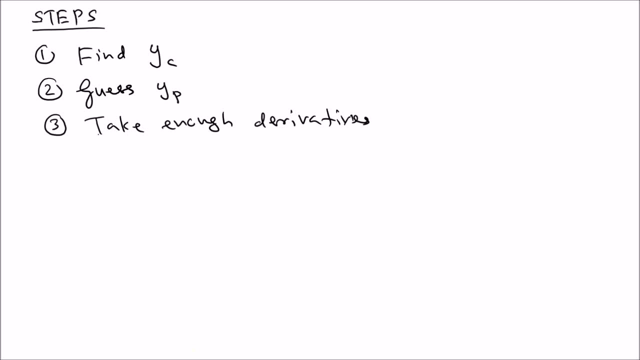 derivatives. it's a third order differential equation. you need three derivatives like that. let's say: enough, okay, sufficient number of derivatives, okay. so it's clear. and then what we're going to substitute the equation. so substitute the equation, substitute into the differential equation at the non-homogeneous one. 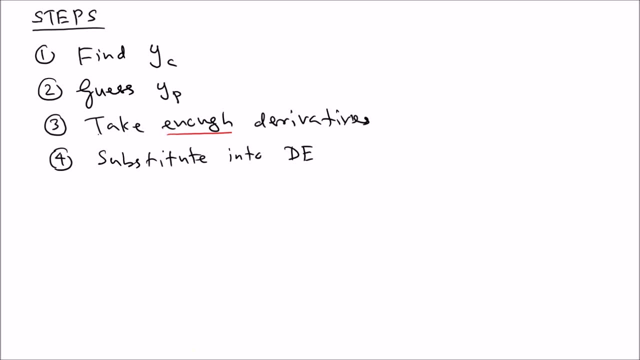 and then we can equate the coefficient of linearly independent terms. so number five: equate coefficients of linearly independent terms, a terms linearly independent terms. you're going to equate the coefficient linearly independent terms and then uh terms to find uh, to find unknown coefficients. 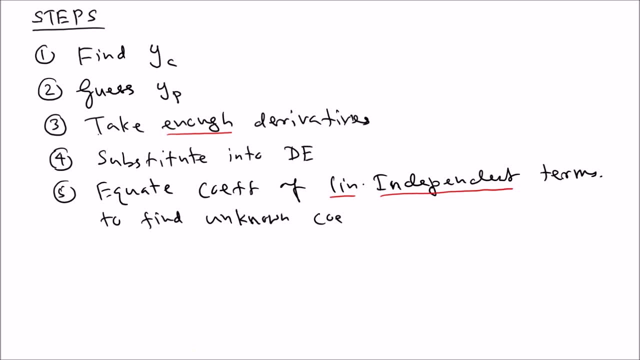 that's how you find unknown coefficient, find unknown coefficients, the undetermined coefficients, and then, after we find that, uh, write the general solution. write the general solution, ah, in the form the c's appeared in yc. okay, use initial conditions. that's the last step. use initial conditions, uh, at the end. 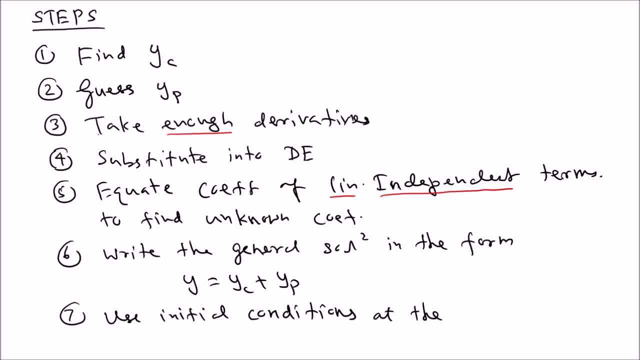 at the end to find c1 and c2. so that's we do the initial conditions and c2. so that's we do at the end. that's the last initial one we use at the end. so okay, so that's. those are the kind of steps to solve a problem using the undetermined coefficient. 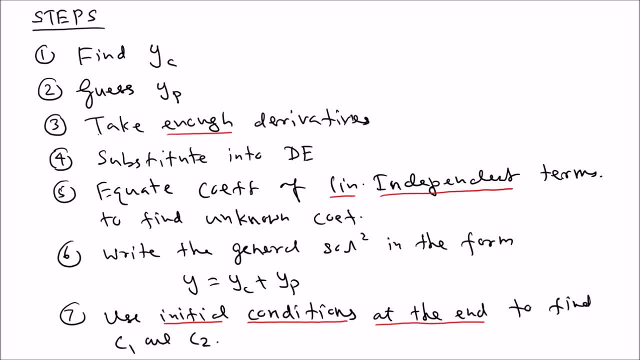 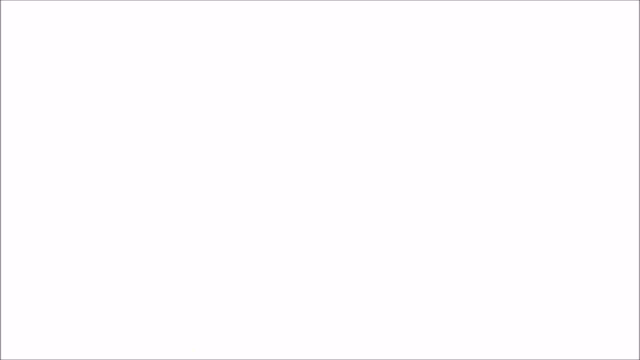 method. so let's just do one example to cover all those things. okay, let's do one example. okay, so let's do this one. so example: solve the initial value problem: y double prime minus y prime minus 2. y equal 6 plus 8 times e to the negative 2 t. 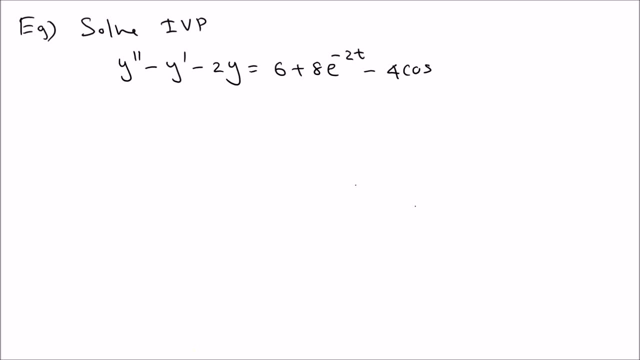 minus 4. cosine 2: t with y 0 equals 0, y prime prime 0 equal 2. so this is a complete second order initial value problem and with a complicated, uh, non-homogeneous term. let's go step by step. the first step is find the characteristic. 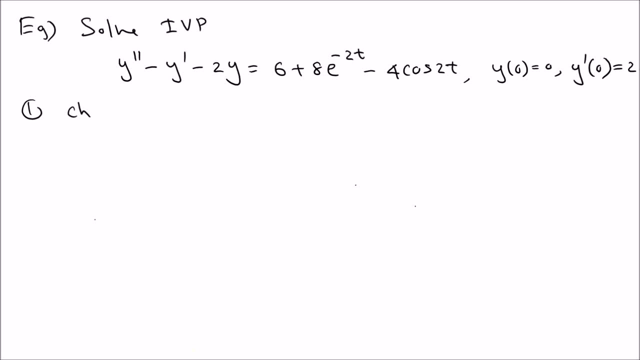 equation. okay, so, uh, the characteristic uh equation of the homogeneous equation by double prime minus y, prime minus 2 y equals 0, is simply lambda squared minus lambda minus 2 equals 0.. the next step is factoring. it's very easy to factor, so 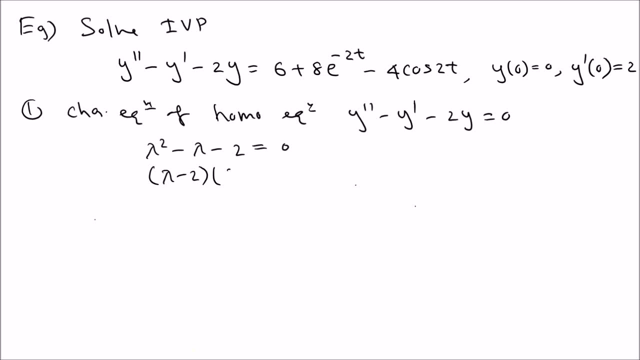 you're going to get lambda minus 2, lambda plus 1. this is going to give you the lambda values: lambda equal minus 1 and 2. so we're going to the yc. so the yc equal c 1 e to the negative t plus c 2 e to the. 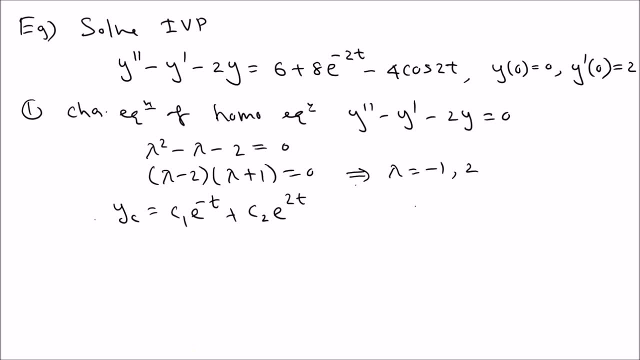 2 t. okay, now you can see that that 2 and that one is different, so that means you don't need that extra t for this one, so we can write the yp. that's why we need that first, to see whether that's the right form. so right. 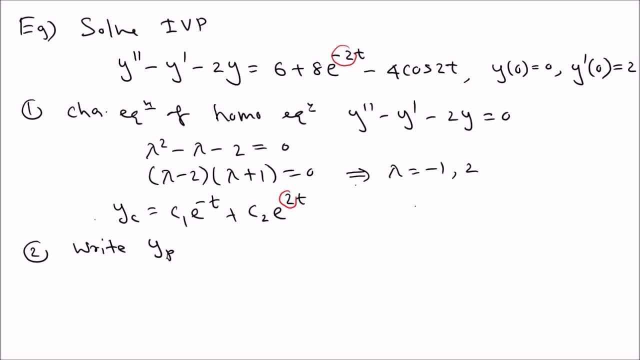 yp. so yp is the right form, so yp is- let's go term by term: 6: 6 is a constant. that means we add a a for that, and then that's the polynomial part, and then we have 8 e, the exponential term. so that is b. 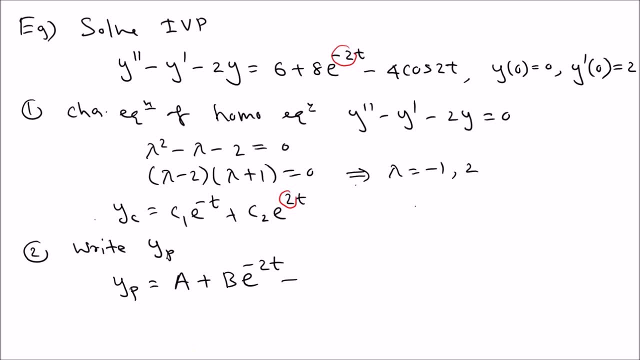 e negative 2 t. and then we have sine cosine, so it's a cosine. so we're gonna go with c, uh, cosine 2 t, and also you need to have the sine term. so that's the rule. okay, good, whether you have two or one, you still need to add two. 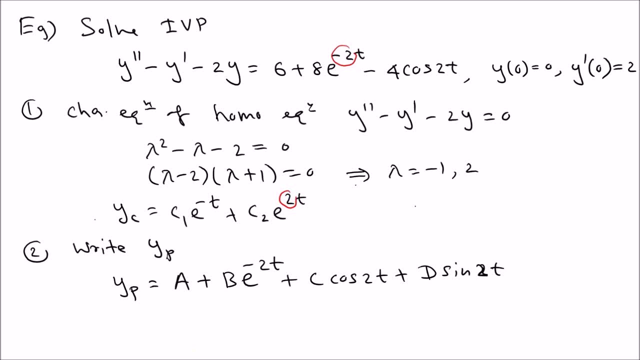 uh. the next step is take derivatives. so number three: derivatives, so you can take derivatives. uh, so we're going to get y p prime. uh, so that's a zero. so you get the exponential function when you have exponential function when you take the derivative. you get the exponential function when you take the derivative. 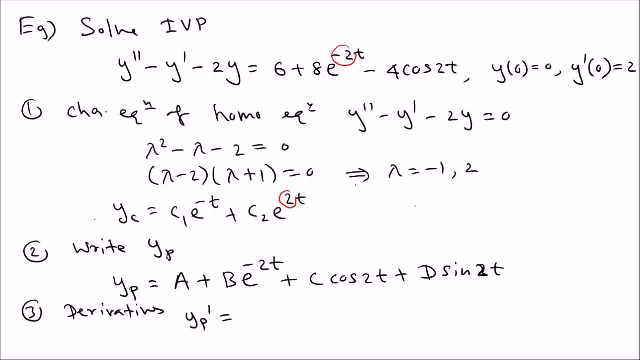 you get the exponential function when you take the derivative, uh, that the constant comes out, that we know. so that means it's going to be negative to b e to the negative 2 t. so that's what you get. from that the constant comes out, and then it's a cosine. cosine is going to take the little is going to be a. 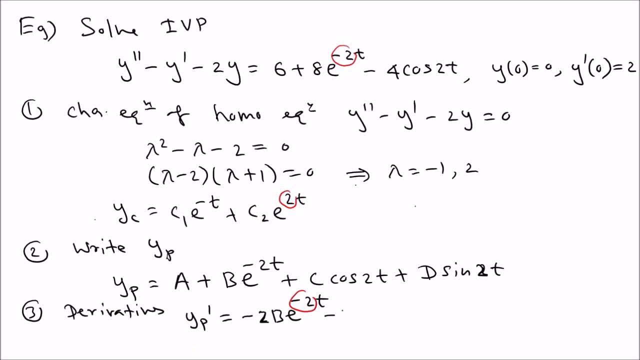 negative sign. also 2 comes out, so it is negative: 2 c sine 2 t. now this is sine, become cosine. 2 also comes out, so 2d cosine 2t. so that's what you give me, the first derivative. now take one more derivative, because the equation is second order. so y p. 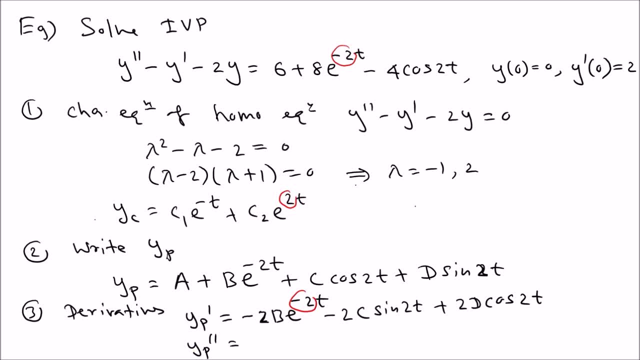 double prime. another negative root comes out, so it becomes 4 b, e. to the negative 2 t sine become cosine. 2 comes out, so the negative 4 c cosine, 2 t cosine becomes sine, so negative: 4 d sine, 2 t. that's what you get. so we get all the derivatives now. 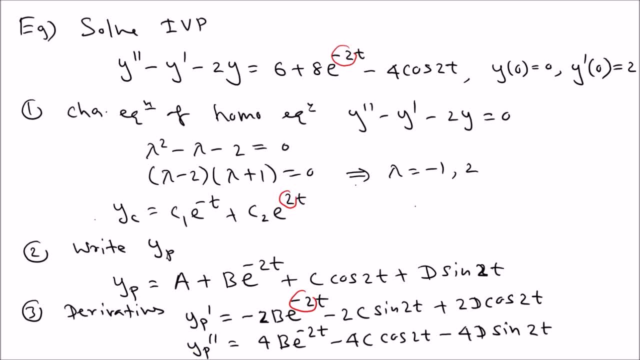 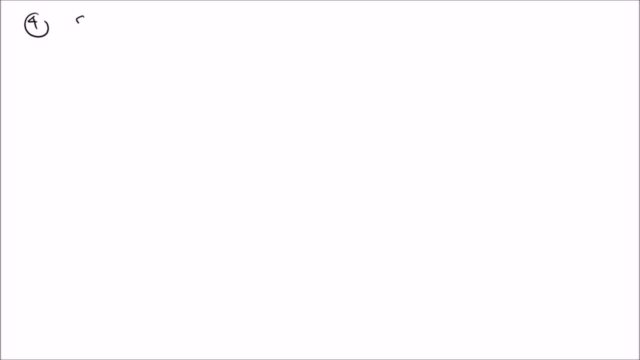 and y p, so we can substitute that into the equation. so let's do that. step four: substitute: substitute into the equation. so let's do that. so step four: substitute: uh. so y double prime, so y double y. so we're going to put the y double plane term first. so if you want, you can repeat the. 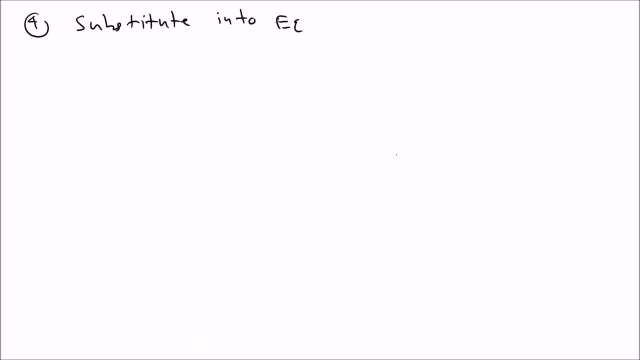 equation here: uh, so it is y double prime minus y prime minus 2 y, equal f t. that's the function we have. so let's put that so y double prime terms first. so it is 4 b e to the negative 2 t, my negative 4 c cosine, 2 t minus 4 d. 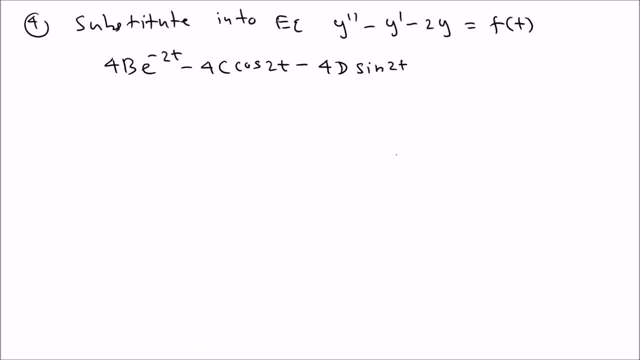 sine 2 t. so that is the y prime term. now we're going to go with the first derivative term. it's a minus. you're going to get negative 2 b e to the negative 2 t. negative 2 c sine 2 t. so that's the y prime term. 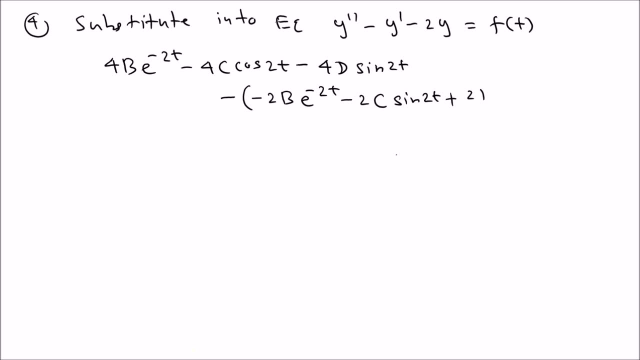 plus 2 d cosine 2 t and then ah, the y term which is negative, 2 times the y term which is a, that's the longest term, 2 e negative 2 t plus c cosine 2 t plus d sine 2 t, which is a negative 2 t. 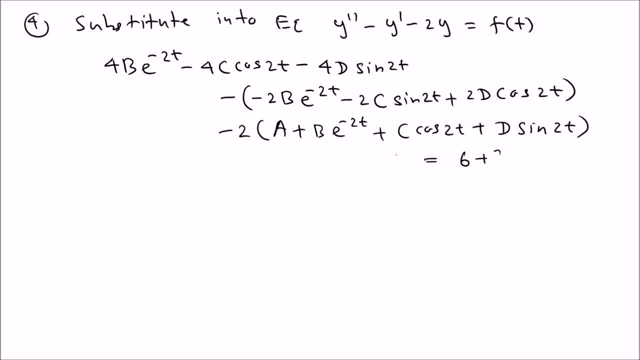 equals to the f t, which is 6 plus 8 minus 2 t minus 4 cosine 2 t. good, so that's the expression we get. now what we can do, we can equate the coefficients of linearly independent terms. so what are the linear independent terms? you can see. 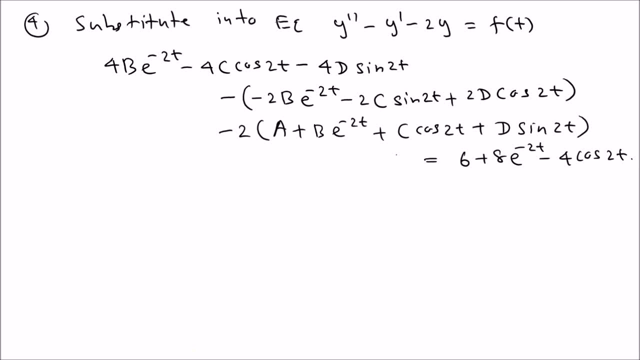 here you have a constant, which is a linear independent term, and then we have our exponential function, which is linear independent. we have sine, which is linearly independent. we have cosine, which is also linearly independent. so those are the four terms that we have here which are linearly independent. so 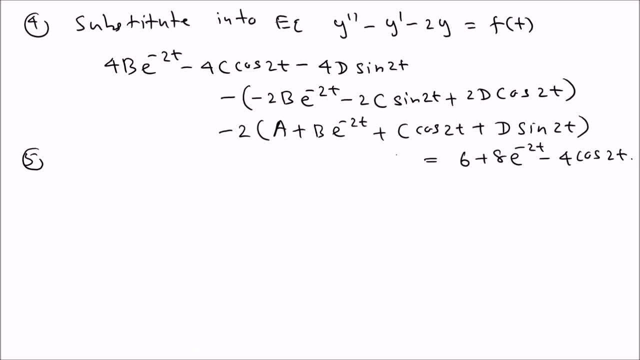 step five: uh, equate. uh, equate coefficients of linearly independent terms. so we start with the first term. we will start with the constant. so start with the constant. uh, you're going to see a is a constant and that's the only term we have. and then other side 6. so we're going to equate those two. so we have negative. 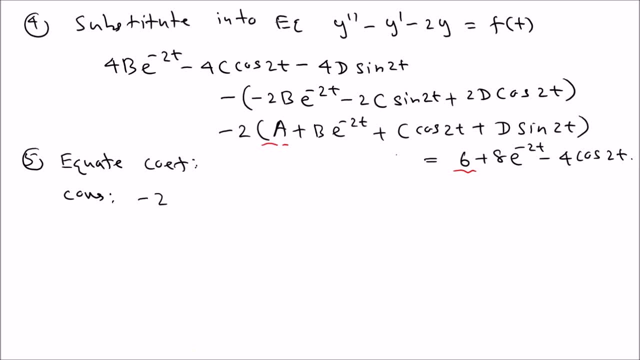 2 a equals 6. this directly going to give a, a has to be negative 3, so we all know the a value, same thing. let's go to uh, exponential function next. so e to the negative 2 t, so you equate the cohesion of that. it was also any independent term. 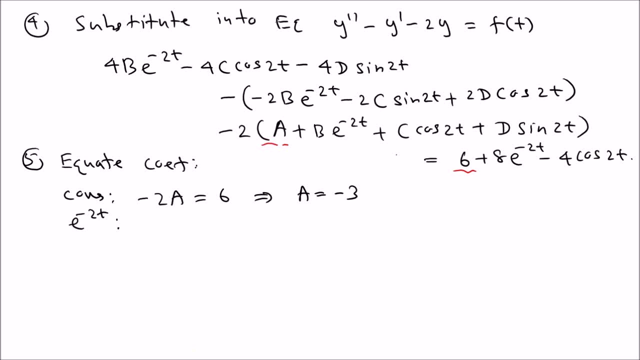 so let's start with that, so you can see, we have that uh e to the negative two t, and then we have this one and we have that one, and on the other side we have this. so those are the uh four terms that we have. so three on this side, three on the other side. so we 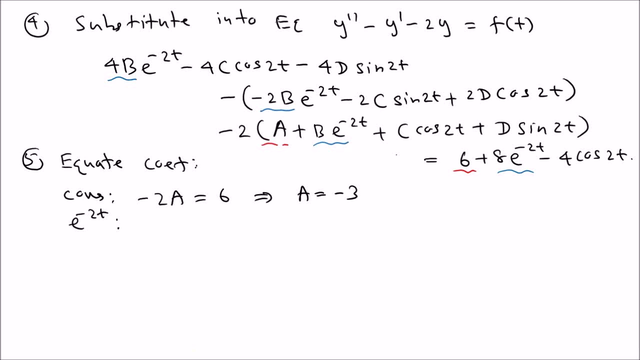 have 4b, and then we have negative, negative positives, two negative positives, two negative positives, and then we have uh, negative, 2b, uh good, and then equal. on the other side we have 8.. so how this simplifies. you can see this and that get cancels. 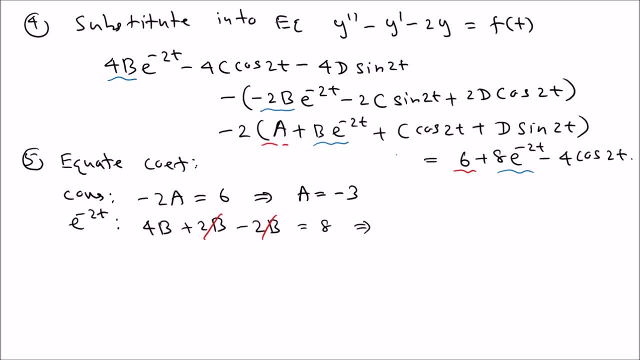 so you will get 4b equal 8, in other words, b equal 2.. so we already know a, we all know b. now the only thing that we need to do is, uh, find the coefficient of sine and cosine. so let's go with one of them. so let's go. 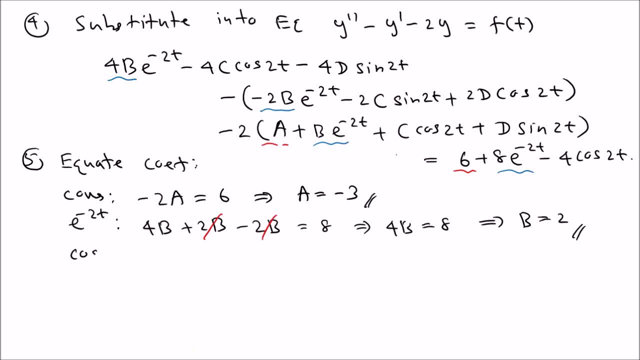 with cosine 2t, so they are all also linear independent. so if you go with that, we have cosine term here, we have cosine term there, there and then this. so those are the four terms, so let's go with one by one. so the first one is: 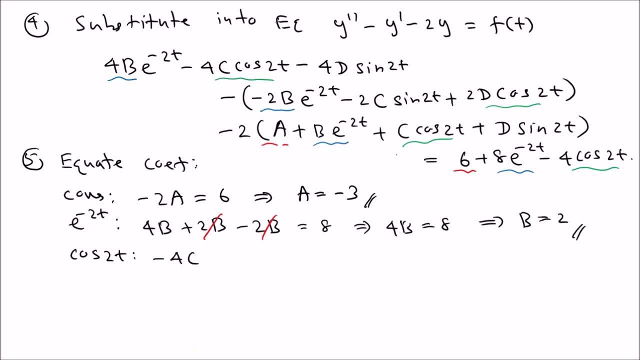 negative 4c, the next one is negative 2d, the next one is negative 2c. those are all the terms on the left side, equal, the right side, negative 4.. see whether you can simplify this a little so you can see negative 4c to negative 4d. 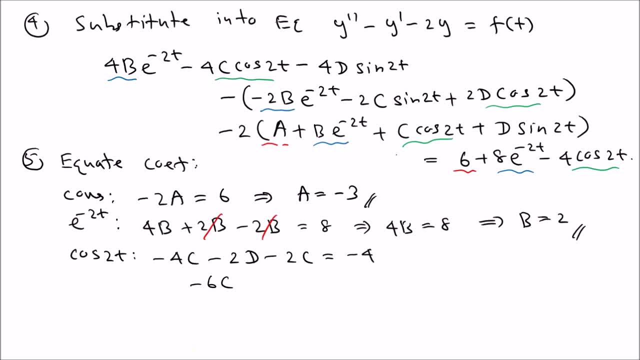 negative 6c. so negative 6 c minus 2d equal negative 4. what we can do is we can divide this sum by negative 2. if we divide this by negative 2, you're going to get equation uh 3c plus d equal 2.. so i'm going to call this: 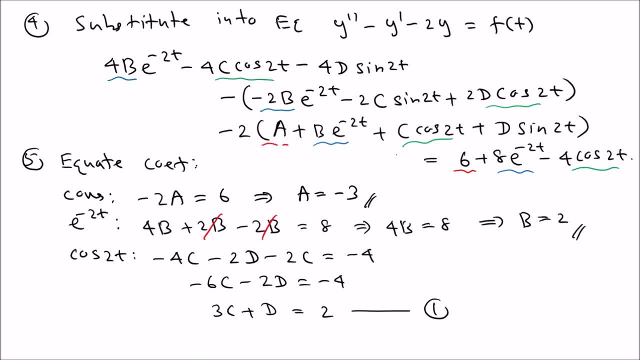 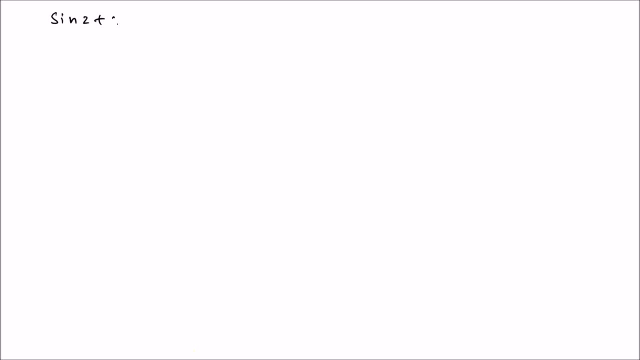 equation number one. now what we can do. we're going to create a similar equation for uh sine 2t and solve the 2.. so let's see what you're going to get for sine. for sine, we have a sine 2t, we're going to get negative. 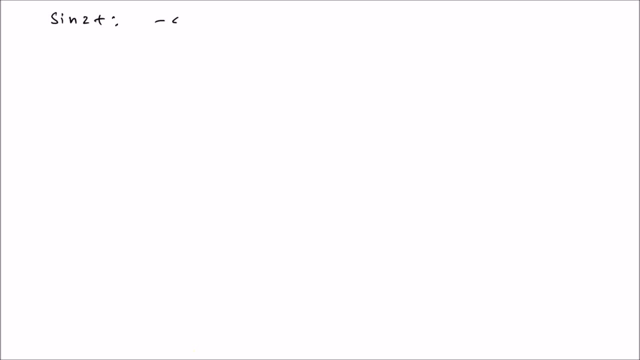 4d and then plus 2c minus 2d equal 0. we just know sine term. on the side this simplifies to negative 6d minus 2d. so we have negative 4d plus 2c equals 0 and if you divide this by: 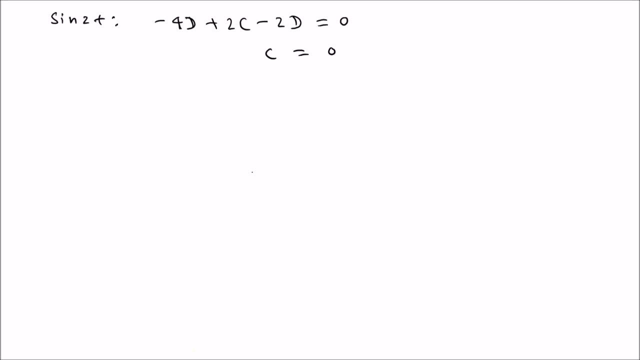 okay, i'm going to write it here. so this is going to give you negative 6d plus 2c equals 0. if you divide by 2, you're going to get c minus 3d equals 0.. i'm going to call this equation number 2.. 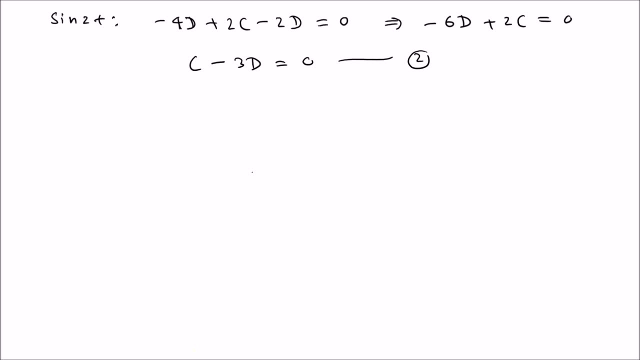 so now what we're trying to do? uh, we can simply get rid of d term by. so i'm going to multiply the first equation by 3 and add to the second equation. when you do that, you're going to get 9c plus c minus plus 3d, minus 3d, which is equal to 6. 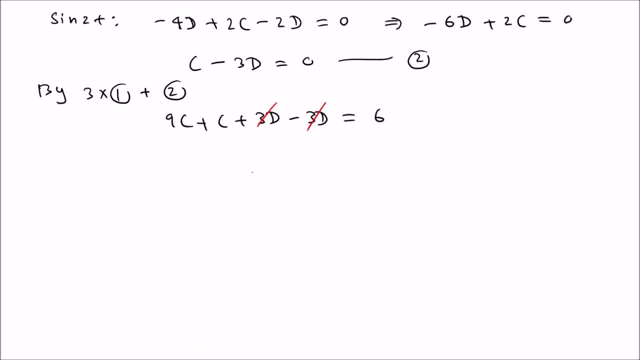 and you can see this gets cancelled out. so you're going to get the value of c. so 10c equal 6. it says that c equal 6 over 10, in other words 3 over 5. ah, and then we can use: uh, the second equation. 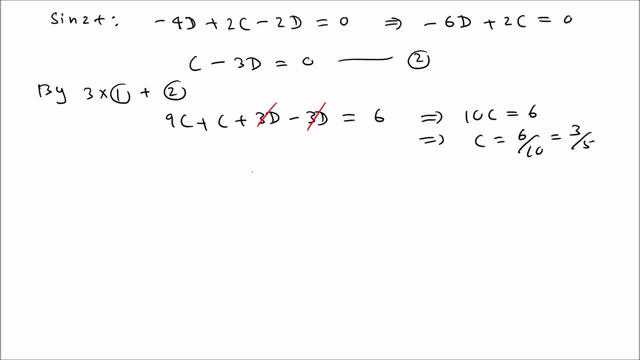 so this is one third of that. so this says that d equal one third of c, which is one fifth. so we find the two third, one third of that. now we can write the general solution. so thus the yp, now the general solution. yp is negative 3 plus. 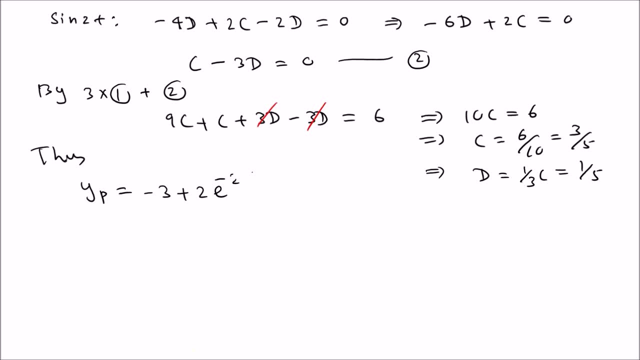 2 e to the negative 2 t plus three. fifth cosine two t plus one. fifth sine two t. so we get all the terms. now what we can do, uh, we can add the general solution, so number six, the general solution. so the general solution is y equal y c plus y p. uh, so you can substitute, is c 1 e to 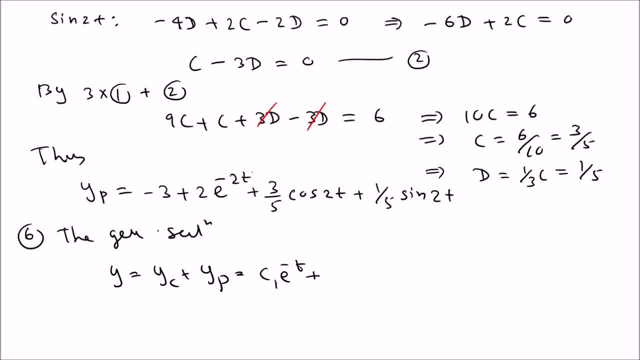 the minus t plus c 2 e to the 2 t and then minus 3 t. let's add them plus 2 e minus 2 t plus 3 5 cosine 2 t, my plus 1, 5 sine 2 t. so in the exam, like you know, you're not going to. 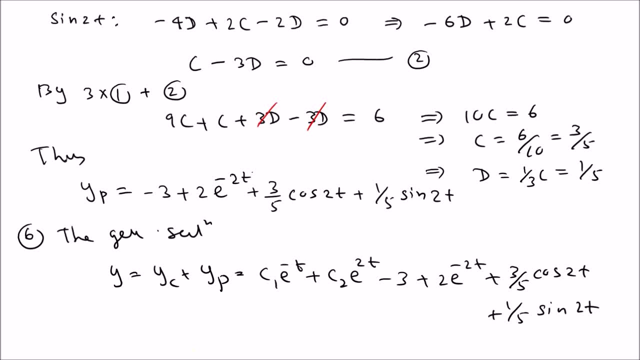 get a question like this this long. but here i'm telling you like you can manage all of them together, but you will get like one or two terms, not like a lot like that. okay now, the last step is now we can use the initial condition or to find c1 and c2, so you can see. 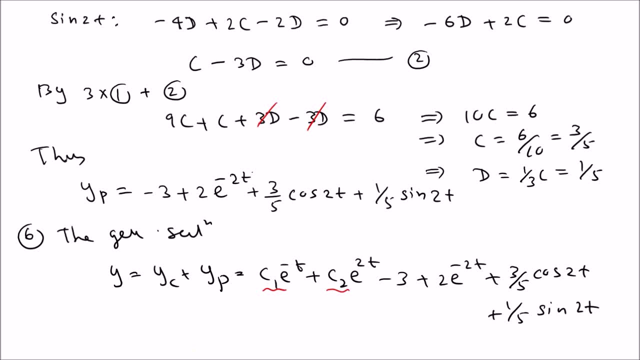 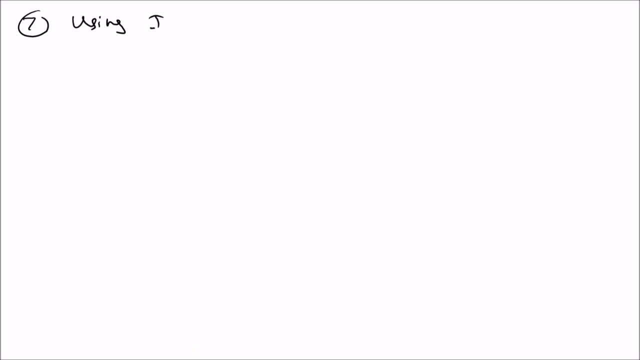 that the only thing that we don't know is c1 and c2. to find that, uh, we can use the initial conditions. so initial conditions we use at the end. that's what you remember. so the step 7 are using the initial conditions. we have y 0, so 0, which is y 0, that means you plug in 0. we have a. 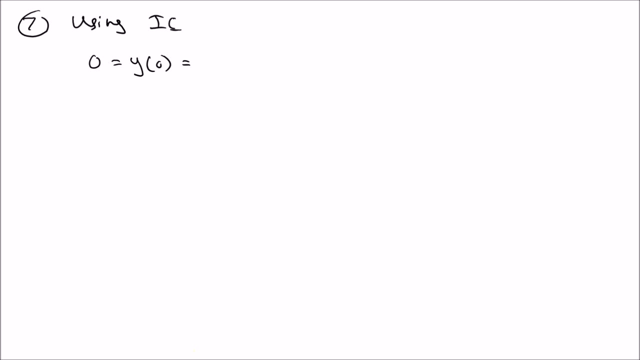 uh, so you're gonna get. uh, what are you gonna get? so let's write a separate equation for that. yeah, i'm gonna write it like that. it's much easier like that. uh, you've seen, initial using initial condition: y 0 equals 0. we have 0 equals c 1 plus c 2. 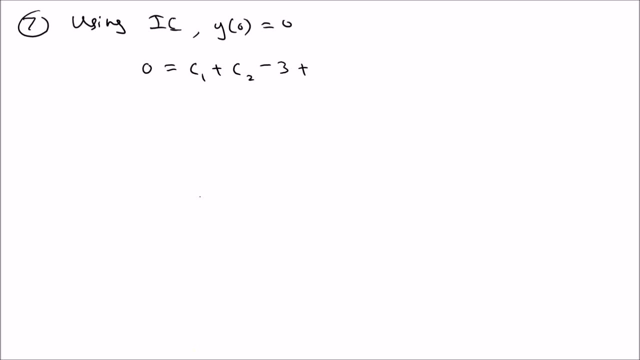 minus 3 plus 2 e 0 plus 3. 5th cosine 0 plus 1. 5th sine 0. now we know that sine 0 is 0, cosine 0 is 1 e 0 is also 1, so this is going to give you an. 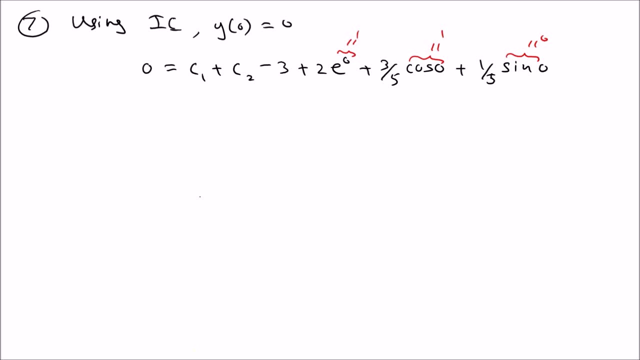 equation. so what, what equation is going to give you the equation you're going to get? you're going to get 0 equals c 1 plus c 2, uh, c 2. we have, uh, what we have? we have minus 3, uh, and also we have three. 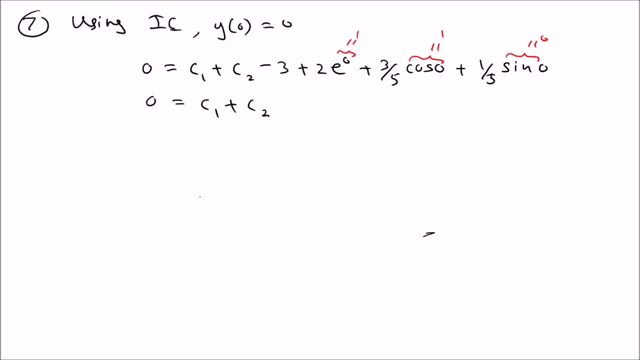 minus three and we have two here, so it's a minus one plus three fifths. that means minus two fifths, let's certificate. so i'm gonna call this equation number uh. 3, because we already have one and two. number three, because we already have one and two. 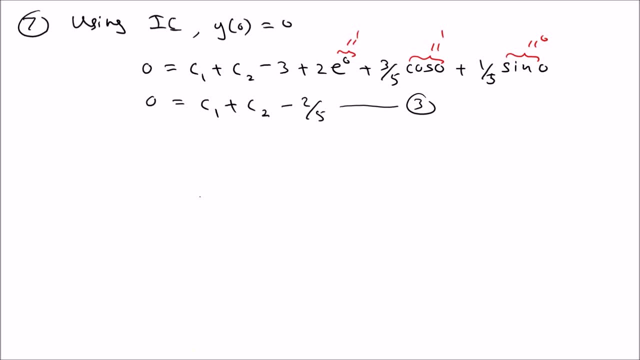 now the same thing. let's try to use the other conditions so you get one result here. now first we take in derivatives. taking derivatives first, are we going to get y prime t equals to negative c, 1 e to the negative t plus 2 c, 2 e to the negative t费 plus 2 c. 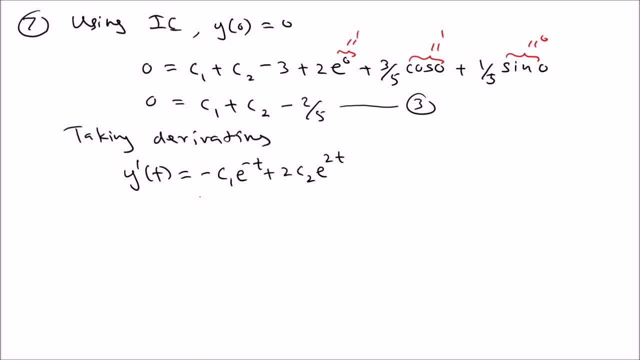 plus 2 c 2 e e to the negative t plus 2 c 2 e to the negative t plus 2 c 2 e e minus 0 minus 4 e negative 2 t minus six. fifth uh sine 2 t plus 2, 5th cosine. 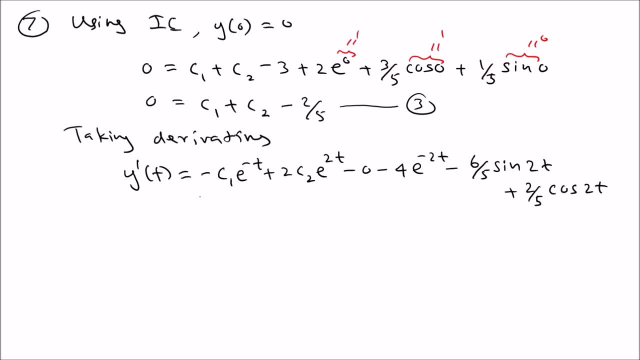 2, t. and now what we're going to do? we're going to use the condition uh, using y prime zero equal 2. we're going to get this equals to negative: c 1 plus 2, c 2 minus 4 and the negative 6. 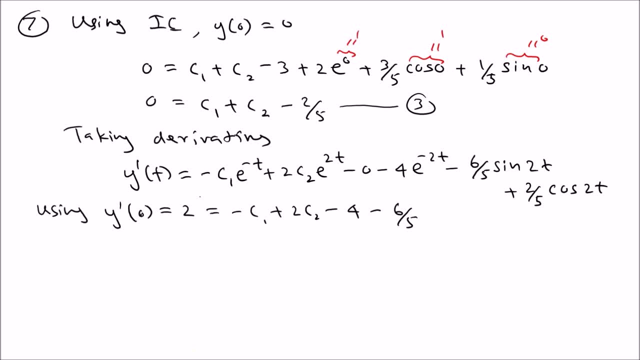 5th sine is 0, so that's gone plus 2. 5th cosine: 0 plus 0. okay, so if you plug in the values, because again this is 0 and this is 1, you're going to get a few more negative for the other side. 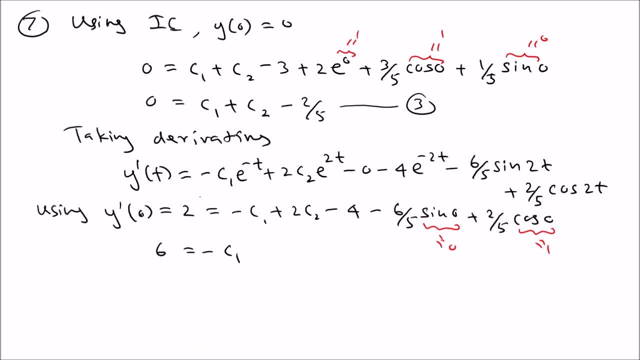 6 equal negative c 1 plus 2. c 2 plus 2. 5th, i'm going to call this equation number 4.. now what we can do, we can add them. once you add them, this is going to cancel out. you get c. 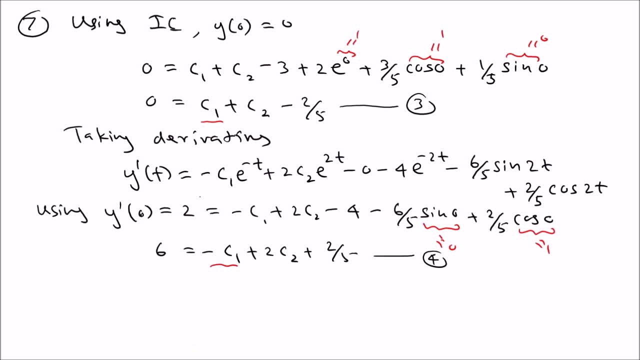 2. so let's do that. and also, you see, this is negative, this is positive, they cancel out also. so that's interesting. so by 1 plus 2 we have 6 equal 3, c 2, in other words, c 2 equal 2, and then you can use the equation number. 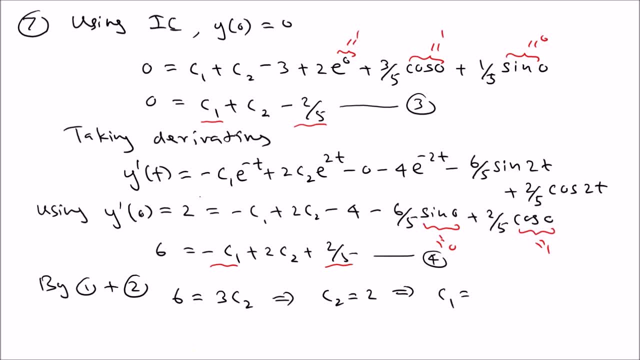 1 and then you can use one of those equations. so let's say c 1. if you use the first equation, c 1 equal negative c 2 plus 2, 5th, and we can plug in so it's negative 2 plus 2, 5th equal negative 8 5th. 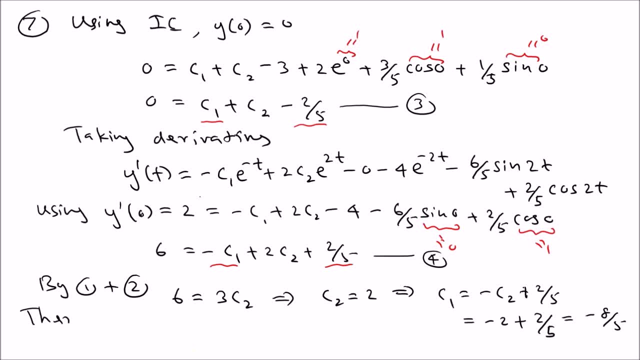 so we get the solution. so therefore we have the solution: y as negative 8 5th e to the negative t plus 2 e 2 t minus 3 plus 2 e, negative 2 t, and then 3 5th cosine 2 t plus 1 5th sine 2 t. 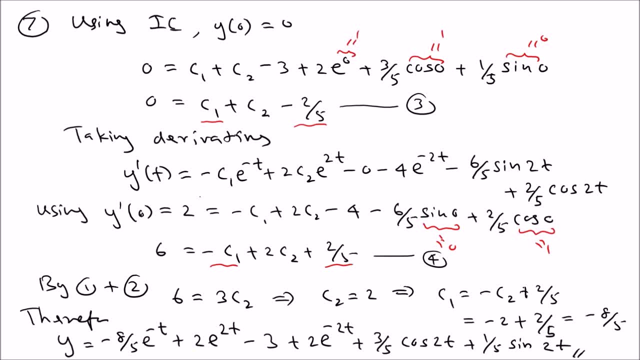 you can see that none of the terms are zero. that's very interesting. okay, so that's the solution. so it's just like a writing few terms, but otherwise it's not that difficult. uh, but you want to make sure that you kind of follow the pattern against the proper, uh. 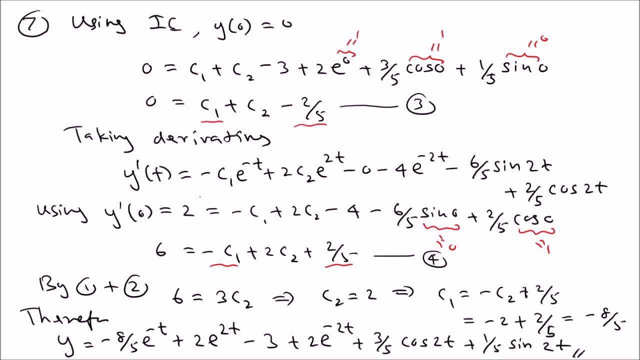 yp term and then after you get the general solution so you can see, the most lenders part was to find c 1, c 2. otherwise the problem was not that difficult. the finding c 1, c 2 was not that difficult. takes time because of a lot of terms. but if i say 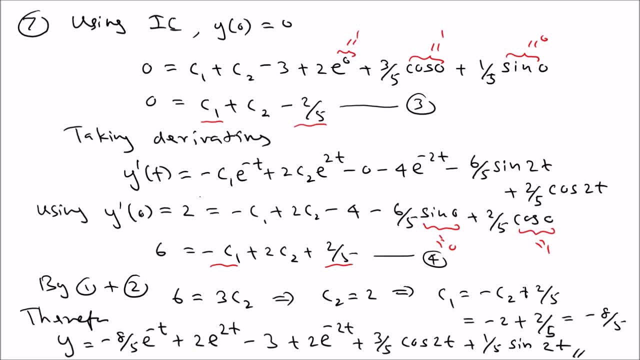 find a general solution. it won't be a very difficult problem. okay, yeah, let's expect something like that. good, so the next topic is the uh variation of parameters and the last. that's the last one we're going to talk about in this, this part of the review, uh, in the next one we're going to talk about the series. 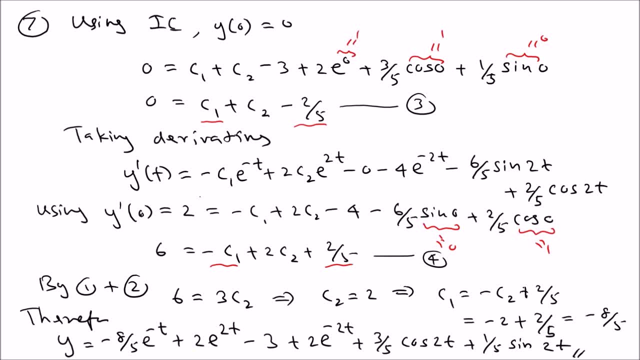 solution, laplace, transform and the system of equations. so the only thing we are discussing this one is the uh variation of parameters. but that's the that's easy one because you're allowed to use the formula. so i'm going to discuss the formula and the technique, so let's talk about that. 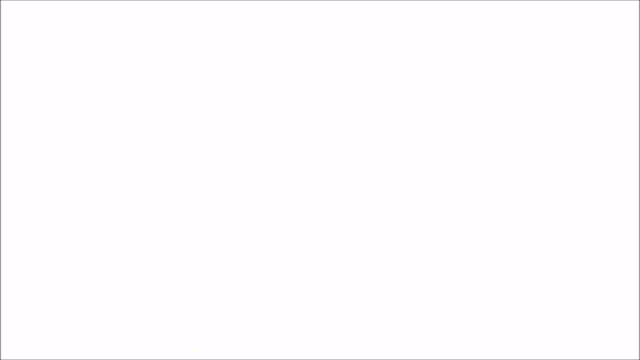 so let's talk about the last topic, the variation of parameters uh method. um, so, this is 22 uh, the variation of parameters. variation of parameters method. we know that the undetermined coefficient method only works for three cases, so the problem is, what if you have something else? uh, so we can use a variation of. 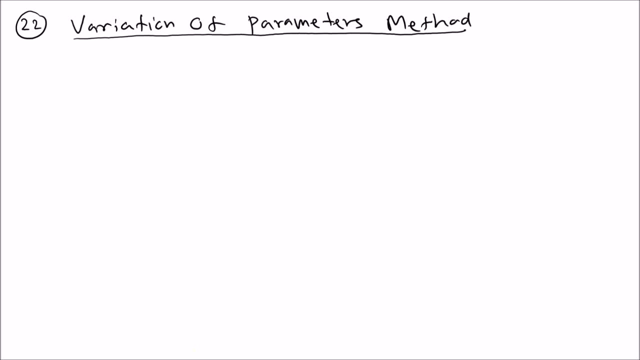 parameters in those, those cases. so this is a little bit more powerful than the undetermined coefficient problem. so why we use this one? we use this one to find the find, find, yp, the particular solution of uh y double prime plus p, x y prime plus q x, y, equal fs, we. it's the same problem but it has to. 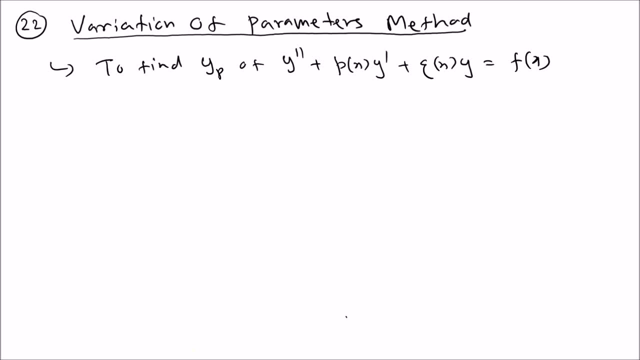 be in the in this form, so we write that standard form. okay, if it is not in the standard form, you have to bring it to standard form first. so these are the steps. so let's go with the steps, okay, uh, so the first one: find. uh, two linearly independent solutions find. 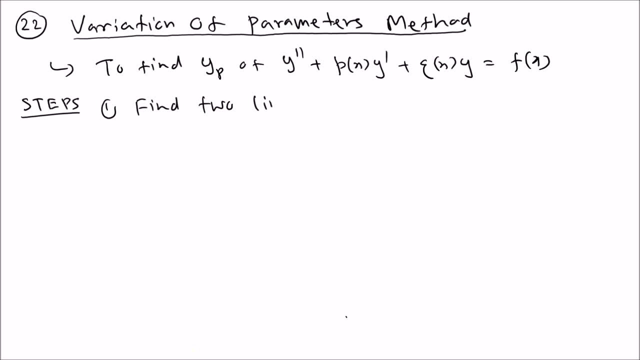 two linearly independent, find two linear independent solutions of the homogeneous equation: y double prime plus e x, y prime plus q x y. so so we have to solve this first. uh, so it can be constant coefficient, or maybe, uh, koji euler. so that's the first thing. 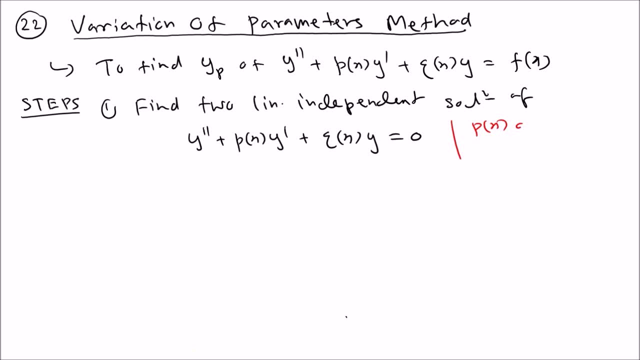 and then also, uh, the p x and q x may be, no need not, maybe a constants, maybe constants, okay, so that's the first. you find, uh, two solutions, so let them be so linearly independent. so, uh, and then let them be, let them be y1 and y2, so let's call those two. 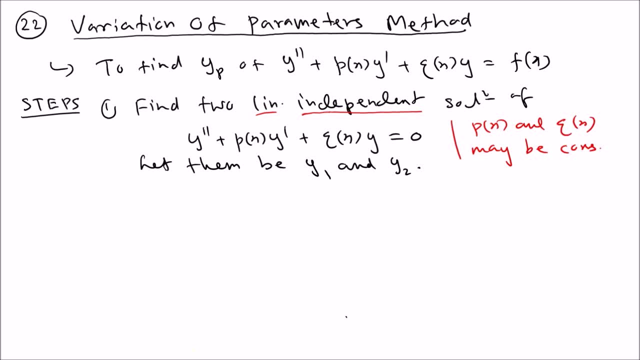 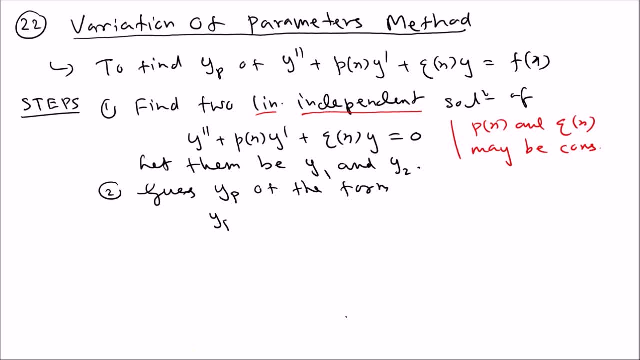 form guess: yp. of the form ypt, of the form yp, u1, y1 plus u1 y2, y2. so for the non-homogeneous, we have a one, one other, one other term. if you are the homogeneous, it's only u1 by one. 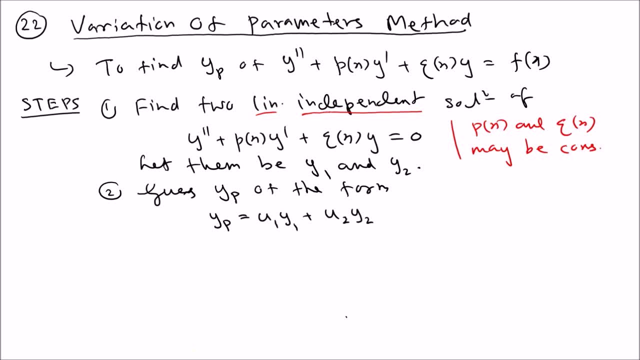 but when we have non-homogeneous, we add one more term. so the goal is to find this u1 and u2. so that's the goal: how to find this u1 and u2. so we now need to find our, take the derivatives and plug in to the equation and uh, get to uh. 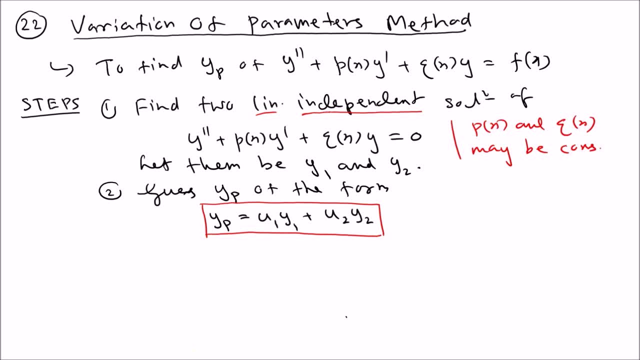 two equations to solve for u1 and u2. so you can see where, uh, we are. u1 and u2 are unknown functions, are where u1 and u2 are unknown functions, so we need to find those two. okay, so the goal is to find u1 and u2. uh, so what? what's going to? 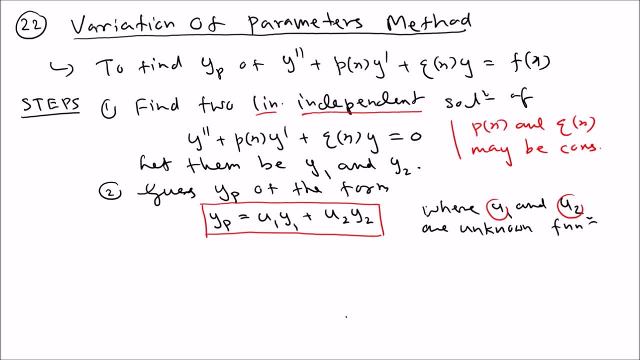 happen when you plug in. you're going to get uh, so i'm going to skip the other part. so we're going to get end up with these two equations. so we're going to solve the two equations. solve the two uh equations. so we're going to solve the two equations. 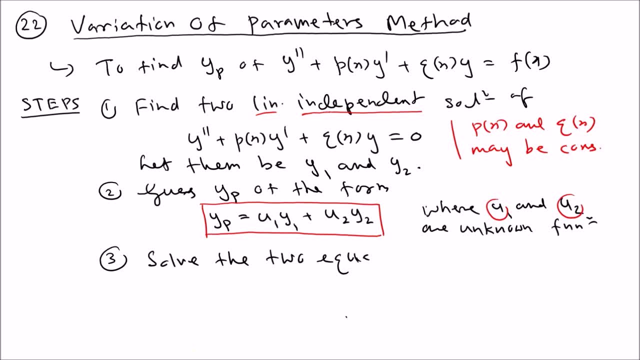 solve the two equations. so the two equations to find u1 and u2. what two equations? these two? uh, it is u1 prime- y1 plus u2 prime- y2 equals 0. that's one equation. the other equation is u1 prime- y1 prime as well, plus u2 prime- y2 prime. 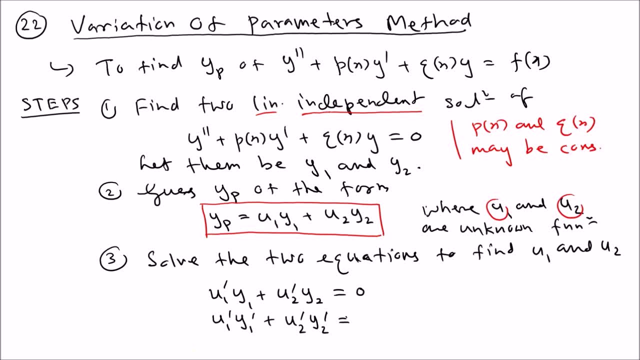 u1 prime, y1 prime as well, plus u2 prime, y2 prime equal the function fx, so we can solve these two equations. uh, that's always the case. you're going to end up with these two equations. so the goal is to solve these two equations and find u and u2, and then, after you find u and u2, you're 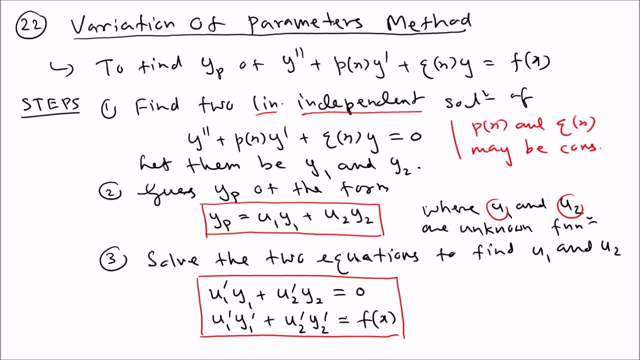 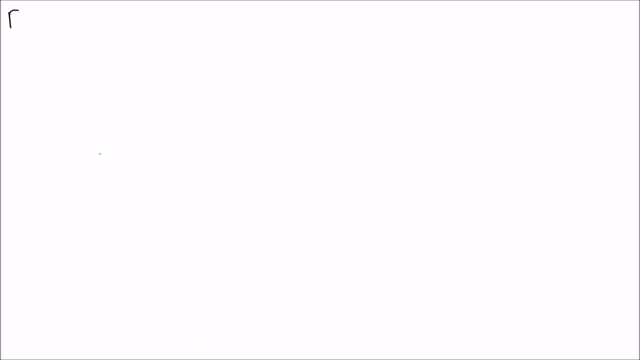 going to plug in here. you get yp, so that's how you find the solution. so let's use this thing to solve the two equations. so we're going to go ahead and solve it by using the undetermined coefficient method. now what we are going to do is we are going to give us the idea of a looks like. 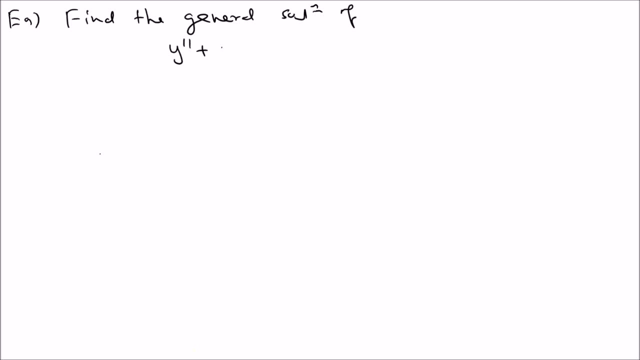 find the general solution of find the general solution of general solution of uh, y double prime plus a fraud, or y double plus or z equal tan x. so if you have this equation you cannot do uh. you can solve this using undetermined coefficient, because tan doesn't work. 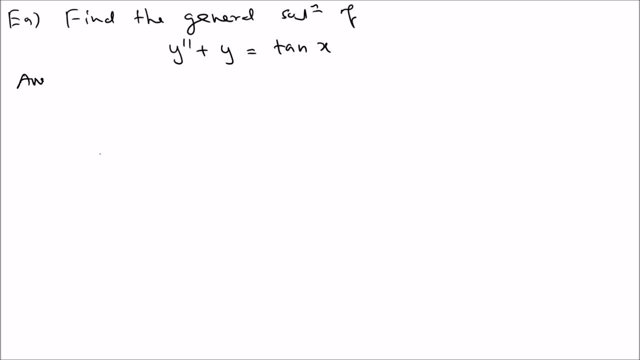 so the uh problem. so what we're trying to do is just try to find the two solutions to linearly independent solution of the homogeneous equation so that we can do very easily uh, the, the characteristic, uh, the characteristic equation, uh, of y double prime plus y equals 0 is lambda square plus 1 equals 0.. 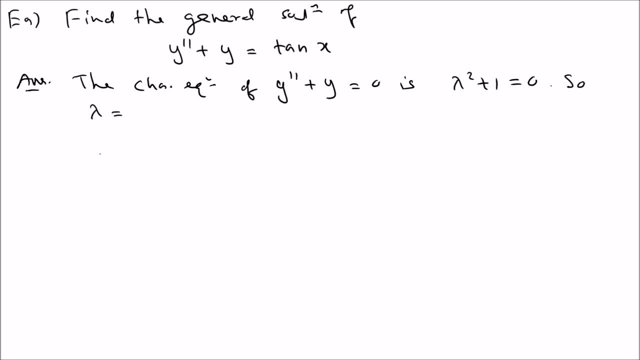 so, lambda, equal plus or minus i, which you can write as 0 plus or minus i. so thus, using the constant coefficient argument, you don't get the exponential term, you only get the sine cosine terms. so that means y c has the form c 1 cosine x, plus c 2 sine x. now what we can do, we're going to pick. 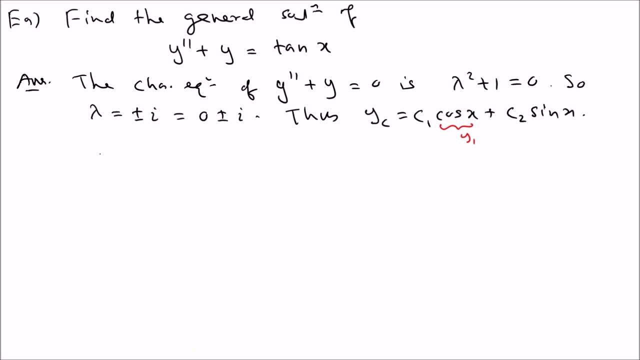 these two functions as y 1 and y 2. the order doesn't matter. so let y 1 equal cosine x and y 2 equals sine x. so let's pick those two functions. uh, now, what we can do is now we're gonna. ah, so suppose. 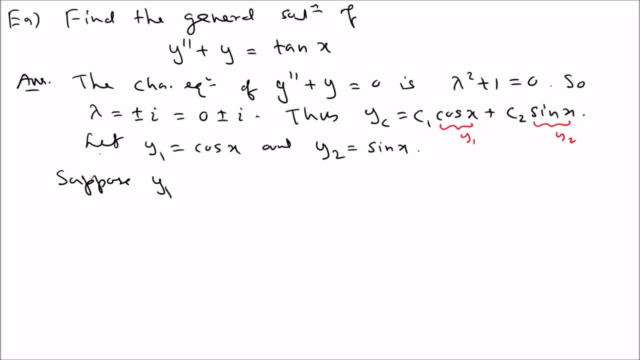 i assume y p of the form u 1 y 1 plus u 2 y 2, in this case y 1 x 1, u 1 cosine x plus u 2 sine x. now we can take derivatives then. uh, from the equations, the two equations we're going to get, 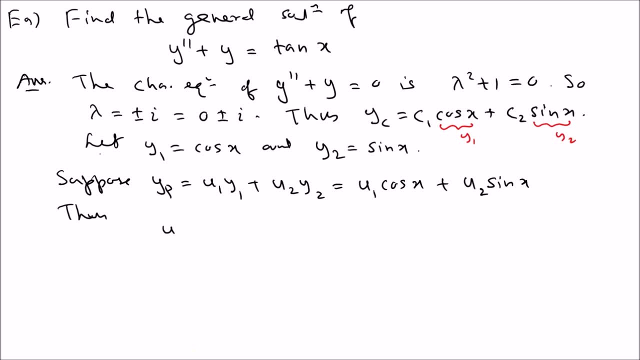 u 1 prime cosine x plus u 2 prime sine x equals 0 as the first equation. the second equation says: u 1 prime, take the derivative. so once you take the derivative of cosine it is negative sign. so it is negative sine x. plus u 2 prime cosine x, we take the derivative. 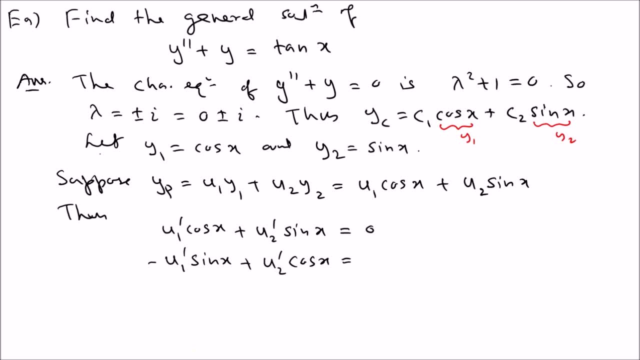 which is equals to whatever on the other side. so in this case, tan x. so those are the two equations that we need to solve, one and two. now we're gonna think of how to solve, why we're going to use the elimination type of argument. uh, you can use the elimination type of. 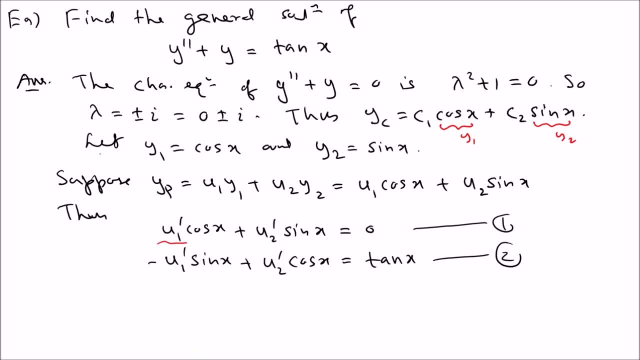 argument. you can see, you can eliminate u one term easily. what we're going to do, we're going to multiply by the missing term and add them. it's going to go away. so that's the kind of idea. so let's do that. so simply by. we're going to multiply the first equation by sine, the second equation by: 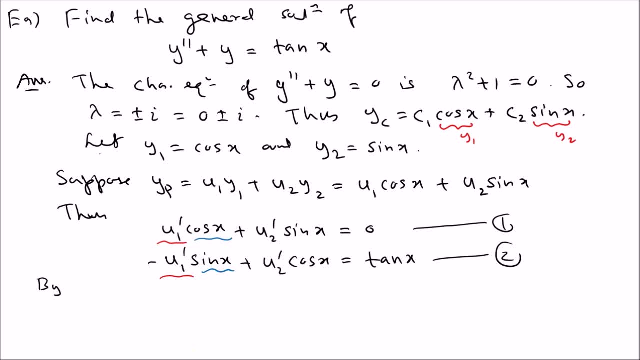 cosine, because those are the missing term. we multiply these two and add them, so you're going to go away so by 1 times sine x plus 2 times cosine x. if you do that, when you add them, this is going to go away. on the other side, what will happen? 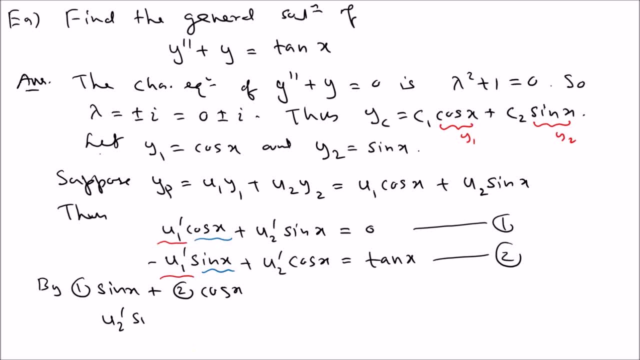 are you going to get u 2 prime sine squared x plus u 2 prime cosine squared x, equal. so the bottom one you multiply by cosine, so it is tan x times cosine x. uh, which is what is the tan means the sine cosine is sine x, so which is equal to sine x, if you. 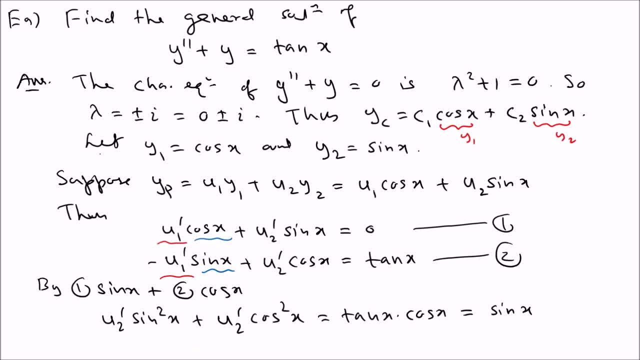 simplify. and here what's going to happen? uh, you can see, this is one, so you're gonna get simply u 2 prime. this is sine squared x plus cosine squared x, which is equal to sine x, but this is one, so this implies u 2 prime equal sine x. now what you can do? you take the integral. 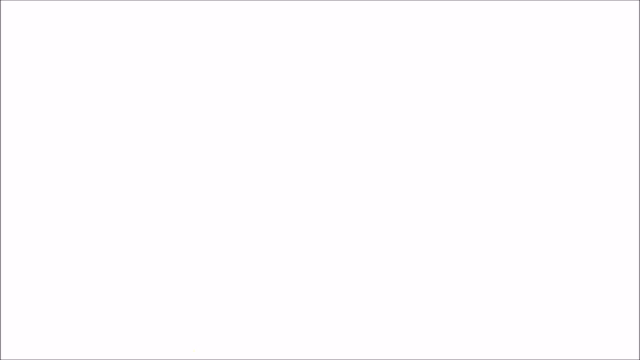 integrate, so u2 is simply the integral of u2 prime dx. uh. so that means uh. you just integrate that, so that is sine x dx. that means negative cosine x, so that is u2. now by 1 by 1 you have u1 prime cosine x plus. 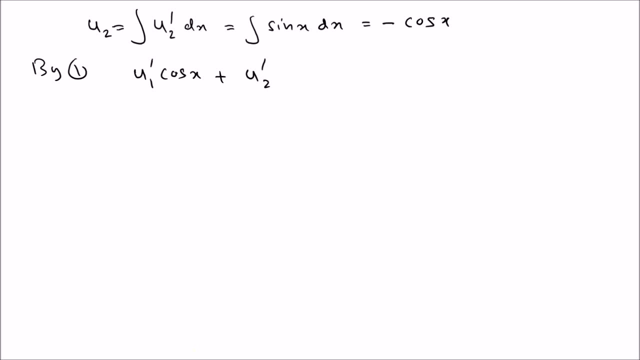 u 2 prime sine x. so if you plug in you're going to get u 1 prime cosine x plus sine x. that's the derivative of negative cosine times sine, which is equals to 0. that's i says now if you look at the last equation. 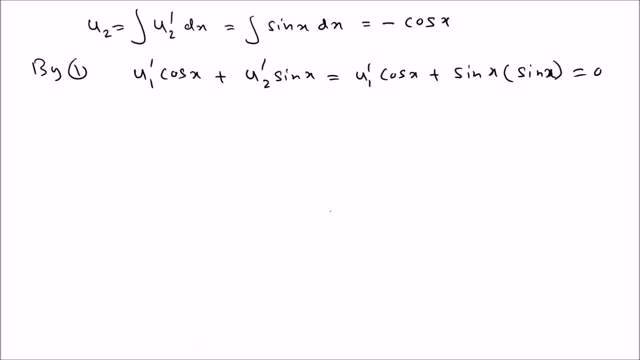 the last equation is power minus sinx, which says that u 1 prime is sine squared, so negative sine is squared divided by cosine x. that's how you get now what we can do. we have to think of how to integrate this work. so what we can do is we can write the: 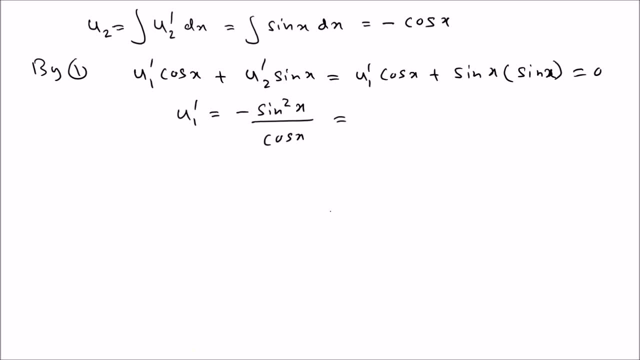 top. as cosine squared x minus 1 over cosine x is, you can split it as cosine x minus 1 over cosine means secant x, so that means it's very easy to integrate. so, uh, u 1 is the integral of u 1 prime dx. uh, so let's integrate the two separately. 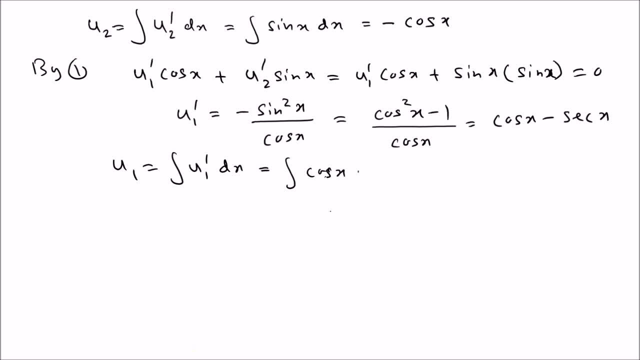 so cosine x dx minus the secant x dx. and we know the cos cosine cosine means the sine x, so that's the easy part. uh, and then uh, so we have uh minus. we know that the secant secant means natural log, secant, tan, secant x plus tan x. that's the formula. 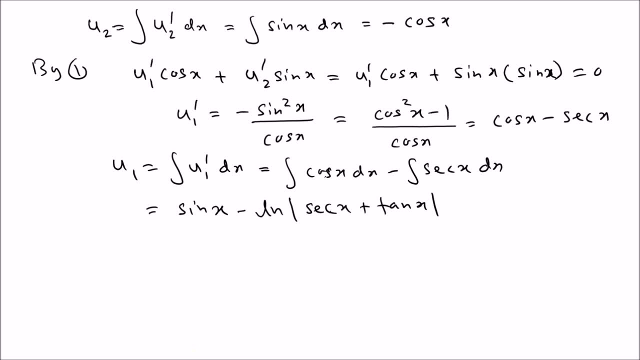 from calc 2.. uh, we are going to add c, so calc 2. okay, so that's a. that's a formula. so that's the formula from calc 2. you know, the secant, uh integral of secant is sec ln, secant, tan. that's a formula. okay, so now we have that. 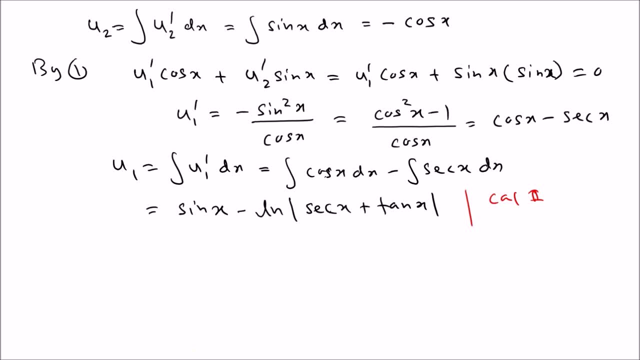 so that means we can write the solution now: uh. so the yp is simply u 1 y 1 plus u 2 y 2, which is equals to cosine x times sine x minus uh minus ln. secant, x plus tan x plus u 2. uh u 2 means negative cosine. 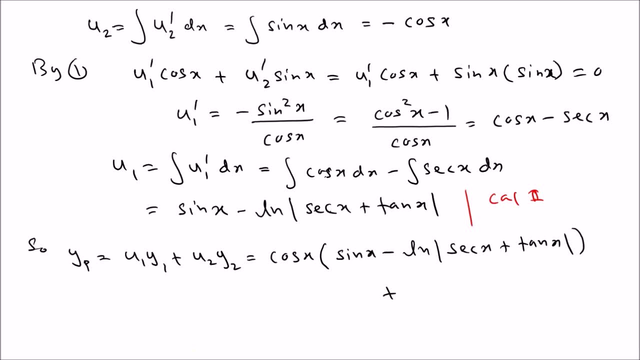 uh, so it is sine x times negative cosine. now you can see that this and that get cancelled, so you only get the last term, uh, which is the last term. so that means the yp is negative cosine. x, ln, c, can x plus tan x. so the general solution. 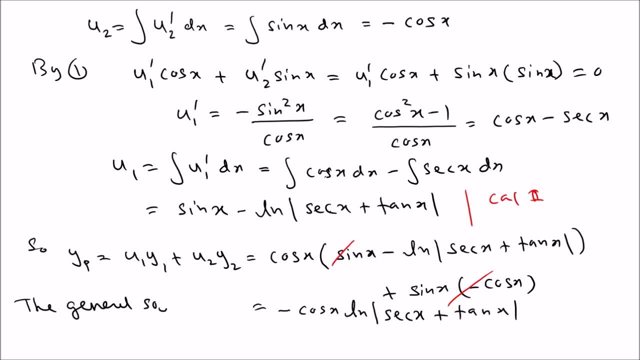 the general solution is: y equal y c plus equal y, c plus y p, c. 1 cosine x plus c, 2 sine x minus cosine x, ln secant x plus tan x. okay, so that is the general solution, which has two constants, c1 and c2. good, so that's. 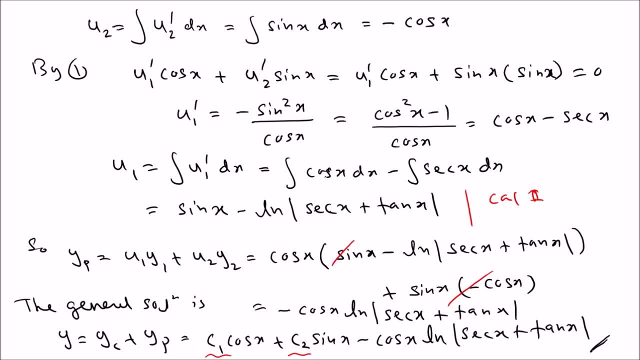 the kind of idea how to use the various parameters method. uh, you're gonna write the two formula, two equations for u1 and u2 and this: uh use the elimination method to remove one of them and solve for one, and then use one of those equations again to solve for the other one. uh, 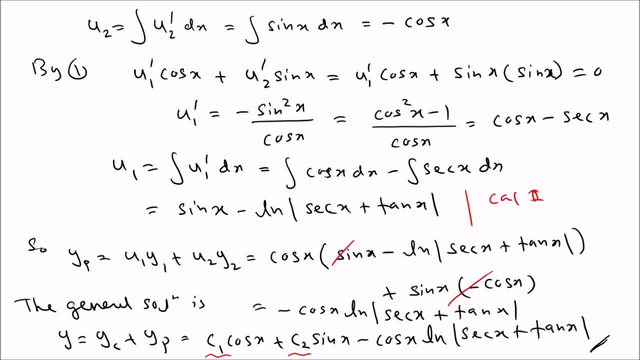 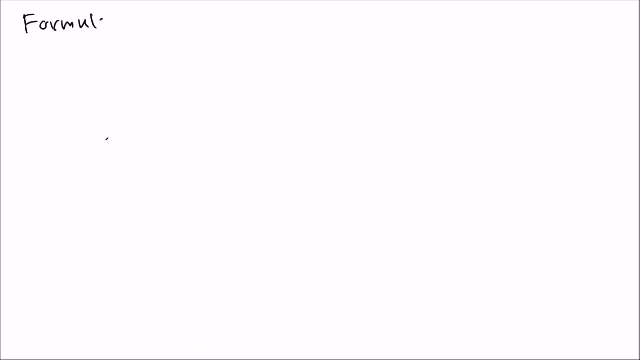 the variation of parameters also has a formula, so let's discuss that. and you are allowed to use that in an exam. so let's talk about the various parameters formula. so, uh, it's a formula, a formula for uh, variation of parameters, variation of parameters method, so let's talk about that. uh, 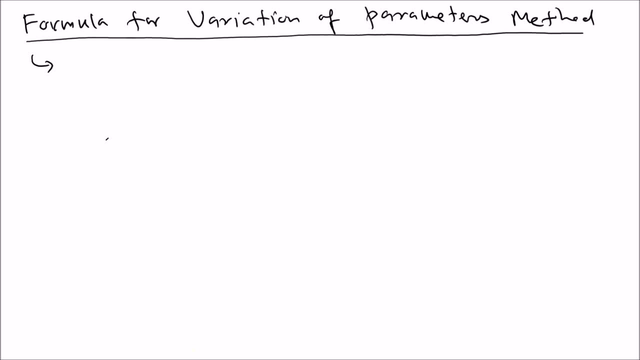 again the same idea. uh, let's say two. let's say two linearly independent solutions to independent solutions of y, double prime plus p, x y prime plus q x y equals 0 a r. let's say y 1 and y 2, that's always. 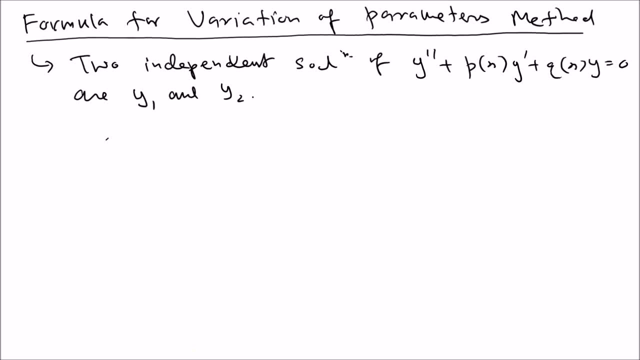 the first step. we find two linearly independent solutions of y double prime. we find two linearly independent solutions of the standard equation. and then are: the particular solution is given by a particular solution, particular a solution of y double prime plus p, x, y prime plus qx, y, equal fm. 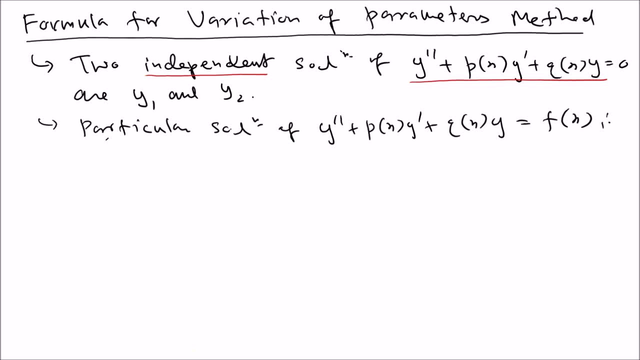 qx- y equal. fm is given by by p equal. it is simply u 2 y2 y1 fx over the wranskian y1- y2. order matters minus y1 y2 fx over the same wranskian y1 y2 dx. so you can remember this formula. 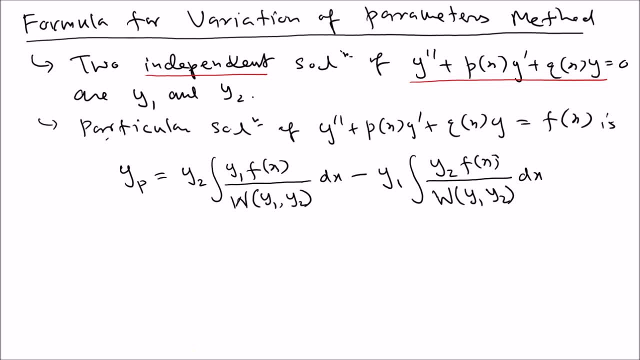 and use uh when there is a variation of parameters type of problem, because there are a lot of problems that you can use the undefined formula, so you can use the undefined coefficient method, but this works. only problem is whether this integral can be done, because sometimes what happened 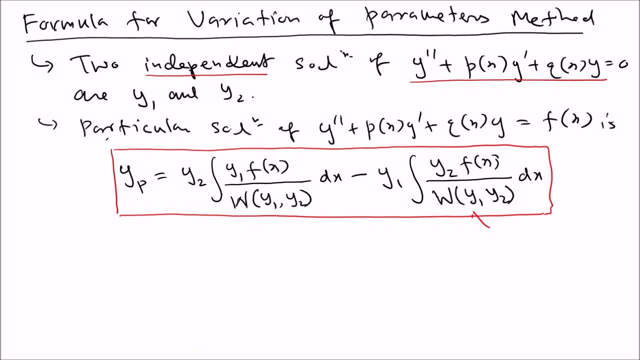 this is not going to work. okay, sometimes it's even this. so this is simply the wranskian. now you know that. why? uh, the solution has to be independent, otherwise the wranskian can be zero. so we make sure that it's not equal to zero. 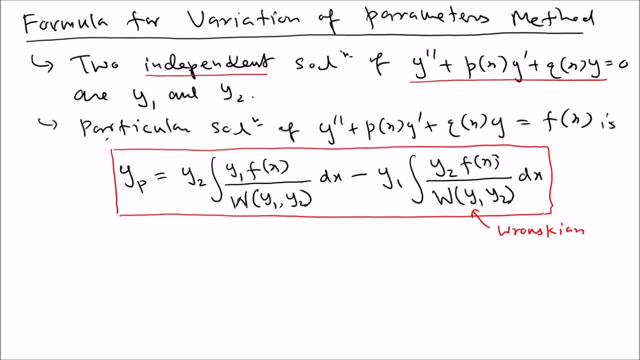 because we divide by that. okay, let's just do one example from that, just to see how it works. um, so let's do this problem so uh. so let's say a use, use, uh, the variation of parameters method, variation of parameters method, method to find the general solution of the wranskian method. 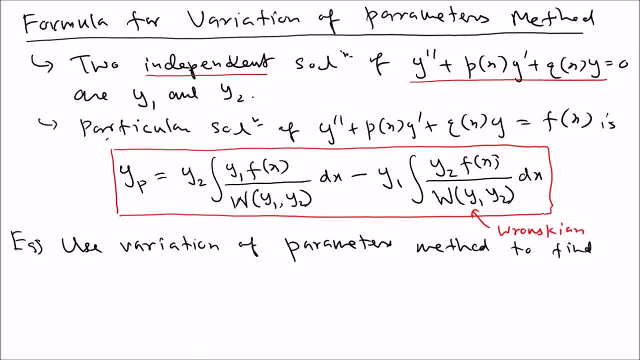 so let's do this problem. so the general solution of: to find the general solution of solution of this equation: y double prime minus 2, y prime plus y, equal e, x over x to the fourth. you can see that, uh, this, see, this one you can cannot do using the integ. 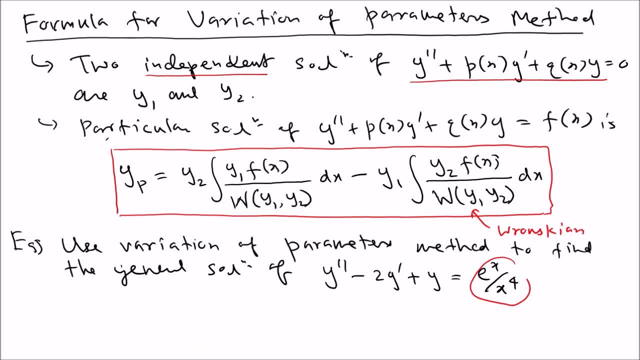 undetermined. undetermined coefficient method- see the format- because there's something in the denominator. so then you cannot do it. so when you take the derivatives, you're going to powers, get more and more and more, so it's not going to work. okay, so let's use the uh variation of. 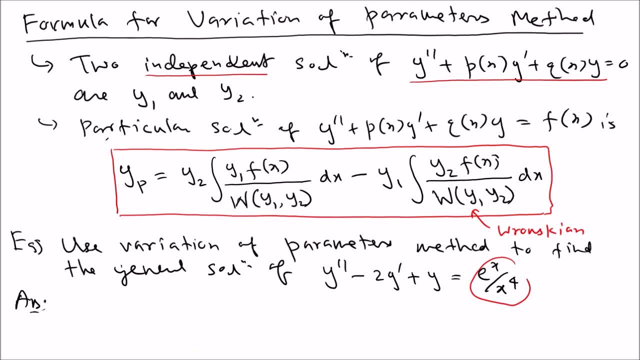 parameters. so the answer. so first we can look at the characteristic of the homogeneous equation. so the characteristic equation of the homogeneous equation is: lambda squared minus 2, lambda plus 1 equals 0.. okay, so if we were to imagine that, uh, the zeros are zeros, are you can see, it is a lambda minus. 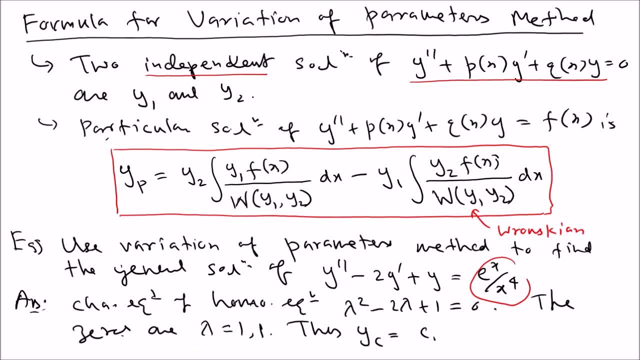 one square. so that means lambda equal one one that's a repeated solution. so thus the y, c is c. what's where the x goes to 코로, for n set the panda values. so lambda equals. ex means 1.5, or in other words, what comes with dude equals claudius. what does c equal to create the working force? 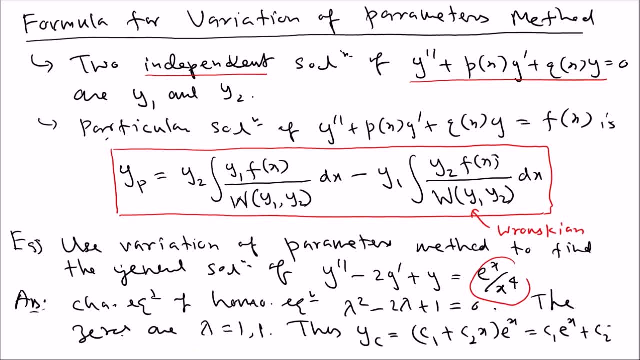 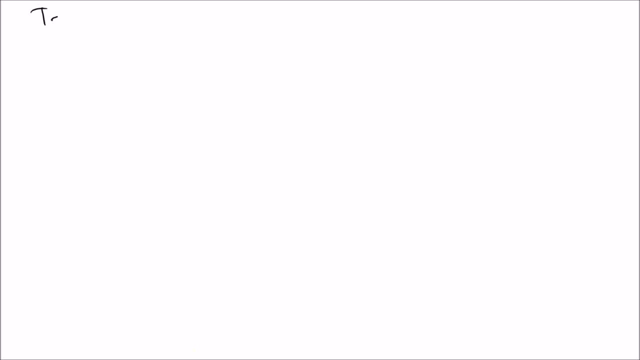 c1 e x plus c2 x e x. so that means those two are the y1 and y2, the two solutions y1, y2, so uh. so take or pick or select. y1 equal e x and y2 equal x, e x. uh, as two. 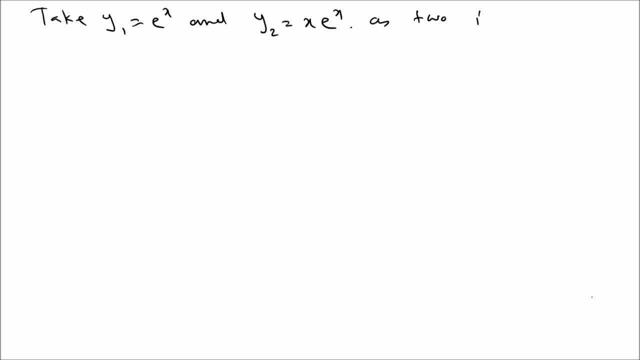 independent solutions. independent solutions. uh, now the wronskian w y1, y2, so y1 first, y1, y2, y1 prime, y2, prime. so if you plug in, you get e x, e x, x, e x. that means e x plus x, e x. if you multiply through, you get: 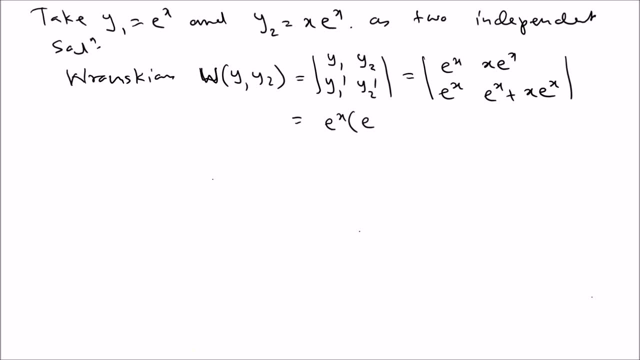 e x times e x plus x, e x minus x, e x times e x. so you can see: uh, this and that get cancelled out, so you get e to the 2x, which is not t equal to 0.. perfect, okay, so that's the wronskian, now the solution. so the particular solution. 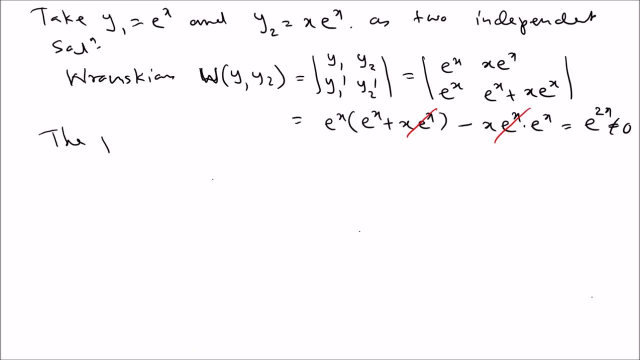 is the particular solution by the formula. this one is yp is. this one is 있�u. it is yp, equal y 2 y1 fx over the wonskian y1 y2 in that order, minus y1 y2fx over w y1 y2 in that order. so the same same thing, not change with the negative sign. 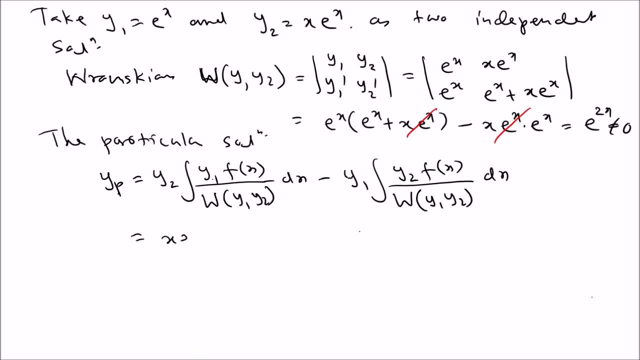 you're going to get x, e x, e x, that's y 1, and we have e x over x to the fourth power, over wronskian, which is e to the 2x dx minus y 1, that is e x. we have what we have. 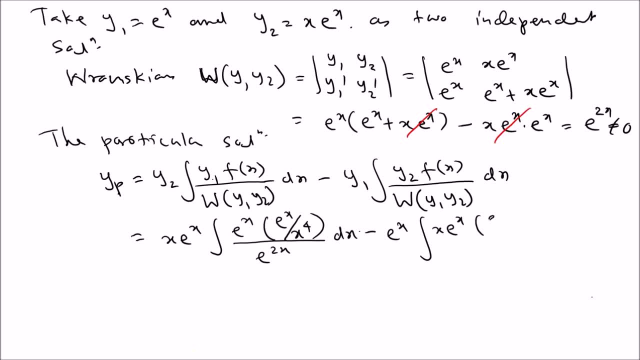 x, e, x, again e x over x to the fourth, over e to the 2x dx, and you can see there are a lot of cancellation going on. e, uh, this cancels. with that, the same thing happen on the other side, so you simply end up getting x e x, the integral of. 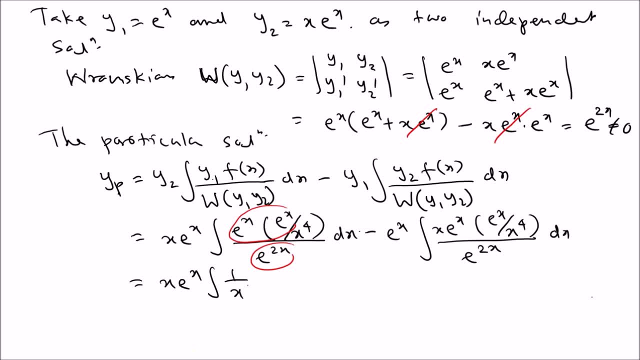 1 over x to the fourth, dx minus e, x times the integral of 1 over x to the cube. so these are very easy to integrate. so if you integrate them you get x e x times x to the negative, 3 over negative 3, negative e x times x to the negative, 2 over negative 2. if 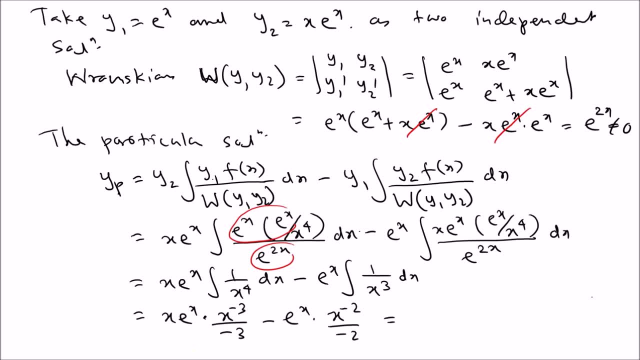 you simplify y, you get what do you get negative e x over 3x squared, plus e x over 2x squared. if you add them, you get e x over 6x squared. okay, that's the yp. now what you do, how you write the general solution. 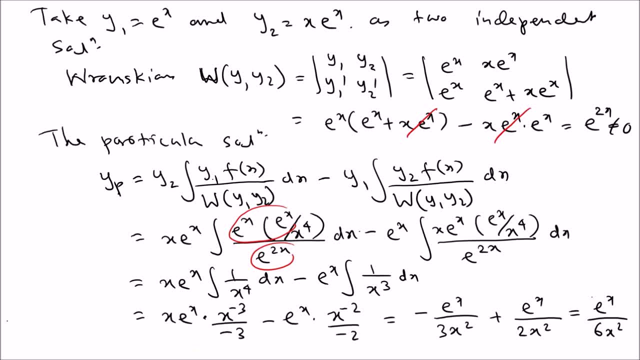 so the so this is the solution, the general solution: y equal the sum of the two, y c plus y, p, y c is what which is c 1, e x plus c, 2 x, e x plus e x over 6 x squared. so that is the general solution, using the formula so. 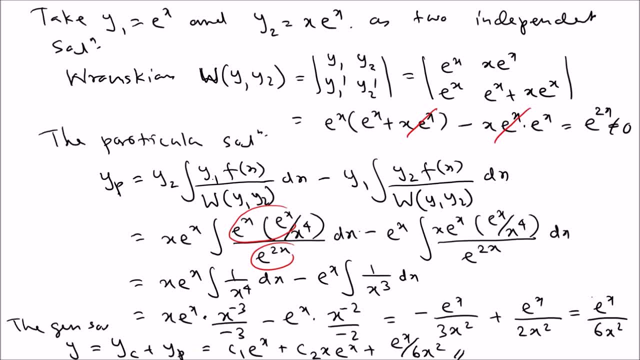 it's not long, uh, but you need to simplify the integral. this is the end of the review two. so next we can talk about uh, review uh. in review three we can talk about the series solution- at least two examples- and the laplace transform and the eigenvectors method. 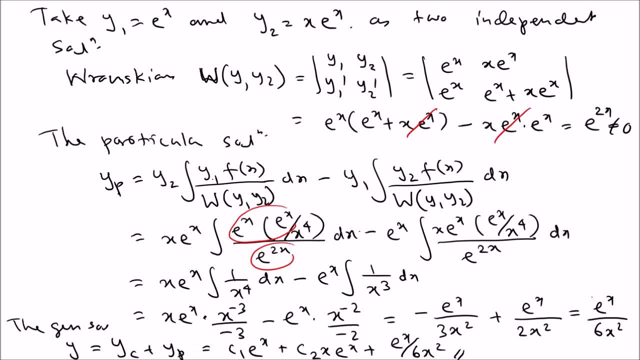 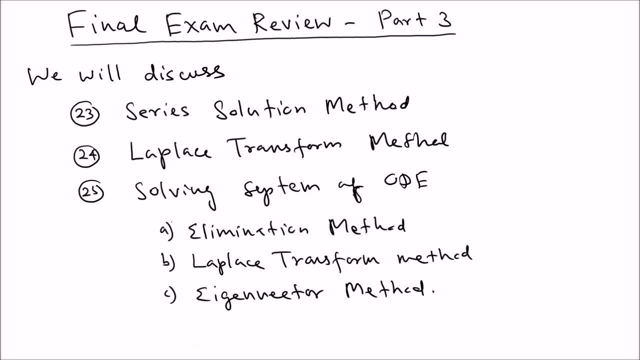 so this is an example of the sequence of the difference equation. this is the part three of the final exam review of the difference equation class. in this review we are going to talk about three topics. the first one is the series solution method. we will discuss two problems first order. 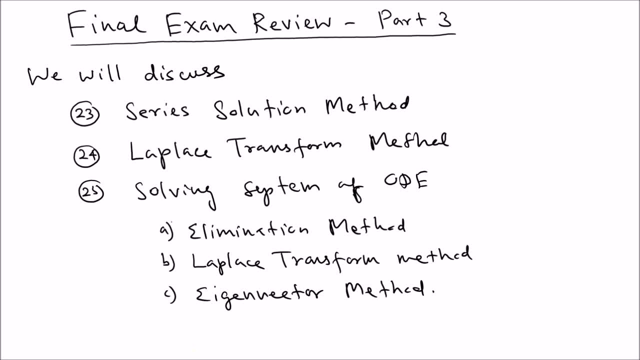 and second order and then we're going to go to the series solution method and then we're going to be talking about the general solution. so we will go with the definition and then how to solve a differential equation and the convolution and the heaviside function or the. 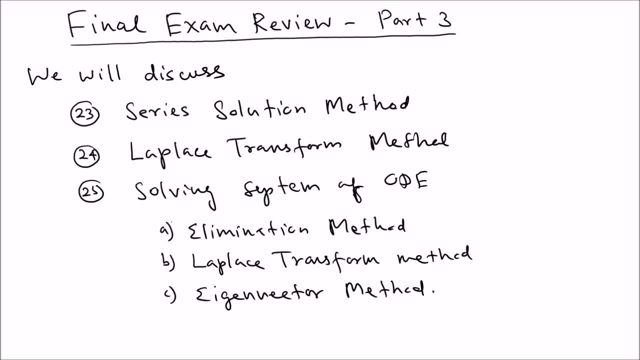 switching functions, and then the direct delta functions and then finally, we're going to talk about the solving a system of ode. so we will go through the three techniques: the elimination method, and then the laplace transform method and the eigenvectors method. so let's start with the series solution method. 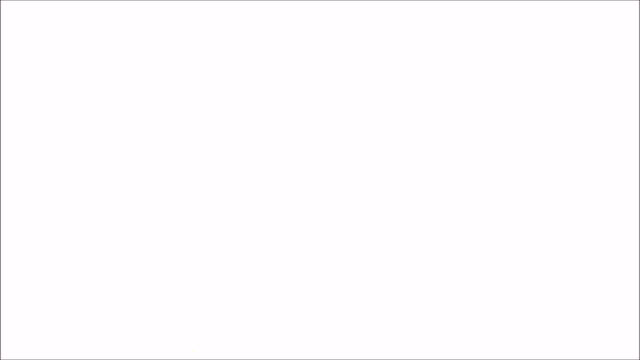 uh, so it is number 23, the series solution method. series, a solution, a method. so this is a kind of a last resort type of situation because there are a lot of different solutions. so let's start with the series solution method. so let's start with the series solution method. 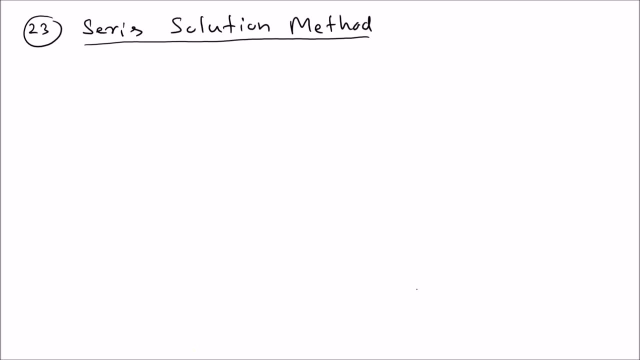 so what we're going to do is we're going to assume a series solution. we assume there's a solution given as a power series and then we try to find the coefficients of that. uh, once you know the coefficients, you pretty much know the solution. so that's the kind of idea. so uh, 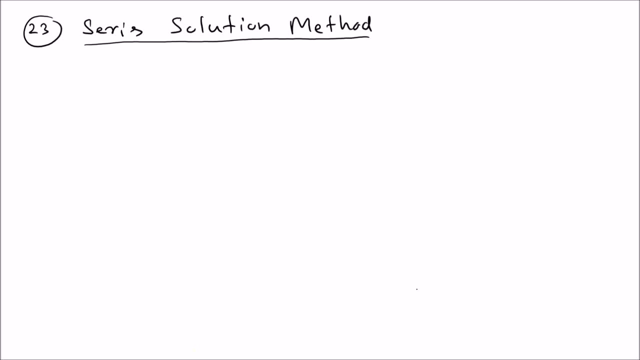 we normally deal with second order differential equation in this, um course, uh, mainly. so we have a equation like this: so a s, so a x, uh. let's say y double prime, uh plus uh plus b, x, y prime plus c x y, uh equals zero. so let's say the 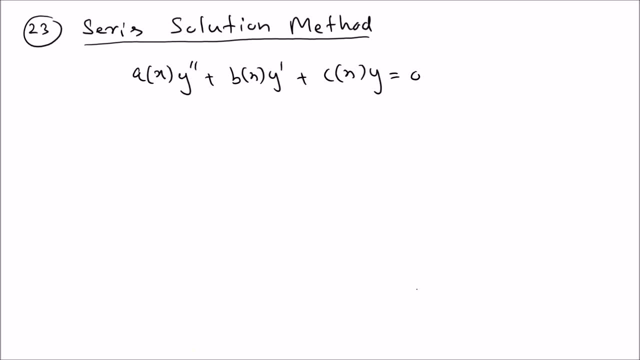 homogeneous equation. so what we're going to do, we're going to assume. so, the first step, we're going to assume uh, assume a solution of the form, assume a solution of the form of the form: uh, y, equal sigma, uh, n, going from zero to infinity, c, n, x. so we assume that the solution can be written in this form, and then 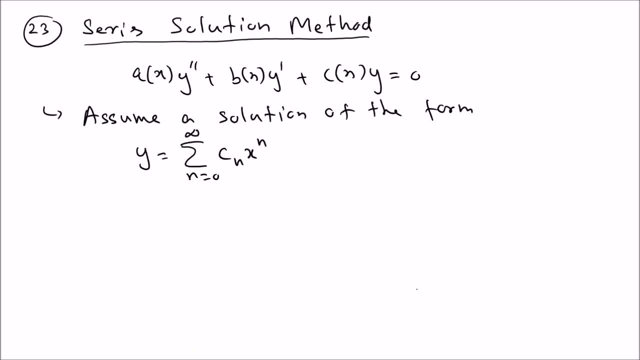 after we do that, we're going to assumption and then we can do: we can take the derivatives of this one. so we're going to take derivatives. so we're going to take derivatives. so, depending on the differential equation: is the first order, you need one derivative. if it is second order, you can need two derivatives. so take. 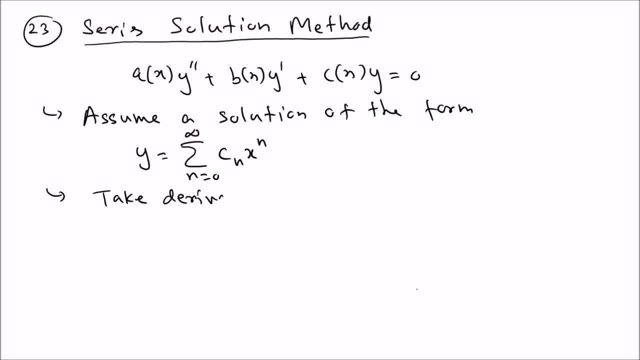 derivatives. uh, that's the uh second step. uh and uh plug-in. so we take the derivatives and plug into the equation and plug in uh to the um equation, so we can take derivatives of the series and then plug into the equations. so we have two steps. so we have two steps. 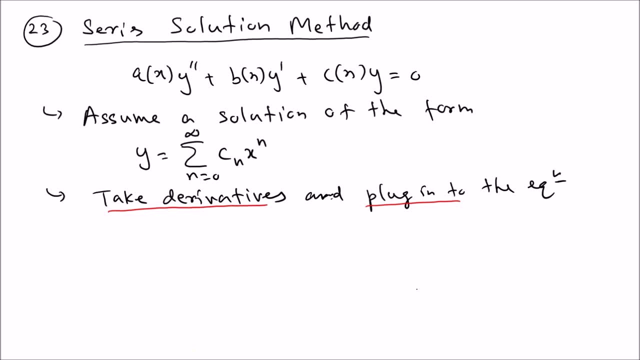 so we can take the derivative and plug into the equation. third, one is after the plug in the equation. we try to find a relation, uh, between the coefficients. so we can try to find the relation among the coefficients. okay, so find a relation, final relation um, among coefficients, okay, 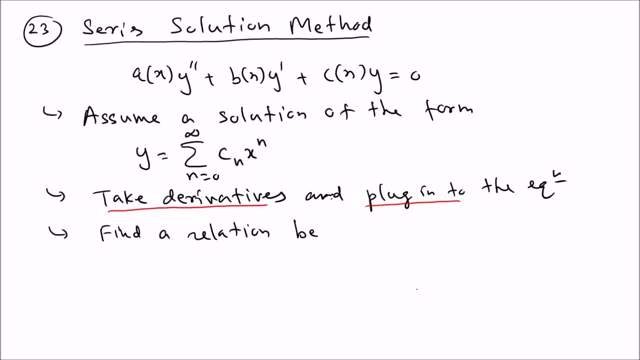 violation. we can say, uh, a coefficients. so it will be clear what we mean by that, because sometimes you can express uh, like what we try and do. we can try to find a solution for c n plus 1 or c n in terms of other coefficients. okay, that's a relation. we find a relation between the coefficients and 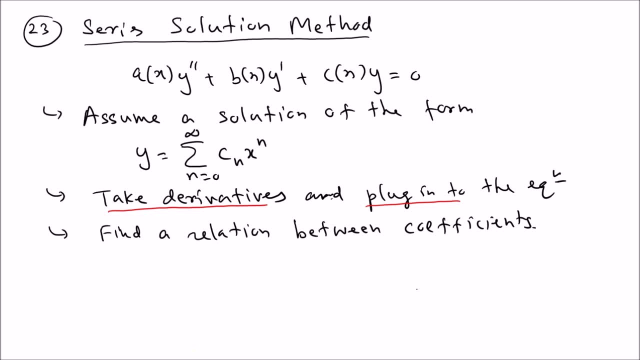 then what we can do. we can evaluate uh, uh, few coefficients. so, uh, after that we're going to find uh c naught, we can probably have it. so then we're going to find the rest. so we're going to find, we're going to calculate field and, if possible, if possible that we don't. 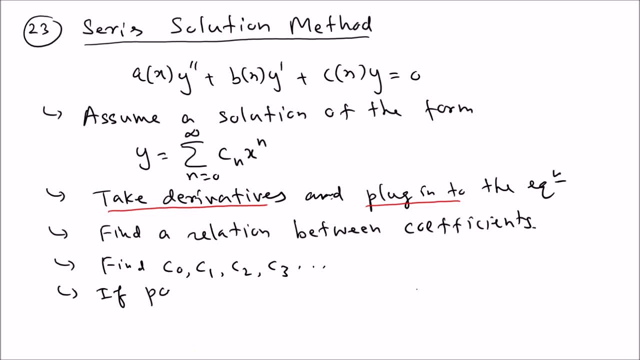 know if possible, we can say if possible, a finer formula for uh c n or c? n plus one, normally c? n plus one. so we try to find a formula, but that's sometimes it's impossible, like i mean you can, but it's going to be like very complicated after that what you're going. 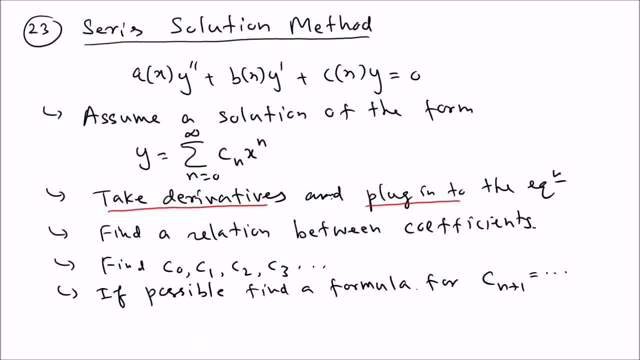 to do? we're going to plug in them and then write the solution. and then, after we do that, then we could write the solution: uh, right, y, which is sigma n, going from zero to infinity. we're going to plug in here, so c, n, x, n, so, like you know. so, if you look, 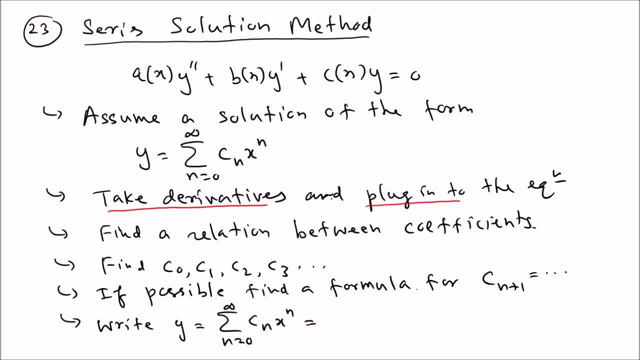 at the formula, you can see that we're going to plug in c n, x, n, and then we're going to plug in c n, y. so if you look at the expanded versions like that, so we can just plug in for the coefficients, because that's what we found earlier. 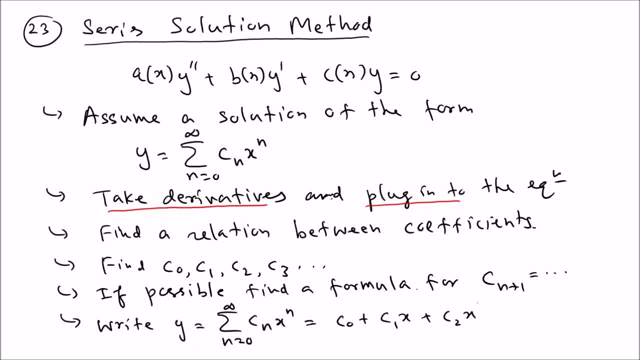 so we're gonna uh plug in here. so that's the kind of uh point. we do that and sometimes we can see a pattern and find a close form solution. but that's not always the case. so find a closed form solution, uh, again, if possible. so that's not always the case, so find 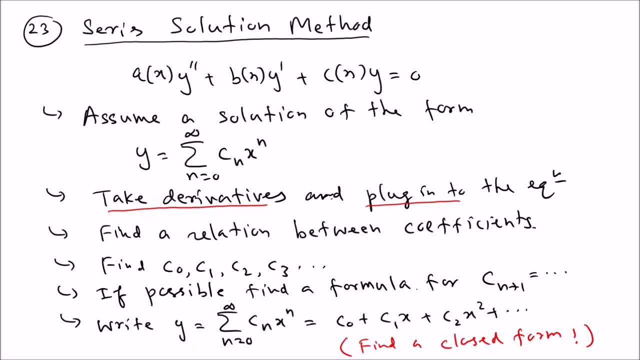 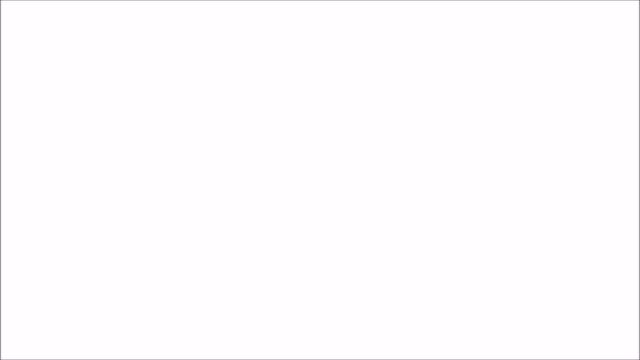 okay, these are the common steps. uh, to do a problem. so let's look at a problem and see how it gonna work. so we can start with the first order equation. so let's say, um, for example, find a series solution, find a series solution. find a series solution. 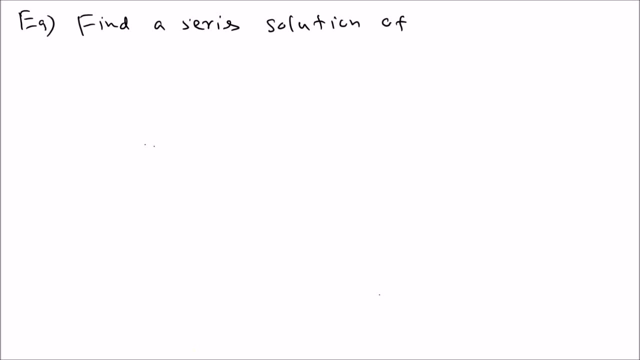 of find a series solution of y prime plus three y equals zero. so we're going to try to kind of find a solution for that: y prime plus 3 y, y prime plus 3 y equals 0.. okay, we're just going to follow the steps. 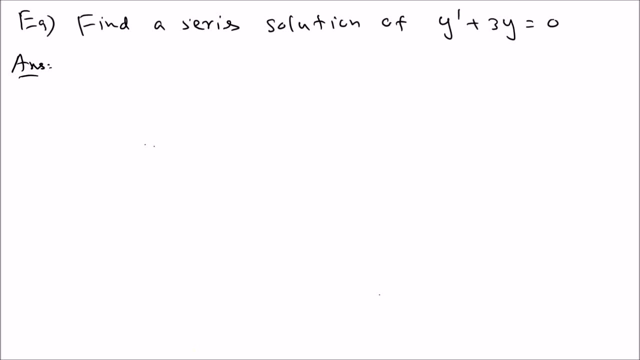 uh, so the steps are: assume. so assume y equals 0.. a series solution. so y is given as a series. so that's the assumption. we assume that now what we can do, then we can take the derivatives. so you can see that when you take the 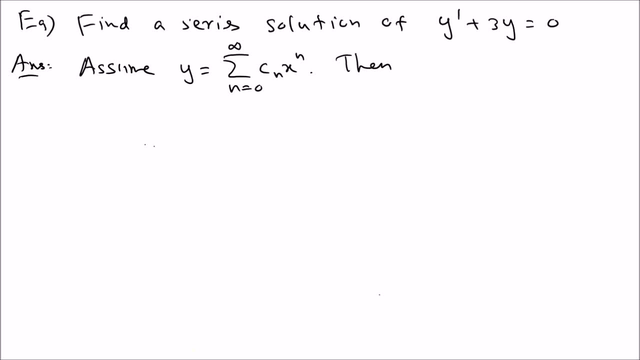 derivatives. the first term is a constant. so when you take the derivative, what will happen? the first term disappear because a constant. so that means, uh, we're going to start with y prime, which actually start with any constant equal 1, because the constant term goes away. so we just take the derivatives. so 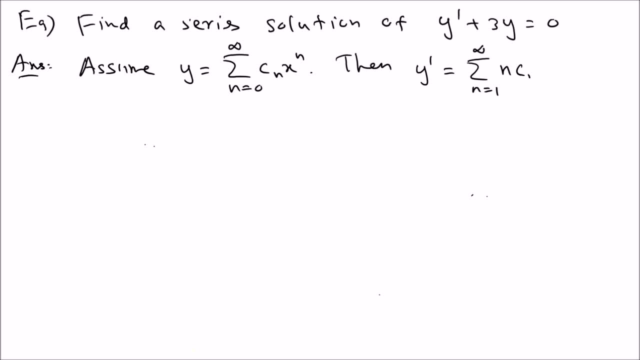 if you take the derivative x, n, that means n, c, n, x is abstract. once that's the derivative and you can see that the important thing start with 1 because the constant term disappear. so if you take one more derivative it is going to start n equal to, because now the first term is a constant. so if 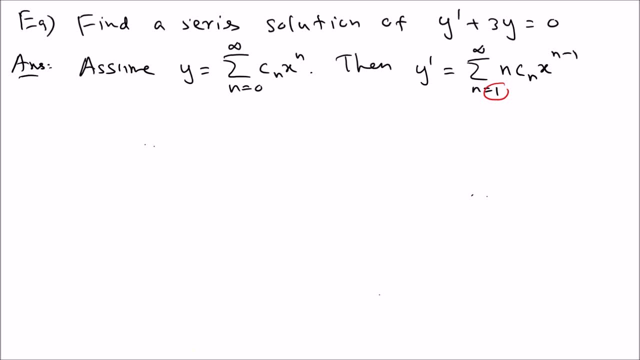 you take the second derivative, it is going to go away. so that's something we need to remember. okay, good, now our figure is 2.2.. so once you substitute uh, what will happen is y prime plus 3y equals 0, so that means you're going to get y. 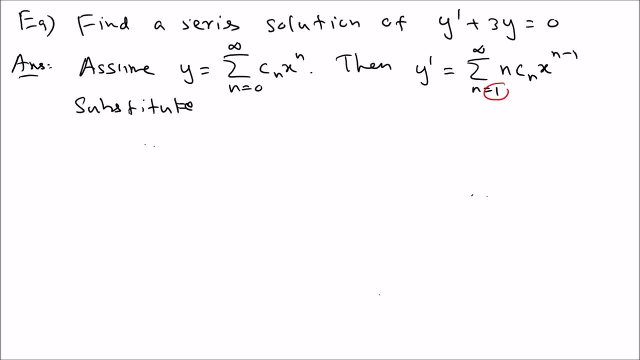 prime that means n equal 1 to infinity n, c, n, x, n, minus 1 plus 3 times y. y means n going from 0 to infinity, c n, x, n. so that means you're going to go from 0 to infinity, c n, x, n, which is equal to 0 on the other. 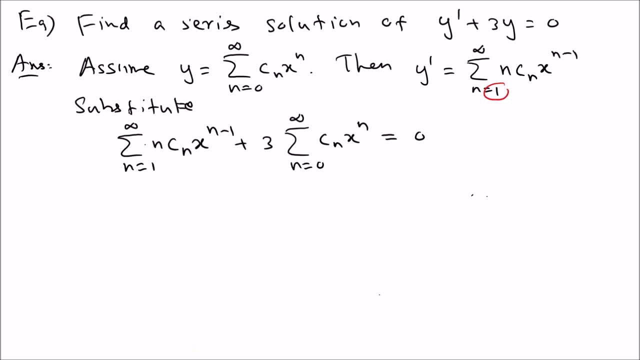 side. okay, so that's so, we plug it. so that step is over, we plug it. okay, the derivatives, and then plug it. now what we're going to do, you can see that we check what terms we're going to get, um. so, for example, let's plug in the first: 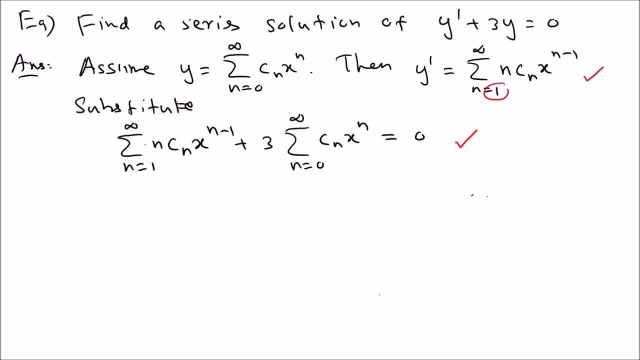 value in the index so you can see. for the first series the first value is n equals 0. so if i n equals 0, i'm sorry. first value is n equal 1. if you play n equal 1, you get x to the 1. minus 1 means x to the 0, so you get x to the. 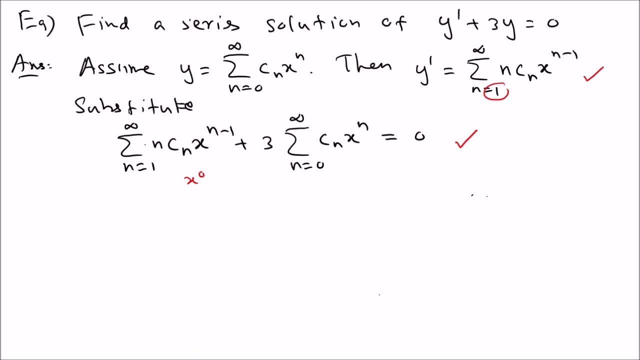 0 in the first one. second one, you can see: the index value is n equals 0. when you plug in equal 0, you get x: 0.. so that means that's a good one. that means you get the exact same number in both. but if you do not get the exact same, 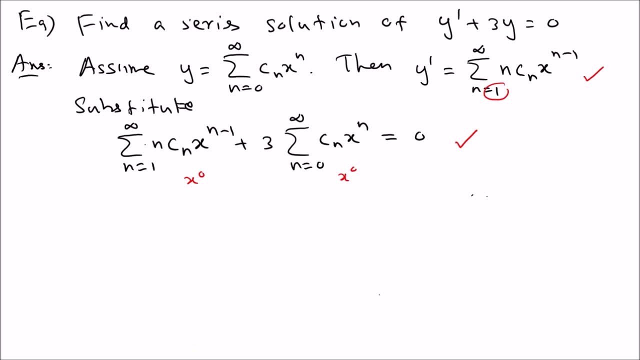 number. we need to write the uncommon terms first. we can write the uncommon terms and then start writing the common terms. so that's we're going to see in the next example. but here you can see everything start with x here. so everything looks great. now what we can do: we can use the seesaw method. 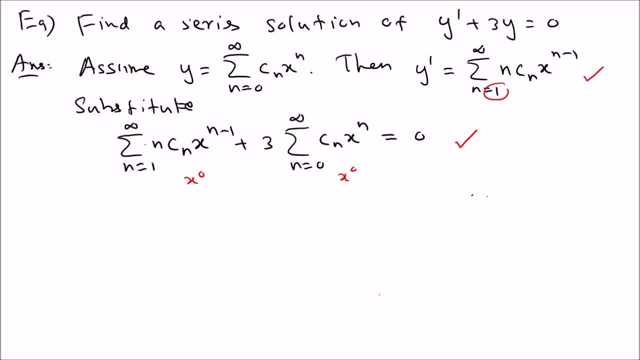 remember the seesaw method. uh, so we're going to use the seesaw method to re-index. i'm going to write it here. so next, what we do, i use the seesaw method. so see so method. you can use the seesaw method to re-index. 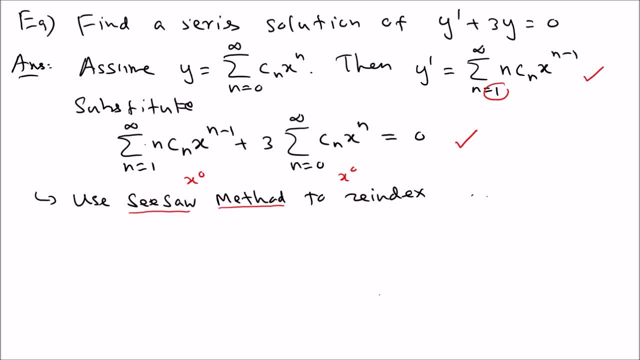 so it's a method that i introduced so you can find them in other books. okay, so you can look at the video about see some method it's there. so what you can do, uh, it's very simple because you can see the second. uh, second sum is x: n. we try to get the x n in the other. 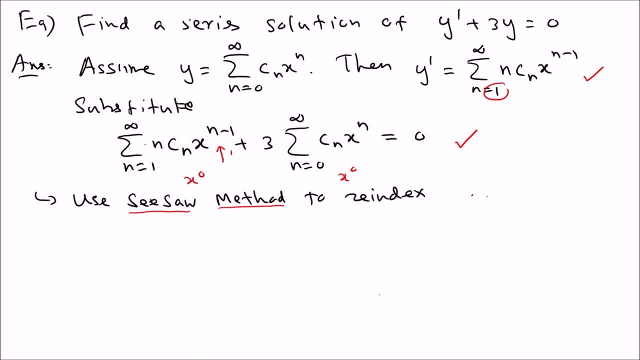 one as well how to get x n. you can see, to get x n you have to increase the index by one. so you can increase this one by one. what we do, we? because one goes up, the other goes down. so that's the kind of idea. so it's like: 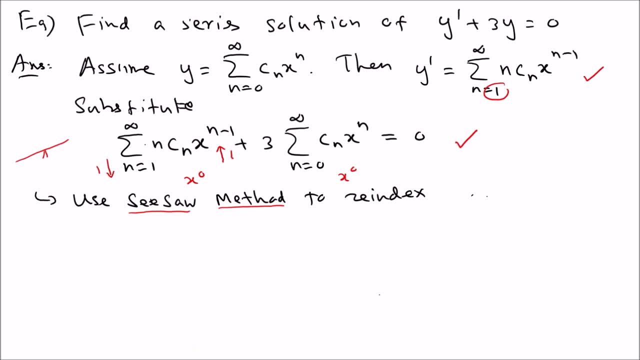 a see-saw. so this side goes up, then this side goes down, so that this stays the same. you see that the middle never change, but one goes up, one goes down. so that's the kind of idea here: when one goes up, the other goes down. so that's what you call the. 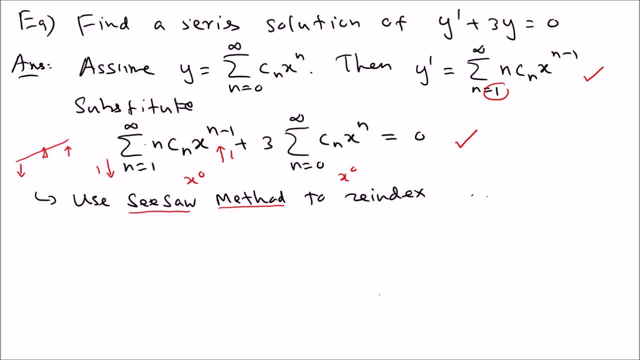 see-saw method. so it's very simple. it's going to make the calculation much easier. so if you use that, so outside you can increase by decrease by one, that means your sigma going to start with 0, because you would go down by one. inside you can increase everything by one. that means n become n plus one. 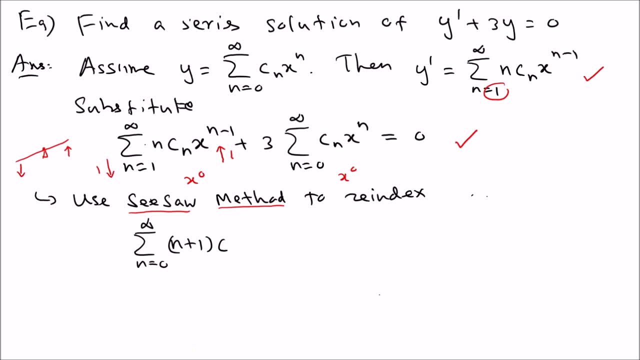 c n become c n plus 1. x is in minus 1. if you add 1, it becomes excel, perfect. and then here i'm going to bring the 3 inside. so this is 3, c, n, x, n. now, when you make the calculation, both have the exact same index, exact same uh, exact same power: xn. 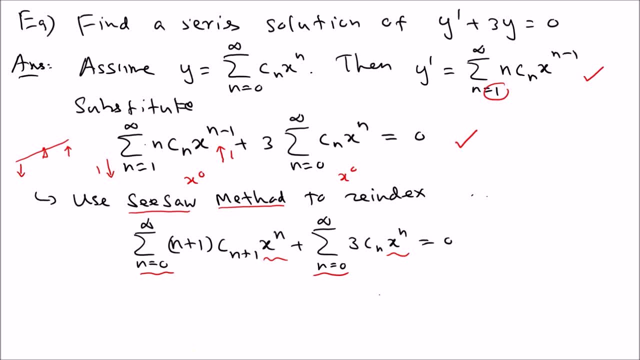 and exact same index. that means you can combine. so we'll combine them into one, so we can write this one as sigma and going from 0 to infinity, n plus 1, c, n plus 1. i'm not going to write the accent term, i'll leave it, and then from the other one you get 3. 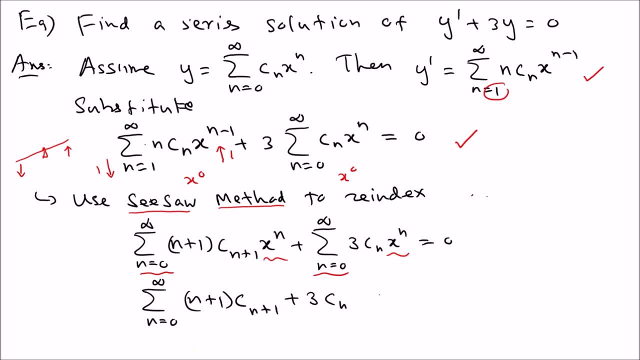 c, n. now we can write the common x, n outside. so now what this is? this says that the whole series equal to 0. the only way this can happen is this term has to be 0, because there's no other way- that the whole series is 0. so that means this implies that 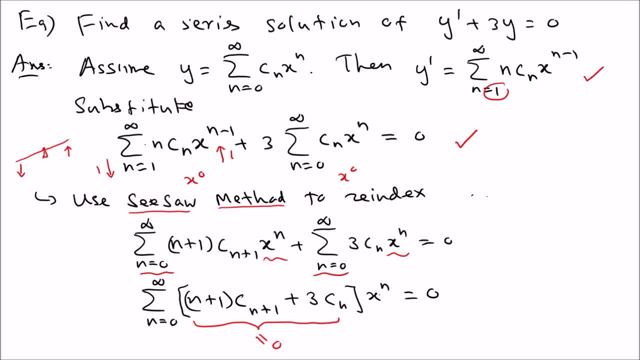 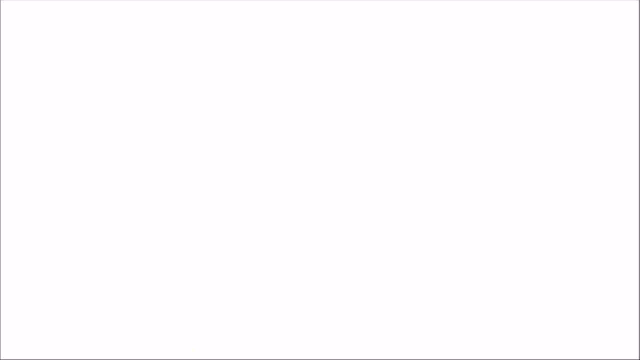 this term, the coefficient is 0 and that's exactly what we need. so let's write that. so we're going to get that. so we need that. c? n plus 1 plus 3 c? n equals 0 for the index signal. index values are starting with- you can see- 0. 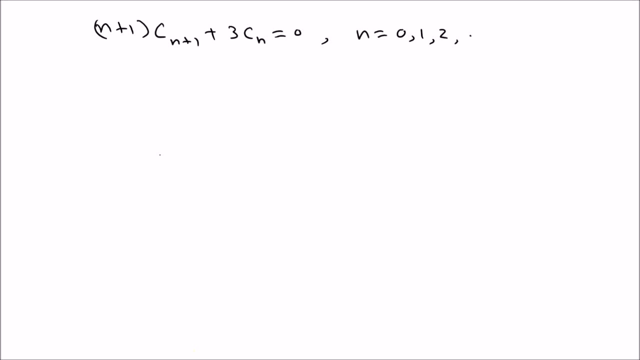 1, 2 like that. so it's always coming from the sigma, whatever the value you're going to put it there. ah, now we can solve for c? n plus 1. so c? n plus 1 is if you move, the other side is a negative 3. 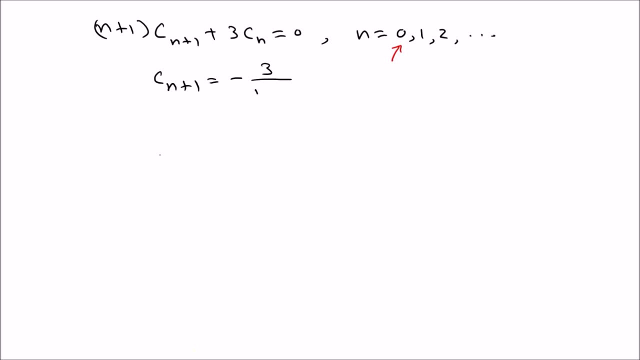 over n plus 1 times c n. so that is the relation, that is the, actually the relationship between the coefficient. okay, so you find a relation. again. this is only valid for n going from one, two, three like that. it's only valid for those. now what you 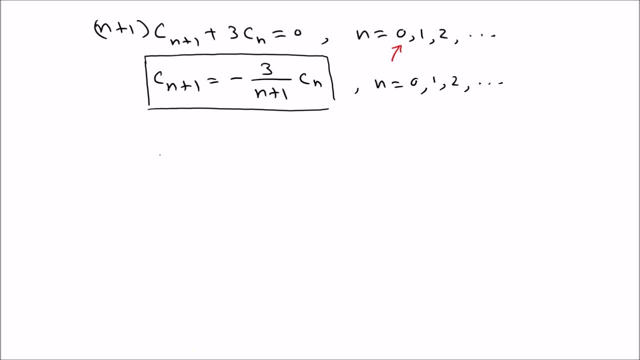 can do: just calculate few v values. okay, so we can start with this first value: n equals zero. so if n equals zero, you're going to get c 1. let's plug in the first value: n equals zero. just plug in equal zero. so you're going to get negative. 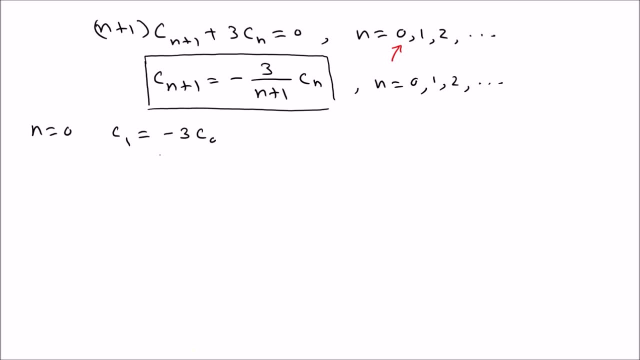 uh, three one, so it's negative three c naught. that's what you get now. uh, we're gonna plug in equal one. we plug in equal one, you're gonna get c two, it's become minus. if you plug in equal one, you get three halves c one. but we already know what is c one, so let's plug in the c one value when. 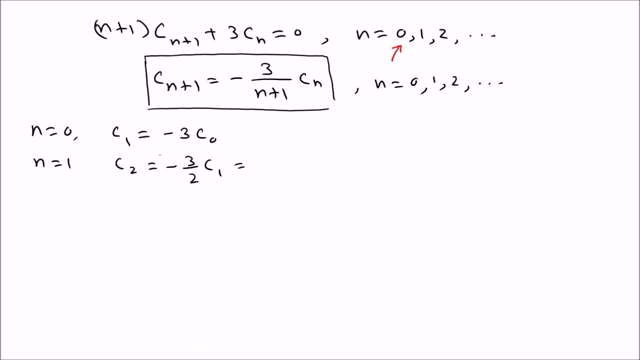 you plug in the c one value. what happened is you get negative three. you multiply another negative three. that means negative three squared. you leave it like that and in the bottom you get two c naught. that's what you get for the second coefficient and then go with n. 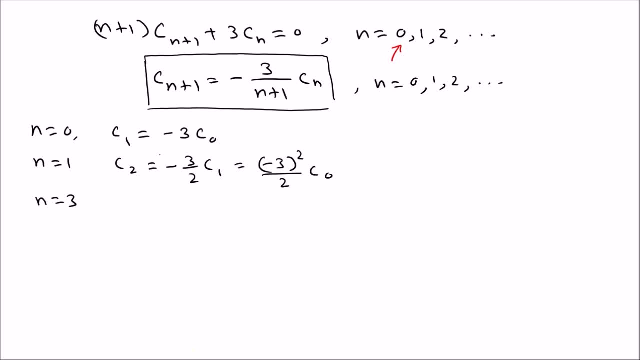 equal three. so keep writing and until you see a pattern. so if you plug in equal three, what happens? it's still negative three. if you plug in three, this become uh. so if you plug in one, you get two when you plug in. oh actually i missed the value. uh, this n equals two. 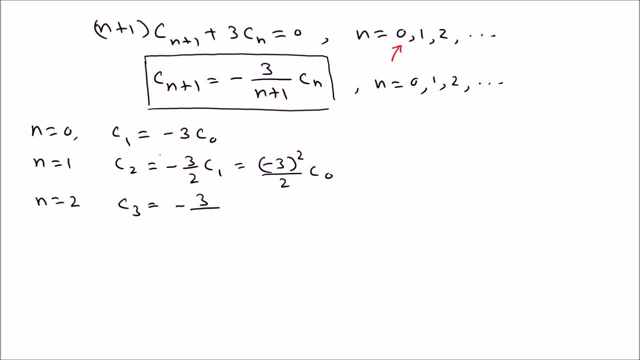 for n equal two. then you get that and then, uh, it's become three, c two. now we know c two, so we can find the c two value here. so you need to see two value because c two comes from the previous step. you can see you get another negative three. so i'm gonna write it like that. 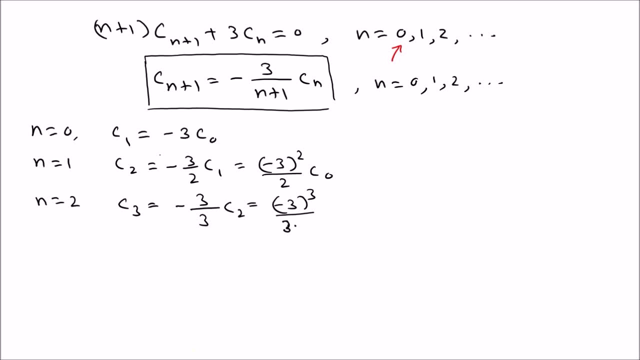 over uh three times two here c naught so and then you can see that. what happened every time? you're going to multiply by uh the same index, like that you can just divide by that, so that term comes extra. that's gonna you add it to the. 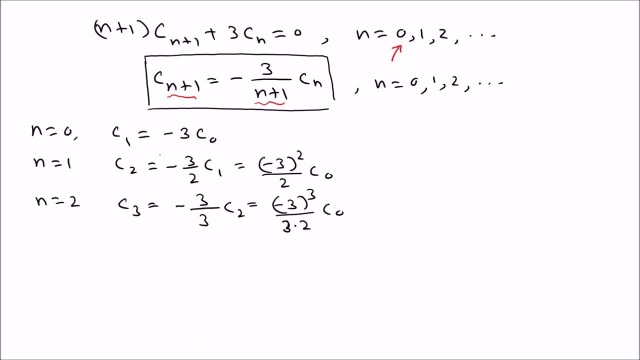 previous one. so that's what you see. so that means, uh, if you want to keep going like that, so at the n step what's going to happen? you're going to get c n. so let's say, in minus one step. if you go in minus one step, you're going to get c n equal minus. 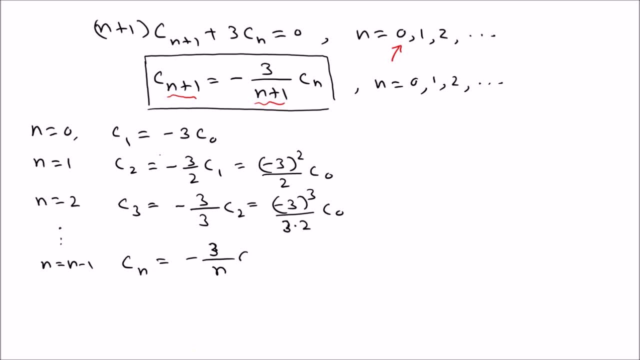 3 over n. here it is c n minus 1 that you can simplify, you can substitute. so what will happen when you substitute like that? you're going to see that it is negative three. so you can see that when you have one, it is negative three, only one of them, when 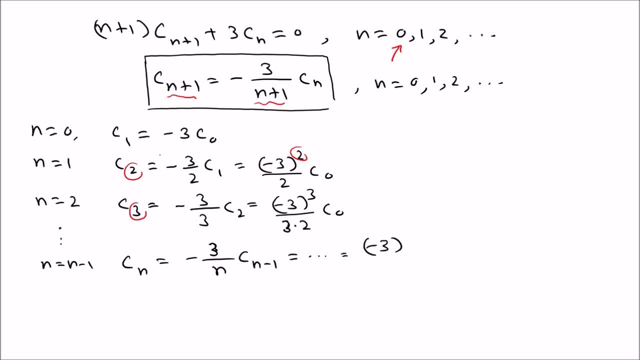 you have two, there are two. when you have three, three. so that means in this case you're going to get n of n in the bottom. you can see that that also, that number exactly must the bottom number. so that means in the bottom you're gonna get n, 2 and then 2 and that's, that's the one. 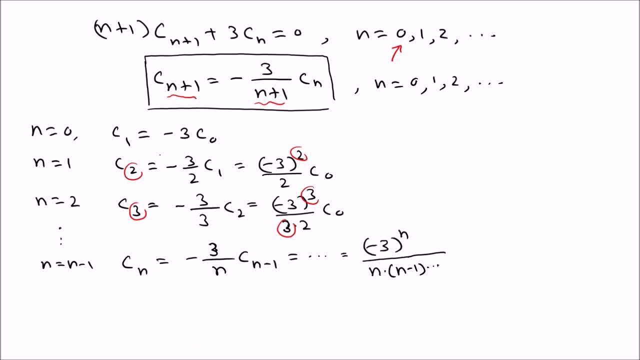 times n minus 1, times like that. that's simply the factorial. so times c naught. so if you go back what you have, gain is negative. so if you go back and you can fill this now because you see the pattern now, so it is negative 3. 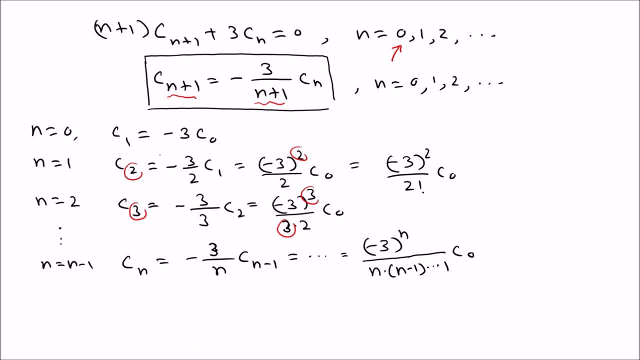 squared factorial 2, c naught, this become negative 3 cube over factorial 3. now this is negative 3 to the n over factorial n, c naught. so that's what you get. so that is the uh general coefficient. now, what we're going to do, we're going. 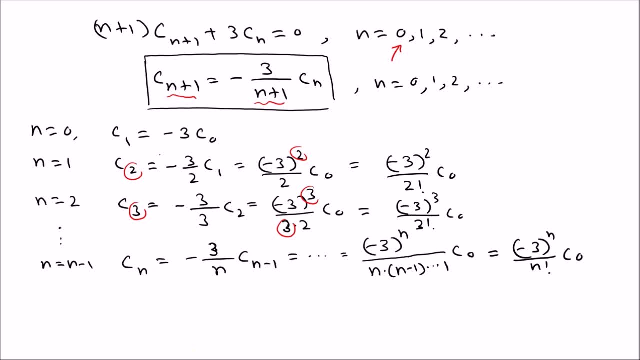 to plug in that in the equation. so we found the coefficient, so let's plug in. so, therefore, or then you can see y, which is sigma n, going from 0 to infinity: c, n, x, n. so if you plug in for c and you can see it is negative 3 to the n power of a factorial n. 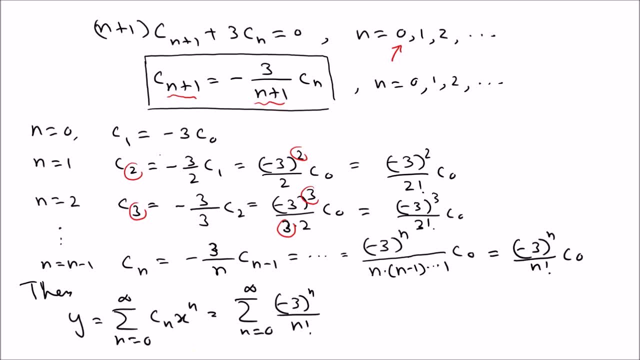 and then i can write the c naught outside. so x? n i will write the c naught outside. let us kind of uh make it simple. so it's equal: c naught. i write c dot outside is common. so why what's going on here? so you can see this is simply c? naught times. 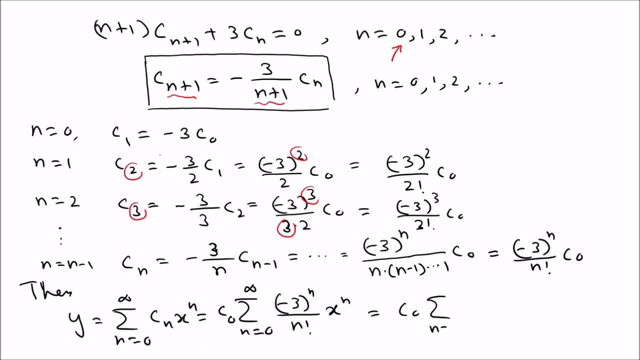 n, going from 0 to infinity. you can write this one as negative: 3, x to the nth power. if you combine, if you now, what is this? so you can see, this is simply the taylor series of e to the negative, uh, 3x. so this is simply c? naught e to the negative. 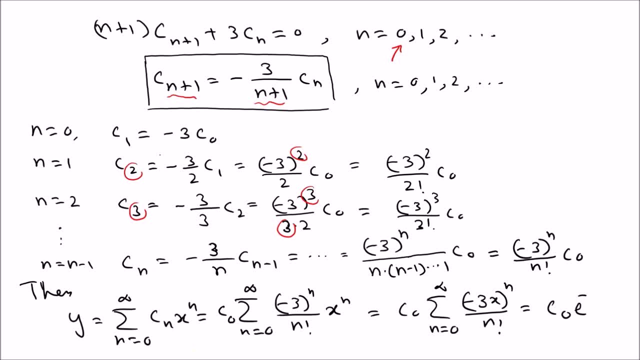 3x, as expected, because we know that this differential equation is one of the most important thing in the equation, so we can write this one as one of the four fundamental equations. we already know the solution. it is c naught e to the kx. uh, in this case k is negative 3, that's. 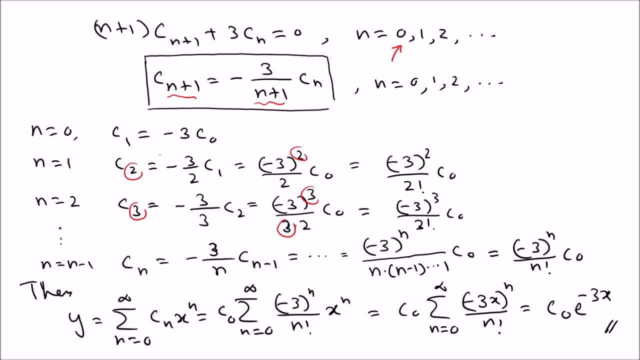 exactly. so we exactly get that. so if you forgot what i'm writing here, we know this formula, uh. so e to the x is sigma n going from 0 to infinity x, n over factorial n, and you can see that's exactly what we have here, here x. 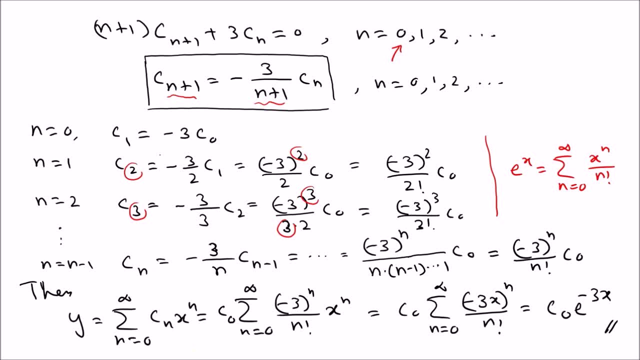 is negative 3 x, so that means you get negative uh 3x like that. so so so this is the solution of the differential equation and you can see that's not that difficult. after you find the relation, try to evaluate few and see whether you can um find a pattern and if you can find a 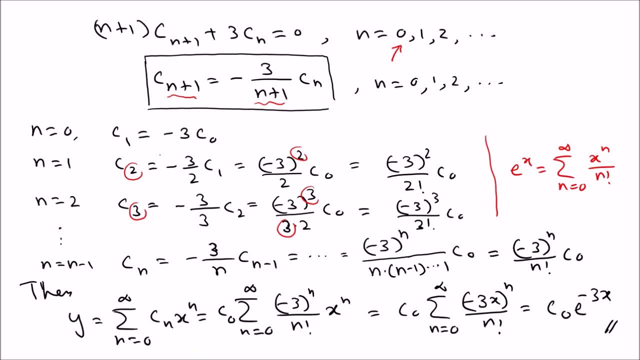 pattern. you can nicely simplify like that. so, um, yeah, so that's about that. so i'm going to do one more example, uh, from a little like a higher, like second or differential equation. so so let's do a little bit of a complicated one, just to see what we can do. 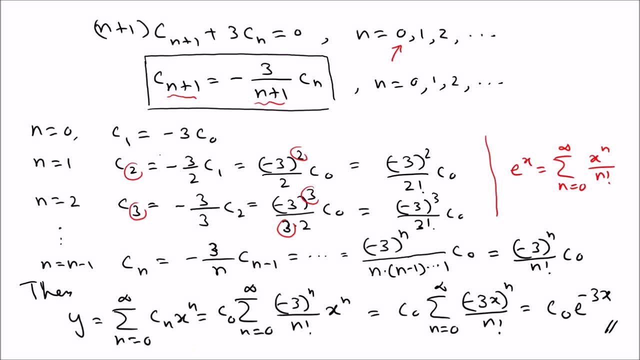 but in the exam the question is going to be reasonable, so you will get a reasonable question. but here i'm going to do like question, just to see what's what's going to happen. okay, so this is like a three term differential equation, three term- good, so let's do that. so the next example. 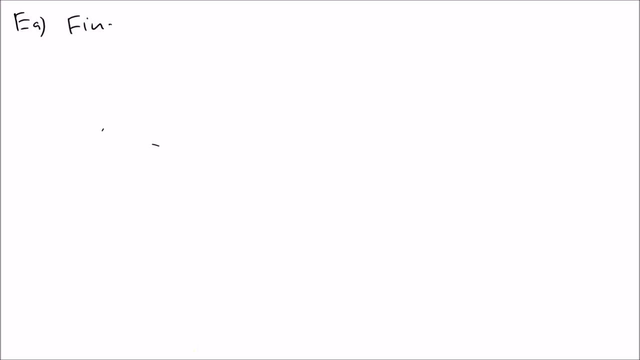 again, find a series solution. find a series uh solution of find a series solution of uh x minus one, y double prime minus x, y. prime plus y equals zero. so that is the differential equation we're going to solve the same idea, but this is second order, so it doesn't really matter. so, but only 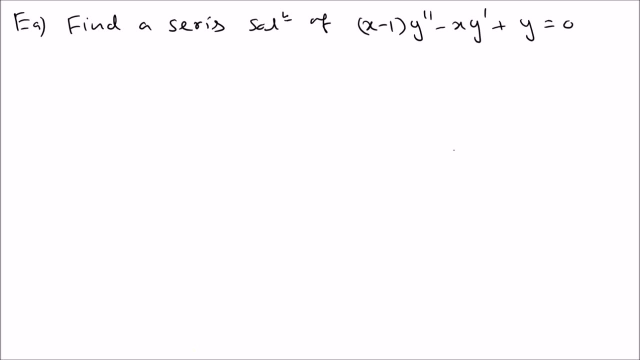 thing is we need to take two derivatives. so the answer, so we're going to say: assume so a solution of the form, assume a solution of the form y, equal sigma n, going from 0 to infinity, c, n, x, n. this step is always the same. now we take the derivative. 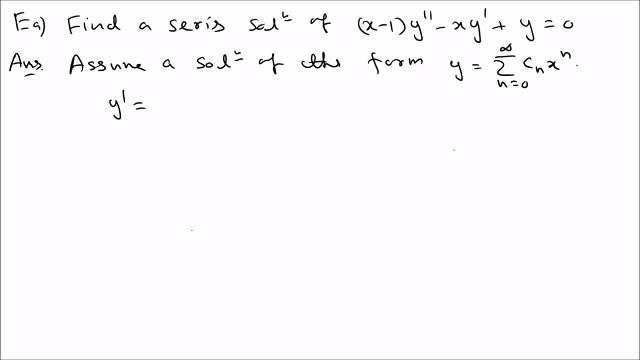 as we discussed. once you take the derivative, you can see you can start with n equal 1, because the first term goes away. so you get n, c, n. take one more derivative so you're going to get the new first term. i'm going to go so because that's a constant, so you can. 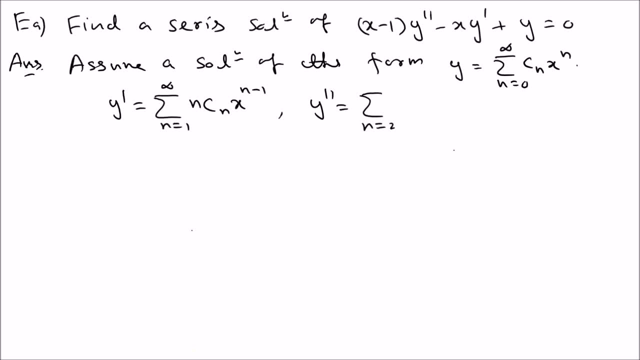 start with n equal 2, and then you have one more, so it's n n minus 1 c n no change. x to the n minus 2. now, okay, so there are two things to focus on, this and that here, this and that. ah, good, so those are the written. now what we can do. we can write it as a 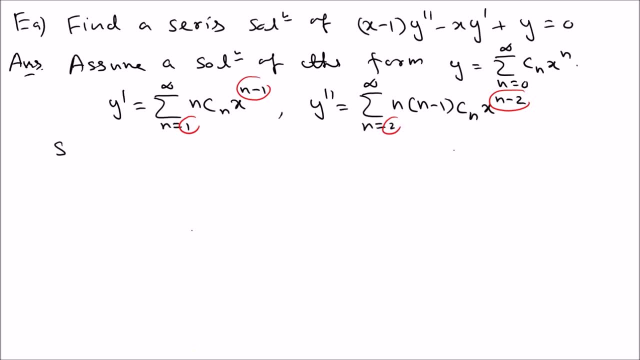 substitute into the equation. so substitute. substitute uh into the equation. so if you substitute what we get uh, we have x minus 1, that's a term- and then y, double prime. so that means the sigma n going from 2 to infinity and n minus 1. 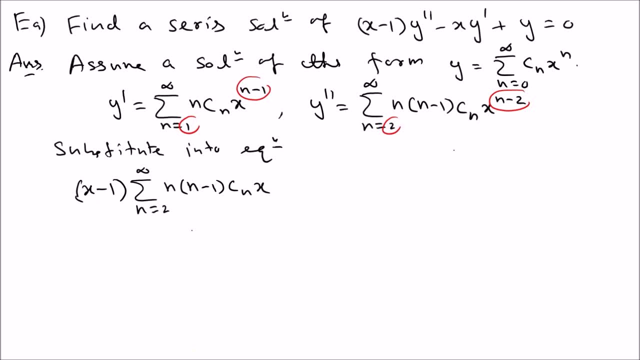 c, n, x minus 1, then minus x, the first derivative which you can start with: n going from 1 to infinity, ah, 1 to infinity n, c, n, x, n minus 1 plus y, which is sigma, n going from 0 to infinity, c and x. so we write that. so next step is we try to bring this. 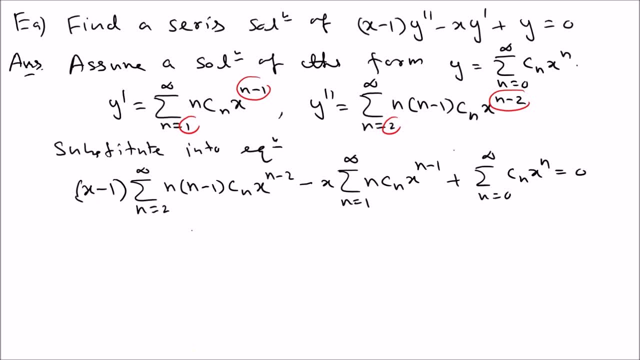 inside before we change the index. so we write that, so we write that. so next step is we try to bring this inside before we change the index. okay, we can multiply through. so let's multiply it through. if you multiply through, what will happen? um, you can see this x term once you multiply by x term. 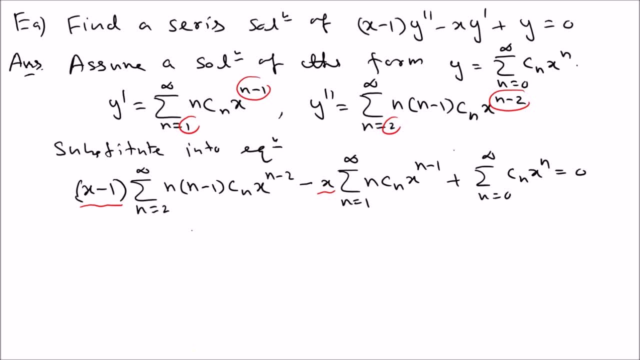 inside it's going to be x to the n minus 1, and then there's a minus 1 in front, the minus 1 multiplied by this. so we can start with that. so that means the first i'm going to be. now. that's the highest one, so we're going to. 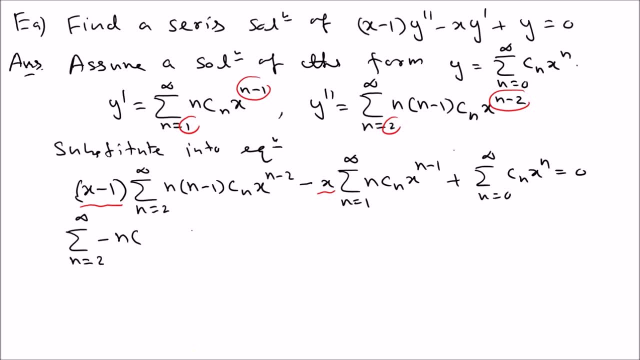 go with that, so it is minus, and go inside. if you have i plus one and you're going to go with that, so it is minus, and go inside. if you're n minus 1, c, n, x, n minus 2, because i multiply by the minus minus 1 and then let's start multiply with x. 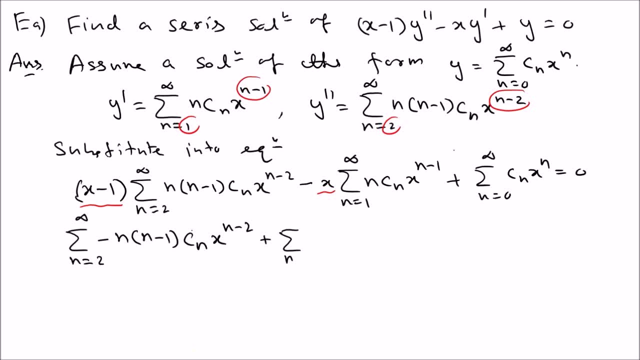 when you multiply with x, you get: uh, it's still n, going from 2 to infinity, no changes with the index: n, n minus 1, c, n, x. when you multiply by x, you become n minus 1. okay, because you multiply by x star, and then from the next one we can bring the x. 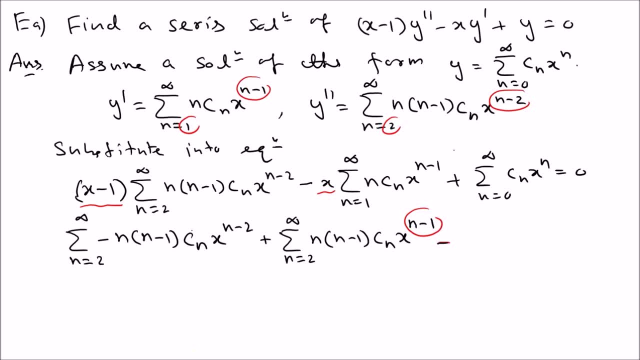 inside. uh, so if you bring the x inside, it's going to be sigma n going from 1 to infinity. n, c, n, x, n. why? because you multiply by extra x, so in minus 1 become n, and then the last term was the last term: sigma n going from 0 to infinity. 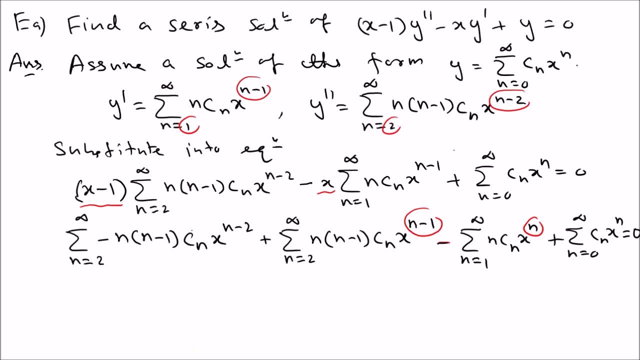 c, n, x, n equals zero, so you get uh now. so so we substitute and bring the x outside, x term inside. that's the next one. now, what we're going to do, we're going to see where the what are the starting terms. so that's what we check. so let's check. 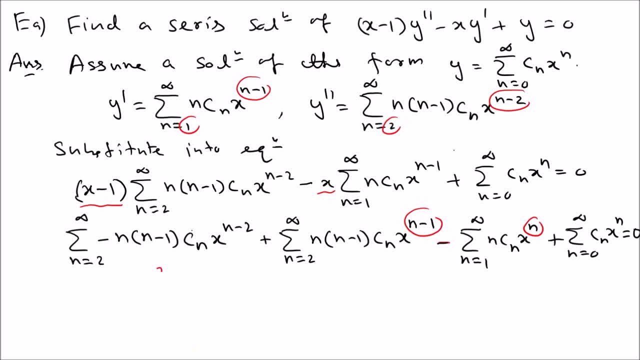 the starting term. if you buy n, equal to the starting term is x to the 0.. if you apply n, equal to the starting term is x to the 1. okay, so that's slightly different. again in the next one, if you apply n equal 1, starting term is x to the 1. 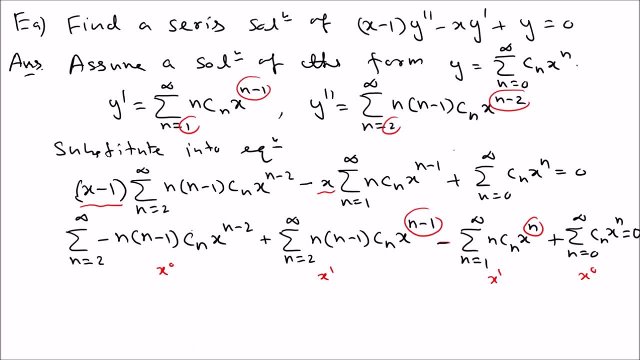 the last one, x to the 0.. so that means there are uncommon terms because, uh, in the first one, the last one, there's x, 0 term. that is uncommon because the other series, the other two series, does not have that term. so what we're going to do, we can write. 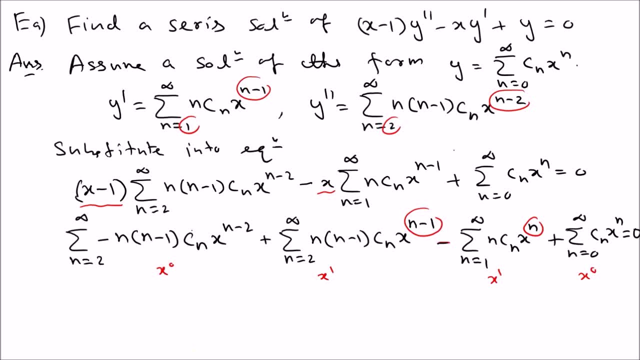 the uncommon terms first. so let's try the two uncommon terms. there's a one uncommon after that. if you start with the next index, that means n equal 3. you can see that you get x 1 in the last one. also, if you start with n equal 1, 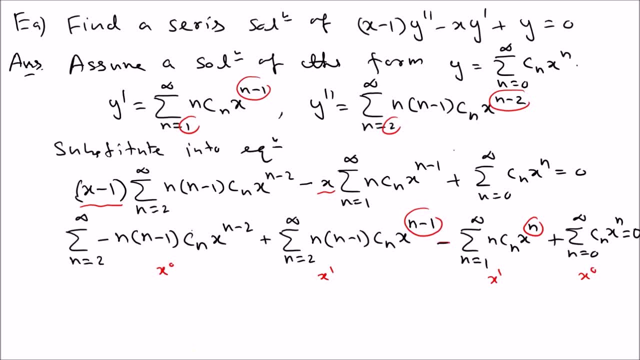 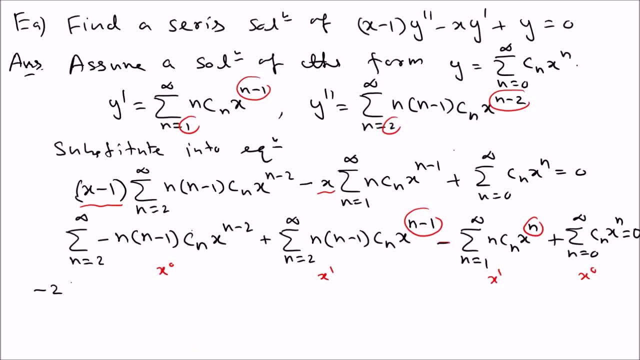 when you buy n equal 2, so that means it is negative 2, 2 minus 1, c, 2, x to the 0. that is the uncommon term from the last one. find the last term. you also get uncommon term when you play n equals 0, so we write that and then what we can do, we're going to 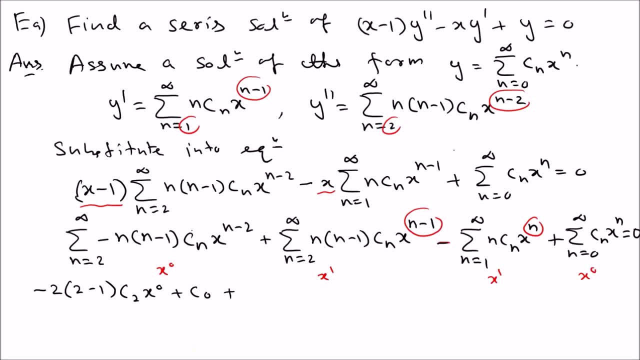 write the rest of the terms using the proper index. so in the first one. now you can see that n equal 2. we already plug in, so we apply n equal 3. now. okay, because we the first one. we already wrote so minus n, n minus 1, c, n, x, n minus 2. no change, it's just the. 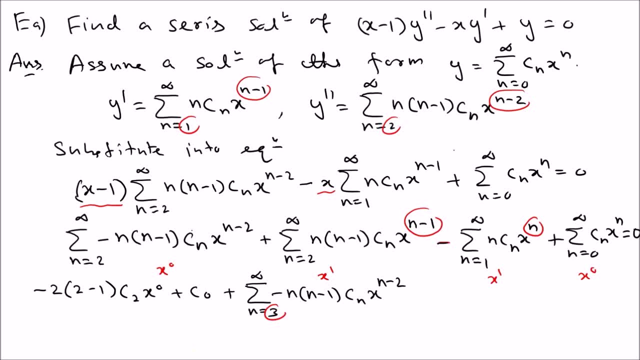 index. so we write that down, just the index. the next term: no change, because only for the uncommon term. so no changes here. yeah, there's a lot of writing i don't know even in our space here, and then i'm gonna write here negative. uh, no change, because still this is a common term. 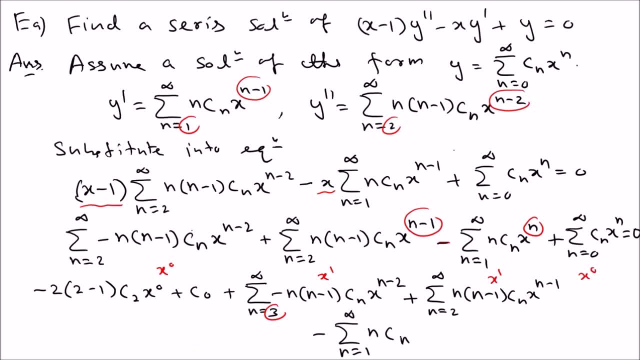 so we can write n, c, n, uh, x to the n from the last one. it has to start with n, equal, not zero, but one, because we already wrote the first term there. so that is what we do next. so we write, we change the indexes only for those uncommon terms. now, what we're going to do, we're going. 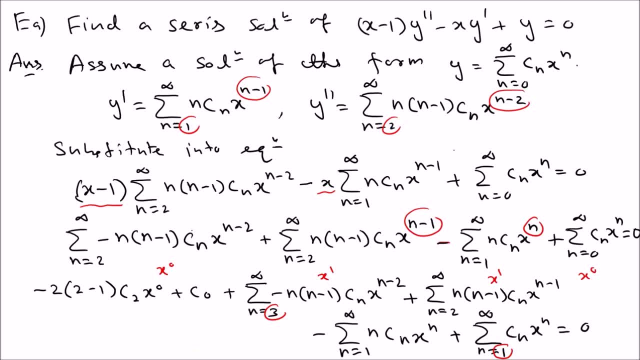 to use the c so method. now we're going to re-index. now we can re-index and see whether we can bring everything into one common index. that's very easy to do. so let's look at the terms. now you can see we need to bring it to xn if possible. so 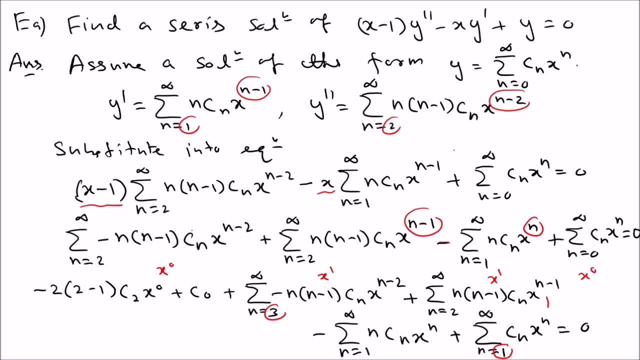 how to do that. we're going to, uh, bring this one by up by one, this one down by one, so then it's going to be xn, power, xn. here you can see, you want to bring this one up by two, so this one down by two, uh, and then everything else in xn. so point. so we only need to change. 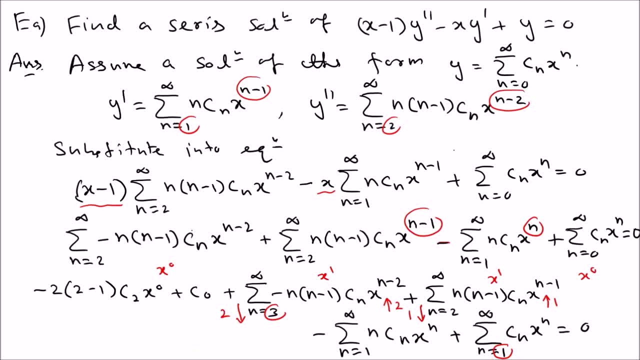 the index of two, just two series. so let's do that. uh, so we're gonna get, after we. uh, re-index. uh, so we're gonna get. so we're gonna start with the. uh, we'll start with the, with the first one and then, uh, only the. 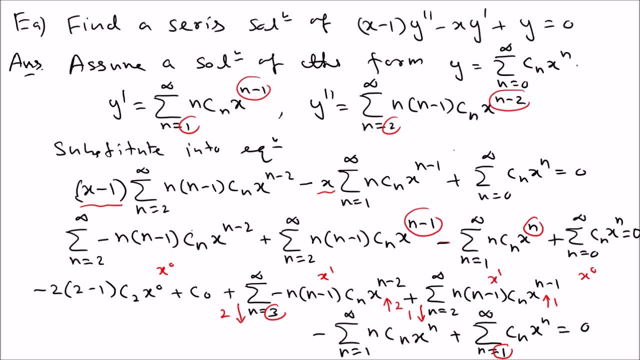 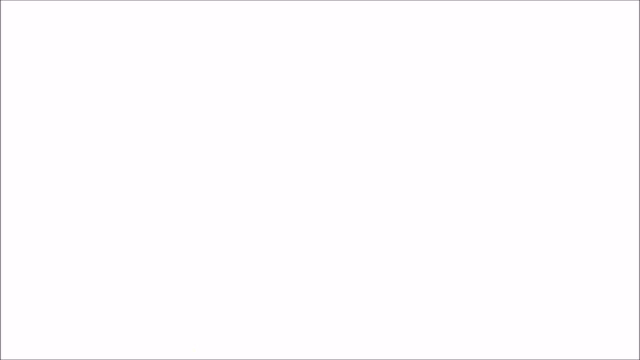 the first two, and then we have uh, the other two. we can combine them also, because you can see the last two, you can actually combine them into one uh. so let's uh do that. so we're gonna get uh. so we have this now. so we have negative 2 c, 2 plus c, naught, we have that, and then 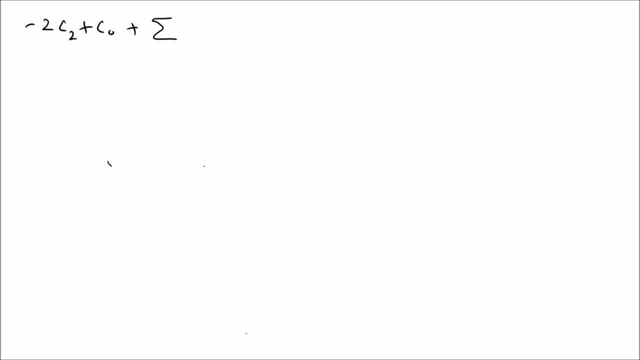 we're going to use the c so method for re-indexing. we're going to bring it down by 1, down by 2, down by 2, so it's becoming equal 1, because we had n equal 3 before it become 1 infinity. no change now. inside you can increase everything. 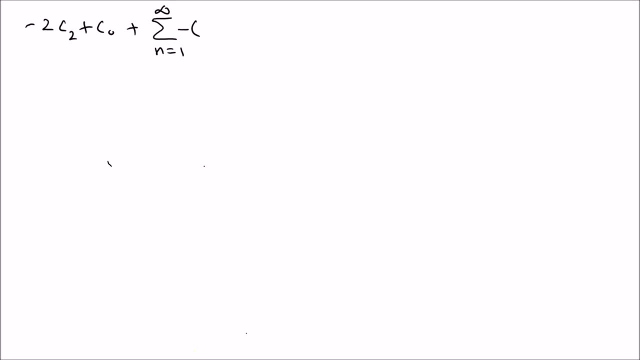 by 2. so you add 2 outside, you subtract 2, inside you add 2, you can end the product and you'll get this n become n plus 2.. uh n minus 1 become n plus 1. c uh n become n plus 2. 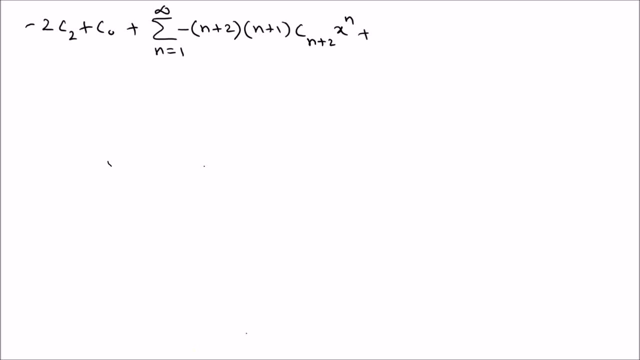 x n minus 1 become x n plus. let's go to the next term, uh. in the next term, uh, we need to bring it uh down by 1, so it's become n, going from 1 to infinity. so you add 1, become n plus 1, and then we have n minus 1 that become n. this is c become n plus 1. 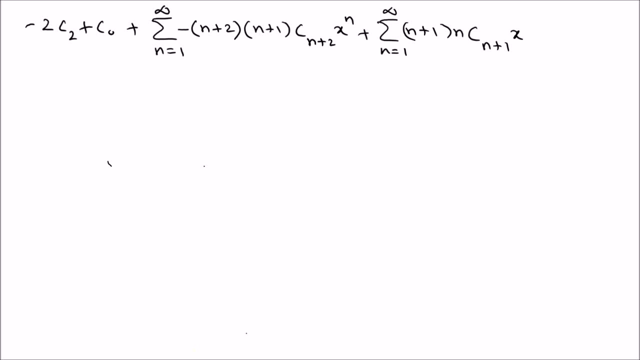 that is a plus uh. and then we have x n minus 1. that become x n and uh, what we can do with the last two? we can actually uh combine them into one because you can see they are the same. so we can combine them, uh. so we have uh. 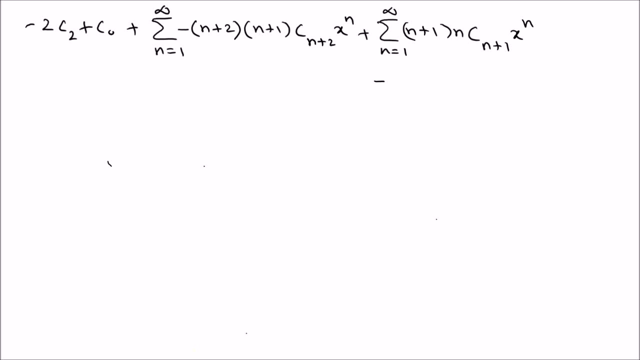 so, if you want, we can just leave it, because, just to keep the argument, so we are going from one uh to infinity, uh, n, c and x, n, and the last term is n, going from 0 to not 0, it's again 1 to infinity. 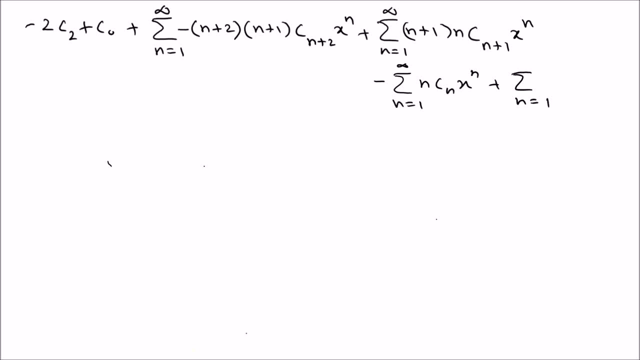 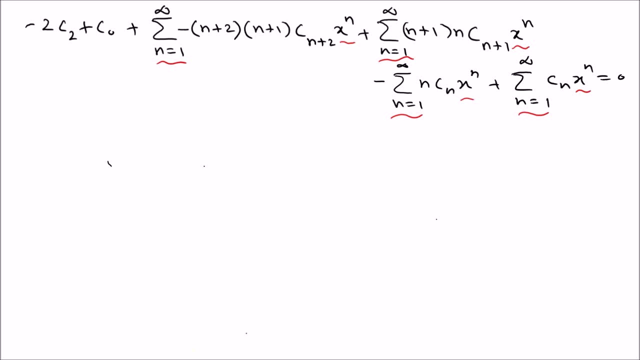 them. so we're going to combine them. so let's combine them. uh, negative 2 c, 2 plus c. naught. now let's combine. let's write the common index outside. so the common index is n going from 1 to infinity. that's the common index and let's put those t those terms. 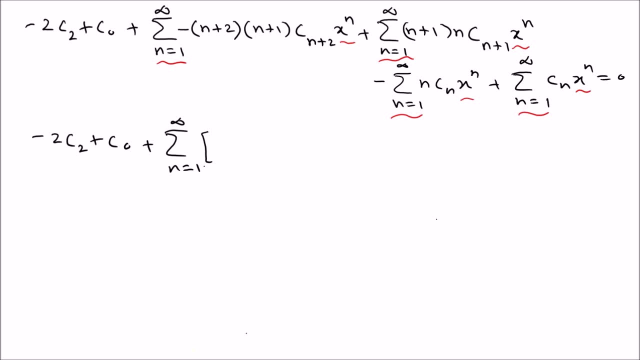 together. from the first one you're going to get my negative n plus 2, n plus 1, c n plus 2. that's the first one, and from the second one you're going to get plus uh, n n plus 1, c n plus 1, and if you combine the next, 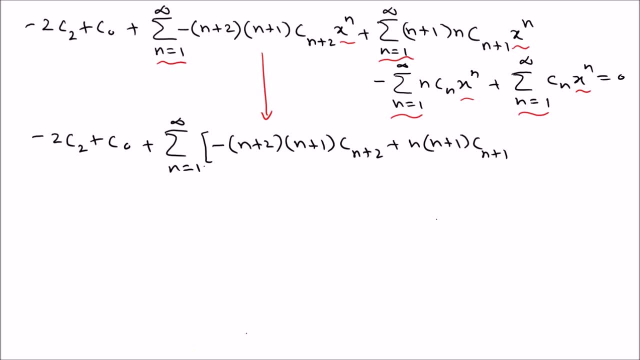 two. you can see, uh, one has a negative n c n, the other one has c n. so you can see you can write this one as uh. if you order the plus sign, it is 1 minus n c n. you can write it like that. uh, one has a negative n c n, the other one has c n. so we can write like that. and. 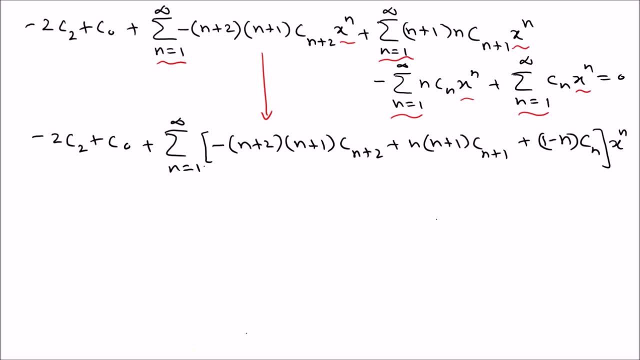 then write the x, n power outside, which is: whole thing equals to zero. now again, if this whole thing equals zero, what we're going to do? we're going to equate the coefficients of each term, each linearly independent term. so you can see that this implies that 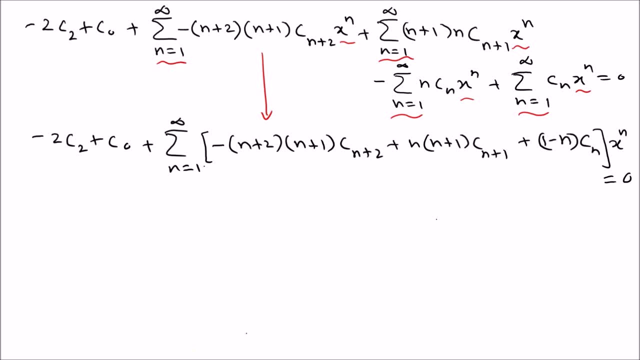 the first thing implies, that is, this has to be zero. the other thing is that this term has to be 0.. so that's what you get. so let's put those two together, let's set them equals zero. so if you said the first one equals 0, 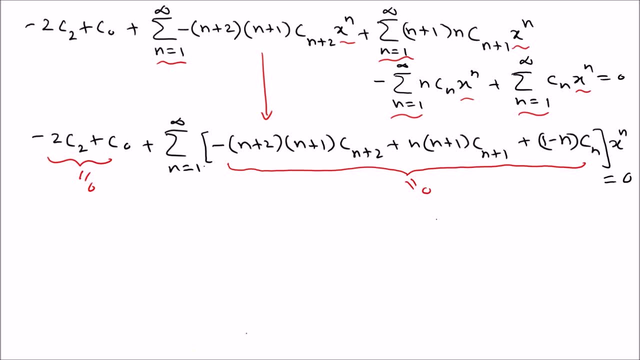 uh, so you're going to get. you can solve for c2. you can see that the c2 equal 1, half c naught. that's what you get. if you said this equals 0 and solve for c2, you get that, and from this c n plus 2. so i'm going to solve it here, uh. so if you solve for c n plus 2, 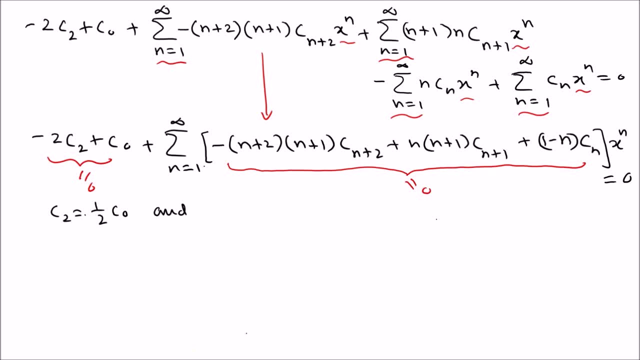 just set this equal to 0 and solve for c, n plus 2, so you're going to get simply n plus 2, equal. uh, you can see n plus one term get cancelled from the first two terms, so you get n over n plus 2, c, n plus 1 minus, and then you're going to get: 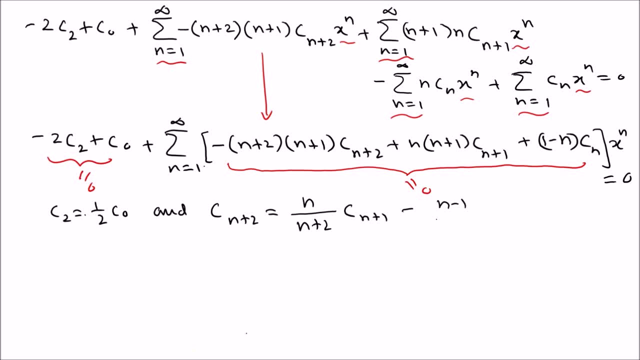 n minus 1. i put the minus 1 outside, it's easy. and then we have here: we have here, we have n plus 1 over n plus 2. so n plus 1, n plus 2, c, n. so that's what you get, okay, and this is valid for n going from. 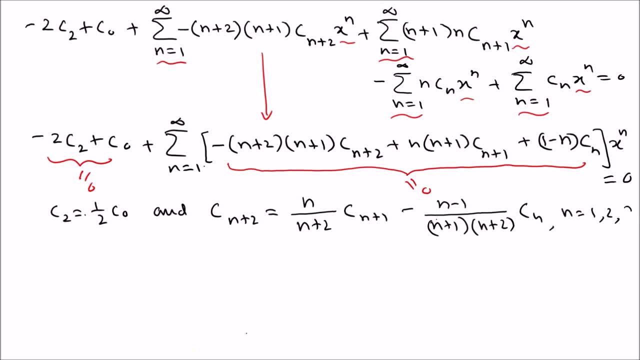 what is the index value? one, so starting. one, so one, two, three, you can see that's the exact same indexing value here. see, that's the starting. okay, so that's the relation. so that means, uh, we know the, uh, we know the relation. though what we can do is we can. 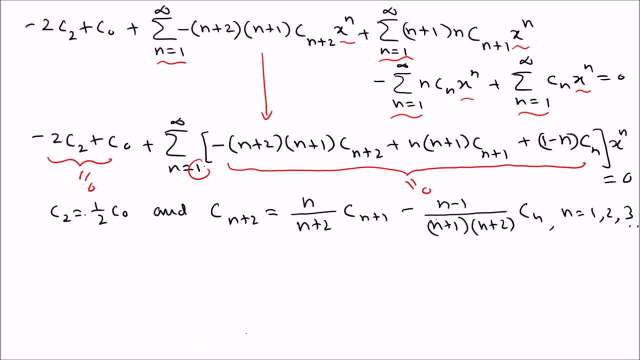 calculate few. we can start. we start plugging the values and then try to calculate a few of the uh terms. so let's do that, okay. so after that, after you get the relation, okay, so after that, after you get the relation, okay, so after that, after you get the relation, we can start calculating values. 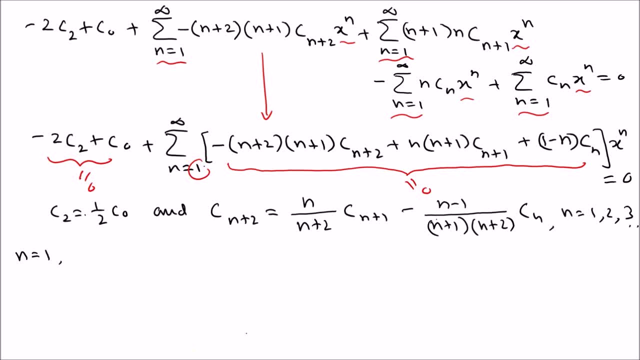 we can start calculating values. so we can start with the first indexing value: n equal one. if you write n equal one or you're going to get c 3, so let's plug in. so if i n equal 1, what will happen is a 1 and then 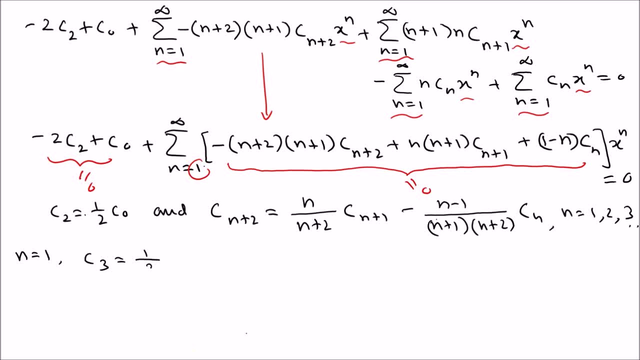 over n plus 2, that means 3 c. n plus 1, that means c 2 or minus. if you put n equal 1, what will happen? n minus 1 becomes 0, so you get 0 times c, uh, c 1. 0 times 0 times c 1, that means c 1. 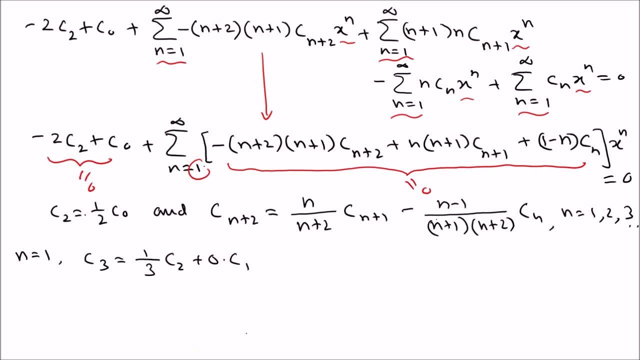 disappear with 0 times. okay, so that's what you get, um. so, in other words now what we're going to do, we're going to substitute for c 2, because c 2 we already know from the previous step. see: c 2 equal one half c. no, so let's plug in there, since. plug in there, you. 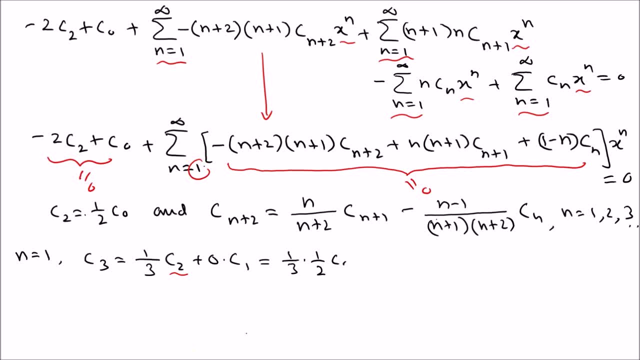 get 1 over 3, 1 over 2, c naught um. in other words: uh, you can see that later it is factor- factorial three c naught. factorial three means what? what is factorial three? factorial three means three times two times one. so you're gonna see that. 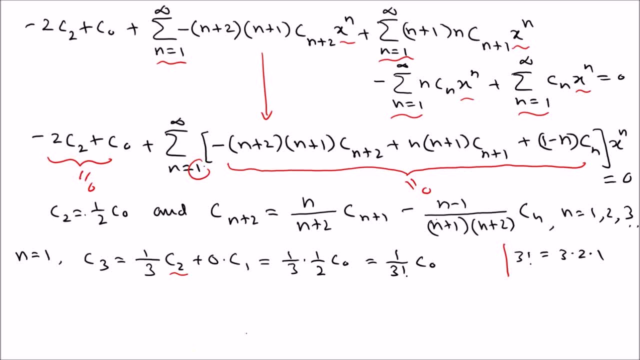 gonna appear here. okay, but if you don't see, that's okay. when you write few more terms, you're gonna see that. now let's try to calculate the next term. so we're gonna calculate n equal two. so by n equal two, this becomes c four. so let's plug in equal two in the. 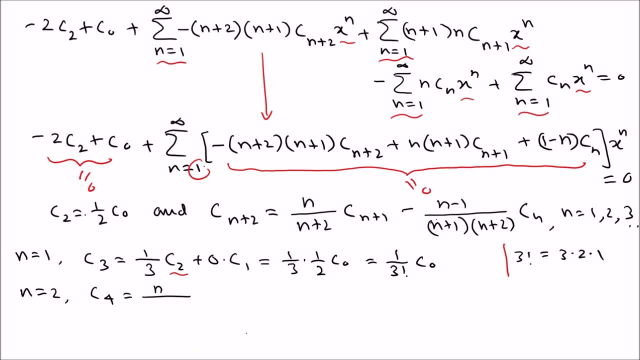 equation. it's a two over, nope, it's a two over. so it is uh, two over uh. so when you plug in two, it becomes four c, three actually, i don't want to write that large. so it is two over man. so it is two over four c. 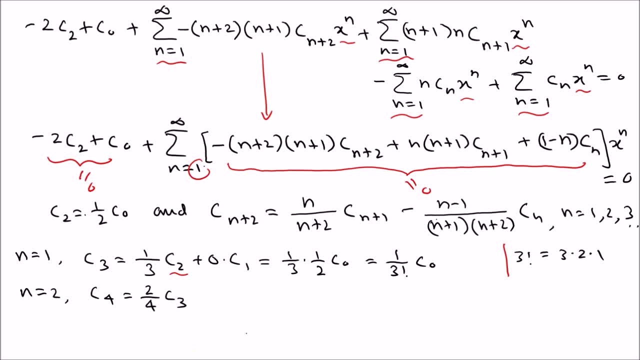 three and then, uh, minus if i n equal two, that means for one over. what do you get here? when you play n equal two to the equation, you're gonna get three times four. so four times three c two. that's what you get now, what we can do. 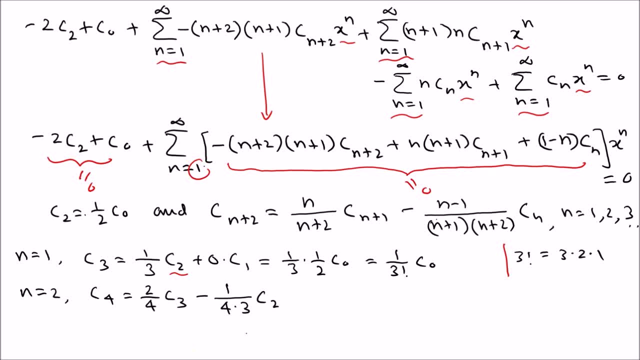 we're gonna plug into c two and c three, both of them. so let's plug in. see, plug in what you get from the first one. you get two over four, c three. what is c three? it is factorial three c naught minus one over four times three. plug into c two. c two is one half c. 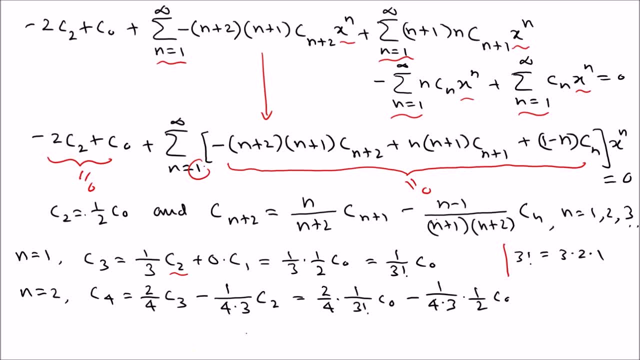 naught. now you can see that this is: they have the exact same denominator. that means they have the exact same factorial four, and then in the top it is two minus one. two minus one means one. so that means it's nicely simplifies to factorial four c naught. that's interesting. 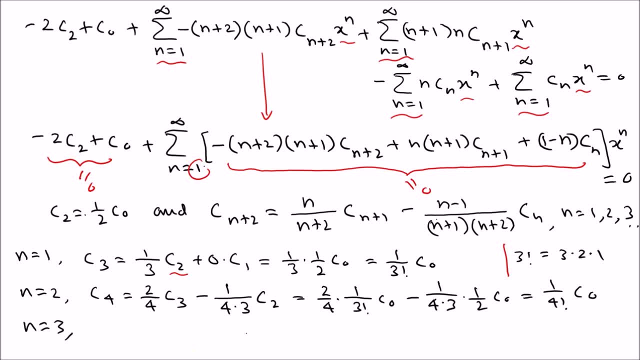 the same thing: n equal three. let's choose one more, then you can see it's clear. so you're gonna get three over um five times four c four minus one over e by n equal three. so it's gonna be five times four, uh c three. so let's plug in here. 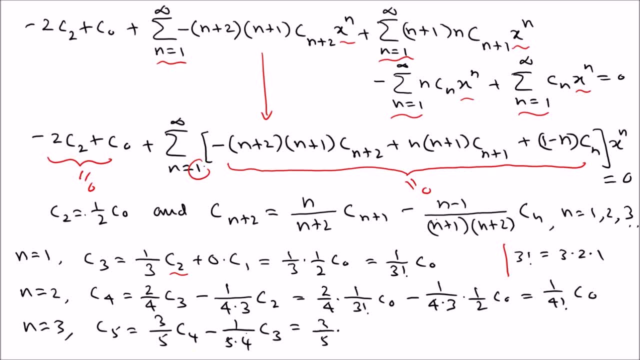 so you get three, four, three, fifth c. four means factorial four c naught minus five. four c, three c, three means factorial three c naught. denominator is simply factorial 5 now, and the top is 2 minus 1 again. so that means uh, uh, is that right, uh? 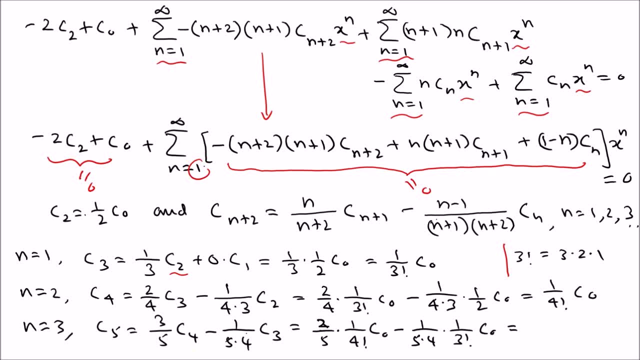 so, uh, yeah, actually there's a, there's some typos here, so it is not two, this is three, and also this is not one anymore, so this is three, so three or five, and then, uh, here it is. uh, you plug in: equal three, this one, two. you have two or two divided by five. 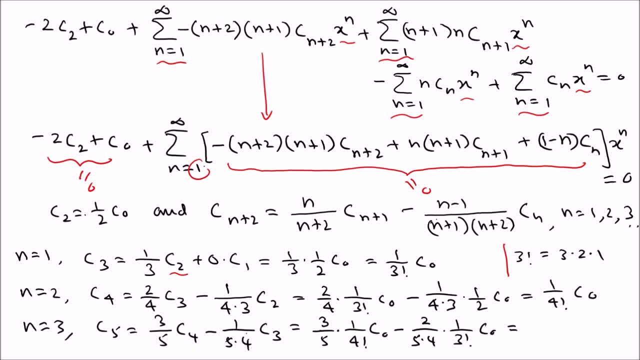 fourth, because n minus one- and you can see now it's again simplifies very well. same denominator: the top is 3 minus 2, that means 1, so it's going to be 1 over factorial 5 c naught. so that means you can guess. 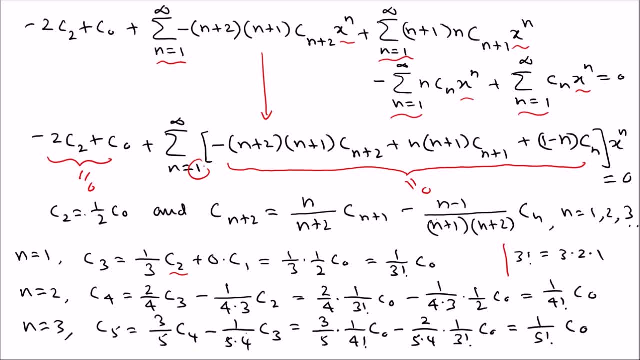 what's going to happen with for c n. c n has to be 1 over n- factorial, so that means you can guess what's going to happen with factorial c naught. so in general. so that's why. so once you write few terms, you're going to see a pattern. okay, so try to find. you just write few. 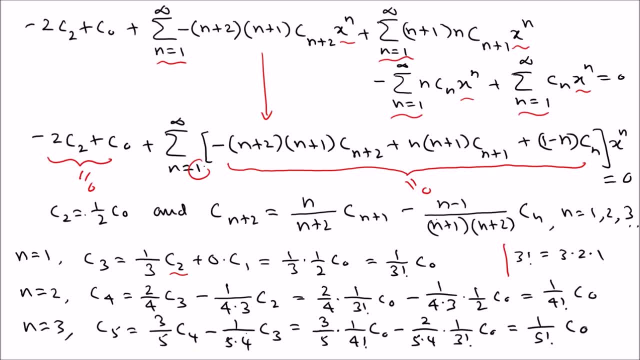 terms until you see a pattern, or if it's a difficult problem, what's going to happen? uh, the problem will ask you to write just the first five terms of like four terms. five terms like that if it's a difficult one, but if it is like like this problem, 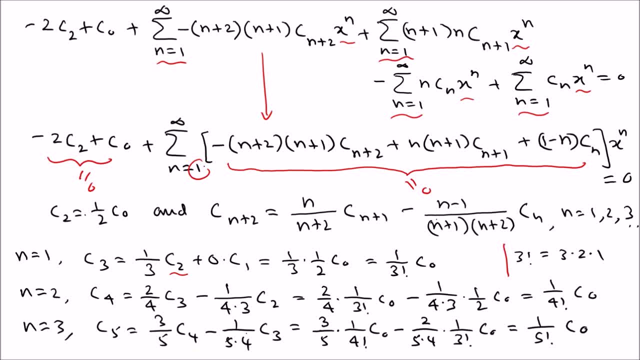 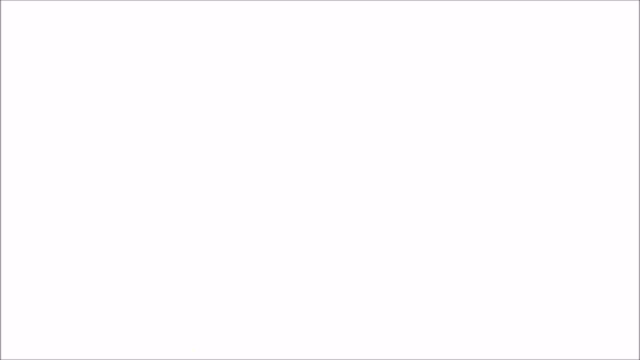 very nice, you can solve them. you can simply go forward and find it okay. so it depends on the problem. it's a difficult one. just like, few terms is enough, okay. so let's now you can see in general. okay, in general, you can write c, n, which is: 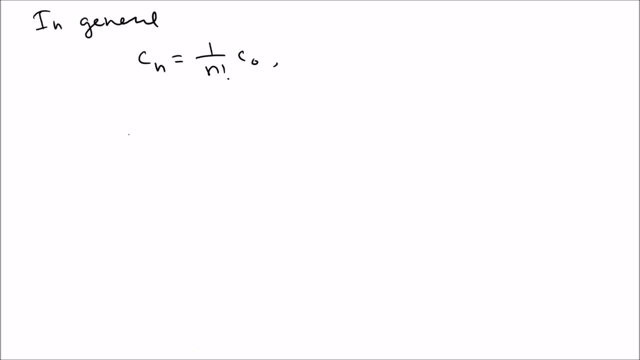 1 over factorial n c naught, which is valid n going from: uh. so what's the starting value? uh, we can start with n equal 3, right? uh, yeah, because we apply n equal 1, but we start with c3, so that means starting with 3. so 3, 4, 5, like that. 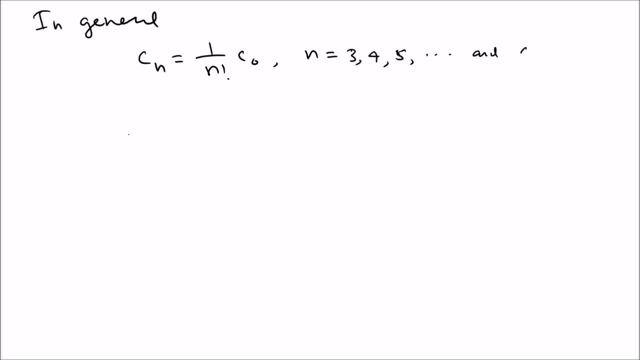 but uh, we also know that and we know that c 2 is one half c naught see fortunately that also the exact same format. so that means we can simply write this one as c n is factorial. uh, five factorial c naught for n going from uh. 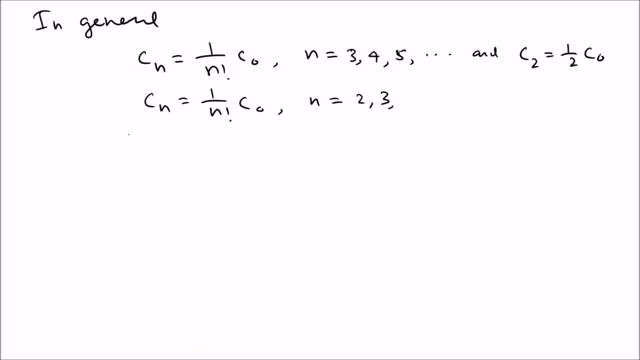 2, 2, not just 3, because it has the exact same format. you see, this is the exact same format. good, so that means now we know the general form, so let's plug in: okay, so, uh, we can substitute that in the equation. so substitute. so when you substitute easy y, uh, which is: 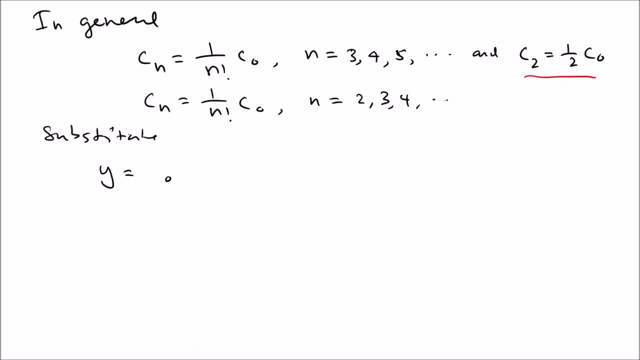 c, uh. so let's write the formula. so this is the sigma notation. so we can do, we can plug in that. so in going from zero to infinity, c and x, n, so which is c naught plus c, 1 x plus c, 2, x squared like that. so let's plug in. 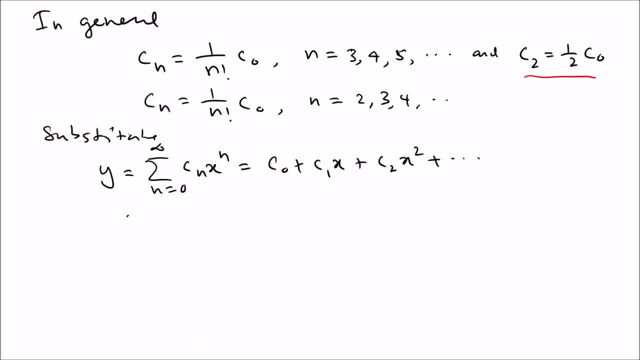 here. so when you plug in what you get, uh, so you're going to get, uh, we like c naught, we leave c 1, we don't get from here, so we can leave that. and then, starting with uh, c 2. we have a formula, so it is 1 over factorial 2 x squared 1 over. 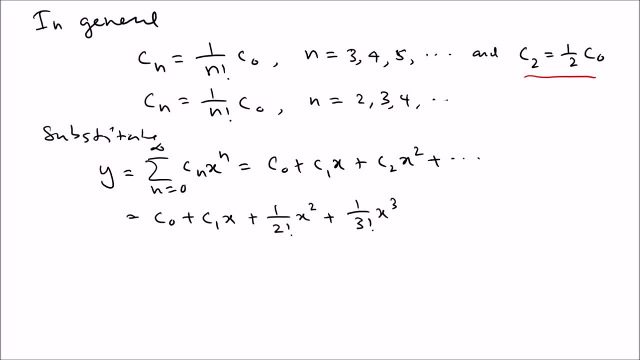 factorial 2 x squared cube like that. uh, actually, uh, and also, we forget the c? naught term. so let's write that, so i'm gonna. yeah, you can put that top. so this is c? naught. there's a c? naught um everywhere. you see no times. 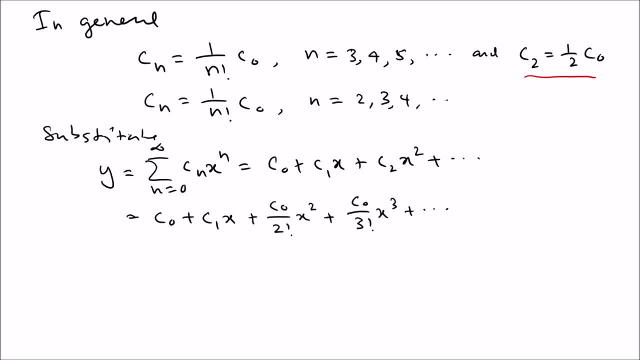 okay, so you can see. so that is the case now what i'm gonna do. um, you may or may not see a pattern here. the only thing that you can do is you think missing here is the c naught term for the x to the first power. so what we're going to do is we can write like this: now we 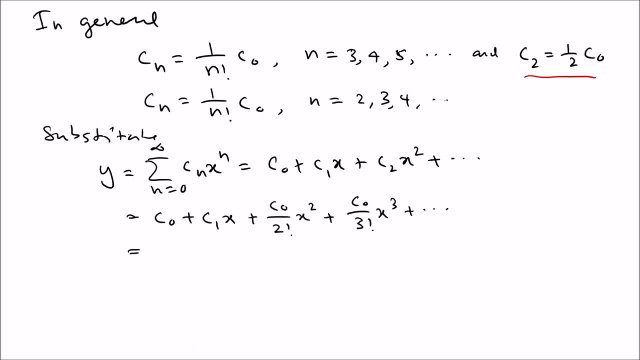 can write this one, as i'm going to add and subtract that term. so, um. so, what we can do, i'm going to add and subtract so we can write c 1 minus c naught x. that's the first term, x 1 term, and from the rest i'm going to add here to c naught. 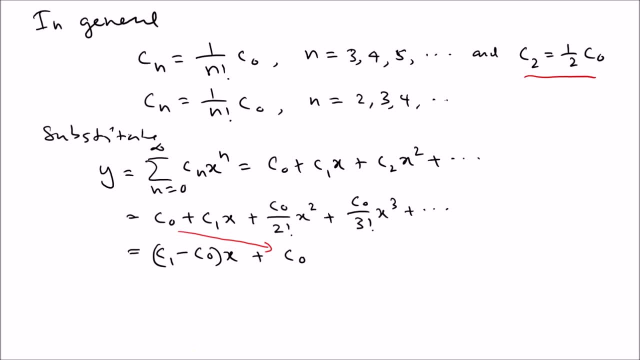 coming here. that's that c? naught term. so i'm going to write the rest. so here we can add the c? naught term. so this is a c? naught x term. that's the one i add. so this is subtract i add. so add that subtract now, write the rest. just write the rest. 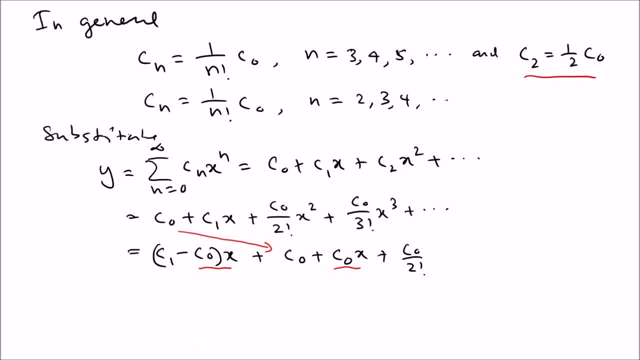 so what's the rest? c naught over 2 factorial x squared. c naught over 3 factorial x cube, like that, and you can see from the rest. so this c 1 c naught is just a constant. i'm going to say it's a big. 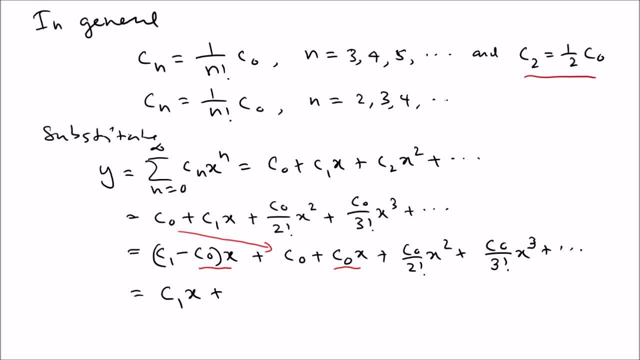 c, 1 plus. what's going to happen here? here we have the c naught uh term so you can pull the c naught out. so if you pull the c naught out, uh, it's just like just a term. um, so what do you get? you get 1 plus x plus1 2. factorial x squared plus. 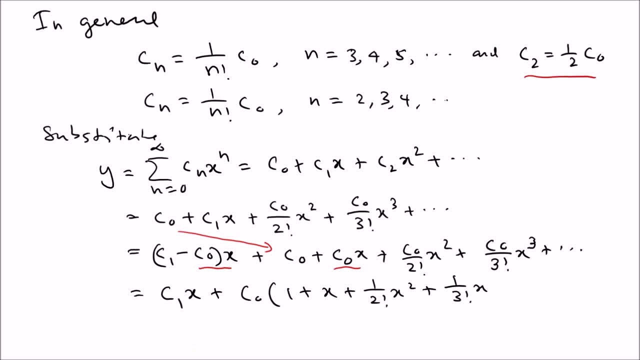 3 factorial x square. this is simply the e to the x. so that means you're gonna get, uh, this c1 is not the c1, this c1 is simply equal to c1 minus c. naught, so i'm gonna. i just, it's just a number, that number i. 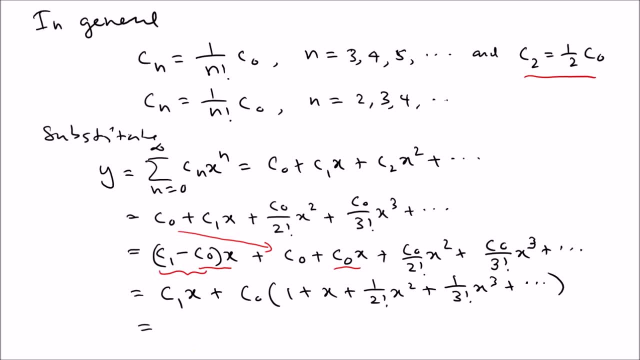 call c1, uh, the big c1. so we're gonna get, uh, uh, c1, x plus c, naught e to the x. so that is the solution of the differential equation. it's very easy to get of the differential equation. it's very well simplified and sometimes this happen. you know you can do that, but not always. 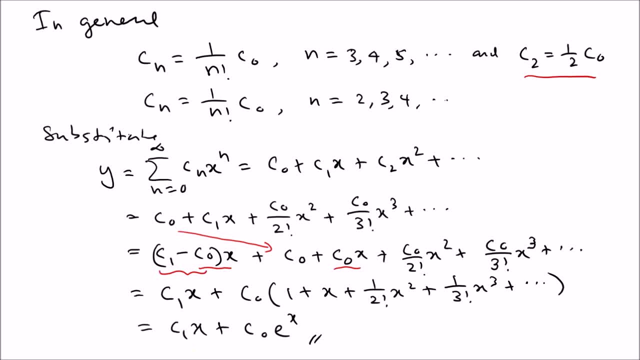 so this is the kind of thing, uh, but in a final exam, in exam, this may not be possible unless it is like a, like a short problem. uh, the first problem is okay, um, but you know you will get a manageable problem, but this is a pretty long, a little long. 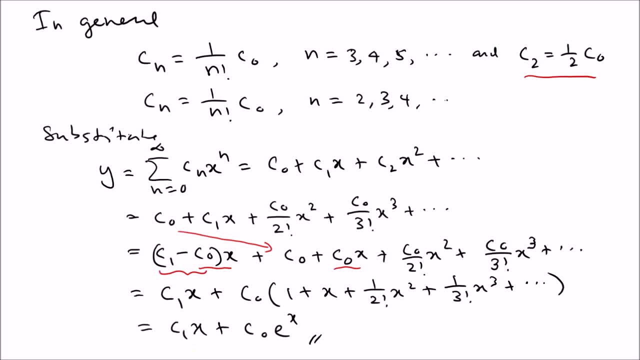 um, unless you can do it really really fast. but in exam we don't expect that, because you know where you have a lot of things to do. so but what? i'm going to show you how it works. okay, this is how it works. sometimes it works very well, uh, so you will get something manageable, okay. 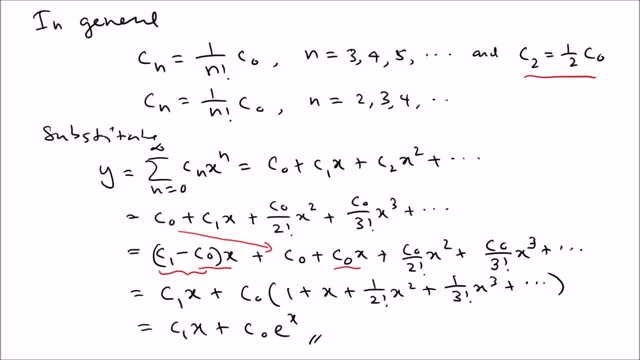 not like this long, so you can look at the problem that you get for exam one. i think it's like: okay, good, so so that is the uh power series method and you can like do any problem like that. so it's not difficult, but you can see, it's like a simple thing. so 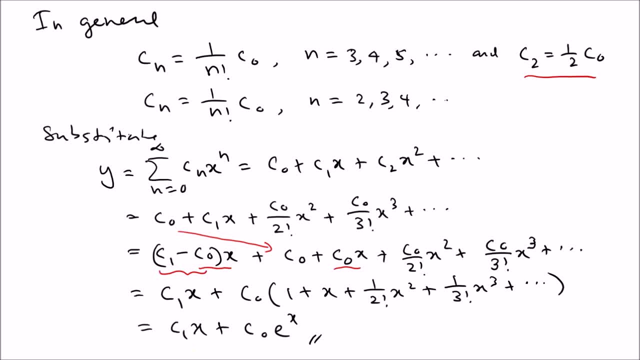 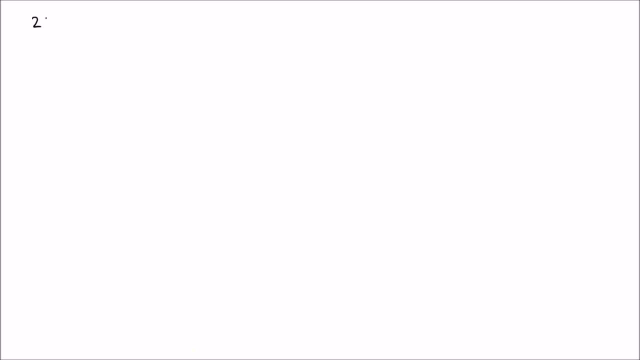 next, uh, we're gonna do is the. we're gonna talk about laplace transform and method. uh, so let's talk about the laplace transform method. so it's a number 24, uh, the laplace transform method, a plus a transform a method. so this is again a very powerful technique. you can do a lot of problems. 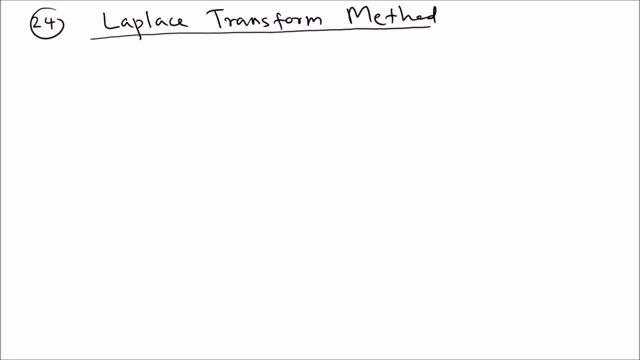 using this technique because we know that we get stuck when you try to find the solution with the undetermined coefficient meter, because there are only three, three uh problems that we can do, three type of problems that we can do, and then also, if you try with the 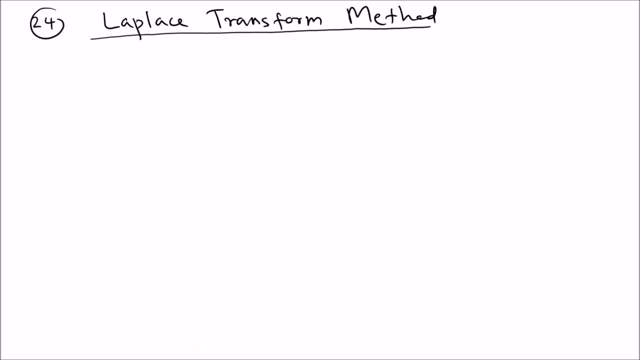 variation parameters. uh, you get integral. that may be impossible to um like, get the cross form solution. then we have this new technique, the vertical laplace transform method. so let's try to uh look at the definition of laplace transform. so the definition. let's say you have a function, so uh, for. 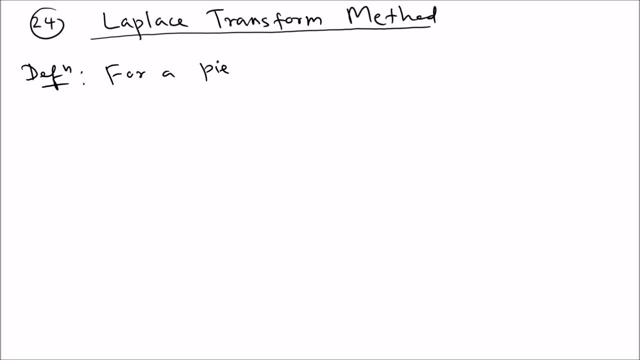 a piecewise continuum, piecewise continuous, piecewise continuous and exponential order function. for a piecewise, continuous and exponential order, that means it's going to grow slower than and like an exponential function that's exponential- other functions, or at least at the level of, at most at the level of exponential function, lean expenses. 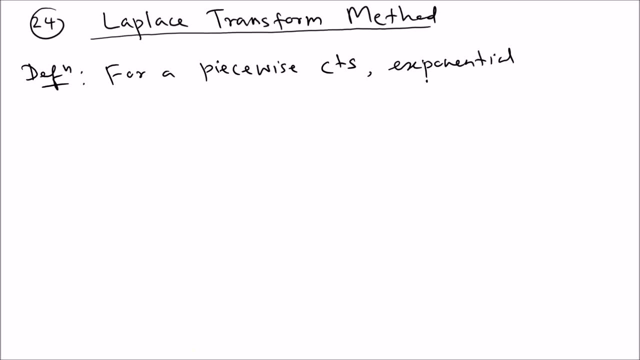 function. it doesn't grow faster than that. so, um, piecewise, continuous and exponential order function. exponential order: okay, so that means it's slower than e to a k t function: slower than that. so maximum is like that. uh, exponential order function. rf. the laplace transform is defined to be the laplace transform. 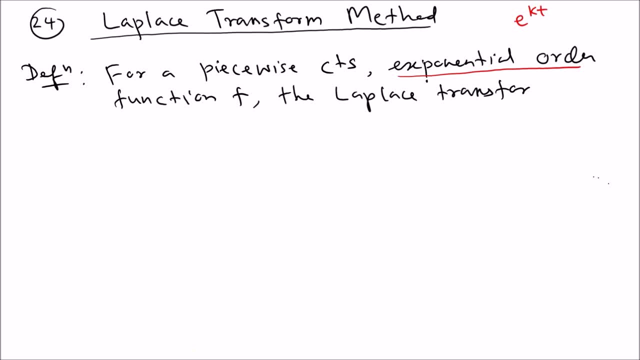 laplace transform is defined to be uh- we can use this notation- curly rf is defined to be l, uh, f, equal. it is from zero to infinity, e to the minus s, t, f, t, d, t. so you get in, you integrate with respect to t and the limits going from zero to. 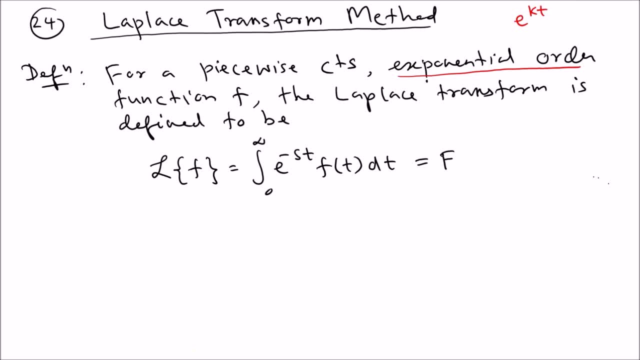 infinity. uh, we write this one as f? s, because once you integrate you get the function of s, so we write it like that. so we use uppercase f for that. so that is the definition of a laplace transform. okay, just an improper integral. you learn improper integrals in calc. 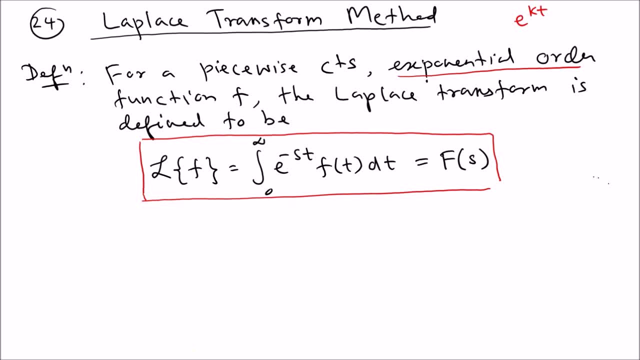 2. so we use that both side here. okay. so let's use the definition to find a laplace transform. it's just a simple function. so let's say, example: find the laplace transform of, let's say, 2t minus 3. just use the definition to see how it. 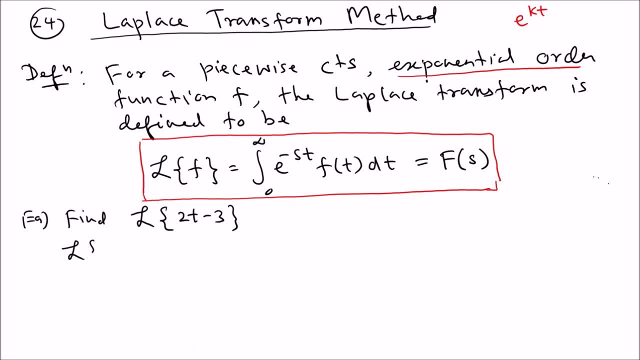 works. so the laplace transform of 2t minus 3 is, by the definition, zero to infinity, 2t minus three times e to the minus st dt. you can see this is a good candidate for um integration, but parts. so let's do that. seventy is a regular technique. you can use the di method, no. 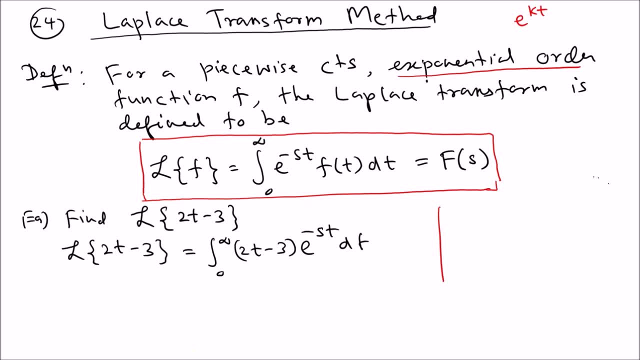 problem. so if you use a regular technique you has to be 2t minus 3. dv is negative. my e t is equal length. we take the derivative of this one, so du equal 2 dt. we take the integral of this one. s as a parameter is a act as a constant. 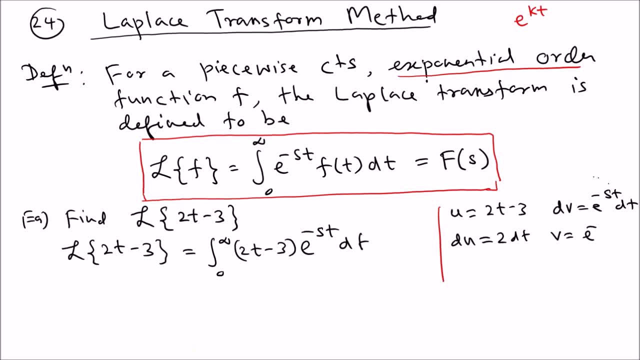 so it is e to the minus s, t divided by minus s, because you divide by the constant term. that's how you integrate a exponential function. that's a constant, you divide by that. okay, so we have that. let's plug in here. uh, so if you plug in and you're going to get um, so it's a uv minus. 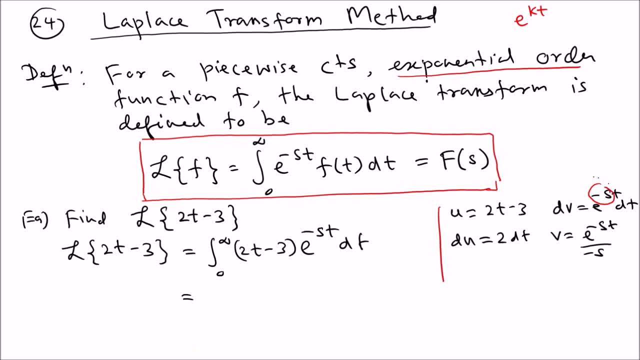 vdu, so uv. so it is 2 t minus 3, that's a u, uh, v is e to the minus s, t over minus s in limit going from infinity to zero, and then uh, so uv, minus, vdu minus, but there's a minus sign. 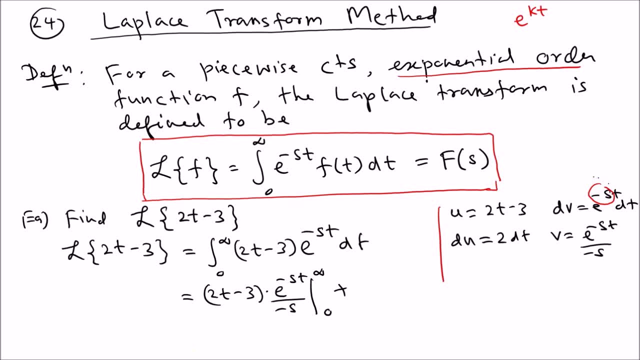 there, so it's become plus. uh, there's a two. i'm going to write it down: so uv minus, vdu minus, but there's a minus sign there, so it's going to write the two outside. so um, um so vdu. so you can see. the first product is the top row. 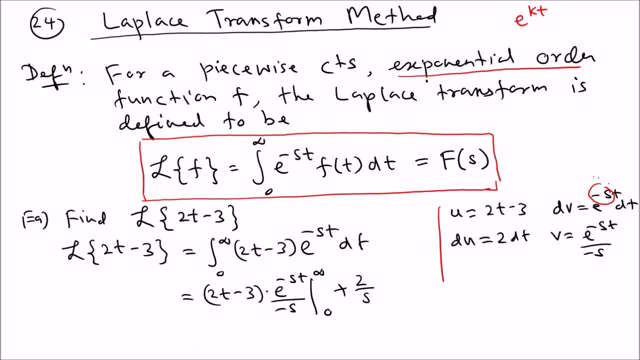 that's the integral. integral is the top row, the other one is the bottom row, you can see. so that's the bottom row you get. now we are not writing, so it's 0 to infinity the bottom row. so let's try the bottom one in some space. 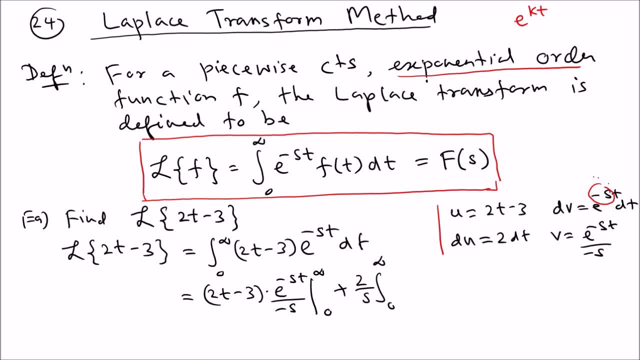 here. so, um, so, let's try the bottom row. that's the bottom row. it is uh, so with the minus sign, so it become plus 2, so we multiply this, so i write s outside, so you only have negative s t dt. that's the bottom row. top row is the integral. 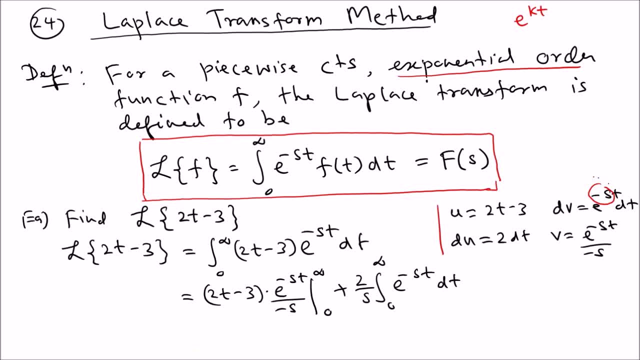 bottom row is the second integral here. that's how you remember the integration parts. okay, now you can see: uh, let's plug in here. so if you plug in infinity, uh, now there are some problems because you see that one goes to infinity, one goes to um, one goes to zero, one goes to infinity, because the polynomial goes to infinity. 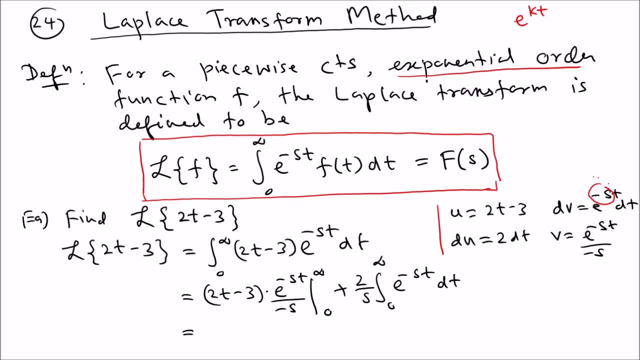 so when? so that means the indetermined situation. so you have to use the lopita's rule. but there is like a small result that you can remember: when you try to compare with the exponential function, exponential function always win. so that means, whatever happened, the exponential function. 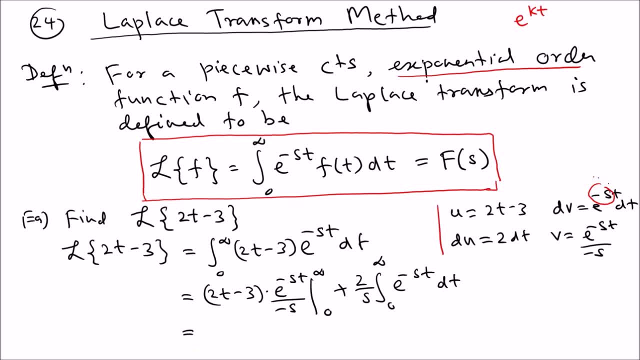 everything happened, the whole thing. the same thing happened, had happened to everything. so in this case, exponential function, exponential part, goes to zero. that means the product has to go to zero. so that's the result when you have a exponential fun function and a polynomial exponential function wins. okay, so the 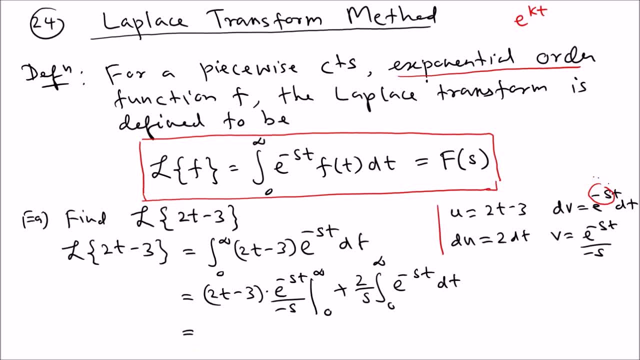 whatever happened to the exponential function, the same thing happened in the product. so that means, when you plug in, infinity is zero, okay, so you get zero, uh. when you plug in infinity now, when you plug in zero, because this is the uh we're applying for t, so you plug in zero for t, uh, so you're. 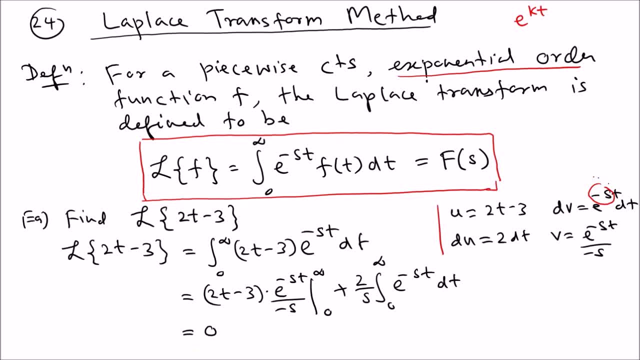 going to get uh, uh. so t term is zero is gone, so e to the zeros is gone is one. so you have three over s, but there are two negative sign and also there's a negative sign coming from the. when you subtract there's another negative sign. that means there are three negative signs, so you get. 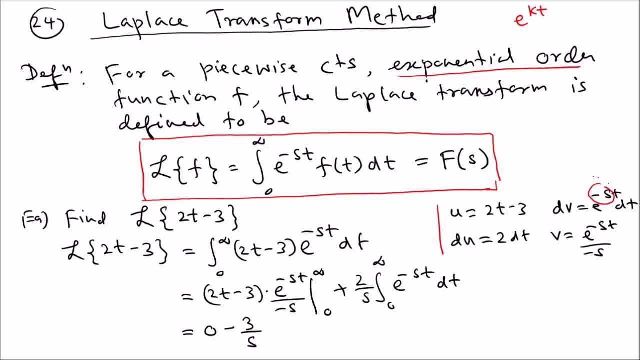 negative three over s when you plug in zero. okay, now the next one, uh, next one. what you can do? uh, you want to integrate that. so if you integrate, what will happen? so you have plus 2 over s when you integrate, you're going to get one more negative sign. so that means you're going to get 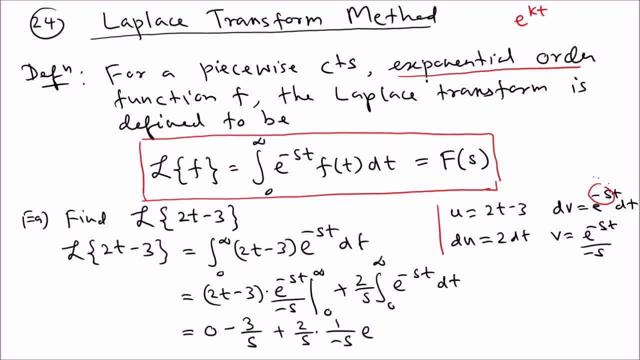 one over negative s e to the negative s, t. the limit: uh, infinity and zero. the same argument: when you plug in infinity, it is gone. when you plug in zero, uh for t, so it's one. with the negative sign, it's become plus, so that means uh, you end up getting uh. 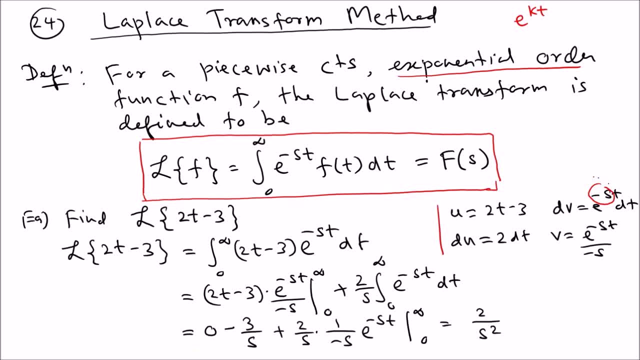 2 over s, squared minus 3 over s. so that's what you get when you finish the integral, and you can see that's not that difficult. so this is so this is just use the definition to get this one. okay. so what's gonna happen? we are not gonna do that, like every time when you. 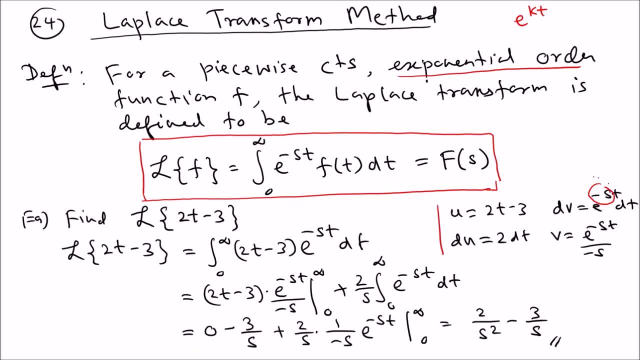 get this one. we use the table. so let's look at the common, few common values, uh, that you want to remember, and in the exam you will get the table. okay, so you get the uh, get a table that you use before. so, uh, these are the common ones, uh, so 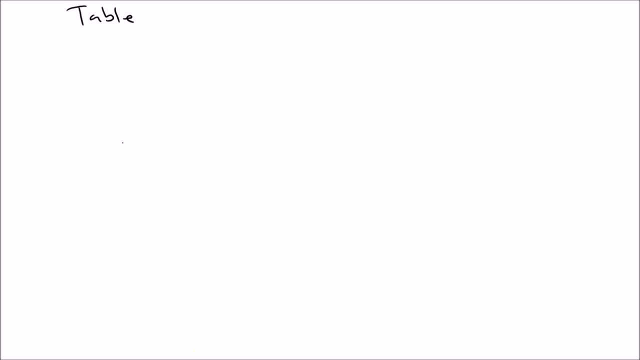 table of laplace transforms. this you need to remember. i mean it can help you. table of laplace transforms so um. so let's write the function and the laplace transform. so start with 1. laplace transform: 1 is 1 of s. uh, that's very easy to find using the. 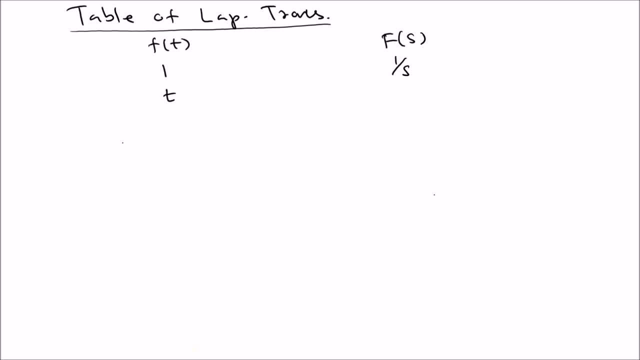 definition laplace, transform, t is 1 over square, those those you you kind of need to remember. and then we have t to the nth power, which is our factorial n, factorial n divided by s to the n plus 1. and then we have sine, omega, t. omega is a constant, uh, which is omega. 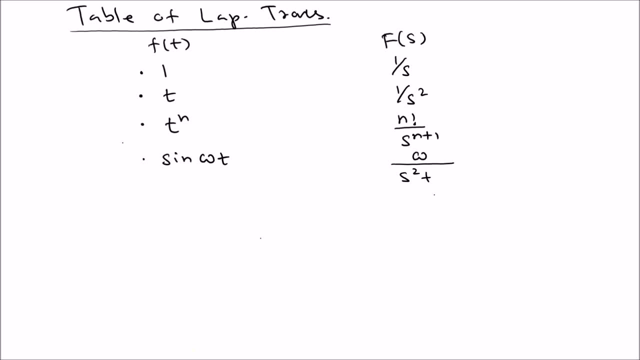 divided by s squared plus omega squared, and then we have cosine omega t, which is s s divided by s squared plus omega squared, and then, uh, we have the eat function e to the minus a t. so if you have e to the minus 80, uh it. 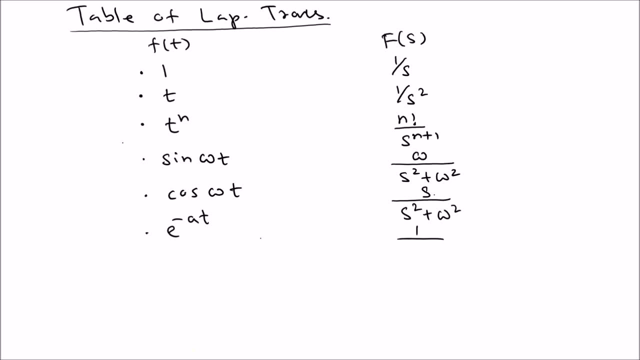 is 1 over s plus a, see the sign change uh. and then we have the um um heavy side function, u t minus a, which has uh e to the minus a t s over s. actually, you have to be careful. um, we divide in the whole thing by s. okay, so it is e minus a. 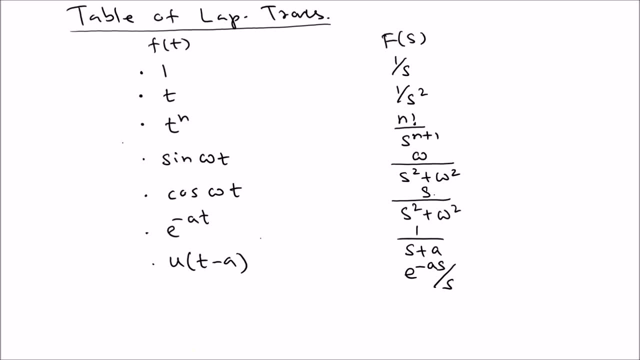 divide the whole thing by s, not just the uh minus a's part. and then we have the uh. first shift in theorem. it is e minus a t, uh eat ft. so if you get eat ft, the answer is you just get the laplace transform and then you get the laplace. 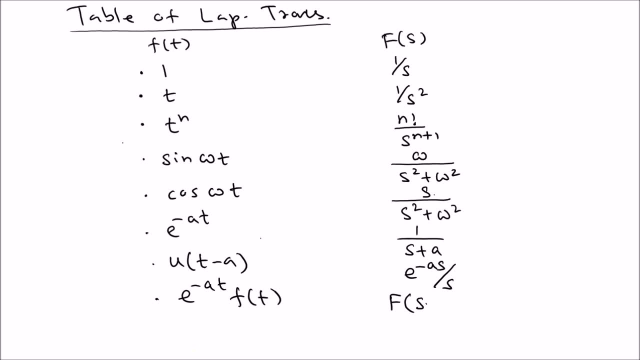 transform. and then you get the laplace transform, the function. you replace uh s by s plus a. so again, opposite sign. okay, opposite sign. so it's a good thing to remember. but in the heavy side function, same sign uh. and then uh, the second shifting theorem, uh, which is u. 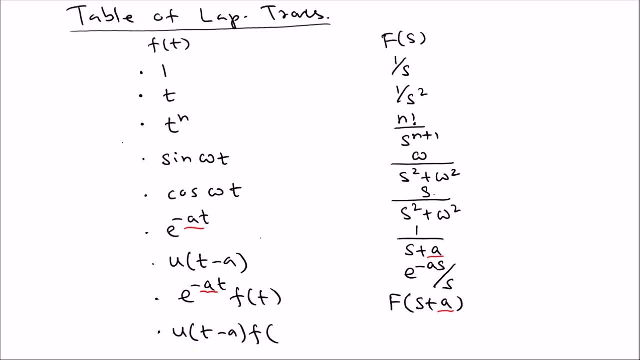 t minus a, f, t minus a, which is simply e minus a, s, f s. so this is what we call the first shifting theorem and this is what we call the second shift. so these are useful, uh, uh, when you try to uh find the laplace transform of the inverse laplace transform. so this is the 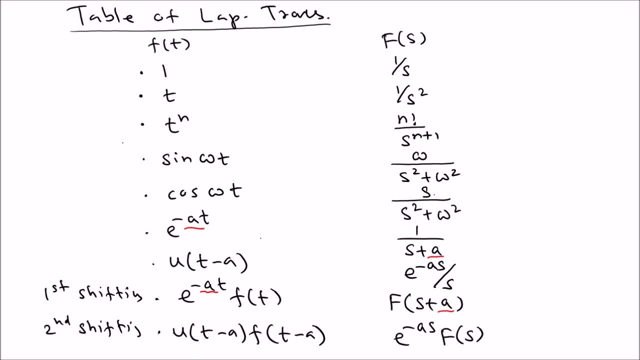 kind of thing that you cannot remember, because it's not that difficult. if you remember them, it's easy to uh find those inverse and laplace transforms. okay. so, um, and then there are some four facts about these uh, linear transformations- i'm sorry- the laplace transforms. one of the big fact is: 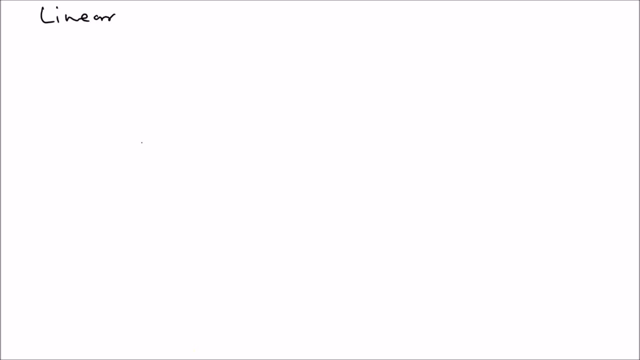 is linear. this is a linear operator. okay, it's a linear operator. what does it mean? uh, if you have a sum like that, if you try to find the laplace from the sum, it is simply the first one- plus or minus, it doesn't matter whatever. and then g. so that is the first condition. the second condition is: 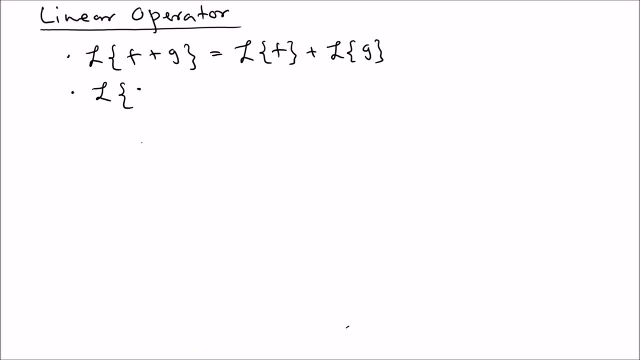 if there is a constant, you can simply pull the constant out. so those two properties can make life easier. uh, because it just act like we, as we expected. so let's try to kind of do our two problems from that. so let's do this one. uh, find the laplace. 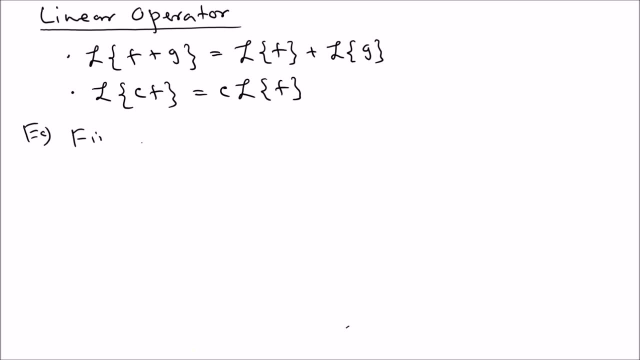 transform of find l, f, f, 4. the first one is: let's say: if t equal r, 2 t minus e, to the negative 2 t plus sine 3 t. so let's try to find the laplace transform. uh, soil f is. uh, it's a two times laplace transform of. 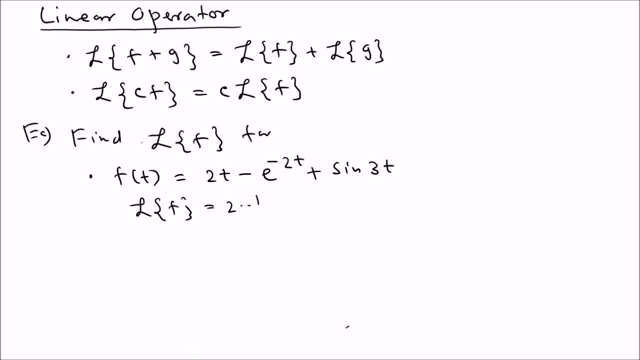 t is 1 over s t, so f is 1 over s squared minus. this is the eat function here- a equal 2, so that means 1 over s plus 2 and this is a sign we know this of table is omega or s plus s squared plus omega squared, so it's a. 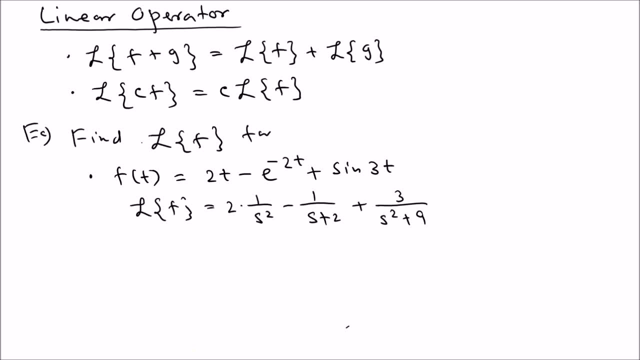 3 over s squared plus omega squared means 9.. ah, so that's the answer. i mean you, you can't do much with this, so we leave it like that. uh, let's do another one. uh, how about this one? let's say you have f t equal e to the negative 2 t plus omega squared. 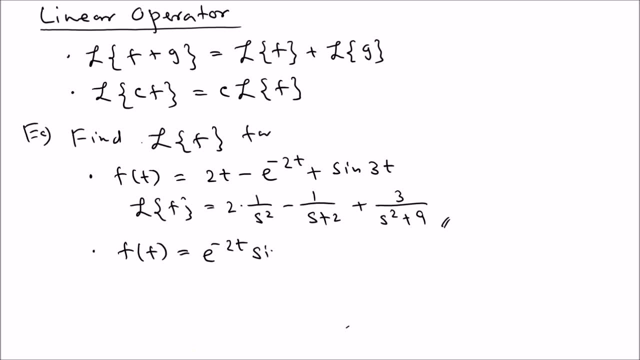 e to the negative 2 t sine 3 t. so if you're something like that, that's the eat function. so according to that, uh, your answer is what we can do. we first find the laplace transform of the major function, the sine 3t. so we can do that first. 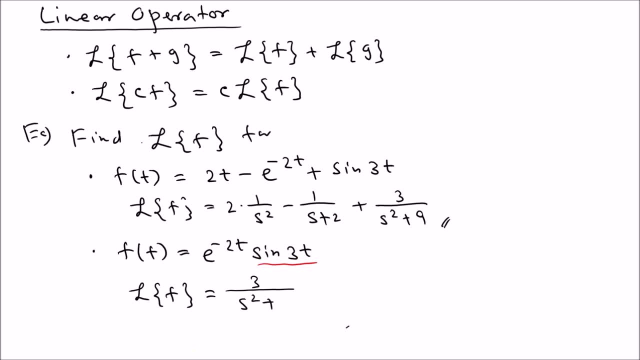 it is 3 over s, squared plus nine. and then what we're going to do? we're going to shift s because we have uh, uh, that's the number, so that means plus 2. okay, so when you have a, remember the format. there's a negative sign here, but we're going to go with the plus sign. 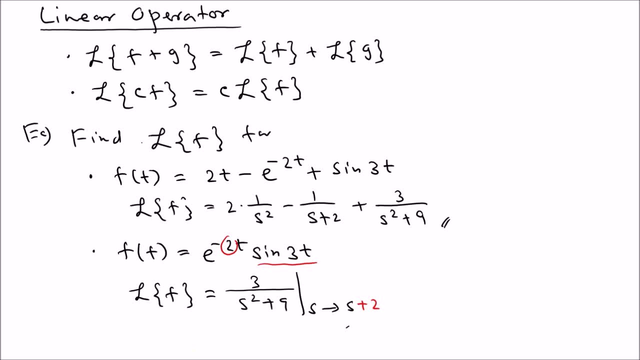 so that means- uh, it's going to be. you simply replace s with s plus 2. so if you do that, you end up getting 3 over s plus 2. you place s with s plus 2, squared plus 9, so you replace s with s. 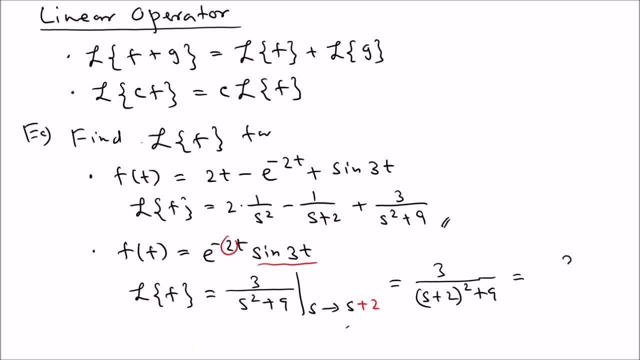 squared plus 9. if you want, you can simplify the bottom. that's not a must. if you do that, if you expand up, add 1, add 9, you get s squared plus 4s, uh plus 13.. so that's how to get uh. so that's laplace transform of that. 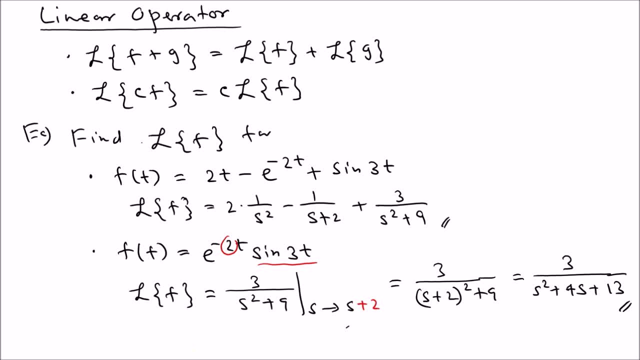 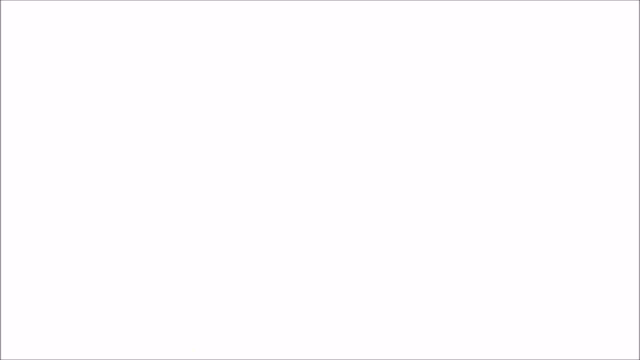 okay, so it's not that difficult, but this is how it works. okay, now let's talk about the inverse laplace transform. so we're going to define the inverse laplace transform kind of in a like a interesting way. uh, so, inverse laplace transform. uh, so how we define inverse laplace transform? uh, we're gonna say: 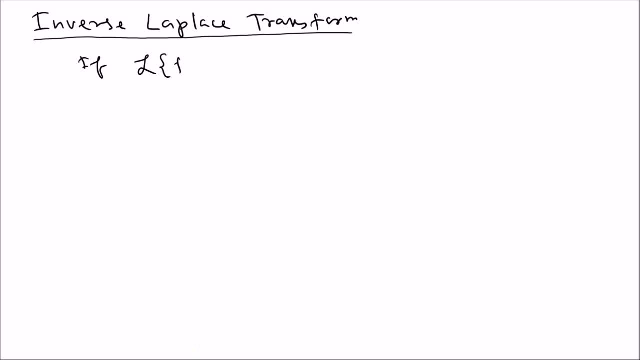 if the laplace transform of a function is f, s, if, and only if, let's go backward, uh, and for example, i'm sorry for saying was it s, let me write s. all the way is good. uh, yeah, if you turn theINV of s to fs. 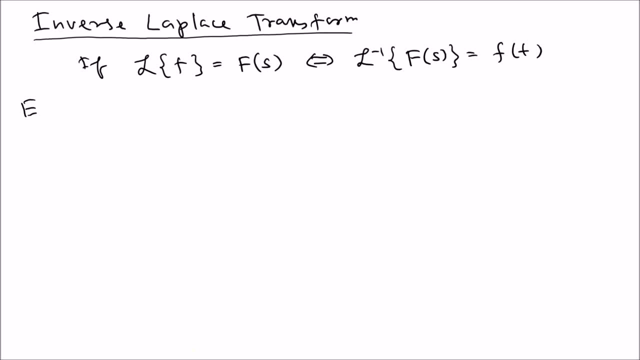 is the ft, so that's the kind of idea. so you can transform backwards. so i mean, that's how we define the inverse transform. that means if you know the laplace transform, you can simply find the inverse la place transform. ah, let's start with this one. ah, so the first one. 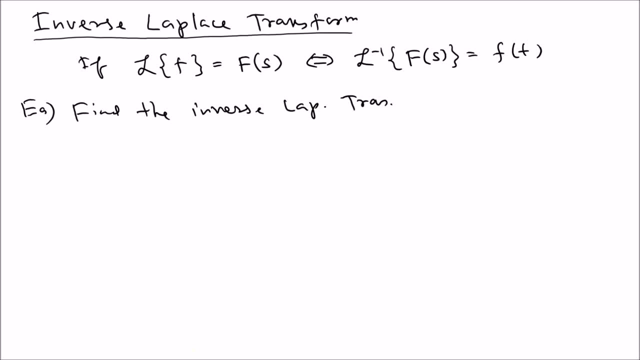 inverse laplace transform of 3 over s plus 2 minus 1 over s minus 1, squared. how we do this, it's all defected, uh, otherwise we have to find partial fractions. but it's already given. so b is the linearity, so it is. you're going to take 3 out, so it's l inverse. 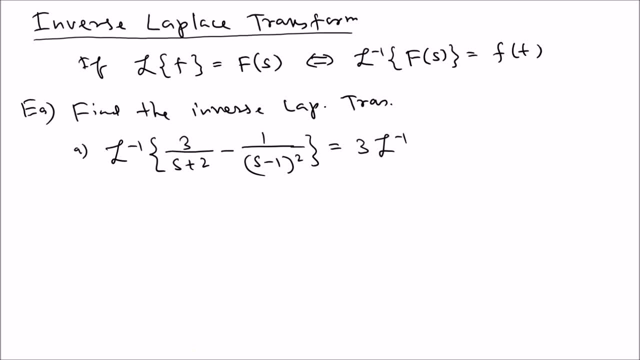 1 over s plus 2, and here you can take the minus sign out. it is l inverse: 1 over s minus 1 square. okay, now let's see how we can do it. so the first one is easy: it is 1 over s plus a we. that's one of the formula in the table. 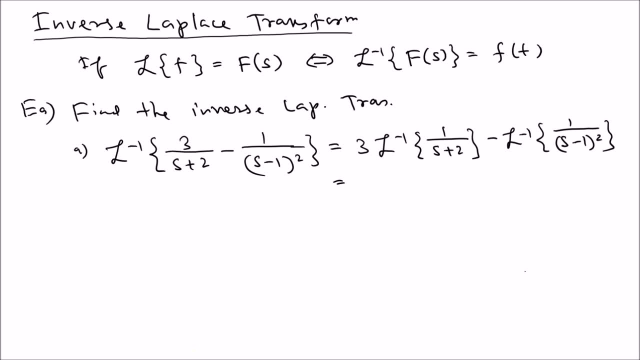 so that means this is simply 3 over s plus a. so that means this is simply 3 over s plus a. 3 e to the minus 2 t opposite sign. okay, let's say it's 1 over s plus a minus. how about the second one when you want to do the second one? 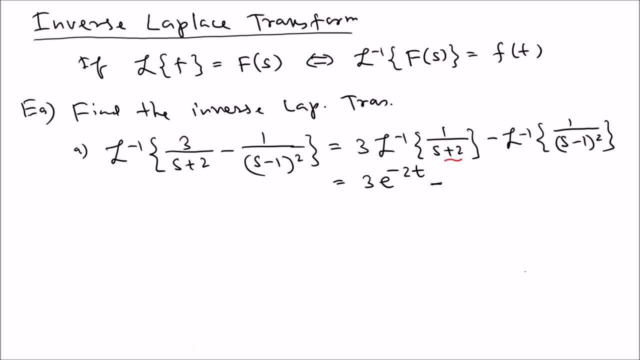 you first need to figure out. it's a shifting version. that's a shifted version. you want to figure out what is the base function here? the base function is 1 over s squared. if the base function 1 over s squared, we know that 1 over square is corresponding to: 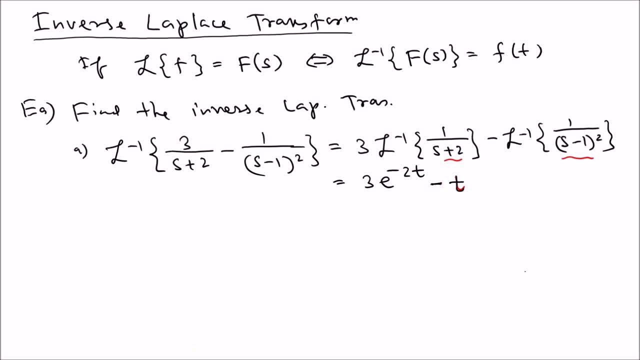 t. so we write t because that's 1 over square, because that's a base function. here the base function is 1 over s square, you see, and then, and then you shift it, then the shifting part comes, that means the e term comes. so in this case the 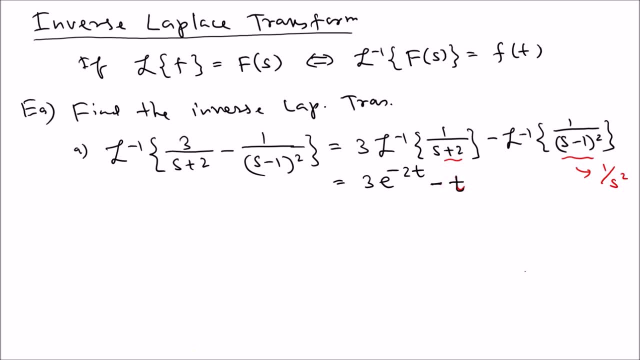 shifting part e, but it is minus 1, so that means it is plus 1, so it's a plus 1 t. so that's what you get, okay, so it's simple. so you need to figure out what is the base function. the base function: 1 over square. 1 over square is corresponding to t. 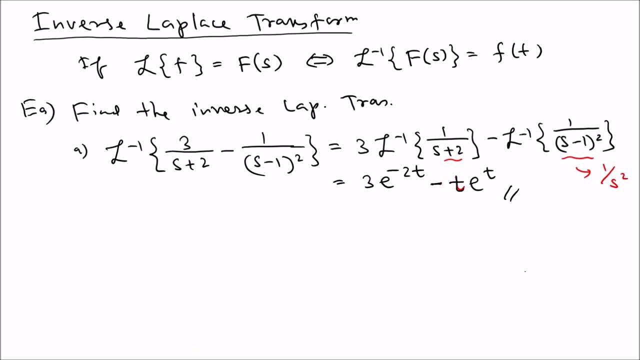 and then you do the shifting. so that's what you get. that means you multiply by uh e to the t, so that's the eat function example. okay, so what i use here is: i'm gonna write it here. so what i use here is: we know that if you are e to the minus a, 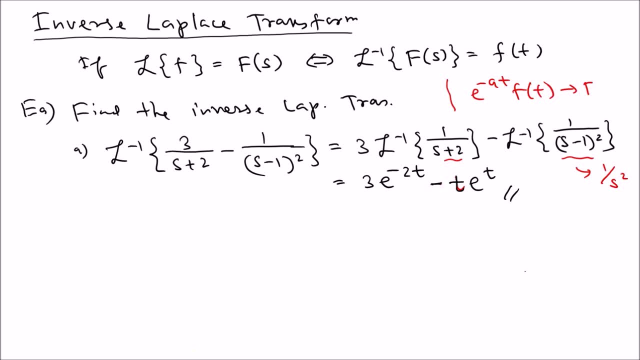 t, f, t, it is simply f? s plus a, so that's the one we use. good um. so let's do one more example. uh, how about this one? uh, let's say: uh, l inverse 3 plus 2 s over s squared plus 4.. 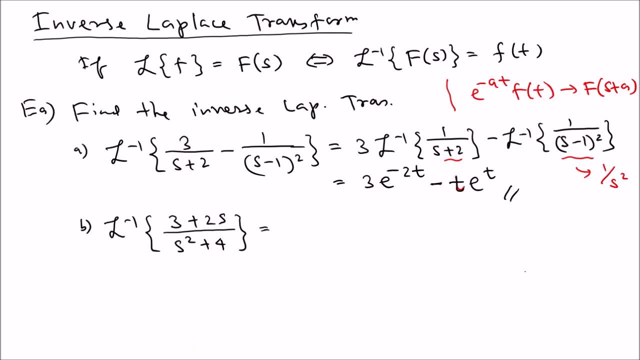 so if you get something like that, uh, what we can do- ah, it's not directly something that we know. so, what we can do, we can split this. we can split this into two fractions. so what are the two fractions you can see that i'm going to take? 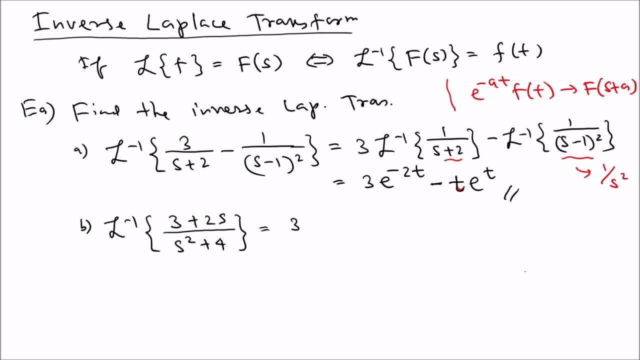 three out l inverse. first one: i'm going to write s squared. so what is missing here? we know that this is very close to the sign, but if you sign the square root of 4 is missing, that means 2 is missing. so what we do? we multiply and divide by 2. 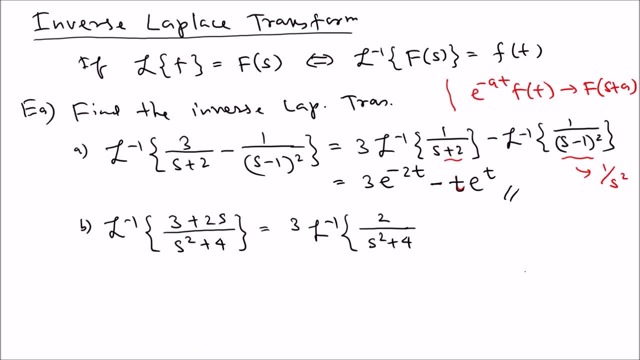 so that's what we do. we're going to multiply and divide. so we're going to multiply here by 2 and then divide here by 2.. so that's the first one. we do plus because the linear. so things are easy: you take the 2 out. 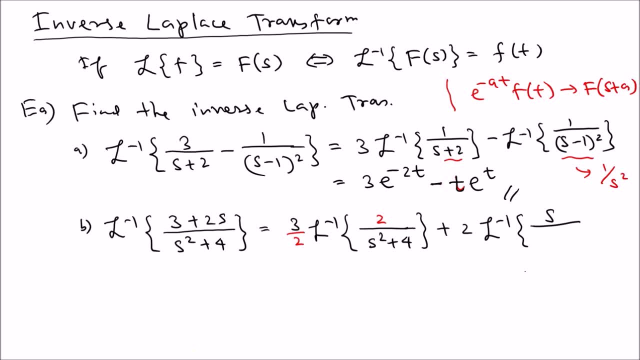 so we write l inverse s over s squared plus 4.. so now we know all the both. so the first one is simply uh, 3 half sine 2 t. second one is 2 cosine 2 t. so it's very simple. okay so, but we have to uh. 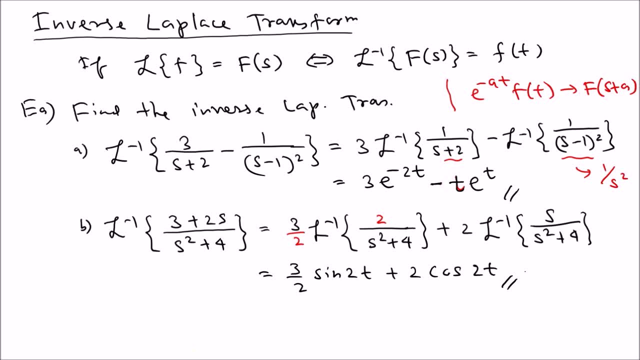 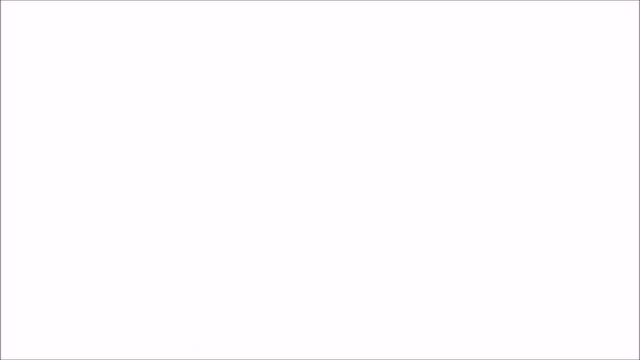 break it into two split and then you can see it's right there. it's simply coming from the table. the next major method is the- uh, partial fraction method. so let's discuss that now. so the partial fractions method, partial fractions method. so if you don't know much about this, you can just write it down and then you can. 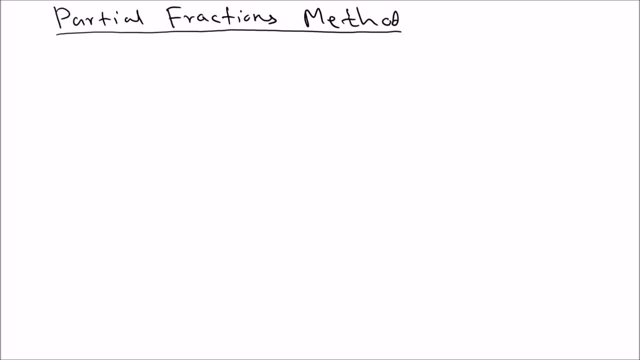 a little bit more detailed about that. there's a video, uh, that i did for my calc 2 class. there, like i explained like a, like a vast majority of questions in different types, so you can look at that and there are like shortcuts, a lot of shortcuts. 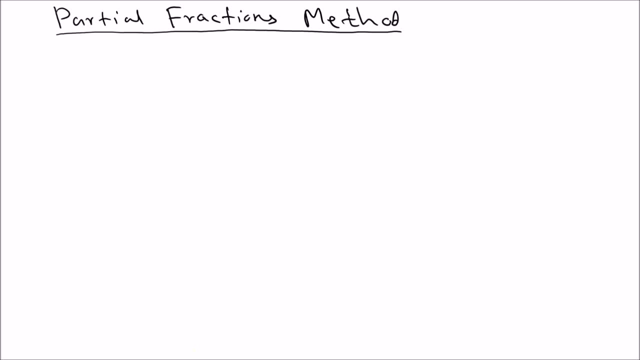 are to find the fact, the coefficients, and i increasingly discuss that there, so maybe you can look at that if you have enough time, okay, uh, yeah, let's say when i posted earlier also. so let's do a problem like this. so let's say: um find the independent. n阳我们 2019. 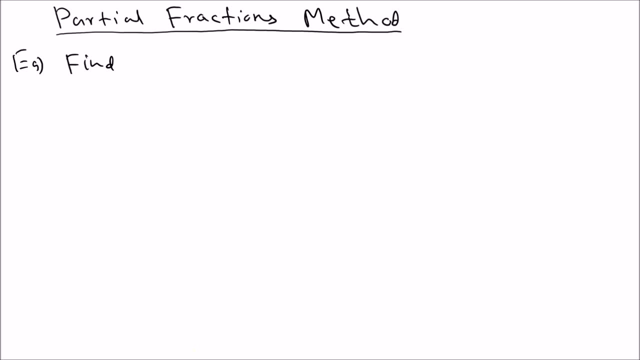 so find the inverse laplace transform, inverse laplace transform. so like uh, let's say, you get like a, something like this: l inverse, l inverse, uh, 2 s plus 3 over s plus uh, i don't know. yeah, actually, i, i'm going to, let's, let's slightly change the problem to this one. 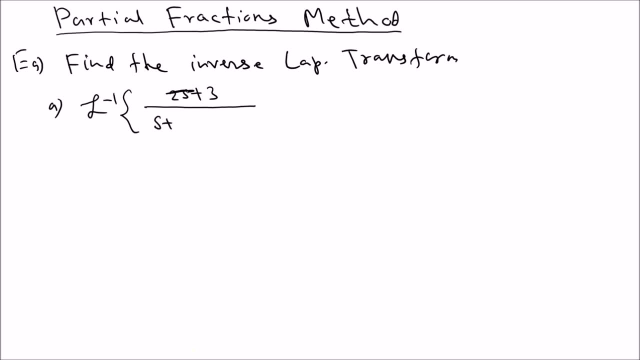 this can be like a little bit difficult. that's we can do as a second example. let's do this one first: uh s plus 2 over. uh, let's say s plus 3 um and s minus 1, something like that. let's do this one first. 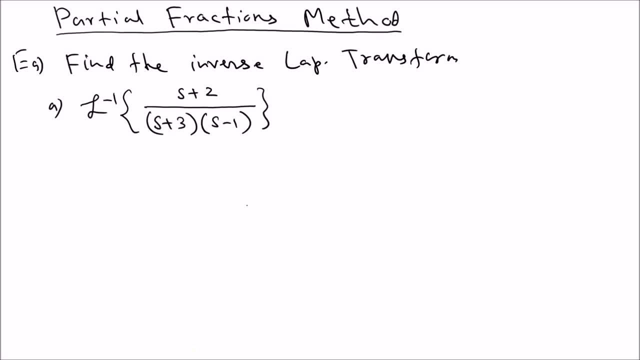 but this is easy to do, like if you have linear factors. those are very easy to do. so let's look at how it can work. um, so we can write the partial fraction decomposition, so it's: plus 2 over s, plus 3, s minus 1 is identical to. we can write the linear factor, so it's. 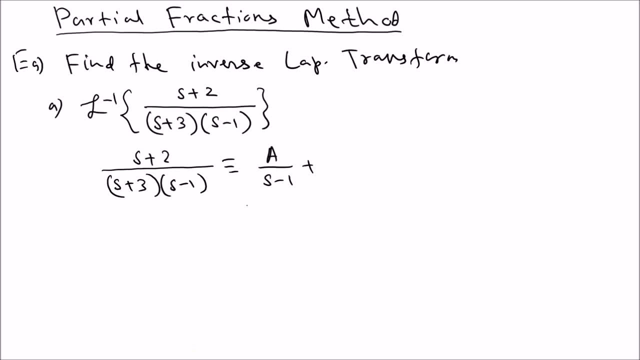 a over s minus 1. there's no order, just pick one s plus 3, and then what we can do, we're going to multiply the common denominator, so we can write this one as s plus 2, identical to a times the other one plus b times the other one. you see, you get the other denominator. now what? 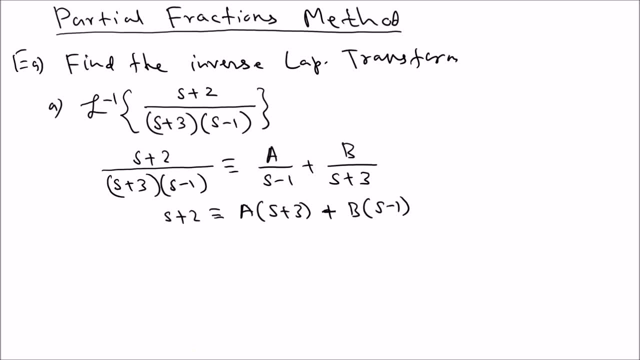 you can do, just substitute. okay, that's the easiest way to do this, so you can substitute. so you're going to substitute. let's say you want to find a, so you try to make this term zero. so that means you plug in s equal one. so you plug s equal one. if you do that, you 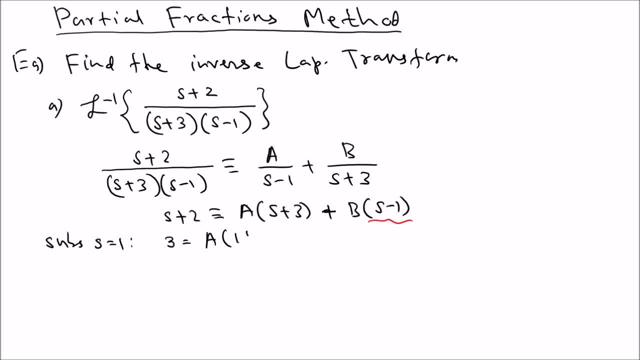 get three equal a one plus four. this is that, a equal three. fourth, uh, this is s plus three, so, uh, three-fourth, and then, um again, uh, we're gonna substitute uh s equal negative three to find the other one, so, negative three you're gonna get. 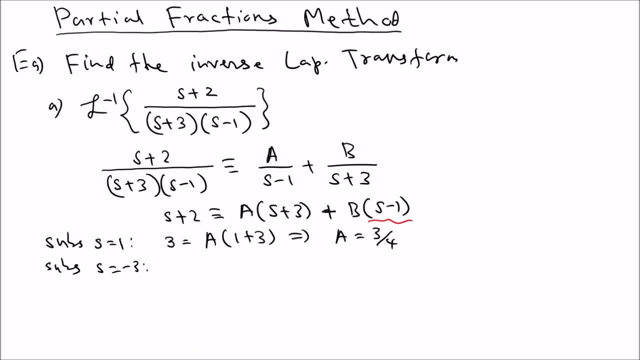 negative one on this side, so you're gonna get negative one on this side, so you're gonna get negative one on this side. equals: uh, the first term is zero now, and then from the other term b, you're gonna get a negative, uh, four, because negative three minus a negative. 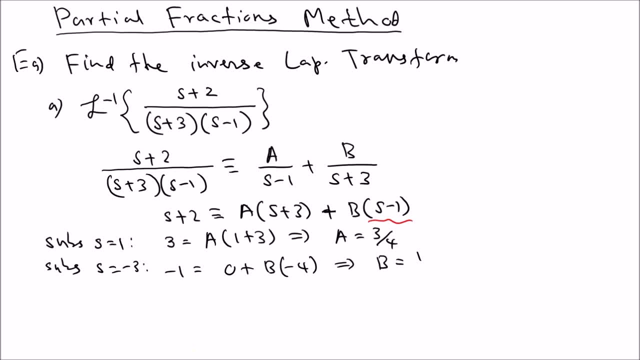 four. so this says that b equal uh one fourth. so that's it. so you can find the two fractions uh, two, uh coefficients. so that means, if you go back and substitute a equal three, fourth uh s minus one, b is one fourth uh three uh s plus three. good. 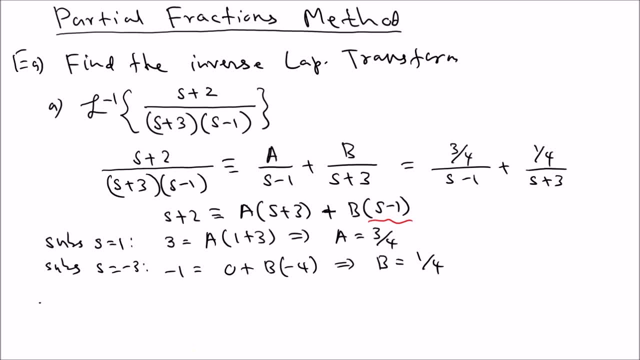 so we have those two now. what we can do: we can find the inverse now, so we can start with inverse which is uh over s plus two, s plus three, s minus one, which is equal by the linearity. what we can do: we can write this as a: 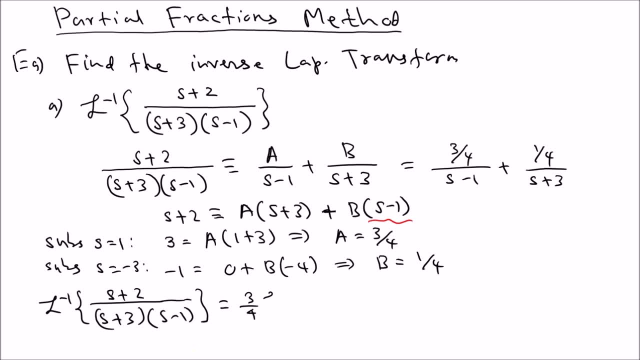 two separate one, so it's three. fourth: uh l inverse one over s minus one plus plus one. the other one is one. fourth, l inverse uh one over s plus three. so now what's going to happen? uh s minus one. we know the inverse of s minus one, that is e to the t, so it is. 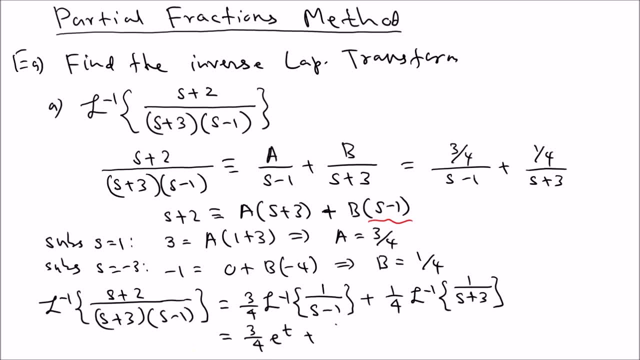 three fourth e to the t plus one fourth uh e to the minus three t. so that's it. so you can see it's very easy to find. only thing that we need is partial fraction decomposition. so if you know how to do that, everything looks great. okay, let's do one. 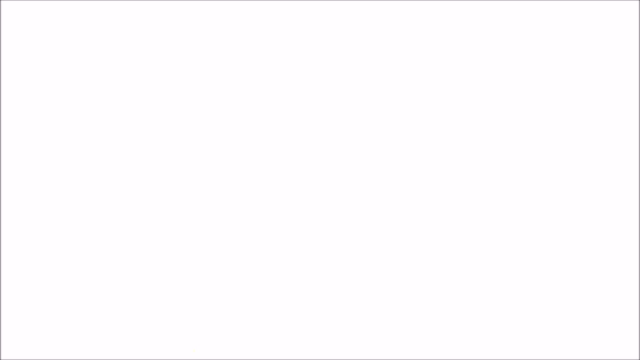 more little difficult example. uh, so b, let's do the other one that we suppose we're trying to do. so let's say we have 2 s plus 3 over s plus one squared uh s squared plus 4.. so we know how to write the partial fraction decomposition for that. 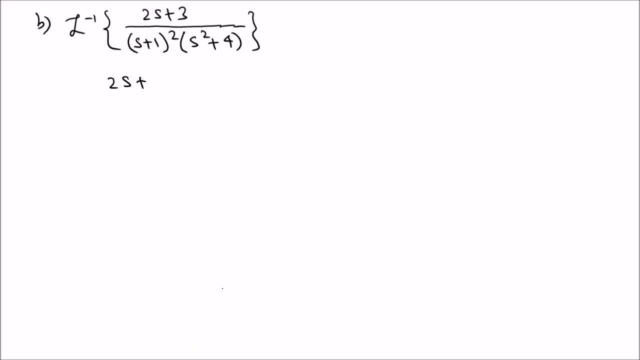 so this is: we can start with 2 s plus 3 over s plus 1 squared, and then s squared plus 4. this is identical to. so when you have a repeated factor, linear factor- what we're going to do? we're going to start with the. 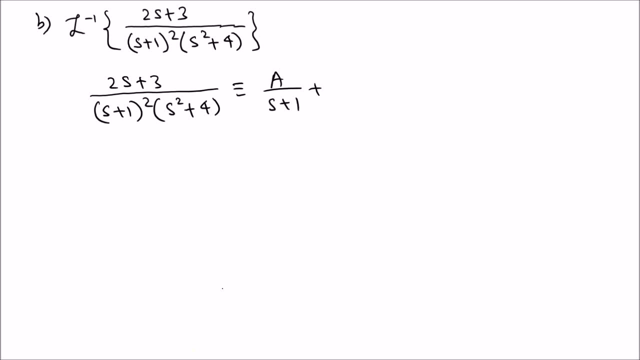 smallest one and then the next largest. so that's how we do it. and then plus this is s squared plus 4, and we know that b has the exact same format as a when they repeat, but here that's not the case. this is the irreducible factor, so we 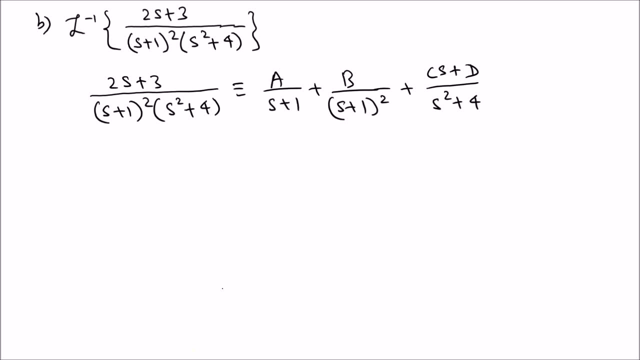 have right: c s plus d. so that's how we write it. now what we can do is the same thing, so we write 2 s plus 3, 3, uh, identical to write the missing term here. the missing term of uh. 1 of s plus 1 is missing. s squared plus 4 is missing here. 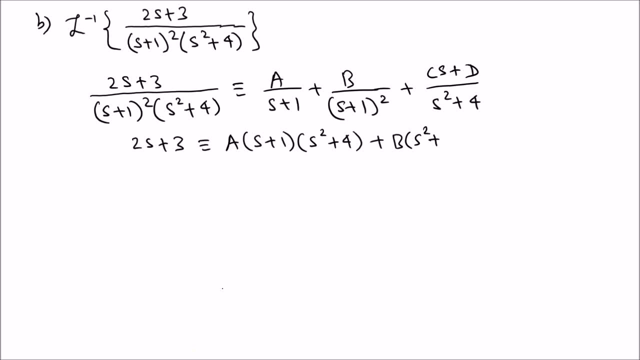 b. only s squared plus 4 is missing here. c s plus d, you can see s plus 1 squared is missing. uh, now, what we're going to do? uh, we're gonna always. we do the substitution first and then the coefficient. that's the easy way to do it. so we're. 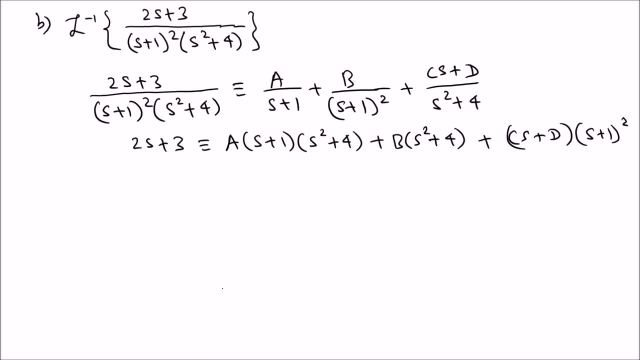 going to go with the substitution. so we can see that this term is common. so we're going to substitute s equal negative 1 to find b. so we substitute uh s equal negative 1. if you do that you get 1 equal 0 plus b. if you plug in negative 1, squared that means 1 plus. 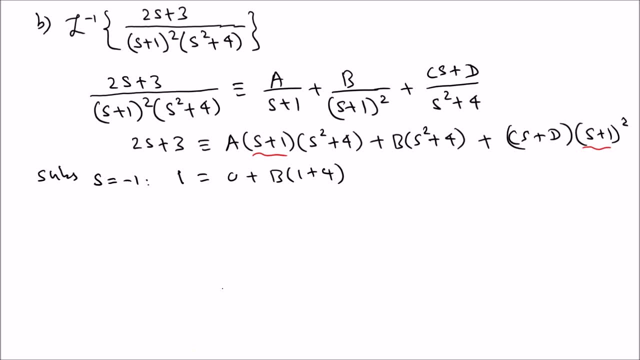 4. so you're gonna get uh. so you can see you're gonna get b equal. and then also, this term is zero. so this is that b equal one-fifth. so we already find the b value. now what you can do, you can see that you can plug in anything else and directly find. 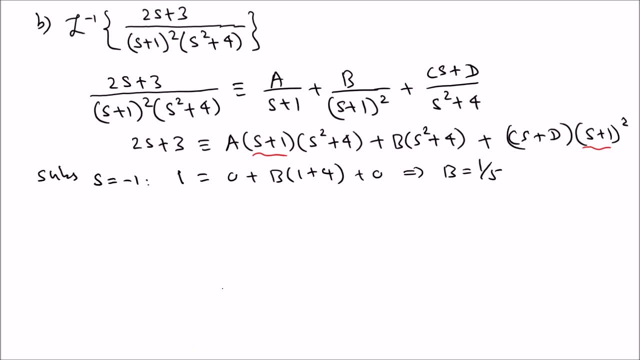 either any other values, any other coefficients. so what we're going to do, we're going to go with the coefficients. so we always start with the largest coefficient that we discussed several times there. what's the largest term that you're going to go with? s you can see s cube. 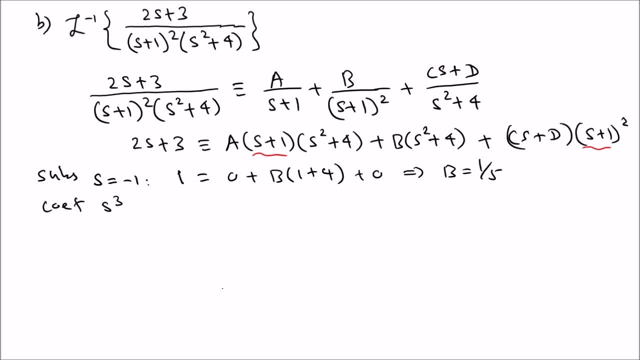 is the largest, so we're going to go with that. so there's no s cube term here. uh, so that means it is zero, uh, and then you can see you get a s cube term and you multiply these, so that means the coefficient is simply a. the same argument. 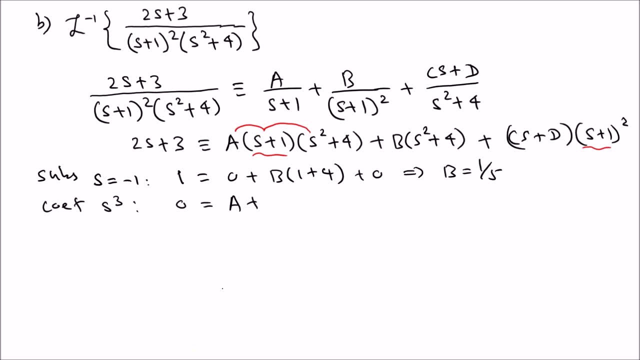 uh, from the next one you're gonna, you are not gonna get one, but from the last one you will again get this s squared s. so that means there's a. uh, another s cube term, that means c. so those are the coefficients. that means a plus c is 0.. that means, if you know one, 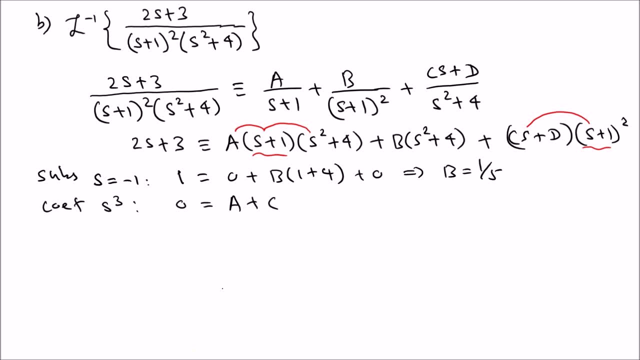 you can find the other one. and now, what we can do? uh, we can write a equation for s squared. so what we need is just three more equations, because we have three unknown. we need three more equations. uh, i'm gonna go with uh, because you know that all of them. 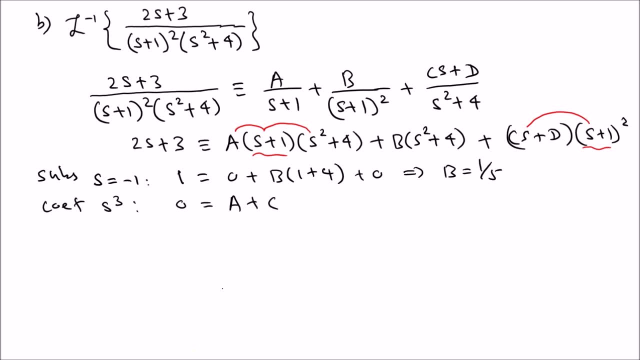 related with uh, a. so, because of that, because a has, like uh is constant, has a s has a square, has a s cube has a. so i'm going to go with not s squared, i'm going to go with s. okay, coefficient of s. if you go equation s, it is 2 on this side. 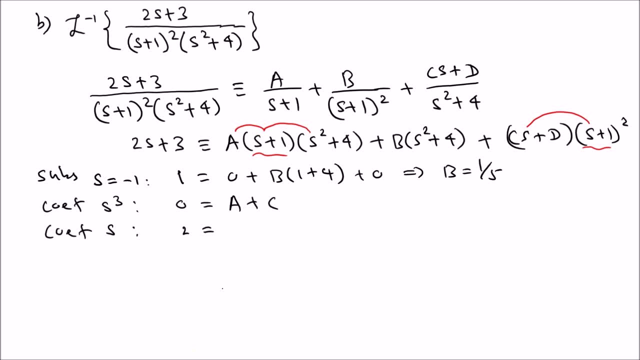 uh on the other side. uh, you're gonna get the from the first term- the coefficient of s is 4a- from the first one and then from the second one there's no uh term. so this is easy from the last one. let's expand uh, this one. so if you, 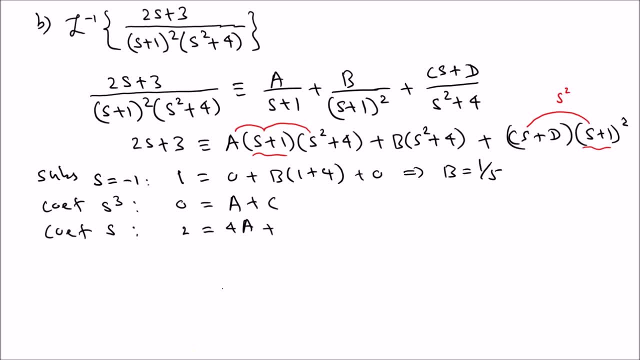 expand s plus 1. squared, it is s squared plus 2, s plus 1.. so it's going to help you to figure out what is the coefficient. so what is the coefficient of s to get s? uh, one way to go to s is uh. you can see, you can multiply one with c, s. so it's a. c is a coefficient. 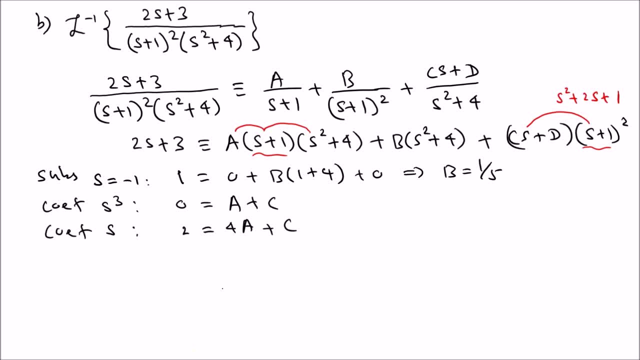 and to get another s, you can multiply the one with um with c, yes, or 1.. so you get two coefficient. yeah, of that way, um you can use. ah, the coefficient of s is 1 and you get s to get 2. 2s. so that means 2d is a coefficient. now what we can do, we know that. a plus. 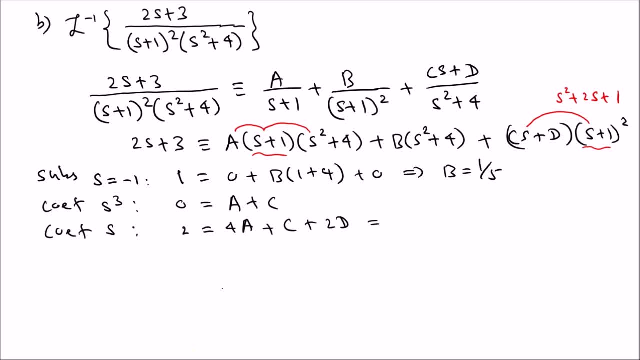 c is 0, so that means you can remove 1 of a plus c from this. so if you remove 1 of a plus c, you only have 3 a plus 2 d, so that's easier compared to the original one. and then let's go with the constant term. so if you get the constant term, 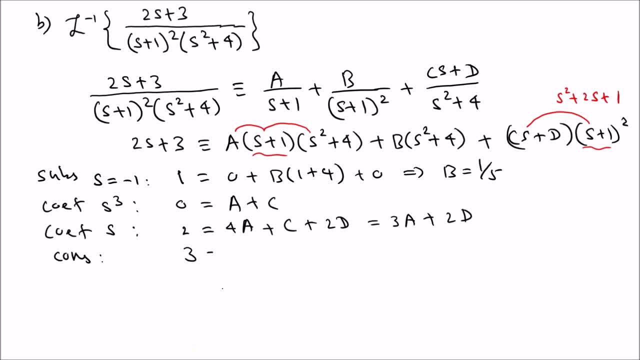 you get 3 on this side. what is the constant here? 4a is a constant, 4b is a constant, and from the last one you can say d is a constant, uh, so now what we can do is um, so we need, uh, two equations with the same variable. 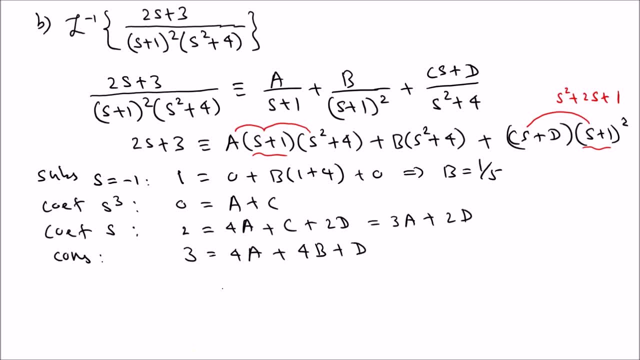 so to get that, what we can do is you can substitute for b in the last one. so if you substitute b in the last one, uh, what are you gonna get? uh, so you can see. uh, so you can see, uh. uh, if you substitute a, b for the last one, uh, you can see it, the b is one. fifth, 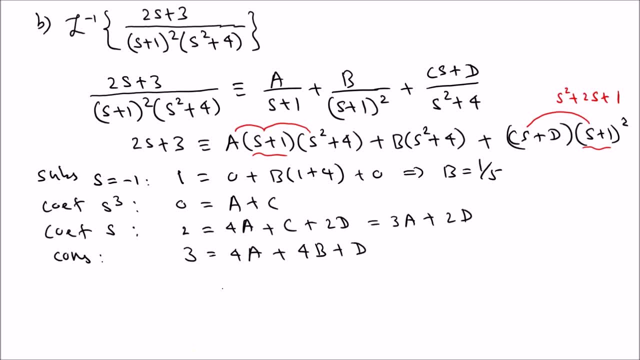 so it is a 4a. so this is that 4a. this is that 4a plus d. 4a plus d- uh equal 3 minus 4b. but what is 4b, which is uh 3 minus 4b. 4, 5th, that means 15 over 11. so that means you're going to get equation. 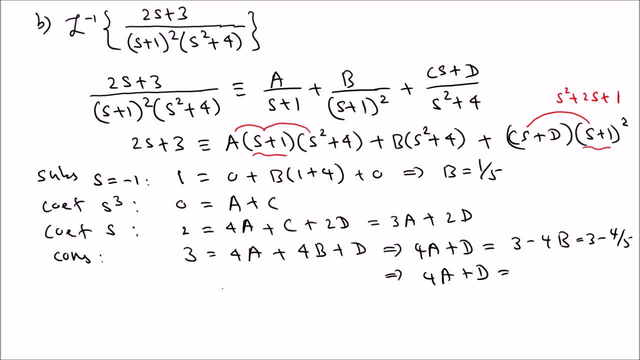 4a plus d equal 11 over 5.. now what we can do is we can solve the last two equations, 4a plus 2d and 4a plus d? um, and if you solve those last two equations and you can see that you can get a easily. 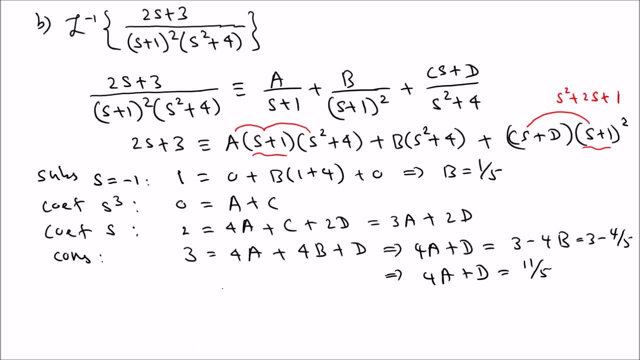 because you can multiply the second one by two and then subtract uh the top one uh. so if you uh do that, so okay again, i just write the two equations here. so we have 2 equal 4a plus 2d, and here we have 11. 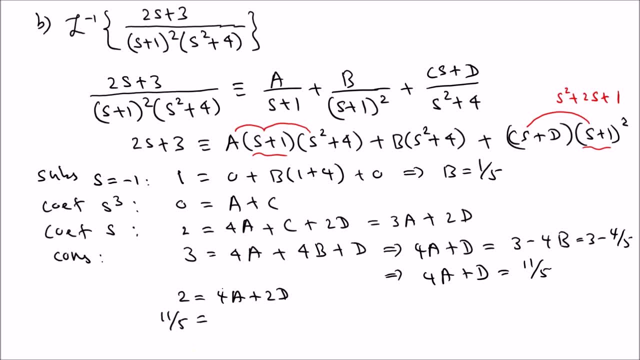 5th. 5th equals three, not four. eight, three, eight, three plus d. so what i'm gonna do? uh, we can solve these two. i'm gonna multiply the uh, second one, uh by two, and then you're gonna subtract the first one. so once you do that, uh, you're gonna get. 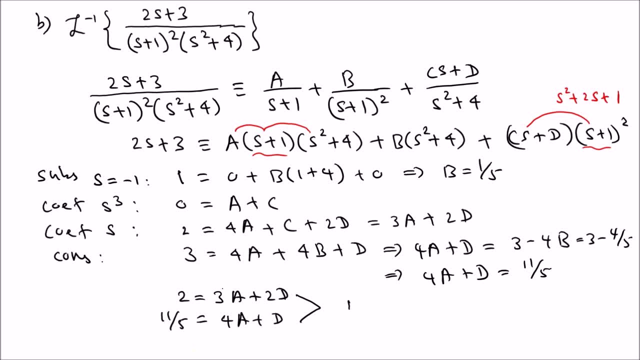 uh 12 over fifth, equal is 8 a minus 3, 5 a. so this is going to give you the a, so a equal uh 22. uh a equal. actually, what do you get? 12, 12 over 25, so a equal uh 12. 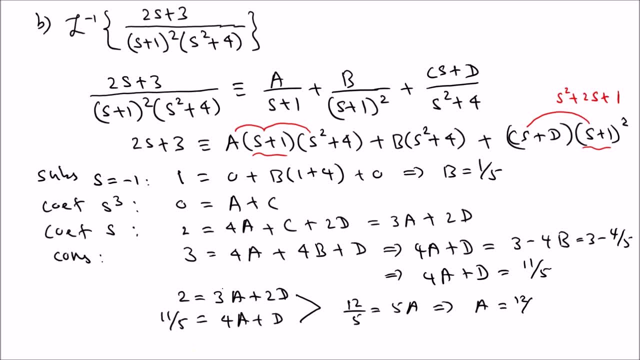 over 25. that's what you get for a. uh, and then uh, we know c. because of that, then c is simply minus a. so this is negative 12 over 25. so, and then we can find d from one of those equations. um, so we can find d from one of those equations. 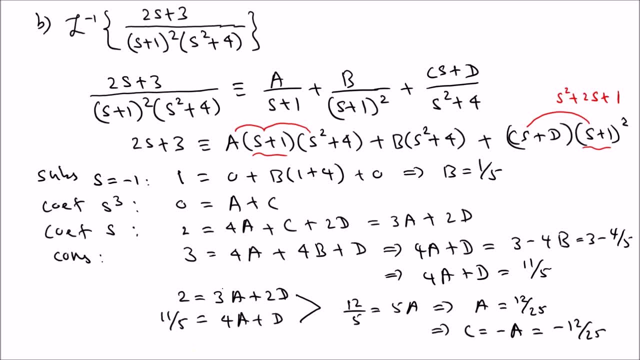 um, and then, uh, we can find d, so i'm going to write the value so you can verify. so this implies that d equal. just plug into one of those equations: um, so it is d equal 11 15 over 4 a. so 11 15 minus 4 a, so this can give you the d value. 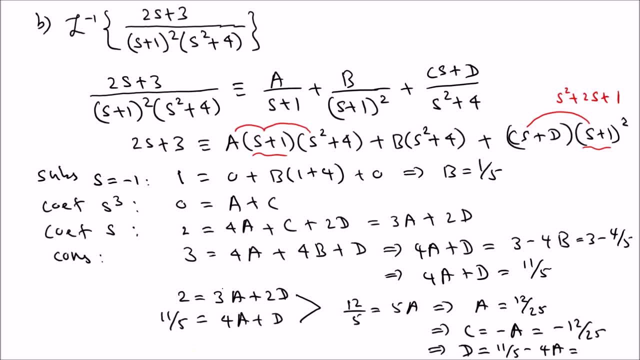 uh, which is 725. okay, so we find a b, c, d over 4 a, so this is a b, c, d over 4.. okay, that's the only part like taking time, uh, otherwise just the method is easy. so after we know all four, so then we can write. 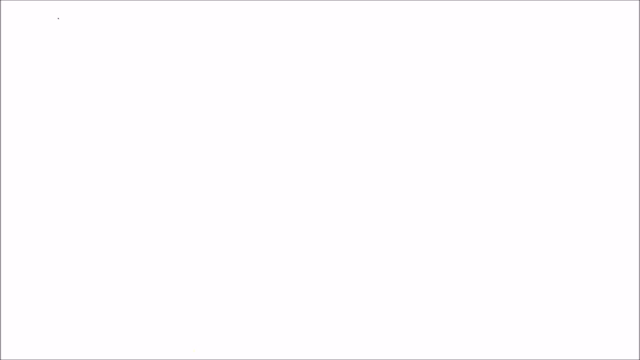 um this expression. so we had- i'm going to rewrite this- one, 2 s plus 3 over s plus 1, squared s, squared plus four s squared plus four, uh, equal, uh. we had 22 over, uh, it's just 22, or uh, a equal, actually 12 over 25.. so it is 12 over 25. 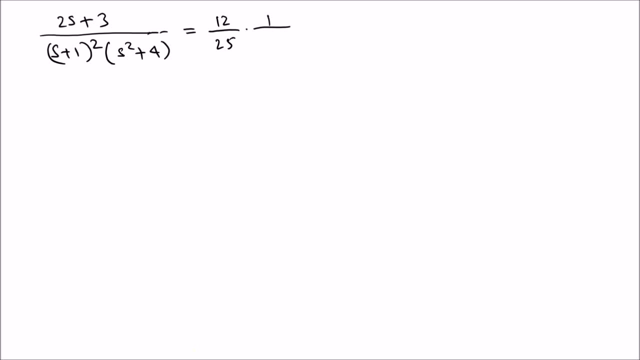 1 over s plus 1, uh, and then we have 12 over 25. then we had b is 1: 5, 1 over s plus 1 squared, and then we had 11.. negative 2: 12 over 25 c, that's a c value. 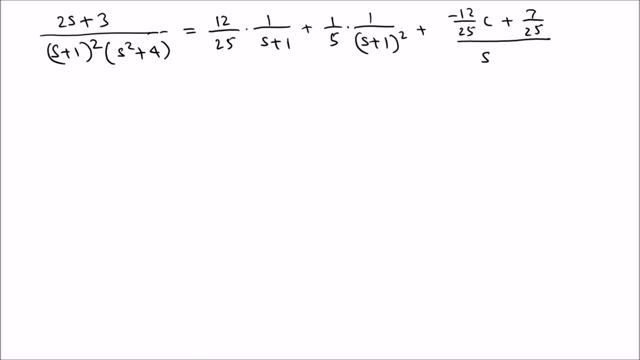 the d was 7 over 25 over s squared plus 4, but you can split these two to get, uh, not the c, yes, to get a sine and cosine term. okay, now we so the inverse of this: 2 s plus 3 over s plus 1, squared s squared plus four. 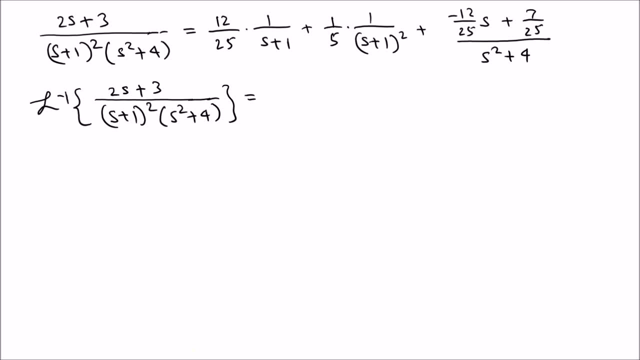 equal. so, um, so we're going to find the inverse of each term. so that means this can give you: uh, 12 over 25, ah, l inverse. i'm just writing this one. this is not really necessary, but for completeness i'm writing. and then one, fifth, l inverse: 1 over s plus 1, whole thing squared. 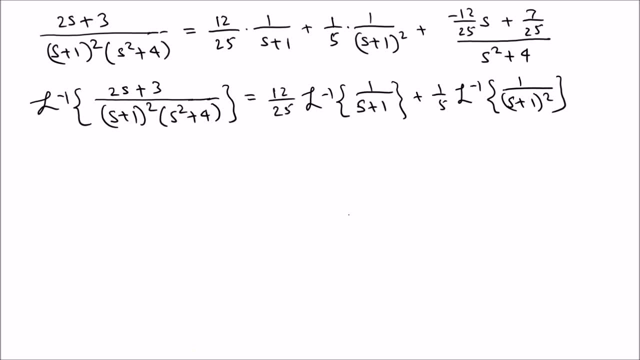 the next one. what time i'm going to split? that's into 2, so we have negative 12 over 25, l inverse, the first one, which is s or s squared plus 4, which is a cosine plus 7 over 25th t e to the negative t. that's the second one. how it coming from. 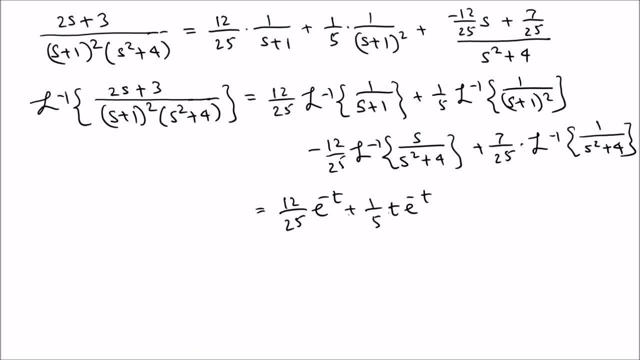 because s plus 1, that means 1 over square. s plus 1 square, that means 1 over square, is the term, that means t, and the shifting is e to the negative t, that's the shifting term. and then we have, uh, negative 12 over 25, the cosine. 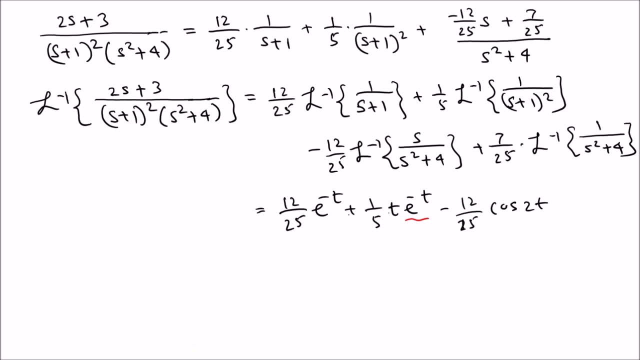 to t and then here what's going to happen is the sine uh 2 is missing. so you multiply and divide by that, so that means you're gonna get uh 7 over 50 sine 2 t. okay, but uh, it's like. this may be like little long. 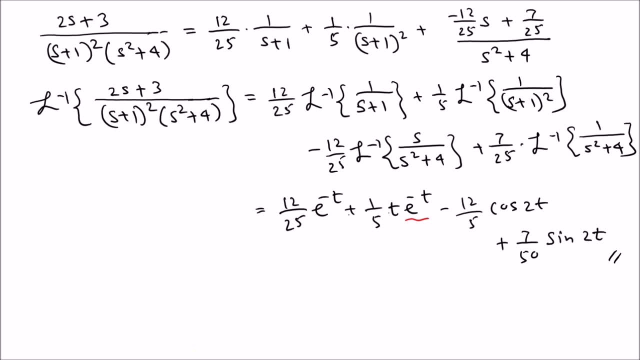 uh to an exam, so you will get something. uh, you can manage. um, this is like a little long compared to other problems. okay, good, but i want to show you, like how it works. it's not that difficult. only problem is the how to find the uh, the, the. 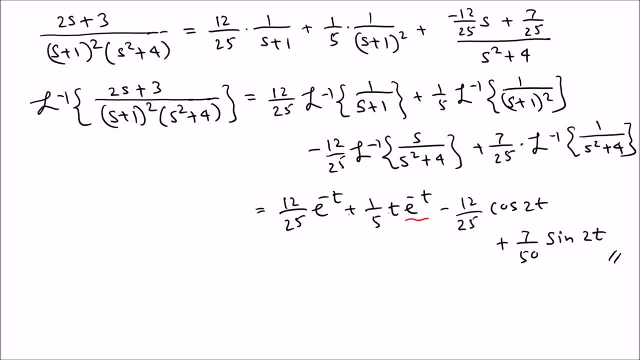 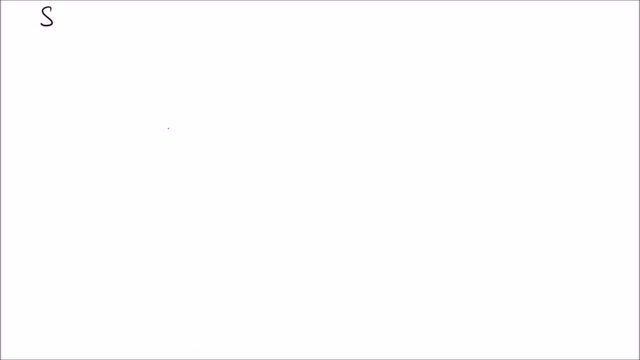 partial fraction decomposition. um, good, that's about that. and then, uh, let's talk about how to solve a differential equation using the laplace transform method. that's the most important one, so solving, solving differential equations using laplace transforms a method. solving differential equations using the laplace transforms method. 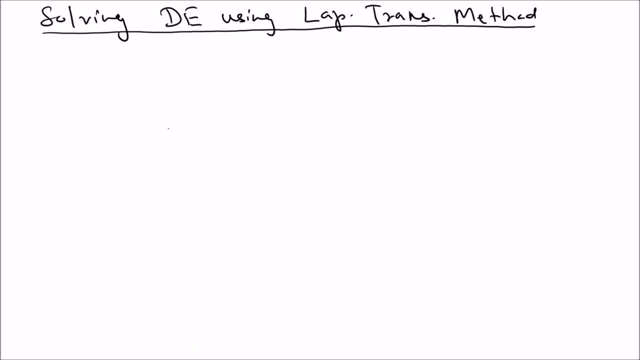 ah, so let's start with the laplace transform of derivatives. laplace transform of derivatives. we know these results. so the laplace transform of the first derivative is s and the derivative of the first derivative is s. if s minus f0, the laplace transform of the second derivative is: 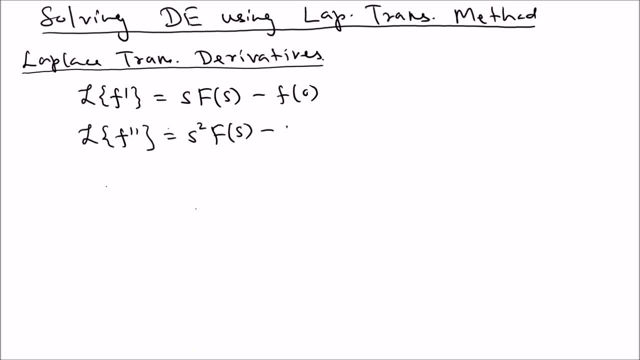 s squared f s minus s, f 0 minus f prime, you can see first term is positive. everything else is negative. there's something you can see if you write the third derivative, so you can just keep doing it. you write the third derivative, which is s cube, f s minus the power of s goes down. so 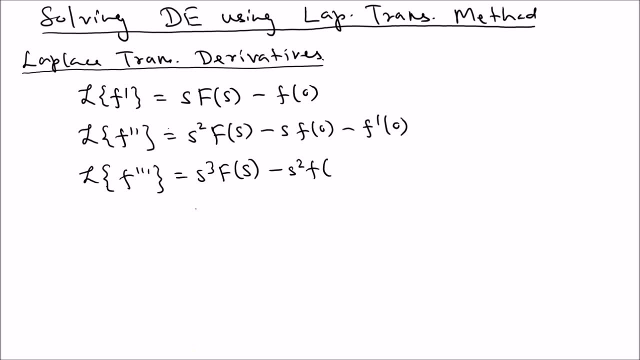 that means squared f: 0 and then s f prime zero minus s double prime zero. so you can see all the terms after the first terms are negative. so that's something you can remember. okay, these terms are negative, okay, and then. so you can continue like that. 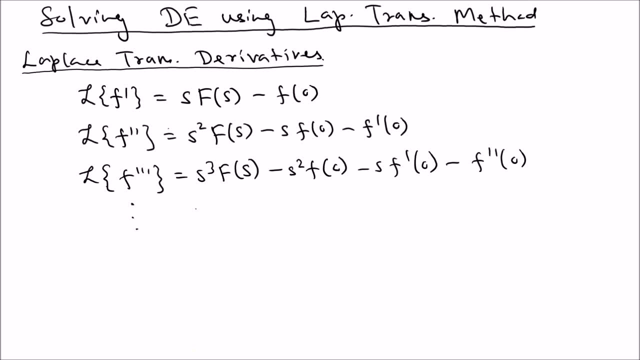 so you can have the general one. so it is a laplace transform of f to the nth. there is. so the nth derivative is s n f s minus s to the n minus 1 power. f 0 minus s to the n minus 2 power f prime. 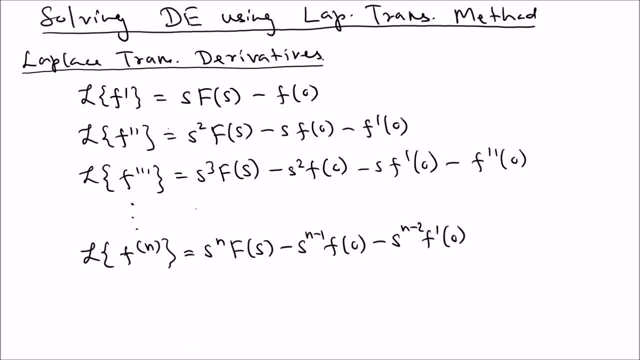 0, like that. and then you're going to be, uh, if f to the n minus first derivative zero. okay, so that's the idea. so you can see that, except the first term, everything else is negative. so there's a negative sign. okay, all negative, only the first one is positive. good, uh. so now let's see how we can use this. uh. 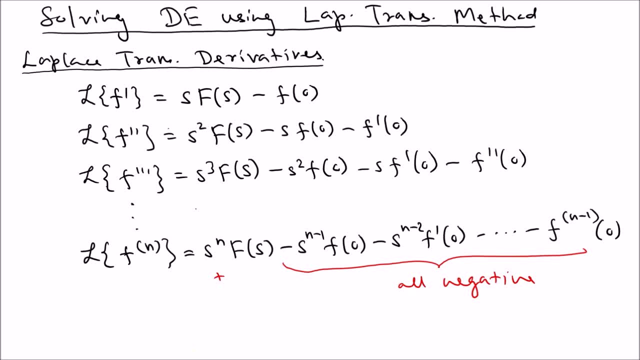 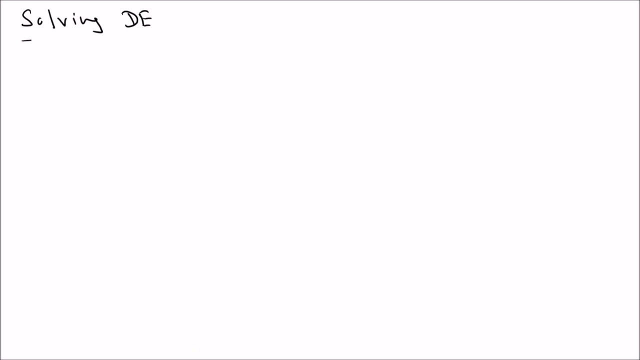 to solve a differential equation, so let's do also solving differential equations. so let's look at this example. so, uh, solve x double prime minus x prime minus 6 x equal. let's say 5 e to the negative, 2 t, along with x 0 equal 1 and x prime minus. 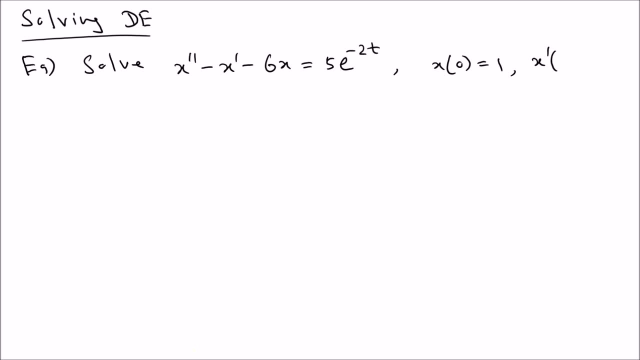 equal 1, and x prime 0 equal negative 2.. so if you get something like that, uh, so what we normally do is, uh, we can take the laplace transform of the equation- that's what we're trying to do- and then we can use the initial. 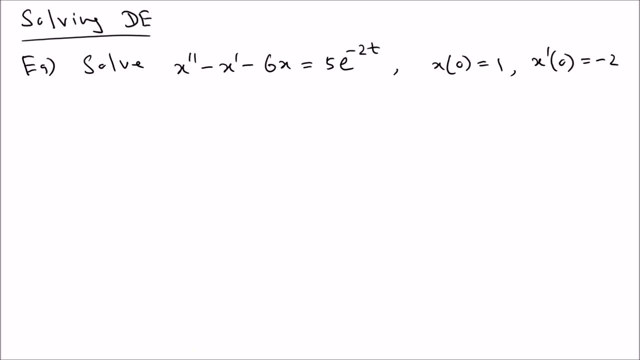 conditions given. um so so the answer. so let x s equals laplace transform of the expected solution. so let's say x s equals laplace transform of the expected solution. so let's say x s equals laplace transform of the expected solution. and then what we're going to do? our table laplace from the equation. so 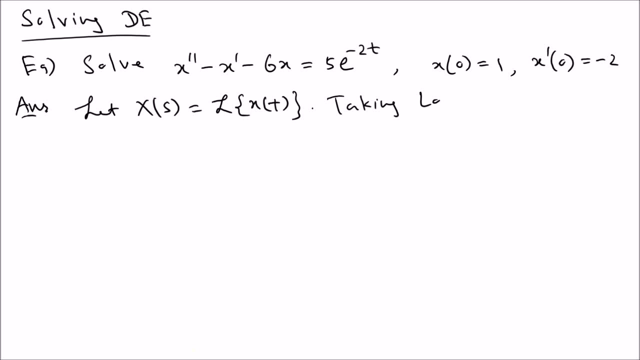 taking uh laplace transform of the equation, you're going to get s squared x s, uh minus s x 0. these are small, one minus x prime. that's the first term and then we're going to do the second. second term says minus. there's a minus sign, so let's plug in. 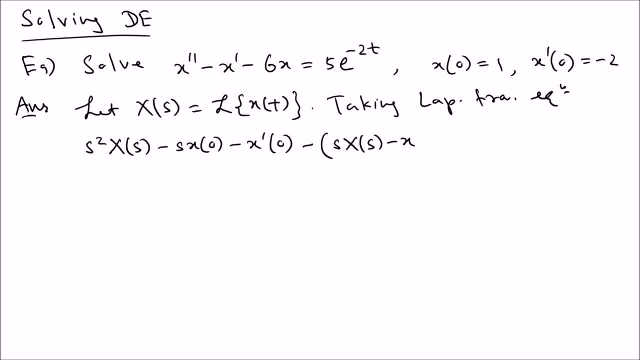 here. so s x, x minus x. it's a good idea to write this: one uh to avoid uh errors, and then minus uh, six xs equal la la la plus transform of that term is a five and it's each function, so it is s plus two. so, starting it now, what we're going to do? we're going to substitute uh the con uh. 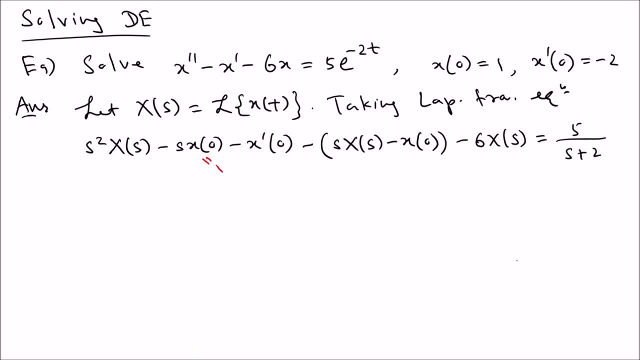 this equals to 1, this equals to 1 and this equals to a negative 2. so if you plug in that uh, then you can bring, so you have a negative s term. you can do the other side and we have negative 2 so it become positive 2. 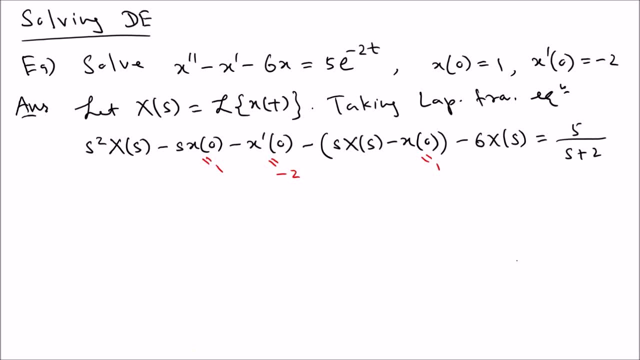 and positive 1, so it's 3. so we have negative s plus 3. so you can bring it to the other side. take the common uh. so we have s squared here and then we have minus s, and then we have we have negative 6. 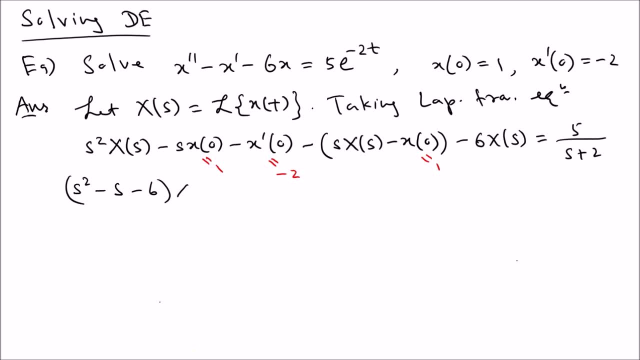 uh, xs, and you can see this is exactly equal to the characteristic equation, but with the s, not the lambda, but the s, so that that happen always. and then now we're going to bring the other terms to the side, so we have s minus 3 plus 5 over s plus 3, and then we have negative 6. 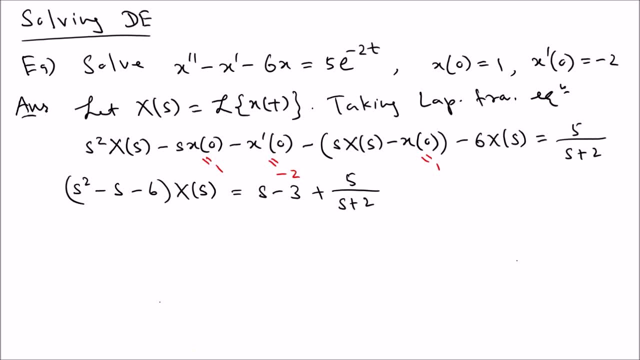 plus 2.. now, what we can do: we can divide by that and then you can see this. we can actually factor. what are the factors of this? uh, the factors are s minus 3 and s plus 2. those are the factors. so let's divide. so, when you divide, uh, 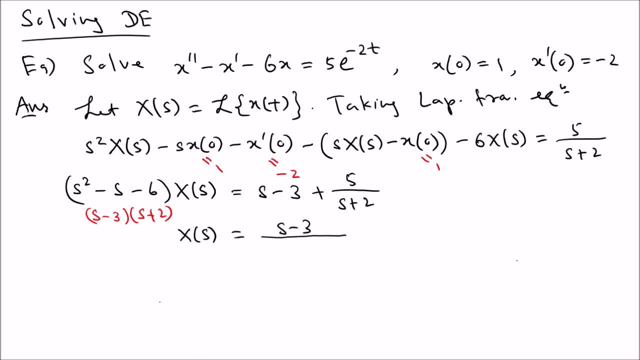 what's going to happen? we have s minus 3 here, and then we have s minus 3, uh s plus 2 plus 5 uh over. so we have uh s minus 3, we have s plus 2 and there's another s plus 2. 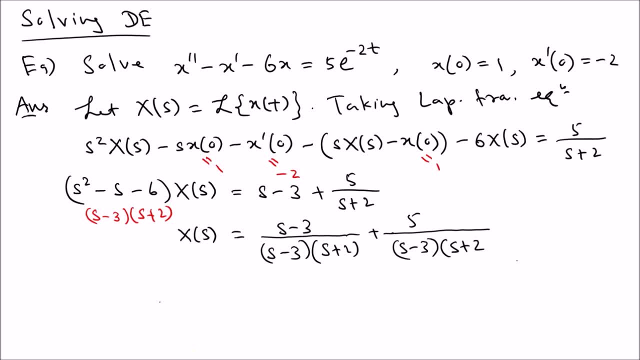 already over there. so that means this can be s plus 2. whole thing is squared. and the interesting thing is sometimes, uh see, this could cancel, so it simplifies well. so we only need to find one partial fraction, but otherwise what we're going to do, we're going to simplify this here, so we 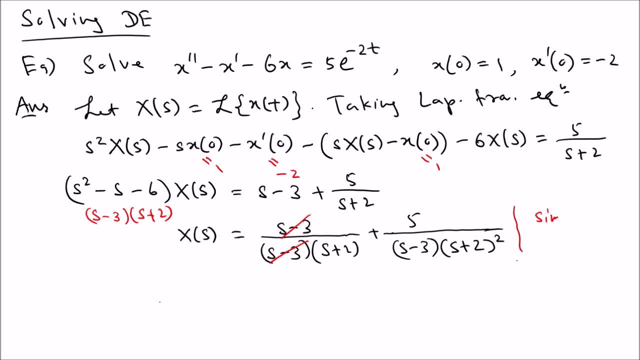 normally what we do here here is we simplify this. we simplify this before we find the partial fraction so that it's going to make the calculation much easier, because it's going to be an internal calculation. that calculation is going to, like you know, take care of most of the terms, so it's always a good data to simplify. 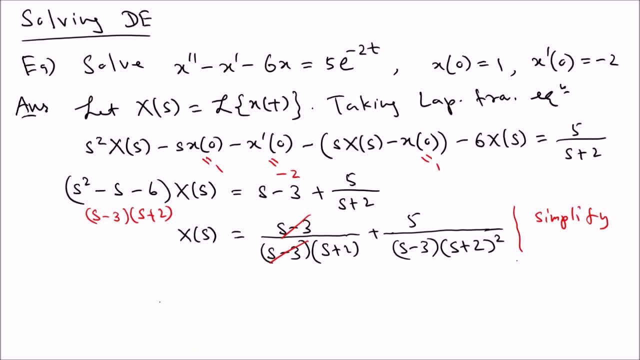 this first, but here you can see: um, we don't need that, because that term cancels, so we have like nice one already. uh, so it's, so we can separate those two terms, okay, so, uh, so what we have is 1 over s plus 2, so we leave that there, because we already know. 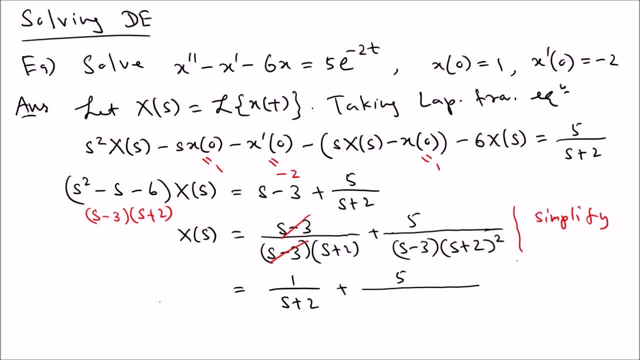 the inverse of that, and we only need to find the partial fraction of this term: s minus 3, s plus 2, whole thing squared, normally what we do. we're going to simplify this because it's going to make the calculation easy, so let's try to find. 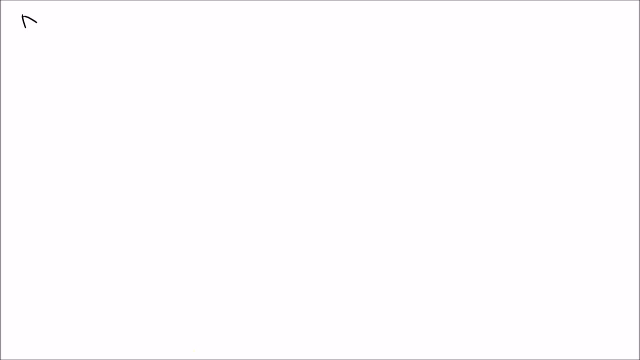 the partial fraction of that, uh. so now we're going to go with the partial fraction of that. so it is 5 over s minus 3, uh s plus 2, whole thing squared, which is equal to a over s minus 3 plus b over s plus 2. 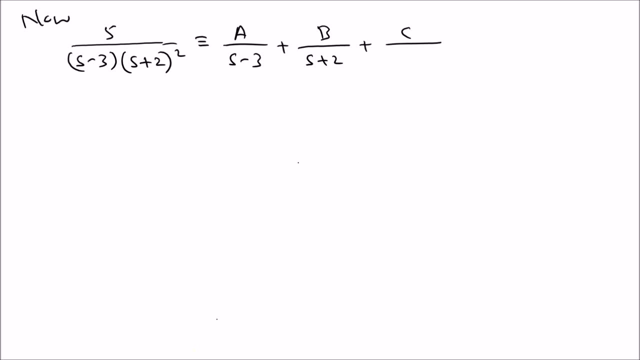 plus c over s plus 2 squared. uh, so we're gonna, uh so, and then after that we're going to get 5 equal a the missing part. so we're going to get 5 equal a the missing part, missing term. missing term is s plus 2, whole thing squared. in the next one: 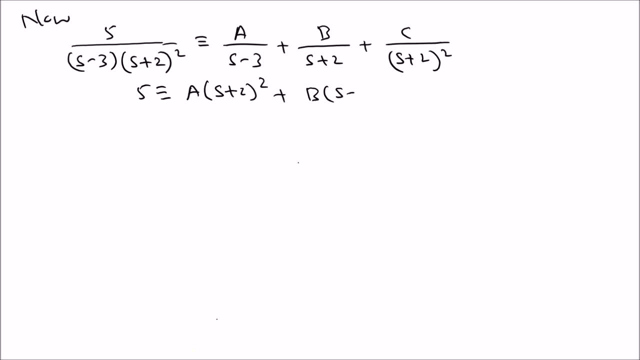 the missing term is: uh, one of the s plus 2 is missing, s minus 3 is missing. last one: only s minus 3 is missing. so we can use a substitution technique now. always use substitution first so we can substitute, let's say, s equal 3. if you do that, you 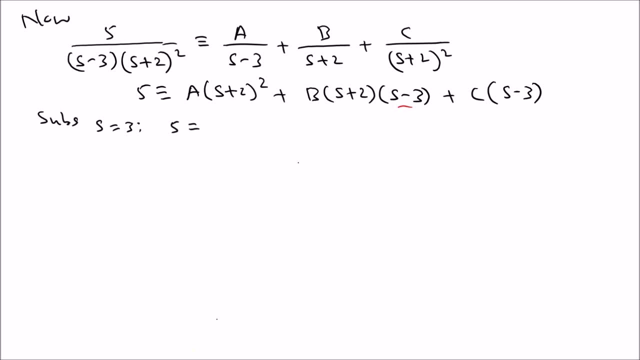 get 5 equal. you can see that you get 5 equal. you can see: plug in 3. this goes away, so you get a. so a. if you plug in 3, this is s equal 3. so it is 3 plus 2 squared plus 0 plus 0. this is going to give you a. 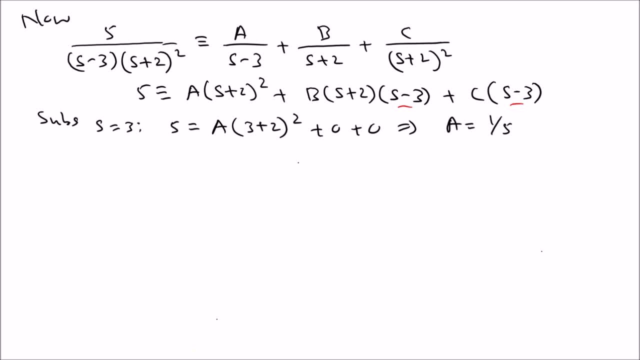 equal 5 over 25, so one fifth, that's a. now we're going to substitute uh, let's try to find, uh, find. what is the other common term you can see. this is common, see, so that means you can find c. so you plug in c. 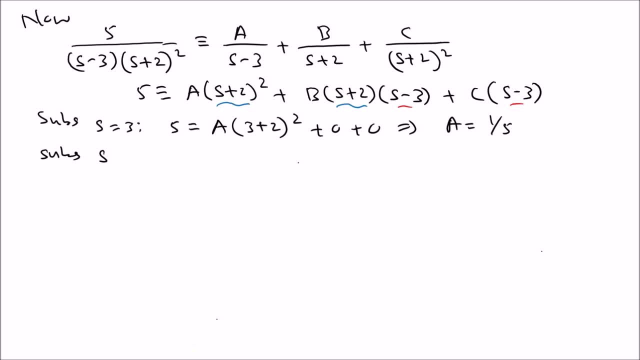 equal negative 2.. so you apply s equal, negative 2. uh 5, equal is a, 0, another 0 and c. if you plug in negative 2, this is negative 2, negative 3. this can give you uh 5 divided by 5. 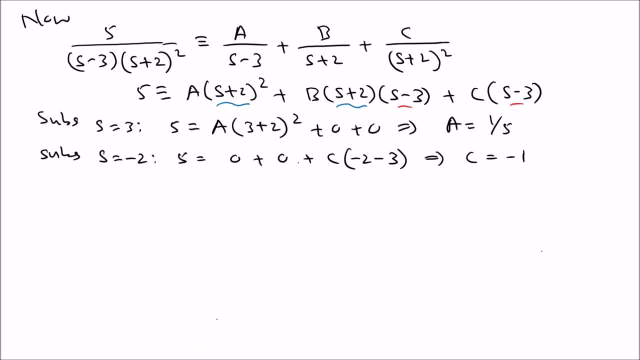 the c equal negative 1, okay, and then, uh, so after. so we only need to find one more. what we normally do is find the equal, the coefficients of the largest term. remember that, okay, because that's going to make the calculation much fast. so, coefficient of the largest term. what's the largest term? 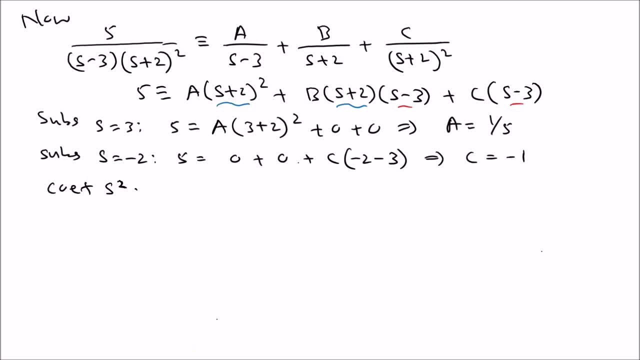 s squared. so we're going to go with the coefficient of s squared, the largest term, so it is 5, largest degree. so you can see how to get s squared term. the first one going to get squared term, the coefficient is a. in the next one, when you foil, you get s. 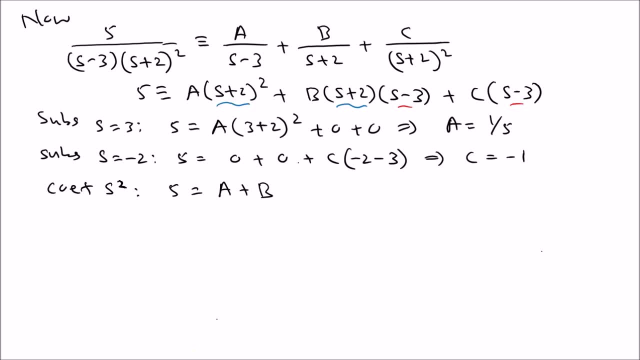 squared b, so that's the next one. since we already know a, we can find b from this one. so this is that b equal 5 minus a, uh, so that means uh, uh, no, actually. so what i did? there's no zero uh here, so there's a problem here. uh, so uh, you can see, there's no uh. 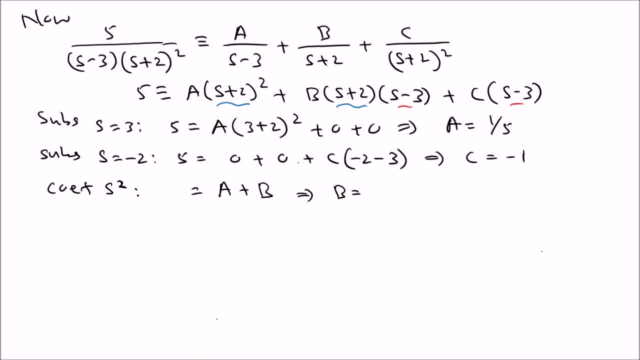 there is no square term, so this is zero on this side. okay, there's no square terms, it's zero. so you get b equal minus a minus c. so, since you already know a, so it is negative one. fifth, sorry for that. okay, so it's zero because. 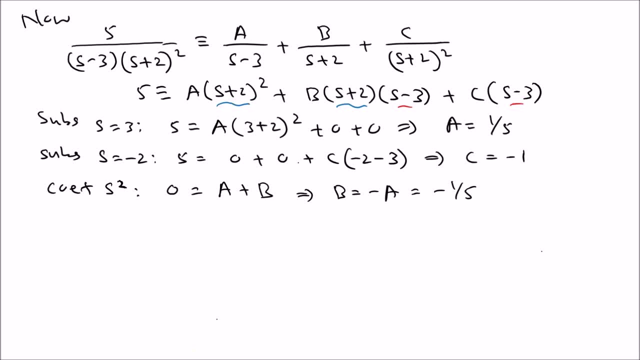 there's no square term on this side, so it's zero. so so you can, so you get a b3 like really quickly. now what we can do, we can substitute that uh, so that means uh. so is one over uh, five over five over five over s minus three, s plus two. 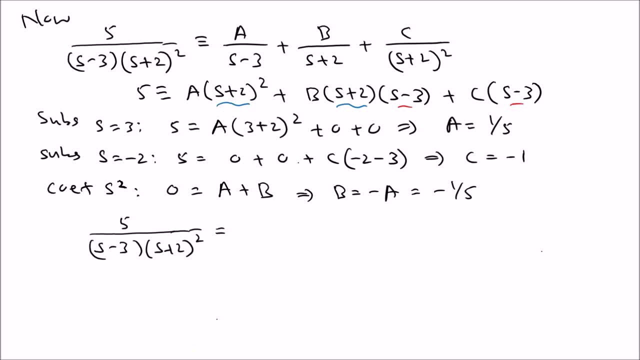 equal. you can write equal. now it is one fifth. uh s minus three. uh, actually, let's write the ss term. it's not this one, because we already know uh yeah, so let's write the ss one. it's very important. so if you write s term, so what do you get? uh, so xs. 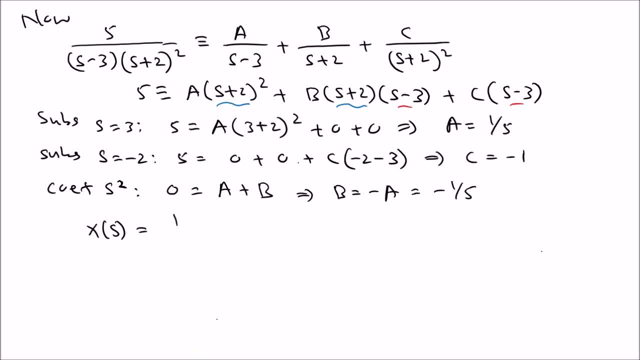 which is 1 over s plus two, plus the partial fraction of these. okay, so we're gonna have the partial fraction now. you see, 1 over s plus 2. we had already, so let's try the partial fraction here. so it is one-fifth, uh over. 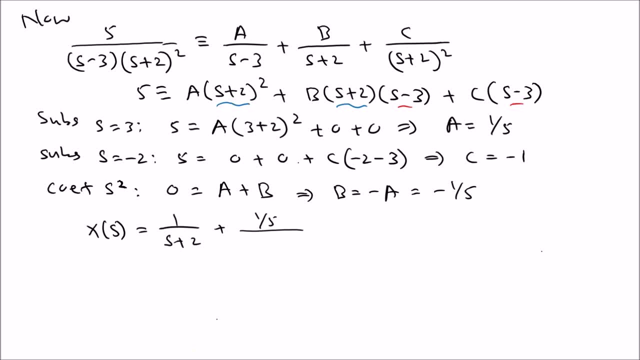 uh, one-fifth of s minus one-fifth of s minus three. so, yes, minus three, that's a. and then we have b, so it is one-fifth of s plus two, one-fifth over s plus two, and the c, uh, which is uh negative one. so it is negative one over s plus two square. that's what you get. 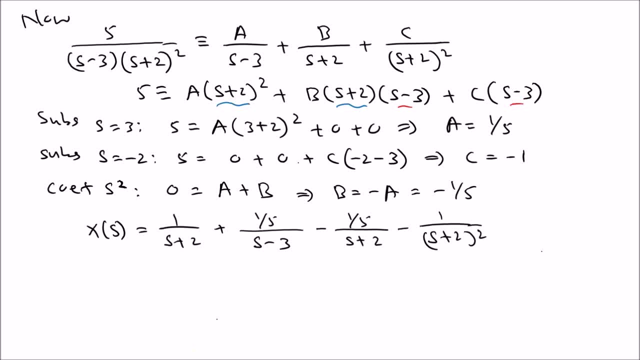 and you can see that you can combine these two. so they're going to simplify. so they're going to simplify, so you're going to get uh uh, so you're gonna get uh four. fifth, so we have four fifth s plus two uh plus one. fifth uh s minus three, minus one over s plus two. 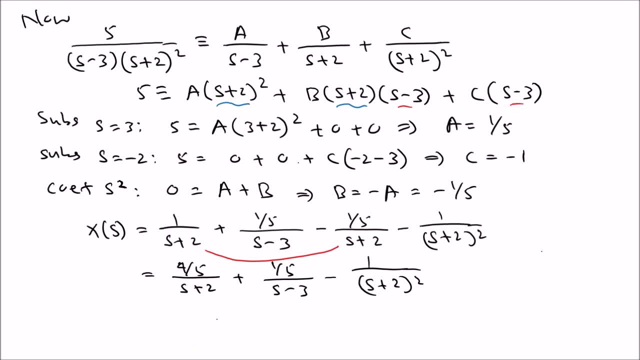 squared so we can find the x t now. so x t is simple. so i just wrote like completely, but some steps, you can even do that, okay. so this is the inverse of this. so we're gonna go term by term. so the first one says it is uh, one four, fifth e to the negative two t. 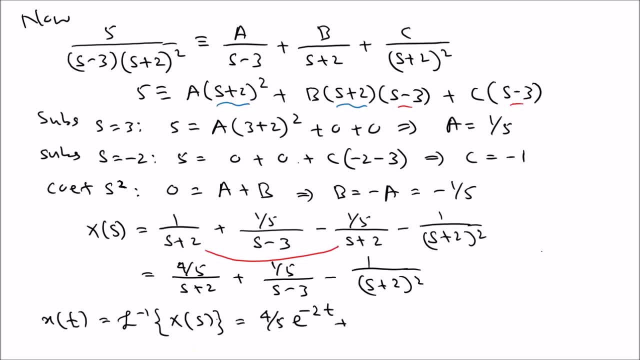 next one says one fifth e to the three t. the next one is: you can see, it is the. the base function is one noise squared. that means a t e to the shifting is negative two t. so that is the. so this is the inverse of this. so we're gonna go term by term. 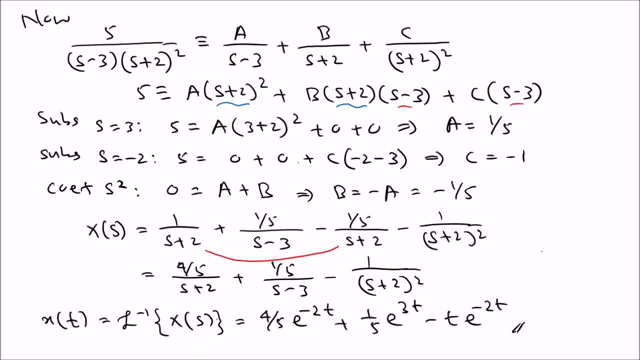 this is the solution of the differential equation. this one is not that long. uh, it's like i came uh quickly, uh even like it's not that difficult to find the partial fraction decomposition for that. so this is a kind of good problem, uh, especially for a final exam. 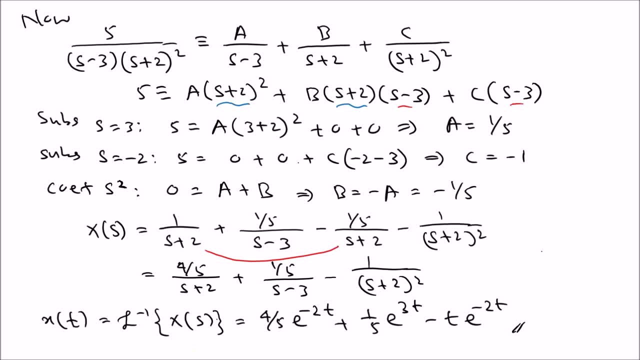 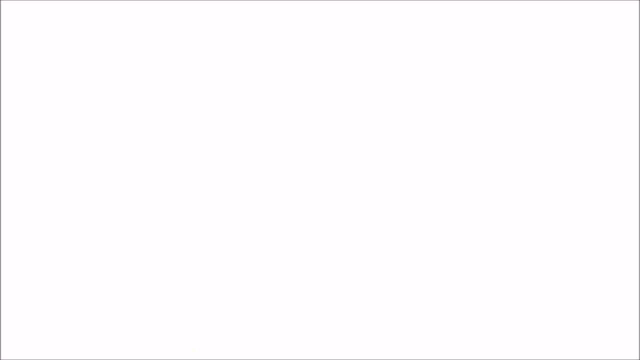 good, uh, next we can talk about the convolution method. so let's discuss the convolution method. convolution method: so, um, we know that the laplace transform is linear. that means, if we have a sum, we can write this one as l f plus l g. so we can do that. 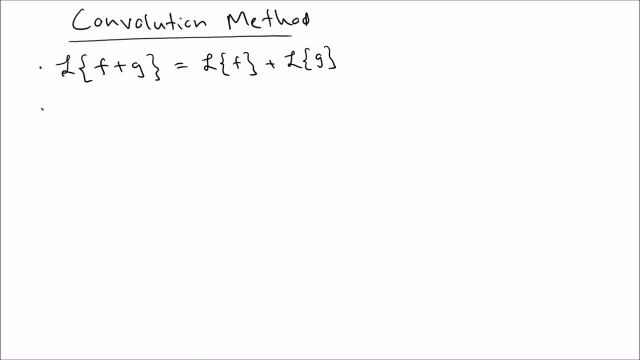 um, if you have a product f times g, this does not equal to the laplace transform of f times laplace transform of g. so there's no such result. so instead we have what we call the convolution. so let's say, let's look at the definition, so what we call the convolution product. 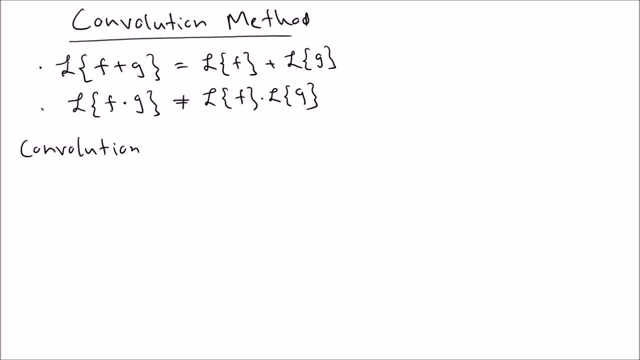 convolution product. so the convolution is defined as an integral. so the notation is star. so if star g, that's the convolution of f and g, so which is from 0 to t, what we're going to do? we let's introduce a new variable called tau, so it's f, tau, g, t minus tau, so t is the variable. 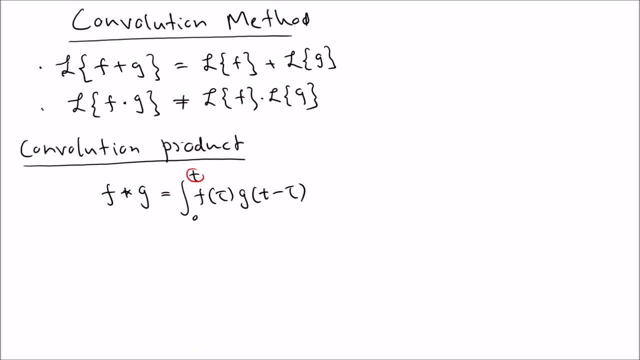 serine name and d tau. o is the variable serine name. or you can even switch the order so you can see. you can put the t minus tau for the first one and then g tau for the second one. the interesting part is they are you get the exact same. 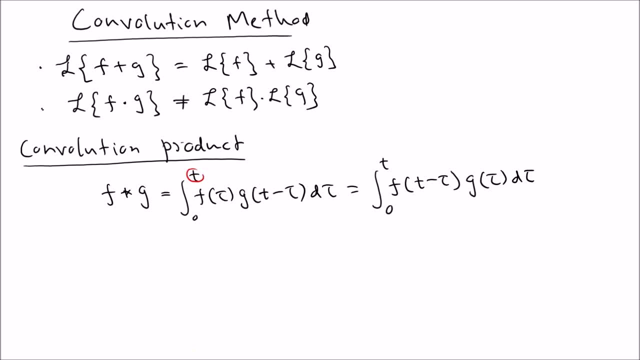 answer from them. so in other words, this means that, uh, this product is uh, so you can, you can switch the two. so that means it is uh, commutative, so you can write it like that. that's what it means. you can switch the order, you still get the same answer, so you. 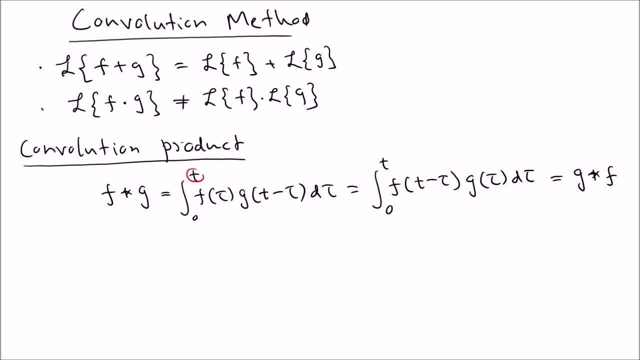 get the same answer. so now the question is: uh, we put t minus tau for the easy one, so that is easy to integrate, so that's how you're going to pick it. so, whatever the easy one, so we're going to see. uh, when you look at a problem, it will be. 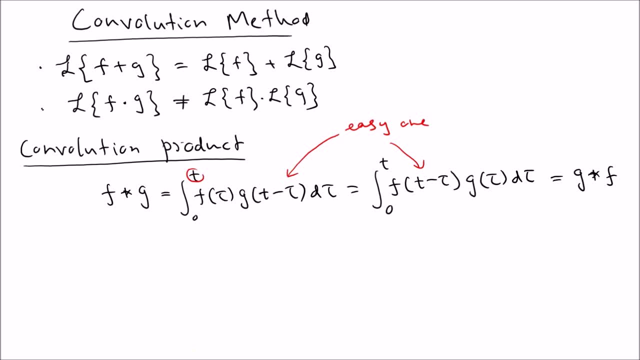 clear what we mean by easy one, and then we have this major result. so the theorem is that it says, let's say, f, g are piecewise continuous, are piecewise, piece wise, continuous and exponential order. ah, and the exponential order and of exponential order. we need that to guarantee that the laplace transform exists. 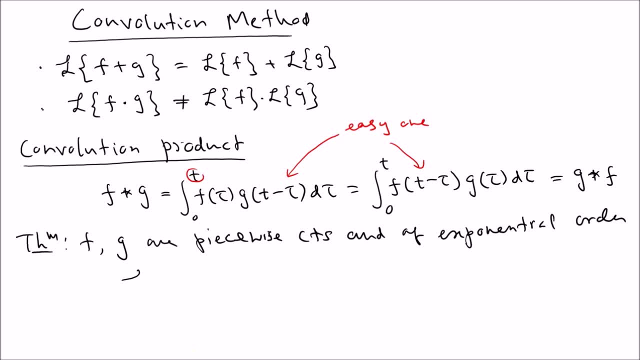 then what happened? the laplace transform of the convolution product f. star g is a, the product of the laplace transform of f and g. so in other words, we write this one as f s times g. this is just the product. so this is the major result. uh, this is. 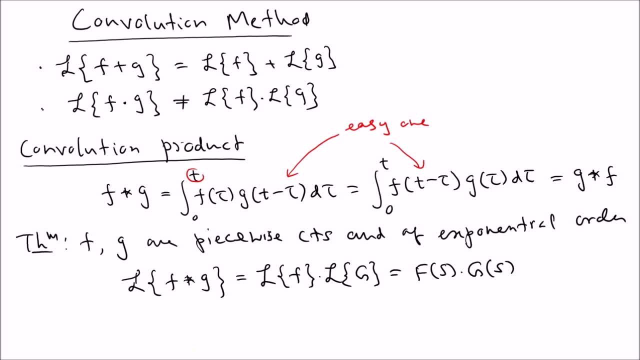 very useful, uh, so that's what we have. so if you look at the convolution laplace from the convolution you're going to get the product of the laplace transform. so the benefit is, this is very useful when you want to find the inverse. so that means, uh, so let's try this as a not. so that means: 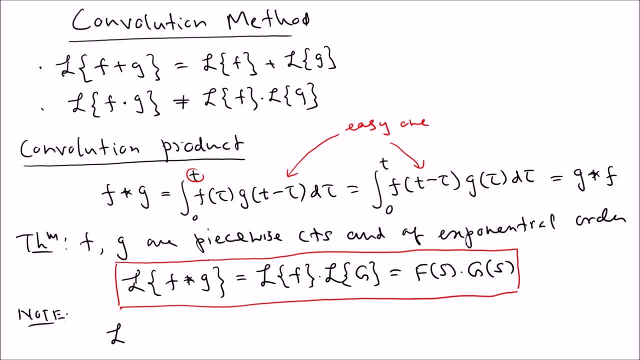 so if you have inverse of the of a product of two transforms, if you know that the two functions, what are the two functions are? just take the convolution. so that's the idea. so this might be much faster compared to, uh, partial fraction or other terms. so that's the idea. 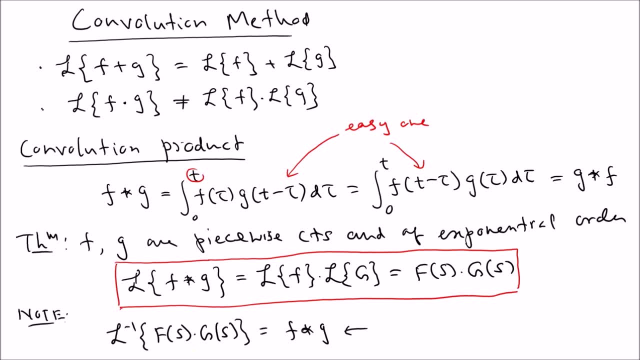 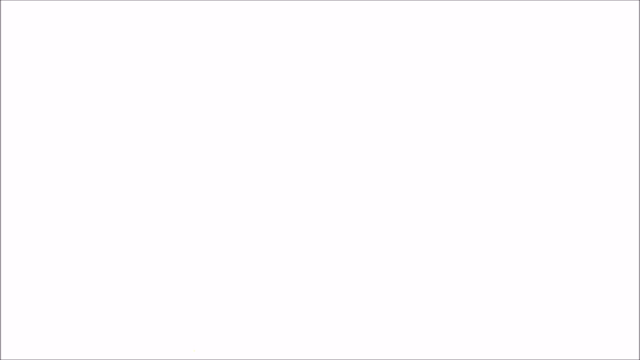 so that's, that's how we can use it. so useful are useful when uh finding inverse. useful when finding uh inverse, uh inverse laplace transform. uh, so let's uh look at that in a in a problem. so let's try to do this uh. so so, example, i find the inverse laplace transform. 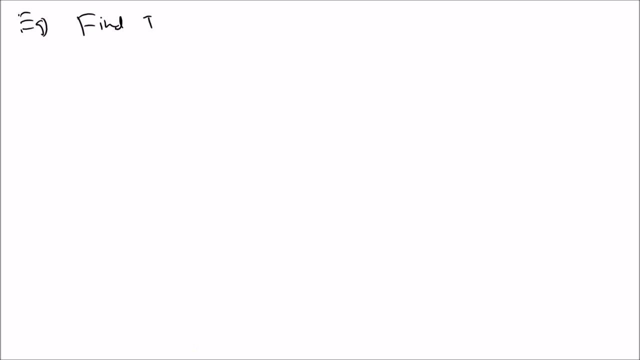 find the inverse uh, laplace transform. so let's do the first one, uh. let's say uh l inverse 1 over s plus 2 times s squared, something like that. so we know how to do this one using partial fraction method. we write the form: find the uh, abc. uh, because there are. 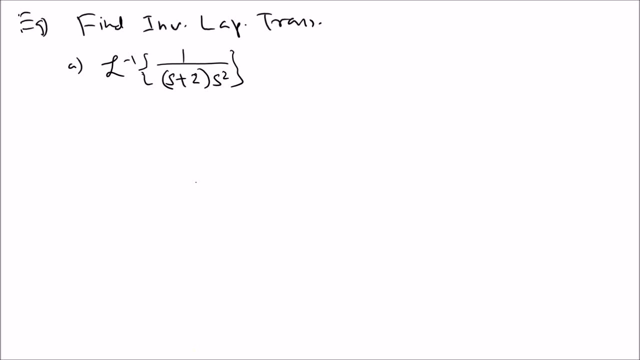 abc. uh, because there are three terms now, and then invert. but how to use the convolution? so we know that. so we're going to kind of try to identify so we can write this one as one over s plus two times s squared. so we isolate that. now we can see. 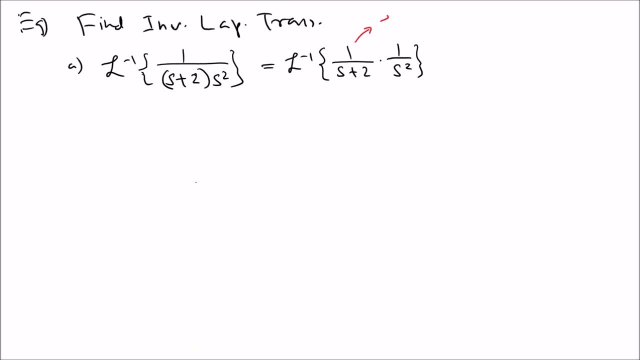 uh, this function is corresponds to e, to the minus 2 t. this one corresponds. so those are the two functions, uh, and then if you tell a person those, that's what you get. so that means, according to the theorem, this is simply the convolution between those two. 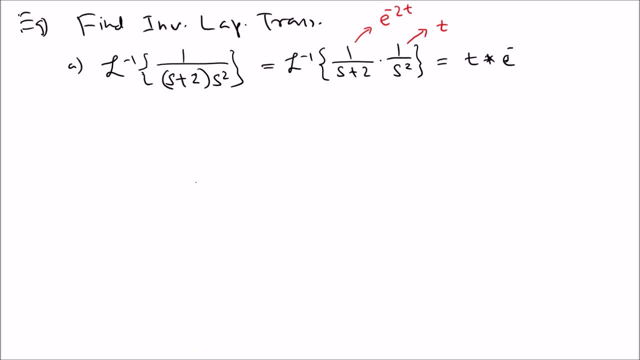 functions. so that's the idea. just take the convolution of those two. so now what we can do, we can use the definition and try to find it. so, uh, the question is which one? uh, we're gonna put t minus 2. so when you have exponential function, it's always a nice idea to put the t. 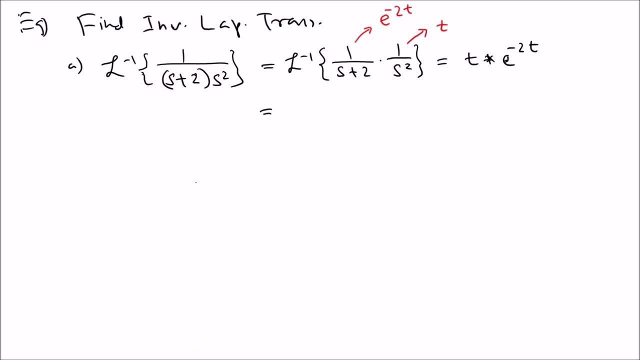 minus 2 to the exponential function. so so we can do that. so 0 to t, uh e to the negative t. we put t minus tau here for the exponential function. other one is just become tau d tau. so the reason is: you can see, you can. 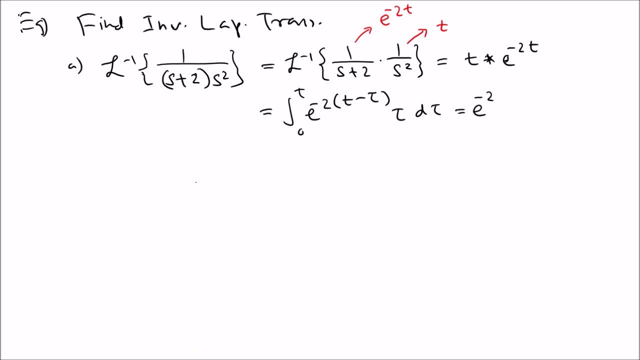 pull out e to the negative, uh, 2t, because that's a constant now, and then 0 to t, uh, e to the negative or negative. if you get negative, negative, you can pull out e to the negative, 2t, tau, d, tau. so this is a very easy integral using partial. 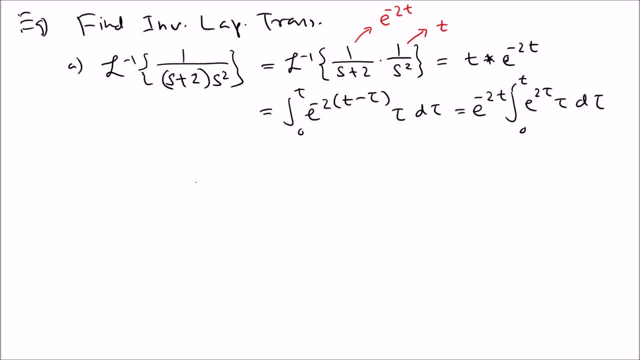 uh, integrated by parts, um, so let's do that. so it is e to the negative 2t. now we're going to see integrates by parts. so we're going to. we can use the d? i method for this one. so let's use the d i method. 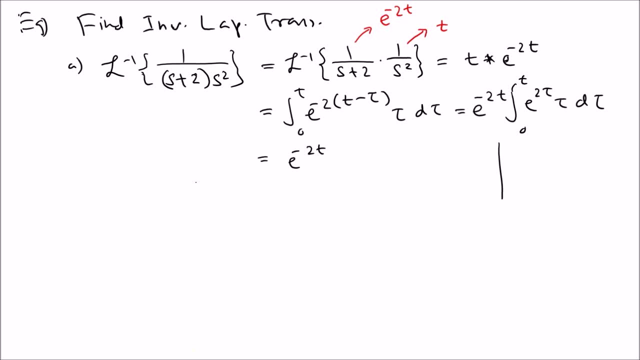 d and i. so we're going to say: for the d, we put tau, i, we put e to the 2, tau. so take the derivative 1, take the integral 1. so we're going to say: for the d, we put tau i, we put e to the 2. 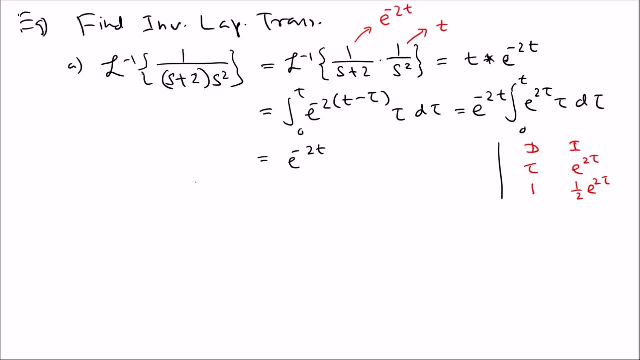 integral: 1 half e to the 2 tau. take the derivative 0, so that means 1, 4 e to the 2 tau. and then what we do? we multiply plus minus, so that's what we get. that means the answer is simply: uh, we're going to multiply the two, so 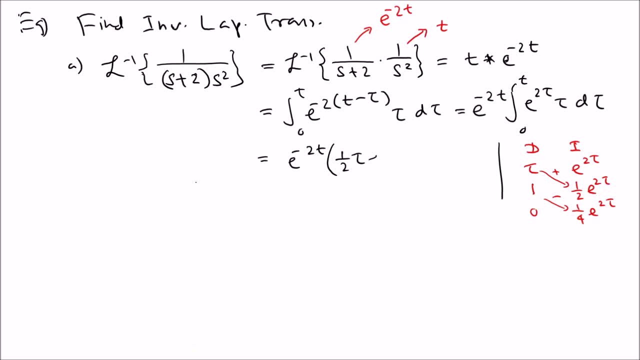 it's a one half tau e to the 2 tau and then minus uh, you get one fourth uh e to the 2 tau and then we can evaluate that uh. so let's change that. we can evaluate that uh at t and 0. so that's it. so that's the answer uh. 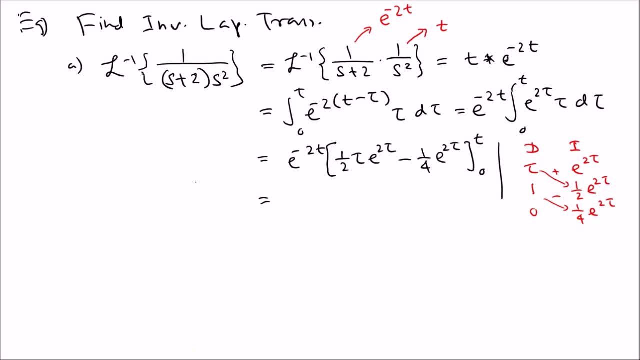 so what? we get uh. so you're gonna get uh e to the negative 2 t uh when you plug in t. so you get uh e to the negative 2 t uh when you plug in t, so you get uh, you get uh. you get a one half t e to the 2. 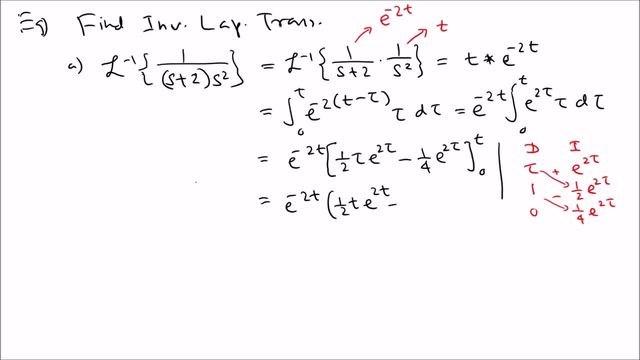 t and then minus one fourth e to the two t, and then, when you plug in zero, the first one is gone, the next one becomes simply one fourth. and then what we do? we multiply by e to the negative 2 t, so you get one half t. 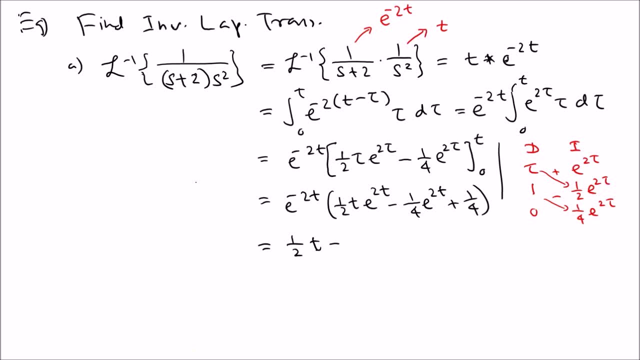 minus, oh, um, uh, yeah, so it's gonna be plus one-fourth, uh, good, uh, one-fourth, and then we have no, that's, that's, uh actually. so it is negative because we we multiply negative 2t with 2t, so you get negative. 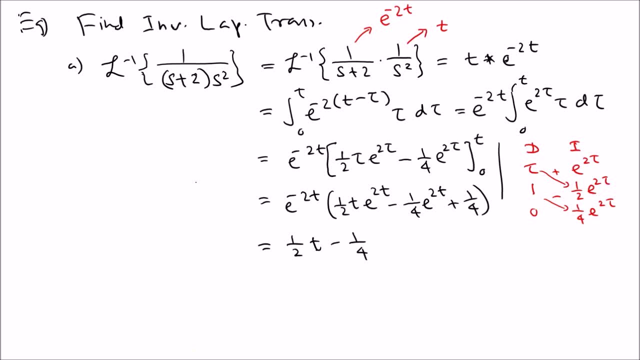 one-fourth, and then the last term gonna be uh plus one-fourth e to the negative 2t. so that's the answer using the convolution method. so it looks like it's a little faster compared to the partial fraction, because we just need to evaluate a simple integral here. 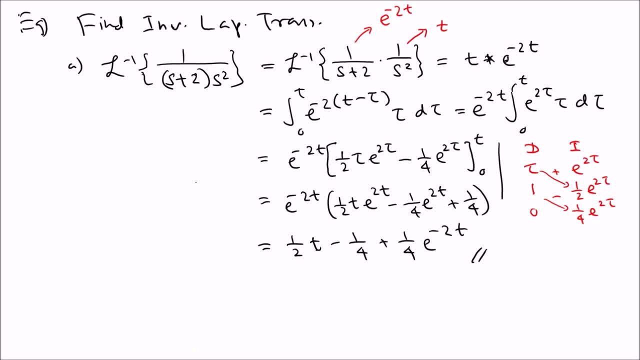 good, um good, so let's try to do one more. uh, so let's do this one. so the laplace inverse laplace transform of 3 over s squared s squared t. so let's do this one square plus four, so this one. if you do the regular way, it little lengthy. 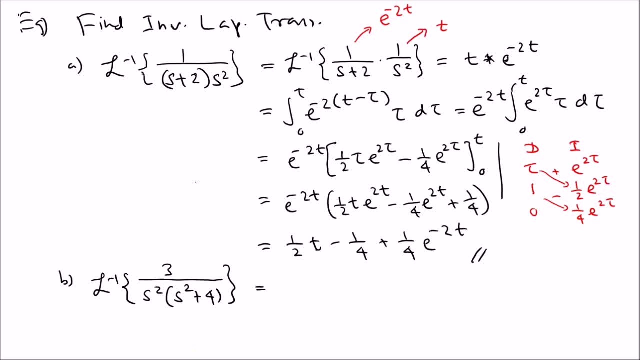 but let's see how uh it's gonna be now. uh, so what we can do is: uh, we know that if you look at square plus four, that's related to the sine. so what we do? we take uh two, we multiply and divide by two. uh, so this: 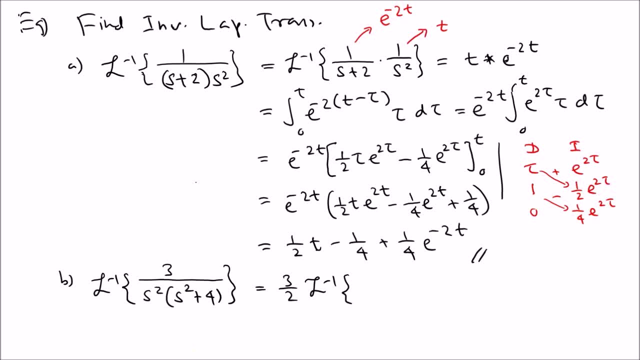 is l inverse, so we're going to arrange it so: 1 over s squared times 2 over s squared plus 4.. so we can write it like that. now you can see: uh, this is t, this is related to sine 2t. so we have the two functions. now what we need is, according to the theory, this: 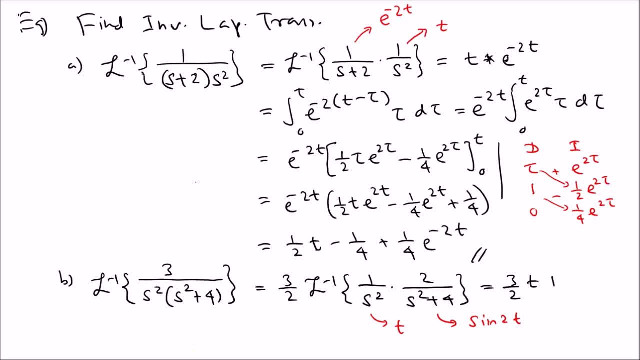 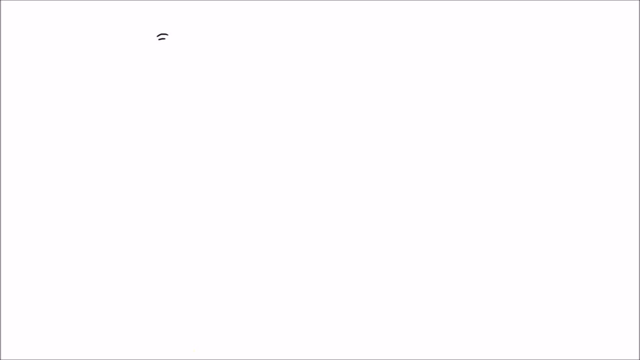 simply becomes three halves. that's there. t convolute with sine 2 t. so that's what you get now what we're going to do. we need to find the simple convolution and you get the answer. so that means this is equal to the integral. so we have. 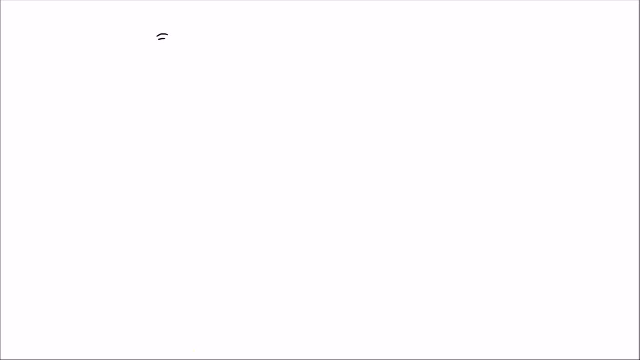 again, we can use the uh, d, i method for that. so the d and the i, so d uh. first let's write: the integral representation is a two-third, three halves zero to t uh. i'm going to put t minus tau for the first one, and then sine two tau d tau. 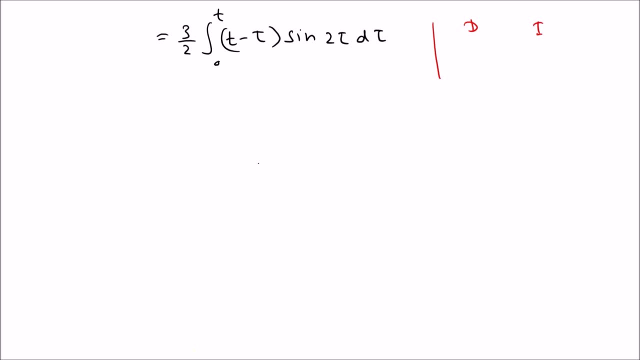 so this one we can use uh do using the uh d i method. so t minus tau goes here sine 2, tau goes to tau is the variable. so we state the derivative t is a constant. so you get negative one here and the other side you get negative one half cosine. 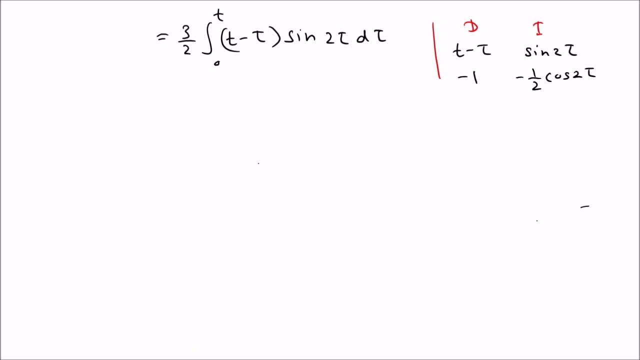 2 tau. and then i take one more derivative zero, so uh, so, cosine, that means you can divide by one half, so it's a negative one. fourth, sine: two tau, two tau. so uh plus, uh minus. so we can all right then now. so you're gonna get. so let's plug in that, so we know the two. 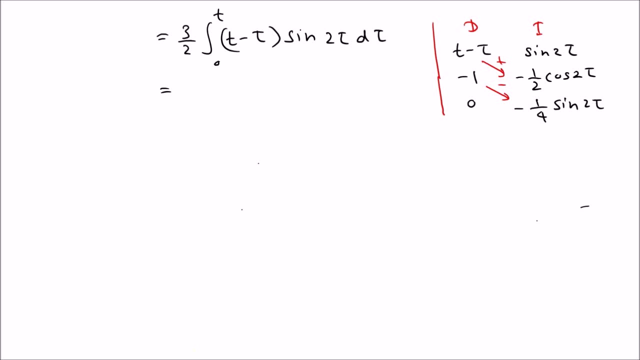 product here. so let's plug in that. so it is three halves uh. the first one is uh. negative one half t minus tau. cosine two tau minus one it's a uh, because oh, we have three minus sign. this is minus one. fourth sine two tau. we can evaluate that at t and zero. 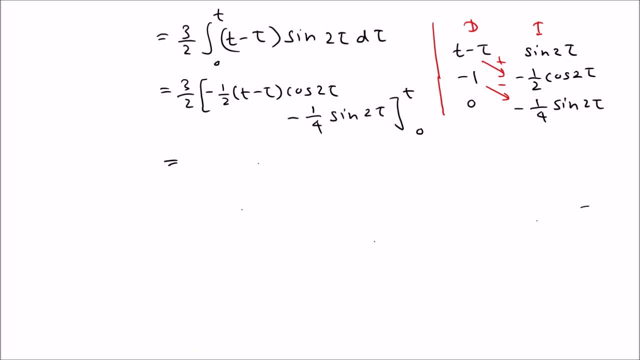 so if you evaluate, if you plug in t, the first term is zero. ah, and if you plug in zero, so you get r t hat f and then uh from the next one. when you plug in um zero, you get zero. for negative t, you get negative one. fourth: 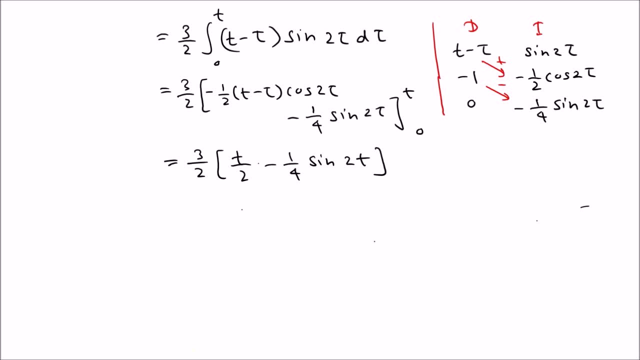 sine two t. and then finally, if you multiply through, you get three fourth t minus three eighth sine two t, it looks like. so it's very simple compared to the partial fraction method. uh, that little ending. so like it's up to you, like you know, whether you want to use. 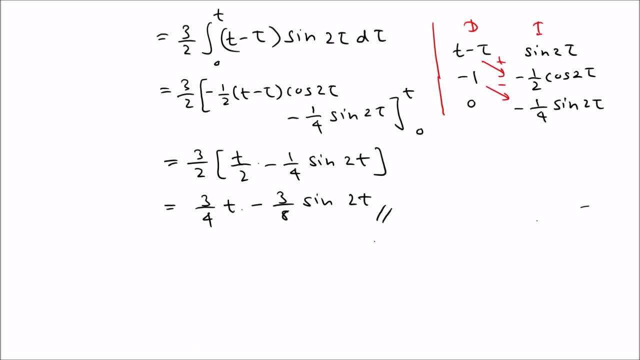 the convolution or partial fraction method when you get a problem, unless it says that use the convolution. so that's the kind of idea. um, so how about this one? so how about this laplace transform? so this is another example. so find the laplace transform of the integral from 0 to t sine 3 tau. 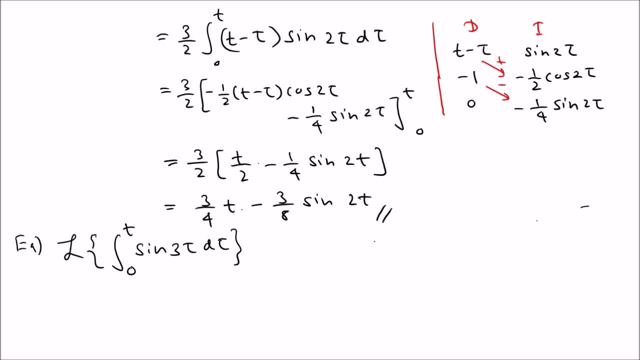 theta. so you can see that this is a convolution problem. what happened why you don't see the t minus tau's term? because that's a constant term, so that means it is simply convoluted with one. so that's why you don't see the t minus tau, because 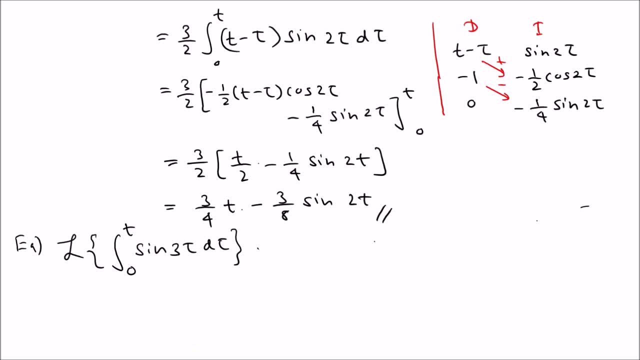 you can put the t minus tau to the constant. so that means this is simply the convolution between one and the sine 3t. so if you do that one, so uh, so that's the convolution. so actually we, we'd write it like that. so this is the convolution of. 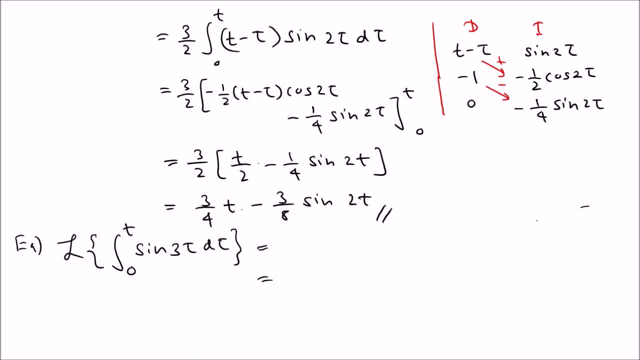 this i like. it's the convolution between one and sine 3t. so by the product, this is the convolution of one times the convolution of sine 3t. so if you use uh laplace also, 1 is 1 of s times 3 over. 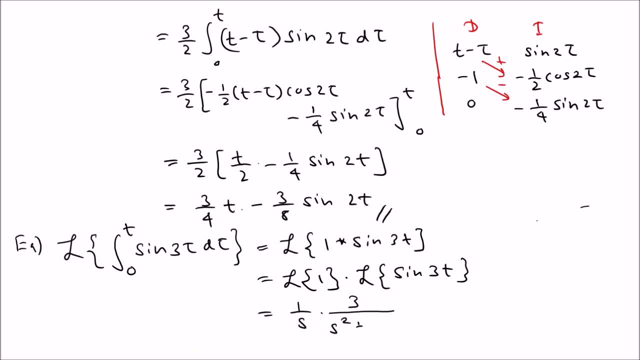 s squared plus 9. so if you write as just one single explicit s times s squared plus 9. so, uh, so we can do that. so, like, sometimes it's not really visible, you know what is there. yeah, so that's a good one. and then, uh, so we can, we can use convolution's. 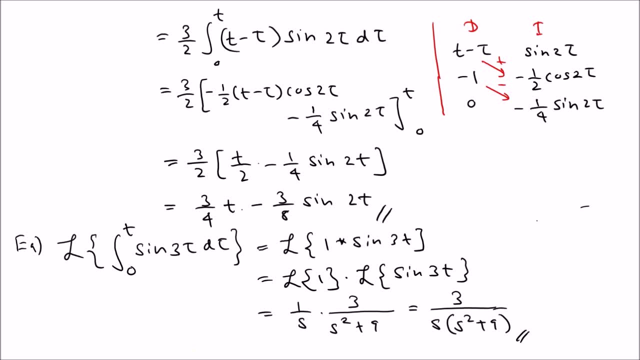 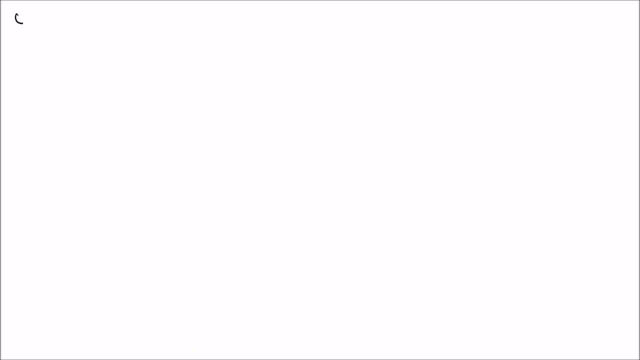 if you want to find the inverse, okay, so let's. uh, so let's put it off in words so we can say, uh, use convolution, not a must, but you can, okay, use convolution when finding inverse, finding inverse laplace transform. so let's go to the next topic. uh, that's the heavyside function. 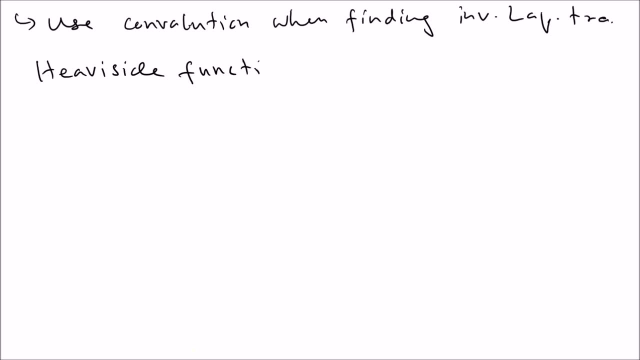 a heavy side function and switching. so, uh, we talk about the switching. you know, when we have a piecewise function, you can use this as a switch. so let's go with the definition of a heavy side function. oh, you need step function. let's see. so if you look at the graph, it looks like. 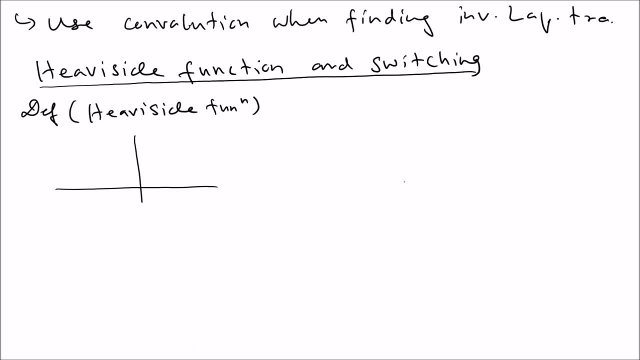 that. so what's going to happen? until 0 is 0, and then, at 0, it can jump to 1 and it stays at 1. so that is, uh, uh, the what we normally write as ut at 0, and then we have the shifted version of. 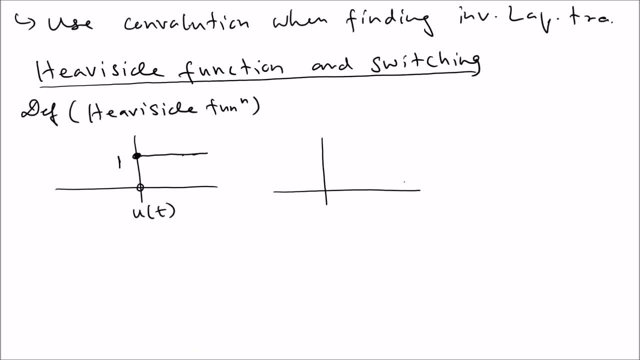 that. so let's say it's going to jump at a. so until there is a and then at one at a, you can jump and it stays there. so that is the uh heaviside function shifted by a. so it is u t minus a um. this is one at that point. so that's the uh function. good now. 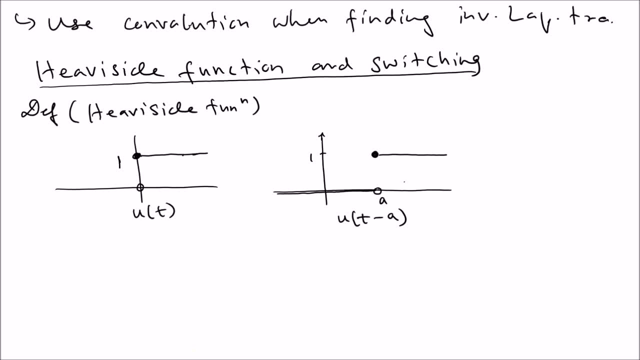 uh, so the laplace transform of those. so we have the laplace transform of the laplace transform of the heaviside function. so laplace transform. so we have laplace transform of u t minus a equal e to the minus a s over s. so that's one. it's very useful. um, it's very easy to show this one, just. 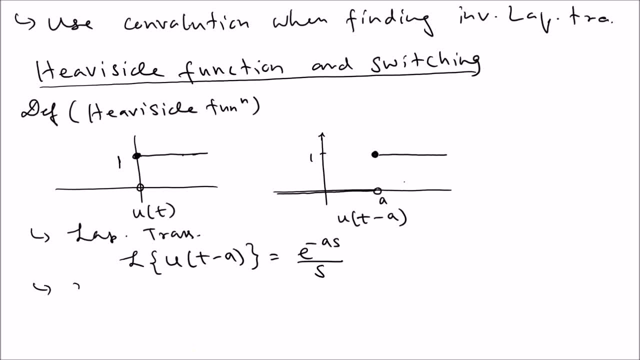 use the definition and then we have also second shifting theorem, second, uh shifting theorem. so what it says? that the laplace transform of u, t minus a times f, t minus a. so it has the exact same format: t minus a, t minus a. so see that t minus a, t minus a term and t minus a t. 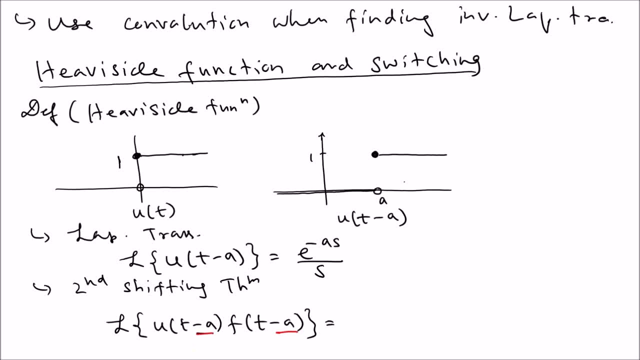 so what's going to happen? this simply become e to the minus a s, so they have the exact same format again. so that's the laplace transform of u, t minus a. again minus a s, times the laplace transform of s. so that's, uh, that's what we call the second shifting theorem. 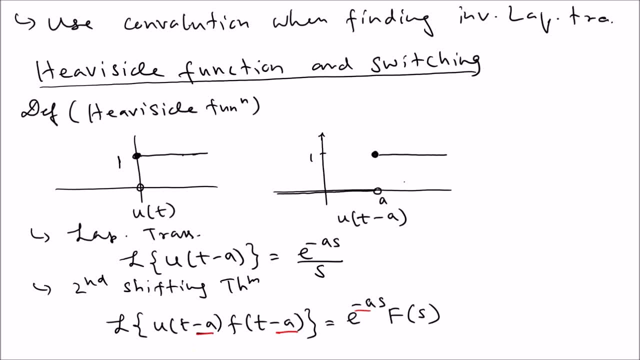 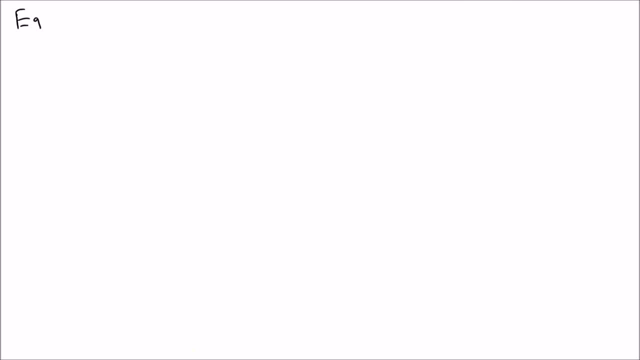 uh, now let's try to uh use this to find the inverse laplace transform of a certain function. so let's do this one just to see how it works. for example, find the inverse laplace transform of a certain function. so l inverse s plus 3 over s squared. 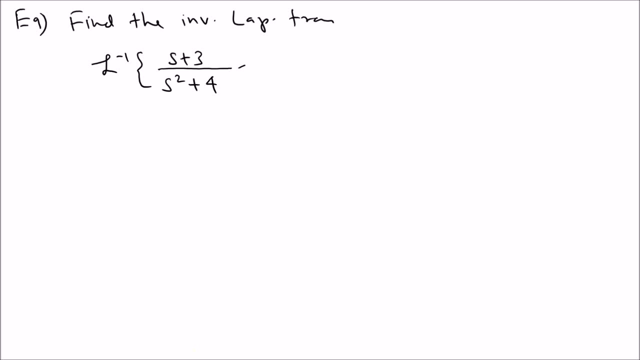 plus 4 e to the minus 2 s, something like that. so let's say you have this one. so it's clear that that is the exact same format that we have, uh, the second shift in theorem version. so what we're going to do, we're going to shift this first uh, so we can write this: 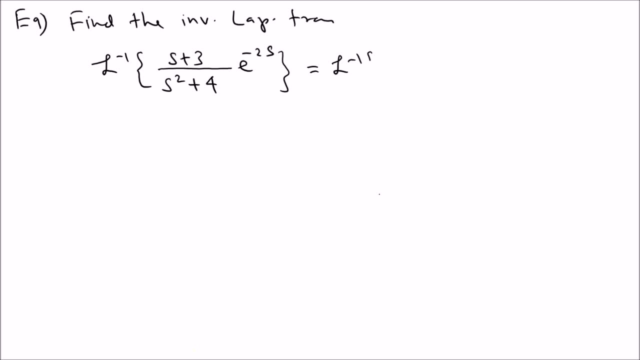 one as l inverse uh. we can go with s first, so s over s squared plus 4 e to the minus 2 s, and then look at the next one, the next one. we have three, but we actually need two. so we can do that: three halves l inverse uh, two, and then we have s squared plus. 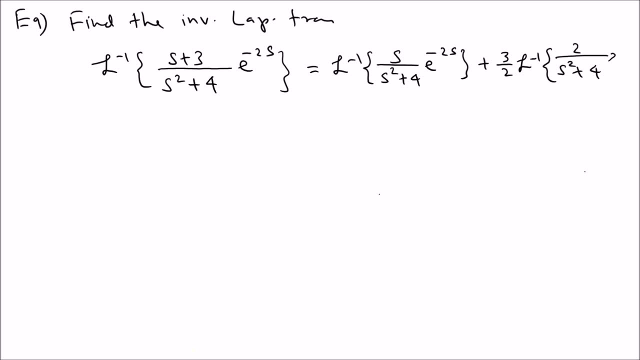 four e to the minus 2 s, like that. now we can see l inverse. this is the cosine r 2 t, this is the sine 2 t. so what we want to do is: uh, from that we need to just shift this. so that means the answer is uh, you can shift by. 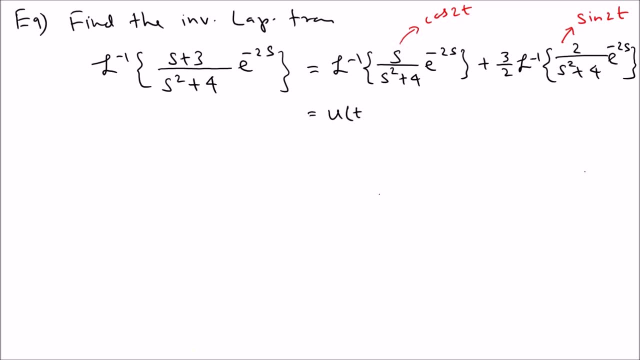 2, so it is u? t minus 2, the cosine 2 times t minus. we have that three halves again: u t minus 2 sine 2 t minus 2, so that is the invariable plus transform. so that is how we use that idea. 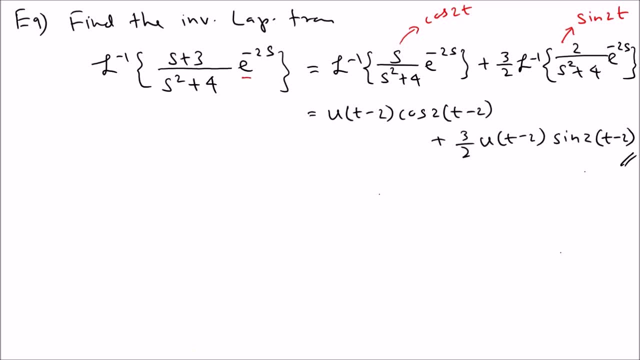 when you have a e to a function like that, it's just a shifting, it just uh gives a second shift in theorem for that. now, uh, let's look at how we use this for uh switching um. so let's do a problem like this. so let's do a problem like this. so 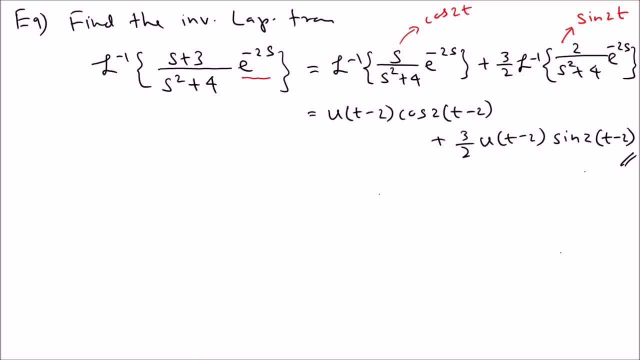 let's use a problem like this: uh, let's do uh, uh, rewriting a piecewise function using uh switches. so rewriting, rewriting a piecewise function, piecewise function, uh. so let's look at the idea like a problem like this. so example: um, so let's say you have a function like this, so let's say rewrite. 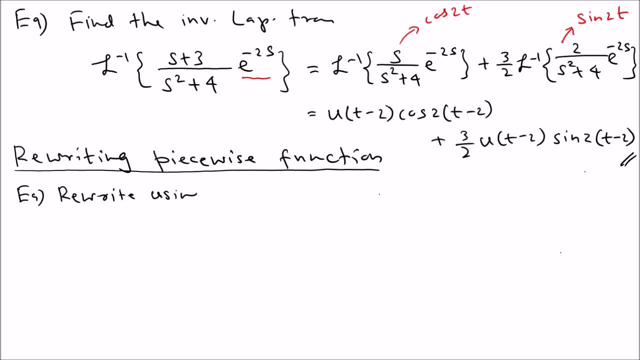 are using a heavy side function. so what we can do, let's say f t, let's see how piecewise function like this: t minus 1 on the interval 0 to 1, and then sine t, uh after that. so if you look at the graph, this is how. 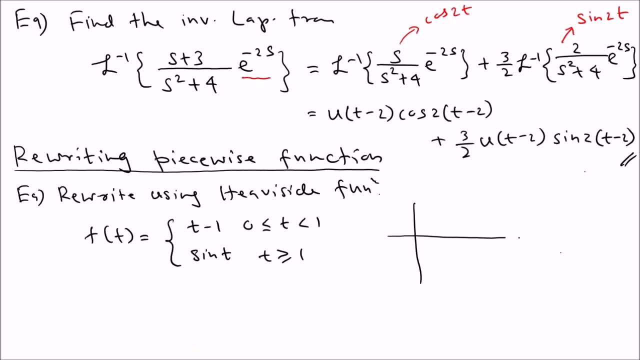 it looks like so, uh, from zero to one, it is a t minus one. so that's the t minus one function. it's gonna go with one negative one. and then what happened? uh, it's gonna jump to the sine function at one. so, sine one, sine one is a number somewhere. 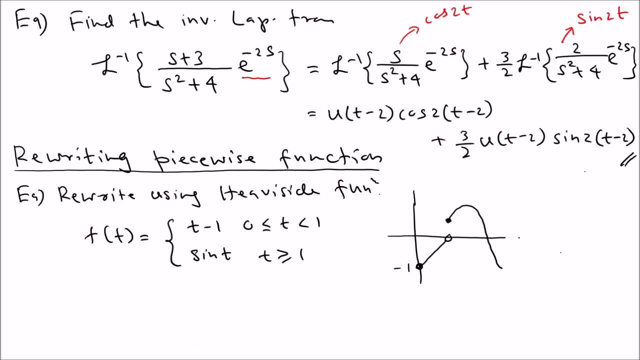 and then it's gonna follow the rest of the sine function. so it's gonna go like that. so that's the idea. uh, after one it's gonna follow the sine function, but until then it's t minus one. so these are. these are what we call piecewise. 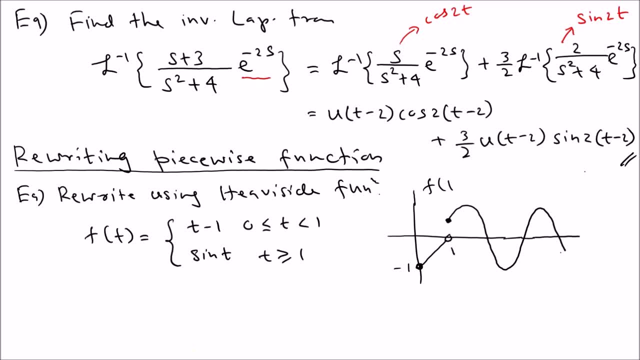 function. so this is a nice uh piecewise function. so the question is how to write this one as a uh, using uh as a single function, as a single function using a heavy side function. so what we can do, we can add a switch here so you can see: uh, we want into the switch for the first interval. 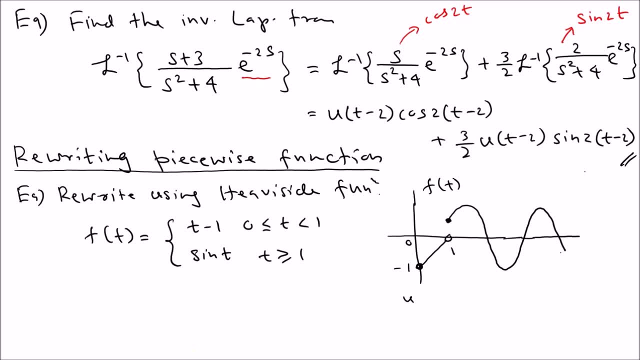 from 0 to 1. the is switch on at 0 and then off at 1, so that's what we do, and the next one we're going to switch on at 1. so that's the idea. so that means we can write this one as a single function, and 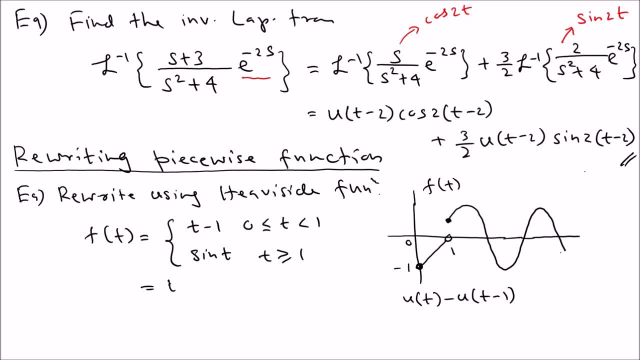 write this one, as we can multiply just by the switch. so we have the function t minus 1. we're going to multiply by the switch, so the switch here is u t minus, u t minus 1 and then plus. that's the first one. let's go switch on only in that interval. 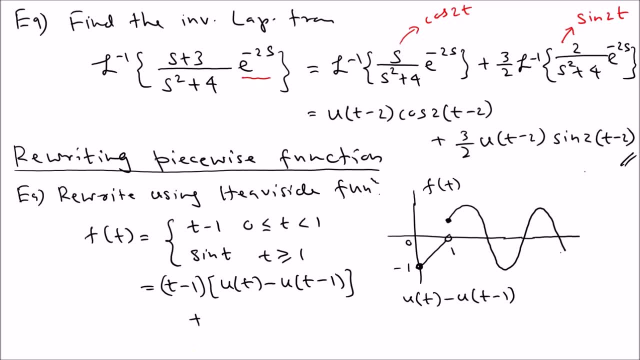 the next one is sine t. uh, that's, you're going to switch on after 1. that means you multiply by t minus 1 the function, whatever the function. so sine t, so that's how you write- are using switches and if you want, you can even combine them into one function for 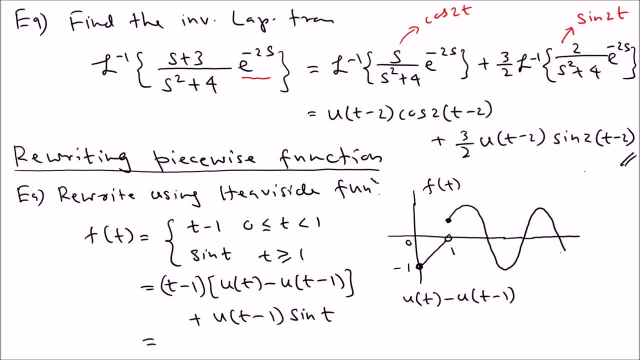 example, there's only one u t function. so that means you can write this one as t minus 1 times u t, and then there are t minus 1 function. there's a t minus 1 here, and then also sine t. that's positive. so what we're going to do? 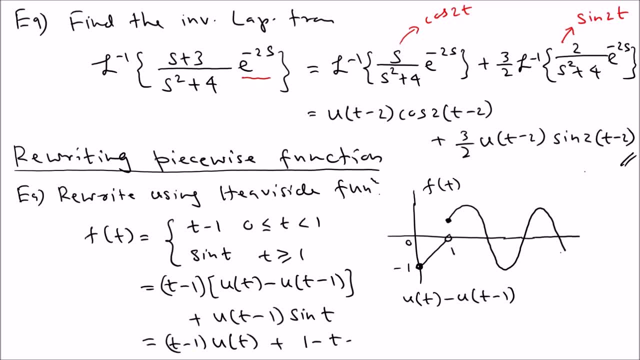 we can write this one as plus 1 minus t, plus sine t times u t minus 1 as two separate uh u functions. so that's how you write this using uh switches. um simple idea: you can switch on at the first node, off at the other node, so that's the off. 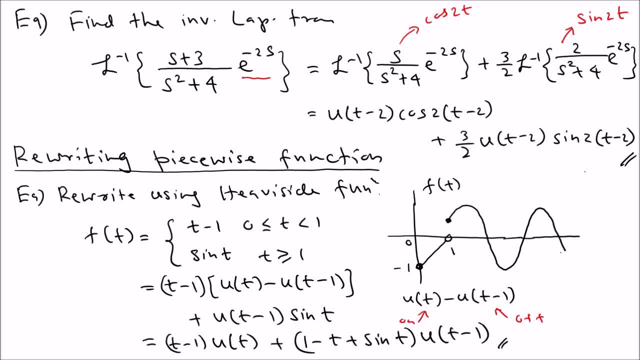 part, that's the on part. uh, yeah, just pick the two values. so that's idea. and then, after what you can do, you can use this theorem to uh proceed with this. so let's just solve one example to see how it works. probably we can combine this and the convolution in this problem. 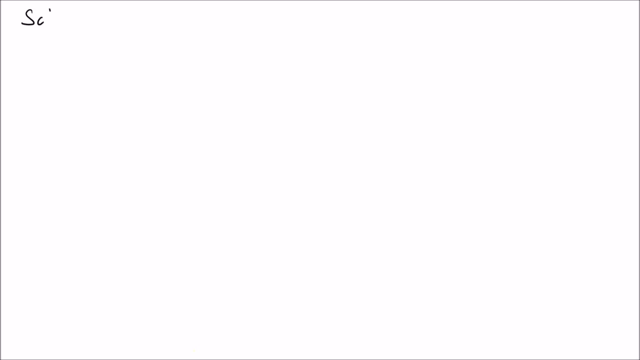 so let's solve this one. so solving, solving a differential equation, solving a differential equation, equation with a piecewise input, uh, piecewise input, solving a differential equation with the piecewise input, like that, uh, so the example is this. so let's solve this one. solve, let's say, x double prime minus, x prime minus. 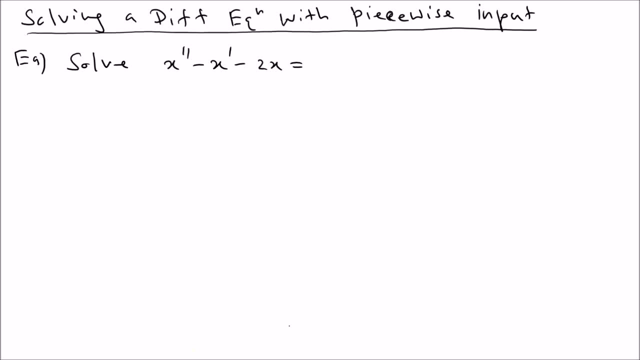 2x equal f t, along with x 0 equals 0. so this is f? t and x prime 0 equals 0, just to make things easy. so where let's say f? t equals something like this: 3 t, 0, t greater than or equal 1 and 0. otherwise, 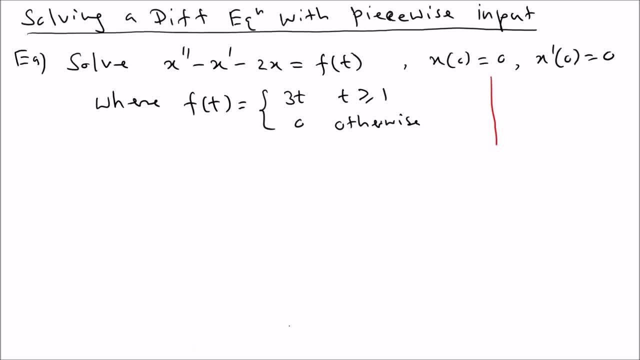 so that means, if you look at the graph, this is how it looks like. so what happened until one is 0 at one is exactly: start with the 3t graph. so that's that. it's going to follow that. so that's the f how the ft function look like: at one. jump to that. and until there is. 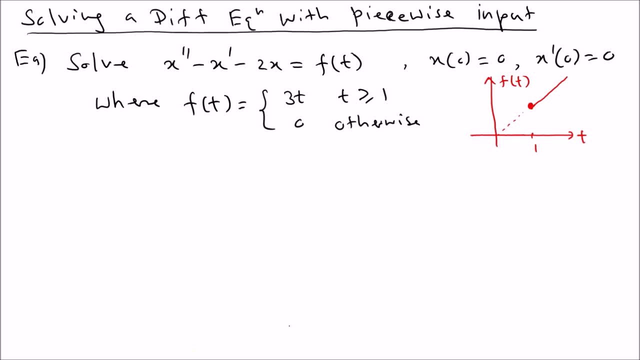 zero, just stay zero, so no input. and all of a sudden it's going to exert a some input, like voltage, current, something like that, which changes, uh, linearly. so this is a. so now what we do if you get a problem like that. we first use the switches to. 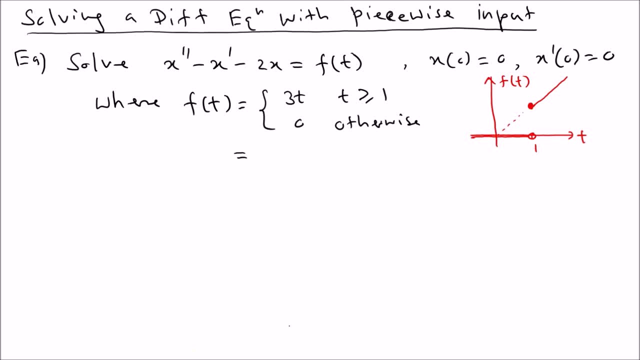 write it so you can see. you want to switch on at one. so that means this is simply 3 t u t minus 1. that's what happened: 3 t times u t minus. this is this is switch on at one um. so the goal is to use the second shifting theorem, because you're gonna. 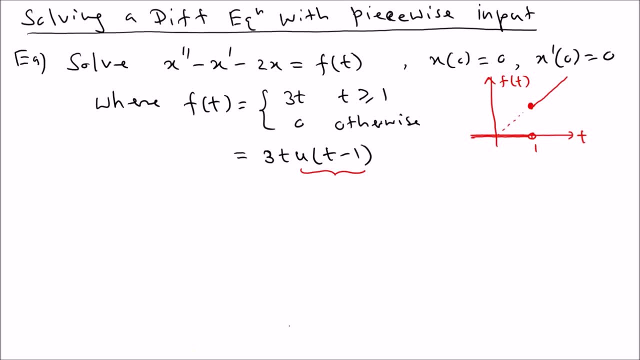 try to use the because there's no other way to do it. uh, you can directly use the theorem like integral. that you can do. you can use the integration and you can integrate this one. that's one way to do it. but if you want to, second, shift in theorem. 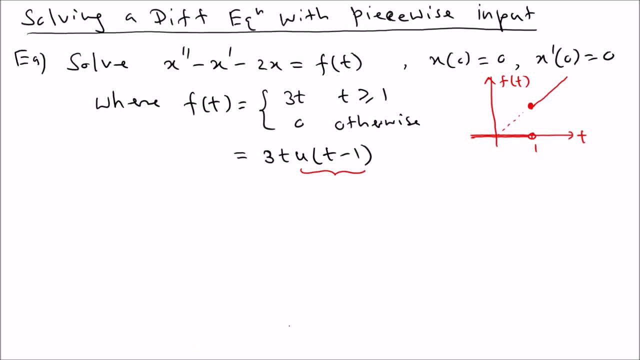 you have to write this in: t minus a form, t minus a form, so a, in this case, is one. so let's do that. so what we're gonna do, we're gonna subtract and add one, so we write this one, like this trick here. so what we're gonna do is we're gonna 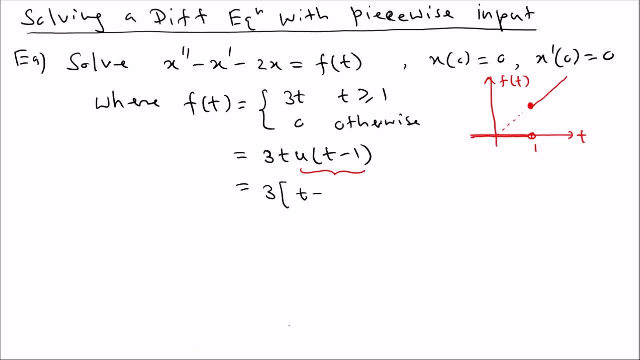 we'll start with t. we're going to subtract 1 and add 1 and then u t minus 1. now if you distribute with the first one, you get t minus 1, u t minus 1. in this case the function is f? t. that's the function: f t equal t, and then 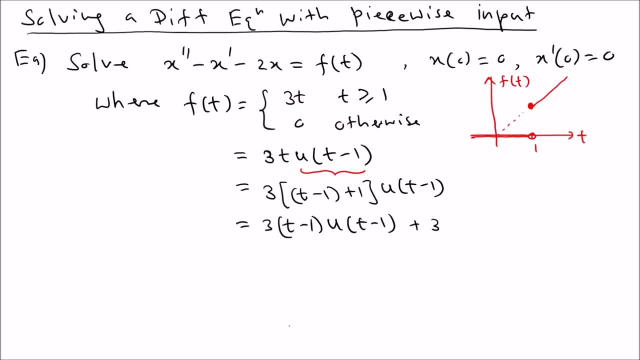 the other function is simply 3 times u t minus 1. we know the laplace transform of that, so that's how we find. so we're going to simply get the two laplace transform of these two. uh, if you write it like that, so that's the. that's the point. 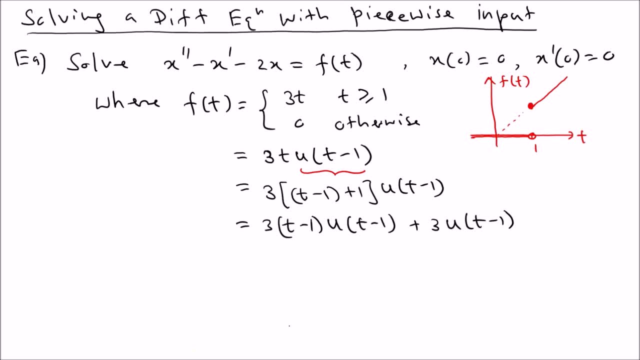 uh. we write it uh in this form, okay, uh. so so the answer here: because you're writing if t in this form, so we write it like that. now we can simply find the uh, the uh laplace transform. so so if this is the case, then the laplace transform of. 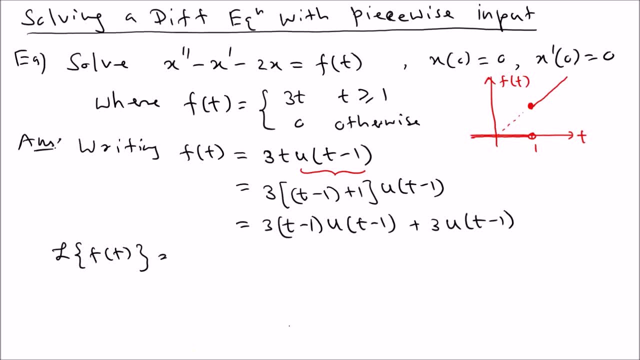 f, t is uh. so it's a three times the laplace transform of t minus one, u t minus one, plus three times the laplace transform of u t minus one. and we know that there are formulas for both. so the first one is simply three. e to the minus s over the function is 1, 0 s squared. that's the laplace. 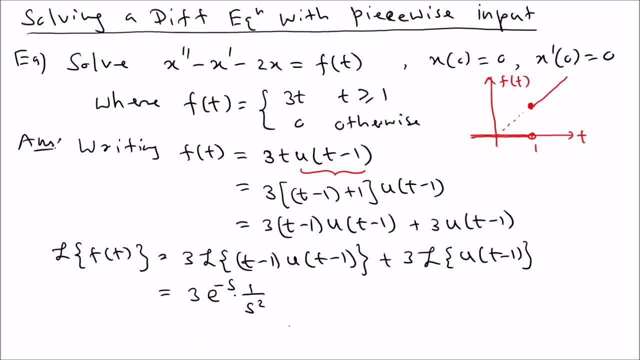 transform of 1 y 1, because that's the function plus the second one, it is 3 times e to the minus s, that's the second one. so what we can do now over s actually. so there's s. so now what we can do, take the common. 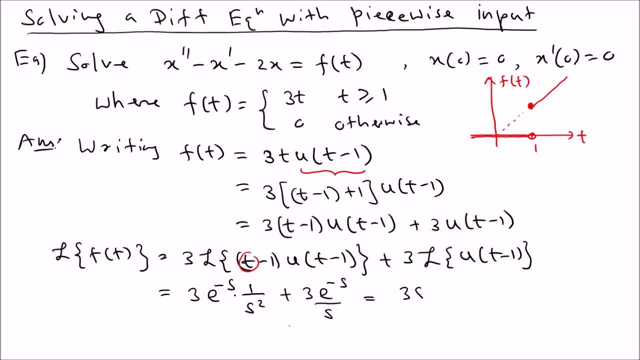 denominator, common denominator is squared, so we can write this one as 3 s plus 3 over s, squared e to the minus s. so you can write it like that. okay, so that's the laplace transform of the signal, the input function. now let's take the laplace transform of. 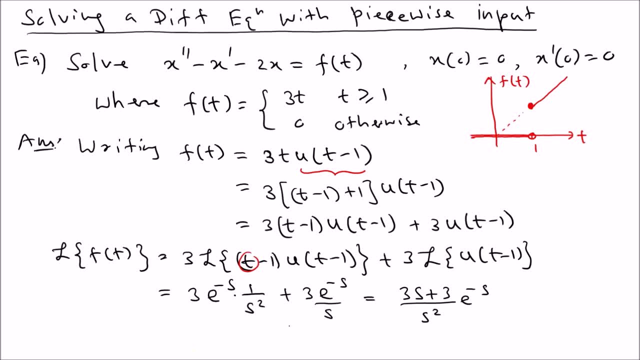 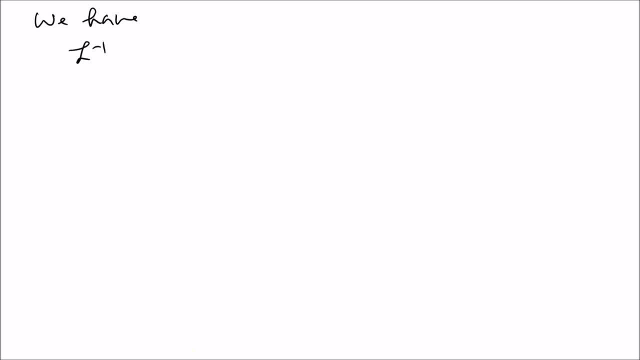 the differential equation. so, uh, so we have uh the inverse, not the inverse the laplace transform, uh, no, yeah, so let's, let's do it like that. so let's say: uh, taking the laplace transform, taking uh the laplace transform, uh of the differential equation, we're going to get s squared. 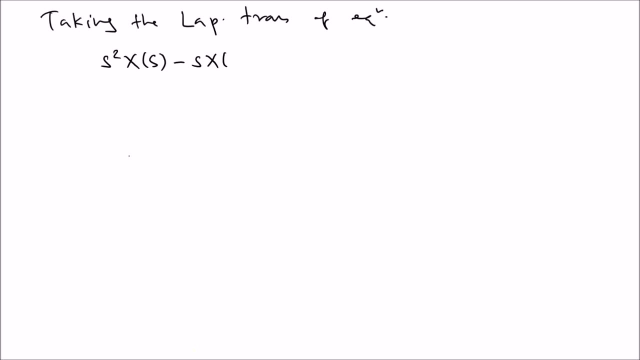 s x. there are no initial conditions, so only the sx terms minus and the minus 2 s x. so this, what we have on the other side, is the s? s that we already know. so this is s squared minus s minus 2 times s x. the other side, it is three s plus one of s squared minus S squared minus 2 times x squared. эта thang ist in wären broke aan. 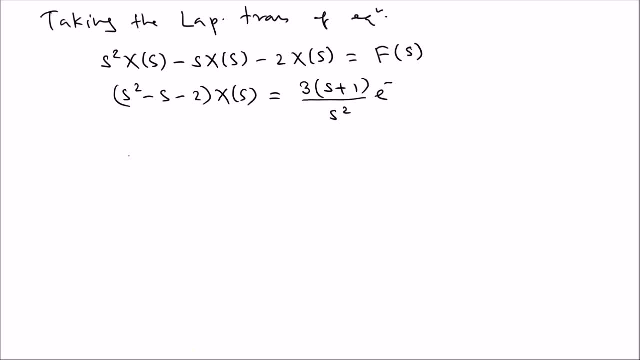 e to the minus s um. so what are the factors of this? s minus 2 and s plus 1. so that means, when you divide, s plus 1 get cancelled. so so you simply get s x. s plus 1 get cancels, you get 3 over. 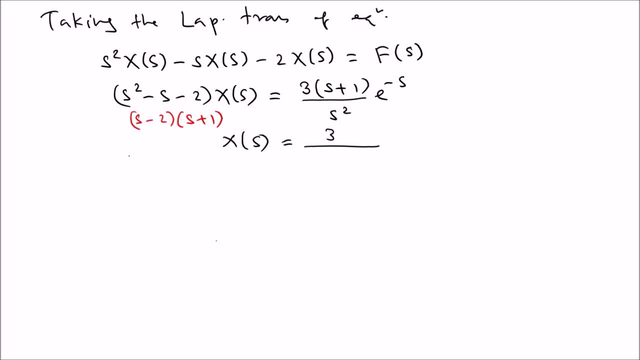 s squared s minus 2, e to the minus s. so if you have e to the minus x, what we normally do is first try to find the laplace, transform the rest of the function and then do the, then use the shift, second, shifting theta onto our transform. so that's what we. 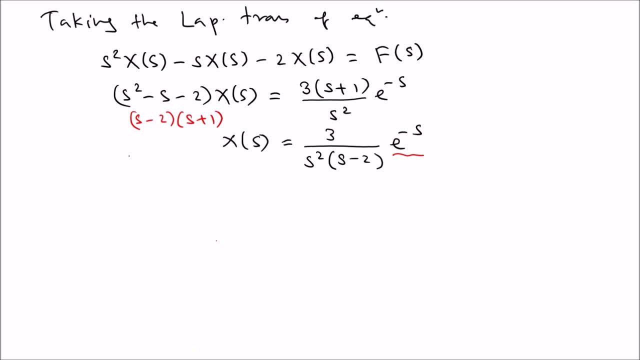 normally do so. to find the uh inverse laplace transform. let's use a convolution now. uh, so we do the inverse laplace transform. let's use a convolution now. let's see, we need the inverse laplace transform of 3 over s squared s minus 2.. 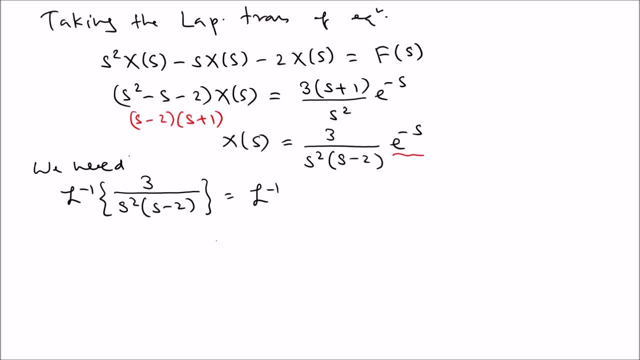 uh, so this is l inverse. we're gonna break this: 3 over s squared times 1 over s minus 2. so this simply says that it is 3 t convolute with e to the 2 t. so to get now we can use the definition. 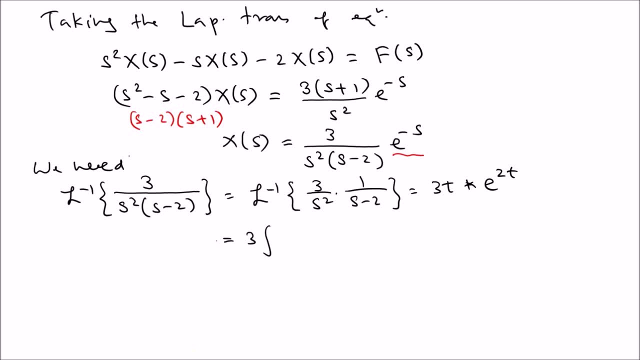 so three times, uh, when you have exponential function, that's where you're going to put the t. so it is 0 t minus tau, so it is tau e to the 2 t minus tau d tau. so we did this a lot, so, uh, now we know what to do with this. 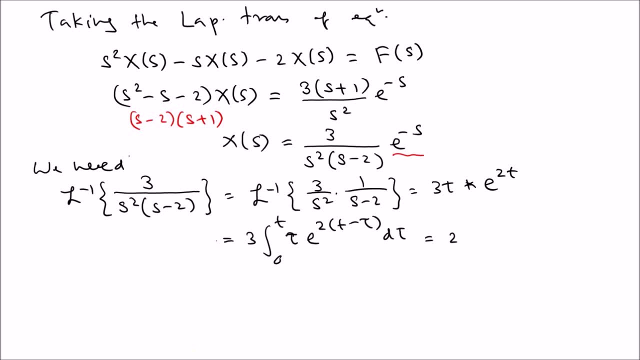 uh, so it is 3 e, 2 t. we take it out: 0, 2 t, tau e, negative 2 tau, d tau. so that's what you get, ah, and then we can integrate this one using the di method again. so so we have tau e to the negative 2 tau, so 1: 0. 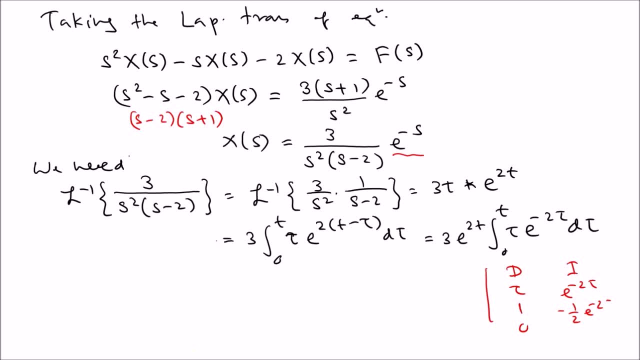 1 half e to the negative 2 tau, and then we need one more, so it is one fourth e to the negative 2 tau. we multiply these two and multiply those two plus and a minus. so now we can write the answer here. so this is simply going to be: 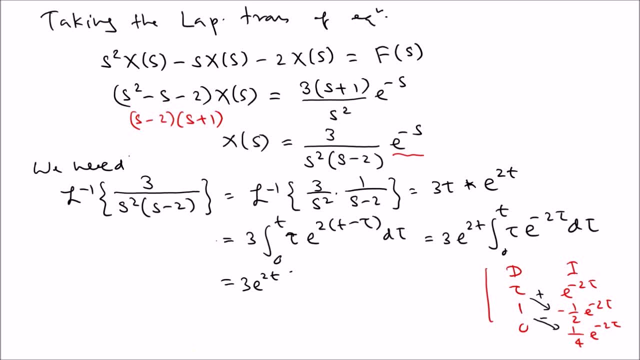 3 e to the 2 t times. let's write the first product, so it is one half tau. e to the negative two tau. next one is one half a negative one. fourth e to the negative two time. and then you're gonna go with t and 0. 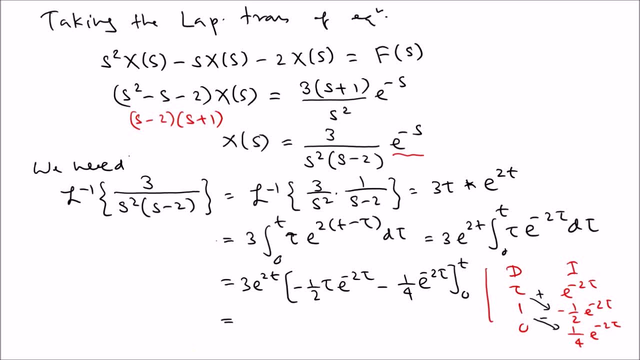 so if you plug in the two, you're gonna know that it's going to be 1 half 1. uh. so what happened is: so you have 3 e 2 t, let's plug in t so you get one half t e negative 2 t, and then, when you plug, 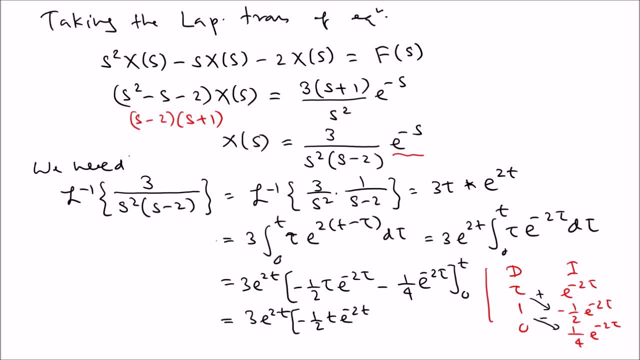 in 0 is gone and from the other one, when you plug in t you get one fourth e to the negative, 2 t and plug in 0 is positive 1, 4. so that's what you get and multiply through so you're going to get. you multiply by: 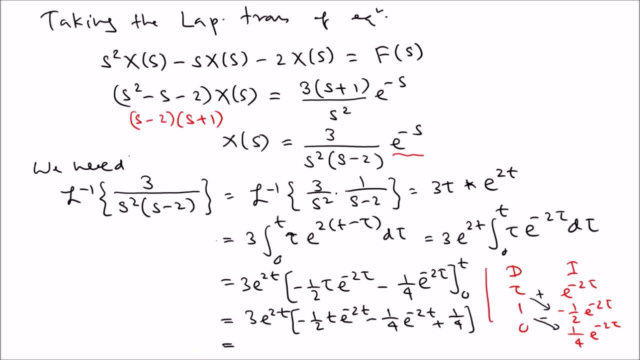 that. so 2 t get cancelled because the negative sign- so you get the first one- is negative 3 halves t, next one is uh 3, 4 and the next one is plus 3, 4, plus 3, 4, uh e to the 2t. so that is what you get as the uh. 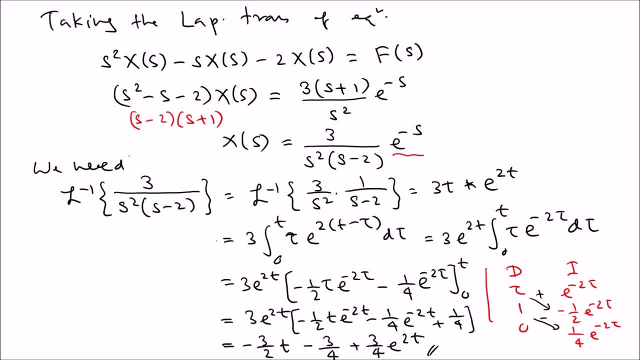 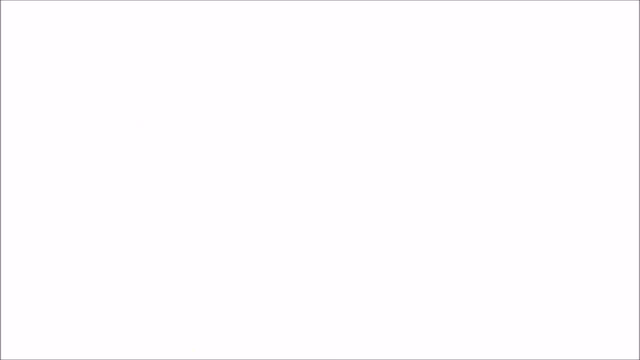 inverse laplace transform. not now. what you want to do is you're going to use the second shifting theorem, uh, to shift. okay, so by the second shifting theorem. so by the second shifting theorem. now we have x, t, which is the l inverse of 3 over. 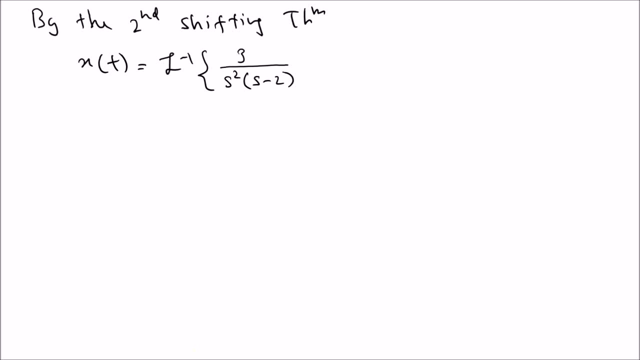 s, squared s minus 2, e to the negative, e to the negative s. so that means you're going to shift by negative 1. so that means everything would be. so we get the function first. so this is the function. so we're going to go with the. 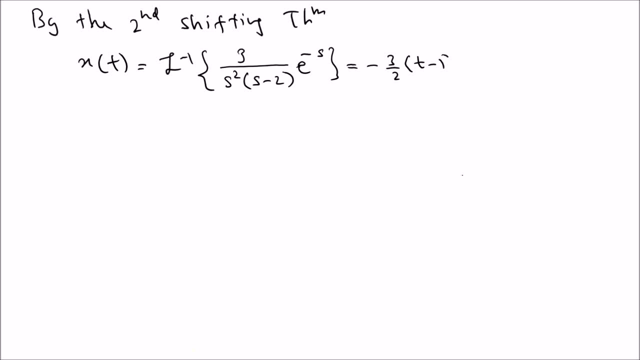 function. you replace t with t minus 1, negative 3, 4. there are no t here- and then 3: 4. we have e to t minus 1 and then everything multiplied by the heaviside function u, t minus 1. so that is the final answer for that problem. 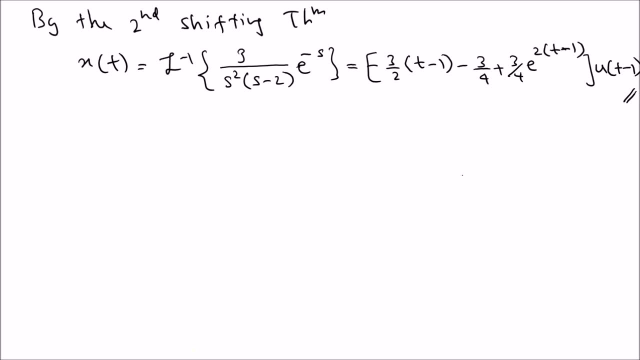 yeah, to get the same answer. you can also use the uh partial fraction method as well. okay, so you may use. you may also use the partial fraction method. good, so now let's try to go to the last topic of laplace transform that we are talking about, the direct delta function. 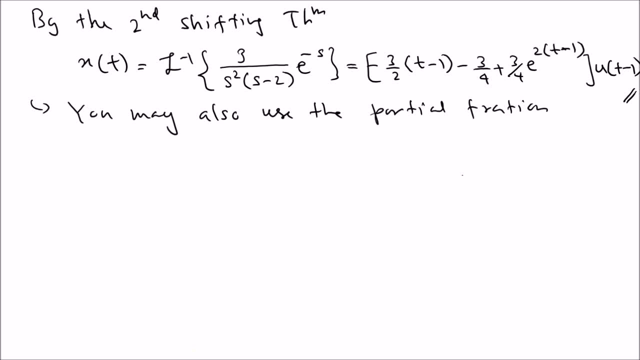 so let's talk about that. uh, so the direct delta function, impeller response, so the direct direct delta function, direct data function and impulse response. impulse, uh, response. um, so let's talk about what's the related function, or there's the impulse, so, like you know, the sudden force, uh, acting like a. 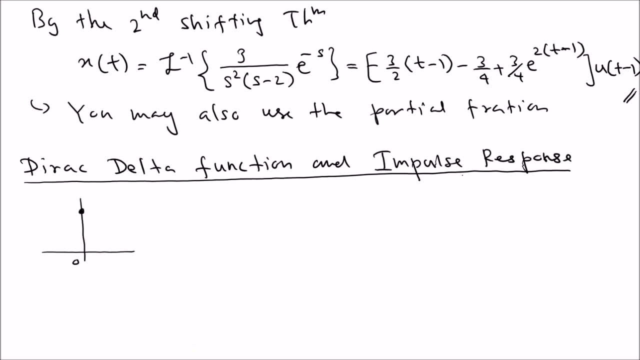 at a single point. that's the kind of idea. so uh, we can write this one as delta t, so like a, uh, so it is acting at the zero points, which is called delta t and then uh. so the shifted version is uh at a, that's impulse at a, so that's it, and then everywhere else it's here. so 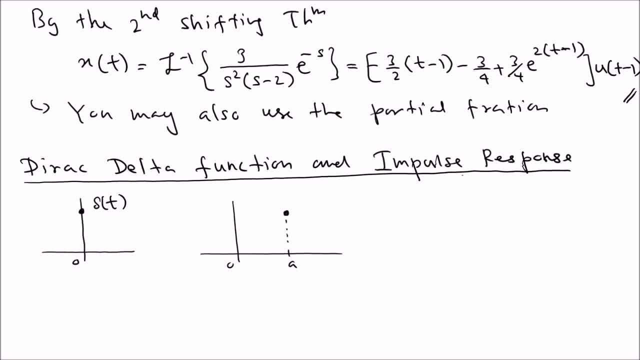 this is what we normally write as delta t minus a impulse at a, and then we have the laplace transform of that. so the laplace term, the first one, is delta t, that is, 1, and then the laplace transform of the shifted version, delta t. 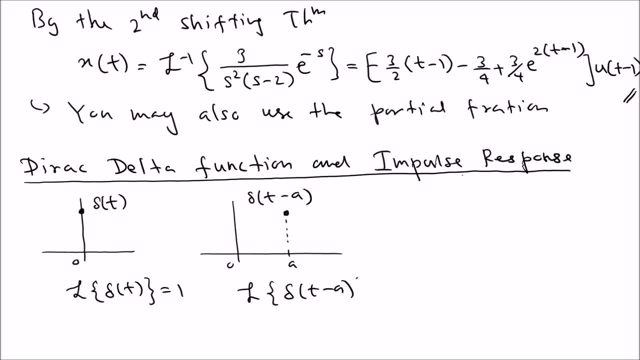 minus a, which is e minus a s. so this is useful, uh, to remember. and if you plug in a equals zero, uh, you get the other one. good, i mean, that's it. so let's try to see how we can use this to find the inverse laplace transform. so let's do a problem like this. 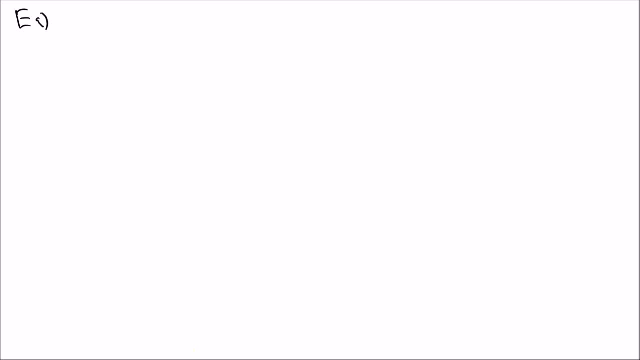 okay, find the inverse laplace transform of uh. so let's say, find the inverse plus transform of the first one, l inverse s plus 3, or the first one 3 over s plus 1, and you can see that this is not a proper uh. this is not the proper fraction. so if you have proper, improper this. 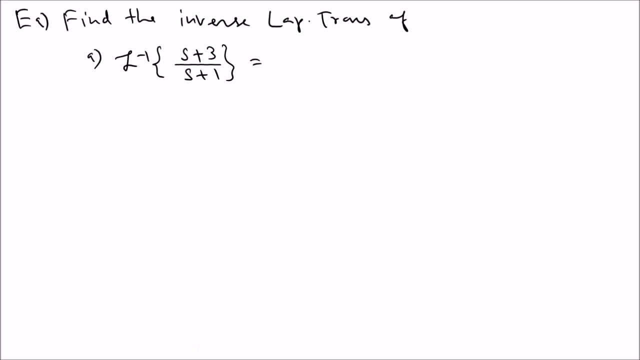 is what you call improper fraction. what you can do is you can do the lone division and find the remainder and the quotient. that you can do. also, you can use some kind of tricks here, so that's much faster. so what we're going to do? we try to create the bottom. 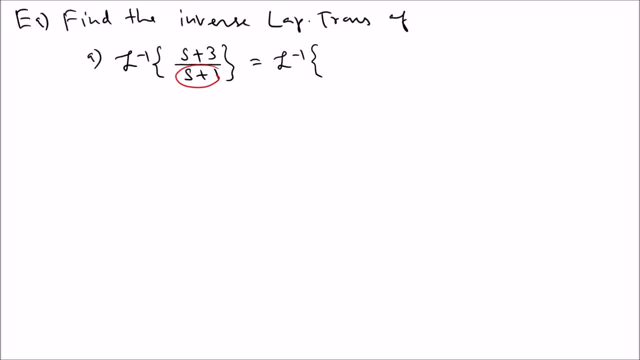 term in the top. that's the. that's argument, so we're going to do that. that's the argument. that's the argument we are doing here. here, that's aani. we can write this one as s uh. we can write this one as s plus one. 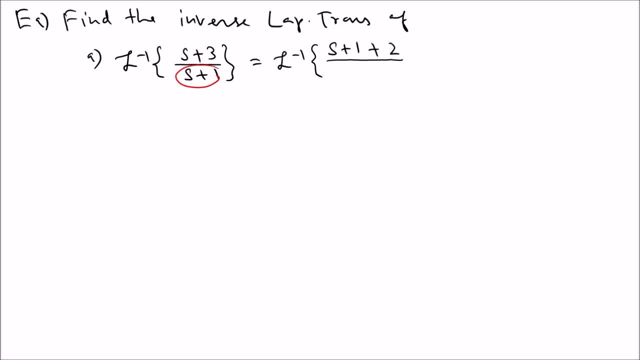 plus two over s plus one. then we can write with this and with the other one, so we're gonna, we're gonna separate this now, so we can write this one as ah, so l inverse s plus one over s plus one, plus two over s plus one. so that means this is simply l inverse. 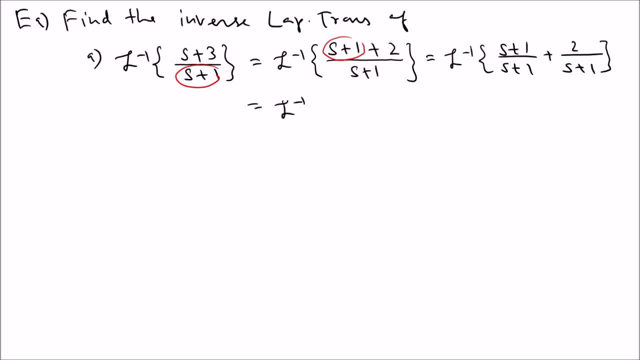 1 plus 2 over s plus 1.. we know that the one that means the delta function, this is delta 1. uh, it's a delta t, that's one, so we can write this one as s plus one plus two over s plus one. 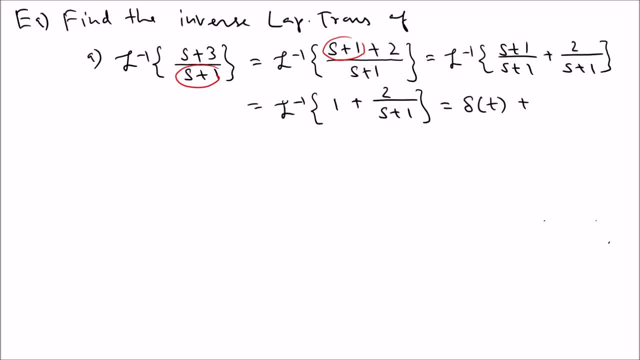 plus uh, 2 over s. 2 over s plus 1 means e to the e to the negative 1 t, because a equal 1 in this case is 2, e to the negative t. so the certificate. so that's how we find inverse when you have a improper uh fraction like that. 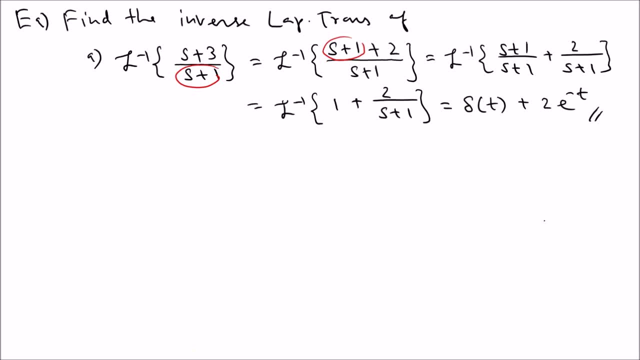 so we. so the delta function comes into play in this case. so let's just do one uh problem, also another problem like that. so how about this one, l inverse? so let's say, uh s doesn't look, uh s e to the minus 2 s plus. 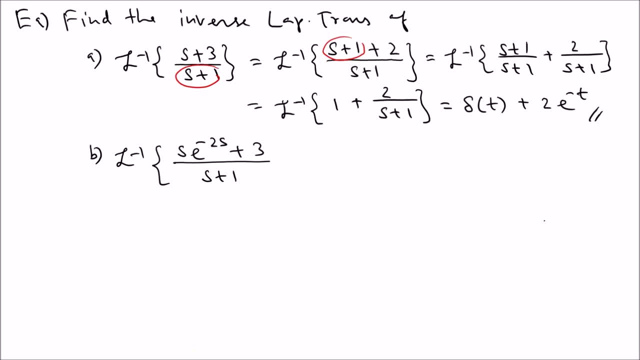 3 over s plus 1.. um, so what we can do with this again, we can split this, so this one we can write as l inverse, so you can see we have s here. so we can do the same idea. so we can write this one as we try to create the denominator, so it's plus 1. 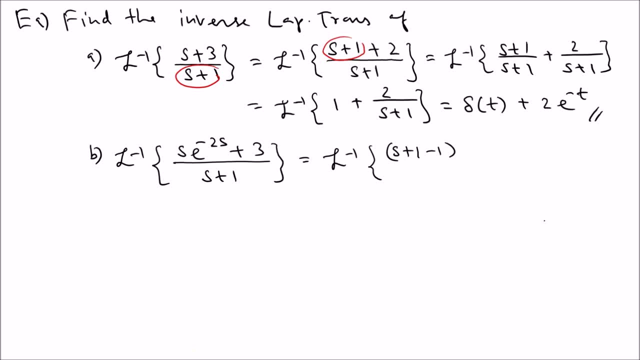 minus 1.. uh, e to the minus 2, s plus 3, ah, so this is over s plus 1, over s plus 1. you can write it like that. now the same trick, so you can go with s plus 1.. so it's. 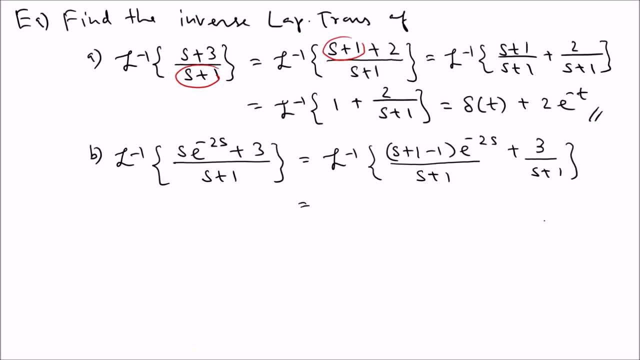 with the bottom term. so that means we can write this one as: uh, if you go s plus 1, you simply get e to the minus 2 s. if you go with minus sign, you get minus 1 over s plus 1, e to the minus 2 s, and then we have this: 3 s plus 1. 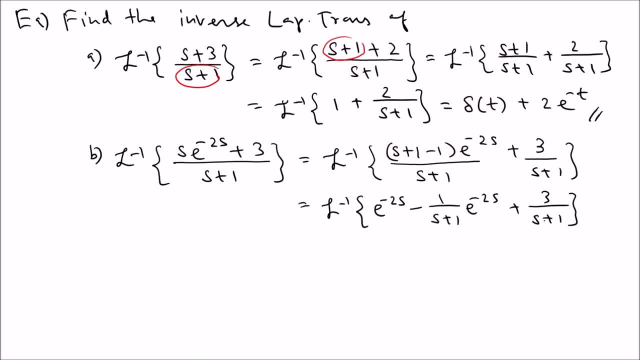 2. now we get term by term. so the first one is simply delta t minus 2, where a is in this case 2, so is the t minus 2. the next one is: so we had to use the heaviside function for this one. we find it, and then we can. 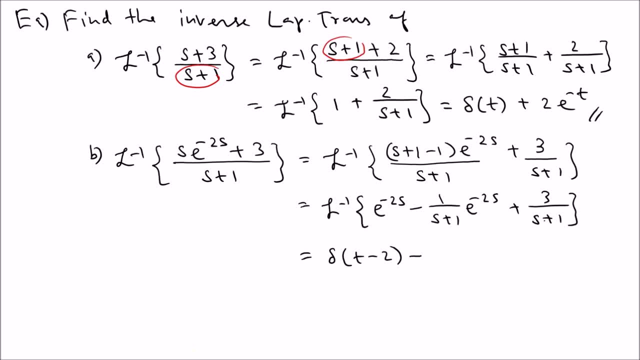 transform that you can see how to. the function is is 1, 0 s plus 1. s plus 1. that means e to the minus t. you replace t by t minus 2. so so it is e to the minus t. you replace uh t by t minus 2. 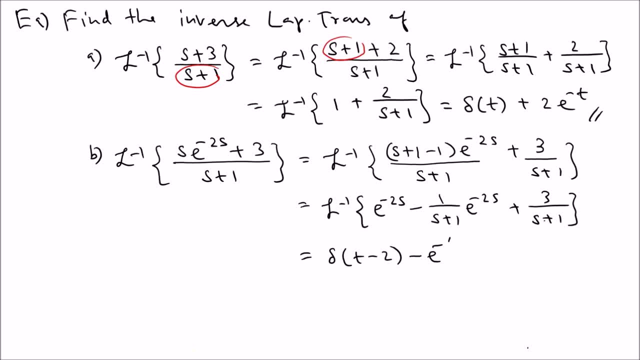 so replace t by t minus 2, multiply by u- t minus 2. that's that, and the next one is simply 3 e minus t. so that's the kind of idea. ah, so this is how we can do it. when you have a term like 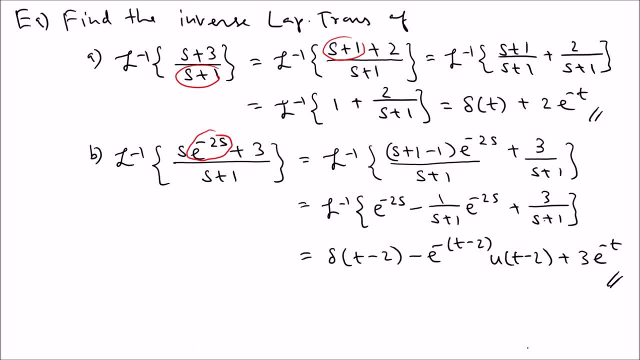 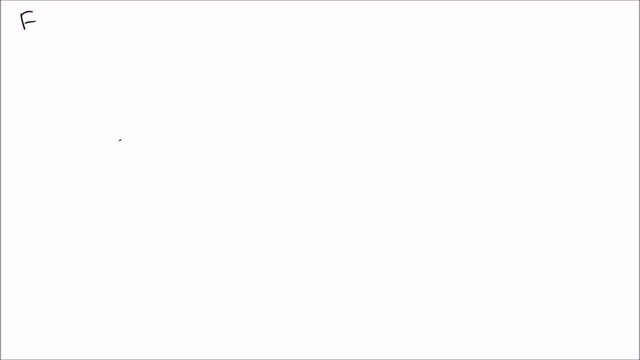 this. this is special case. so you, uh, you either get this or you either get that, so it's gonna come with one of those. good, now let's try to solve uh one problem, uh, using this method. that's the end of uh laplace transform techniques. let's just do one example, uh so find. 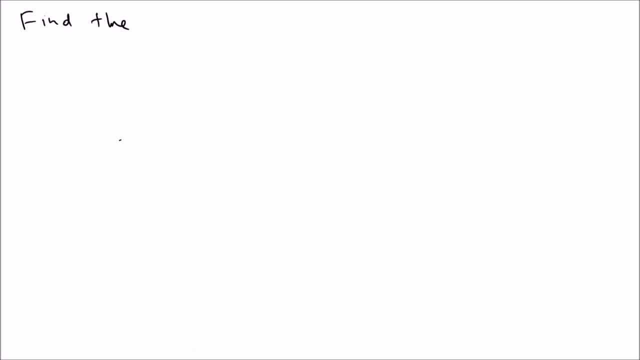 find the impulse response. find the impulse response. find the impulse response of a system. okay, so, for example, let's say: so this is the question. so i'm going to give the exact same wording: find the impulse response. or simply say: solve the differential equation, find the impulse response. 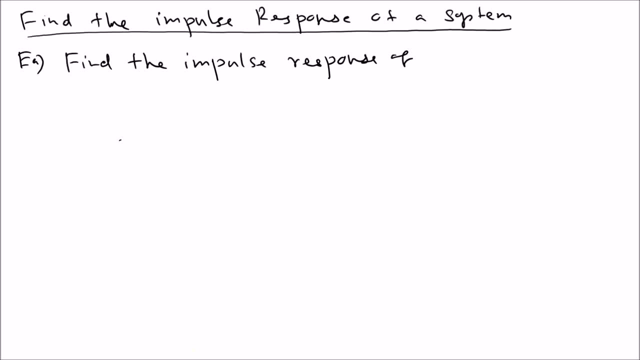 of ah, this one, x double prime minus t. t is the impulse response of a system. okay, x prime minus x equal, let's say 4 delta t minus 3, something like that. okay, so where this is coming from. and also with x: 0 equals 0 and x prime 0 equals 0, just to make things easy. 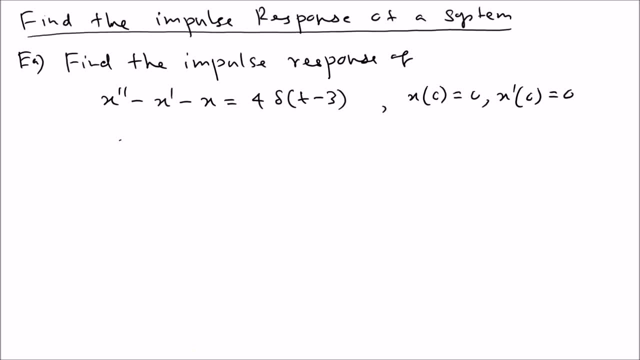 so where are these difference equations coming from? so this is the kind of situation. let's say you have a mass on a table, uh, which connected to a spring, with the friction uh stable. now what we're going to do? you're going to give a sudden impulse. 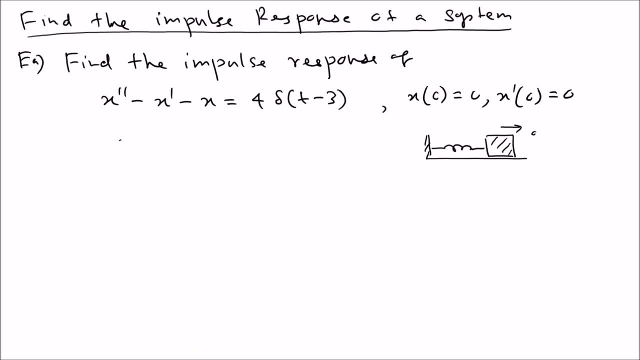 to one direction. at the time t equal 3, so you wait and just give a sudden uh force in one direction. so that's the kind of situation. so now you get a difference equation like that, uh, so let's try to solve and see what's going to happen, so what we normally do. so just the same. 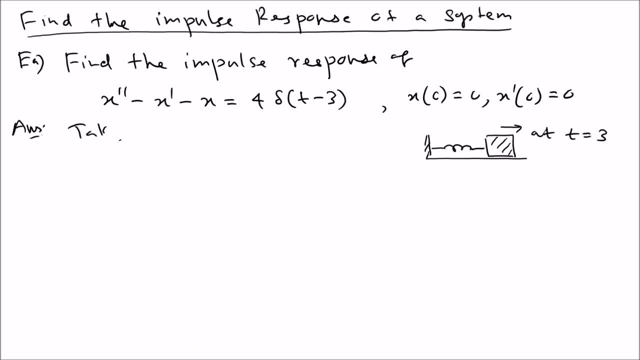 procedure: take the uh uh laplace transform. take the laplace transform so you get s squared: uh s x plus s, x s minus x s, equal. okay, let's write the laplace transfer of that. we know that just the e minus, whatever the number, is 3. 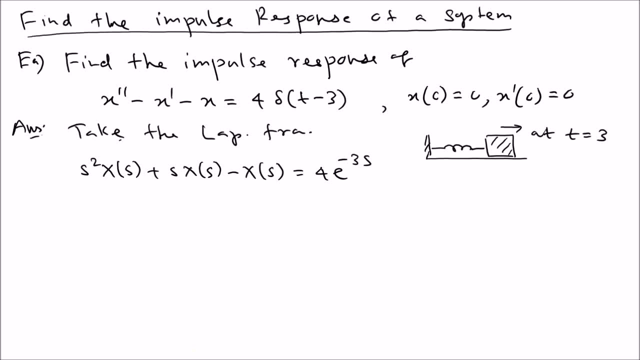 s. very simple, uh, initial condition is 0, so you don't get that. so here we have s squared, and then a number of s plus s is equal to s. yeah, this is minus s squared, minus s, minus one times s. x equal 4 e negative 3 s. 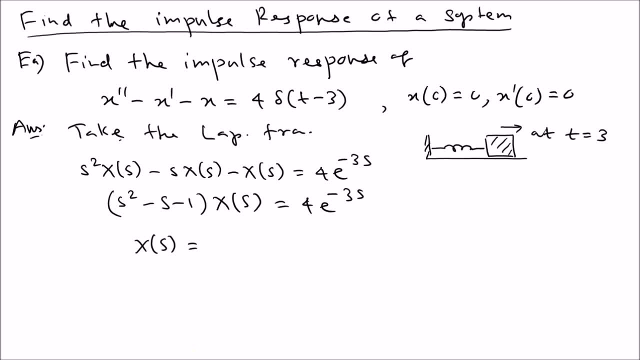 so a 6 equal 4 e minus 3 s over s squared minus x minus 1. and you know that. you can see that there are no factors for the bottom function. so what we can do, we're going to go with the completing square technique. uh, so let's do that. so it is 4 e minus. 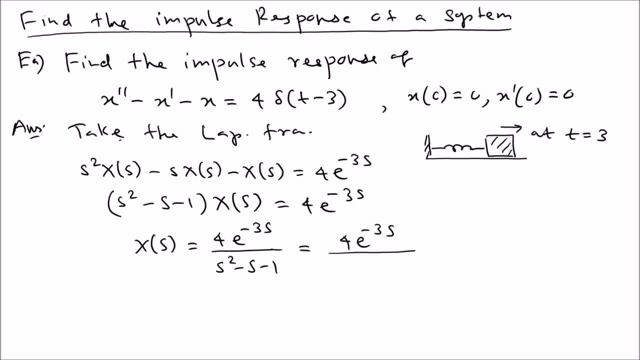 3 s. what's the completing square here? so it is s half of the s term. half of the collision is termed that in one half. we can square that. so it's going to give you the first term of the s squared term. so that means you add, subtract 1, 4. so if you subtract 1, 4, this can be. 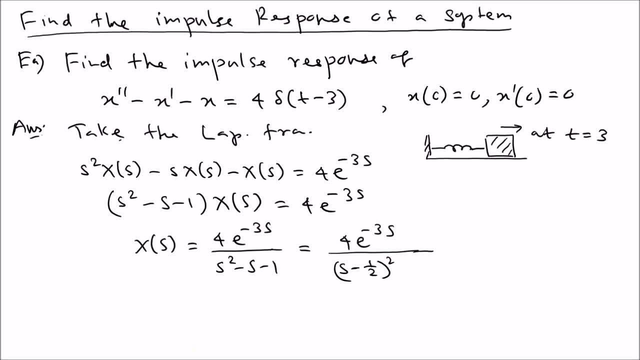 5, 4.. so that's what you get now: uh, this is uh, you can see this, you can invert uh, so. so what's going to happen now is uh, actually, uh. i'm not going to show you how to do that, but i'm going to show you how to do that. so. 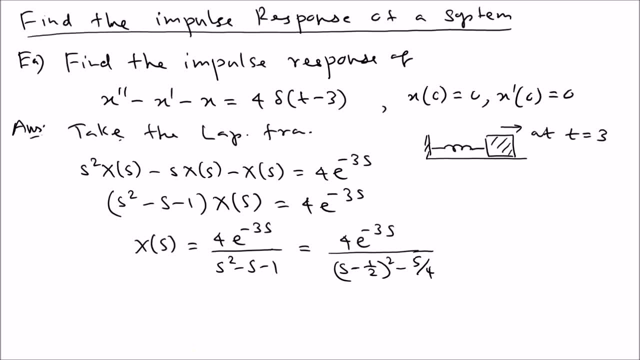 actually, uh, i'm going to change this uh to that number. so it's a change just to plus, plus, plus and a plus and a plus. so it's simply change to that, change plus. i just make things easy. uh, i don't want to make it too complicated, it's already complicated. 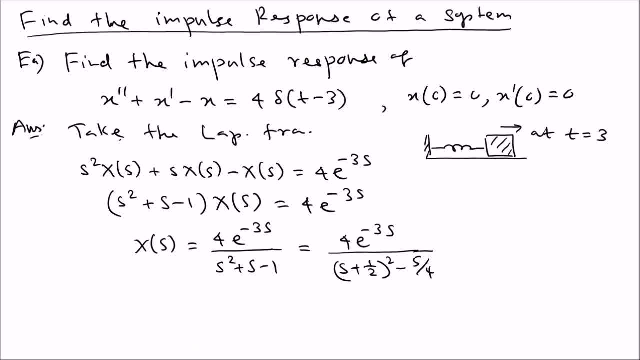 so now, what we can do, uh, we're going to kind of uh clear the terms. so you can see, this is one plus one s plus half squared minus. so what is this? is a shin function. this is shin. uh, we know that there's a form of a hyperbolic sign. 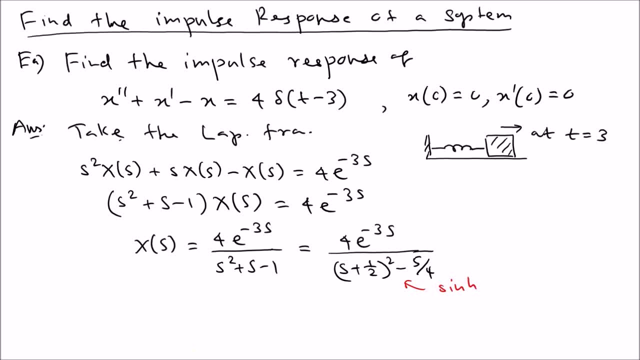 uh. so what is missing is square root 5 over 2. so we're going to uh, multiply and by and divide by that, so it's a 4. so we are missing square root 5 over 2.. so we're gonna divide and multiply. 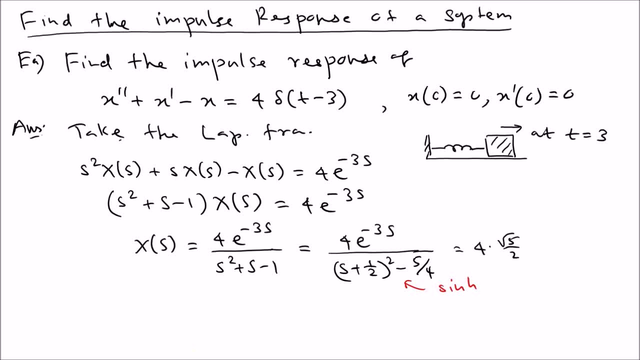 uh, good, so yeah, i didn't write it properly. so what we're going to do? ah, so we can write this one as s plus 1, half squared minus 5, 4.. so square root 5 over 2 is missing, and then we multiply outside. 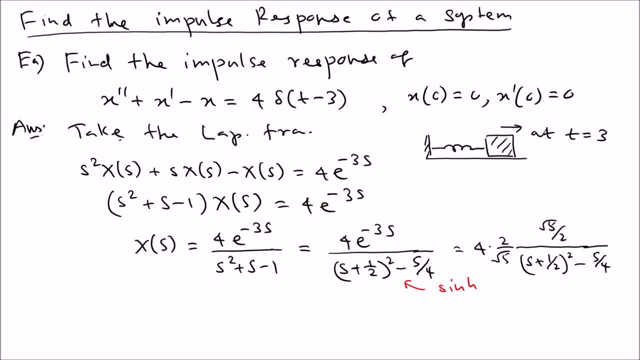 upside down of that. that's what we do. and then we have also e to the minus 3 s term. so this is simply the uh hyperbolic sign part. so that means the final answer. so we can see. so. so this simply gonna occur. this simply corresponds to. 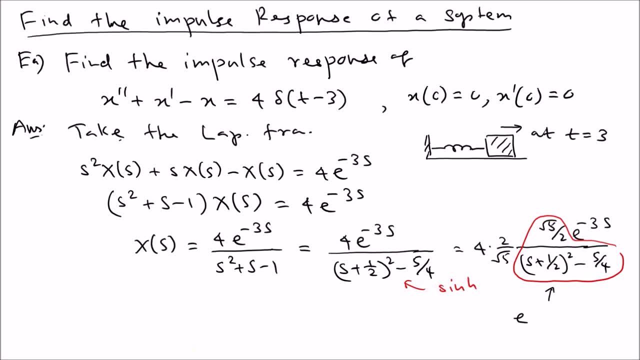 e to the negative one, half t, sin square root 5 over 2 t. so that's the function coming from there that you know already now what we can do. we can use the e to the minus 3s to add a switch here. so taking inverse laplace transform taking. 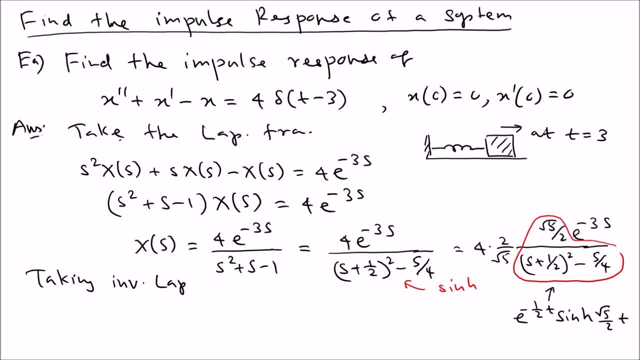 inverse laplace. so what we have is x t equal 2 square root, 5. u t minus 3, u t minus 3 e to the minus one half t. so what we're going to do, what's going to happen? you have to shift by u t minus 3. 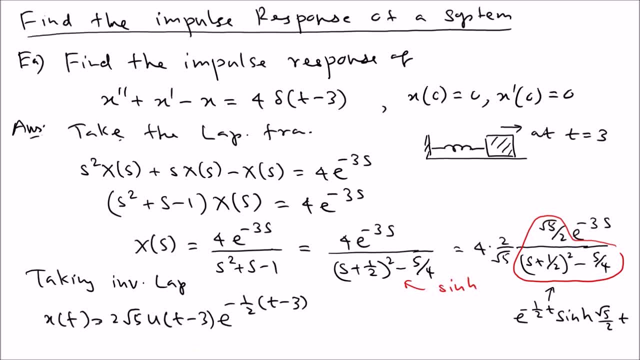 minus 3. so t minus 3 comes there, and then sin square root 5 over 2. this one also t minus 3. this is because of the e term, this coming from the e term. good, so that is the answer for uh, this problem. so you can see that there is suddenly start at uh after three. then that's when. 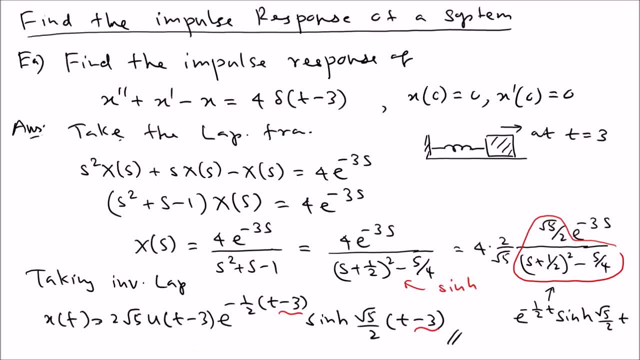 the impulse. so i mean, you can see this, there's the whole problem. so this is like kind of simple problem compared to other problems. okay, good, so that is the end of laplace transform method. next we're gonna do, uh, we're gonna learn how to solve systems so we can talk. 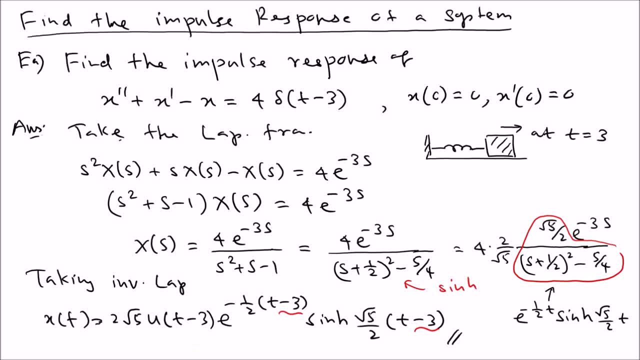 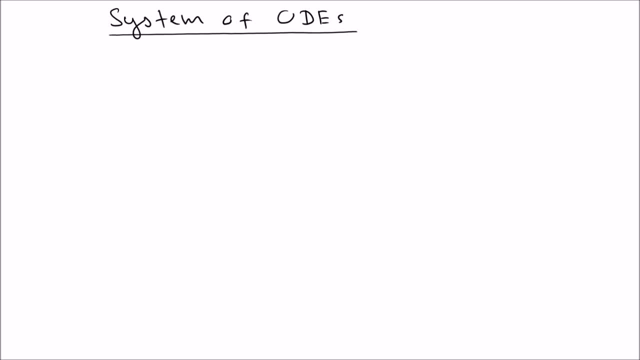 about some examples there in this. uh, we're gonna uh talk about, uh, how to solve system of equations, system of ods in this case. so we're going to talk about, uh, how to solve system of equations, system of ods in this case. so we can talk about three methods. the first one is the 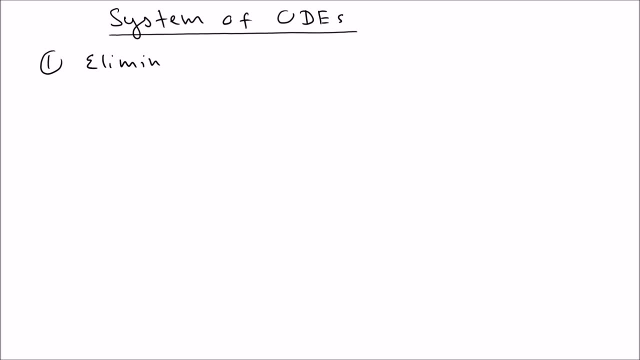 elimination method, elimination method. so there are two type of problems that we can try. so there are two types. we're going to go one by one. and then the next one is the laplace transform method. laplace transform- our method. so this is actually uh, kind of. 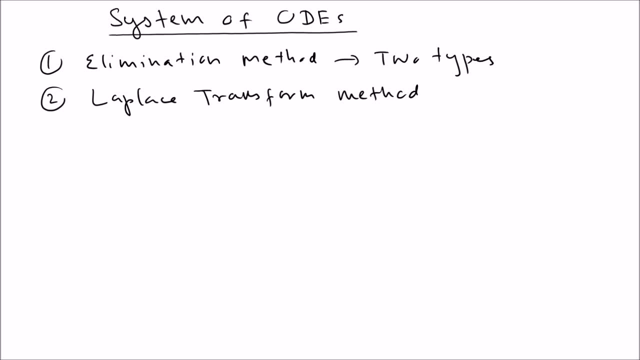 um, sophisticated, because you can do, you can handle a lot of cases with that. and then the third one is the eigenvector method. eigenvector method: so under the eigenvector method we're going to consider two cases. we can do two by two. uh, two by two case is very easy, so we're going to do two by two. 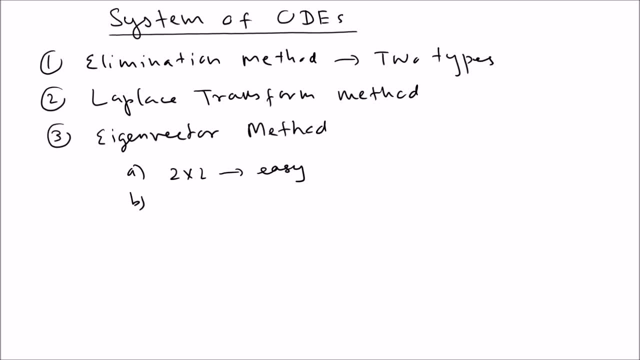 so we're going to do two by two- case is very easy. and then we can do three by three, we can. and then we can do three by three, we can, and then we can do three by three. we can do three by three, do three by three. there are actually three cases to. 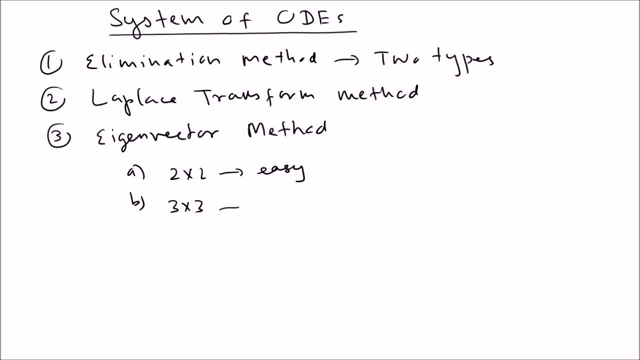 do three by three. there are actually three cases to do three by three. there are actually three cases to consider, consider. consider, um one is there are two eigenvalue case. uh, that's kind of easy, uh, very easy to. uh, that's kind of easy, uh, very easy to. 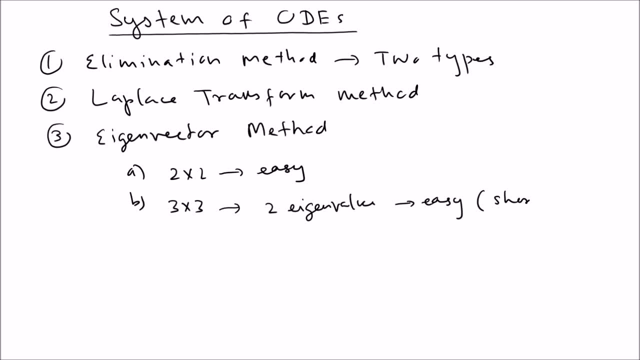 uh, that's kind of easy, uh, very easy to find eigenvectors. we can use shortcut: find eigenvectors. we can use shortcut: find eigenvectors. we can use shortcut for that, for that, for that. so we will use the shortcut and then: uh, so we will use the shortcut and then uh. 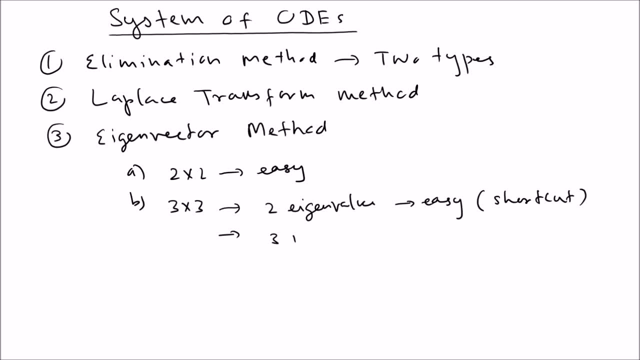 so we will use the shortcut and then, uh, there are, uh, there are, uh, there are, uh, three eigenvalues, three eigenvalues, in that case, what we normally do, we use in that case what we normally do. we use in that case what we normally do, we use the eigen matrices for that. 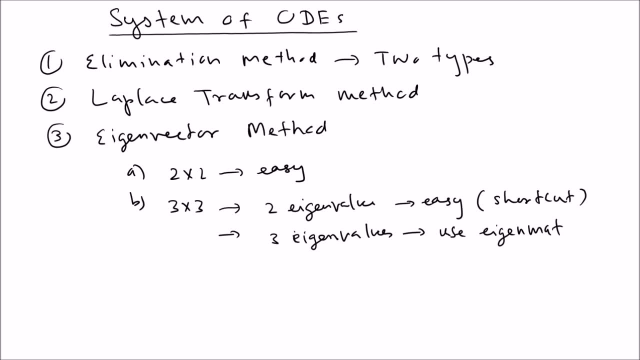 the eigen matrices for that, the eigen matrices for that. eigen matrices, that's the new concept. uh, we discussed, that's the new concept. uh, we discussed, that's the new concept. uh, we discussed that earlier in a different that earlier in a different, that earlier in a different video. so you can look at that and 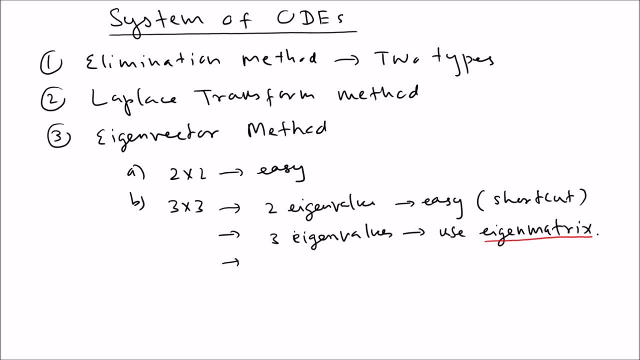 video so you can look at that, and video so you can look at that. and then, uh, there's a case also. uh, then, uh, there's a case also. uh then, uh, there's a case also. uh, what we call defective matrices and we, what we call defective matrices, and we. 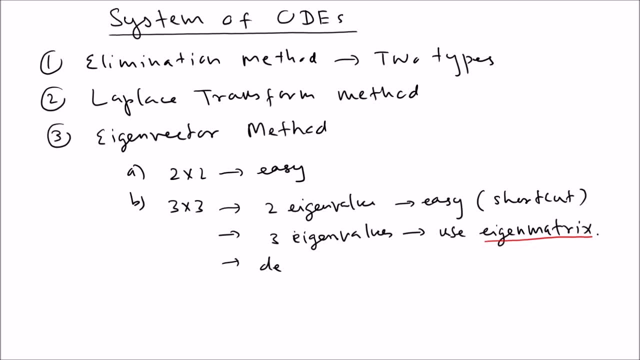 what we call defective matrices, and we are not going to discuss that in this, are not going to discuss that in this, are not going to discuss that in this, but we have that in the but, we have that in the but, we have that in the in another video. so the defective 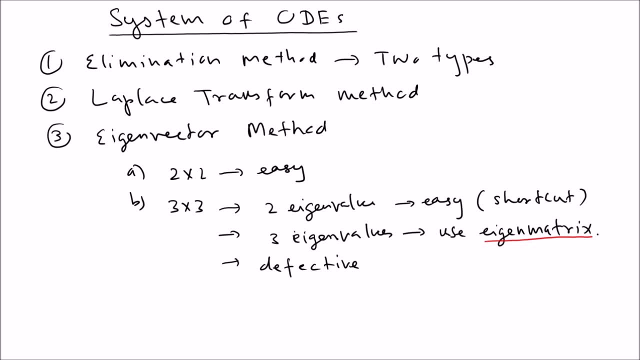 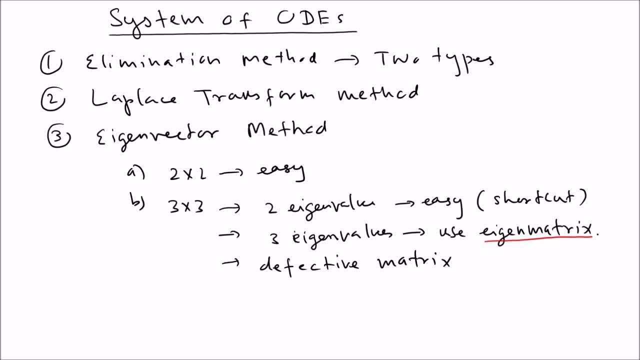 gonna discuss one from two by two, and gonna discuss one from two by two and one from three by three. uh with two eigenvalues. so that's what? uh with two eigenvalues. so that's what? uh with two eigenvalues. so that's what we're gonna do. 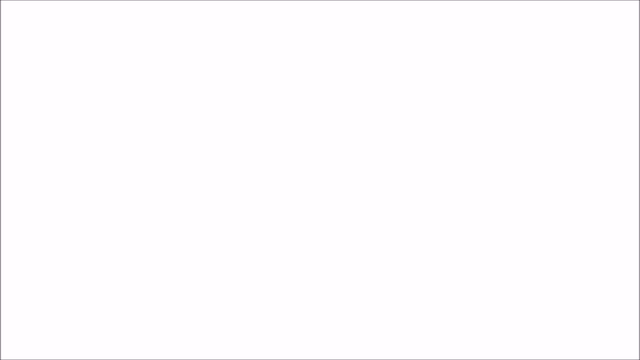 we're gonna do, we're gonna do. okay, so let's start one by one. okay, so let's start one by one. okay, so let's start one by one. now let's do the elimination first. so now, let's do the elimination first. so now let's do the elimination first. so the elimination method. 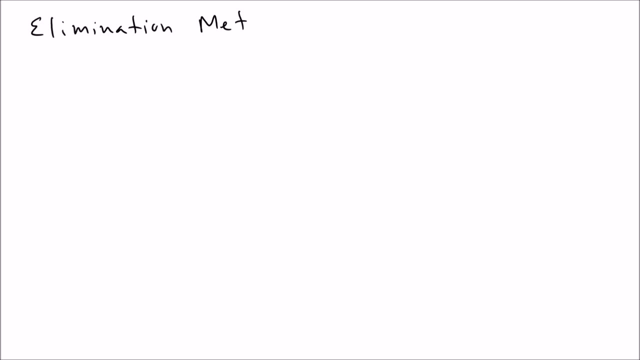 elimination method. elimination method: uh, so there are two types, so let's start. uh, so there are two types, so let's start. uh, so there are two types, so let's start with type, with type, with type one. uh, so let's do that with the problem. uh, so let's do that with the problem. 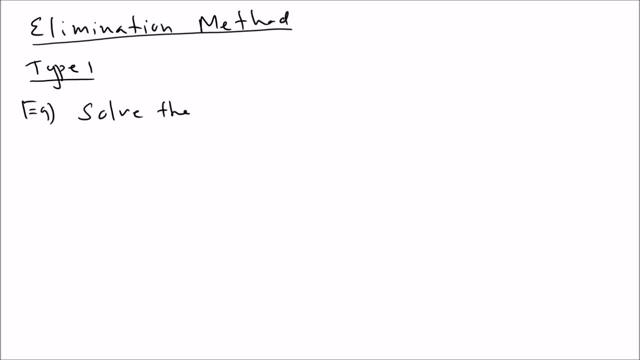 uh. so let's do that with the problem. so let's say so. let's say so. let's say solve, solve, solve, solve, solve the system, solve the system. so let's say 3 dx. so let's say 3 dx. so let's say 3 dx over dt. 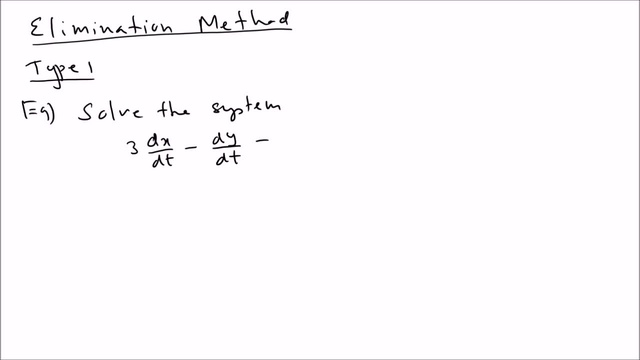 over dt, over dt minus dy, over dt minus dy, over dt minus dy over dt, and on the other side you can see some and on the other side you can see some and on the other side you can see some. function of the independent variable, function of the independent variable. 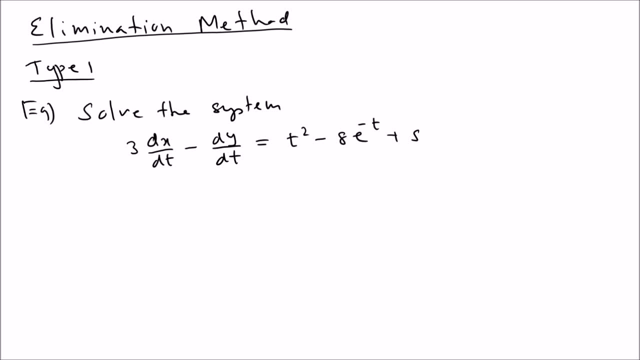 function of the independent variable. so let's say, just put something. so let's say, just put something. so let's say just put something, uh, so like. let's say sine t. uh, so like let's say sine t, uh, so like let's say sine t. and then we have another one: dx over d. 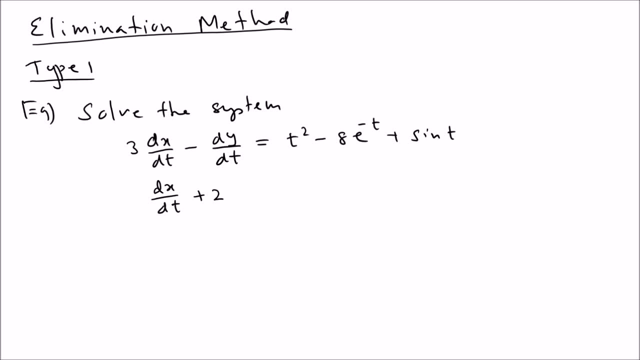 and then we have another one dx over d, and then we have another one dx over d, t, t. t plus 2 times d? y over d, plus 2 times d? y over d, plus 2 times d? y over d, t, which is equals to t, which is equals to: 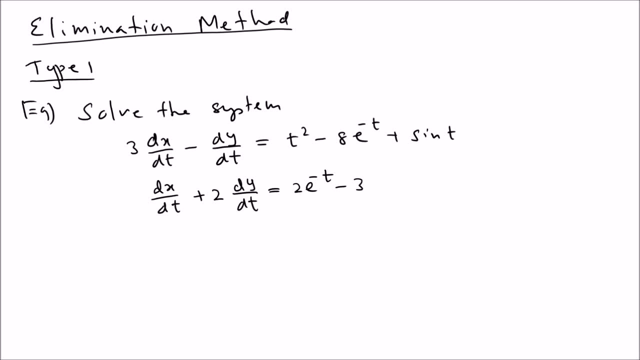 t, which is equals to 2 e minus t, 2 e minus t, 2 e minus t minus 3. minus 3 minus 3. let's say cosine 3 t plus 1. let's say cosine 3 t plus 1. let's say cosine 3 t plus 1. so what we can do, we're going to call. 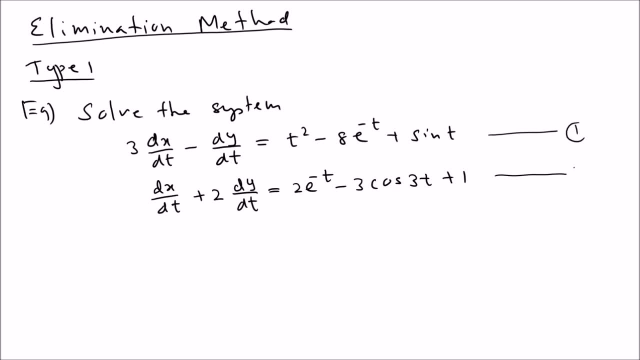 so what we can do, we're going to call. so what we can do, we're going to call this equation 1, this equation 1, this equation 1 and equation 2 for references and equation 2 for references and equation 2 for references. uh, 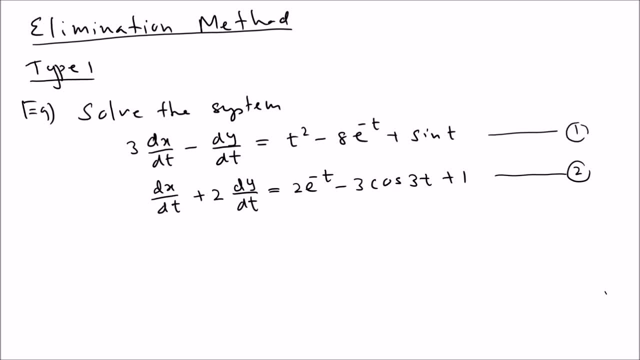 uh, uh. so this is like just uh like how we do so. this is like just uh like how we do so. this is like just uh like how we do this, like as like when we solve linear this. like as like when we solve linear this, like as like when we solve linear systems. 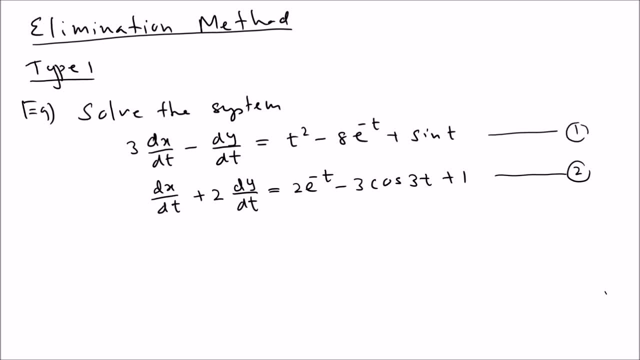 systems systems, uh like when you have like a with, uh like when you have like a with, uh like when you have like a with several variables. if you see like linear several variables, if you see like linear several variables, if you see like linear systems, systems, systems. we know how to do. we can just 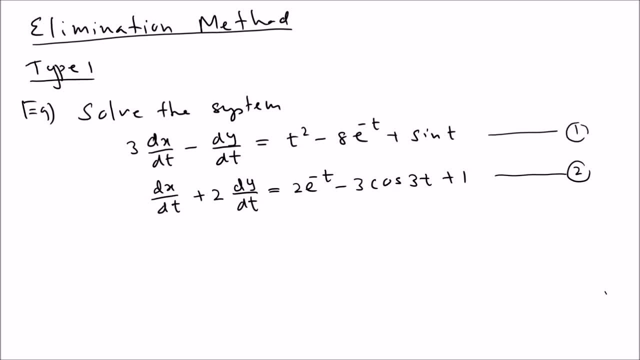 we know how to do. we can just we know how to do. we can just eliminate uh, eliminate uh, eliminate uh one variable, so we can use the same one variable, so we can use the same one variable, so we can use the same argument, for example, in this case, you: 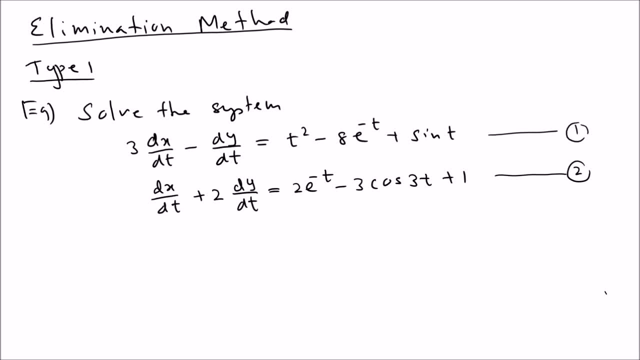 argument, for example, in this case. you argument, for example, in this case, you can see, can see, can see. uh, when you see plus and minus sign. uh, when you see plus and minus sign. uh, when you see plus and minus sign. that's the kind of we're going to. 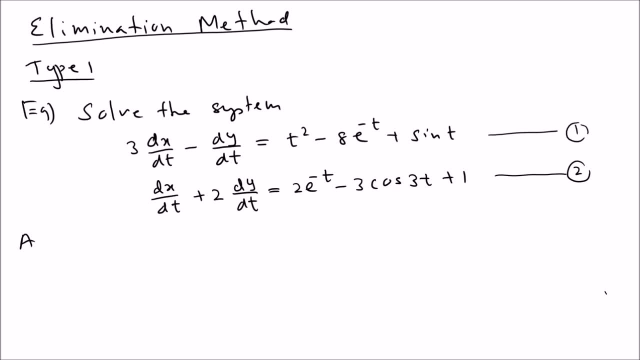 that's the kind of we're going to, that's the kind of we're going to pay attention to, because that's going to pay attention to, because that's going to pay attention to, because that's going to make it easy, make it easy, make it easy. so what we're trying to do is, uh, so in. 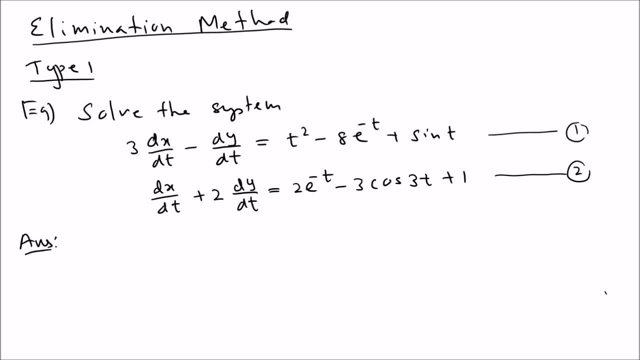 so what we're trying to do is, uh, so in. so what we're trying to do is, uh, so in theory, uh, what we do, eliminate theory, uh, what we do eliminate theory, uh, what we do: eliminate one of the x prime or y prime. so that's. 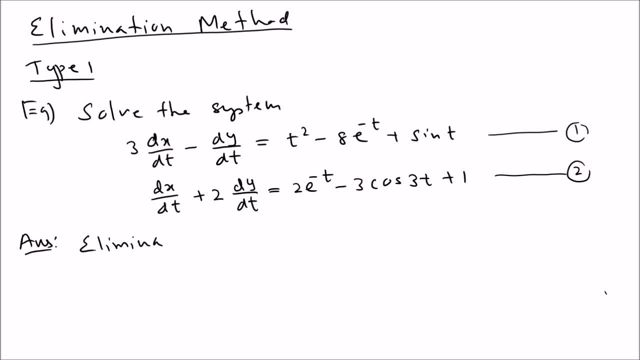 one of the x prime or y prime. so that's one of the x prime or y prime. so that's the kind of goal. so eliminate. eliminate one of x prime or y prime. uh, for example. uh, x prime or y prime. uh, for example. uh, x prime or y prime. uh, for example, uh. when you see plus minus sign, that's. when you see plus minus sign, that's when you see plus minus sign, that's we're going to pay attention to that, for we're going to pay attention to that, for we're going to pay attention to that, for example, if you multiply the first example, if you multiply the first, 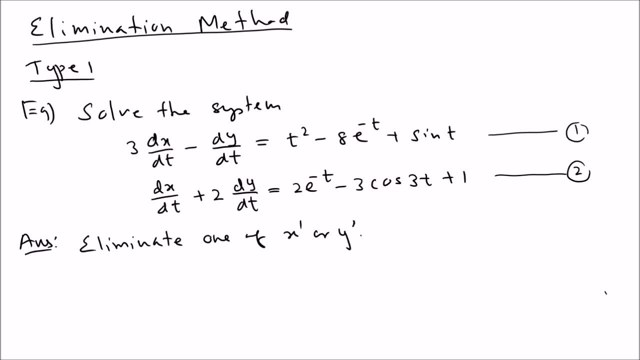 example, if you multiply the first equation by two, equation by two, equation by two, and add it to the second one, you can see. and add it to the second one, you can see. and add it to the second one, you can see the dy term, the dy term. 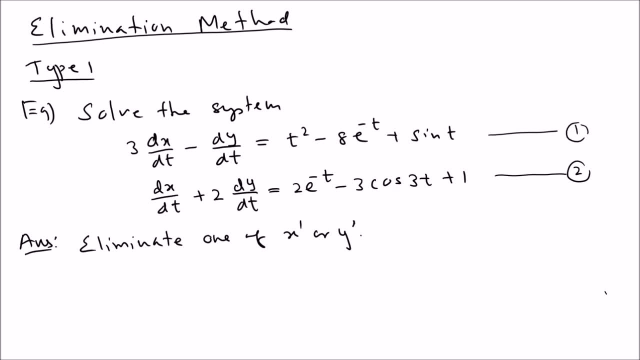 the dy term gonna go like: eliminate it. so that's what gonna go like eliminate it. so that's what gonna go like eliminate it. so that's what we're trying to do, we're trying to do, we're trying to do so. you can see by um two times. 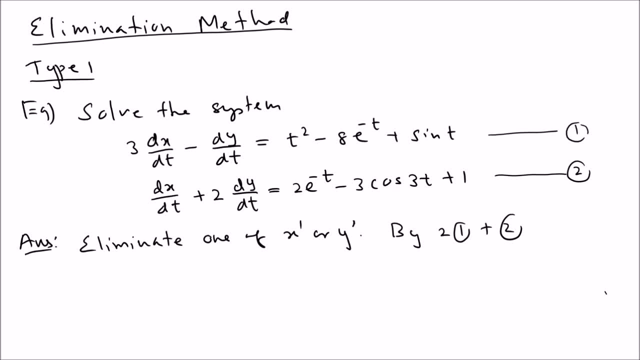 so you can see by um two times. so you can see by um two times the equation one plus two. if you do the equation one plus two, if you do the equation one plus two, if you do that, if you multiply the first equation by that, if you multiply the first equation by. 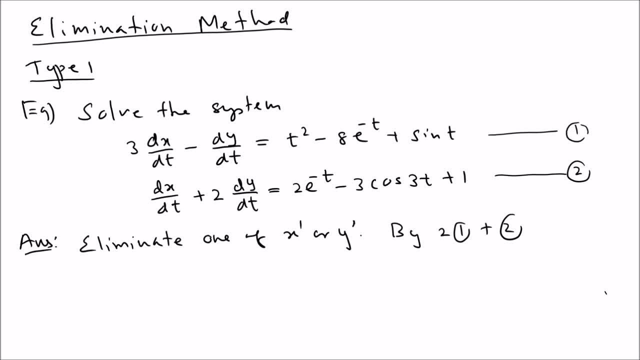 that if you multiply the first equation by two and add it to the second equation two and add it to the second equation two and add it to the second equation, you can see the y term get cancelled. so you can see the y term get cancelled. so you can see the y term get cancelled. so you're going to get. 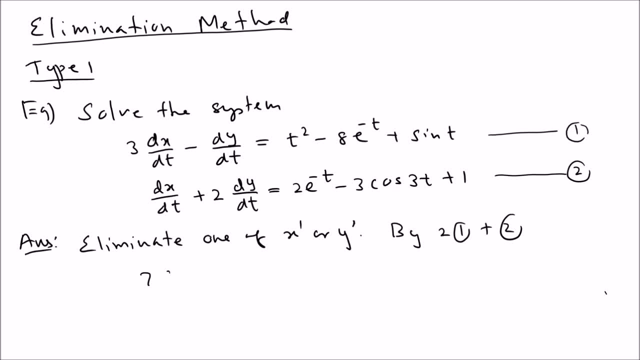 you're going to get. you're going to get two times three. that means six plus one. two times three, that means six plus one. two times three, that means six plus one. so you get seven dx over dt. so you get seven dx over dt. so you get seven dx over dt. uh, equal. so you multiply the first one. 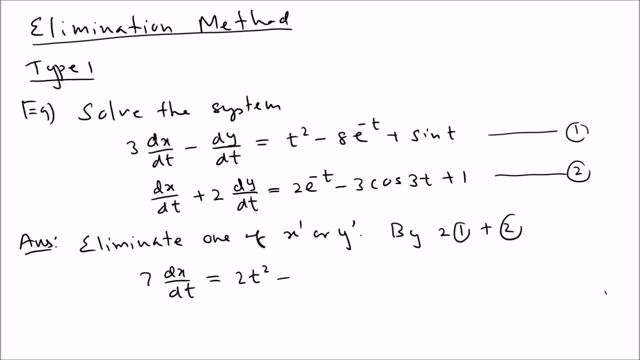 uh equal, so you multiply the first one. uh, equal, so you multiply the first one by two. so that means two t squared by two. so that means two t squared by two. so that means two t squared: uh, minus. okay, let's look at what's going. uh, minus, okay, let's look at what's going. 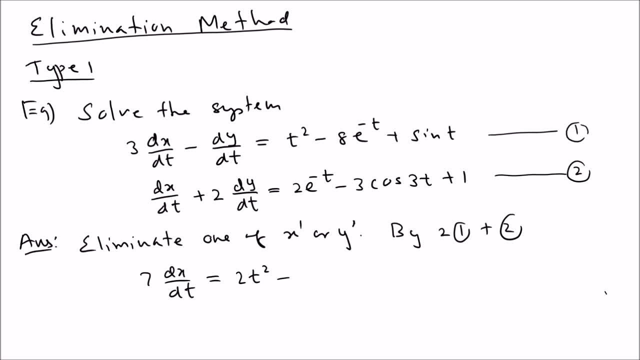 uh, minus. okay, let's look at what's going to happen here. so we're going to to happen here. so we're going to to happen here. so we're going to multiply this one by two, multiply this one by two, multiply this one by two, uh, so you get negative 16 and you add. 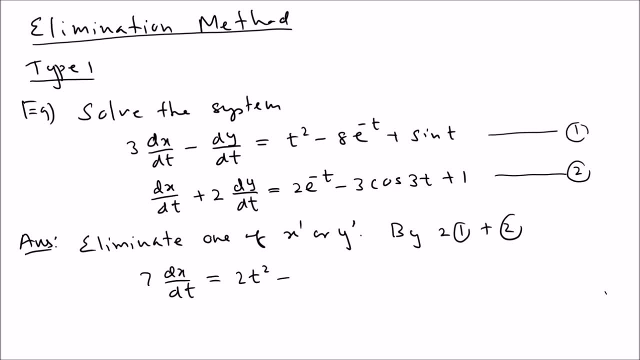 uh, so you get negative 16 and you add: uh, so you get negative 16 and you add: there are in the second equation, you, there are in the second equation, you, there are in the second equation. you also have two. that means you end up also have two. that means you end up. 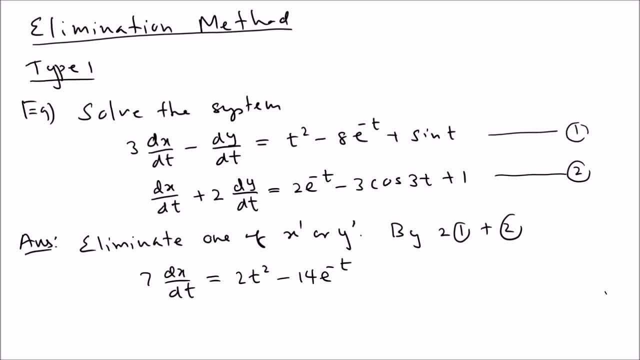 also have two. that means you end up with 14 e to the negative, with 14 e to the negative, with 14 e to the negative, and then we have uh two sine t you're, and then we have uh two sine t you're, and then we have uh two sine t you're gonna get. 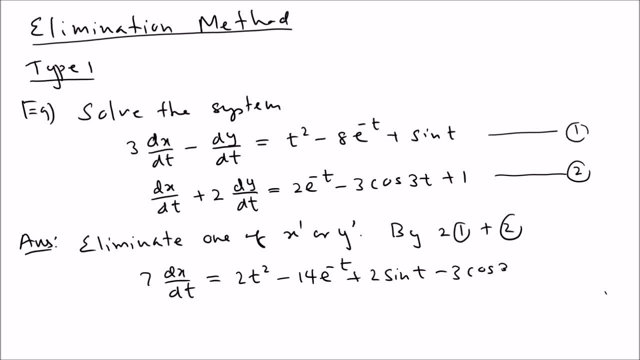 gonna get. gonna get in the bottom. you're gonna get three in the bottom. you're gonna get three in the bottom. you're gonna get three: cosine, uh, cosine, uh, cosine, uh. three t, and then plus one. so that's what? three t and then plus one, so that's what. 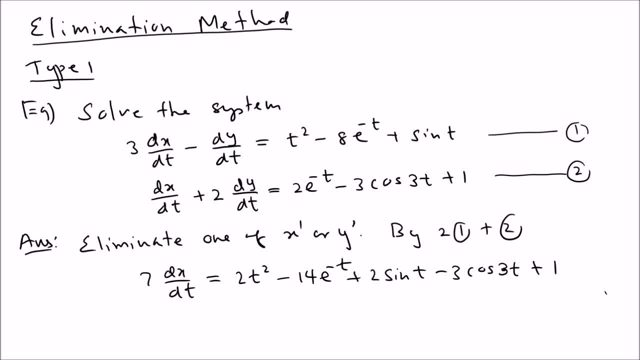 three t and then plus one. so that's what you get, you get. you get uh, just a long expression. because there uh just a long expression, because there uh just a long expression, because there are many terms just integrate now once are many terms, just integrate, now once. 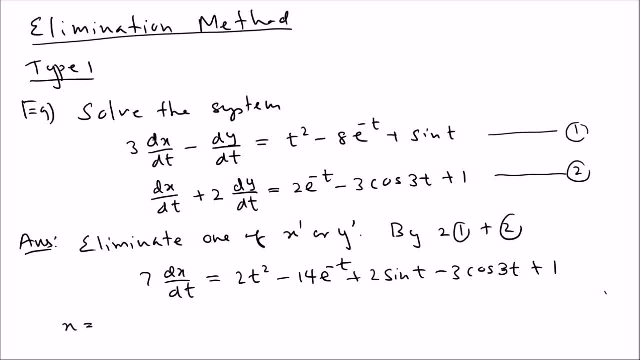 are many terms, just integrate. now, once you integrate, you get x, you integrate, you get x, you integrate, you get x. so x. equal the integral of uh dx over so x. equal the integral of uh dx over so x. equal the integral of uh dx over dt, dt. 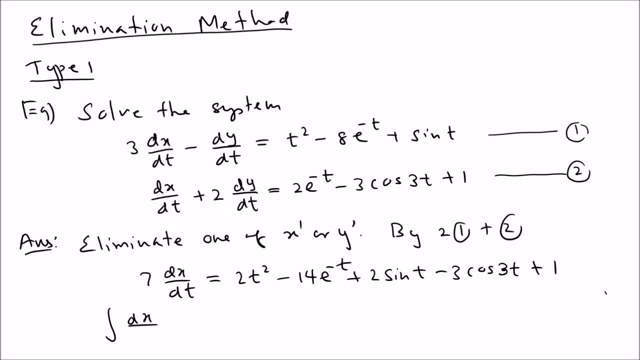 dt: um actually, before we, before we do that. um actually, before we, before we do that. um actually, before we, before we do that, we're gonna divide this. yeah, let's try, we're gonna divide this. yeah, let's try, we're gonna divide this. yeah, let's try that instead. 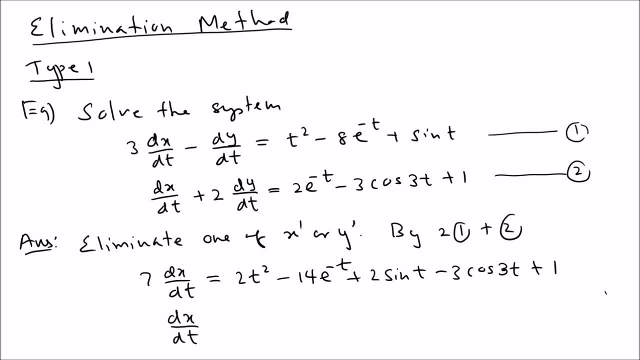 that instead that. instead: so dx over dt. if you divide by seven, so dx over dt. if you divide by seven, so dx over dt. if you divide by seven um, you can see it is seven um. you can see it is seven um. you can see it is seven. it is two over seven. 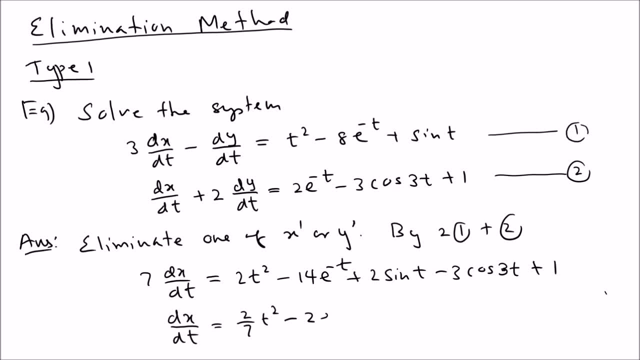 it is two over seven, it is two over seven, two over seven, t squared minus two, e two over seven, t squared minus two, e two over seven, t squared minus two. e negative t. negative t. negative t plus two. seven sine plus two. seven sine plus two. seven sine t minus three. seven cosine. 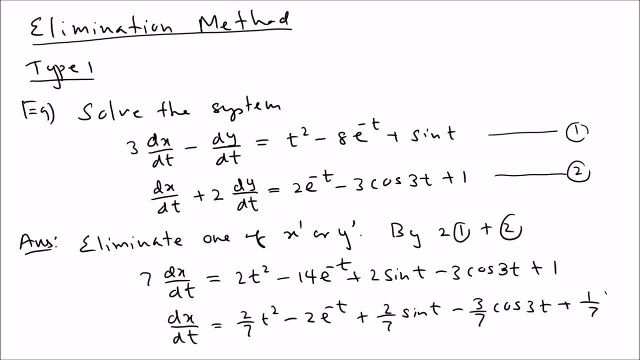 t minus three seven cosine t minus three, seven cosine three t plus one over seven. so that's three t plus one over seven. so that's three t plus one over seven. so that's what you get, what you get, what you get, uh. now, what you can do, uh. 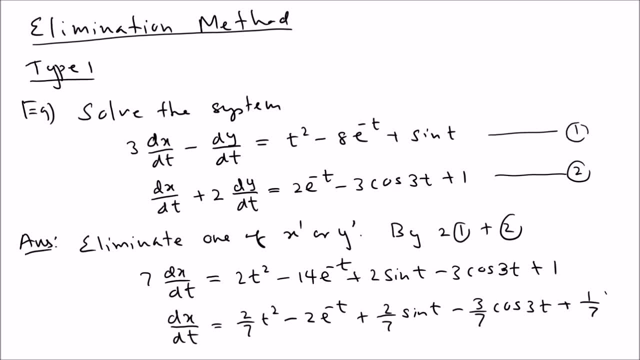 uh, now what you can do. uh, uh, now what you can do. uh, we can integrate the two sides. we can integrate the two sides. we can integrate the two sides. so just integrate with respect to t you. so just integrate with respect to t you. so just integrate with respect to t. you get x. 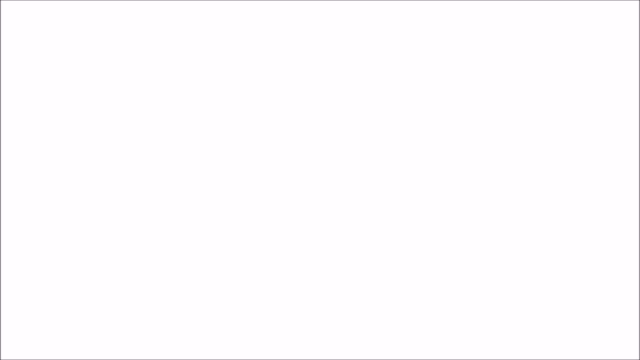 get x, get x, okay. so now what we're going to okay. so now what we're going to okay, so now what we're going to integrate. so, once you integrate, you get x, which is so. once you integrate, you get x, which is so, once you integrate, you get x, which is the integral of dx over dt. 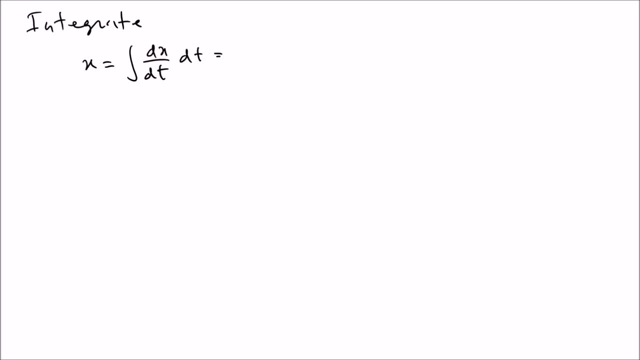 the integral of dx over dt, the integral of dx over dt. one uh, so just integrate one, uh. so just integrate one, uh. so just integrate. so we have a lot of terms. so integrate. so we have a lot of terms. so integrate. so we have a lot of terms. so integrate term by term. so we have two over seven. 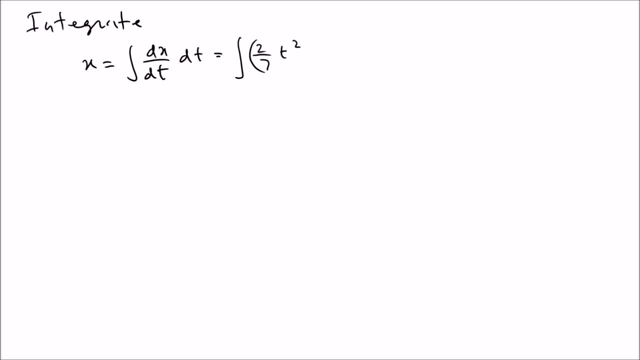 term by term. so we have two over seven. term by term. so we have two over seven t squared. i'm gonna write everything t squared. i'm gonna write everything t squared. i'm gonna write everything, but you can skip this step. it's not. but you can skip this step. it's not. 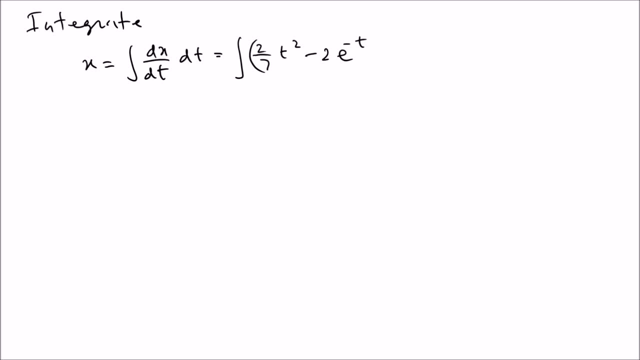 but you can skip this step. it's not really necessary, so it's negative two really necessary, so it's negative two really necessary, so it's negative two. e to the negative t plus two over e to the negative t plus two over e to the negative t plus two over seven: uh, sine t. 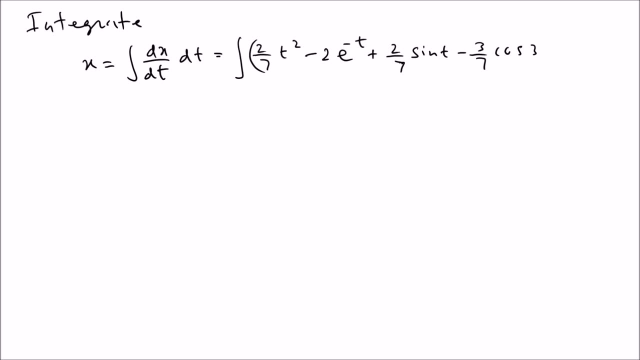 seven uh sine t, seven uh sine t minus three over seven cosine three t minus three over seven. cosine three t minus three over seven. cosine three t plus one over seven, plus one over seven, plus one over seven dt. so if you integrate, i'm gonna write dt. so if you integrate, i'm gonna write. 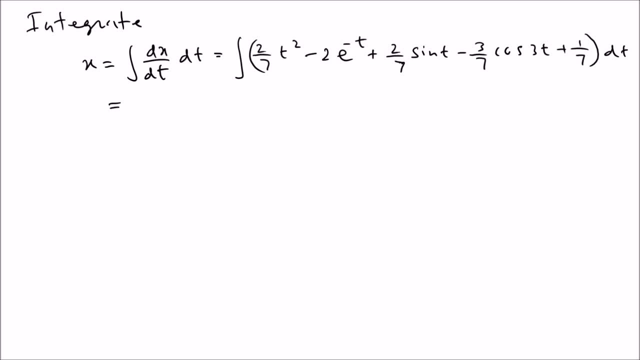 dt. so if you integrate, i'm gonna write the answer here, the answer here, the answer here. so you're gonna get uh. you have to. so you're gonna get uh, you have to. so you're gonna get uh, you have to divide by divide, by divide by three. so it is two over 21. 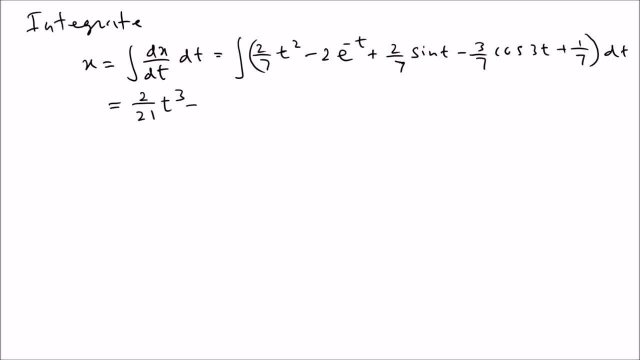 three, so it is two over 21. three, so it is two over 21. t cube minus: okay when you have t cube minus. okay when you have t cube minus. okay when you have exponential function. you divide by the exponential function, you divide by the exponential function, you divide by the constant. so negative one. so that means: 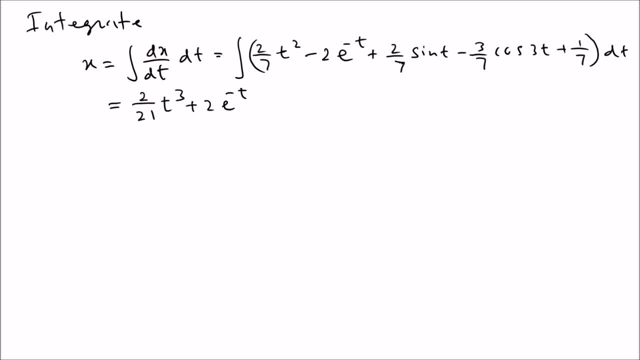 constant, so negative one. so that means constant, so negative one. so that means it's going to be positive to e to the. it's going to be positive to e to the. it's going to be positive to e to the negative t, negative t, negative t uh. sine means negative cosine, uh, so it. 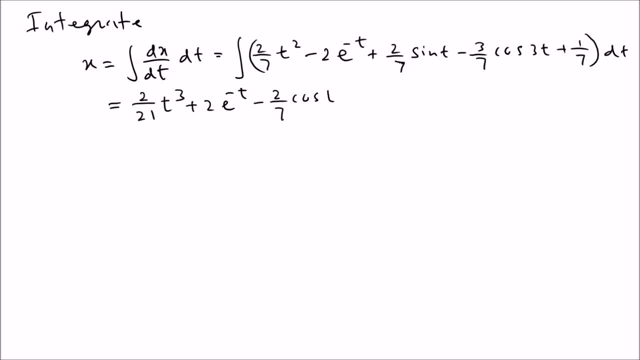 uh sine means negative cosine. uh, so it. uh sine means negative cosine. uh, so it is negative, is negative, is negative. two over seven cosine t. two over seven cosine t. two over seven cosine t. uh in the next one. this is a cosine, but. uh in the next one. this is a cosine, but. 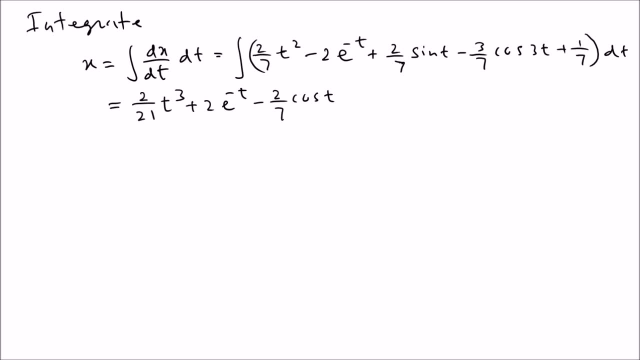 uh, in the next one. this is a cosine, but there's a three. that means you have, there's a three. that means you have there's a three. that means you have divided by three. divided by three, divided by three, it's a cosine you can sign, so it's a. 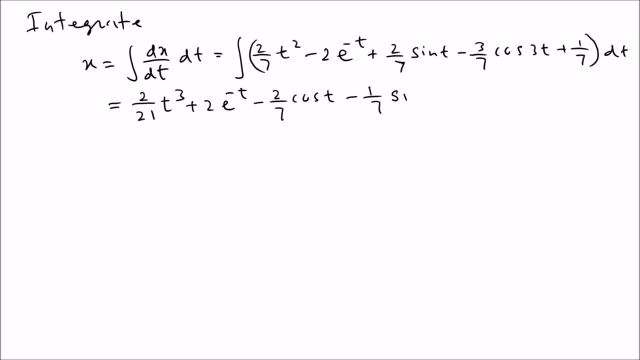 it's a cosine you can sign, so it's a. it's a cosine you can sign, so it's a negative. one third. one seventh negative. one third. one seventh negative. one third. one seventh, sine three t. when you divide by three, sine three t. when you divide by three. 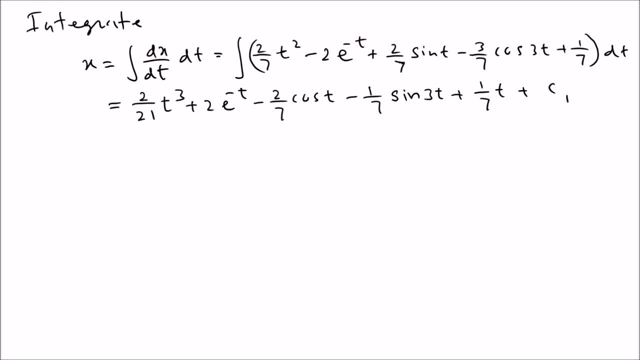 sine three t, when you divide by three plus one over seven t plus c. one plus one over seven t plus c. one plus one over seven t plus c one. introduce a constant name. so that is the: introduce a constant name. so that is the. introduce a constant name. so that is the um solution for x. now what we can do. 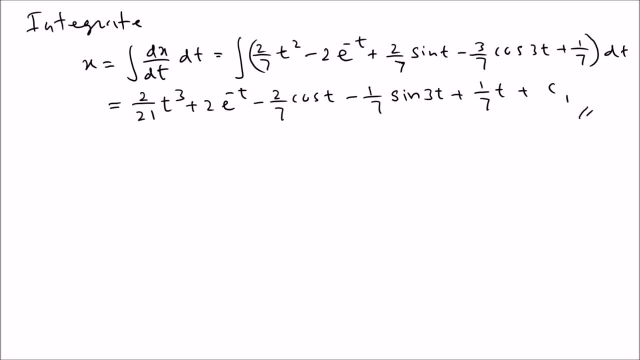 um solution for x, now what we can do. um solution for x, now what we can do. there are two ways to do. there are two ways to do. there are two ways to do, uh, two ways to find y. one way is: uh, two ways to find y. one way is: 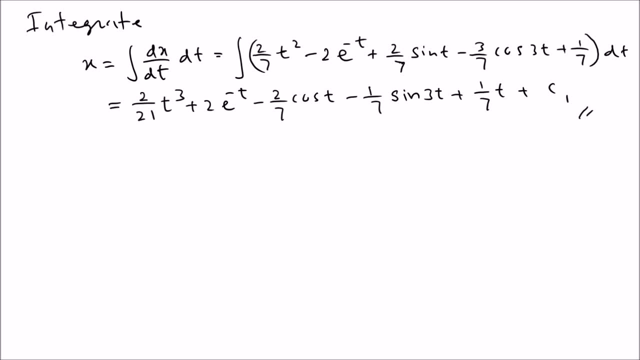 uh, two ways to find y one way is: you can plug in this solution in one. you can plug in this solution in one, you can plug in this solution in one of those equations, of those equations, of those equations, so to plug in that solution, one of those. 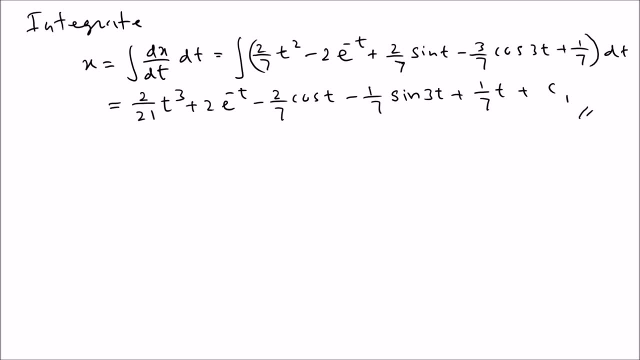 so to plug in that solution, one of those. so to plug in that solution, one of those. equations, equations, equations. you can see that the dx over dt can go. you can see that the dx over dt can go. you can see that the dx over dt can go away. 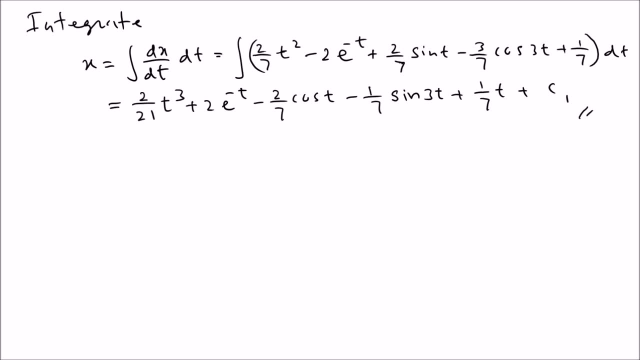 away, away, and then you only have dy over dt then, and then you only have dy over dt, then, and then you only have dy over dt. then you integrate that to find y, you integrate that to find y, you integrate that to find y. the other way is just do the same thing. 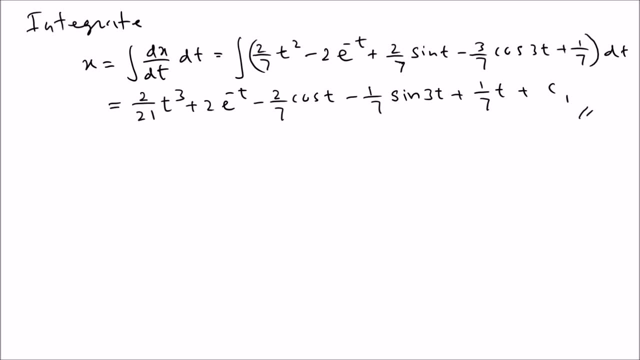 the other way is just do the same thing. the other way is just do the same thing as we did before, as we did before, as we did before: to eliminate the x term dx over dt term. to eliminate the x term dx over dt term. to eliminate the x term dx over dt term, y over dt, as before. 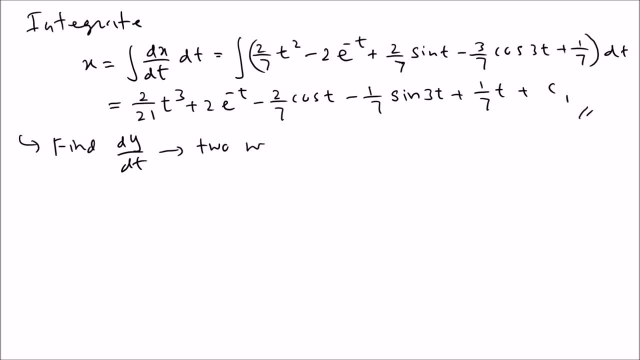 y over dt as before, y over dt as before. uh, there are two ways, uh, two ways to do it. okay, so we can use uh two ways to do it. okay, so we can use uh two ways to do it. okay, so we can use one of the methods. so we're going to do. 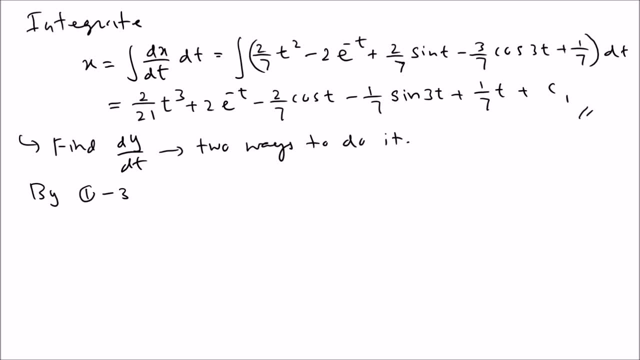 one of the methods. so we're going to do one of the methods, so we're going to do by by, by: uh one minus three times uh, one minus three times. uh, one minus three times two, two, two. why we do that, then you can. because. why we do that, then you can, because 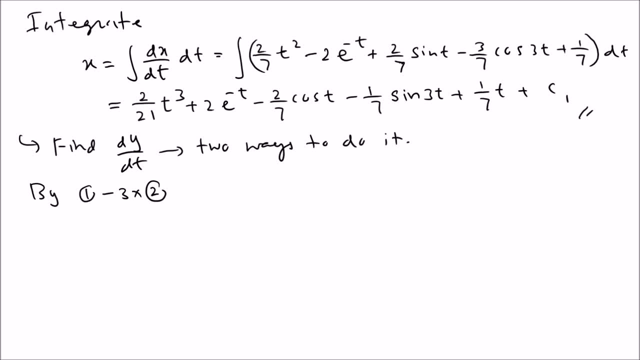 why we do that, then you can, because you have a three and a one. you have a three and a one, you have a three and a one. so if you multiply the bottom one by so, if you multiply the bottom one by so, if you multiply the bottom one by negative three and add: 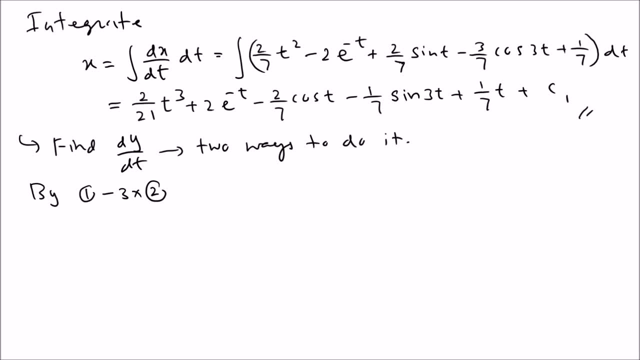 negative three and add negative three and add uh dx or dt gonna go away. uh, so that's uh dx or dt gonna go away. uh, so that's uh dx or dt gonna go away. uh, so that's exactly. so we're gonna get. exactly so we're gonna get. 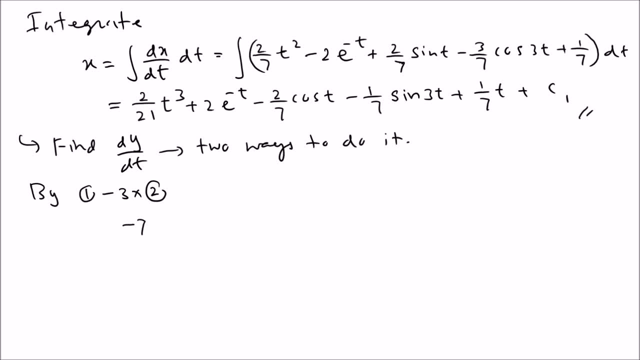 exactly so we're gonna get negative seven where you multiply the negative seven, where you multiply the negative seven, where you multiply the top one by um top one by um top one by um bottom one by three, so you get negative bottom one by three, so you get negative. 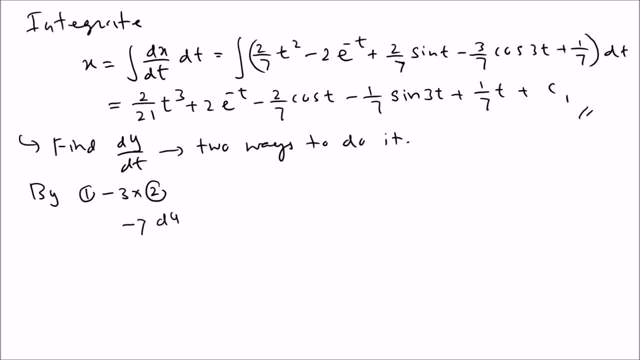 bottom, one by three, so you get negative six and six and six, and there's another one, so it's negative. there's another one, so it's negative, there's another one, so it's negative. seven d y over dt, seven d y over dt, seven d y over dt um. and then you're gonna get 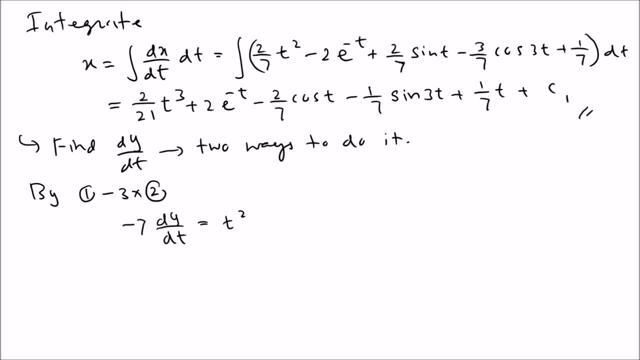 um, and then you're gonna get um, and then you're gonna get: ah t squared. ah t squared. ah t squared, minus 14. e to the negative t minus 14. e to the negative t minus 14. e to the negative t plus sine t minus. 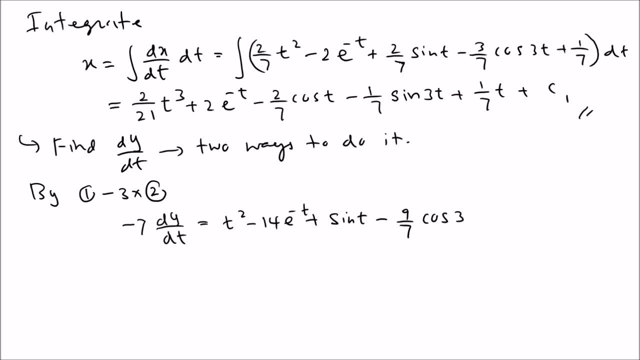 plus sine t minus plus sine t minus. nine over seven cosine. nine over seven cosine. nine over seven cosine three. t uh minus three. t uh minus three. t uh minus three. that's what you get. three, that's what you get. three, that's what you get ah. 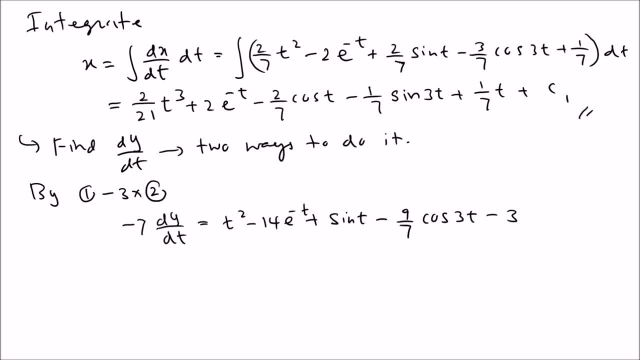 okay, and then what we're going to divide, okay, and then what we're going to divide, okay, and then what we're going to divide by seven as before. by seven as before. by seven as before. so you get dy over dt. so you get dy over dt. 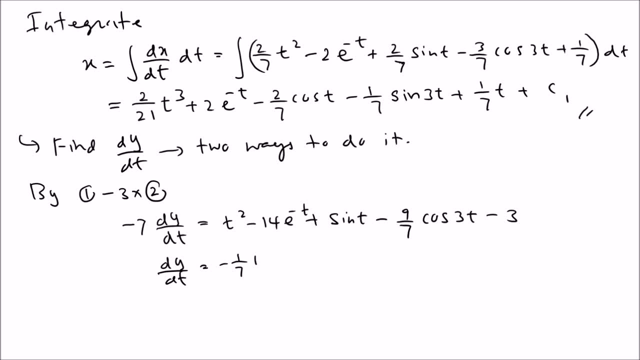 so you get dy over dt. equals equals, so you get dy over dt. equals equals equals. uh negative one over seven t. uh negative one over seven t. uh negative one over seven t. squared, squared, squared. uh positive two e to the negative t. uh positive two e to the negative t. 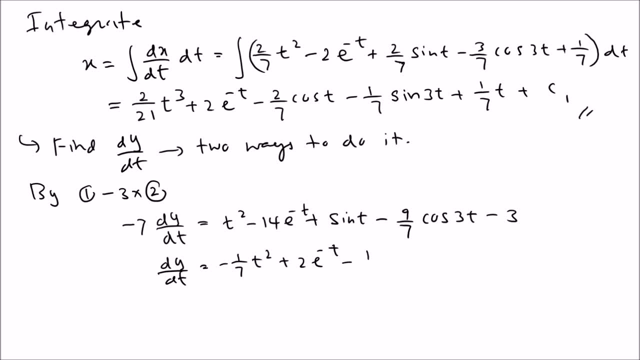 uh positive. two e to the negative t. negative one over seven. uh, negative one over seven. uh, negative one over seven. uh sine t. and then uh pos, uh sine t, and then uh pos, uh sine t, and then uh pos: yeah, it's again negative. uh, yeah, it's again negative, uh. 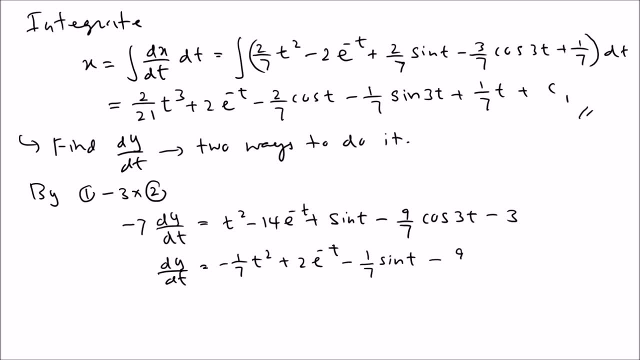 yeah, it's again negative, uh, negative. nine of negative, nine of negative, nine of uh actually uh, so yeah, so that's it. i don't uh actually uh, so that's it. i don't uh actually uh, so that's it. i don't know where there's negative seven, nine or 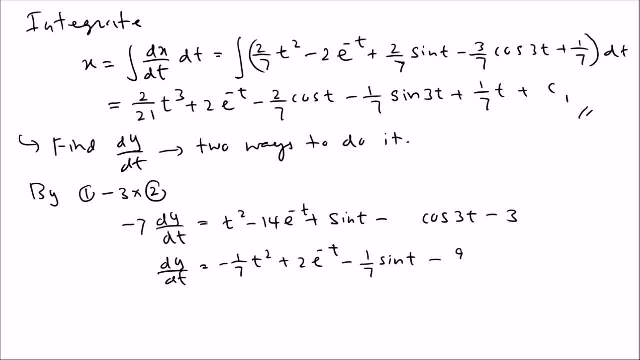 know where there's negative seven, nine, or know where there's negative seven, nine or seven. it's just nine. seven, it's just nine, it's just nine, seven, it's just nine. so you have plus nine here, uh, because we. so you have plus nine here, uh, because we. 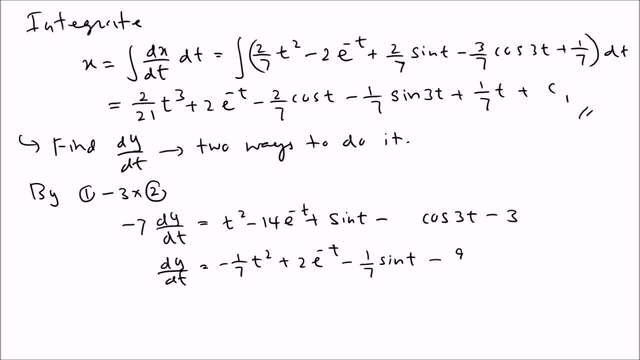 so you have plus nine here. uh, because we multiply um. so let's look at that one multiply um. so let's look at that one multiply um. so let's look at that one again. uh, so we have, yeah, so we can again. uh, so we have, yeah, so we can. 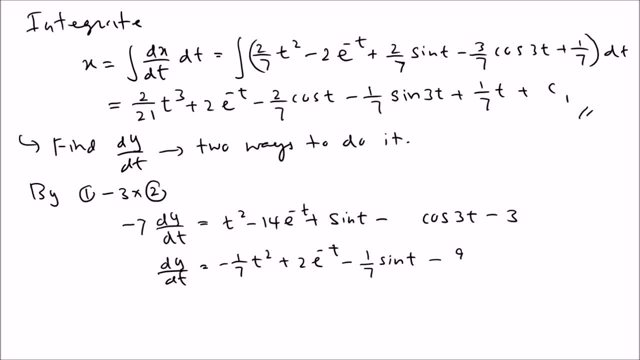 again. uh, so we have yeah, so we can multiply the bottom negative three. so multiply the bottom negative three, so multiply the bottom negative three, so we can positive nine. i don't know why we can positive nine. i don't know why we can positive nine. i don't know why. you're right, positive nine. now here is 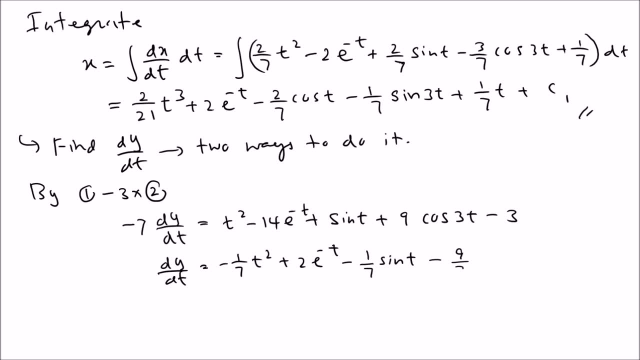 you're right, positive nine. now here is, you're right, positive nine. now. here is going to be um, going to be um, going to be um. negative nine over seven. negative nine over seven, negative nine over seven. uh, cosine, uh, cosine, uh, cosine, three t, three t, three t, and then we divide by a negative seven. 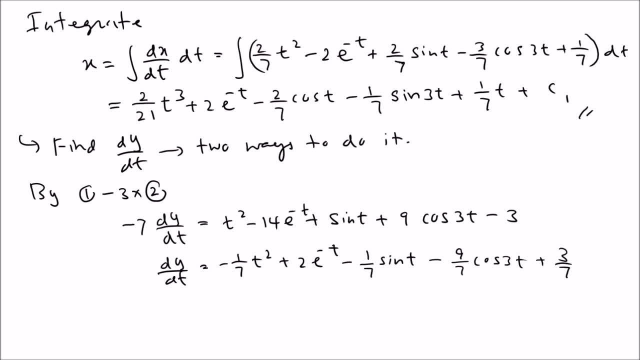 and then we divide by a negative seven, and then we divide by a negative seven, so it's going to be positive. so it's going to be positive, so it's going to be positive. three over seven, so that's what we have. three over seven, so that's what we have. 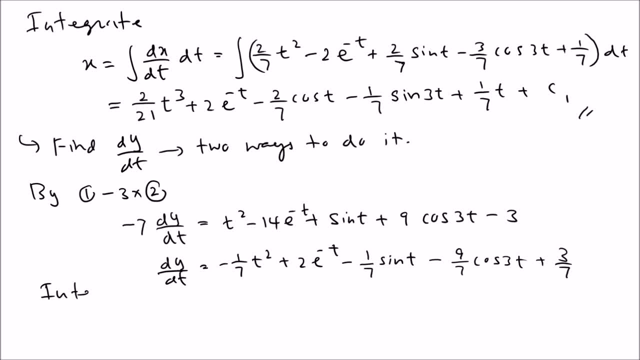 three over seven. so that's what we have, uh, and then integrate, okay, so integrate. so, once you integrate, uh, you're gonna so. once you integrate, uh, you're gonna. so once you integrate, uh, you're gonna get the answer. so y equal the integral of. get the answer. so y equal the integral of. 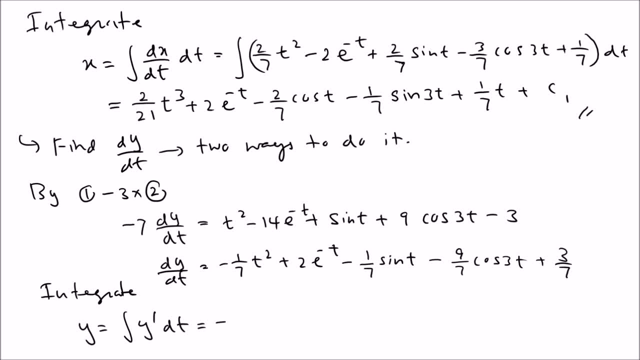 get the answer. so y equal the integral of y prime dt, y prime dt, y prime dt. so just integrate so you can negative uh. so just integrate, so you can negative. uh, so just integrate, so you can negative uh. one over 21 t. one over 21 t. 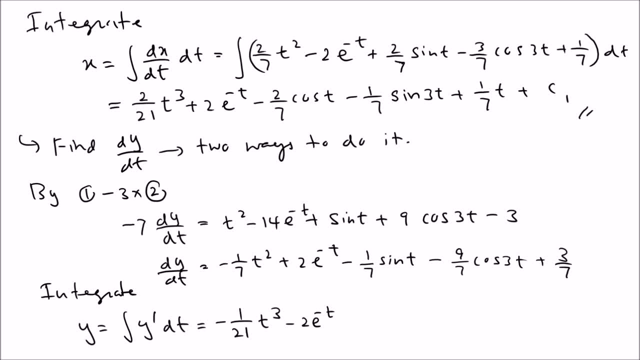 one over 21 t cube negative. two e to the negative t cube negative. two e to the negative t cube negative. two e to the negative t uh, and then sine means uh, negative uh, and then sine means uh, negative uh, and then sine means uh, negative cosine. so it's been one over seven. 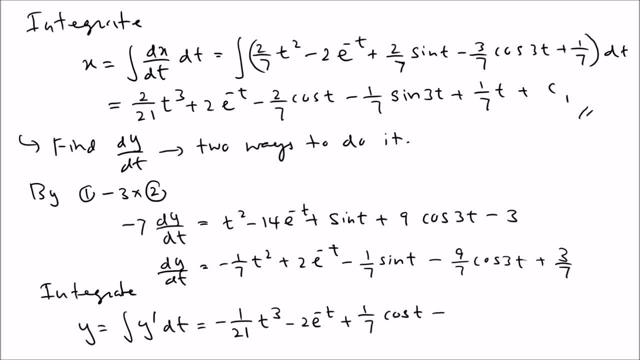 cosine, so it's been one over seven. cosine, so it's been one over seven. cosine t, cosine t, cosine t, uh, and then negative, you divide by three, uh, and then negative, you divide by three, uh, and then negative, you divide by three, so you get three over seven sine. 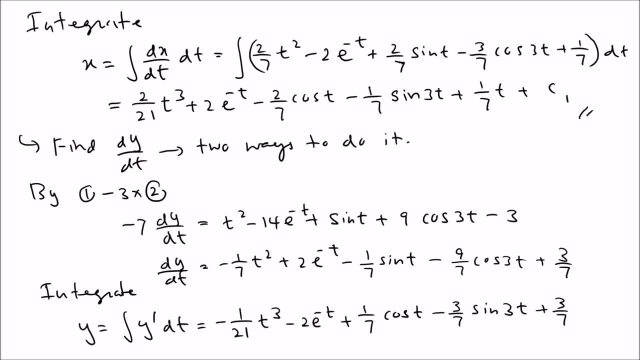 so you get three over seven sine. so you get three over seven sine. three t plus three t plus three t plus three over seven. you add another three over seven, you add another three over seven. you add another constant c2 for that. so those are the constant c2 for that. so those are the. 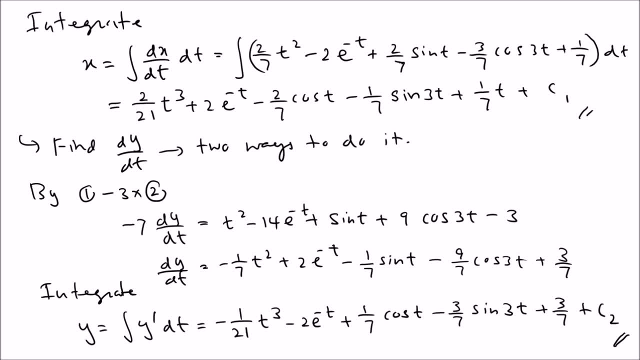 constant c2 for that. so those are the two answers. so we have the x. two answers. so we have the x. two answers. so we have the x and the y- so you can see it's just very- and the y. so you can see, it's just very. 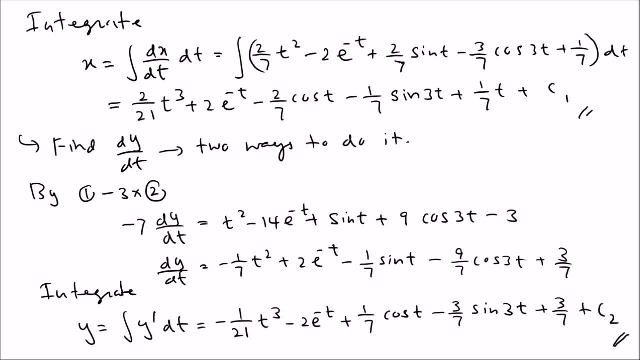 and the y. so you can see, it's just very direct way to simplify that, direct way to simplify that direct way to simplify that. so that's a type one. so let's talk about so that's a type one. so let's talk about: so that's a type one. so let's talk about the type two. so what is type two? 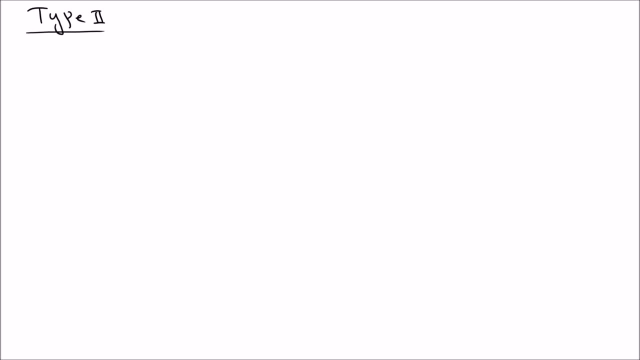 so type two, um so type two, um so type two, um type two, like uh, the situation there. we type two. like uh, the situation there. we type two, like uh, the situation there. we cannot do this, okay, so let's, let's look. cannot do this, okay, so let's, let's look. 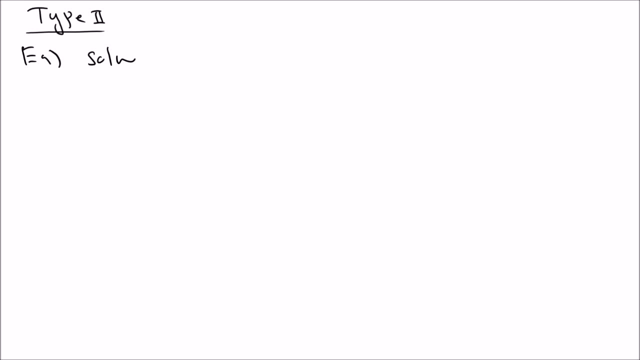 cannot do this, okay, so let's let's look at a problem again, at a problem again, at a problem again. so let's say uh, solve. so. let's say uh, solve. so let's say uh, solve the system, the system, the system solve the system. let's say x prime. 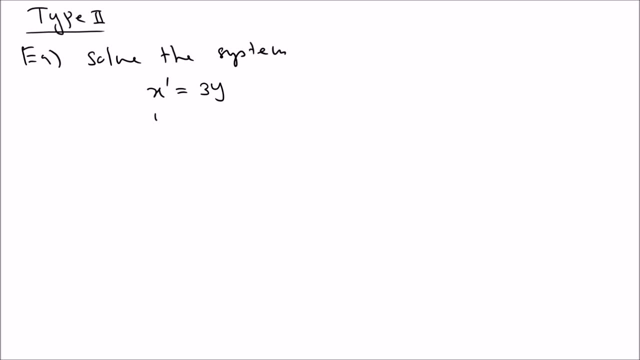 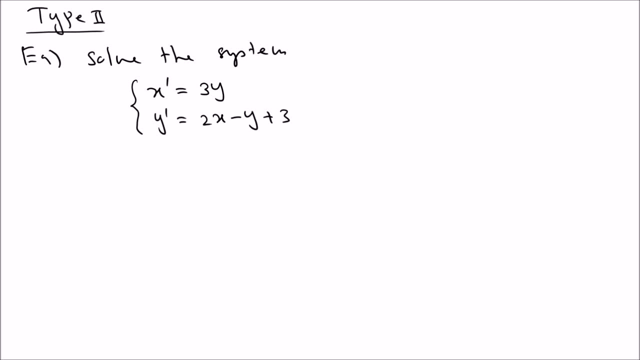 minus y plus 3. so that's the system. minus y plus 3. so that's the system. sometimes we write the curly brace like: sometimes we write the curly brace like. sometimes we write the curly brace like that, that, that it's not really necessary. uh, we're. 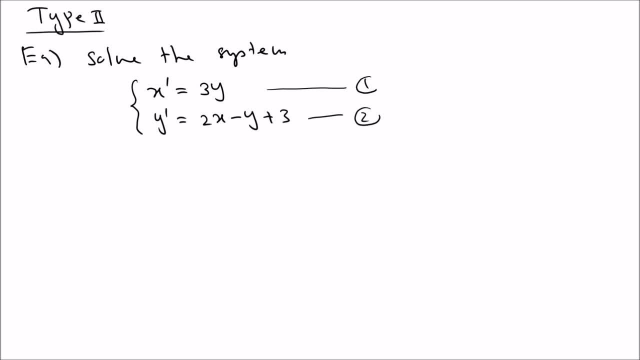 it's not really necessary, uh, we're it's not really necessary, uh, we're gonna call the equations, gonna call the equations, gonna call the equations one and equation two. now you can see one and equation two. now you can see one and equation two, now you can see. uh, there's no way, you can just solve. 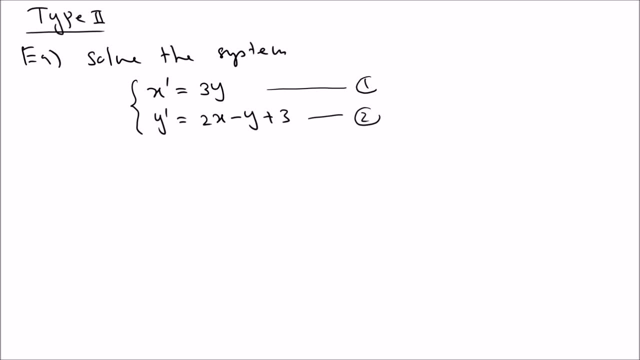 uh, there's no way you can just solve. uh, there's no way you can just solve for one here, for one here, for one here, uh, because there are no other, uh, because there are no other, uh, because there are no other derivatives. so that means the method. 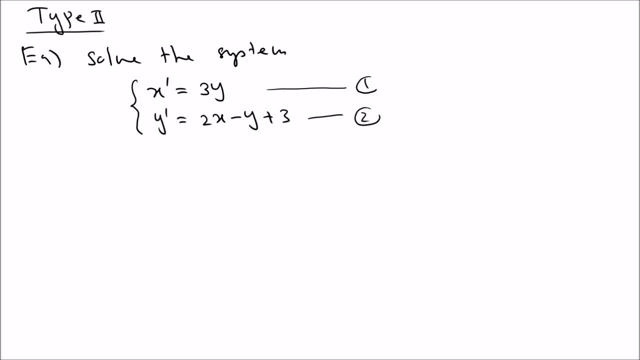 derivatives. so that means the method derivatives. so that means the method that we use for the previous one, doesn't that we use for the previous one, doesn't that we use for the previous one? doesn't work here. work here, work here. so what you're going to do is you're. 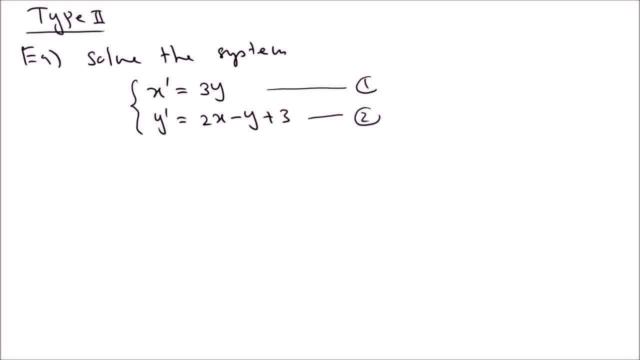 so what you're going to do is you're. so what you're going to do is you're going to take derivatives. we can take going to take derivatives. we can take going to take derivatives. we can take derivatives and then try to substitute derivatives and then try to substitute. 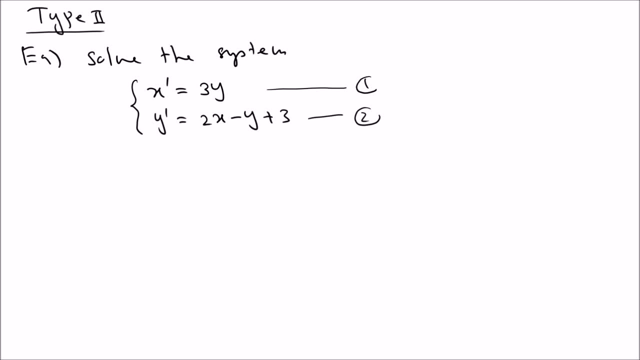 derivatives and then try to substitute from the other one, to remove one from the other one, to remove one from the other one, to remove one variable, variable, variable. now you have two options you can take. now you have two options you can take. now you have two options, you can take the derivative, the first one or the. 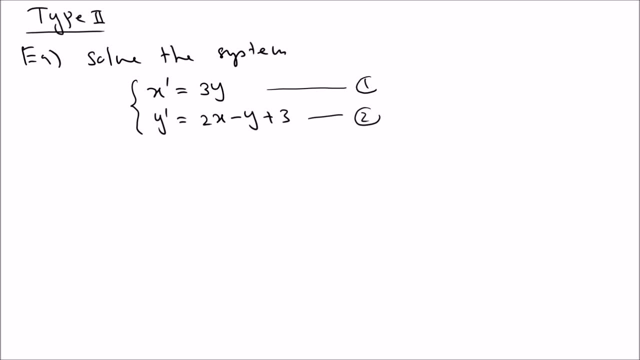 the derivative the first one, or the derivative the first one, or the derivative the second one, but you can derivative the second one, but you can derivative the second one. but you can see the three here, since we have the see the three here, since we have the see the three here, since we have the three here. 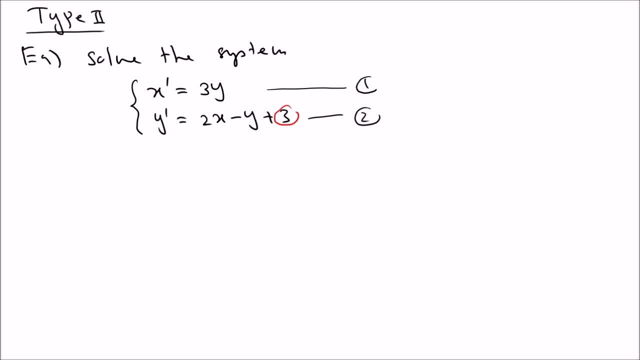 three here, three here to avoid undetermined, to avoid undetermined, to avoid undetermined. uh coefficient method. we can take the uh coefficient method. we can take the uh coefficient method. we can take the derivative of the bottom one, then that's derivative of the bottom one, then that's. derivative of the bottom one, then that's three going to go away. so that's the three going to go away. so that's the three going to go away. so that's the. that's the trick we do, you see. because that's the trick we do, you see, because 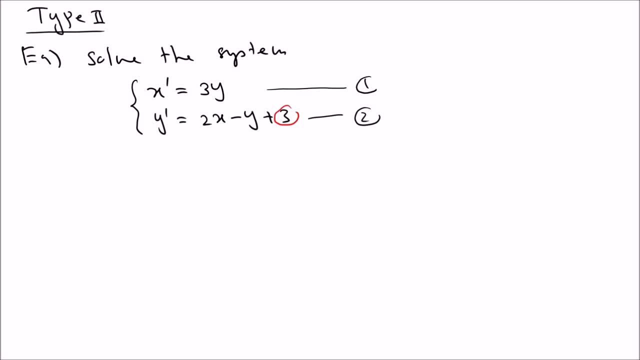 that's the trick we do, you see, because if you take the top one, if you take the top one, if you take the top one, you end up with the equation which is. you end up with the equation which is, you end up with the equation which is undetermined. you have to use the. 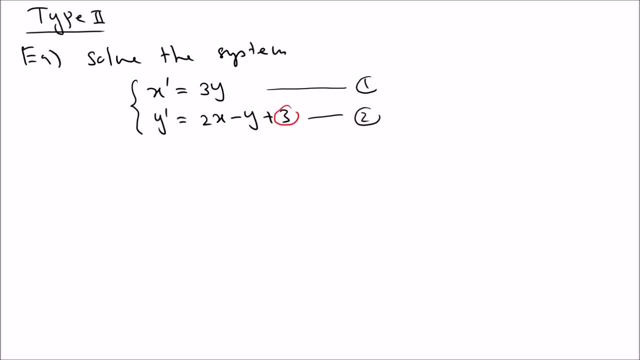 undetermined. you have to use the undetermined. you have to use the undetermined coefficient method. undetermined coefficient method. undetermined coefficient method. so that's going to be a little difficult. so that's going to be a little difficult. so that's going to be a little difficult. so we can avoid that. take the derivative. 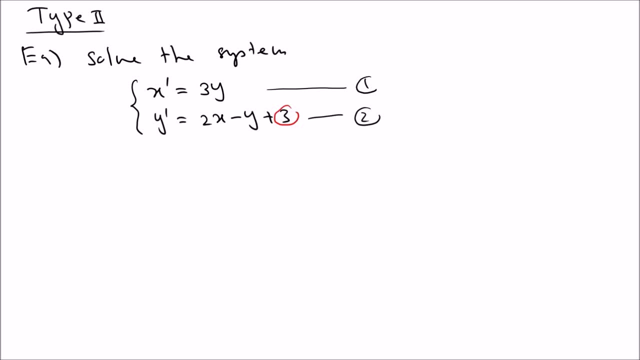 so we can avoid that. take the derivative. so we can avoid that. take the derivative of the bottom one. okay, so we have things of the bottom one. okay, so we have things of the bottom one. okay, so we have things sometimes, sometimes, sometimes. so take the derivative of the second. 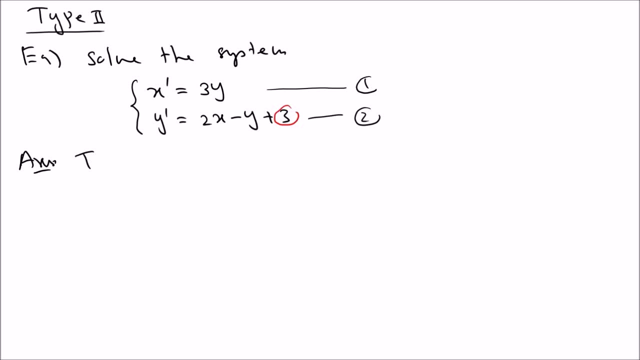 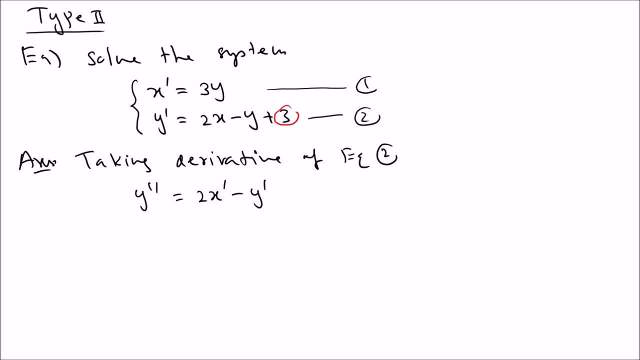 uh, so you're gonna get y double prime. uh, so you're gonna get y double prime equal to x prime minus y prime, and then equal to x prime minus y prime, and then equal to x prime minus y prime, and then plus zero, plus zero, plus zero. so that's going to go away. now what? 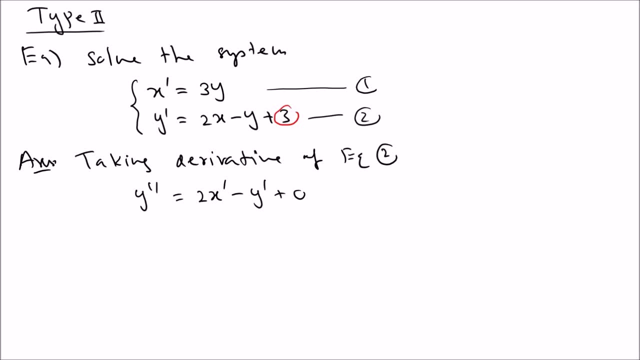 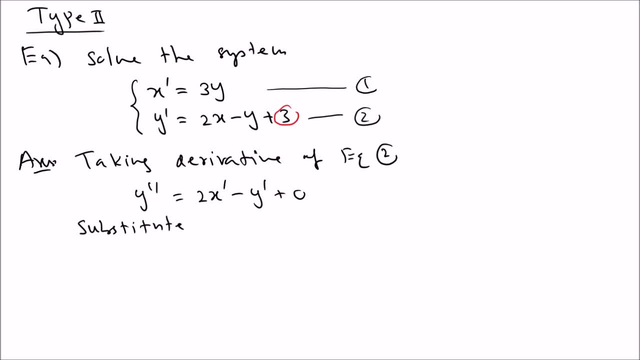 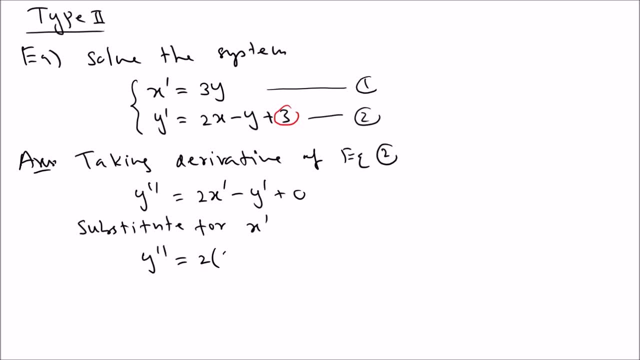 x prime. so if you do that, you get y double prime, double prime, double prime equal two times what is x prime, x prime equal two times what is x prime. x prime equal two times what is x prime. x prime is three y. uh, from the first equation. 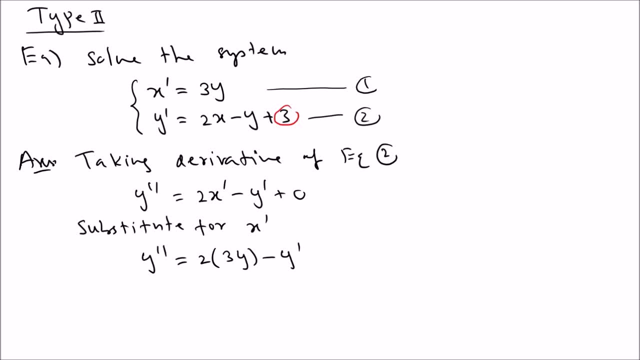 is three y uh from the first equation, is three y uh from the first equation: minus y prime. not now what we can do. we minus y prime, not now what we can do. we minus y prime, not now what we can do. we can bring everything to, can bring everything to. 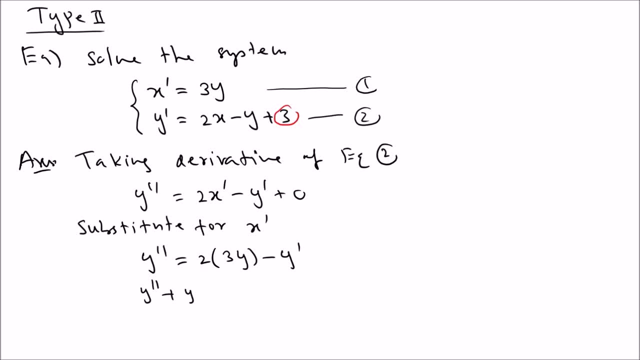 can bring everything to one side. so it is y double prime plus one side. so it is y double prime plus one side. so it is y double prime plus y. prime minus six: y equals zero. y prime minus six: y equals zero. y prime minus six: y equals zero. this is a simple constant coefficient. 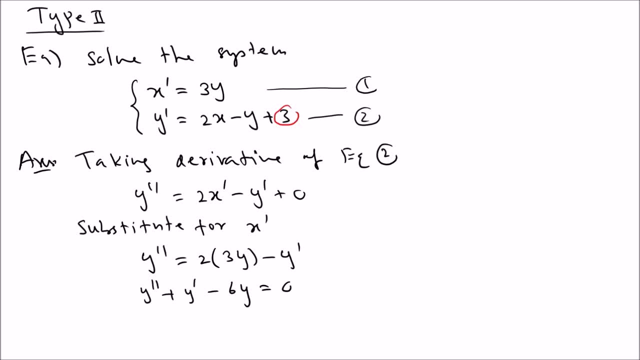 this is a simple constant coefficient. this is a simple constant coefficient. differential equation, differential equation, differential equation, and we write the characteristic equation and we write the characteristic equation and we write the characteristic equation for that. so the characteristic equation for that, so the characteristic equation for that. so the characteristic equation, the characteristic equation is. 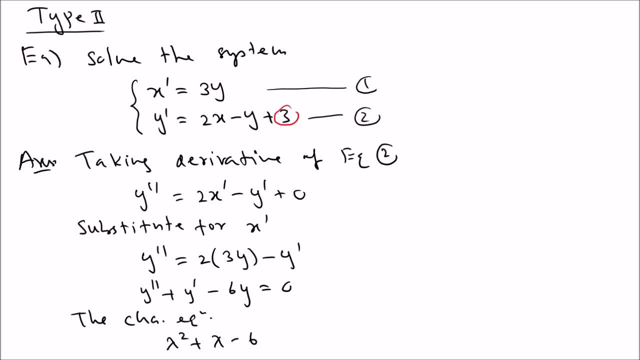 the characteristic equation is: the characteristic equation is: lambda squared plus lambda minus six, lambda squared plus lambda minus six. lambda squared plus lambda minus six um equal zero, and which has factors um equal zero, and which has factors um equal zero, and which has factors uh, lambda minus lambda plus three, and. 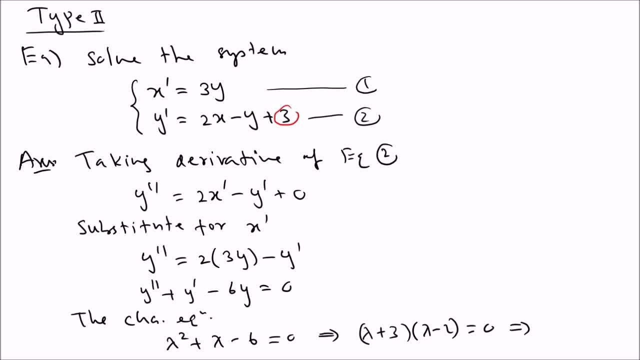 uh, lambda minus lambda plus three and uh, lambda minus lambda plus three and lambda minus two, lambda minus two, lambda minus two equals zero. this is gonna say that lambda equals zero. this is gonna say that lambda equals zero. this is gonna say that lambda equal, equal, equal. uh, negative three and two. so that means: 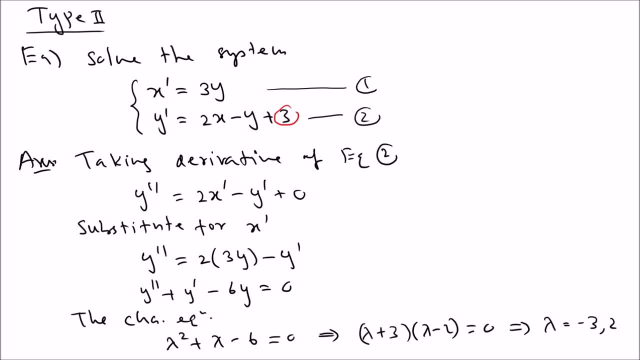 uh, negative three and two. so that means, uh, negative three and two. so that means you can write the. you can write the. you can write the solution. okay, so the y is simply using the formula, so y is simply c1. using the formula, so y is simply c1. 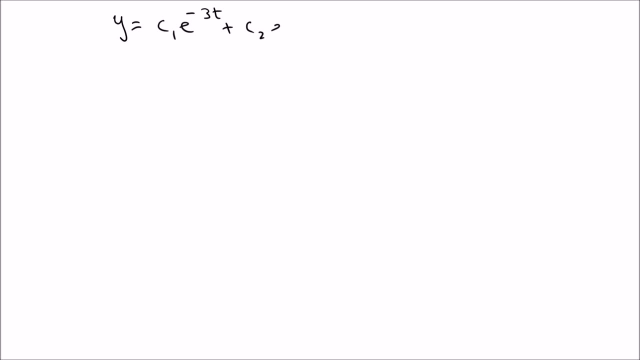 using the formula. so y is simply c1. e to the negative 3 t plus c. e to the negative, 3 t plus c. e to the negative 3 t plus c. 2 e to the 2 t. so that is the y now. 2 e to the 2 t, so that is the y now. 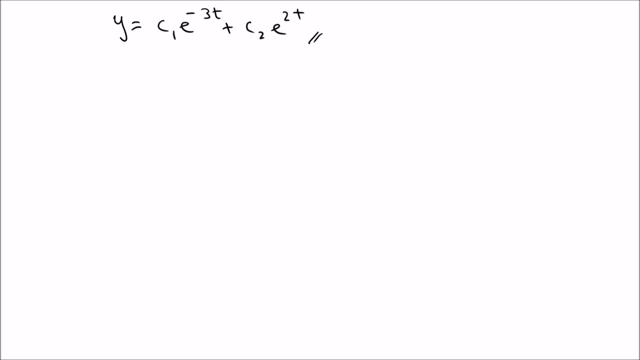 2 e to the 2 t, so that is the y. now what we can do. what we can do. what we can do, uh in this problem, since we know why uh in this problem, since we know why uh in this problem, since we know why, uh you can, because the goal is to find 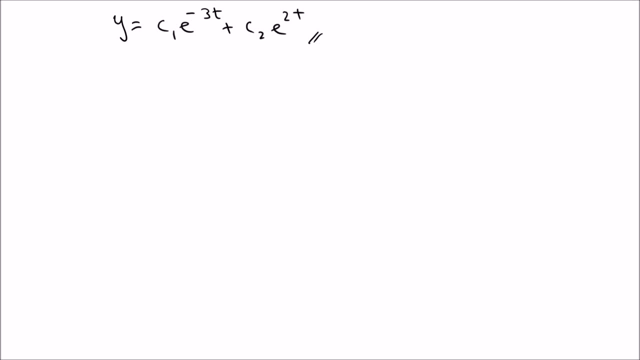 uh, you can, because the goal is to find. uh, you can because the goal is to find x. so what we can do is you can plug in x. so what we can do is you can plug in x. so what we can do is you can plug in that to one of those equations. 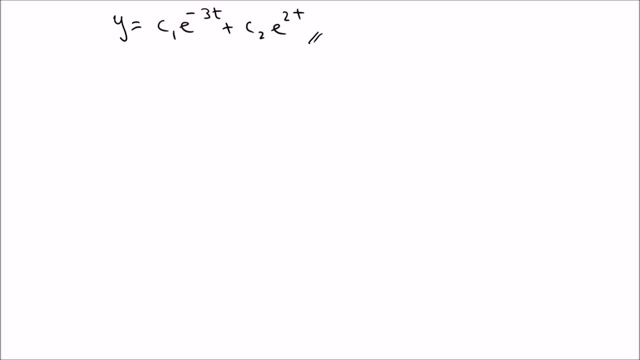 that to one of those equations, that to one of those equations wherever you see y and then solve for x wherever you see y and then solve for x wherever you see y and then solve for x. so you can see that you can do that in two different ways. uh, the one is you can. 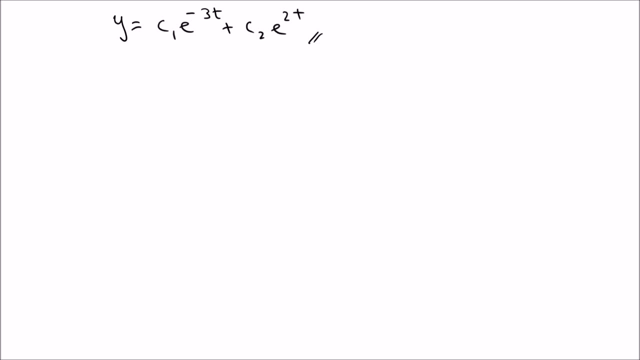 two different ways, uh. the one is: you can. two different ways. uh. the one is: you can just substitute for. take the derivative. just substitute for take the derivative. just substitute for. take the derivative. uh, because we already know what is. uh. uh, because we already know what is uh. 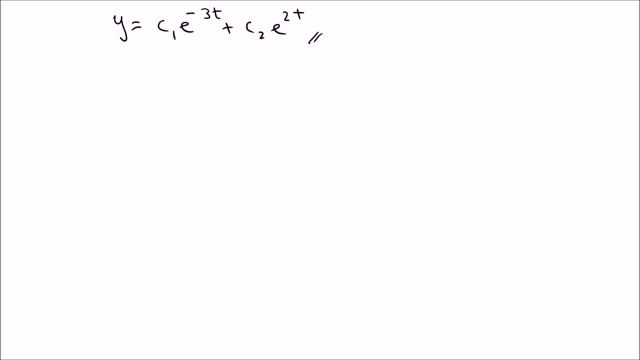 uh, because we already know what is: uh, the derivative y prime, and then we can the derivative y prime, and then we can the derivative y prime, and then we can substitute that substitute, that substitute that. take the derivative and plug into the. take the derivative and plug into the. 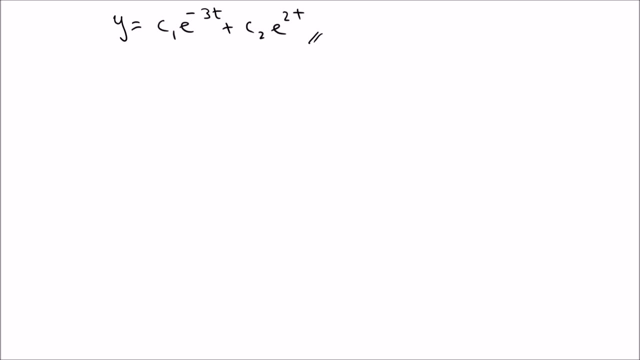 take the derivative and plug into the equation number two. then you get x, equation number two. then you get x, equation number two. then you get x, or substitute in the one in the one, or substitute in the one in the one, or substitute in the one in the one. um, you know, we know that this y value. 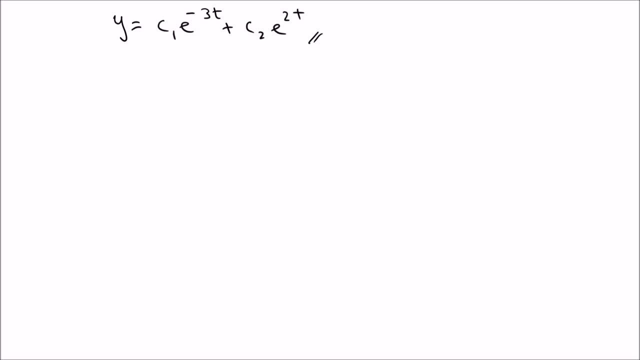 um, you know, we know that this y value, um, you know we know that this y value substitute there, and then integrate substitute there, and then integrate substitute there, and then integrate again, so we can use that one, because again. so we can use that one, because, again. so we can use that one, because that looks little simple. so by one. 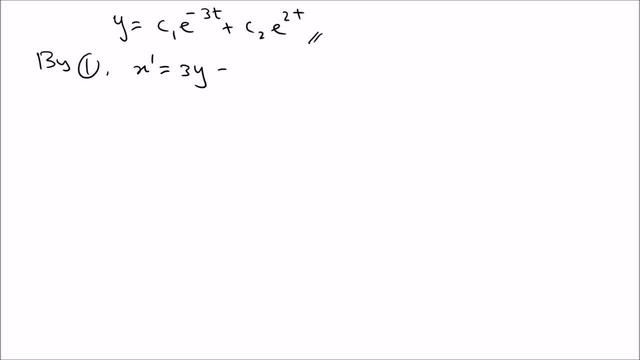 that looks little simple, so by one. that looks little simple, so by one. are we gonna say x prime equal 3 y. are we gonna say x prime equal 3 y? are we gonna say x prime equal 3 y? so now, uh, just apply in for y. 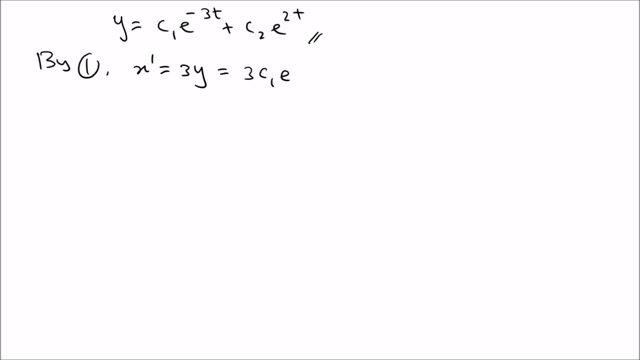 so now uh just apply in for y. so now uh just apply in for y uh. so it is three times c, one e to the uh. so it is three times c, one e to the uh. so it is three times c, one e to the negative, three t plus three times c to e. 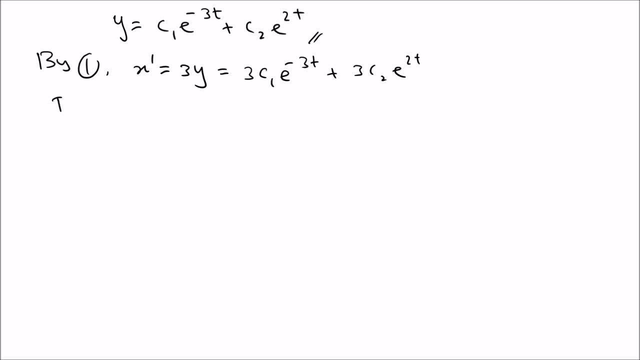 negative three t plus three times c to e. negative three t plus three times c to e to the two t. now what we do integrate to the two t. now what we do integrate to the two t, now what we do integrate. okay, so, integrate, so you're gonna get x, which is the 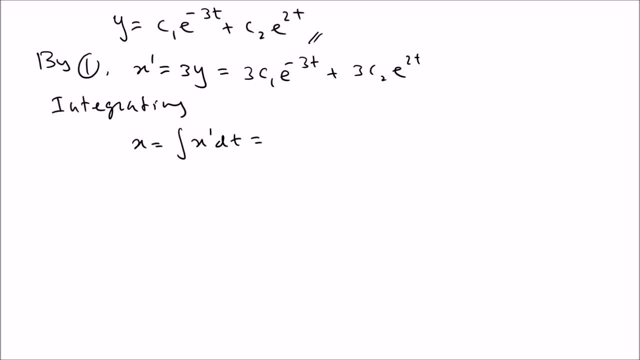 so you're gonna get x, which is the. so you're gonna get x, which is the integral of x, prime dt. integral of x, prime dt. integral of x, prime dt. just integrate the term. so that means you just integrate the term. so that means you just integrate the term. so that means you can divide by. 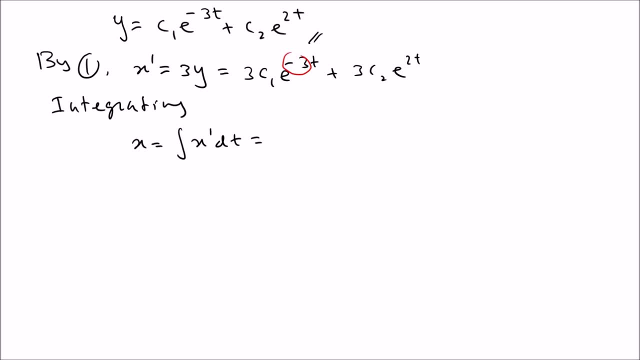 can divide by. can divide by a negative three, um. so you're gonna get uh, let's write. so you're gonna get uh, let's write. so you're gonna get uh, let's write. three c one times e to the negative. three c one times e to the negative. 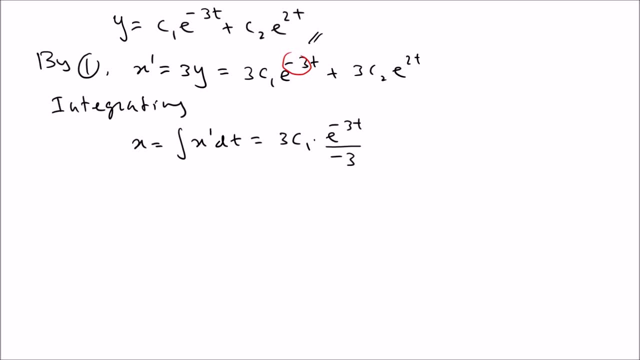 three c, one times e to the negative three t, so this step is not really so. three t, so this step is not really so. three t, so this step is not really so. you can just write, you can just write, you can just write the answer directly. and then here, uh, the. 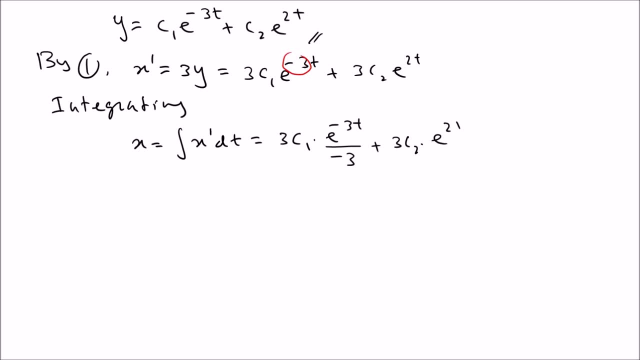 the answer directly. and then here, uh, the. the answer directly, and then here, uh, the same thing. so 3 c, 2 e to the 2 t divided by 2.. now there is a question whether we are going to add another uh constant, and you can see that this is a. we have two first order equations. 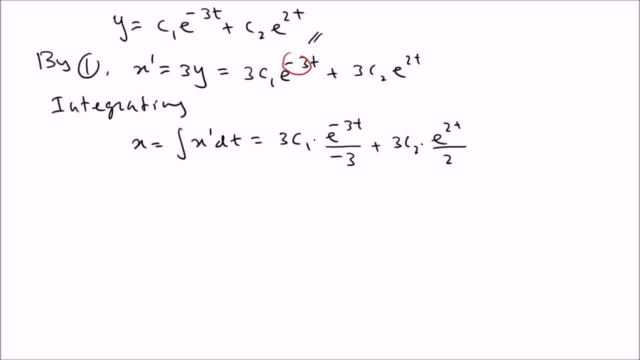 uh, that means you only need two constants. we already have the constants. so that means we are not gonna add anything new. okay, you are not gonna add c3 here, so i will write, but i'm gonna say we are not gonna do that, okay, because we already have two constants. 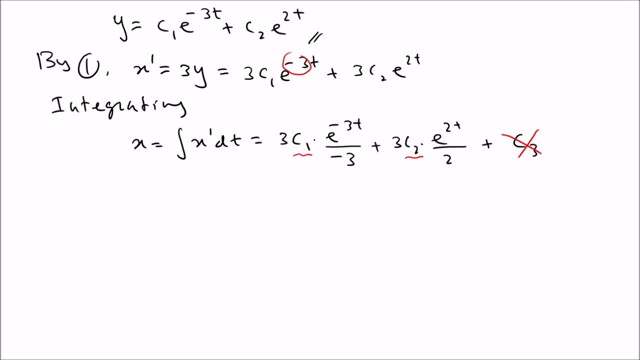 so that's the reason we have c1 and c2. we only need two constants. good, and then we can simplify if you want. so that means the final answer gonna be: uh, negative c1 e to the negative 3 t plus 3 halves c2 e to the 2 t. 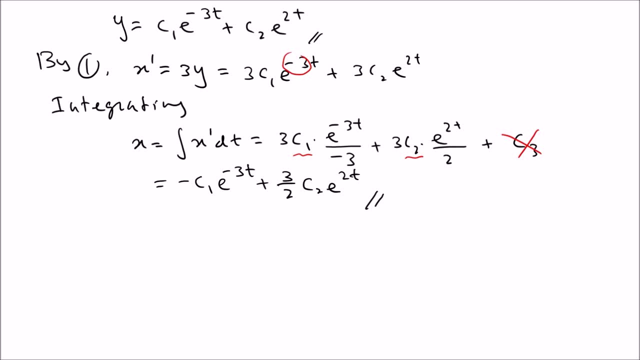 yeah, that's how we do it, uh, so you can see it's not that difficult. but, uh, you have to kind of think before jump, okay, because which one take uh, which one you say the derivative uh depend, um, so you know, can give you like a different answer. i mean, it can be little. 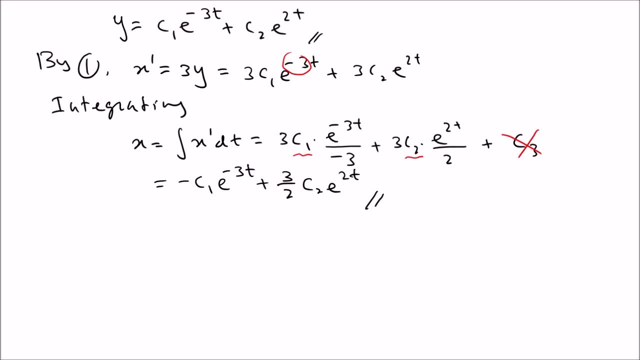 lengthy. if you take the derivative of the first one, because you have a solo, undetermined coefficient, problem, okay. but if you take the data, the bottom one is much easier. so it's always depend on the problem. you can't say beforehand what's going to happen. okay, let's go to the next type, uh, next topic: the laplace transform method. 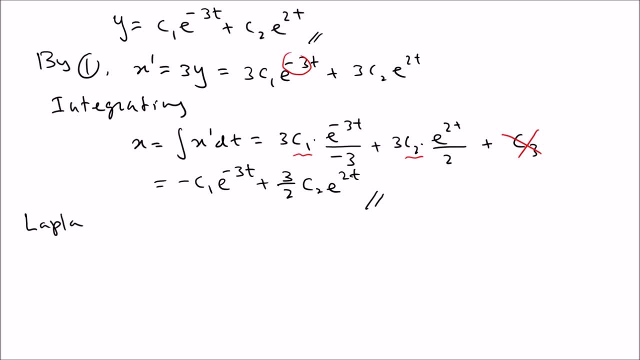 uh, so what we're going to do, let's again look at a problem. so what we normally do is: so let's discuss the argument so we can take the laplace transform of the equation. so, because you can see, it's a system now, so you can see many. 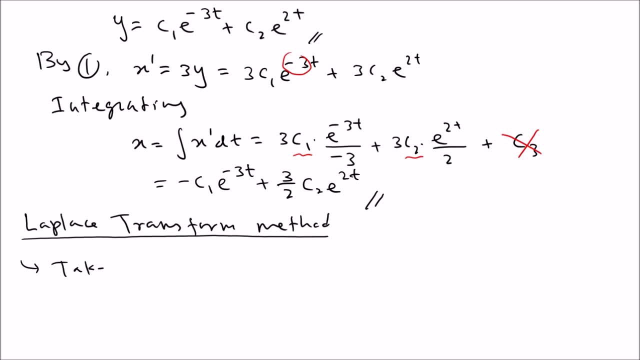 equations. so we take the laplace transform for all the equations. so take uh laplace transform of uh the equations. so we can take the laplace transform of the equations, the equations instead of one equation, and solve. and so, after you get the equations, you're going to see 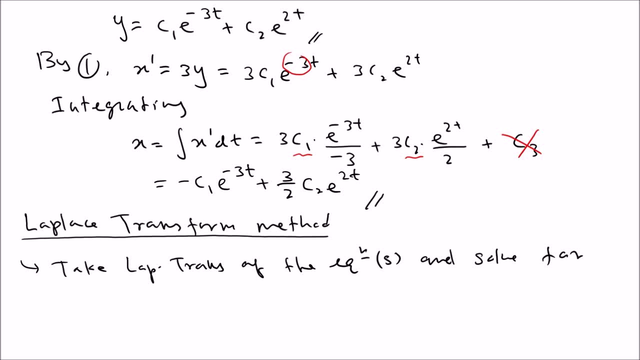 a system with those uh, xs, ys, things like that. so we're going to solve for them as we did before, okay, and solve for uh, x, s, y, s, uh like that, because we don't know how many we have. so solve for them using the elimination method. 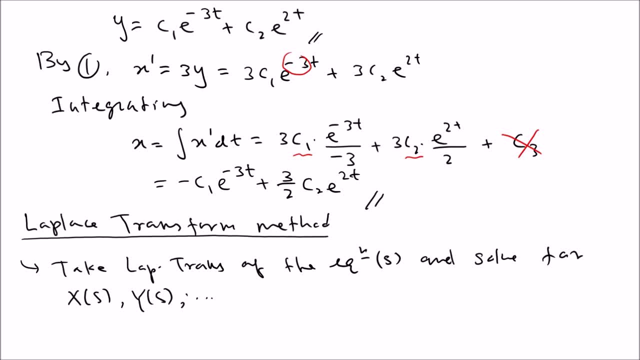 okay, uh, so you can see. uh, yeah, let's try it. uh, i'm gonna say, if you look using elimination, uh, then uh, take the inverse laplace to find uh, xt, yt, like this. so it's a very simple idea: take the laplace, transform so you get a system in that system. you can see. it's just uh, there are no. 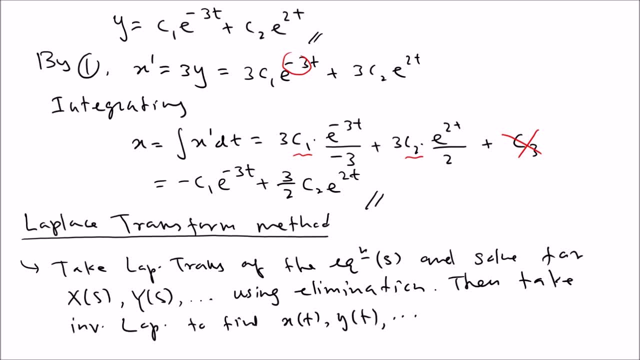 derivatives. we just use the elimination to find them and then take the inverse laplace. so, uh, yeah. so take the laplace transform, eliminate, and then take the inverse laplace transform. those are the steps. so let's just do one problem, but i'm not going to complete- to solve the problem. 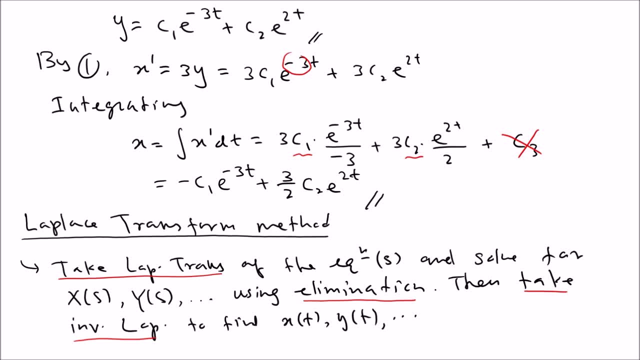 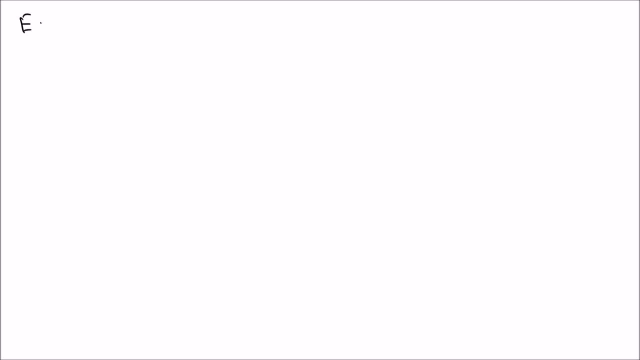 because those are going to be a little lengthy. i'm going to show you the steps and then you can finish this. so let's do this problem. so, example um, solve the system. let's say d squared x over d t squared plus 3x minus y equals something. and then let's say we have d y over d t. 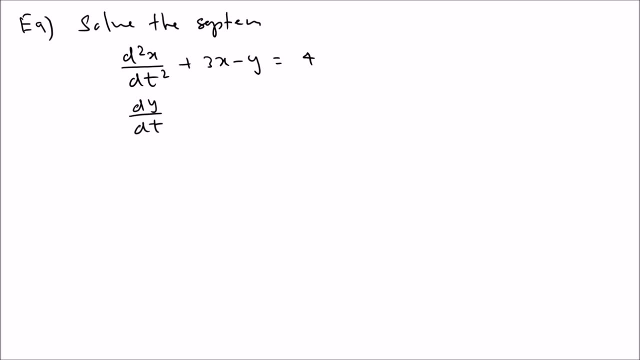 this is a interesting part. you can have anything here, not like before uh. so it is negative 4x plus 2y, some numbers, and then 3 e, negative t with uh. the one of the problem here. you need to give the initial conditions because you can solve. 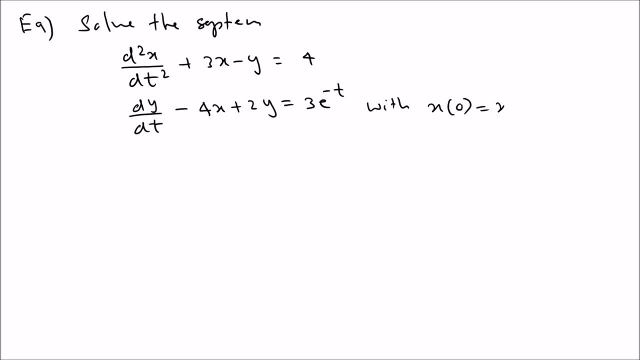 so let's say x 0, y, x 0, x prime 0 and y 0, all of them are 0, just to make a little bit easier, okay. so that's the problem now what we're going to do: take the plus, transform those two equations, okay, so answer. 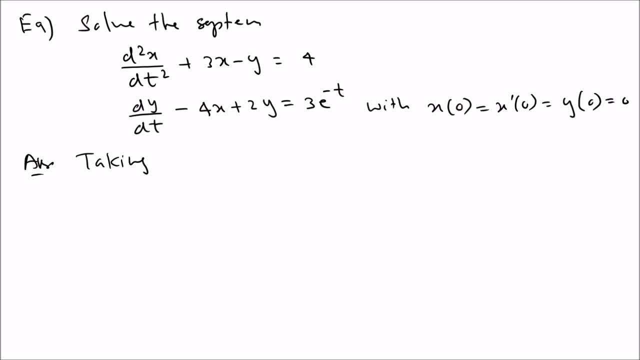 uh, taking laplace transform. taking laplace transform. uh, we're going to have in the first one we're going to have s squared, x s plus 3, x s minus y s, equal. what's the laplace transform: 4, 4 of s. so we'll get that equation and you can see that just x s there are. 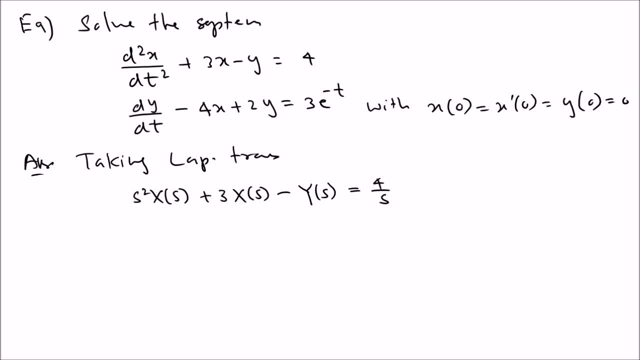 no derivatives, no other powers from the second one. you're going to get s, y s minus 4, x, s plus 2, y s equal 3. this is the it function, so it is s plus 1.. those are two equations that we get uh. so we can uh isolate the s x term as a factor. so, and then you can also: 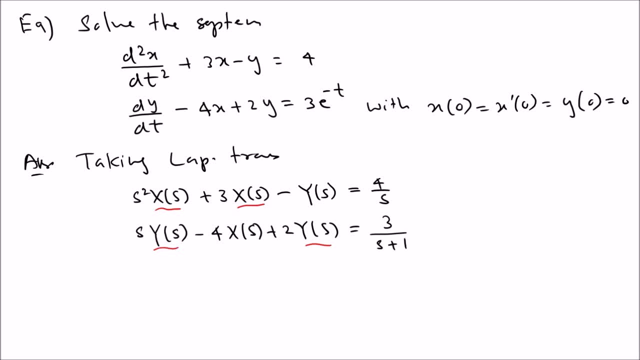 combine these two. so let's do that. so if you combine them, okay. so come on, let's say combining. let's say combining, uh, we have s squared plus three, s, x, minus y is equal uh, 4 over s, uh in the other one. you can see. 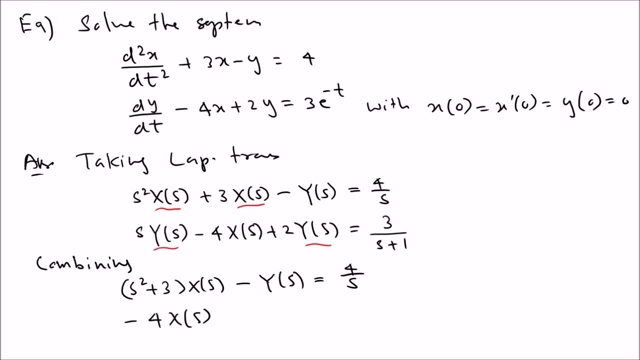 negative for sx it's: it's a good idea to write sx first and then yx next, so that you see the pattern. the other one, you're s plus 2, uh. yeah, let me make this a little closer to there. so it is plus uh, s plus 2, y s uh equal. 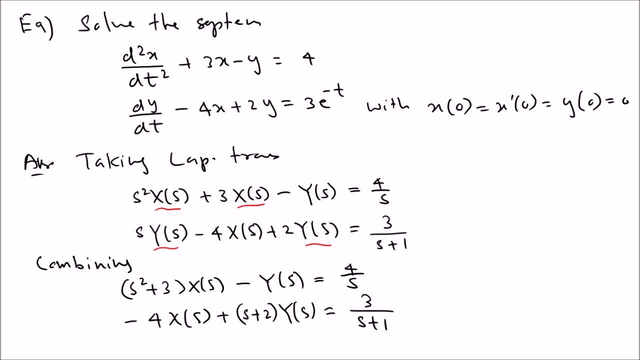 3 over s plus 1.. i'm going to call this equation 1 and call the equation 2.. now think of how to remove, how to eliminate one of the variables. so, for example, you can see, let's try to eliminate the ys. if you want to eliminate ys, you can. 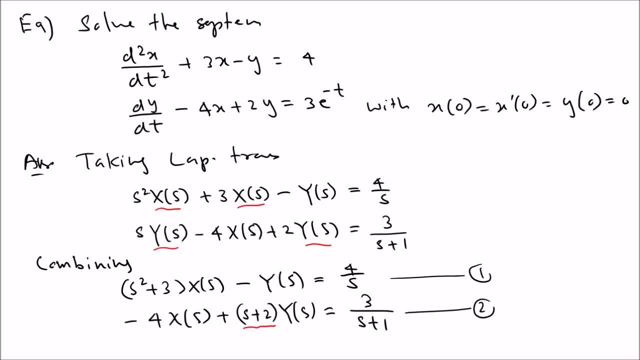 think of this term, because that's the coefficient. so what you can do, we're going to match the coefficient with the opposite sign. so, for example, if you multiply the first equation by s plus 2, the whole equation by s plus 2 and added to the second equation the ys term. 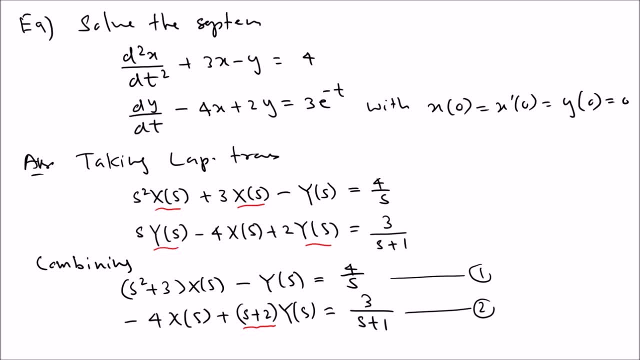 gets away. it's going to go away. okay, if you multiply the first equation by s plus 2 and add it to the second equation, the ys term going to go away. so you can solve for s x. so that's the whole point. so let's do it. 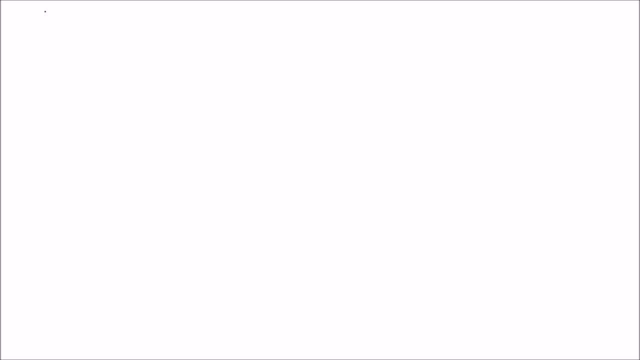 uh. so by uh we can do s plus 2 times equation 1 plus 2.. if you do that, you can see the y s term has the same coefficient. so when you add them, same and opposite coefficient. so when you add them they're going to cancel out. 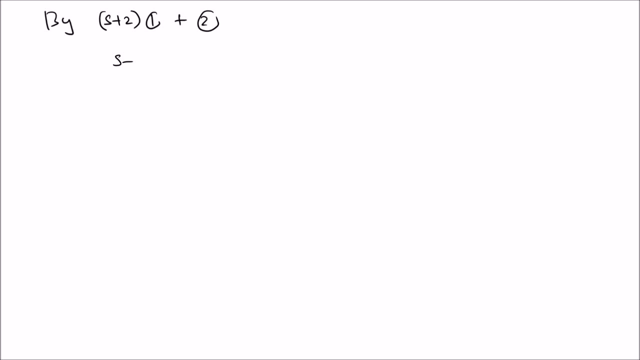 so you simply have s plus 2 times s squared plus 3 minus 4 from the bottom, one times s x. that's what you have. on the other side, you have uh four times s plus two over s, uh plus three times s plus one. that's what you get um. 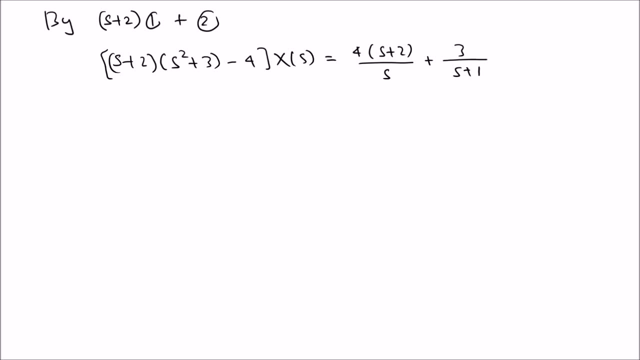 so, if you want, you can simplify this in to get one expression or leave as two. so it's uh how you want to do it. now you notice something. you can see that if you simplify, uh the what is in the bracket, you get s 3 plus 2 s squared plus. 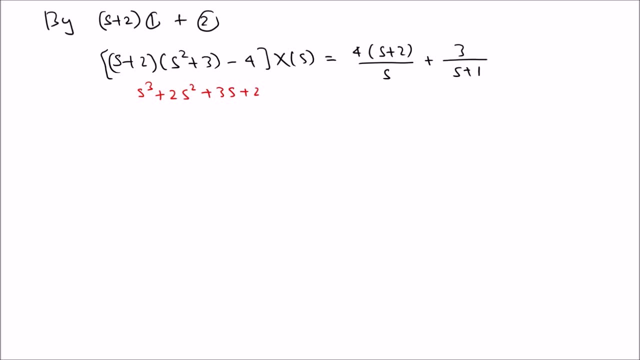 3, s plus 2, and then which has factors s plus 1 and s squared plus s plus 2, and if you don't know how to do this, i'll look at the other video about factoring polynomials so that explain, like how to find factors like this. 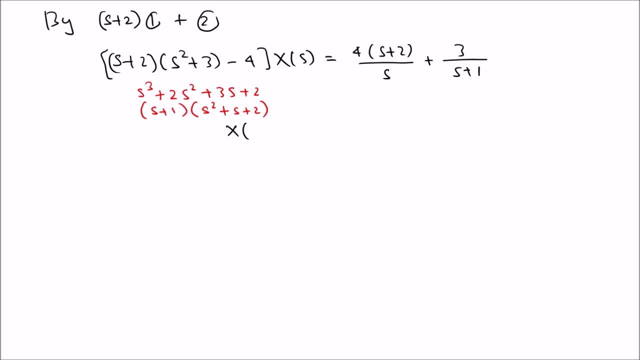 so now what we can do, we can divide both sides by that. so you're going to get s x, so let's divide both sides so we have um. i mean, if you had s plus 2 here, then you can cancel, but it doesn't happen like that, so we get four. uh, um. 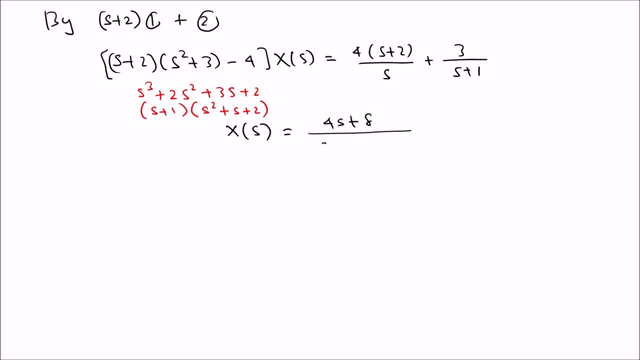 four s plus eight, divided by s plus one, uh s squared plus s plus two. and also we have a extra s in front and plus three. uh, what's gonna happen here? you have s plus one already, so it is s plus two, uh, squared. uh s squared plus s. 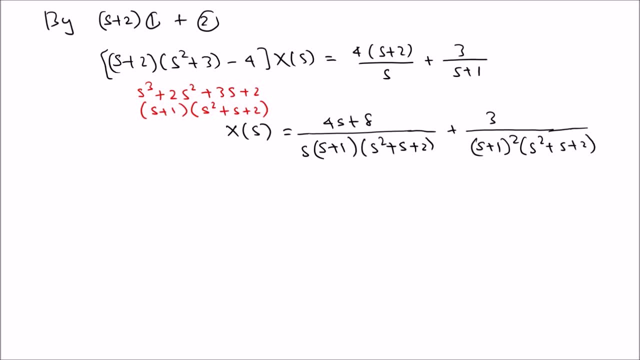 plus two. now what you're gonna do is just invert. so use the- uh, you know, try to find factors, uh, the partial fractions, and invert. so you can do either that way, or also you can use the convolution, uh, if you want to invest, or whatever the method that you use. what you're going to do is you're going to 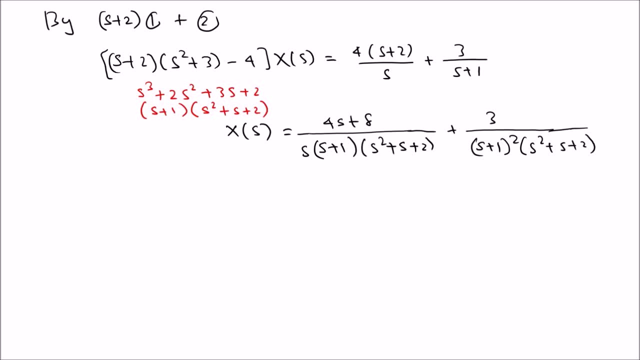 do. what you're going to do now is the inverting. but i will not do that. i will say: okay, so, uh, invert, uh to find xt, and then what you do, uh, you can plug in this xt in one of those equations and solve for ys. or do the same thing as before: try to eliminate. 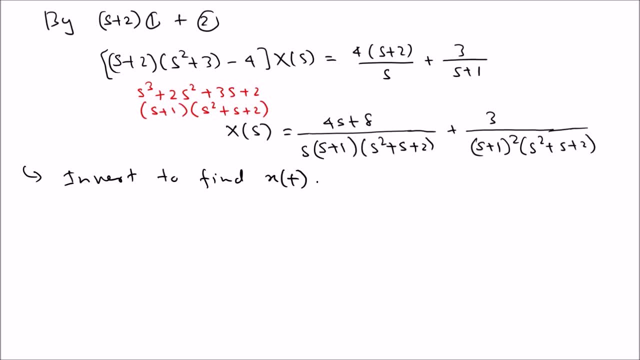 uh, the uh sx term, by just switching the variables and multiplying the opposite one and adding: so you can use one of those methods to solve for um, yx and xt, okay, and then you can say, uh, so you can do, and invert, okay, and then uh, the next one is uh. 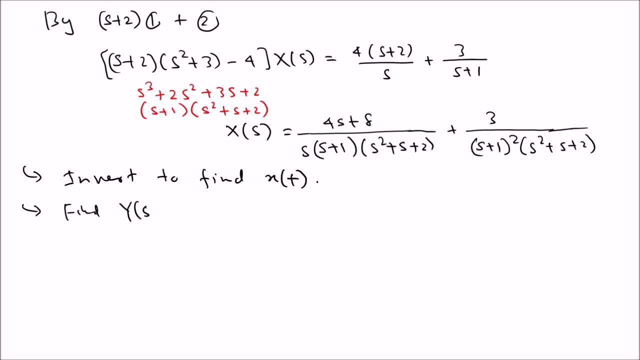 find uh, ys, similarly uh, to do that. to do that uh substitute, substitute xs, because we already know this sx, substitute xs, because you already know this sx. in in two and we can say: solve for ys and invert. it's just one way to do it. the other way is just do the uh. 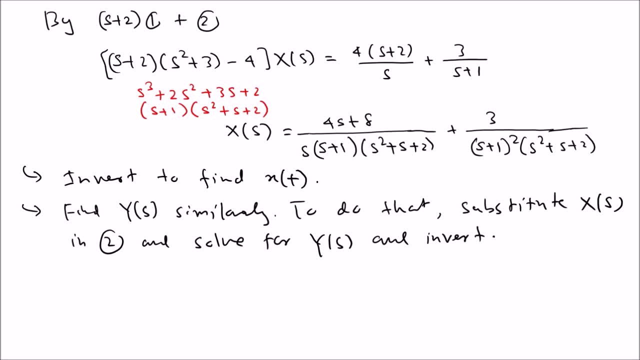 elimination as before and solve for ys. it's sometimes i mean depend on what we have- or or i use elimination to find ys. so you have two ways to do. either you substitute uh into the other one, because we already know uh, ys, we already know sx and solve for ys. 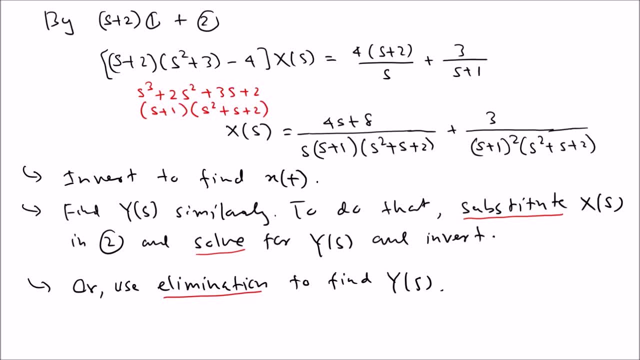 or just use the elimination to find ys. so you know it depends, okay. so that's how you uh finish the problems. i'm not gonna do it because it can take too much time, but this is the way to do it. uh, because this is very useful when you have, like a large system. 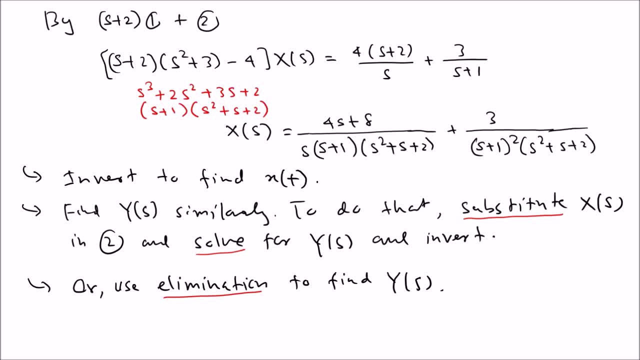 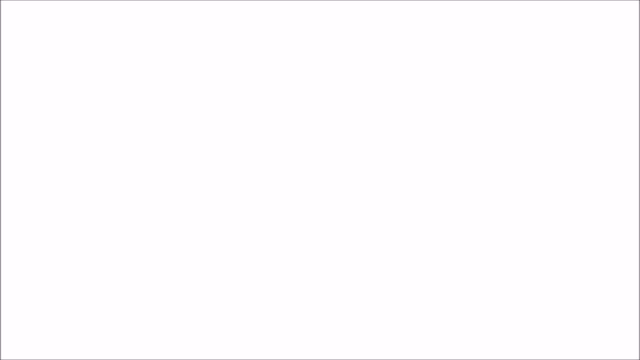 uh, so laplace transform method can help you to find the solution. so so we know the, the method, so let's move on to the, the last one, that is, the eigen vector method. so let's talk about that. so eigenvector method, eigenvector or you can say eigenvalue method. 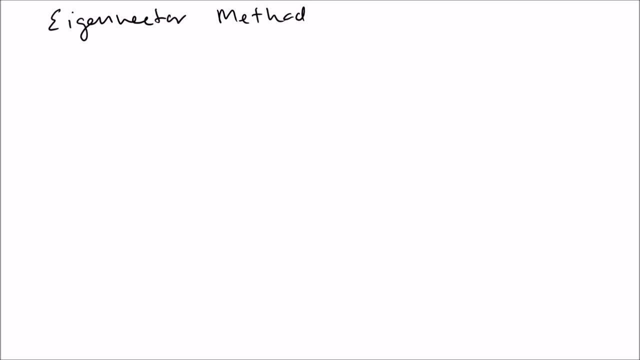 okay, eigenvector method. so let's talk about the, the steps, uh. so we're going to go with the first step, uh, what we're going to do, we're going to write the system, uh, using a matrix form. so write the system. write the system, uh, in. 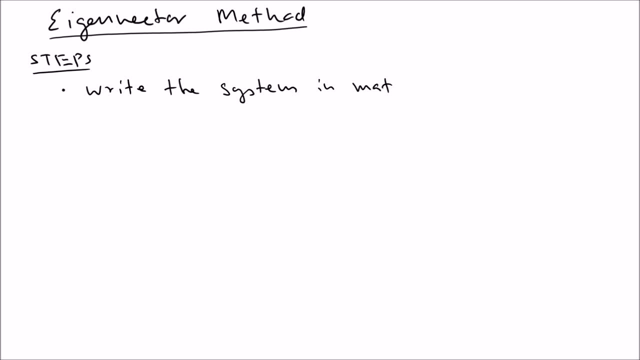 write the system in matrix form. that means x prime equal ax form. that's the first step. and then what we're going to do: find the eigenvalues. find eigenvalues, eigen values, lambda i of a. that's the second step. the third step is: uh, use any of the eigenvalues of. 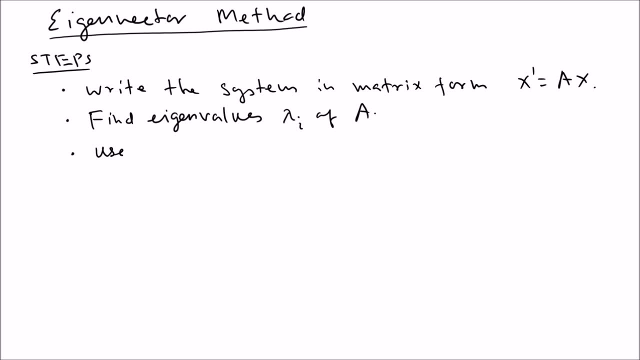 a any method, use any method. uh, so you can either use the shortcut that we discussed earlier- so there are several videos for that, for the two by two case and three by three case. so use the shortcut or shortcut, or or the regular method, the gauss elimination method. okay, the shortcut or the regular method. 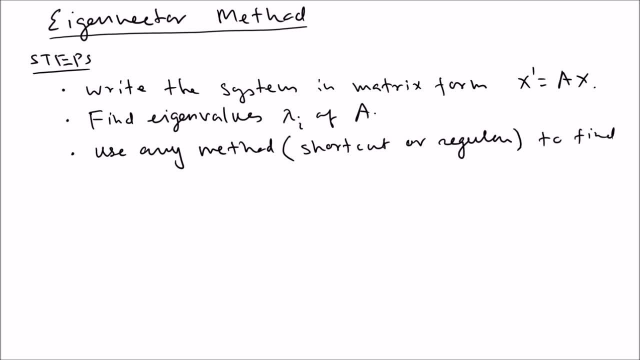 to find, to find the corresponding eigen vectors, corresponding eigenvectors. so you cannot do the shortcut or the regular. the shortcut is really short, okay, so ah, and then, uh, let's say vi, i can make this vs, but there's a lot of um short cuts, so the 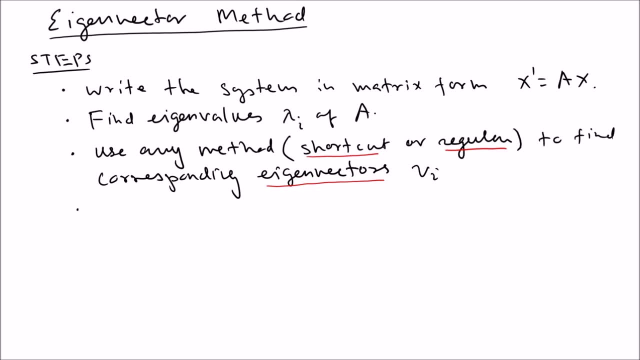 and then we write the solution. so write the um solution, uh, so we know that the solution is x, t, uh, which is given by c 1, the v 1, e, lambda 1, t, so the v 1 is the corresponding eigenvector of lambda 1, and then like, just like that, so we're. 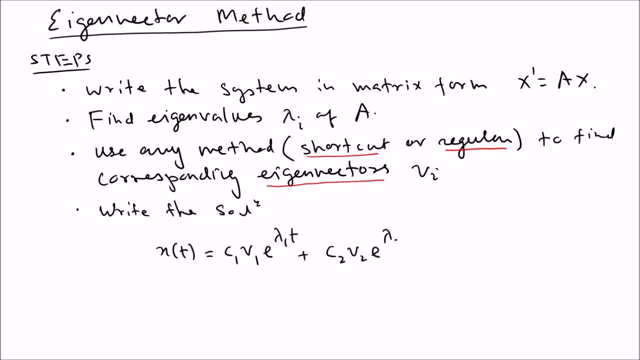 going to go v 2 e lambda 2 t, so like that. so there are n many. so you see n v n e lambda n t, also there are. so not ah. so lambda i's uh may be, uh, equal, may be equal, ah. but the v i's v 1, v 2, v n. 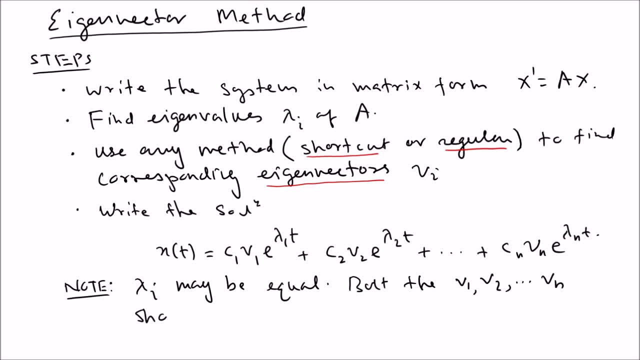 should be, should be linearly independent. linearly so. that's the only requirement we need. those eigenvectors has to be linearly independent. but there's a function um this we discussed earlier. uh, the eigenvectors of different eigen values are linearly independent, always so eigenvectors. 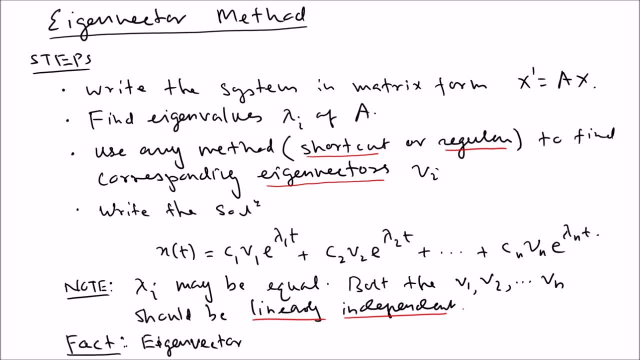 eigenvectors of different eigenvalues are linearly independent. that you can show that's the case. they are linearly independent. but sometimes what happens? even if you have some repeated eigen values, you can show that those vectors are linearly independent. in that case, uh, you can still write the solution in this. 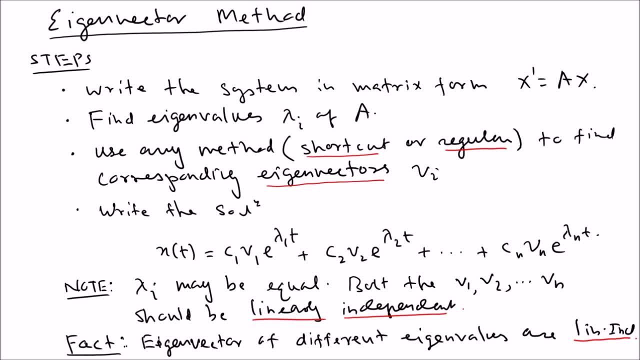 way. okay, so we can use this form for two cases: the distinct eigenvalues or repeated eigenvalues, but with linearly independent eigenvectors. okay, so those are the two cases: one with distinct eigenvalues or one with some equal eigenvalues, repeat eigenvalues, but with linearly independent eigenvectors. 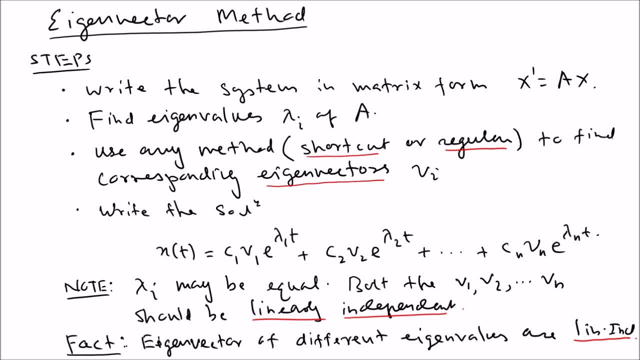 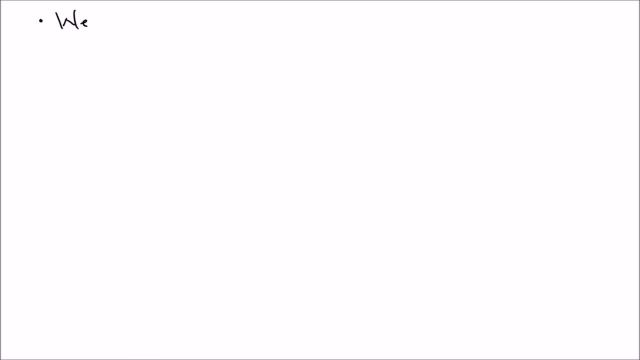 so, if you want, we can like kind of repeat that because that's a kind of important step. so we use this form. we use this form of the solution when for a distinct eigenvalues, for distinct eigenvalues or some repeated eigenvalues. so we use this form. 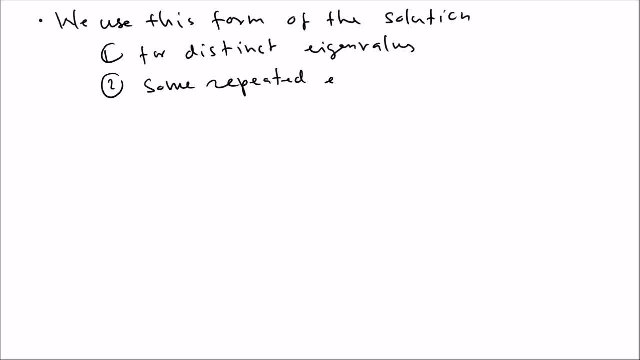 eigenvalues, some repeated eigenvalues with linearly independent. with linearly independent eigenvectors, v1, v2 through vn. so for those two cases we can use this form of the solution. so some repeated eigenvalues with linearly- this important one- in independent eigenvectors. 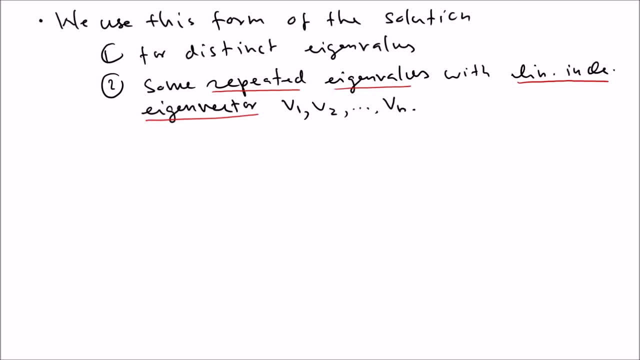 okay. so let's try to do, uh, two examples, one from two by two and another from, uh, uh, three by three. so let's start with the two by two. one so uh. so example one. so let's say, use eigenvector method. we can vector method, use eigenvector method to solve. 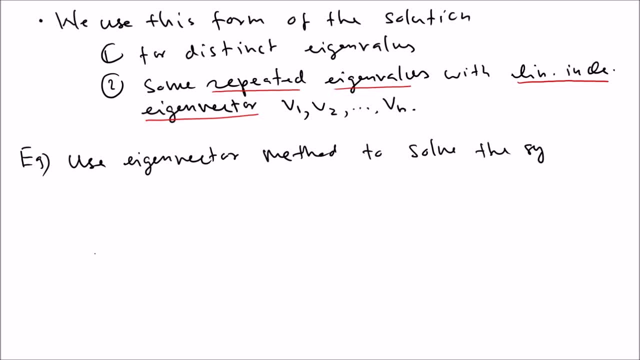 we can vector method, use eigenvector method to solve the system. so the system: let's say we have x prime equal three x plus four, three x plus, let's say three x plus y, and then y prime equal to x plus 4 y. so that's the system. um, so we see that x prime equals equal 2 x plus y, 2 y. 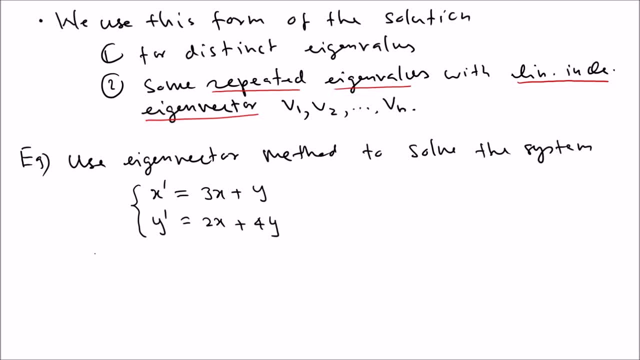 plus 4 y. so this is the system um. so we see that as type 2 elimination method, you can take the derivative and plug in from the other one. you can do that and then eliminate one of the variable. um. let's see how to use the eigenvector method. 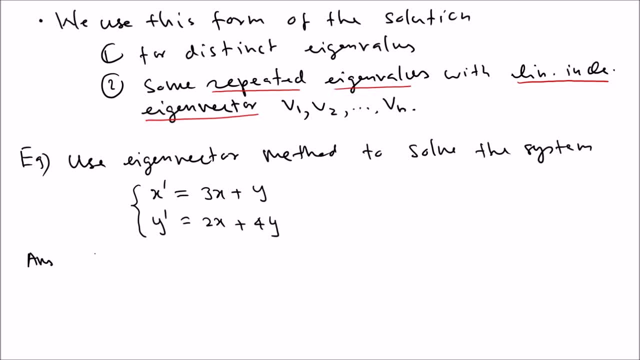 also the answer. so we're going to let x, which is the vector of x and y. those are the solutions. uh, then we know that x plus x prime is simply x prime, y prime. so we can write the system in this form. so, uh, so write the system in matrix form. so the next one is: 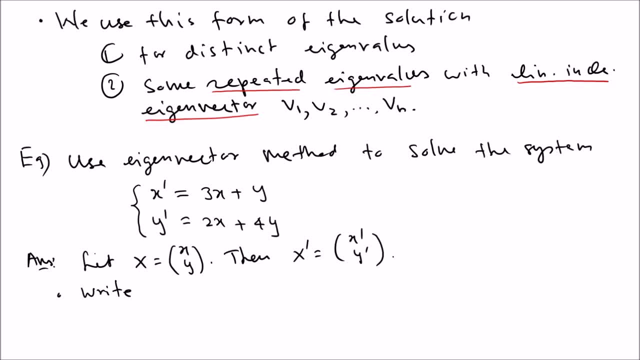 right. so i'm gonna write these steps, but you don't want to do that. i mean, it's just guiding you, but in the exam you don't write those things, so write the system. i mean you can to make it like more logical. so write the system in matrix. 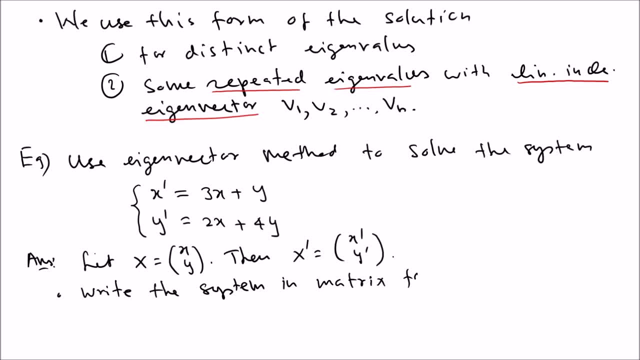 form. so we have x, prime, uh, the coefficients three, one, two, four. so those are the coefficients times x. so we just put the coefficient and put x there. now what we do? we're going to find the eigenvalues. okay, so we're gonna uh. so this is a 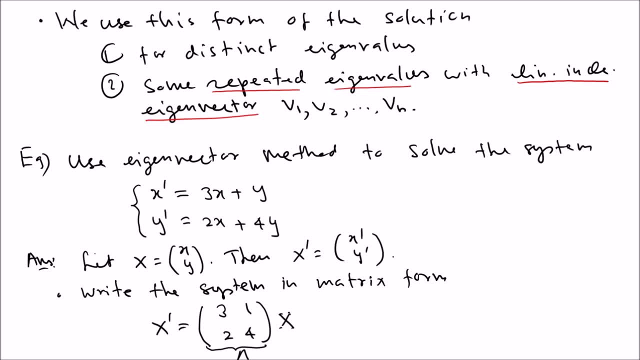 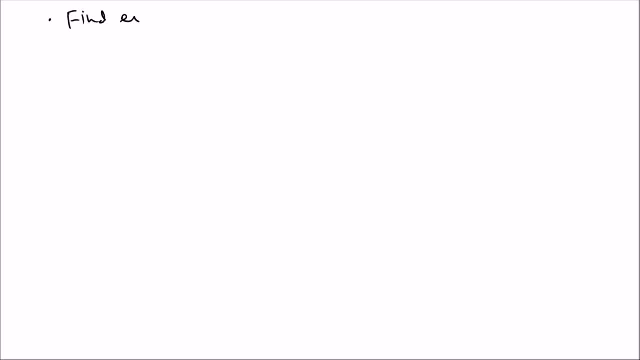 so i'm gonna call this is a. so we're gonna find the eigen values of. next step, find a eigenvalues of a. uh, for that we can look at the determinant of a minus lambda i. so that is the. i subtract the lambda from the diagonal entry, so it is three minus lambda. 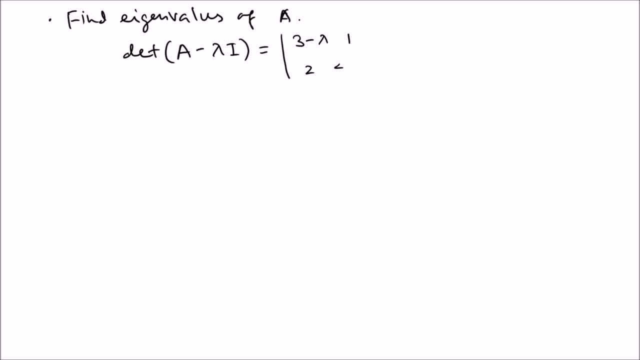 one, two, uh, four minus lambda. so this is simple. so this is a two by two. so we're going to multiply that, so we're going to multiply that, so by two. so that's you can multiply the diagonal first. so multiply the diagonal and subtract the other diagonal. so minus other diagonal means 2 you set. 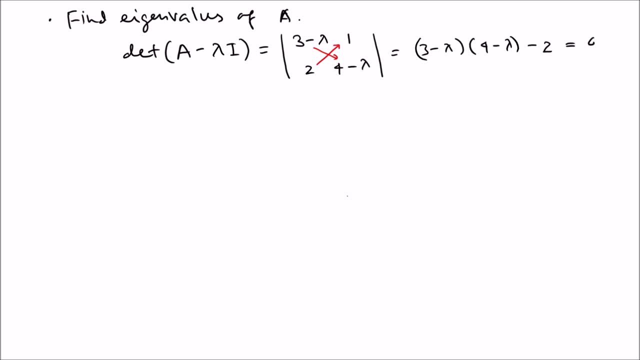 this equal to 0 and you can see that this simplifies to: lambda squared minus 7. lambda plus 10 equals 0. this has factors: lambda minus 2 and lambda minus 5 equals 0. this implies that lambda equal to n phi. so those are the eigenvalues. 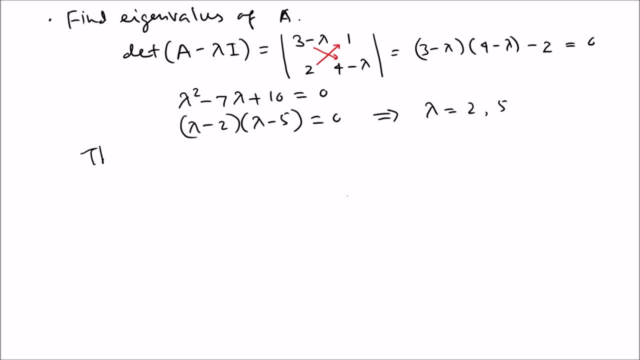 okay, so the eigenvalues are lambda, equal to n, phi. now what we can do, we're going to find the corresponding eigenvectors. so find eigenvectors, find eigenvectors. for that we can use a shortcut method. that means: uh, eigenvectors are simply the columns of the 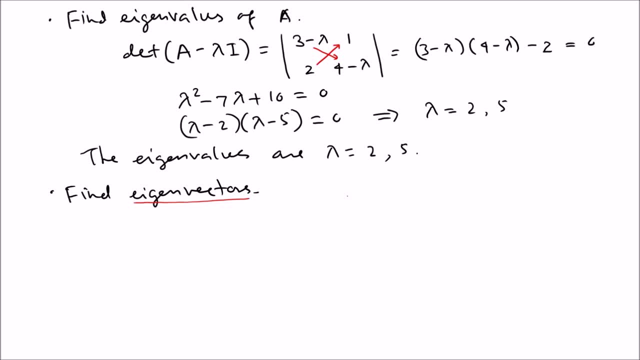 uh, complementary eigen matrix, the other eigen matrix. so remember, the eigenvectors are the columns of non-zero, columns of the other eigen matrix. so we're going to do that. so for lambda equal to lambda, we're going to calculate the kappa matrix of phi, because that's the other eigenvalue. so that means you subtract. 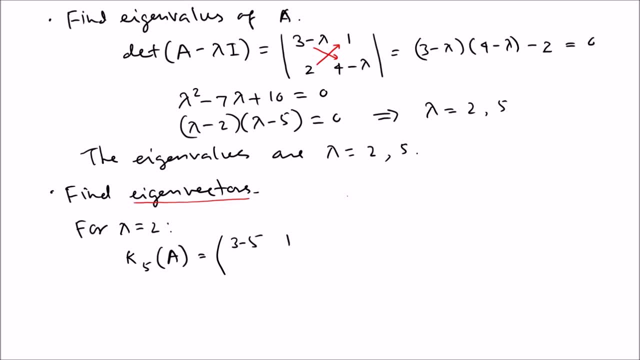 5 from the diagonal: 3 minus 5, 1, 2, 4 minus 5. so you're going to get the columns as negative: 2, 2, 1 negative 1. these are the eigenvectors, and you see that they are just a multiple of each other. so that's the eigenvector. so that means: 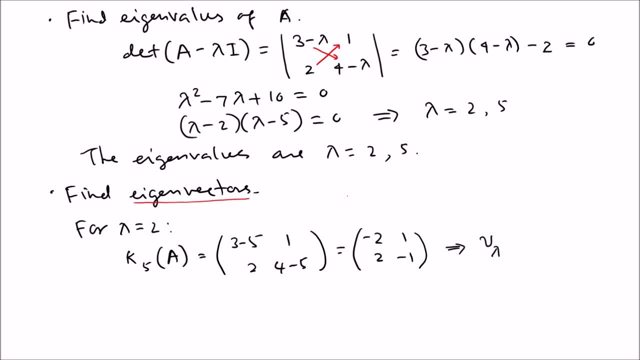 this implies that eigenvectors are just a multiple of each other, so that's the eigenvector. so that means this implies that eigenvector for lambda equal to- uh, the column. just pick any column or any multiple, so one negative one, that's eigenvector. okay, so you simply pick one of them, or 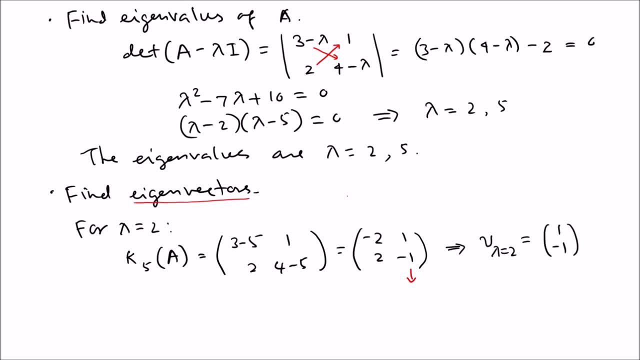 even a scale version of that. so i pick that one, or you can pick the other one, or you can even multiply by something. uh, now what we're gonna do? uh, we can do the same thing with the other eigenvalue. so, for, lambda equals 5. now we're going to calculate the other. 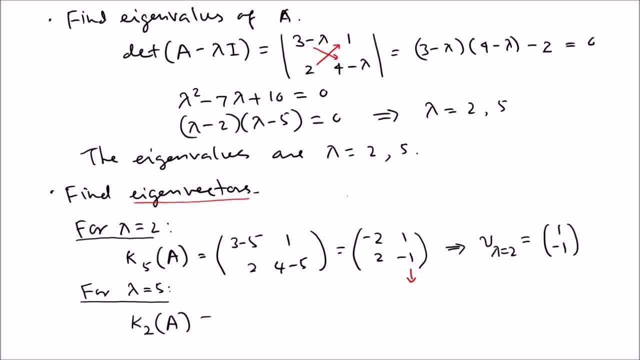 one. so it's going to be 2 here now. so if you use 2 subtract 2, so it is 3 minus 2 and 2, 1, 4 minus 2. so you're going to get 1, 2, 1, 2. so you can see they are the same and 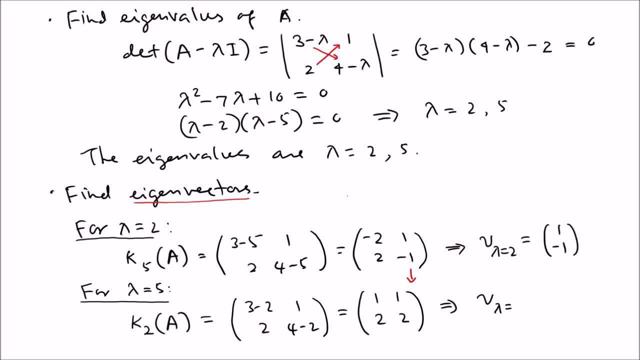 that's the eigenvector 4 lambda 5, so which is: uh. that's eigenvector 4 lambda equals 5: 5, so which is 1, 2. so we find the eigenvectors. now what we can do, uh, just, uh, just use the formula. okay, so very simple. 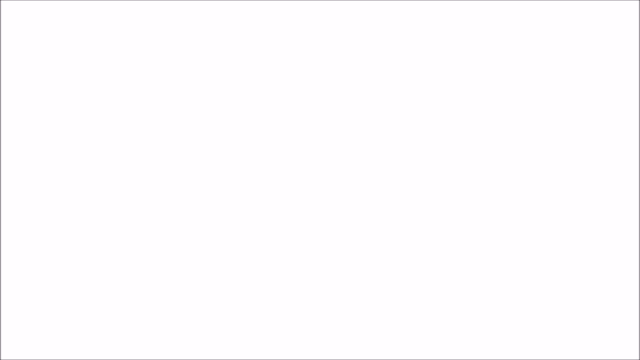 so the formula. so now write the solution. so you can write the solution. so which is x t equals c 1 v e lambda 1 t plus c 2 V e lambda 2 t. so that means c 1 eigenvector of 2 is 1 negative 1, so e 2 t plus c 2 eigenvector of. 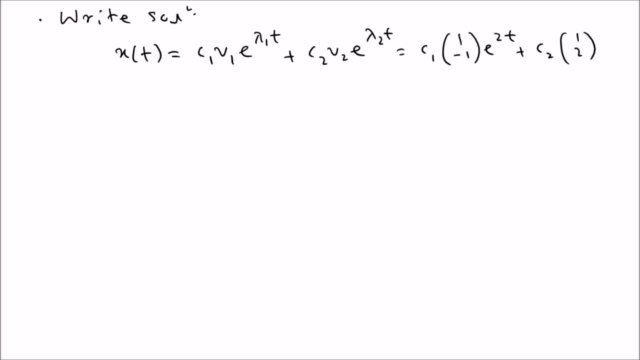 5 is 1, 2, so it is e to the 5 t. so that's the solution. also, um, you can simplify if you want, but that's not necessary. uh, i'm just gonna write it. you know, you may simplify, but that's not necessary. so let's say, uh, how to simplify this one? then you can. 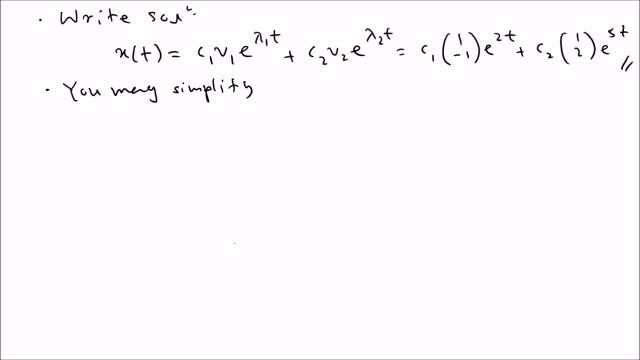 write x, t, so what? we're going to be going to distribute this. so that means you can first say, uh, c 1, negative c 1 times e to the 2 t, and if you multiply by c 2 it is c 2, 2, c 2, a to the 5 t. now we're going to multiply. 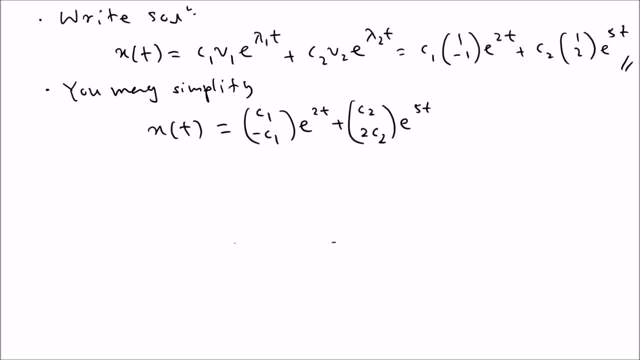 inside and add. so that means if you multiply inside and add we're going to get a negative c 1 times e to the 2 t. so you can add: you're going to get c 1 e to the 2 t from the first one, from the. 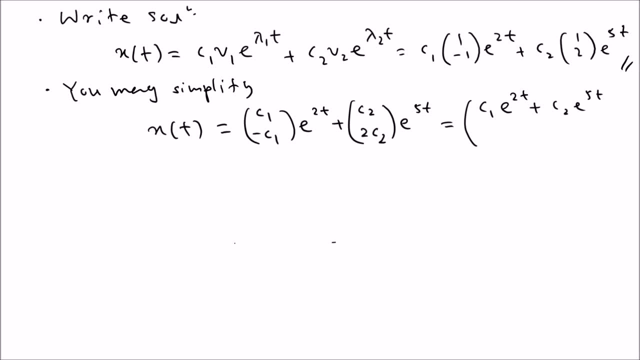 second one: it is c 2 e to the 5 t, and here also it is negative c 1 e to the 2 t plus 2 c 2 e to the 5 t. that means those are the two solutions, so uh. so therefore you can say: uh, the x solution. that's the first. 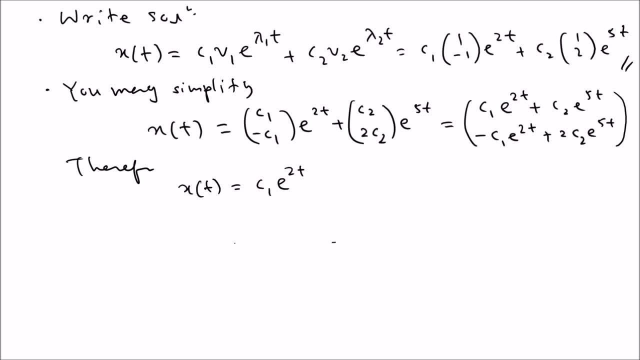 component, which is c 1 e to the 2 t, plus the plus c 2 e to the 5 t and the y t. that's the second component with us how we define the x- uh. so actually this is not simple x, this is uh. 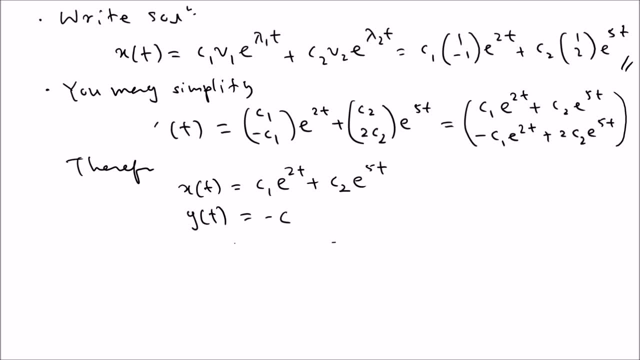 this is the vector x. so this is the big vector uh as a vector solution, yeah, even here. so that's the uh vector solution. okay, so it is uh. and then we have uh c 1 e to the 2 t plus 2 c 2 e to the. 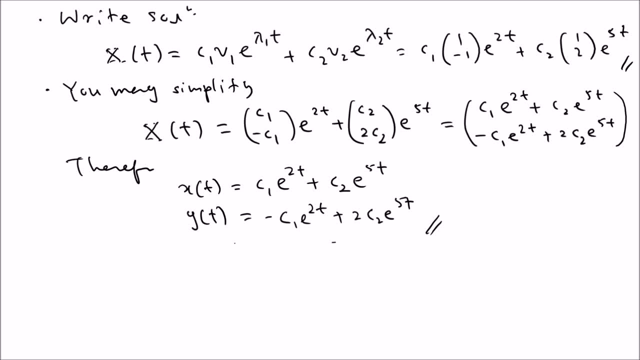 5 t. so that's the solution. so you can write it like that, or you can just leave the first version. that's fine. good, so that's the service holder. a system of two by two. now let's try to do uh one from uh three by three. so let's solve this one, for example. 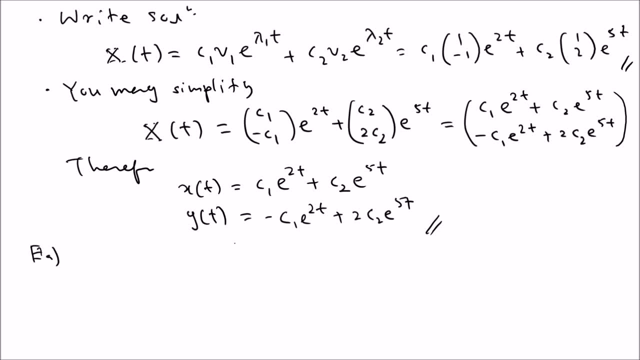 uh, yeah, actually, uh, to be better, we're gonna put everything in one side, okay. and then one more thing: uh, if this is just a, not uh, if initial conditions- if initial conditions are given- are given, uh, we can find, we can find c 1 and initial conditions, just plug in them here and solve for c1 and c2, so it's a. 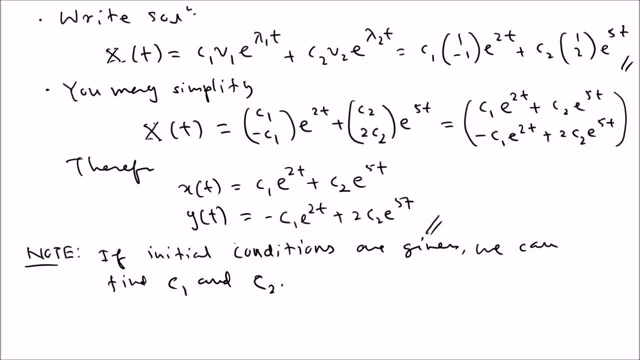 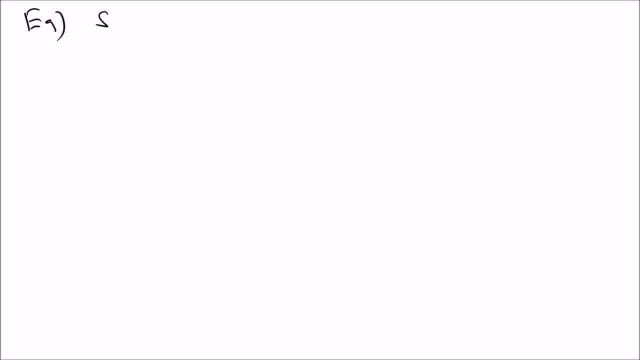 simple, uh simple task, okay, so let's do the three by three now. uh, so the three by three, let's do, uh, just one example, just to remember, uh recall what we did. but there are like a three uh four examples solved in the main lecture so you can look at anything in more examples. 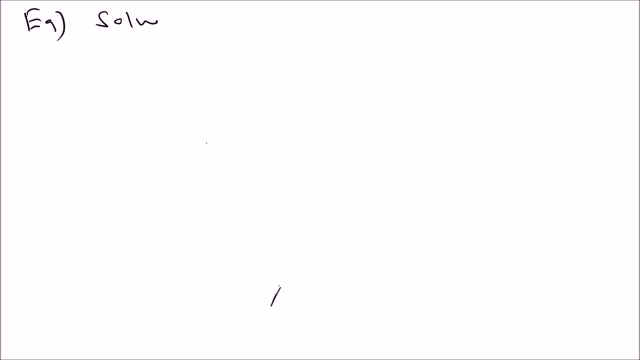 so let's say solve. there are three, uh, solve the system system of ods r. sorry is dx over dt equal 3x minus y minus z, dy over dt, which is x minus y minus z plus y minus z. dz over dt, which is x minus y. 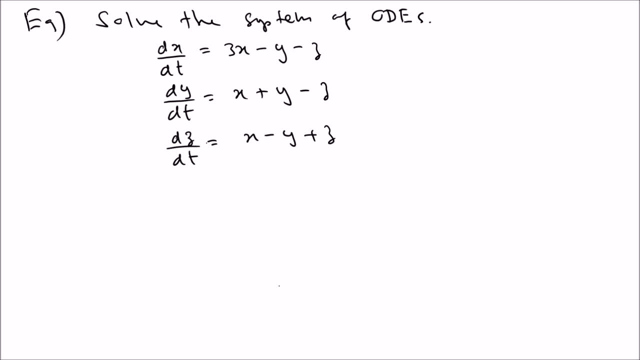 plus c. so what we can do, we can write the system in the matrix form. that's the first step. so the answer: if it is not in the matrix form, write in a matrix form. so, uh, so we're going to define the x vector, which has three components: x, y and z. 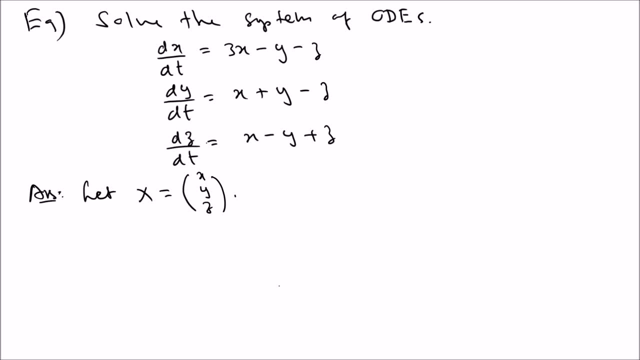 so, uh, now what we're going to write in the system in matrix form. matrix form: okay, writing system in matrix form. so we have x, prime equal, the coefficients: 3 negative, 1 negative, 1, 1 1 negative, 1, 1 negative, 1, 1. 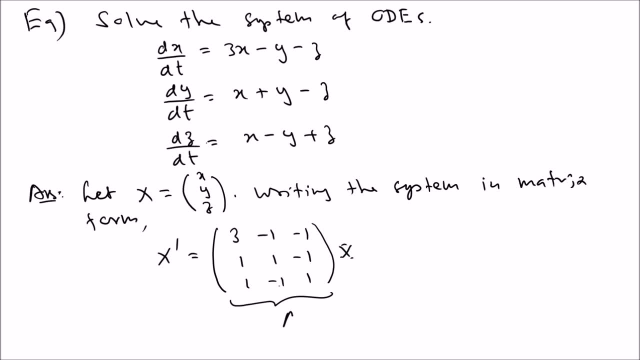 times x. that's the system, matrix a. now what we're going to? we're going to find the eigenvalues first. okay, so find the eigenvalues, find eigenvalues. so the zero equal the determinant of a minus lambda i. uh, so that means you subtract the lambda. 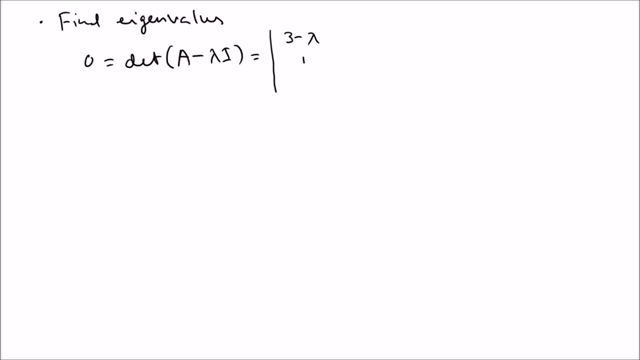 from the diagonal entry. so 3 minus lambda, 1, 1, 1 negative, 1, 1 minus lambda, negative 1 and then a negative, 1 negative, 1, 1 minus lambda. so that's what you get, so you can use the laplace expansion. 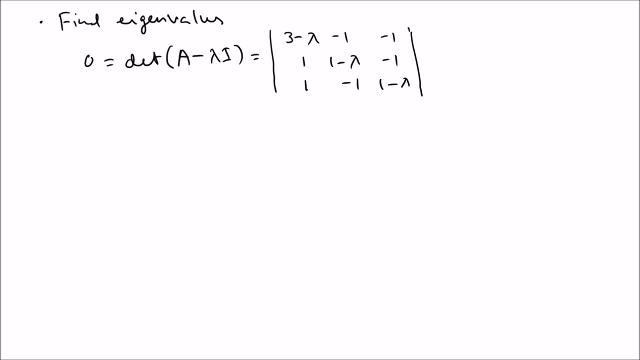 uh or the cofactor expansion to find the get the equation. but sometimes it may be a good idea to use the determinant properties to simplify this first. like you know, try to get like more zeros. you can see they are one one. they are equal. so if you subtract them they are. 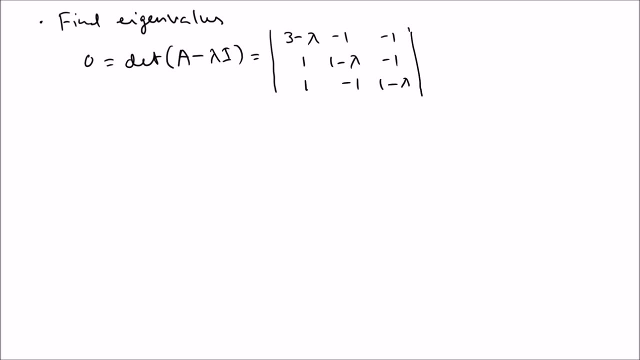 negative one of the other row, you get a zero. so it's always a good idea to get extra zeros. then it's the calculation gonna be easier, so we can do that. so the first thing are we gonna do is: uh, we notice that there's a zero here, there's a. i mean, they are equal. 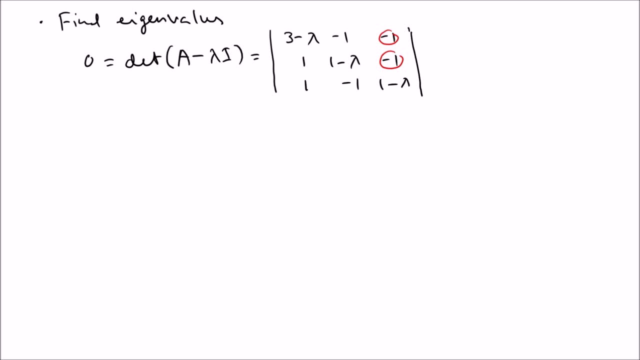 so we're gonna get a zero, uh, so we're gonna subtract. so what we're gonna do is i'm gonna uh subscribe, i'm gonna add the negative uh, uh one of row two to row one, so let's do that. so, if you do that, so let's do that. 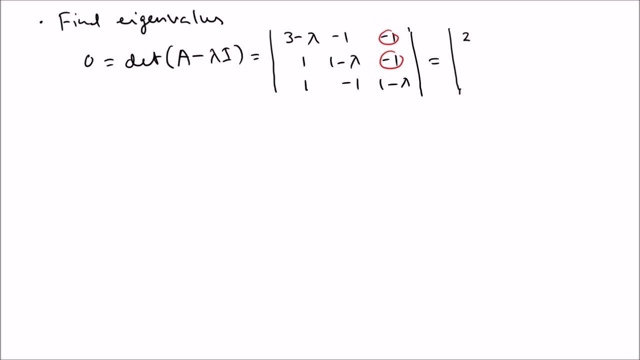 so that means you subtract rho 2 from rho 1, so you get 2 minus lambda and you get lambda minus 2, so they are equal. just opposite sign and this is 0.. so that means you can take the lambda minus 2 as. 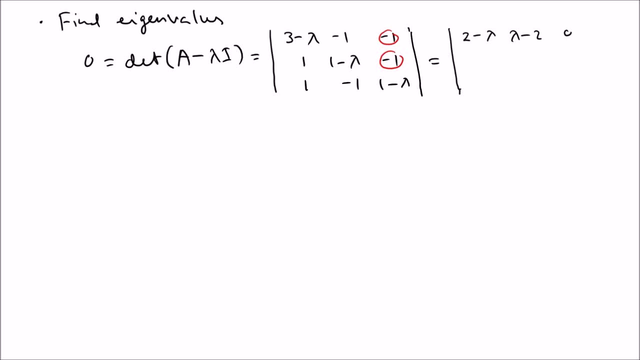 a factor. so that's a good thing. and then here we have 1, and then 1 minus lambda, negative 1: 1 negative 1, 1 minus lambda. so how we did what we did, we want r 1 minus r 2.. now what we can do is we can pull the lambda minus 2 out as a factor. 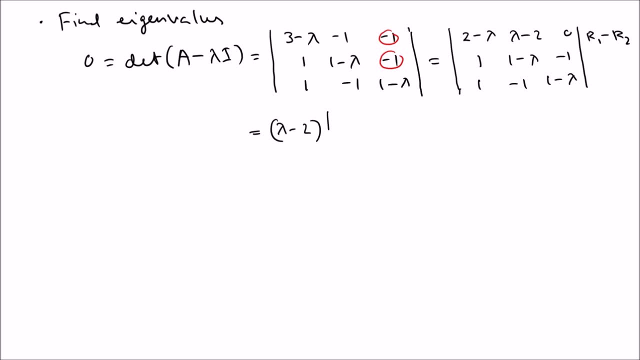 so if you do that, it is lambda minus 2 as a factor from the first row. so you get minus 1 and 1, 1, 1, 1 minus lambda minus 1. so we have a 0 here minus 1, 1 minus lambda. now what we can do is you can add: 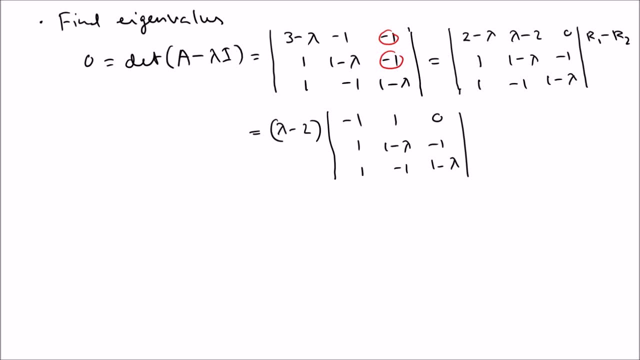 uh, row one or column one to column two to get another zero. so let's do that. so we're gonna do that, so we're gonna get one more zero. uh, by doing so, i mean you don't have to do that, but this is gonna make the. 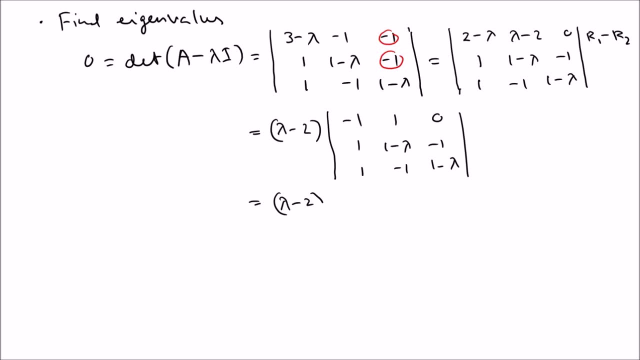 calculation much easier because it's easy to find the factor. so what we're gonna do, are we gonna add: uh, column one to column two, so it is negative one, one one, you get another zero and one minus lambda. uh no, it's two minus lambda. before you add, 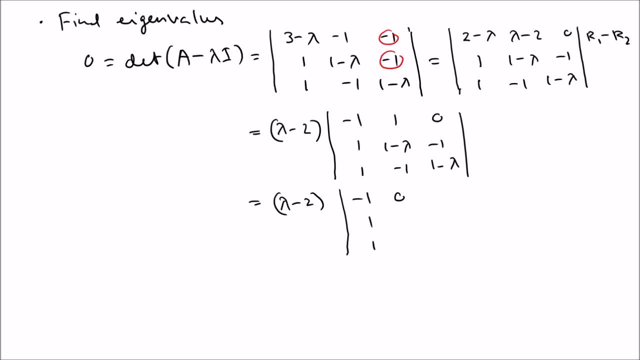 them. so this is gonna be zero, two minus lambda. you add column one to column two, so this becomes two minus lambda. this is zero. and then, uh, zero minus one, one minus lambda. so what we did? uh, we add, uh uh, column one to column two. good, now we can write the expansion. so once you write the expansion, you're. 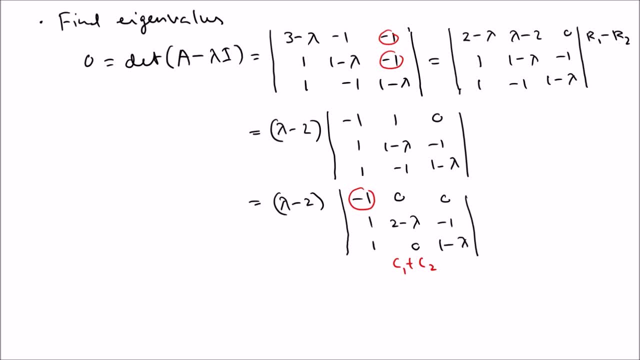 gonna expand uh at this point and you can see you only have one uh term you get. so that means if you write the expansion now, you're gonna get uh. it's a negative because negative one times lambda minus two, the two by two determinant, which is two minus zero minus one, there's a zero here. 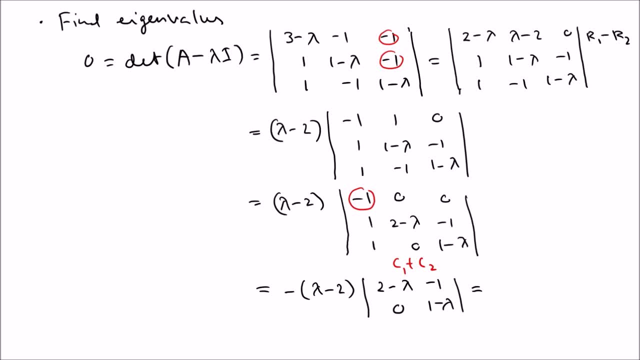 one minus lambda. so that means you already get the factored version negative: lambda minus two. two minus lambda, one minus lambda. okay, so this is simply: uh, if you switch a term, this is lambda minus two squared. one minus lambda. two minus lambda. one minus lambda. two minus lambda, one minus lambda. 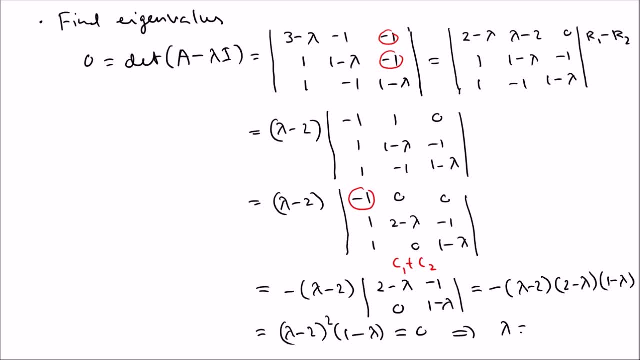 twoanda definitely means you. no mention that last term. and only thing is lacking is i in basic right, drop out. uh, so this sy 된, remember the right expression is: one we can draw out, so two we can draw that down here. two we can draw backwards. 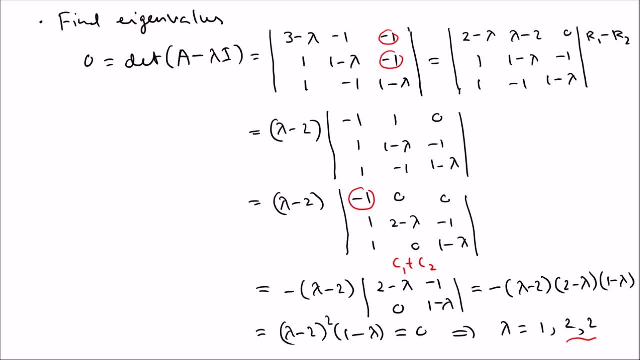 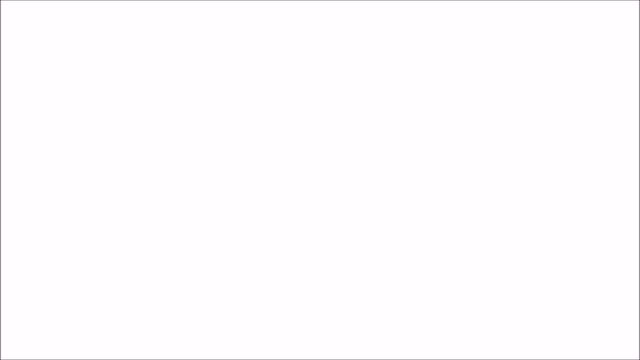 so alpha plus one, two times one. so let's say that one is always two. maybe now that's going to be two and i'm going to startiser, all right, so it's matrices. uh, so the? uh find the eigenvectors, find eigenvectors. so what we do? uh, since there are only two eigenvalues, 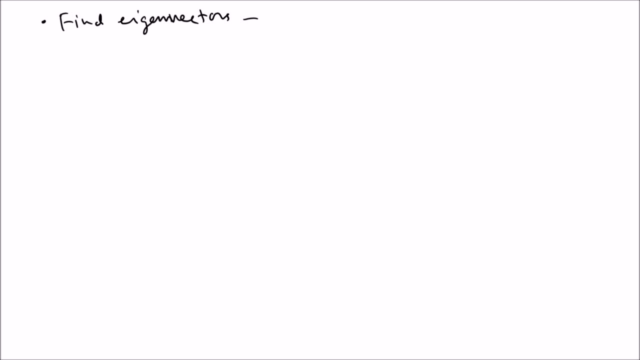 we're gonna, uh, uh, use uh eigen matrices so we can use eigen matrices for that, uh, so what you're gonna get is: so we're gonna, um, do the eigen matrix product so it's a one eigenvalue is one of a times the other, uh, so we just get the two. 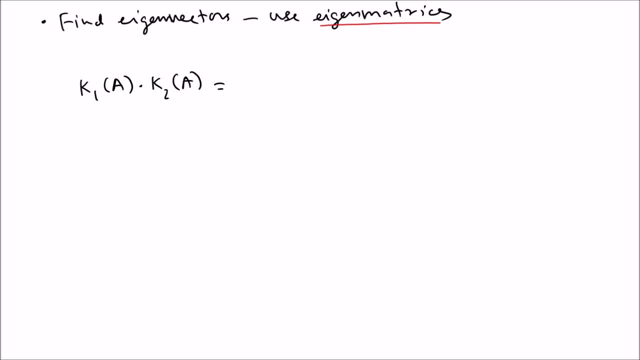 kappa matrices and we're gonna multiply them. so let's do that, uh, so the what is the first eigenvalue? uh is one, so we're gonna subtract one from the uh diagonal, so you're gonna get two. uh, one, one and then negative one. you subtract one, so you get zero. 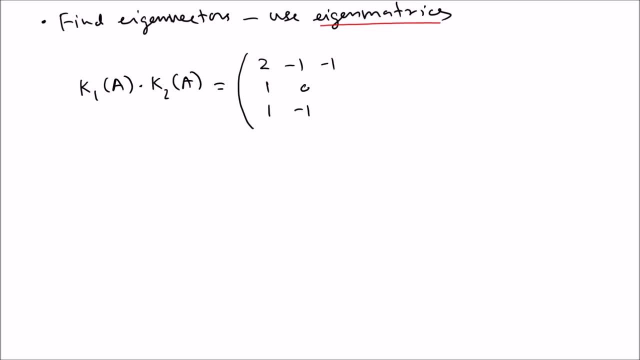 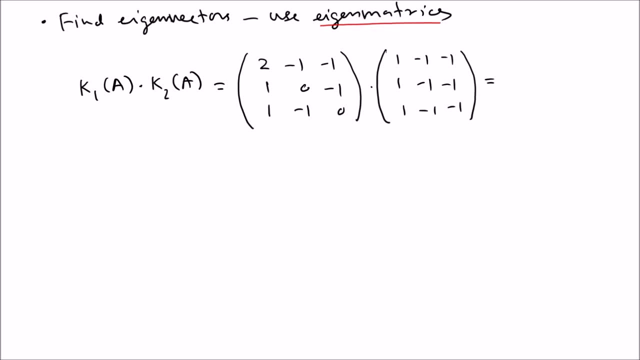 get. if you get zero, you're lucky. the columns are eigenvectors, so you can see that, for example, if you multiply this row with this column, you're going to get zero. uh, the two minus one minus one, so zero, and you can see that everything is zero. 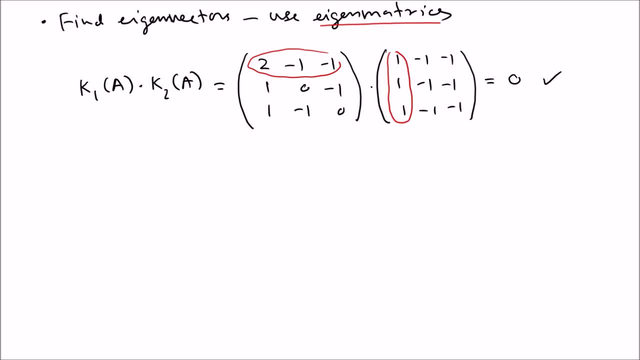 okay, very good, that means the columns are the eigenvectors of the other eigenvalue. okay, so that means: uh, so these are these columns. there are three columns here. these columns are the eigen vectors of lambda equal two and these are the eigenvectors of lambda equal one. so it's always: the columns are the. 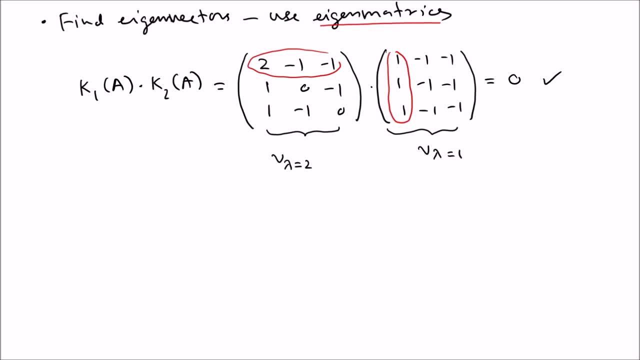 eigenvectors, opposite one. that's a list of eigenvectors. uh, so the eigenvectors are eigenvectors, are for v, lambda one. you can see they are all the same. so it is one, one, one or just multiple of that. so you can see. that's exactly. you see that there, and for a lambda. 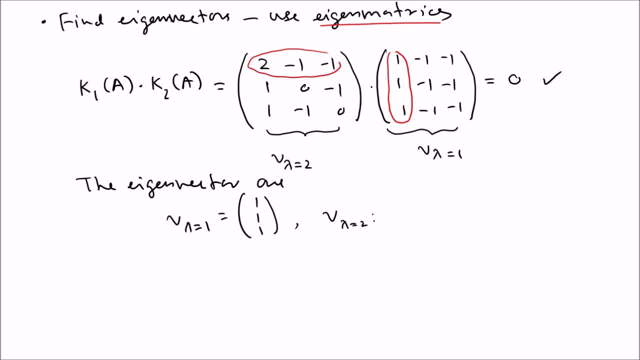 equal two. uh, we need two eigenvectors. uh, just pick any column you like. so any column, or even any linear combination or rescaling, for example, i can divide the second column by negative one, so you get one zero one. uh, and then uh, if you divide the. 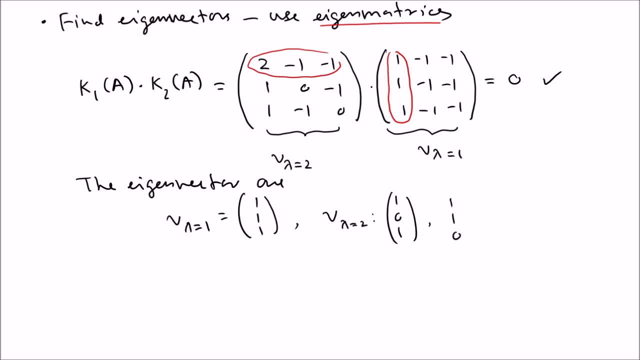 second, third column: by negative one, you get one, one, zero. also there are more things. for example, if you add the column one to column two, uh, you're gonna get one one, so that's another one, uh. so you can do a lot of other things, so you can just add them, you can multiply. 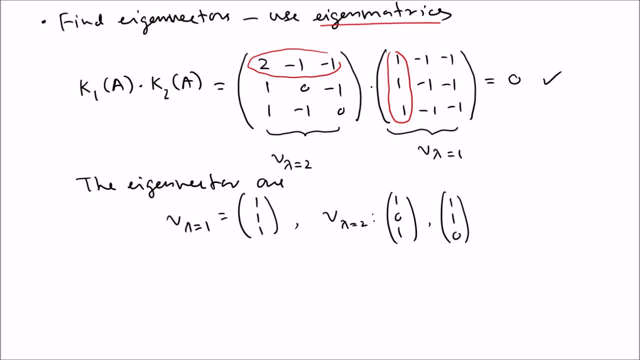 by one something and add them. okay, just any column operation, so, but we need only three. so and then you can also see that those three are linearly independent. okay, so they are linearly independent just by observation, because where the zero is, but when you have a zero like that, it has to be linearly. 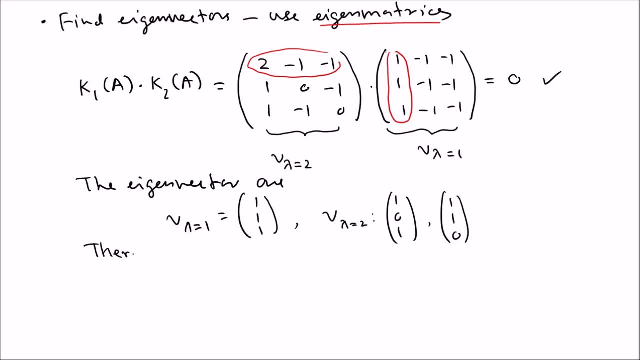 independent. okay, so they are linearly uh independent. okay, this is the early independent. you can have the solution uh. so the solution uh vector x, t, which is simply c, 1 v, 1 e, lambda 1 t, c, 2 v, 2 e, lambda 2 t, c, 3 v. 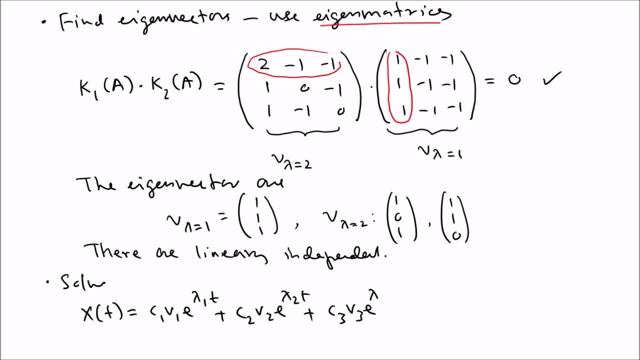 3 e, lambda 3 t. so if you substitute, you're gonna get c 1 times. the first parameter is going to be the solution 1, 1, 1 e to the lambda. what's? the lambda value is 1, so it's t, and the second one is c 2 times 1, 0, 1. 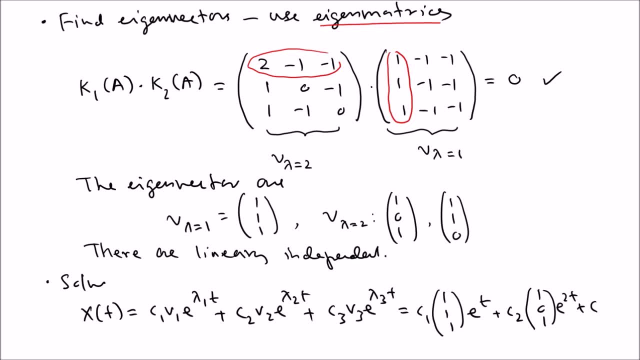 the lambda value is 2 t. the third one is c 3 uh. the eigenvector is 1 1, 0 e to the 2 t. so that is the solution of the system as before. we can, if you want, you can, just multiply it. 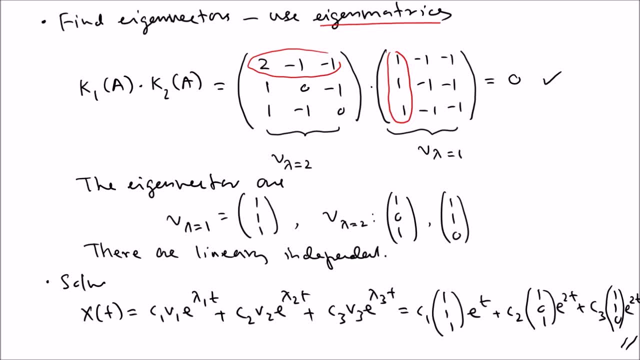 through and add them and then get three equations. but that's not necessary, but this is the solution, okay? um, so this is the solution, okay. so, uh, yeah, c1, c2 and c3 are constants. so you can see, it's not that difficult. very simple, but this is for. 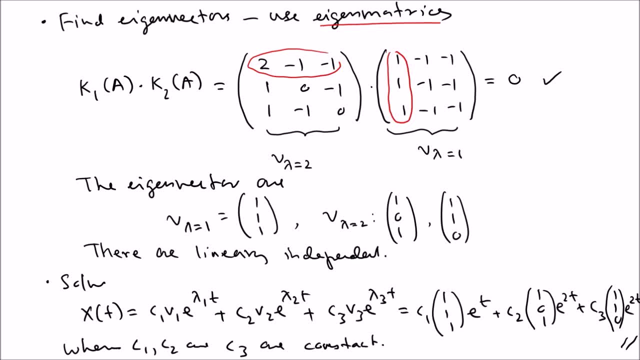 uh, two eigenvalues. if there are three eigenvalues, what we normally do is we're gonna pick. uh like, if you need the eigenvector for lambda one, what we can do, we're gonna pick the other two eigen matrices and just multiply them. just multiply them. but we only need one column multiplied by the 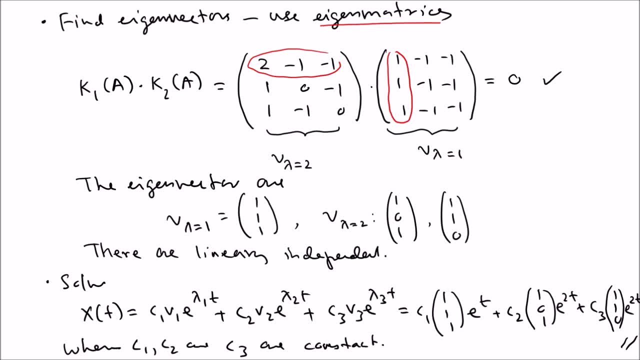 other matrix. so it's very easy. you can get the answer really fast. you only pick one column, normally with many zeros, so we can multiply that with the other eigen matrix so you get eigenvector. just keep doing it for other ones, so you pick the other two matrices.